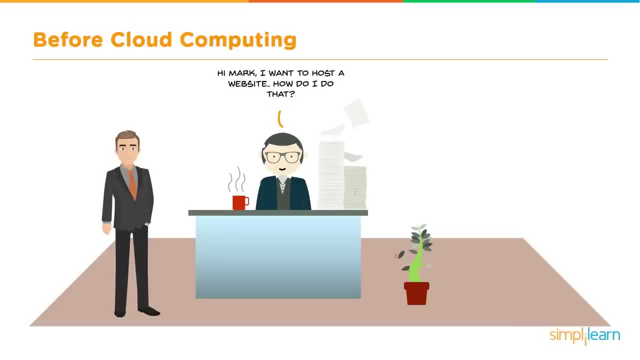 Now he had a smart- not only smart looking, but a really smart- worker in his office called Mark, And on one fine day he called Mark and said that he would like to do business online. In other words, he would like to take his business online. 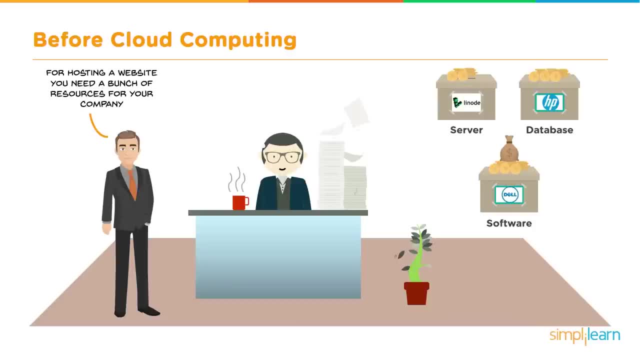 And for that he needed his own business. He needed his own website as the first thing, And Mark puts all his knowledge together and comes up with this requirement that his boss would need lots of servers, databases and softwares to get his business online, which 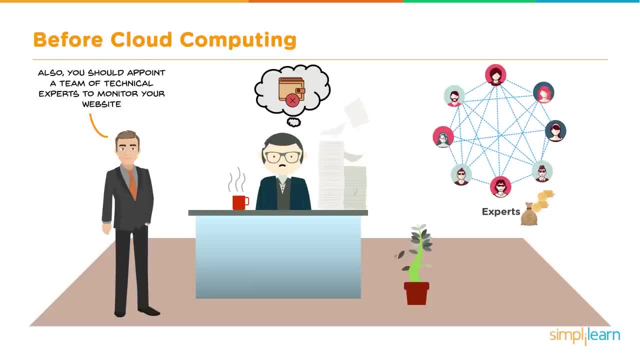 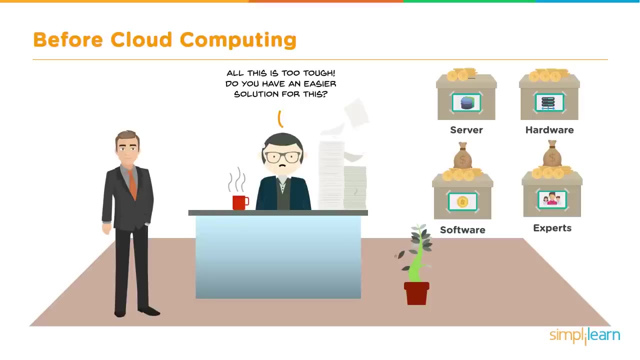 means a lot of investment. And Mark also adds that his boss will need to invest on acquiring technical expertise to manage the hardware and software that they will be purchasing and also to monitor the infrastructure. And after hearing all this, his boss was close. He was close to dropping his plan to go online. 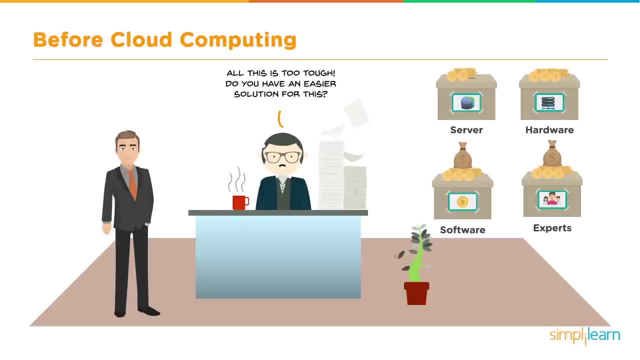 But before he made a decision, he chose to check if there are any alternatives where he don't have to spend a lot of money and don't have to spend acquiring technical expertise. Now, that's when Mark opened this discussion with his boss and he explained his boss about. 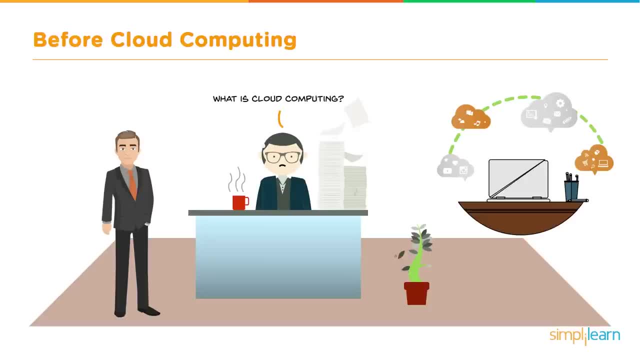 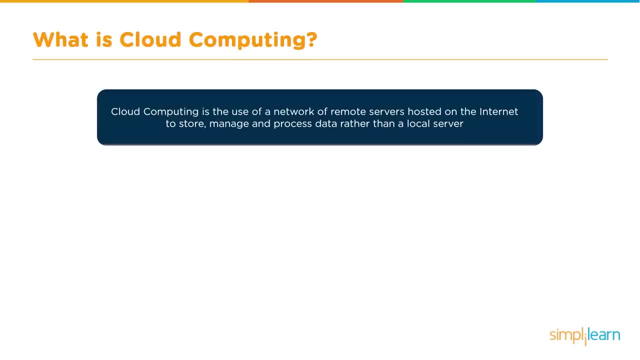 cloud computing, And he explained his boss the same thing that I'm going to explain to you in some time now about what is cloud computing. What is cloud computing? A network of remote servers hosted on the internet to store, manage and process data. 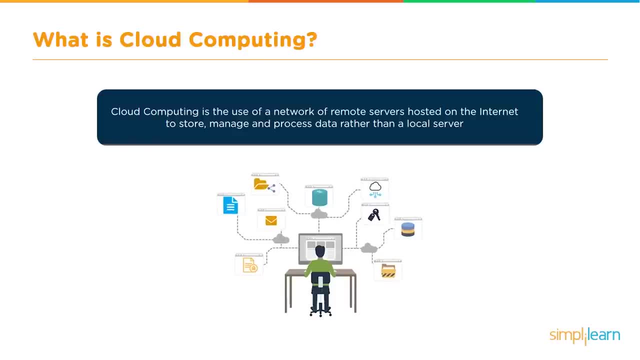 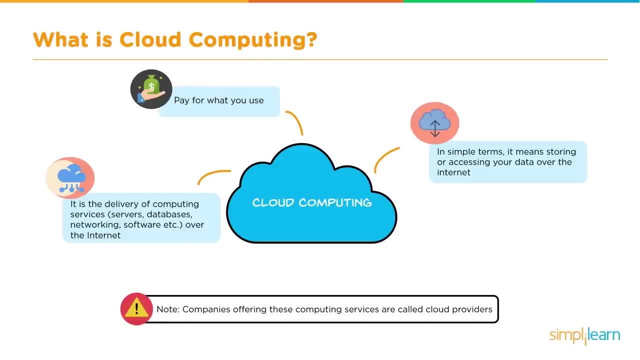 rather than having all that locally and using local server for that. Cloud computing is also storing our data in the internet from anywhere and accessing our data from anywhere throughout the internet, And the companies that offer those services are called cloud providers. Cloud computing is also being able to deploy and manage our applications, services and 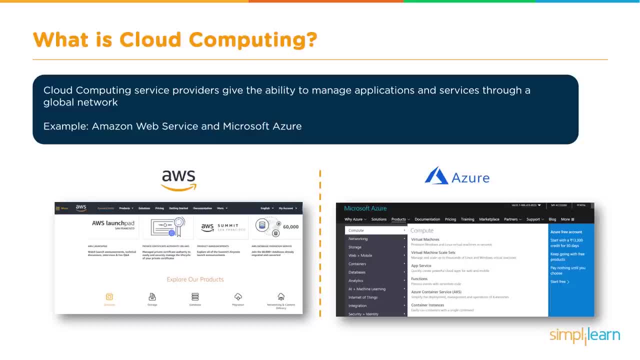 network throughout the globe and manage them through the web management or configuration portal, In other words, cloud computing. service providers give us the ability to manage our applications and services through a global network or internet. Examples of such providers are Amazon Web Service and Microsoft Azure. 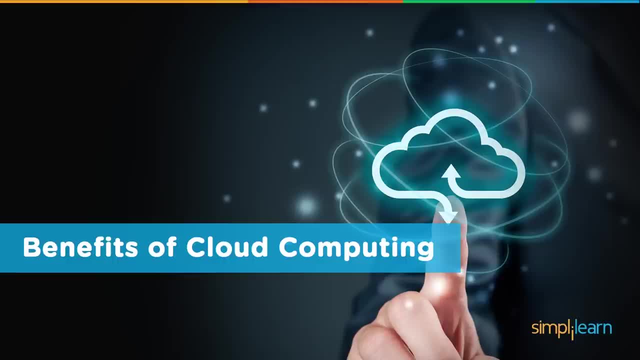 Now that we have known what cloud computing is, let's talk about the benefits of cloud computing. Now I need to tell you the cloud benefits is what is driving cloud adoption, like anything In the recent days. if you want an IT resource or a service, now with cloud, it's available. 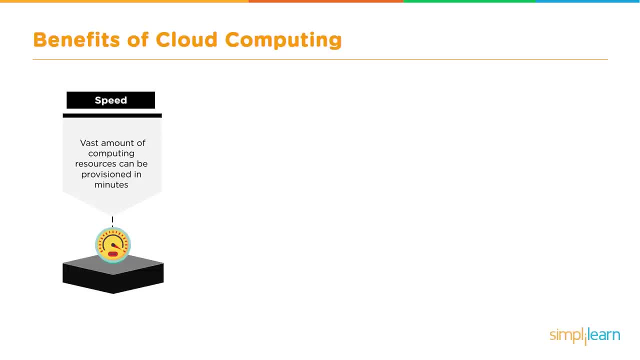 for me almost instantaneously, and it's ready for production almost at the same time. Now this reduces the go-live date and the products and the servers hit the market almost instantaneously, compared to the legacy environment, And because of this, the companies have started to generate revenue almost the next day, if 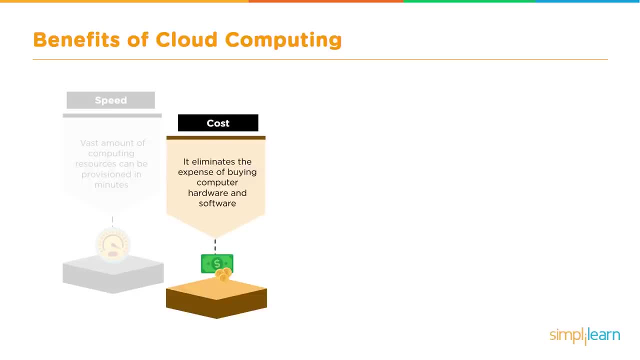 not the same day. Planning and buying the right size hardware has always been a challenge. It's been a challenge- It's always been a challenge in legacy environment, And if you're not careful when doing this, we might need to live with a hardware that's. 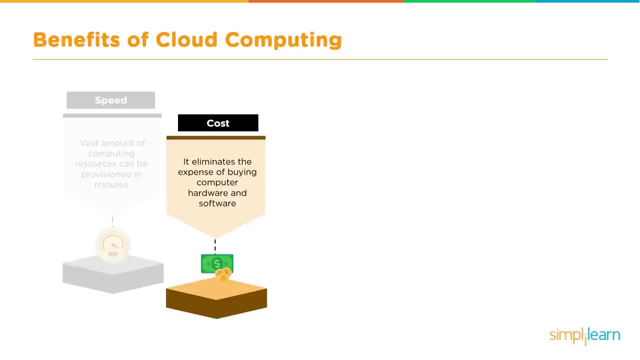 undersized for the rest of our lives. With cloud we do not buy any hardware, but we use the hardware and pay for the time we use it. If that hardware does not fit our requirement, release it and start using a better configuration and pay only for the time you use that new and better configuration. 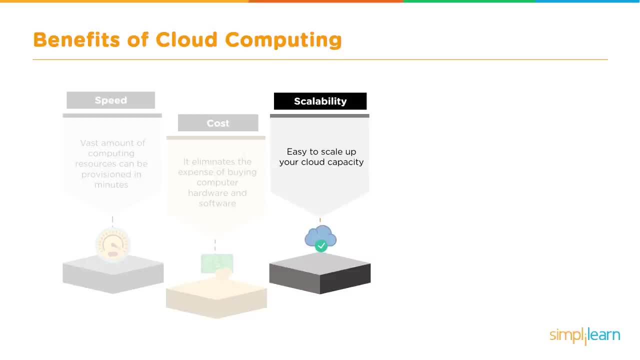 In legacy environments, forecasting demand is a full-time job, But with cloud, you can let the monitoring and automation tool to work for you and to rapidly scale up and down the resources based on the need of that hour. Not only that: the resources, services, data can be accessed from anywhere, as long as we 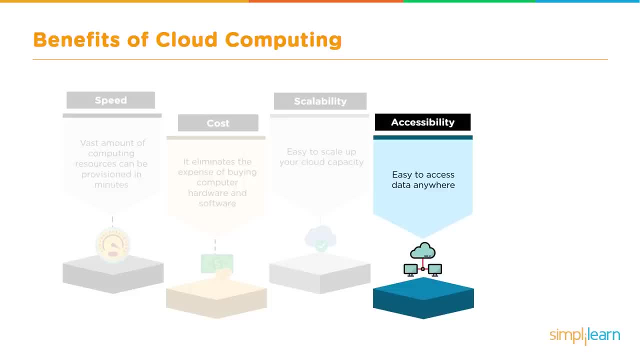 are connected to the internet, And even there are tools and techniques now available which will let you to work offline and will sync whenever the internet is available. Making sure the data is stored in durable storage and in a secure fashion is the talk of the business, and cloud answers that million-dollar question. 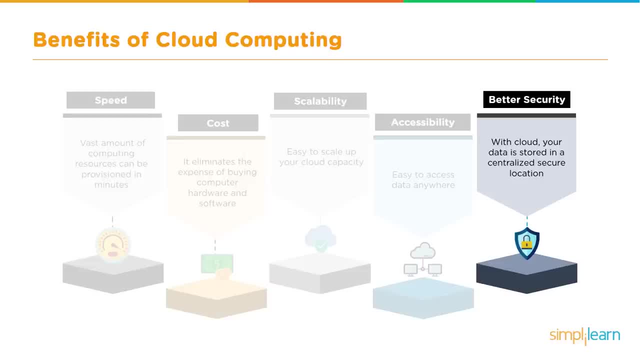 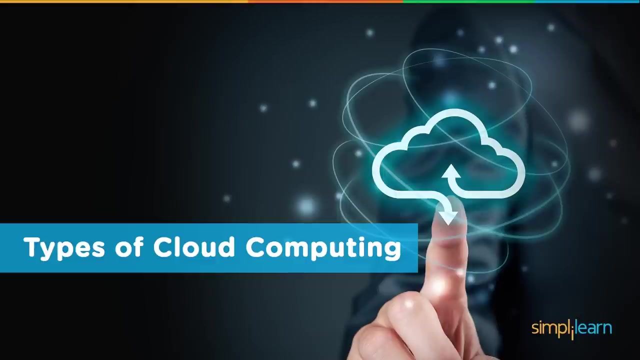 With cloud, the data can be stored in a highly durable storage and replicated to multiple regions, if you want, and the data that we store is encrypted and secured in a fashion that's beyond what we can imagine in local data centers. Now let's bleed into the discussion about the types of cloud computing. 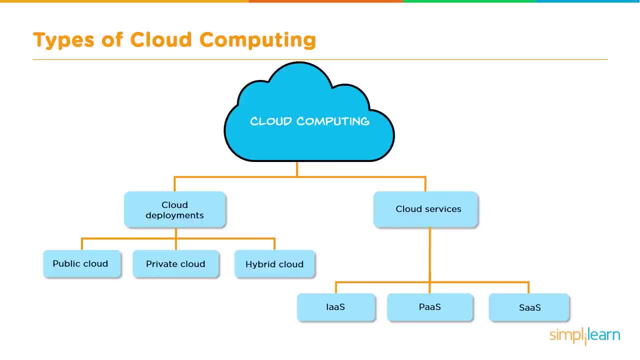 Very lately. there are multiple ways to categorize cloud computing because it's ever growing. Out of all these, six sort of stand out: categorizing cloud based on deployments and categorizing cloud based on services And, again under deployments, categorizing them based on how they have been implemented. 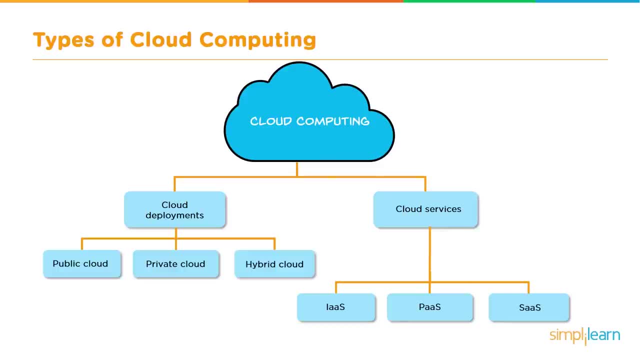 Is it private, Is it public Or is it hybrid? And again, categorizing them based on the service it provides. Is it infrastructure as a service, or is it platform as a service, or is it software as a service? Let's look at them one by one. 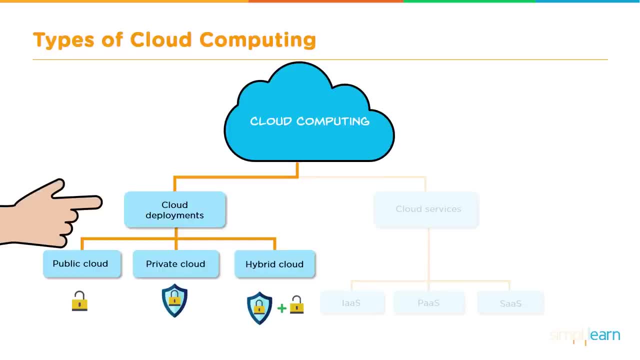 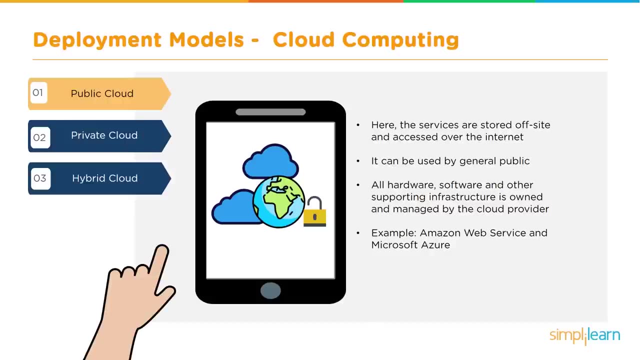 Let's talk about the different types of cloud based on the deployment models. first, In public cloud, everything is stored and accessed in and through the internet, And any internet users with proper permissions can be given access to some of the applications and resources. And in public cloud, we literally own nothing, be it the hardware or software. 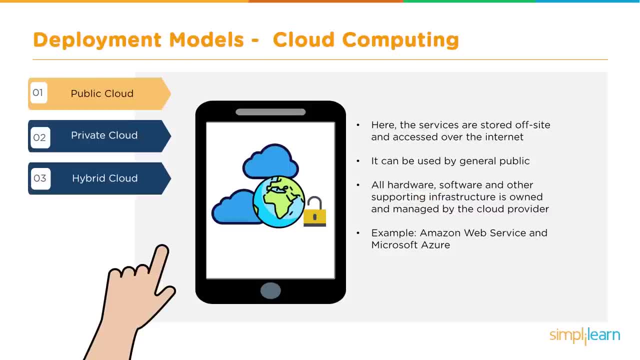 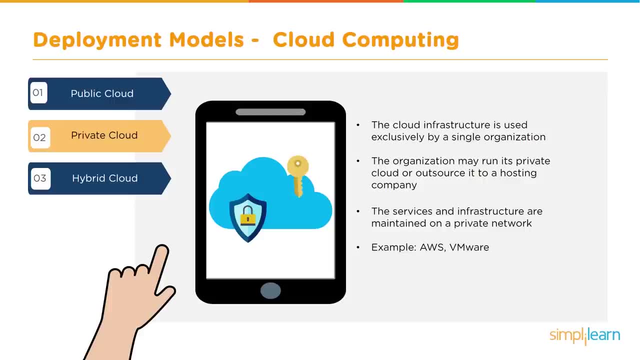 Everything is managed by the provider. AWS, Azure and Google are some examples of public cloud. On the other hand, with private cloud, the infrastructure is exclusively for a single organization. The organizations can choose to run their own cloud locally or choose to outsource it. 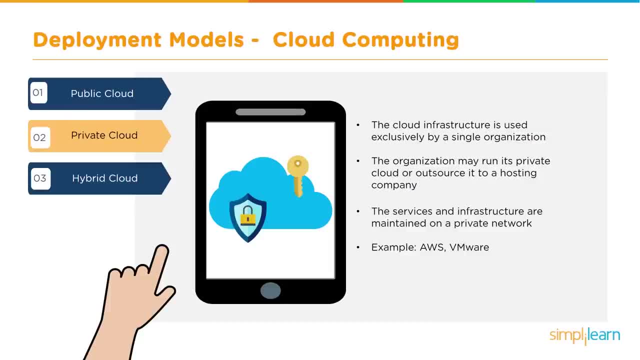 to a public cloud provider as managed services, And when this is done, the service, the infrastructure, will be maintained on a private network. Some examples are VMware cloud and some of the AWS products are very good example for private cloud, Hybrid cloud, Hybrid cloud. 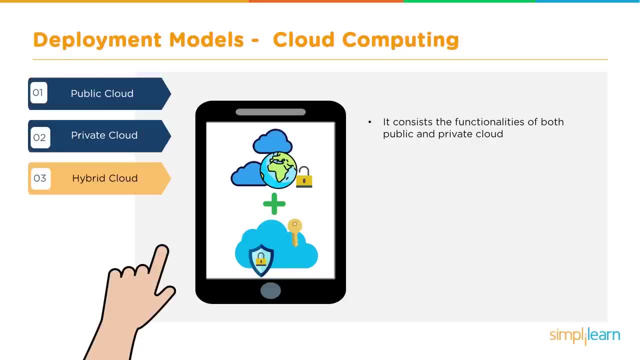 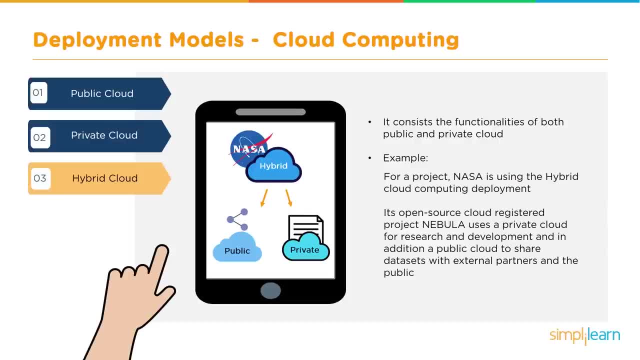 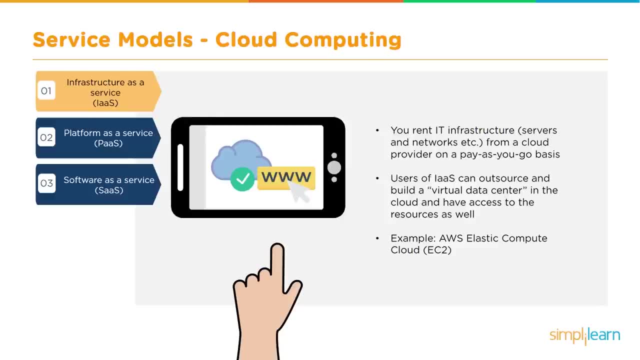 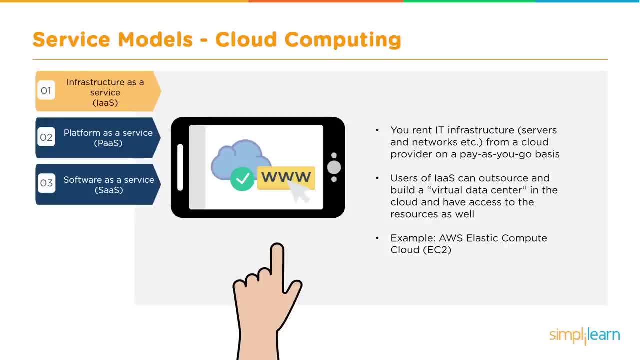 for them in an hourly basis, but we will have access to the resources we provision and for some we will have root level access as well. EC2 in AWS is a very good example. It's a VM for which we have root level access to the OS, and 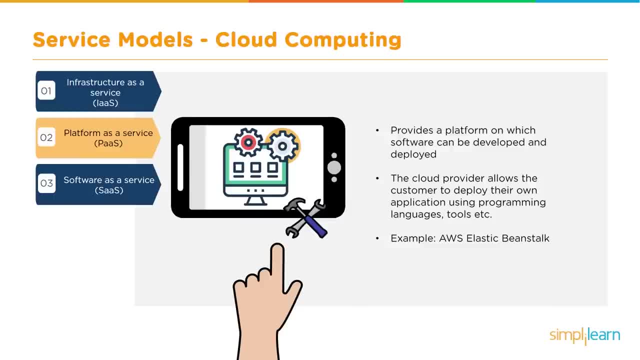 admin access to the hardware. The next type of service model would be platform as a service. Now, in this model, the provider's will give me a pre-built platform where we can deploy our codes and our applications, and they will be up and running. We only need to manage the codes and not the infrastructure. 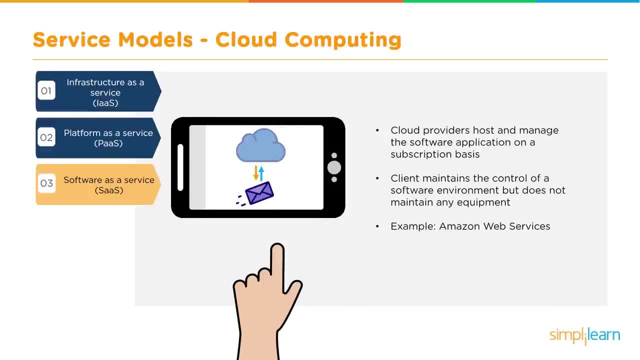 Here in software as a service, the cloud providers sell the end product, which is a software on an application, and we directly buy the software on subscription basis. It's not the infra or the platform, but the end product, Thank you, or the software or a functioning application, and we pay for the hours we use the software. 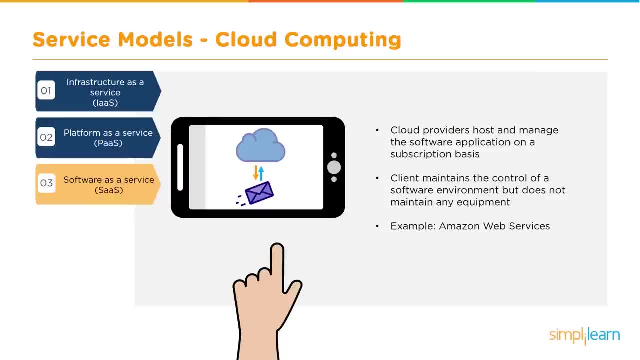 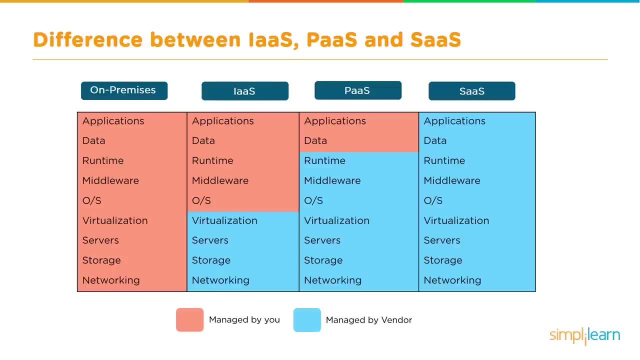 And in here the client maintains full control of the software and does not maintain any equipment. Amazon and Azure also sell products that are software as a service. This chart sort of explains the difference between the four models, starting from on-premises to infrastructure as a service. 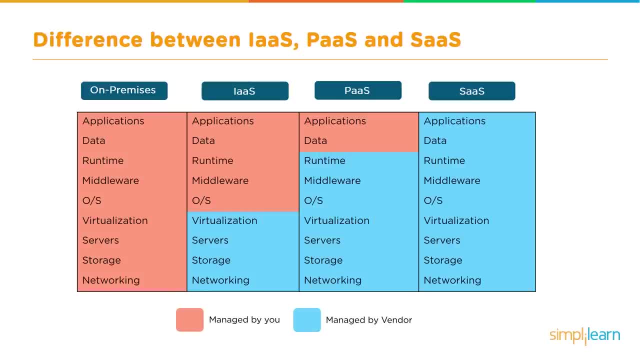 to platform as a service, to software as a service. This is self-explanatory that the resources managed by us are huge in on-premises that towards your left as you watch, and it's little less in infrastructure as a service as we move further towards the right. 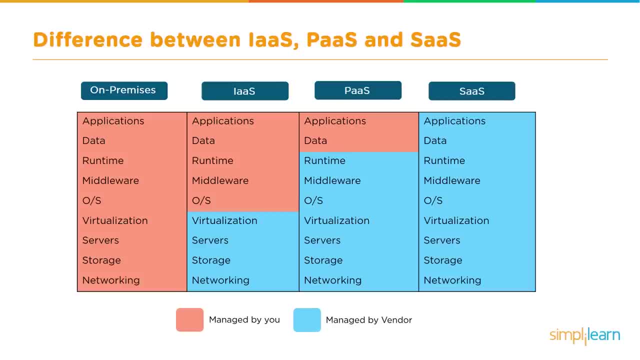 and further reduced in platform as a service. And there's really nothing to manage when it comes to software as a service, because we buy the software, not any infrastructure component attached to it. Now let's talk about the lifecycle of the cloud computing solution. 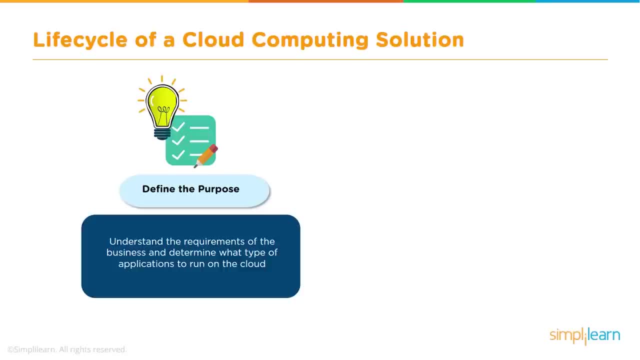 The very first thing in the lifecycle of a solution or a cloud solution is to get a proper understanding of the requirement. I didn't say get the requirement, but said get a proper understanding of the requirement. It is very vital because only then we will be able to properly pick the right service offered by the provider. 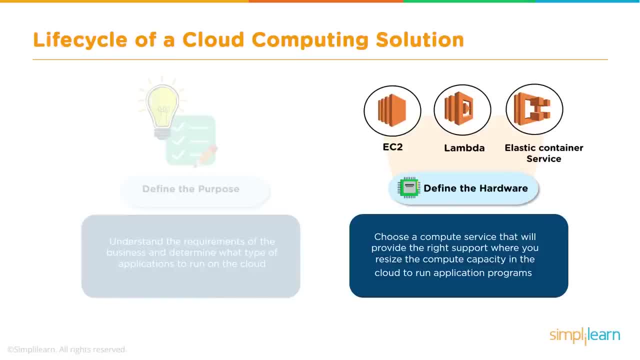 Getting a sound understanding, the next thing would be to define the hardware, meaning: choose the compute servers that will provide the right support where you can resize the compute capacity in the cloud to run application programs. Getting a sound understanding of the requirement helps in picking the right hardware. 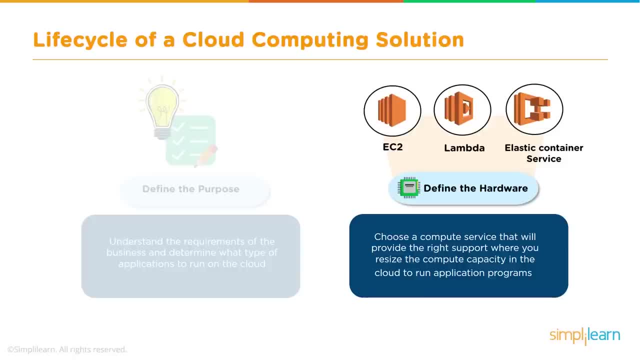 One size does not fit all. There are different services and hardwares for different needs. you might have like EC2, if you're looking for IaaS, and Lambda if you're looking for serverless computing, and ECS that provides containerized service. 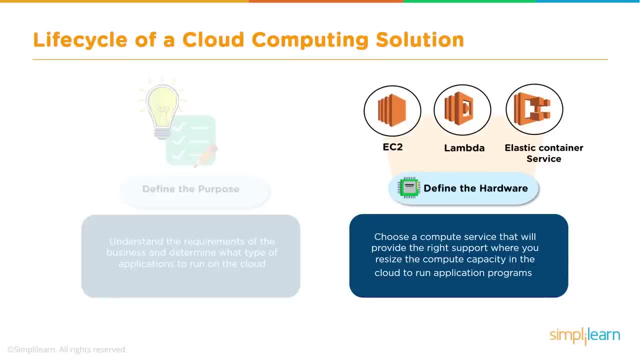 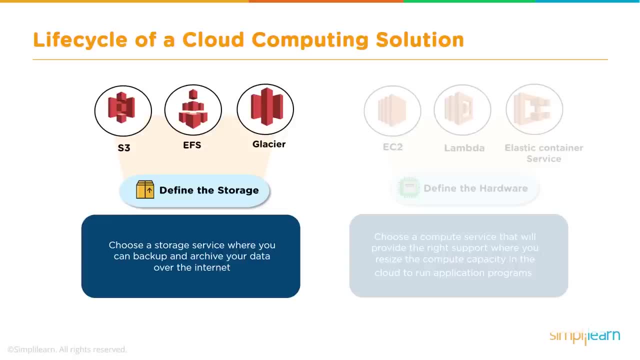 So there are a lot of hardwares available. Pick the right hardware that suits your requirement. The third thing is to define the storage. Choose the appropriate storage service where you can backup your data and a separate storage service where you can archive your data. 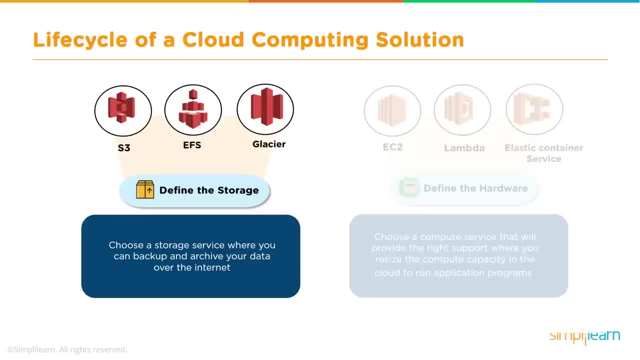 locally within the cloud or from the internet, And choose the appropriate storage. There is one separately for backup, called S3, and there is one separately for archival, that's for Glacier. So you know you knowing the difference between them really helps in picking the right service for the right kind of need. 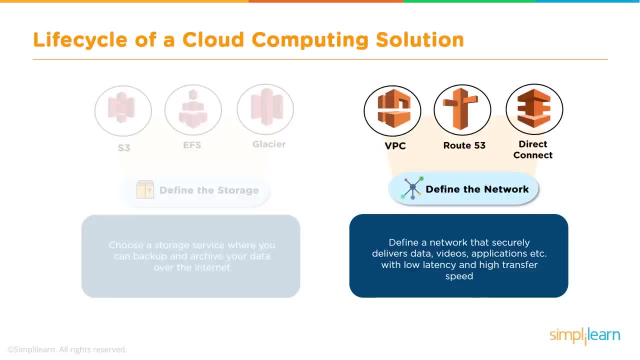 Define the network. Define the network that securely delivers data, video and applications. Define and identify the network services properly, For example, VPC for network, Route 53 for DNS and direct connection for private P2P line from your office to the AWS data center. 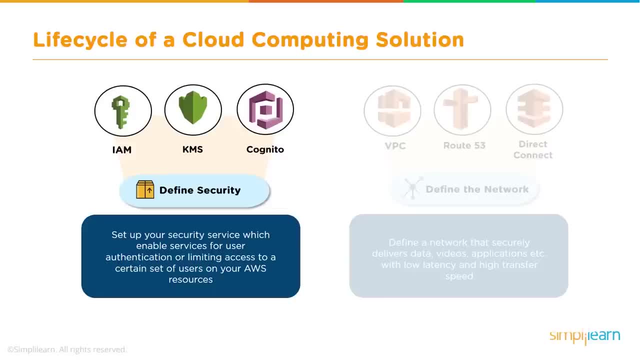 Set up the right security services- IAM for authentication and authorization and KMS for data encryption- at rest. So there are a variety of security products available. We got to pick the right one that suits our need, And there are a variety of deployment and automation. 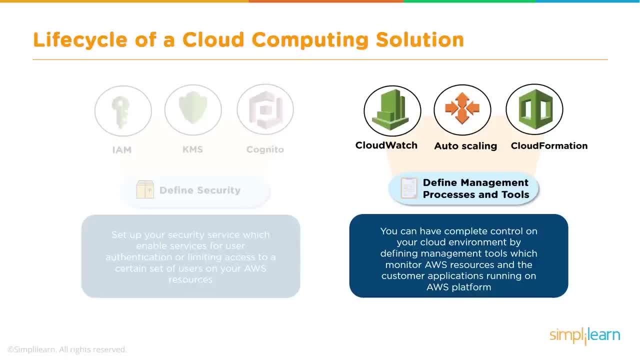 and monitoring tools that you can pick from. For example, CloudWatch is for monitoring, autoscaling is for being elastic and CloudFormation is. define the management process and tools. You can have complete control of your cloud environment if you define the management tools which monitors your AWS resources. 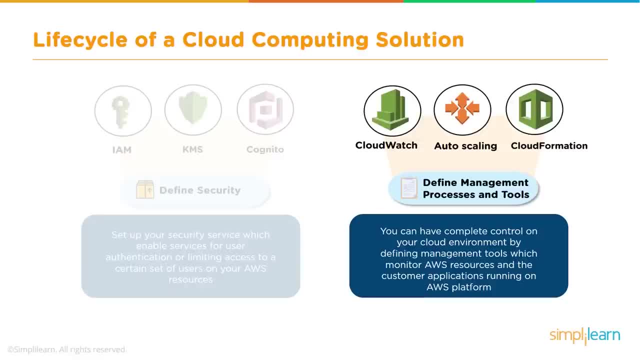 and all the custom applications running on AWS platform. There are a variety of deployment automation and monitoring tools you can pick from, like CloudWatch for monitoring, autoscaling for automation and CloudFormation for deployment. So knowing them will help you And you can also use them to do some of the things. 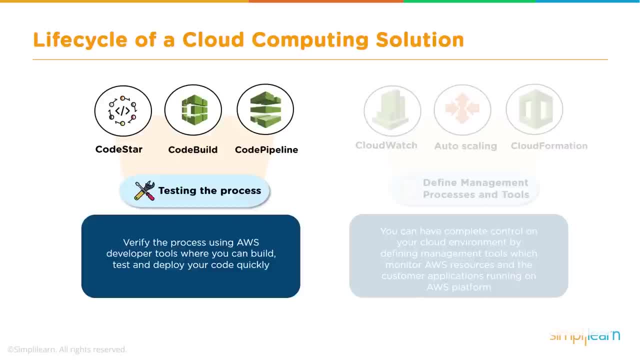 that you can do in defining the lifecycle of the cloud computing solution properly And similarly, there are a lot of tools for testing a process, like CodeStar and CodeBuild and CodePipeline. These are tools with which you can build, test and deploy your code quickly. 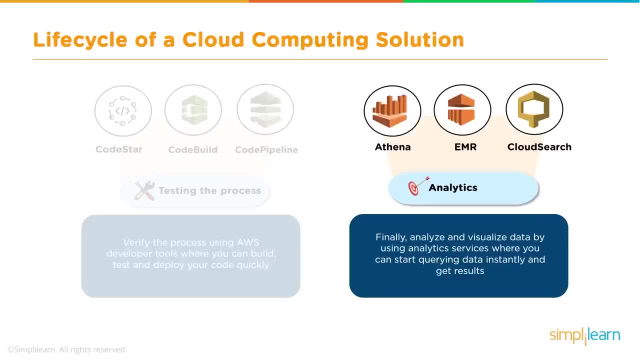 And finally, once everything is said and done, pick the analytic service for analyzing and visualizing the data, using the analytic services, where we can start querying the data instantly and get a result Now, if you want to see the happenings in your environment. 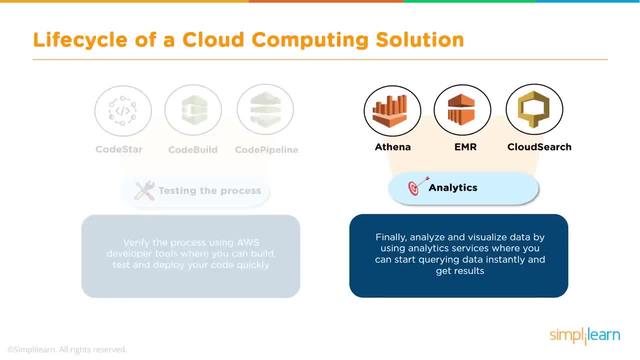 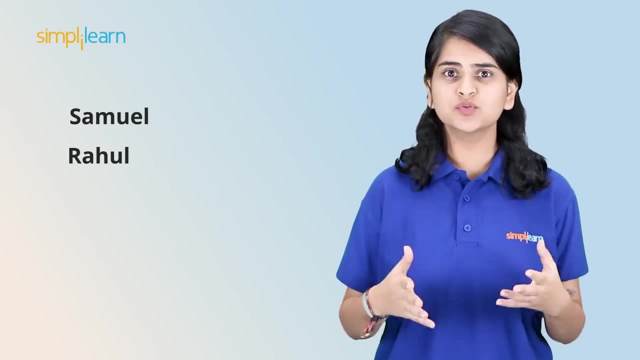 you can pick Athena and other tools for analytics or EMR, which is Elastic Map Produce and Cloud Search. Thanks guys, Now we have Samuel and Rahul to take us through the full course in which they will explain basic framework of Amazon Web Services. 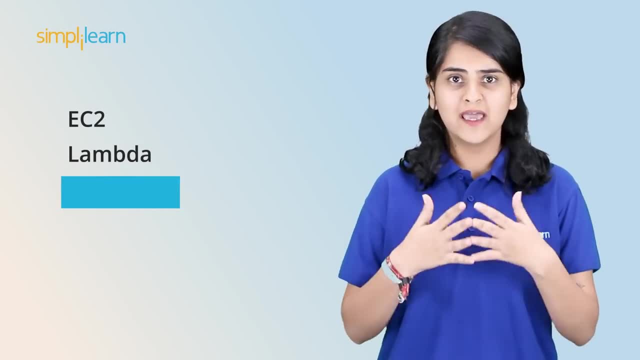 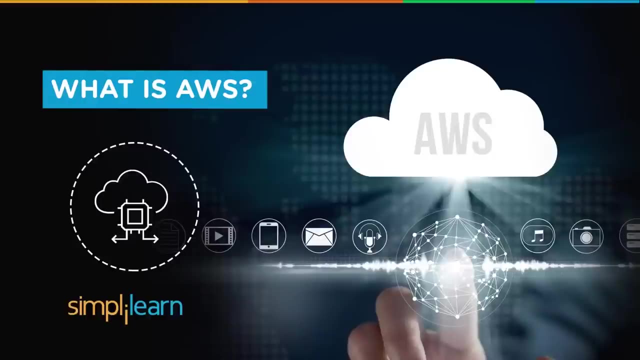 and explore all of its important services, like EC2, Lambda S3, IAM and CloudFormation. We'll also talk about Azure and some of its popular services. Hello everyone, Let me introduce myself: I'm a multi-platform cloud architect and trainer. 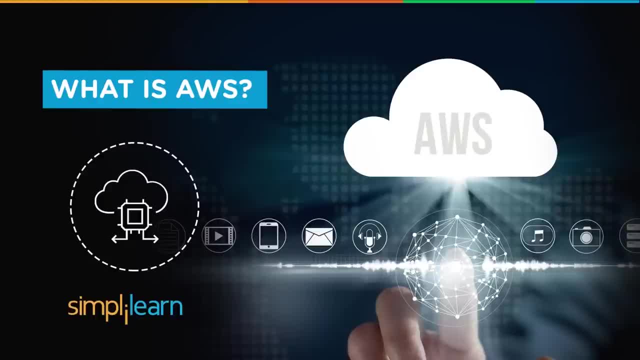 and I'm so glad, and I'm equally excited- to talk and walk you through the session about what AWS is and talk to you about some services and offerings and about how companies get benefited by migrating their applications and infra into AWS. So what's AWS? 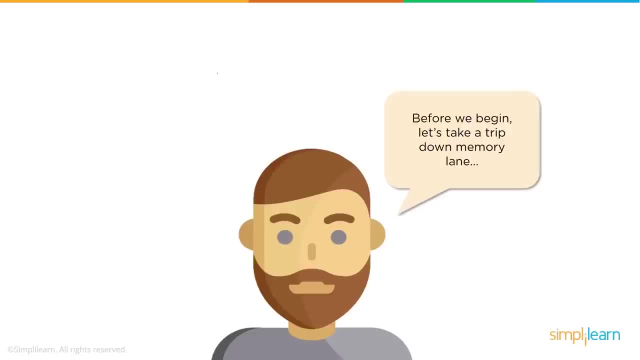 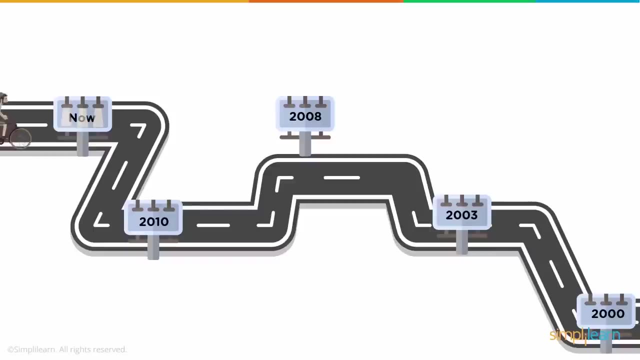 Let's talk about that Now. before that, let's talk about how life was without any cloud provider and in this case, how life was without AWS. So let's walk back And picture how things were back in 2000,, which is not so long ago. 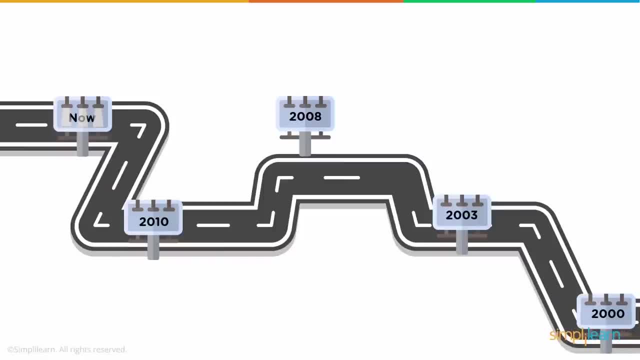 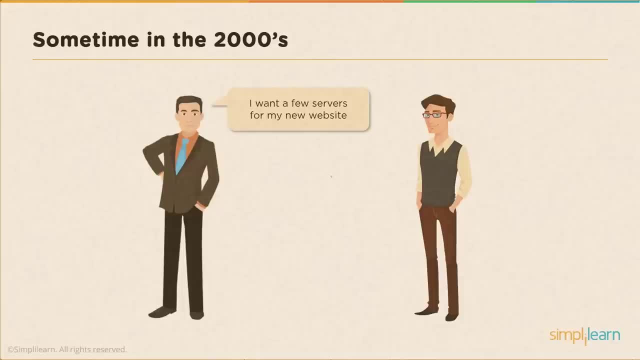 but a lot of changes, a lot of changes for better, had happened since that time. Now, back in 2000,. a request for a new server is not an happy thing at all, because a lot of money, a lot of validations, a lot of planning are involved in getting a server online or up and running. 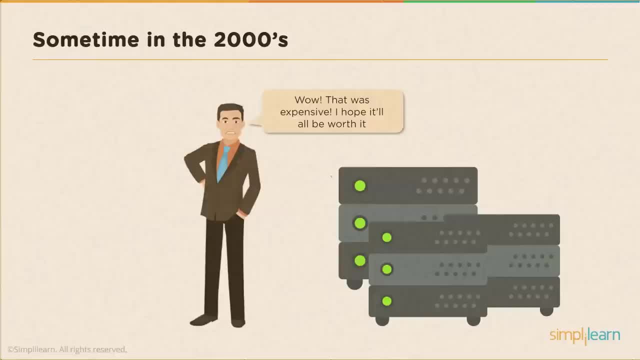 And even after we've finally got the server, it's not all said and done. There's a lot of optimization That needs to be done on that server to make it worth it and get a good return on investment from that server. And even after we have optimized for a good return on investment, 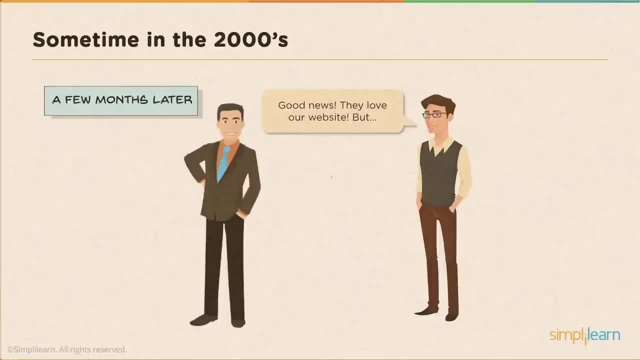 the work is still not done. There will often be a frequent increase and decrease in the capacity, And you know even news about our website getting popular and getting more hits. it's still a bittersweet experience because now I need to add more servers to the environment. 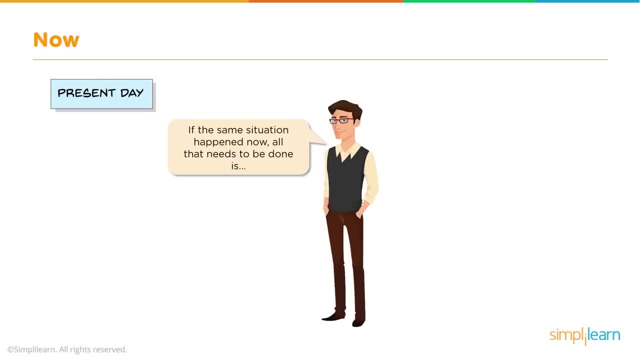 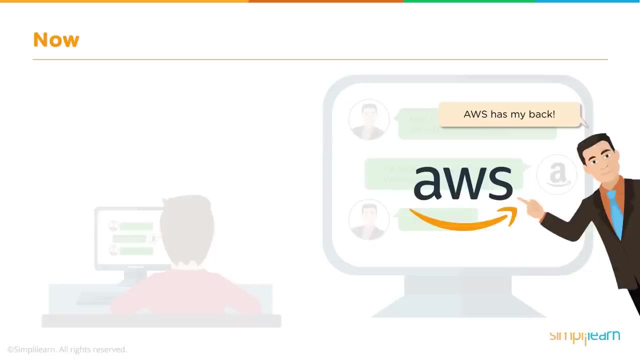 because it's going to cost me even more. But thanks to the present day cloud technology, if the same situation were to happen today, my new server, it's almost ready and it's ready instantaneously And with the swift tools and technologies that Amazon is providing. 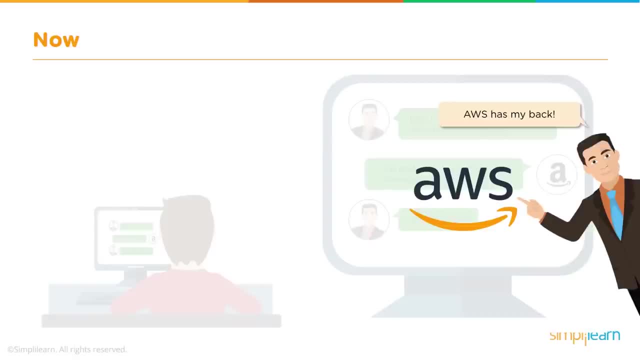 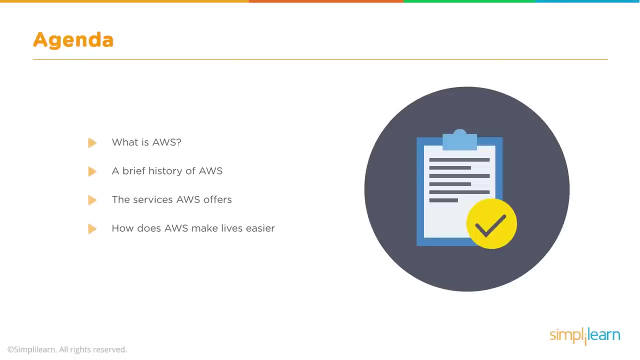 in provisioning my server instantaneously and adding any type of workload on top of it and making my storage and server secure, you know, creating a durable storage, making sure that the data that I store in the cloud never gets lost. with all that features, Amazon has got our back. 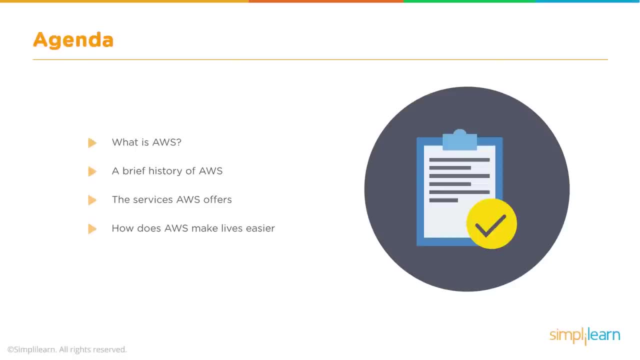 So let's talk about what is AWS. There are a lot of definitions for it, but I'm going to put together a simple and a precise definition as much as possible. Now let me iron that out: Cloud still runs on an hardware, right. 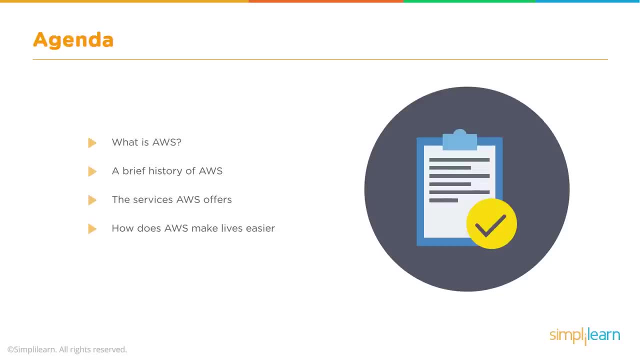 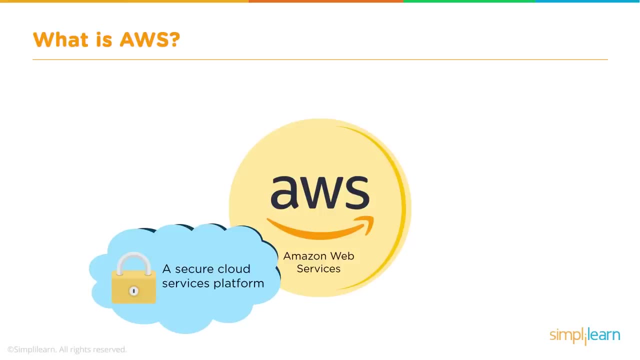 And there are certain features in that infrastructure, in that cloud infrastructure that makes cloud cloud or that makes AWS a cloud provider. Now we get all the services, all the technologies, all the features and all the benefits that we get in our local data center. 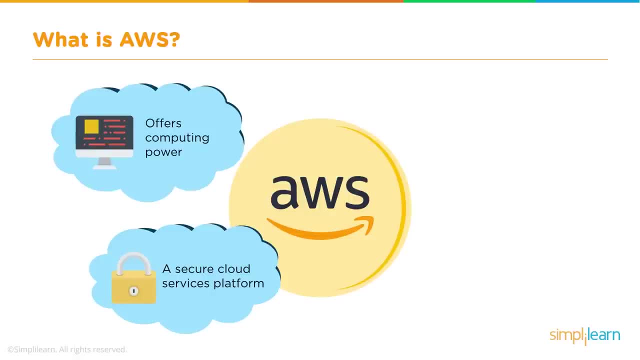 like you know, security and compute capacity and databases, And in fact, you know, we get even more cool features like content caching in various global locations around the planet. But again, out of all the features, the best part is that I get. 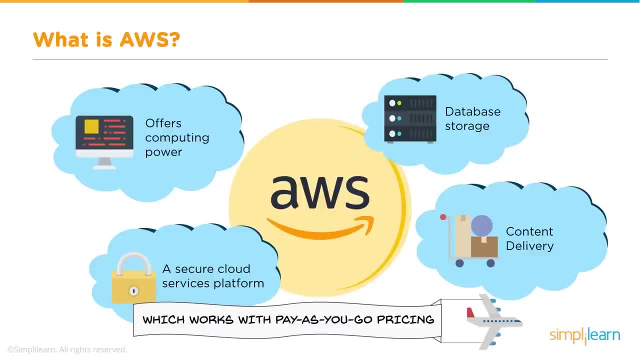 or we get everything on a pay as we go model. The less I use it, the better. The less I use it, the better. The less I use it, the better. The less I use, the less I pay, And the more I use, the less I pay per unit. 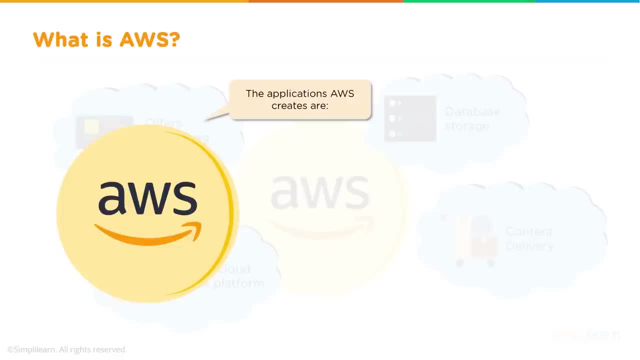 Very attractive, isn't it right? And that's not all. The applications that we provision in AWS are very reliable because they run on a reliable infrastructure And it's very scalable because it runs on an on-demand infrastructure. And it's very flexible because of the designs. 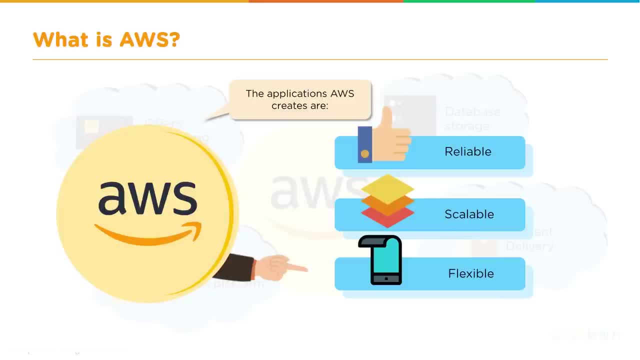 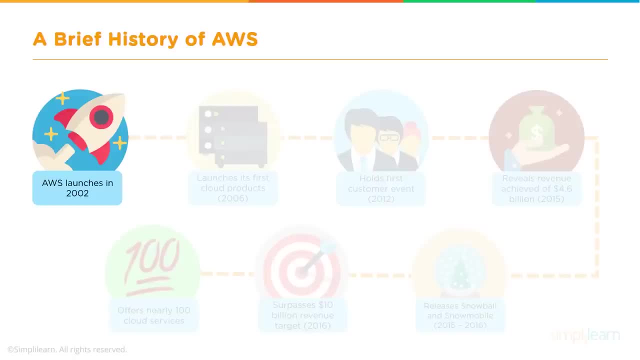 and because of the design options available for me in the cloud. Let's talk about. let's talk about how all this happened. AWS was launched in 2002 after the Amazon- we know as the online retail store- wanted to sell their remaining or unused infrastructure as a service. 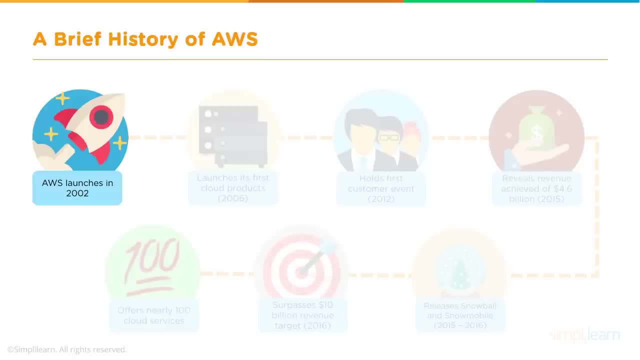 or as an offering for customers to buy and use it from them. You know sell infrastructure as a service. The idea sort of clicked and AWS launched their first product- first product- in 2006.. That's like four years after the idea was launched. 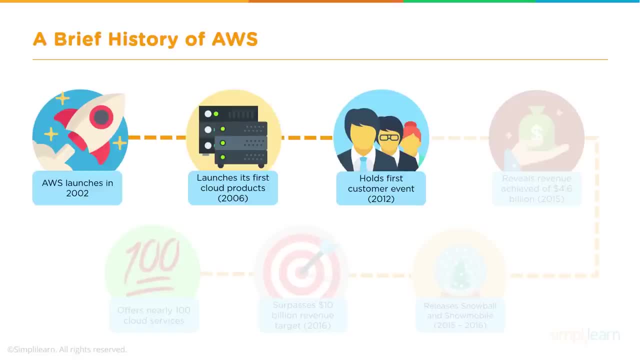 And in 2012, they held a big sized customer event to gather inputs and concerns from customers And they were very dedicated in making those requests happen. And that habit is still being followed. It's still being followed as reinvent by AWS. 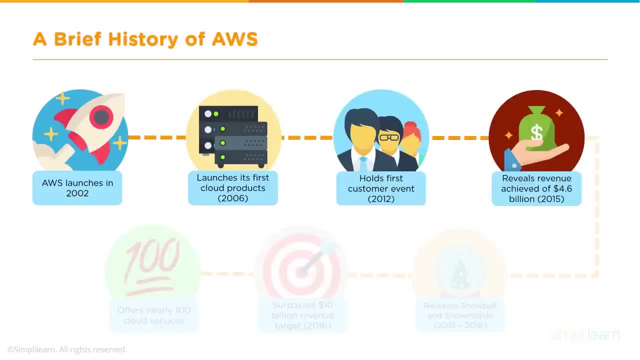 And at 2015,, Amazon announced its revenue to be 4.6 billion. And in 2015 through 2016,, AWS launched products and services that help migrate customer services into AWS. Well, there were products even before, but this is when a lot of focus was given on developing migrating services. 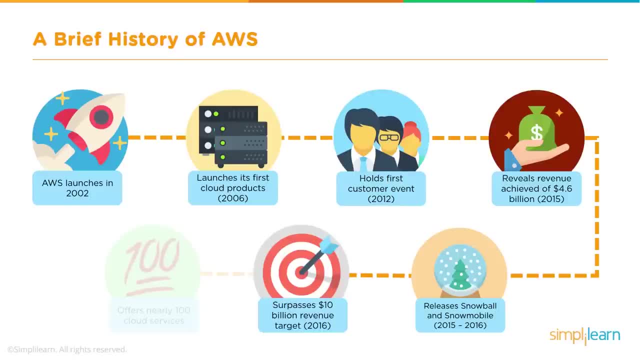 And in the same year, that's, in 2016,, Amazon's revenue was 10 billion And not but not the least. as we speak, Amazon has more than a hundred products and services available for customers and get benefited from All right. 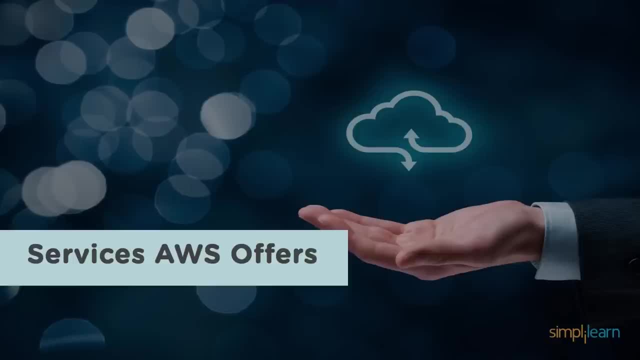 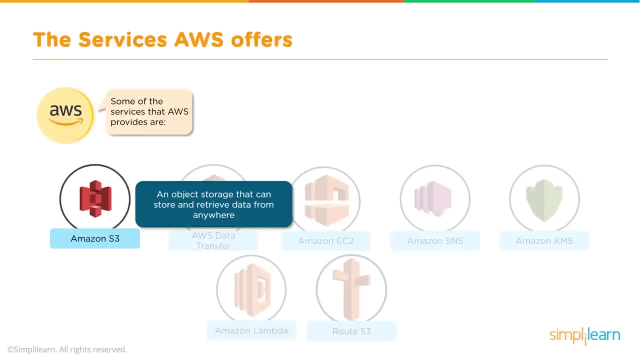 Let's talk about the services that are available in in Amazon. Let's start with this product called S3.. Now, S3 is a great tool for internet backup, and it's it's the cheapest storage option in the object storage category. And not only that. 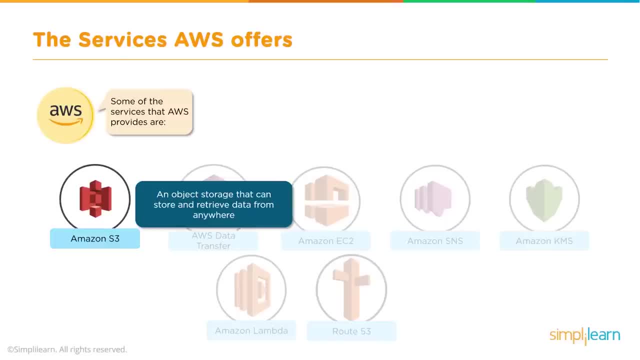 the data that we put in S3 is retrievable from the internet. S3 is really cool, And we have other products like migration and data collection and data transfer products, And here we can not only collect data seamlessly, but also in a real time way. 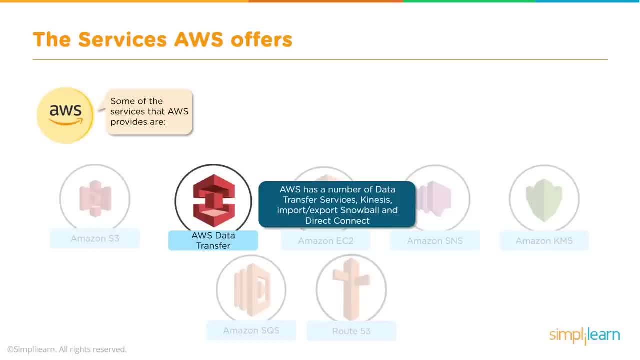 monitor the data Or analyze the data that's being received, That. there are cool products like AWS data transfers available that helps achieve that. And then we have products like EC2, Elastic Compute Cloud. That's an resizable computer where we can anytime. 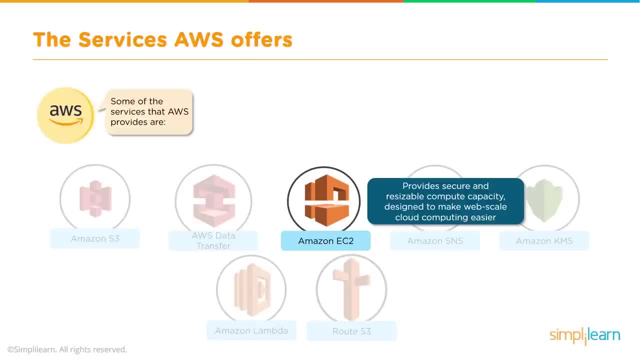 anytime, alter the size of the computer based on the need or based on the forecast. Then we have simple notification services, systems and tools available in Amazon to update us with notifications through email or through SMS. Now, anything, anything can be sent through email or through SMS. 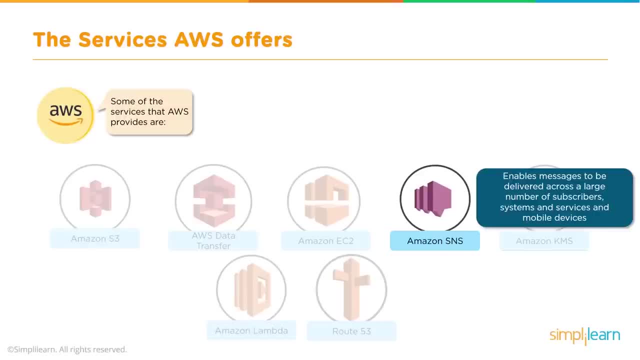 If we use that service, it could be alarms or it could be service notifications, if you want stuff like that. And then we have some security tools like KMS key management system, which uses AES 256 bit encryption to encrypt our data at rest. 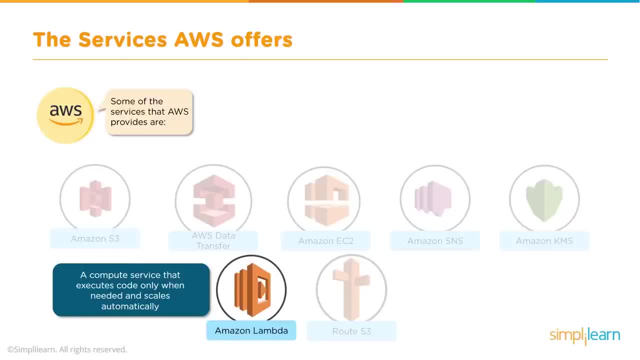 Then we have Lambda, a service for which we pay only for the time in seconds, seconds it takes to execute our code, And we're not paying for it For the infrastructure here. it's just the seconds the program is going to take to execute the code. 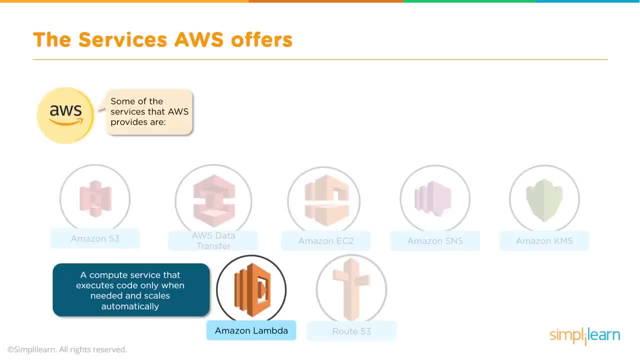 If it's a short program, we'll be paying in milliseconds. If it's a bit bigger program, we'll be probably paying in 60 seconds or 120 seconds. But that's a lot cheap, lot simple and lots cost effective as against paying for service on an hourly basis. 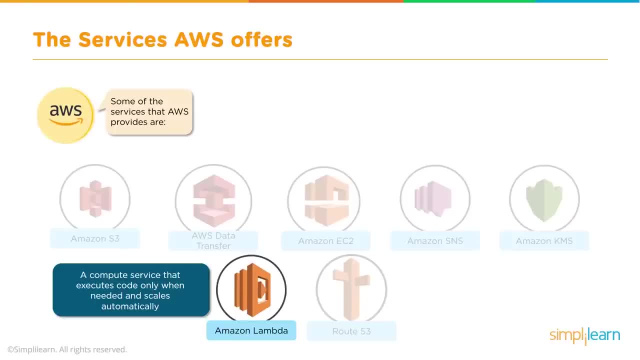 which a lot of other services are. Well, that's cheap, but using Lambda is a lot cheaper than that. And then we have services like Route 53, a DNS service in the cloud, And now I do not have to maintain a DNS account somewhere else. 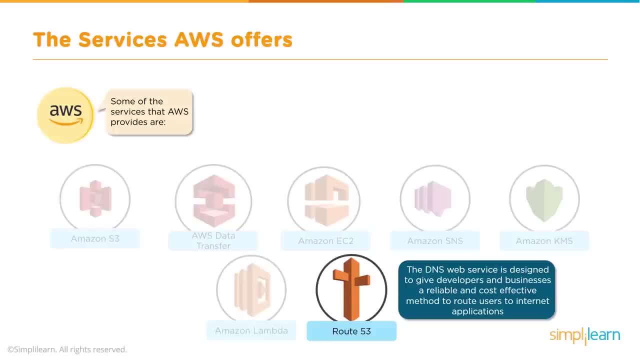 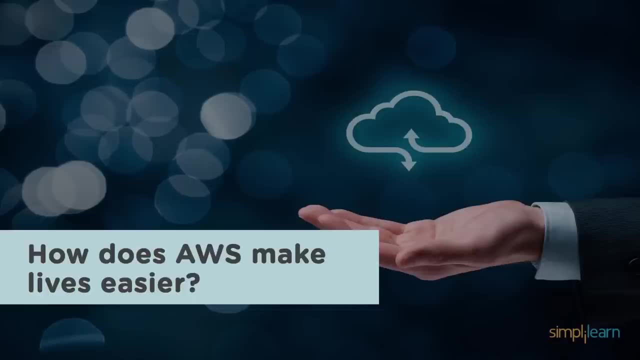 and my cloud environment. with AWS, I can get both in the same place. All right, Let me talk to you about how AWS makes life easier, or how companies got benefited by using AWS as their IT provider for their applications or for the infrastructure. Now Unilever is a company and they had a problem, right. 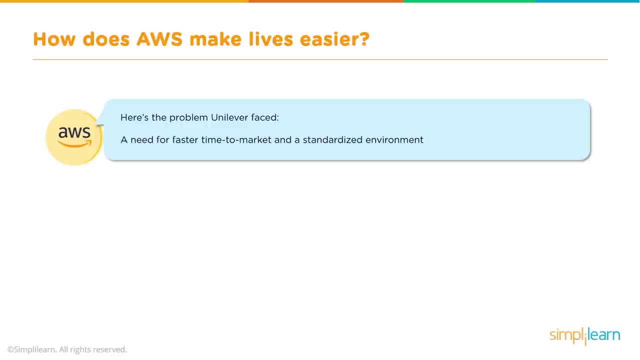 And they had a problem and they picked AWS as a solution to their problem. All right, Now this company was sort of spread across 190 countries and they were relying on a lot of digital marketing for promoting their products and their existing environment. their legacy local environment proved not to support their changing IT demands. 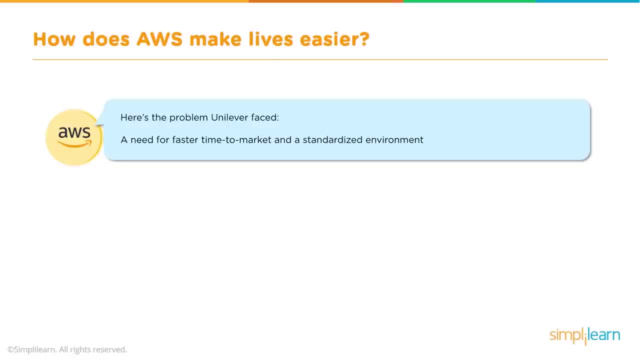 and they could not standardize their old environment. Now they chose to move part of their applications to AWS because they were not getting what they wanted in their local environment And since then, you know, rollouts were easy. Provisioning your applications became easy. 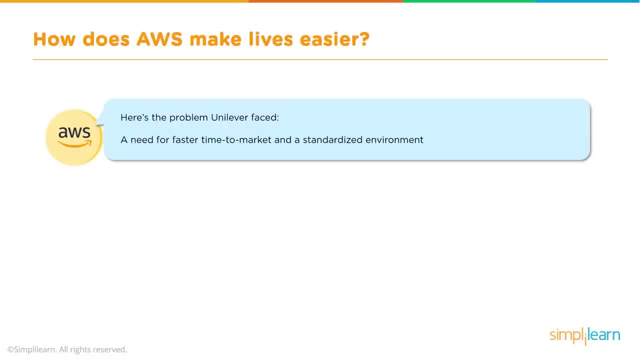 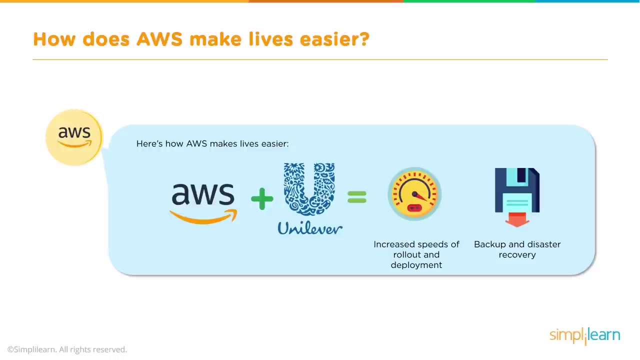 and even provisioning infrastructure became easy, and they were able to do all that in push button scaling And needless to talk about backups that are safe and backups that can be securely accessed from the cloud as needed. Now that company is growing along with AWS because of their swift speed in rolling out deployments. 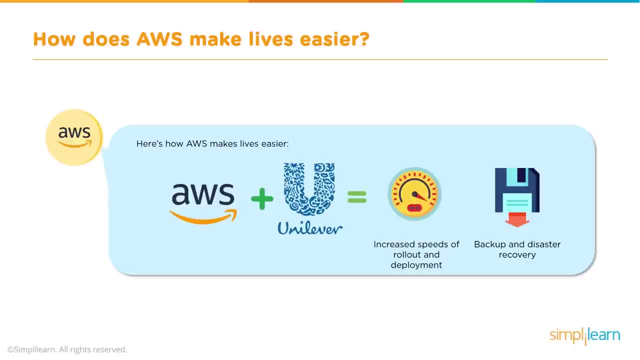 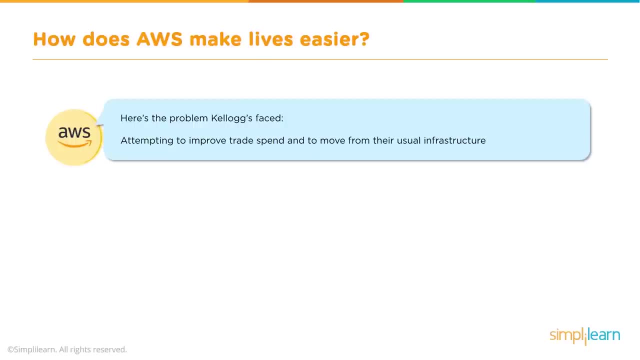 and being able to access secure backups from various places and generate reports- And, in fact, useful reports- out of it. that helps their business. Now, on the same lines, let me also talk to you about Kellogg's and how they got benefited by using Amazon. 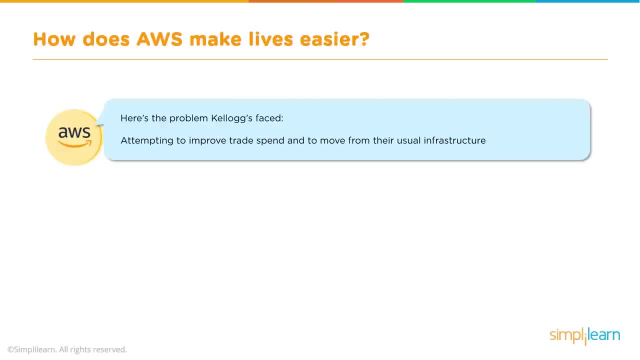 Now Kellogg's had a different problem. It's one of its kind Now. their business model was very dependent on an infra that will help to analyze data really fast, right, Because they were running promotions based on the analyzed data that they get. 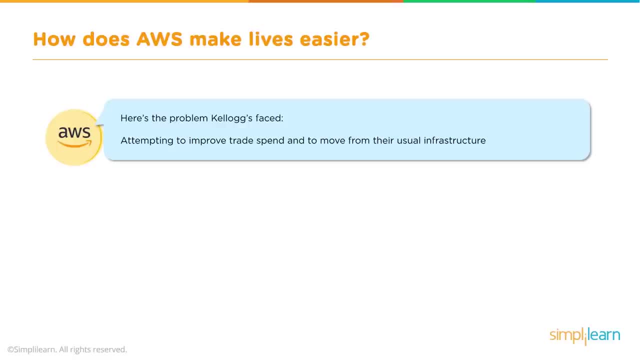 So they're being able to respond to the analyzed data as soon as possible- was critical or vital in their environment And luckily SAP running on HANA environment is what they needed And you know they picked that service in the cloud and that sort of solve the problem. 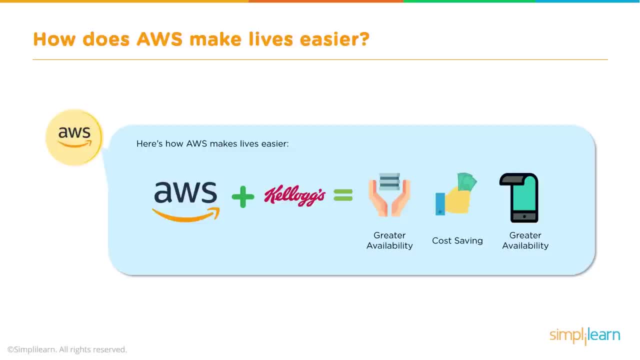 Now the company does not have to deal with maintaining their legacy infra and maintaining their heavy compute capacity and maintaining their database locally. All that is now moved to the cloud or they are using cloud as their IT service provider and an infra And now they have a greater and powerful IT environment that very much complements their 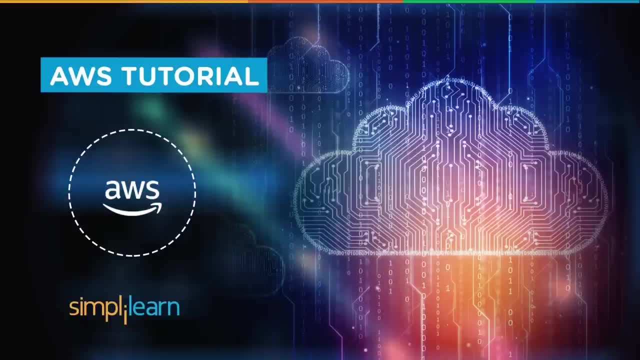 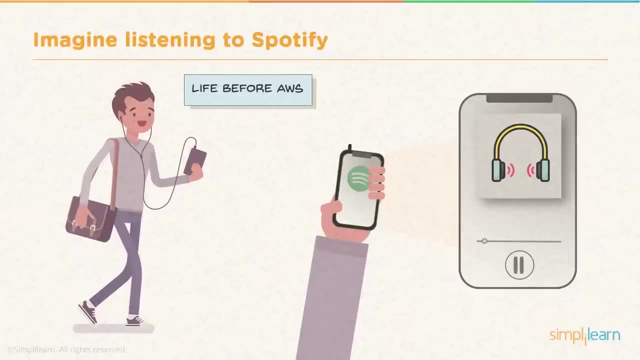 business. Hi there, I'm Samuel, a multi-platform cloud architect, and I'm very excited and honored to walk you through this learning series about AWS. Let me start the session with this scenario: Let's imagine how life would have been without Spotify. 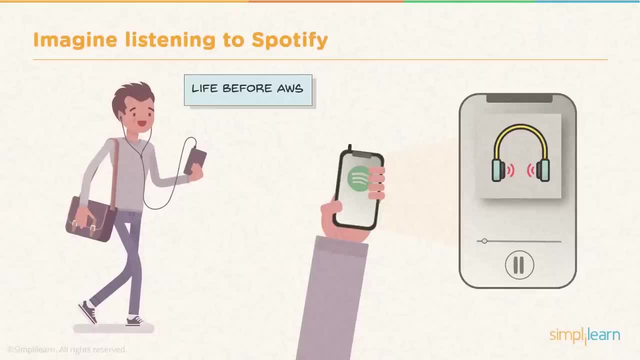 For those who are hearing about Spotify for the first time, Spotify is an online music service offering and it offers instant access to over 16 million licensed songs. Spotify now uses AWS cloud to store the data and share it with their customers, But prior to AWS, they had some issues. 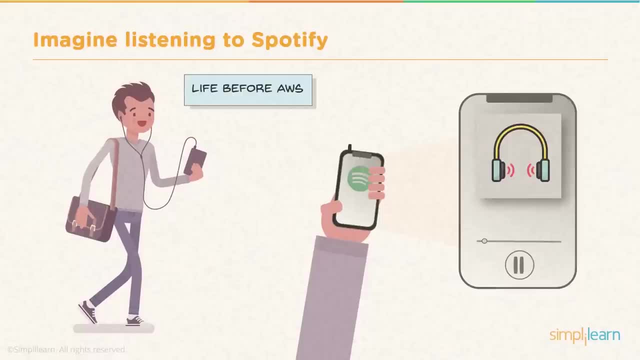 Imagine using Spotify before AWS. Let's talk about that. Back then, users were often getting errors because Spotify could not keep up with the increased demand for storage every new day And that led to users getting upset and users canceling the subscription. The problem: 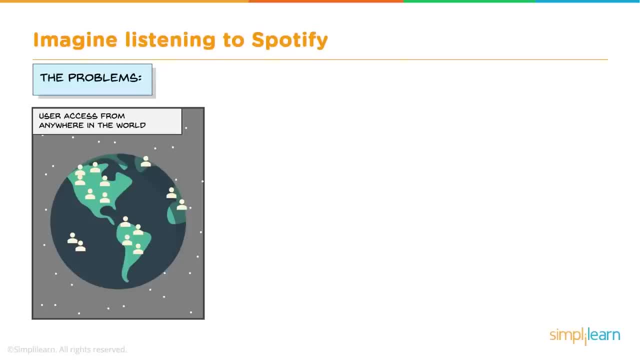 What Spotify was facing at that time was their users were present globally and were accessing it from everywhere, And they had different latency in their applications, And Spotify had a demanding situation where they need to frequently catalog the songs released yesterday, today and in the future. 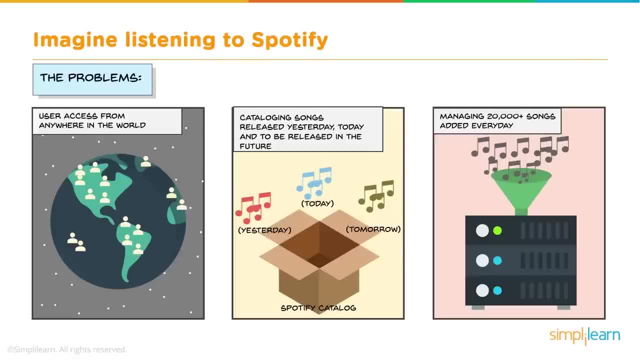 And this was changing every new day, And the songs coming in rate was about 20,000 a day, And back then they could not keep up with this requirement And, needless to say, they were badly looking for a way to solve it. 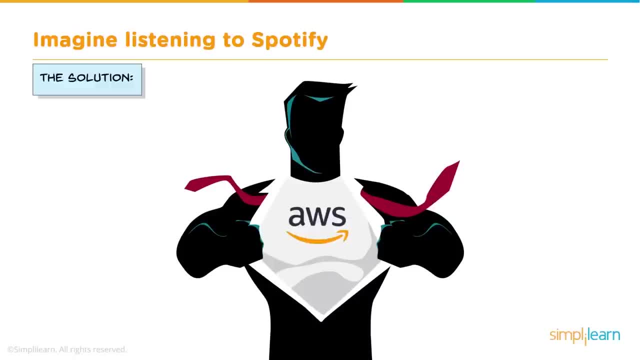 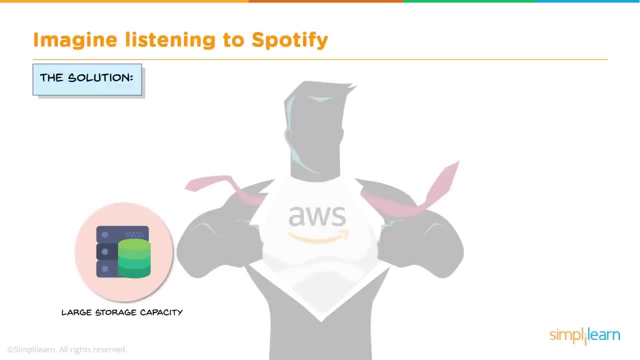 And that's when they got introduced to AWS, And it was a perfect fit and match for their problem. AWS offered a dynamically increasing storage And that's what they needed. AWS also offered tools and techniques like storage, lifecycle management and trusted advisor to properly utilize the resource. 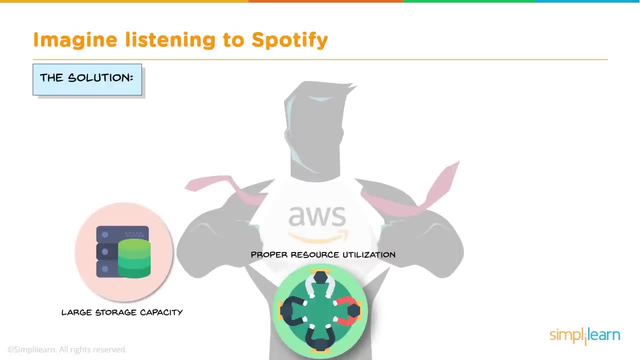 So we always get the best out of the resource used. AWS addressed their concerns about easily being able to scale. Yes, You can scale the AWS environment very easily, And that's what they did. How easily? How easily, One might ask. 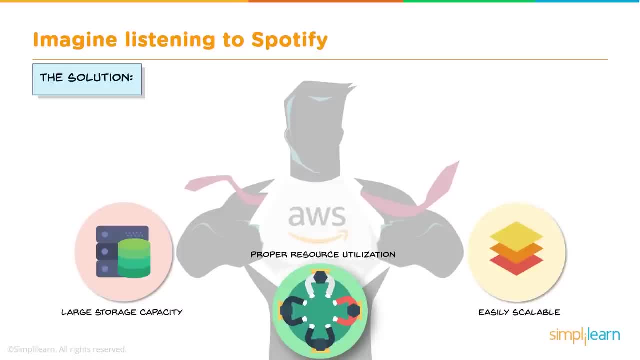 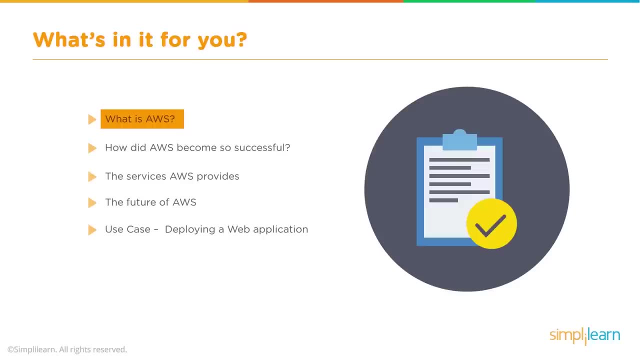 It's just a few button clicks And AWS solved Spotify's problem. Let's talk about how it can help you with your organization's problem. Let's talk about what is AWS first, And then let's bleed into how AWS became so successful and the different types of services. 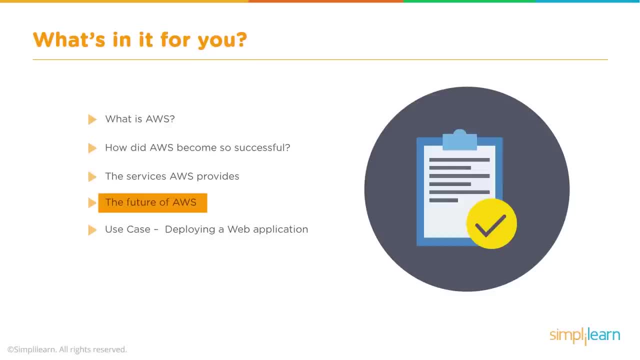 that AWS provides, And what's the future of cloud and AWS in specific. Let's talk about that. And finally, we'll talk about a use case where you will see how easy it is to create a web application with AWS. All right. 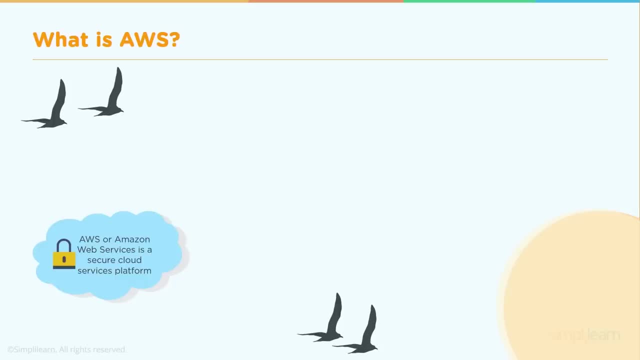 Let's talk about what is AWS. AWS, or Amazon Web Services, is a secure cloud service platform. It is also pay as you go type billing model, where there is no upfront or capital costs. We'll talk about how soon the service will be available. 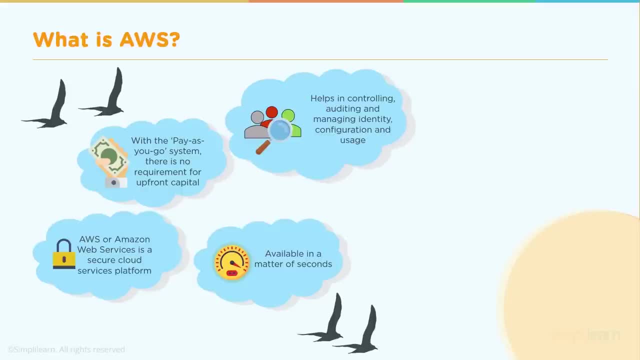 Well, the service will be available in a matter of seconds. With AWS you can also do identity and access management, that is, authenticating and authorizing a user or a program on the fly. Most all the services are available on demand and most of them are available instantaneously. 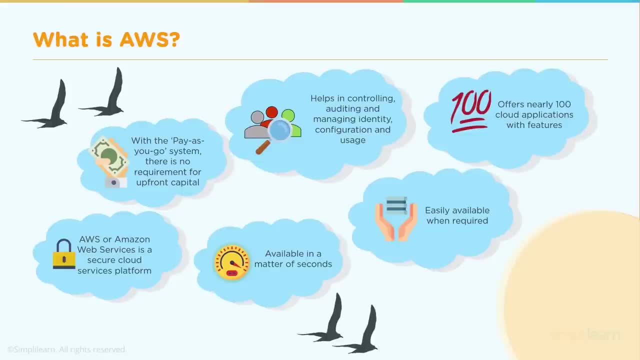 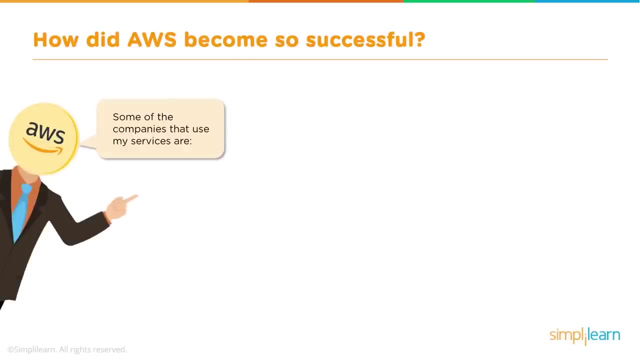 And, as we speak, Amazon offers 100 plus services, and this list is growing every new week. Now that would make you wonder how AWS became so successful. Of course it's their customers. Let's talk about the list of well-known companies that has their IT environment in AWS. 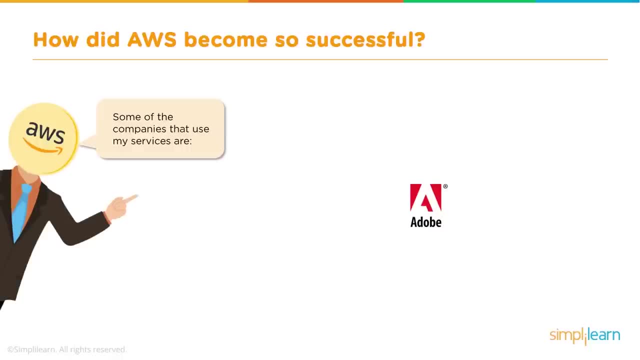 Adobe. Adobe uses AWS to provide multi terabyte operating environments for its customers. by integrating its system With AWS cloud, Adobe can focus on deploying and operating its own software instead of trying to deploy and manage the infrastructure. Airbnb is another company. It's an community marketplace that allows property owners and travelers to connect each 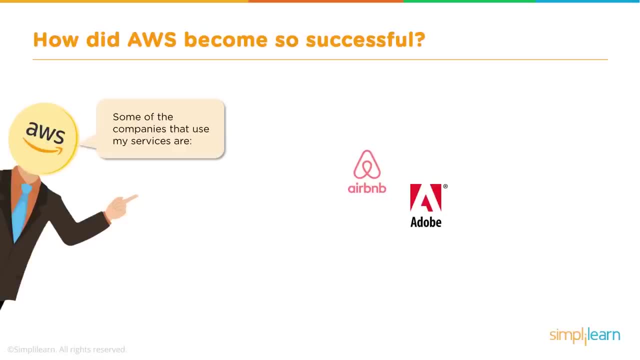 other for the purpose of renting unique vacation spaces around the world, And the Airbnb community users activities are conducted on the website and through iPhones and Android applications. Airbnb Airbnb has a huge infrastructure in AWS and they're almost using all the services in AWS and are getting benefited from it. 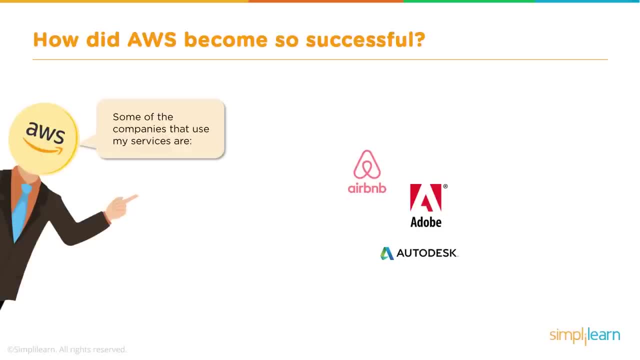 Another example would be Autodesk. Autodesk develops software for engineering, designing and entertainment industries using services like Amazon RDS, or Rational Database Service, and Amazon S3, or Amazon Simple Storage Service. Autodesk can focus on deploying or developing its machine learning tools instead of spending that time on managing the infrastructure. 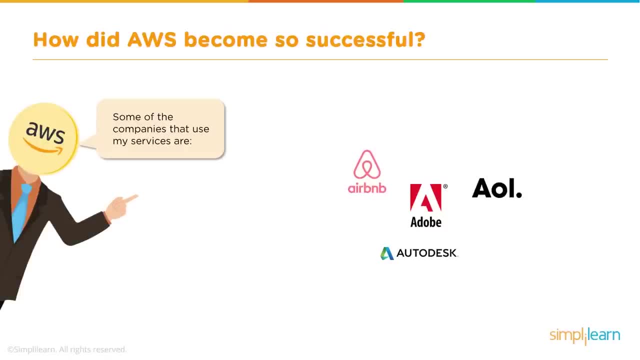 So let's talk about Autodesk. AOL, or American Online, uses AWS and using AWS, they have been able to close data centers and decommission about 14,000 in-house and co-located servers and move mission-critical workload to the cloud and extend its global reach and save millions of dollars on energy. 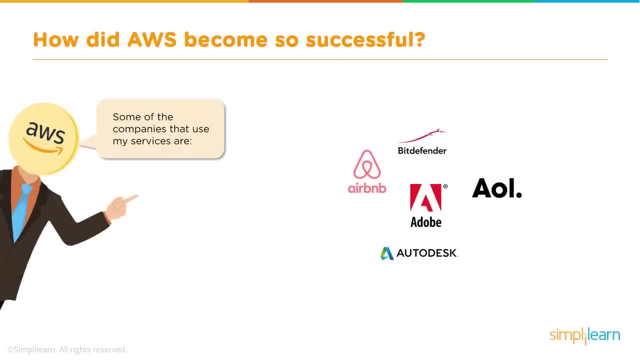 resources. Bitdefender is an internet security software firm and their portfolio of softwares include antivirus and anti-spyware products. Bitdefender uses EC2 and they are currently running few hundred instances that handle about 5 TB of data. They also use Elastic Load Balancer to load balance the connection coming in to those. 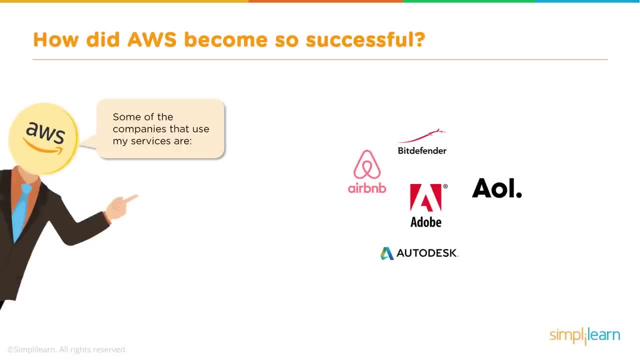 instances across availability zones, and they provide seamless global delivery of service. because of that, The BMW Group uses AWS for its new Connected Car application that collects sensor data from BMW 7 Series cars to give drivers dynamically updated map and map data. map information. canons office imaging products division benefits from faster deployment times. 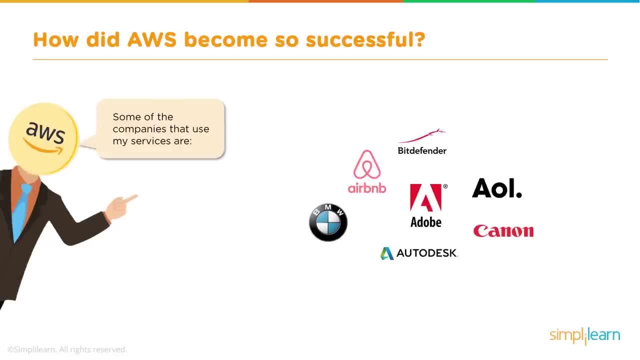 lower cost and global reach by using aws to deliver cloud-based services such as mobile print. the office imaging products division uses aws such as amazon s3 and amazon route 53, amazon cloudfront and amazon im for their testing, development and production services. comcast: it's the world's 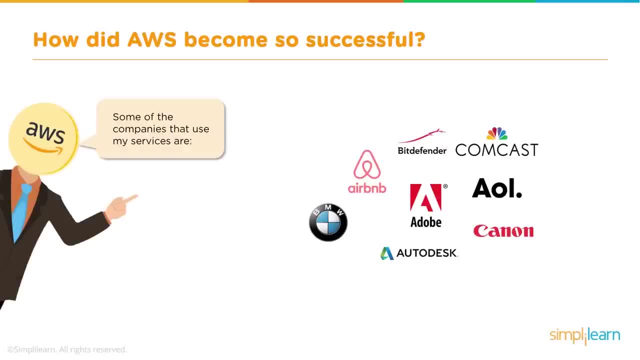 largest cable company and the leading provider of internet service in the united states, comcast uses aws in a hybrid environment. out of all the other cloud providers, comcast chose aws for its flexibility and scalable hybrid infrastructure. docker is a company that's helping redefine the way developers build, ship and run applications. this company focuses on making use of containers. 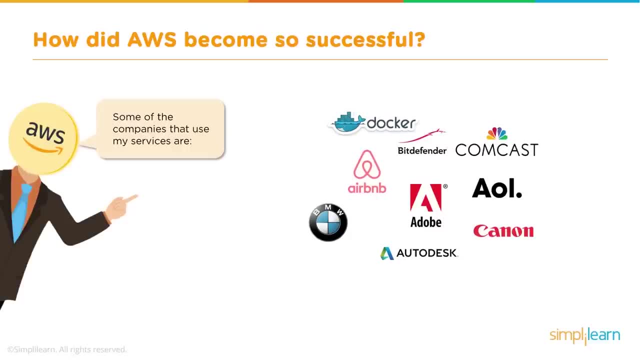 for this purpose, and in aws, the service called the amazon ec2 container service is helping companies to build and run containers for the use of containers for this purpose, and in aws, the service called the amazon ec2 container service is helping them achieve it. the esa, or european space agency, although much of esa's work is done by satellites. 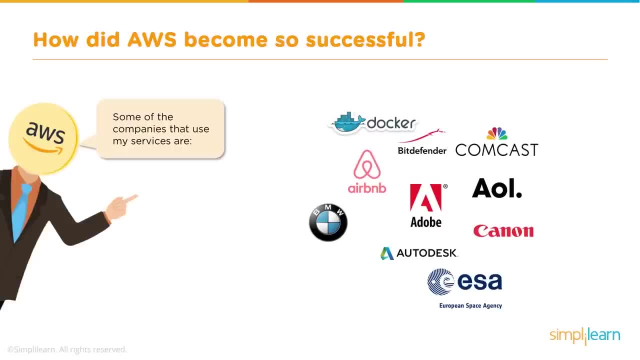 some of the program's data storage and computing infrastructure is built on amazon web services. esa chose aws because of its economical pay-as-you-go system as well as its quick startup time. the guardian newspaper uses aws and it uses a wide range of aws services, including amazon kinesis, amazon redshift, that power and analytic dashboard which editors used to see. 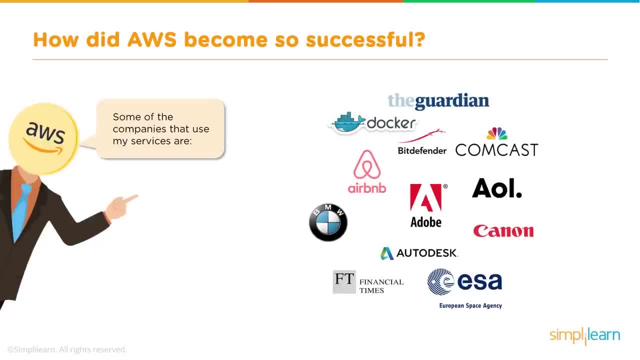 how stories are trending in real time financial times. ft is one of the world's largest leading business news organization and they used amazon redshift to perform their analysis. a funny thing happened: amazon redshift performed so quickly that some analysis thought it was malfunctioning. they were used to running queries overnight and they found that the results were indeed correct. just 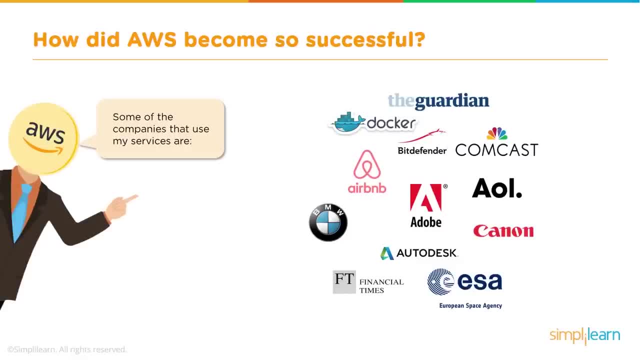 as much faster by using amazon redshift. ft is supporting the same business functions with costs that are 80 percentage lower than what was before. general electric ge is, at the moment, as we speak, migrating more than 9 000 workloads, including 300 desperate erp systems, to aws while reducing 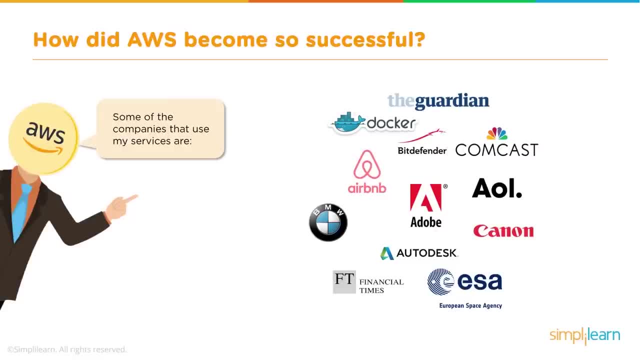 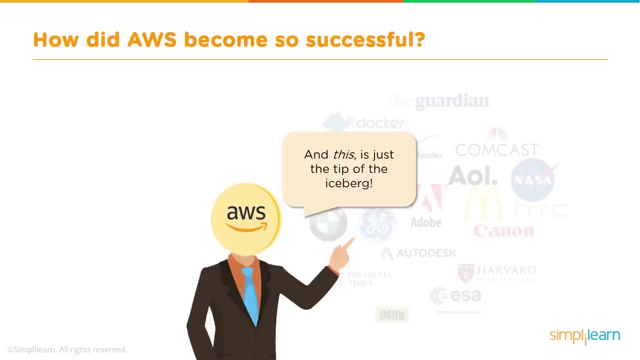 its data center footprint from 34 to 4 over the next three years. similarly, howard medical school, htc, imdb, mcdonald's, nasa, kellogg's and lot more are using the services amazon provides and are getting benefited from it. and this huge success and customer portfolio is just the tip of the iceberg. and if we think, why? 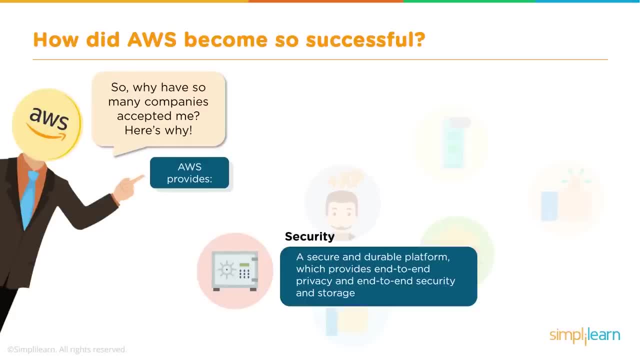 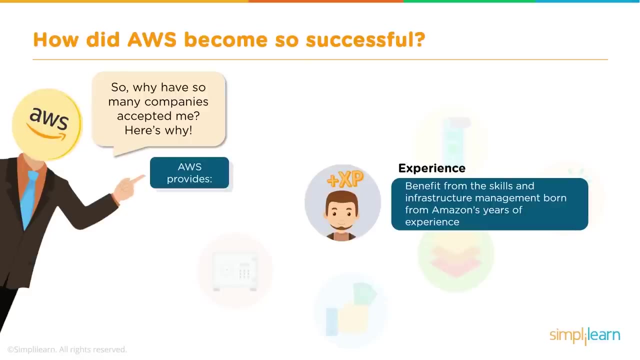 so many adapt aws and if we let aws answer that question, this is what aws would say. people are adapting aws because of the security and durability of the data and end-to-end privacy and encryption of the data and storage experience. we can also rely on aws way of doing things, by using the. 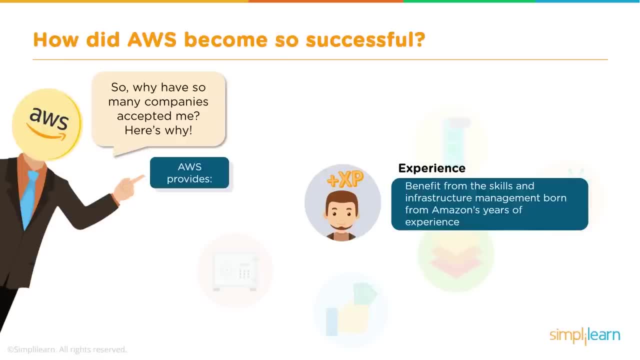 aws tools and techniques and suggested best practices. built upon the years of experience, it has gained flexibility. there is a greater flexibility in aws that allows us to select the os, language and database easy to use. swiftness in deploying: we can host our applications quickly in aws, be it a new application or migrating an existing application into aws. scalability: 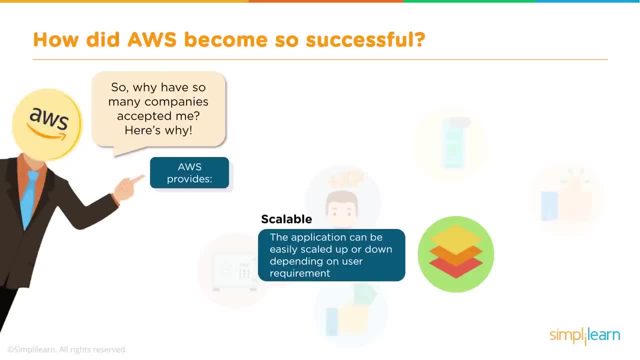 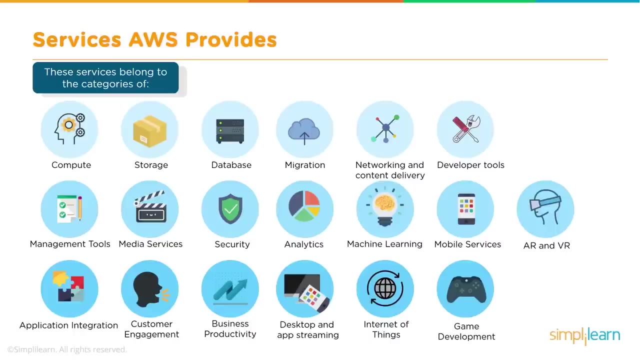 the application can be easily scaled up or scaled down, depending on the user requirement. we only pay for the compute, power, storage and other resources you use, and that, too, without any long-term commitments. now let's talk about the different types of services that aws provides. the services that we talk about fall in any of the following categories. you see, like you know, 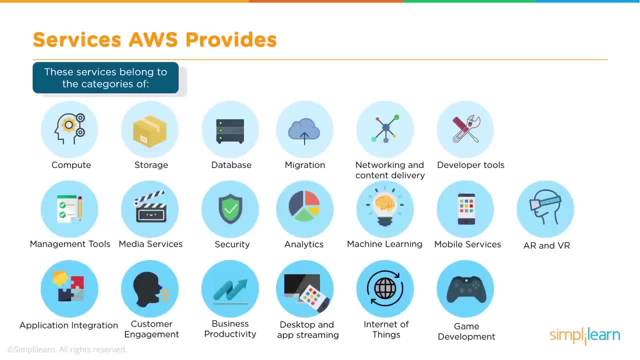 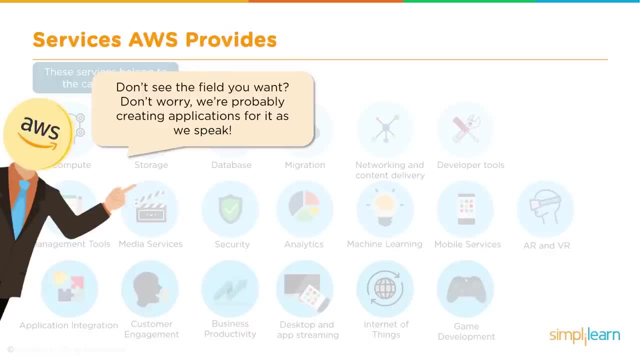 compute storage, database, security, customer engagement, desktop and streaming mission, learning, developers, tools, stuff like that, and if you do not see the service that you're looking for, it's probably is because aws is creating it as we speak. now let's look at some of them that are very commonly used within compute services we have 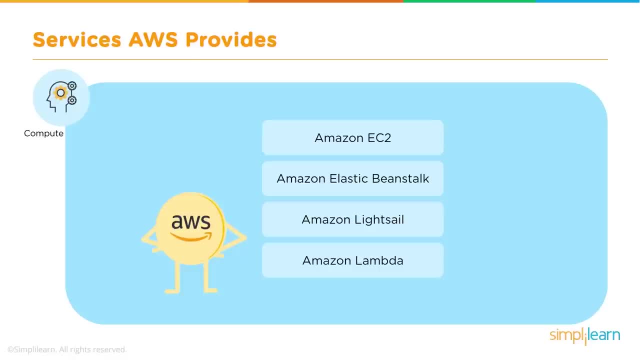 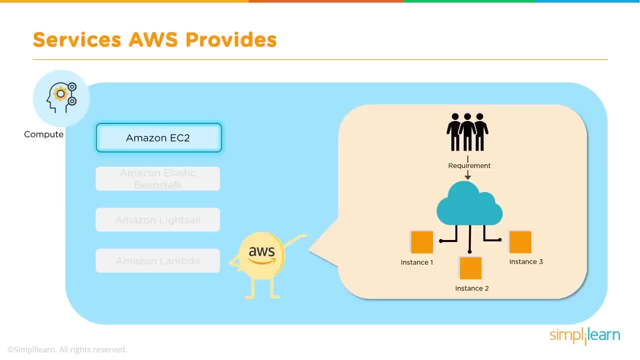 amazon ec2, amazon elastic beanstalk, amazon light sale and amazon lambda. amazon ec2 provides compute capacity in the cloud. now this capacity is secure and it is resizable based on the user's requirement. now look at this: the requirement for the web traffic keeps changing and behind the scenes, in 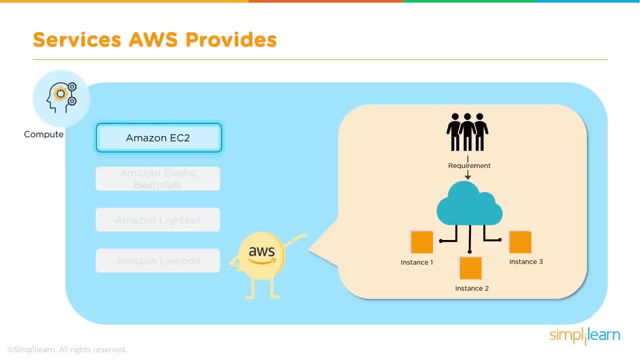 the cloud. ec2 can expand its environment to three instances and during no load it will be able to load. it can shrink its environment to just one resource: elastic beanstalk. it helps us to scale and deploy web applications and it's made with a number of programming languages. elastic beanstalk. 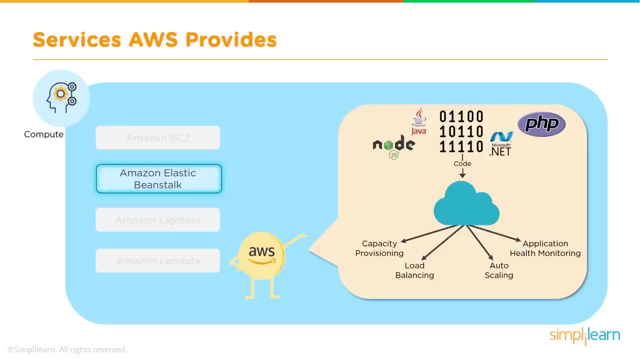 is also an easy to use service for deploying and scaling web applications and services. deployed a beat in java, dotnet, php, nodejs, python, ruby, talker and a lot of other familiar services such as apache, passenger and iis. we can simply upload our code and elastic beanstalk automatically. 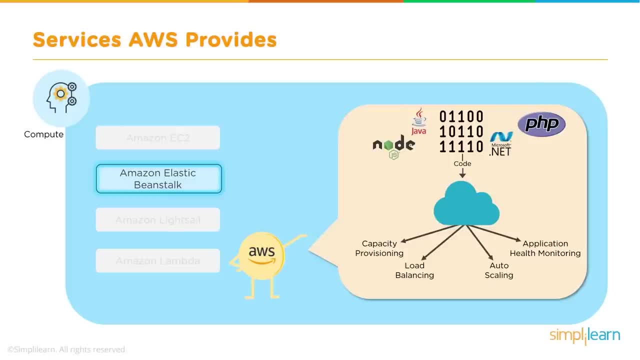 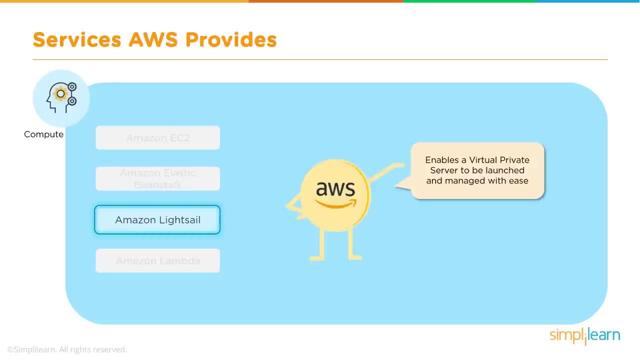 handles the deployment, from capacity provisioning to load balancing, to auto scaling, to application health monitoring. and amazon light sale is a virtual private server which is easy to launch and easy to manage. amazon light sale is the easiest way to get started with aws for developers who just need a virtual private server. light sale includes everything you need to launch your project quickly. 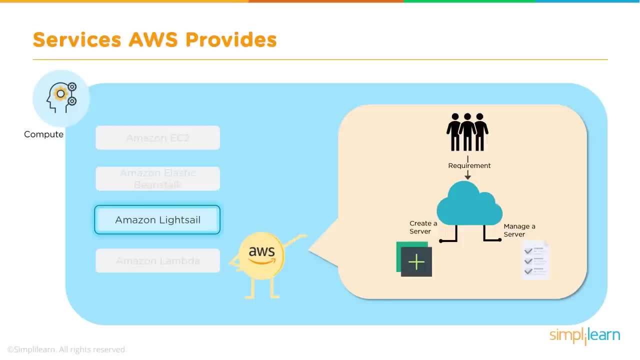 on a virtual machine, like ssd based storage, a virtual machine tools for data transfer, dns, aws lambda has taken cloud computing services to a whole new level. it allows us to pay only for the compute time, no need for provisioning and managing servers, and aws lambda is a compute service that. 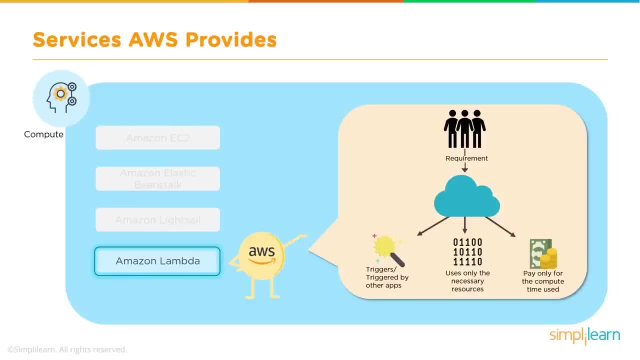 lets us run code without provisioning or managing servers. lambda executes your code only when needed and scales automatically from few requests per day to thousands per second. you pay only for the compute time you consume. there is no charge when your code is not running. let's look at the aps code. 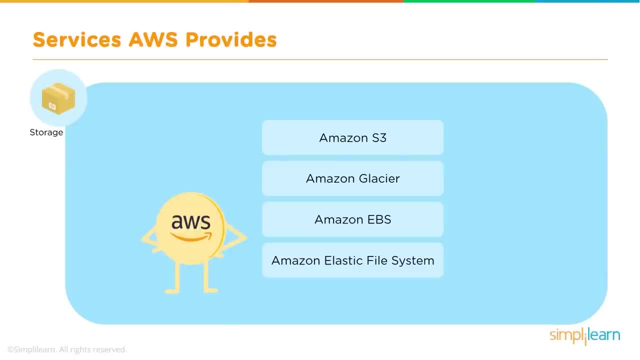 look at some storage services that Amazon provides, like Amazon S3, Amazon Glacier, Amazon EBS and Amazon Elastic File System. Amazon S3 is an object storage that can store and retrieve data from anywhere. Websites, mobile apps, IoT sensors and so on can easily use Amazon S3 to store and retrieve data. It's an 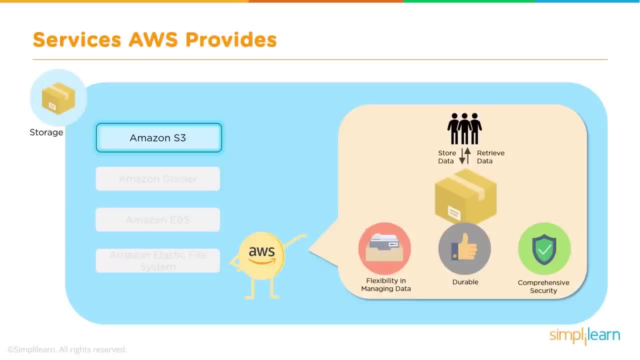 object storage built to store and retrieve any amount of data from anywhere, with its features like flexibility in managing data and the durability it provides and the security that it provides. Amazon Simple Storage Service, or S3, is a storage for the internet And Glacier Glacier is a cloud. 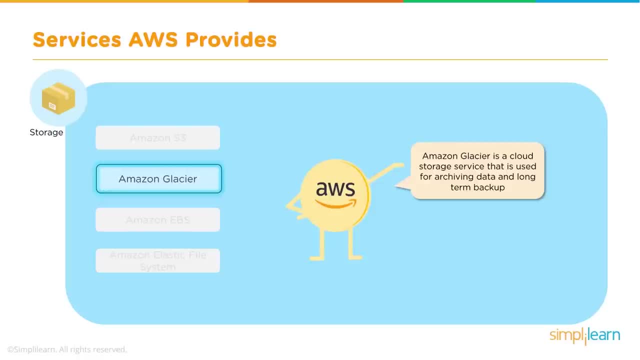 storage service that's used for archiving data and long-term backups, and this Glacier is an secure, durable and extremely low cost cloud storage service for data archiving and long term backups. Amazon EBS Amazon Elastic Block Store provides block store volumes for the instances of EC2.. And this Elastic Block Store is highly available to download as an order for further purchase. Ch preserved An upcoming difficult test. Thank you for watching. Please subscribe. if you have any doubts. You know what. there's nothing you could do about it. All right, bye, bye. 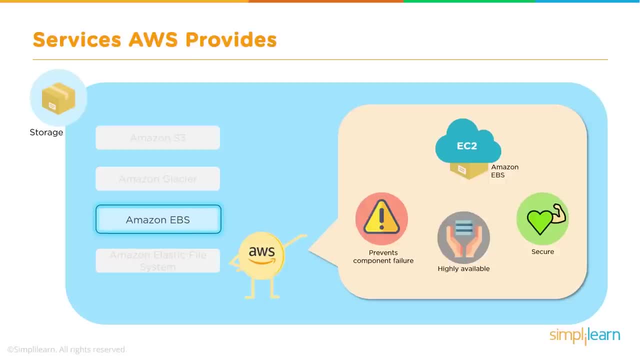 and a reliable storage volume that can be attached to any running instance that is in the same availability zone. EBS volumes that are attached to the EC2 instances are exposed as storage volumes that persist independently from the lifetime of the instance, An Amazon Elastic File System or EFS. 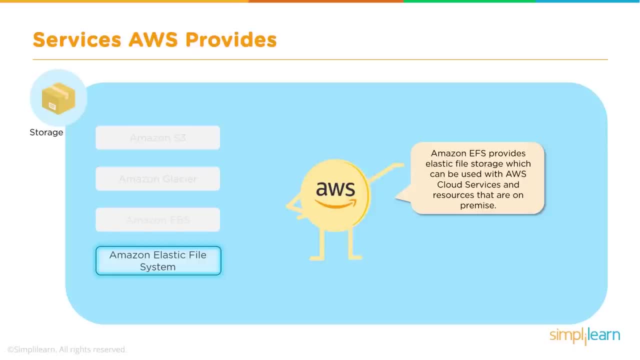 provides an elastic file storage which can be used with AWS cloud service and resources that are on-premises- An Amazon Elastic File System. it's simple, it's scalable. it's an elastic file storage for use with Amazon cloud services and for on-premises resources. It's easy to use and 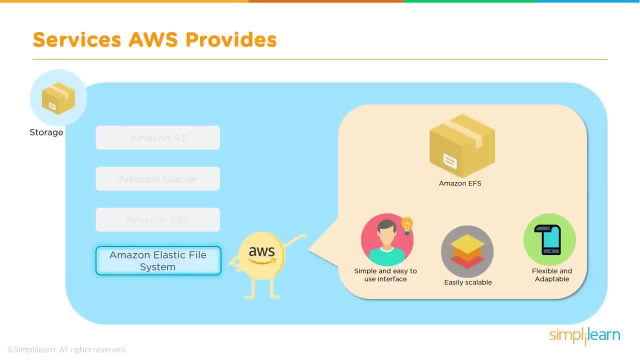 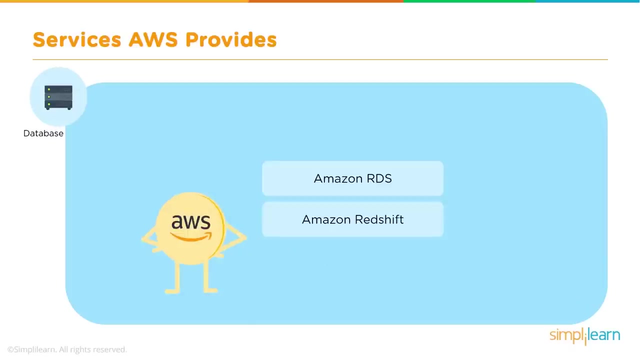 offers a simple interface that allows you to create and configure file systems quickly and easily. Amazon File System is built to elastically scale on demand without disturbing the application, growing and shrinking automatically as you add and remove files. Your application have the storage they need and when they need it. Now let's talk about databases, The two major database flavors. 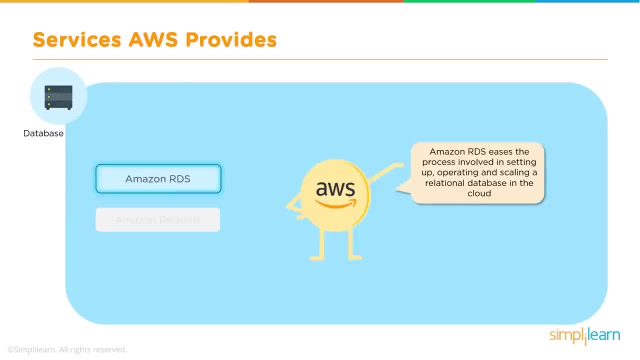 are Amazon RDS and Amazon Redshift. Amazon RDS: it provides an elastic file storage that can be used with Amazon cloud services and for on-premises. It really eases the process involved in setting up, operating and scaling a rational database in. 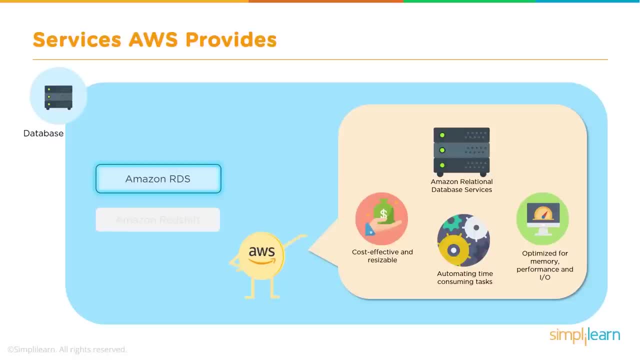 the cloud. Amazon RDS provides cost-efficient and resizable capacity while automating time-consuming administrative tasks such as hardware provisioning, database setup, patching and backups. It sort of frees us from managing the hardware and sort of helps us to focus on the application. It's also 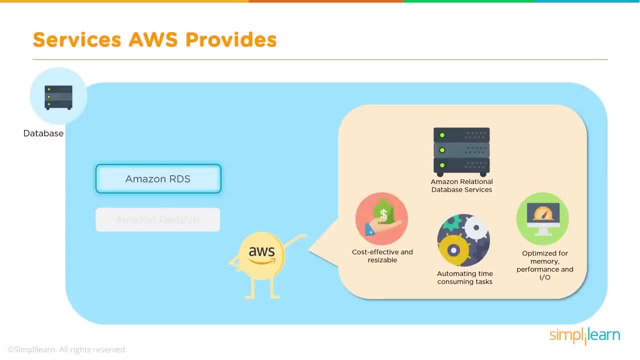 cost-effective and resizable, and it's also optimized for memory performance and input and output operations. Not only that, it's also optimized for memory performance and input and output operations. Not only that, it's also optimized for memory performance and input and output operations. Not only that, it also. 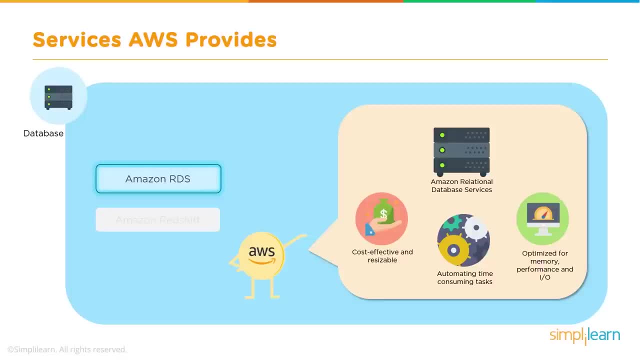 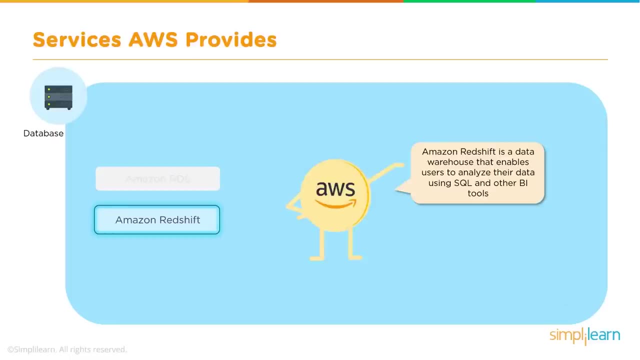 automates most of the services like taking backups, you know, monitoring stuff like that. It automates most of those services. Amazon Redshift: Amazon Redshift is a data warehousing service that enables users to analyze the data using SQL and other business intelligent tools. Amazon. 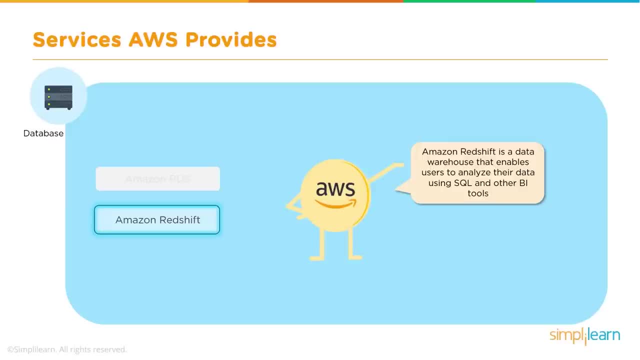 Redshift is a fast and fully managed data warehouse that makes it simple and cost-effective and lays all your data using standard SQL and your existing business intelligent tools. It also allows you to run complex data processing and data processing. It also allows you to run complex data processing. 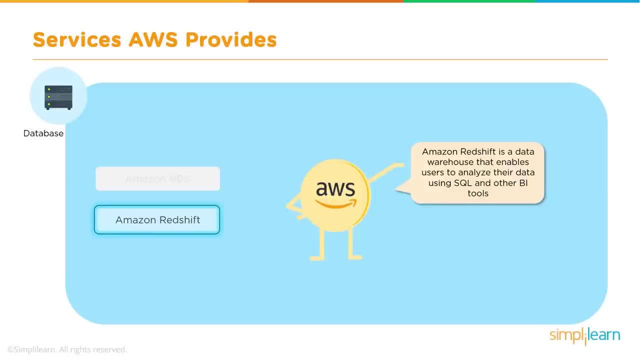 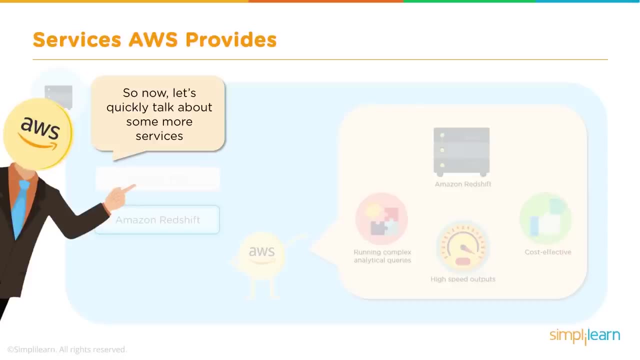 and data processing. It also allows you to run complex analytics queries against petabyte or structured data using sophisticated query optimizations, And most of the results they generally come back in seconds. All right, let's quickly talk about some more services that AWS offers. There are a lot more. 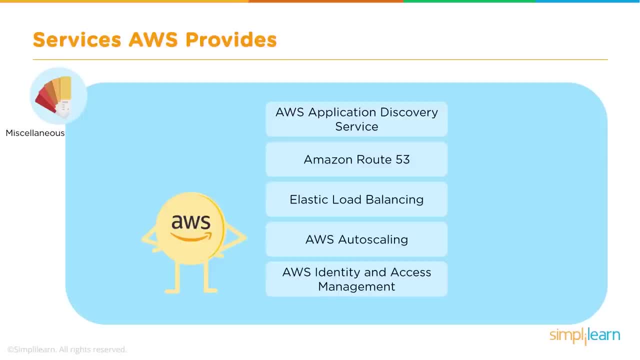 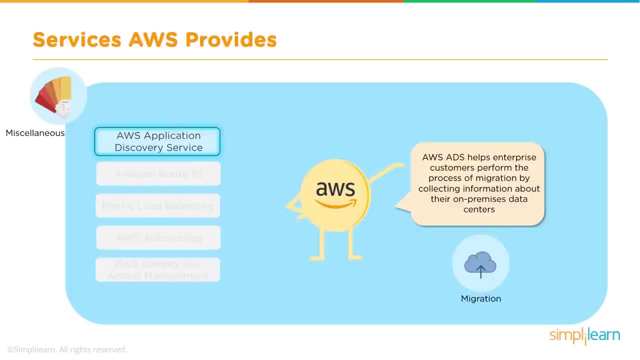 services that AWS provides, but we're going to look at some more services that are widely used. AWS application discovery services help enterprise customers plan migration projects by gathering information about their on-premises data centers. In planning a data center, migration can involve. 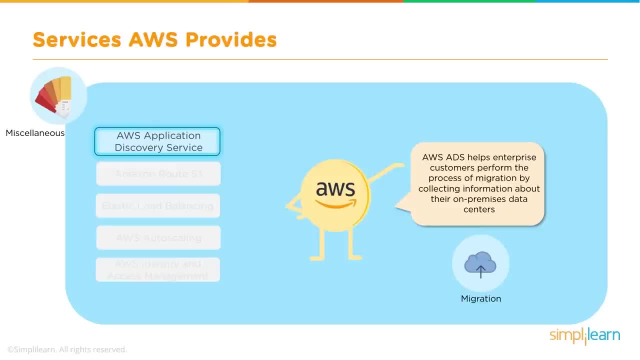 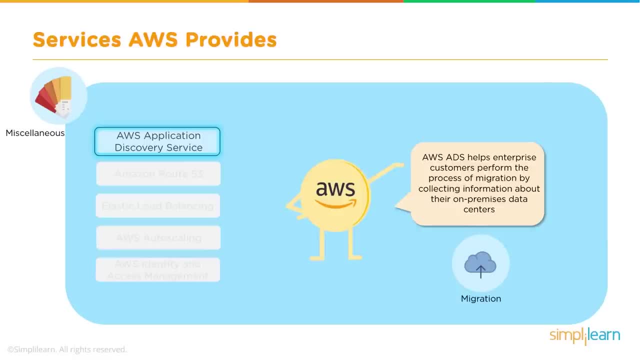 important early first step in migration process, And this AWS application discovery service collects and presents configuration, usage and behavior data from your servers to help you better understand your workloads. Route 53,: it's a network and content delivery service. It's an highly available. 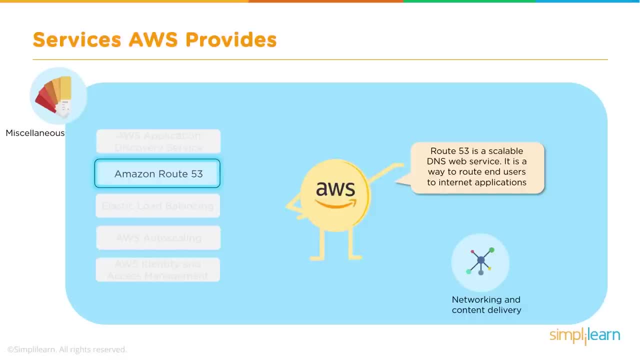 and scalable cloud domain name system or DNS service, And Amazon Route 53 is fully compliant with Route 53 as well. Elastic Load Balancing: it's also a network and content delivery service. Elastic Load Balancing automatically distributes incoming application traffic across multiple 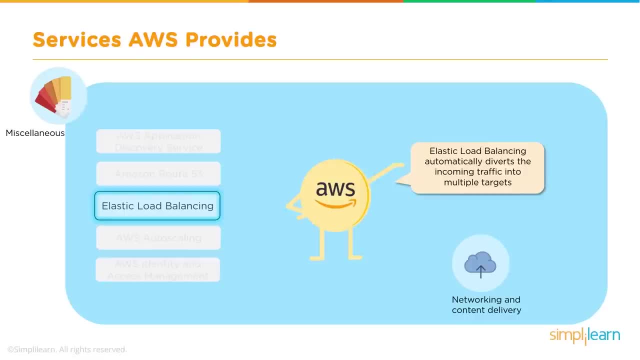 targets such as Amazon EC2 instance containers and IP addresses. It can handle the varying load of your application traffic in a single availability zone and also across availability zones. AWS Auto Scaling- it monitors your application and automatically adjusts the capacity to maintain steady and predictable performance at a lowest possible cost. 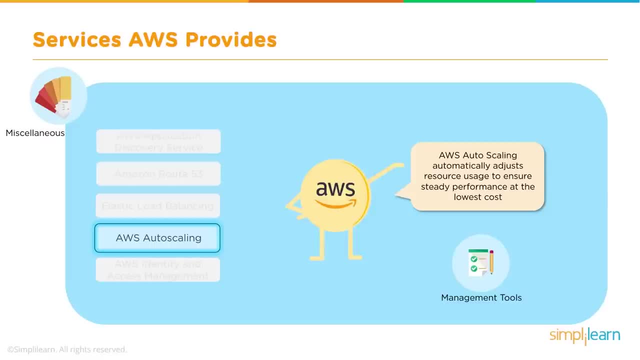 Using AWS Auto Scaling. it's easy to set up application scaling for multiple resources across multiple services in minutes. Auto Scaling can be applied to web services and also for DB services, AWS Identity and Access Management. it enables you to manage access to AWS services. 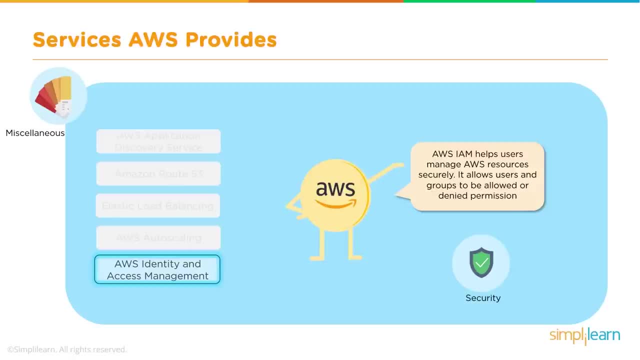 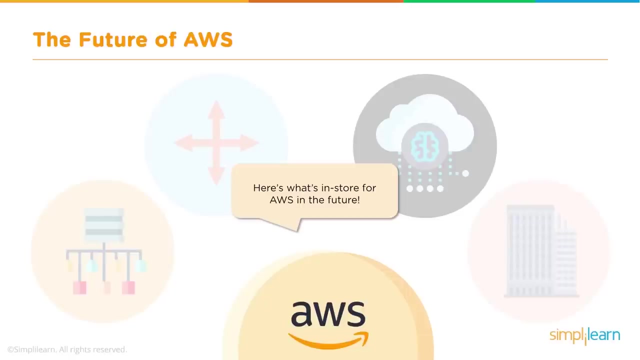 and resources securely. Using IAM, you can create and manage AWS users and groups and use permissions to allow and deny their access to AWS resources, And, moreover, it's a free service. Now let's talk about the future of AWS. Well, let me tell you something. Cloud is here to stay. Here's what's in store for AWS in the 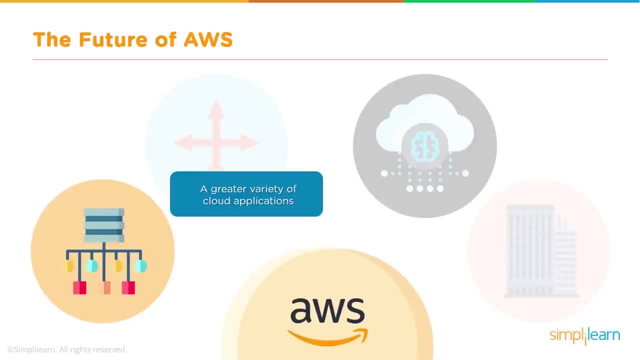 future. As years pass by, we're going to have a variety of cloud applications born like IoT, artificial intelligence, business intelligence, serverless computing and so on. Cloud will also expand into other markets like healthcare, banking, space, automated cars and so on. 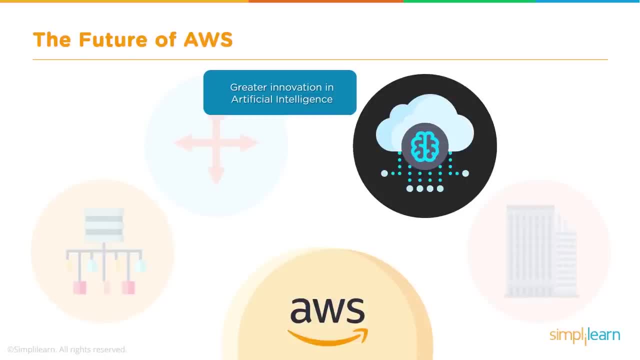 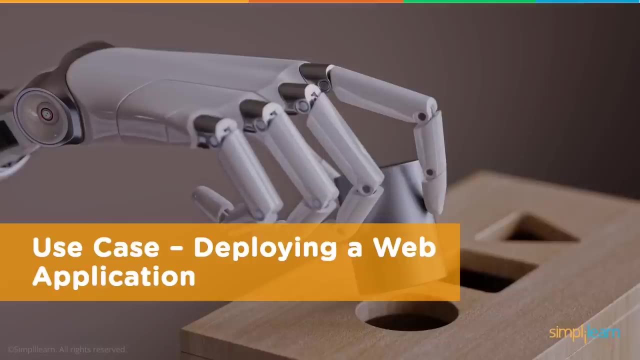 As I was mentioning some time back, a lot or greater focus will be given to artificial intelligence And eventually, because of the flexibility and advantage that cloud provides, we're going to see a lot of companies moving into the cloud. All right, let's now talk about how easy it is to deploy a web application in the 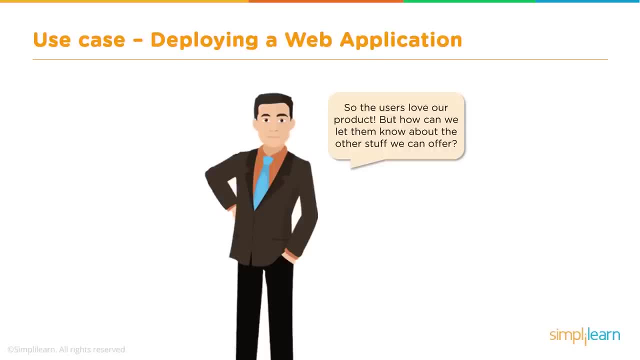 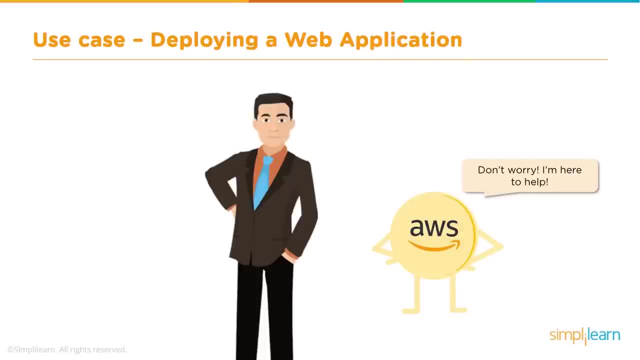 We're going to be able to do a lot of things. We're going to be able to do a lot of things. We're going to have tools and technologies which can help us to achieve it. Now we're going to use services like 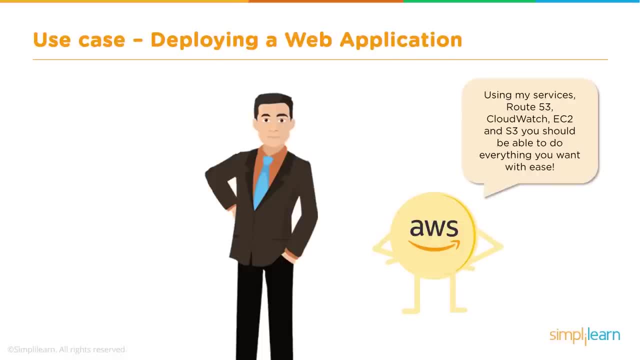 Route 53,, services like CloudWatch, EC2,, S3, and a lot more, And all these put together are going to give an application that's fully functionable and an application that's going to receive the information Like using the services like Route 53, CloudWatch, EC2, and S3, we're going to create. 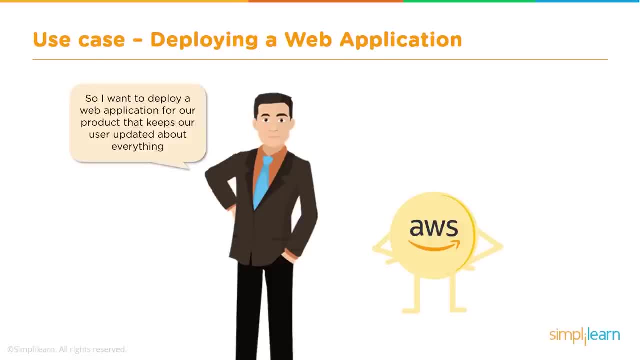 an application and that's going to meet our need. So back to our original requirement. all I want is to deploy a web application for a product that keeps our users updated about the happenings and the newcomings in the market, And to fulfill this. 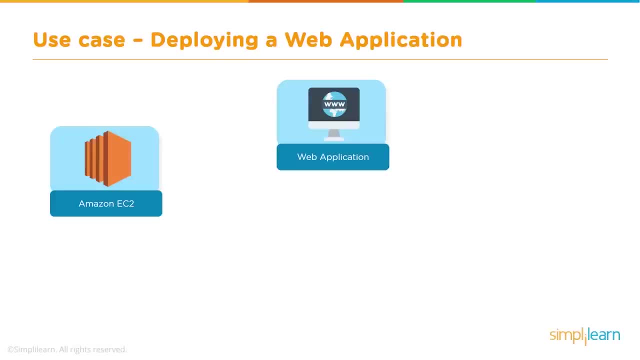 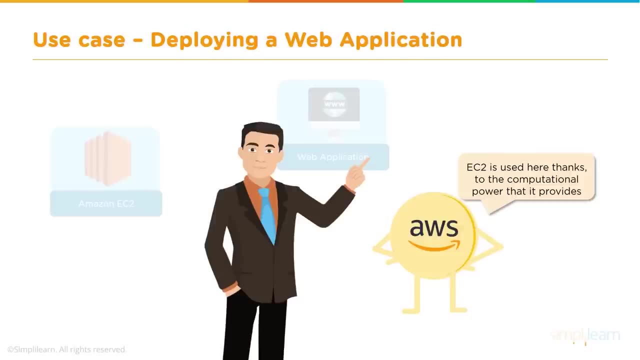 requirement. here is all the services we would need. EC2 here is used for provisioning the computational power needed for this application, And EC2 has a vast variety of family and types that we can pick from for the types of workloads and also for the intents of the workloads We're. 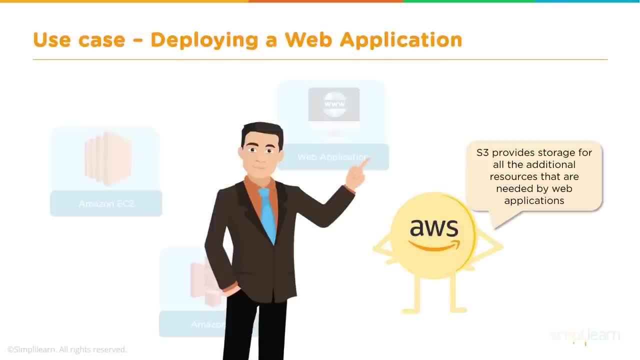 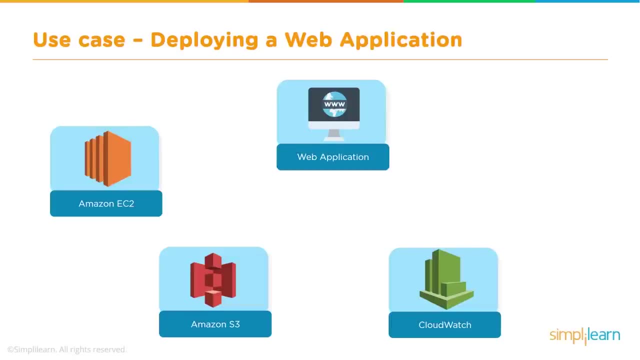 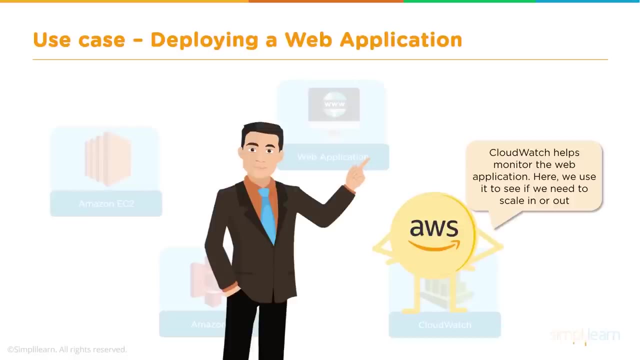 also going to use S3 for storage And S3 provides any additional storage requirement for the web applications. And we're also going to use CloudWatch for monitoring the environment, And CloudWatch monitors the application and the environment and it provides trigger for scaling. 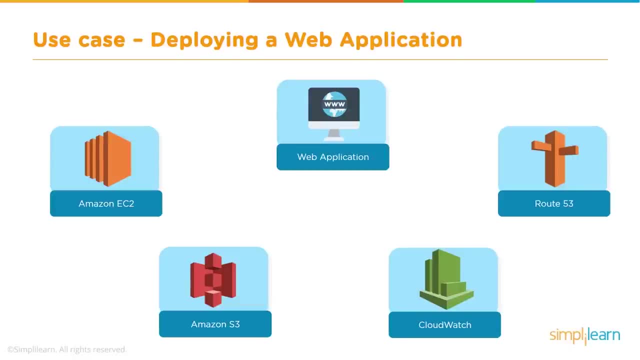 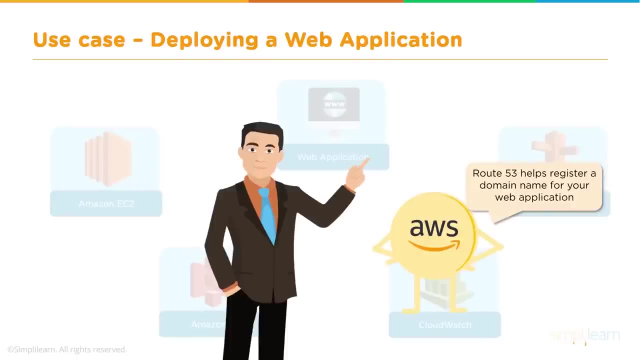 in and scaling out the infrastructure, And we're also going to use Route 53 for DNS, And Route 53 helps us to register the domain name for our web application. And with all the tools and technologies together, all of them put together, we're going to make an application a perfect. 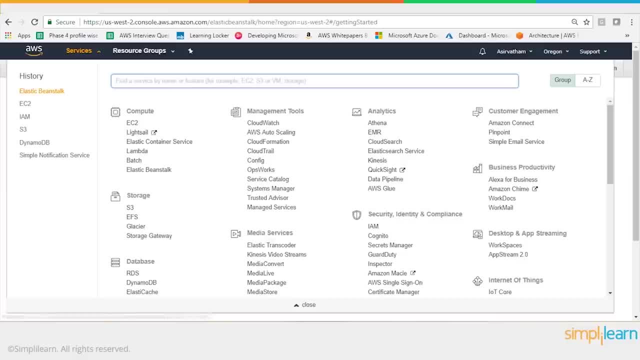 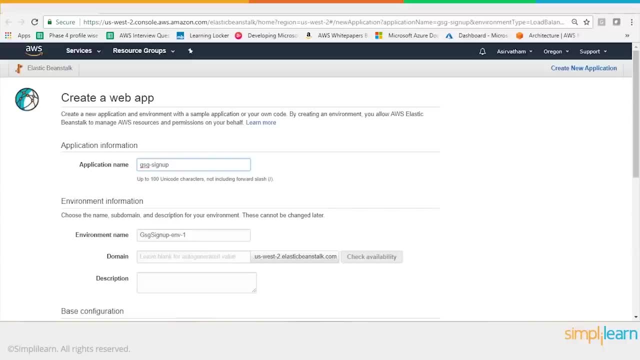 application that caters our need. All right, so I'm going to go ahead and show you how we're going to use Elastic Beanstalk for this project, And the name of the application is going to be, as you see, GSG signup, And the environment name is GSG signup, environment one. Let me also pick a name. Let me 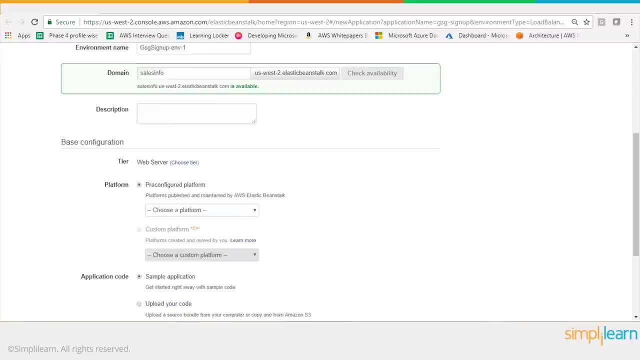 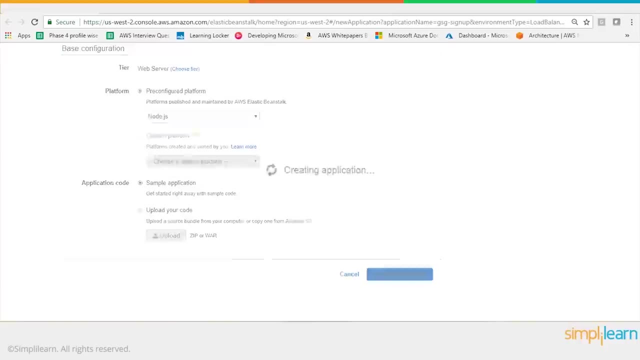 see if this name is available. Yes, that's available. That's the domain name, So let me pick that. And the application that I have is going to run on Nodejs, So let me pick that platform and launch Now, as you see, Elastic Beanstalk, this is going to launch an instance. it's going to launch. 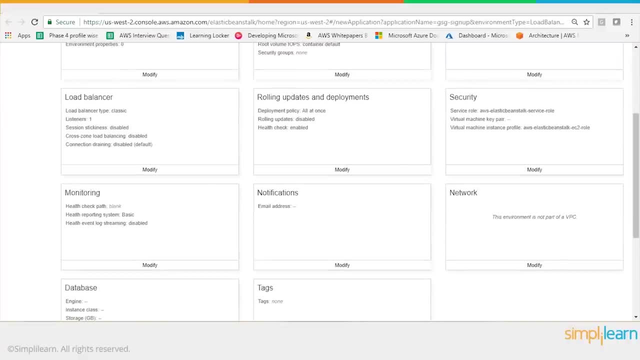 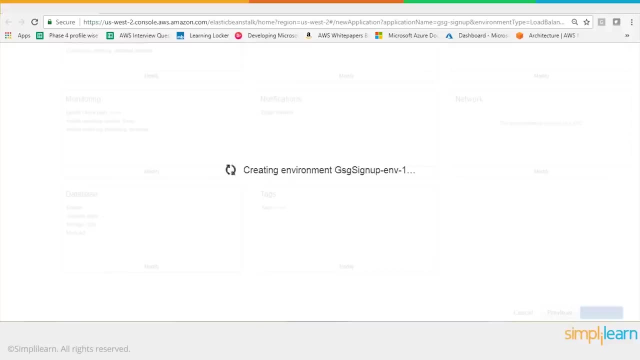 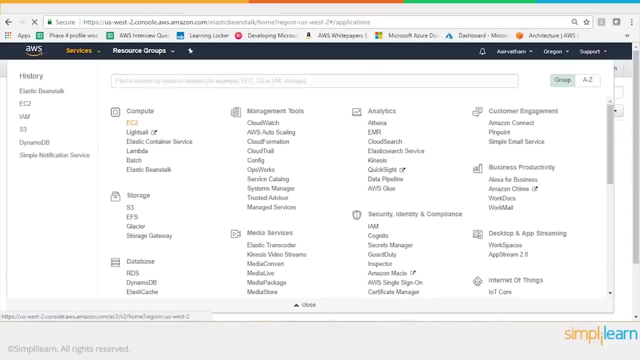 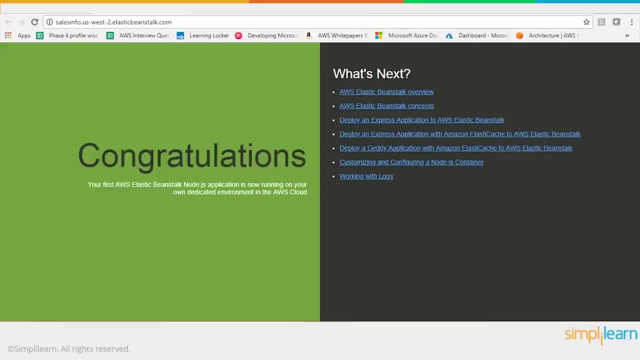 here And it's going to take care of the monitoring setup or the monitoring environment. it's going to create a load balancer as well, And it's going to take care of all the security features needed for this application. All right, look at that. I was able to go to that URL, which is what we gave, and it's now having. 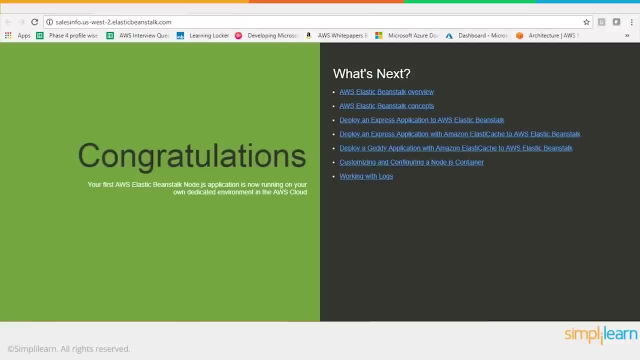 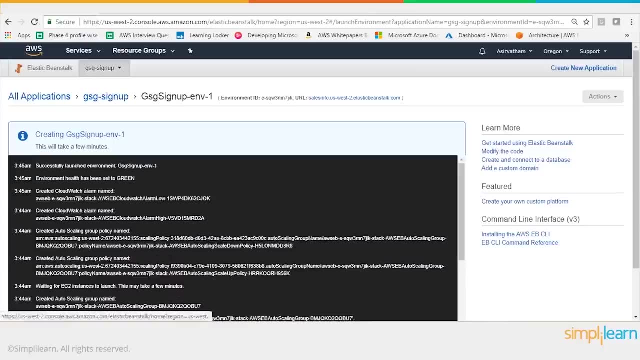 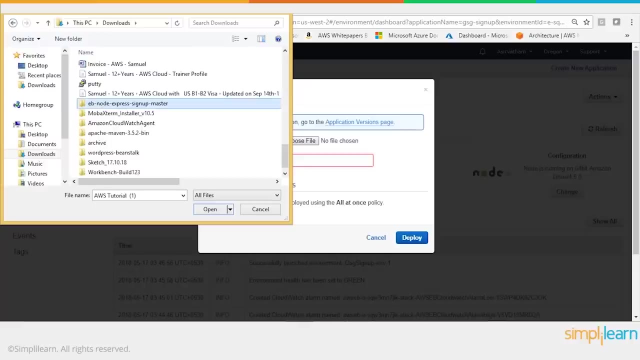 an default page shown up, meaning all the dependencies for the software is installed And it's just waiting for me to upload the code or, in specific, the page required. So let's do that. Let me upload the code. I already have the code saved here. That's my code And that's going to. 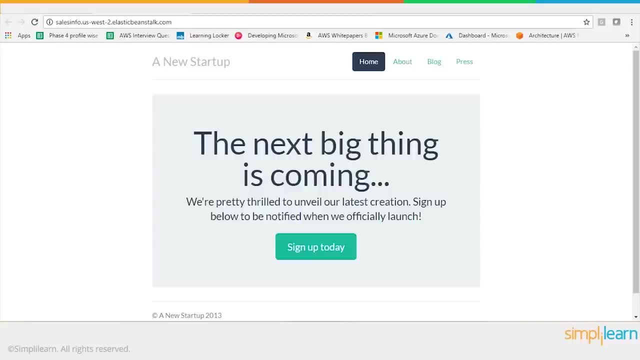 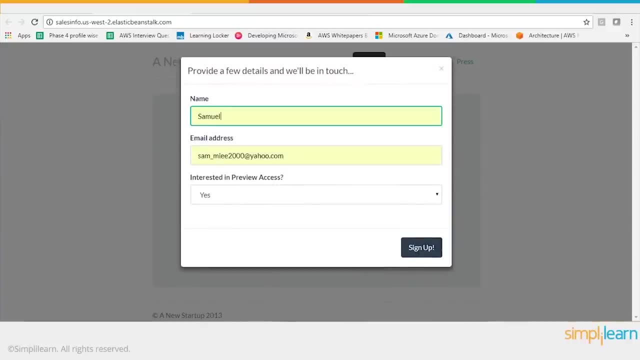 take some time. All right, it has done its thing. And now if I go to the same URL, look at that, I'm being thrown an advertisement page. All right, If I sign up with my name, email and stuff like that, you know it's going to receive the. 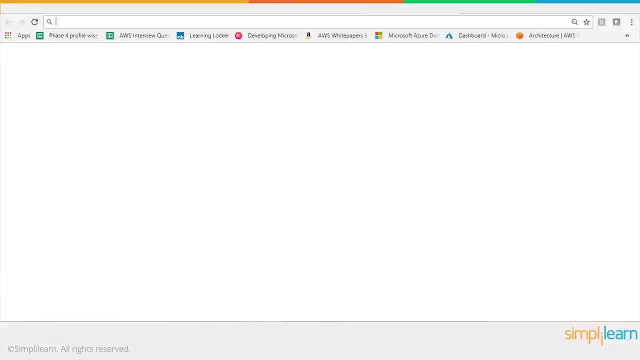 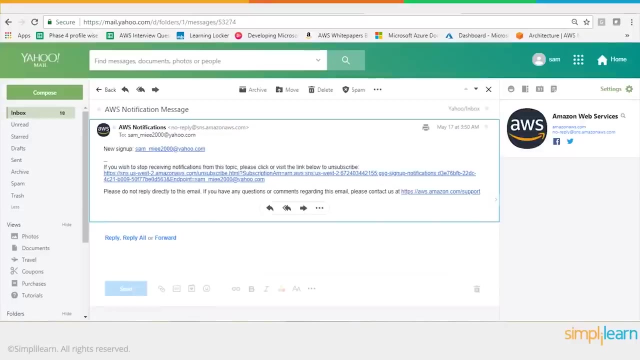 information And it's going to send an email to the owner saying that somebody had subscribed to your service. That's the default feature of this app. Look at that email to the owner saying that somebody had subscribed to your app And this is their email address. stuff like that, Not only. 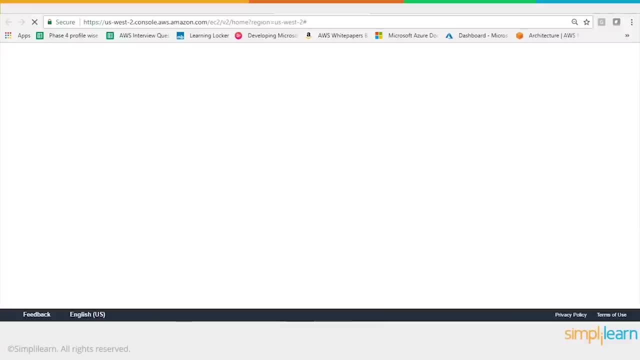 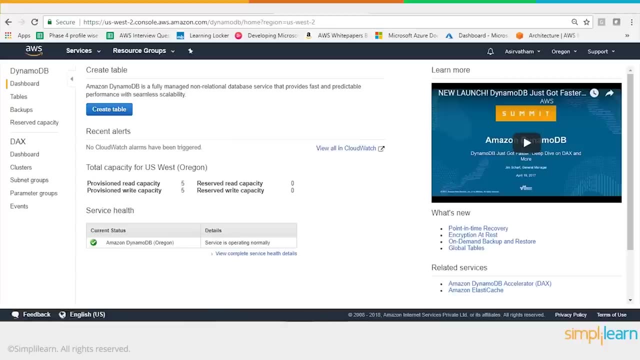 that it's also going to create an entry in the database, And DynamoDB is the service that this application users to store data. There's my DynamoDB And if I go to tables right and go to items, I'm going to see that a user with name Samuel and email. 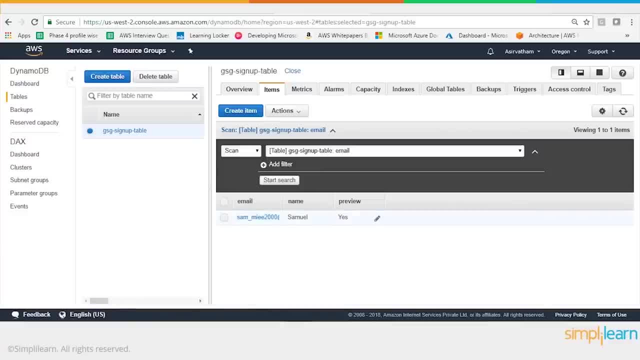 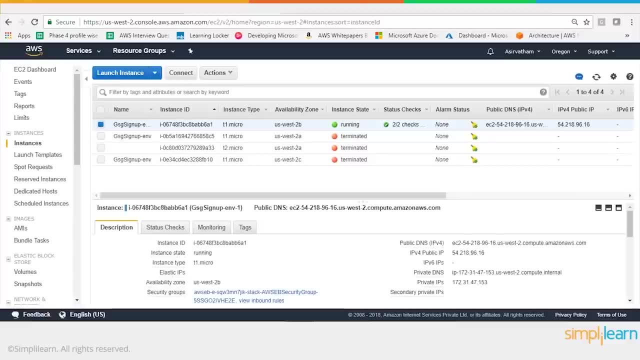 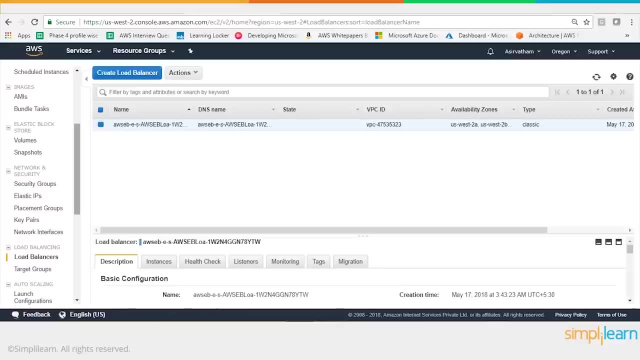 address so and so, has said okay or has shown interest in the preview of my site or product. So this is where this is how I collect those information right And some more things about the infrastructure itself is it is running behind and load balancer? Look at that. it had created a load. 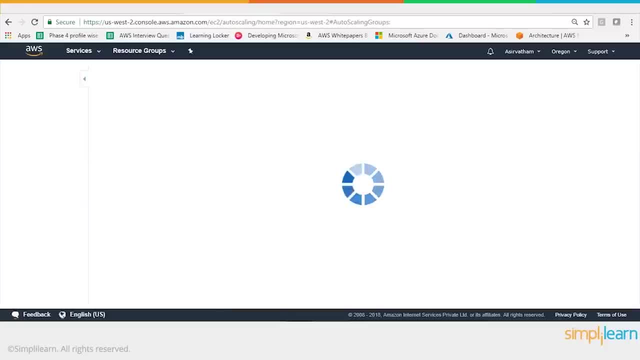 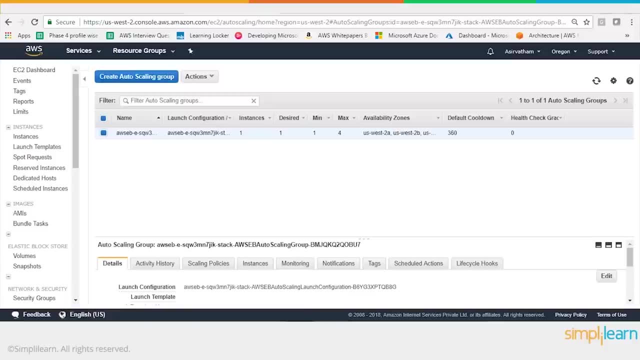 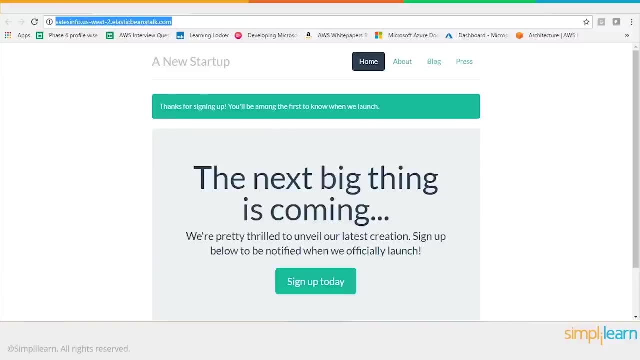 balancer, it had also created an auto scaling group. Now that's the feature of elastic load balance, So that we have chosen. it has created an auto scaling group And now let's put this URL. you see, this it's. it's not a fancy URL, right? It's an Amazon given URL, a dynamic URL. So let's put this URL behind our DNS. 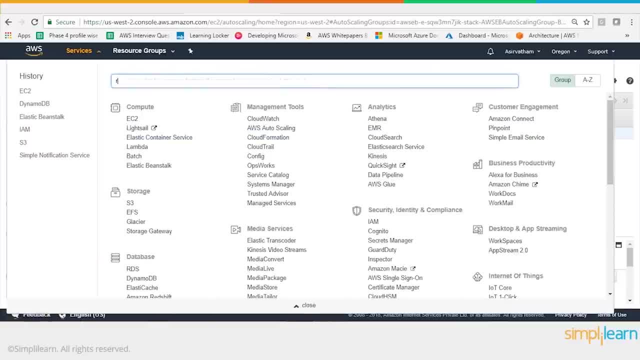 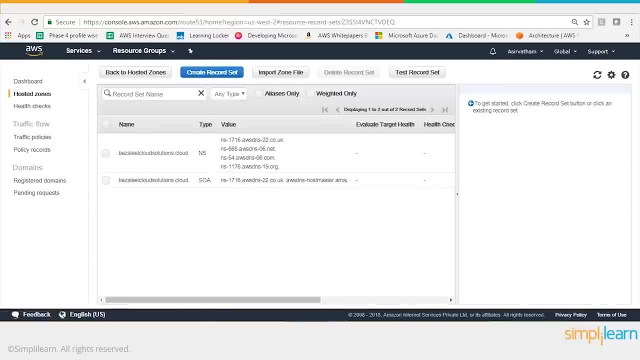 Let's do that. So go to services, go to Route 53. Go to hosted zone and there we can find the DNS name. right, So that's a DNS name, Alright. Alright, entry and map that URL to our load balancer right and create now. 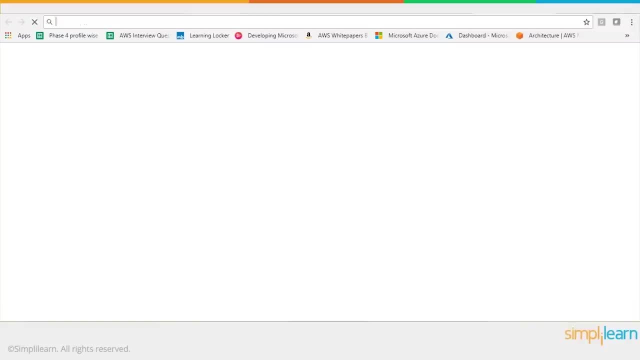 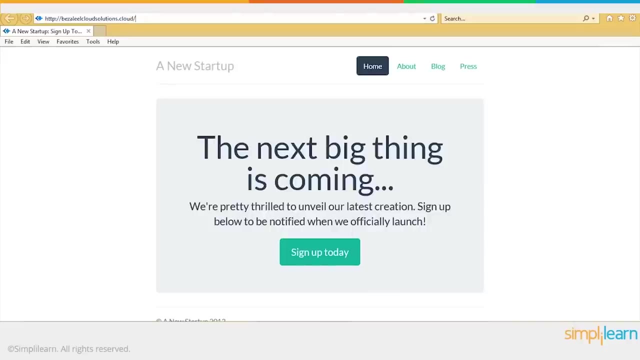 technically, if I go to this URL, it should take me to that application. all right, look at that. I went to my custom URL and now that's pointed to my application. previously, my application was having a random URL and now it's having a custom URL. so what did we learn? we started the session with what is a 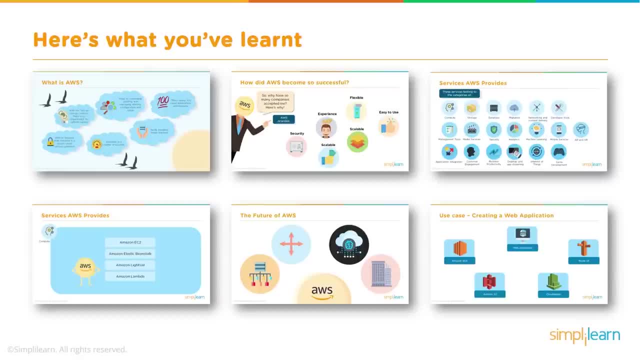 WS. we looked at features and tools, technologies, products that it of Lewis provides, and we also looked at the how AWS became very successful. again, we looked into the benefits and features of AWS in depth and we also looked at some of the services that AWS provides in random, and then we picked particular. 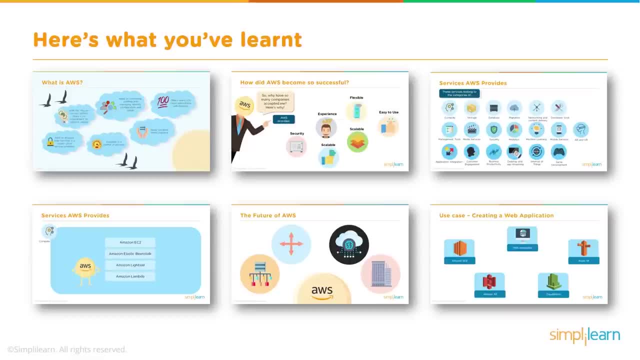 services and we talked about them like easy to elastic beanstalk, light sail, blamva, storage stuff like that. then we also looked at the future of AWS: what AWS holds in you, the store for us. we looked at that. and then, finally, we looked at a lab in which 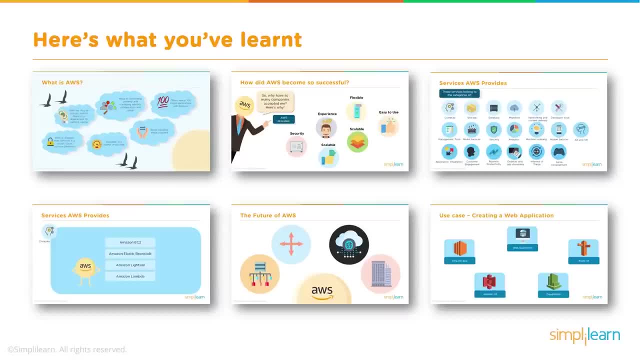 we created an application using elastic beanstalk and all that we had to do was a couple of clicks and boom: an application was there available that was connected to the database and that was connected to the simple notification system. that was connected to cloud watch, that was connected to storage stuff like. 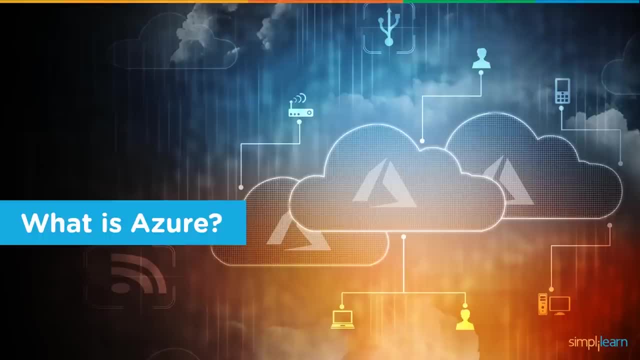 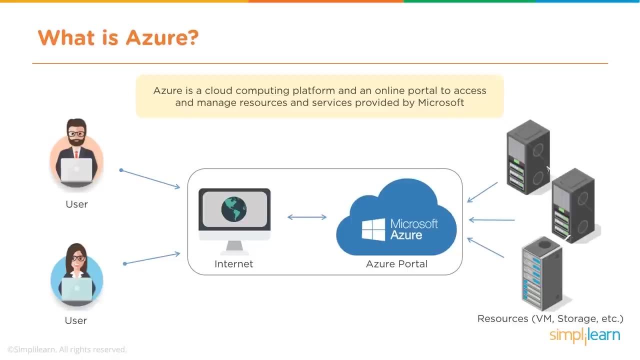 that? what is Azure? what's the big cloud service provider all about? so, as here is a cloud computing platform provided by Microsoft, now it's basically an online portal through which you can access and manage resources and services. now, resources and services are nothing, but you know you can store your data and you. 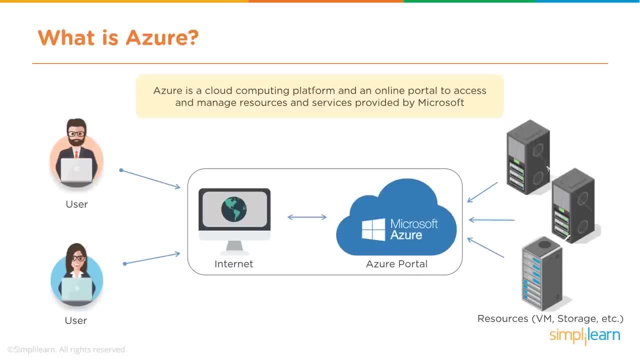 can transform the data using services that Microsoft provides. again, all you need is the internet and being able to connect to the Azure portal. then you get access to all of the resources and their services. in case you want to know more about how it's different from its rival, which is AWS, I suggest you click on the. 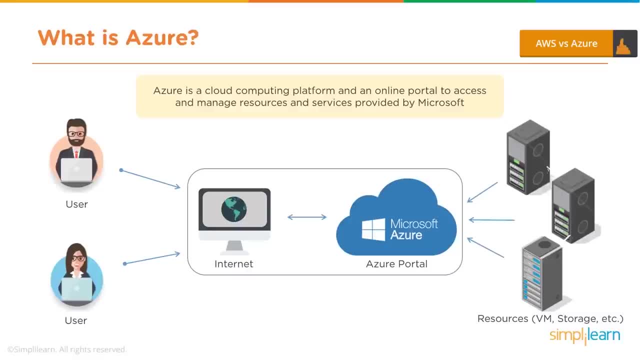 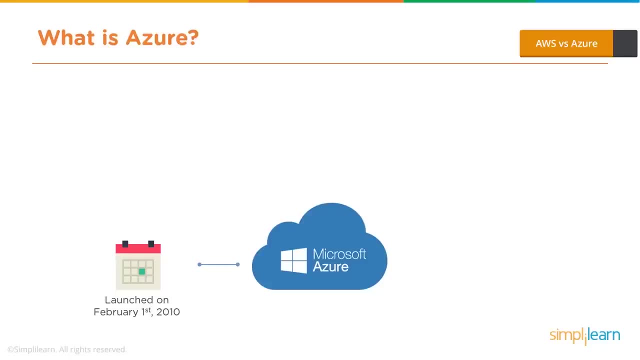 top right corner and watch the AWS versus Azure video so that you can clearly tell how both these cloud service providers are different from each other. Now here are some things that you need to know about Azure. It was launched in February 1st 2010, which is significantly later than when AWS was. 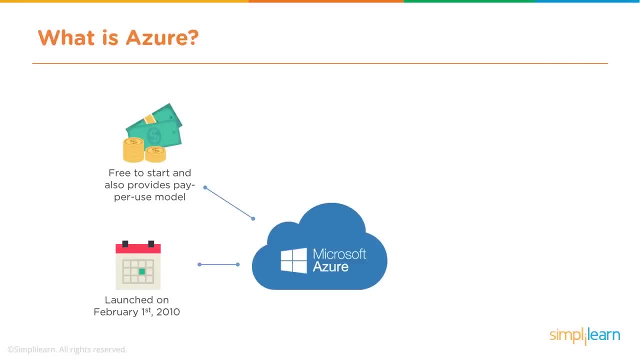 launched, It's free to start and has a pay-per-use model, which means, like I said before, you need to pay for the services you use through Azure, and one of the most important selling points is that 80% of fortune 500 companies use Azure services, which means that most of the bigger companies of the world. 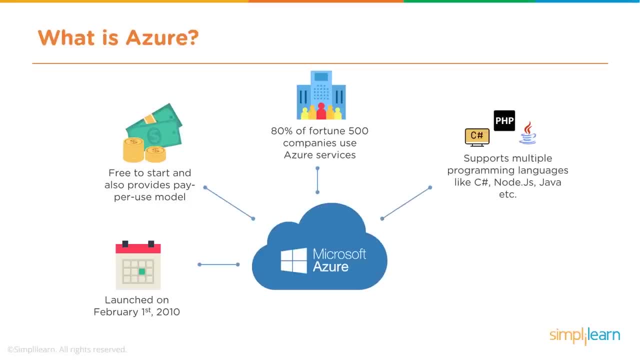 actually recommend using Azure. and then Azure supports a wide variety of programming languages: the c-sharp, no gist, Java and so much more. Another very important selling point of Azure is the amount of data centers it has across the world. Now it's important for a cloud service provider to have many data. 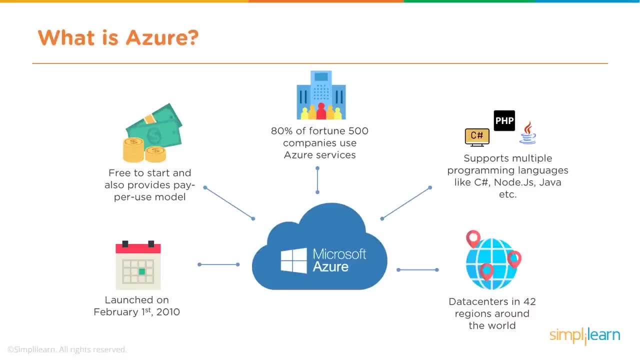 centers around the world, because it means that they can provide their services to a wider audience. Now Azure has 42, which is more than any cloud service provider has at the moment. it expects to have 12 more in a period of time, which brings its total number of regions it covers to 54. 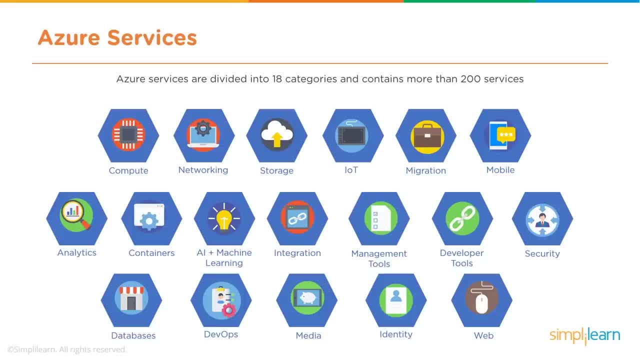 now let's talk about as your services. now, as your services have 18 categories and more than 200 services, so we clearly can't go through all of them. it has services that cover compute and machine learning, integration, management tools, identity, DevOps, web and so much more. you're going to have a hard time trying. 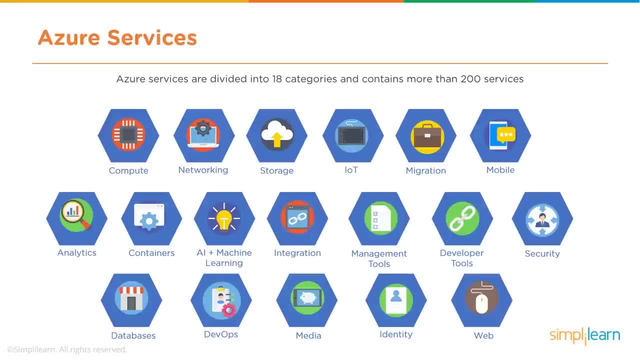 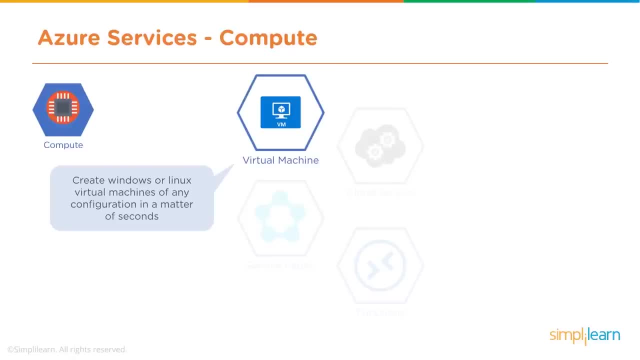 to find a domain that, as your, doesn't cover. and if it doesn't cover it now, you can be certain they're working on it as we speak. so first let's start with the compute services, first virtual machine. with this service, what you're getting to do is to create a virtual machine of Linux or Windows operating system. it's 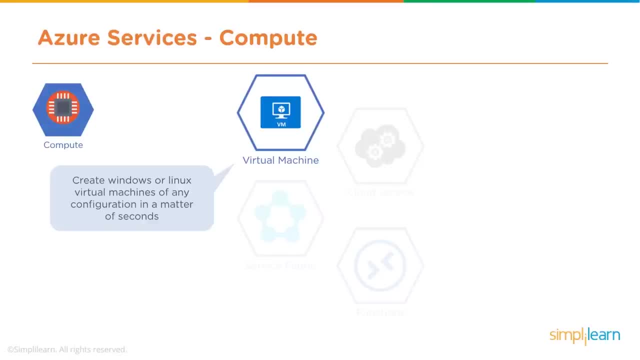 easily configurable. you can add RAM, you can decrease RAM, you can add storage, remove it. all of it is possible in a matter of seconds. now let's talk about the second service: cloud service. now, with this, you can create a application within the cloud and all of the work after you deploy it- deploying the application, that is, is taken care of. 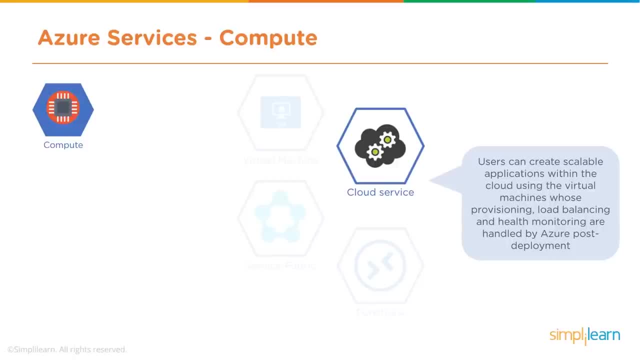 by as your, which includes, you know, provisioning the application, load balancing, ensuring that the application is in good health, and all of the other things are handled by as your next up, let's talk about service fabric. now, with service fabric, the process of developing a micro service is greatly simplified. so 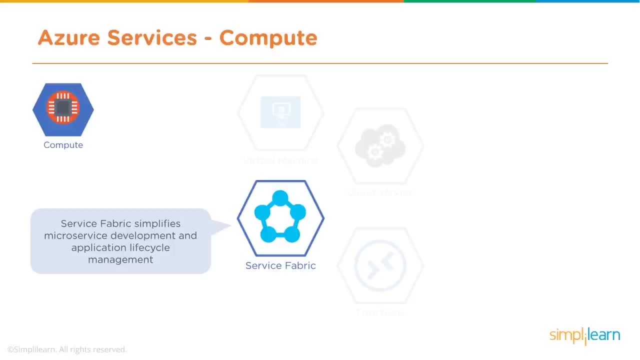 you might be wondering what exactly is a micro service. a micro service is basically an application that consists of smaller applications coupled together, next up functions. now, with functions, you can create applications in any programming language that you want. another very important part is that you don't have to worry about any hardware components. you 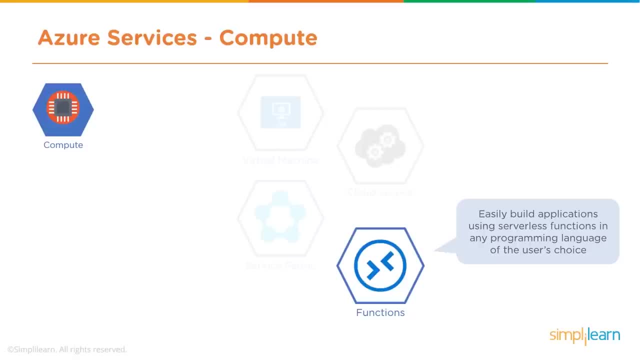 don't have to worry what RAM you require or how much storage you require. all of that is taken care of by as your. all you need is to provide the code to as your and it will execute it, and you don't have to worry about anything else. now let's. 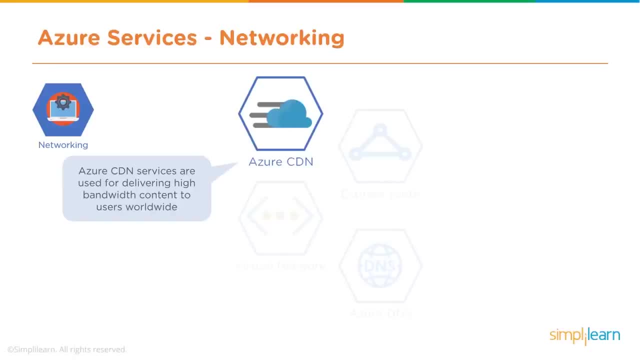 talk about some networking services. first up, we have as your CDN, or the content delivery network. now the as your CDN service is basically for delivering web content to users. now this content is of high bandwidth and can be transferred or can be delivered to any person across the world. now these are actually a 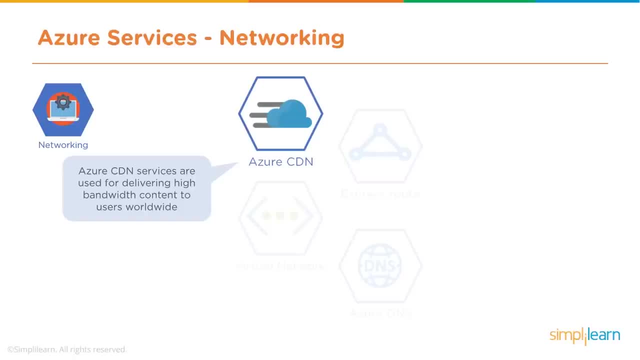 network of servers that are placed in strategic positions across the world, so that the customers can obtain this data as fast as possible. next up, we have a virtual network. now, with this, you can actually connect your on-premise network on to the Microsoft cloud or any of the services that you want through a private 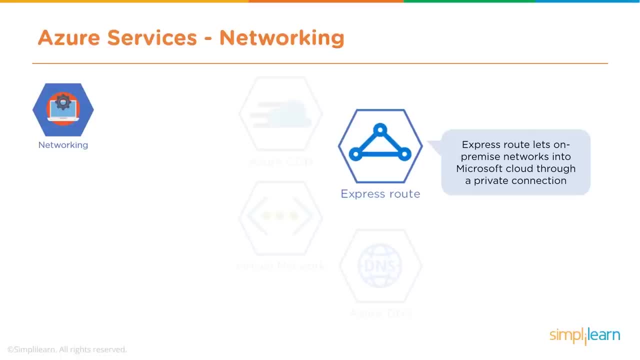 connection. so the only communication that happens is between your on-premise network and the service that you want. then you have virtual network. now, with virtual network, you can have any of the, as your services communicate with each other in a secure manner, in a private manner. next, we have as your DNS, so as 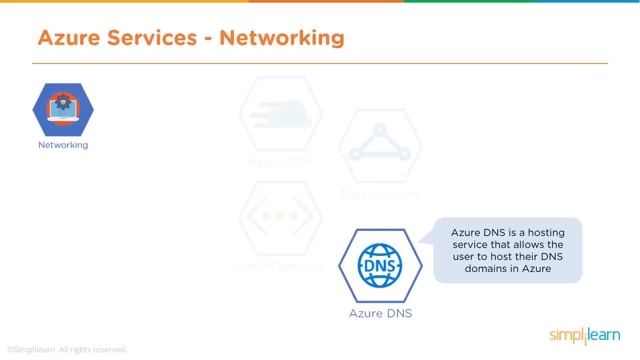 your DNS is a hosting service which allows you to host their DNS or domain system domains in as your, so you can host your application using as your DNS. now for the storage services. first up we have disk storage. with this storage, you are given a cost-effective option of choosing HDD or solid-state drives to go. 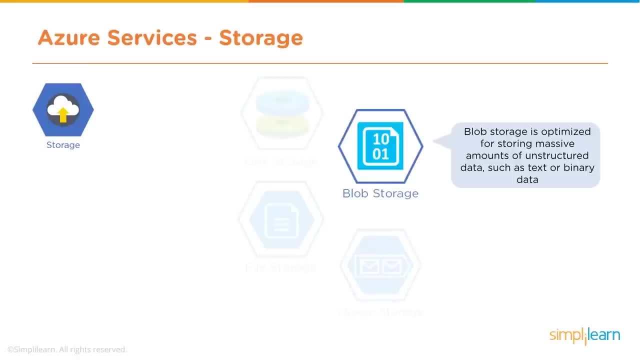 along with your virtual machines, based on your requirements. then you have blob storage. now, this is actually optimized to ensure that they can store massive amounts of unstructured data, which can include text data or even binary data. next, you have file storage, which is a managed file storage and can be accessible via the SMB protocol or 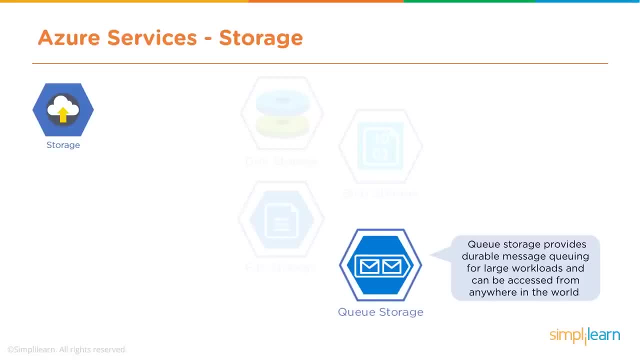 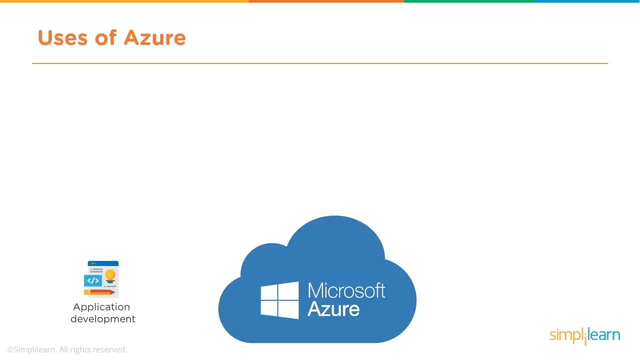 the server message block protocol and, finally, you have queue storage. now, with queue storage, you can provide durable message queuing for an extremely large workload, and the most important part is that this can be accessed from anywhere in the world. now let's talk about how as your can be used. firstly, for application. 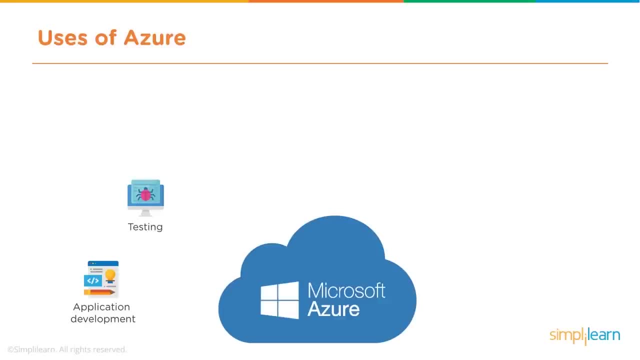 development. it could be any application, mostly web applications. then you can test the application, see how well it works. you can host the application on the internet. you can create virtual machines. like I mentioned before, with the service you can create these virtual machines of any size or RAM that you 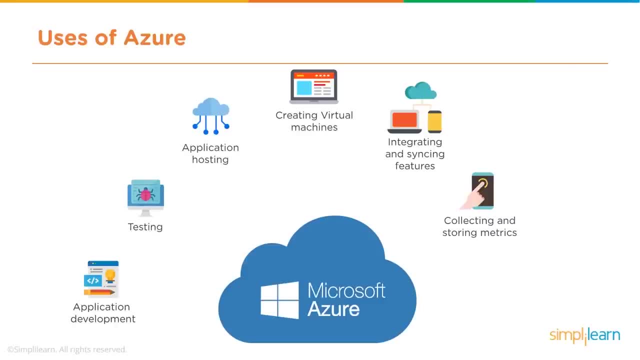 want. you can integrate and sync features. you can collect and store matrices, for example, how the data works, how the current data is, how you can improve upon it. all of that is possible with these services and your virtual hard drives, which is an extension of the virtual machines where these services are able. 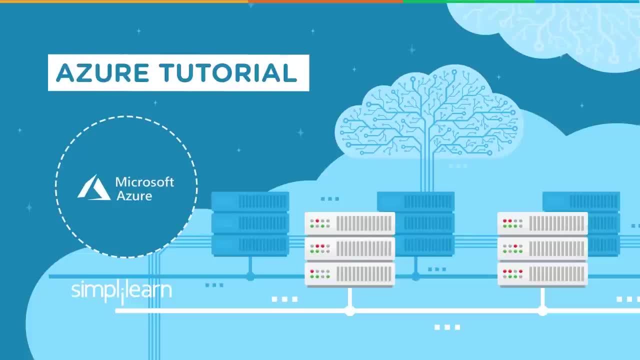 to provide you a large amount of storage where data can be stored. talk about what you are using. where are you using? your data is all through Azure in great length and breadth, and if you're looking for a video that talks and walks you through all the services in Azure, then this could be one of the best video you. 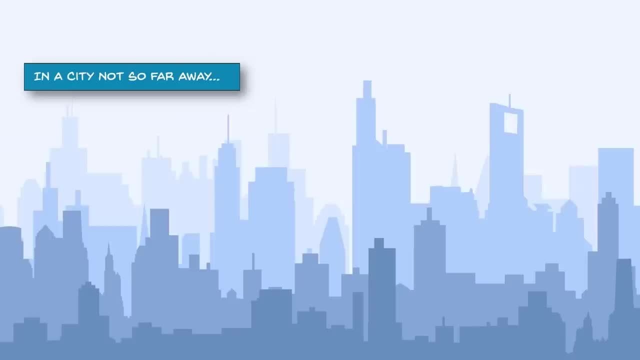 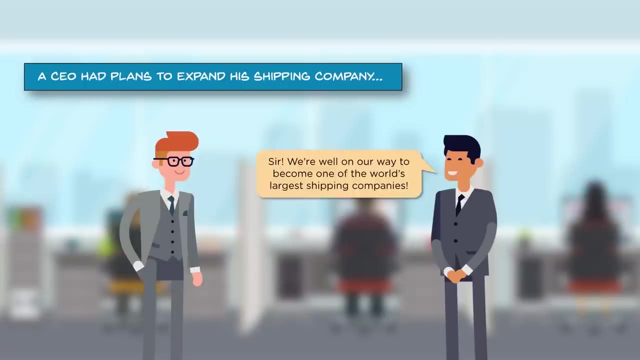 could find in the internet and, without any further delay, let's get started. everybody likes story, is it? so let's get started with a story. in a city not so far away, a CEO had plans to expand his company globally and called one of his IT personnel for an IT opinion, and this guy has been in the company for a long time. 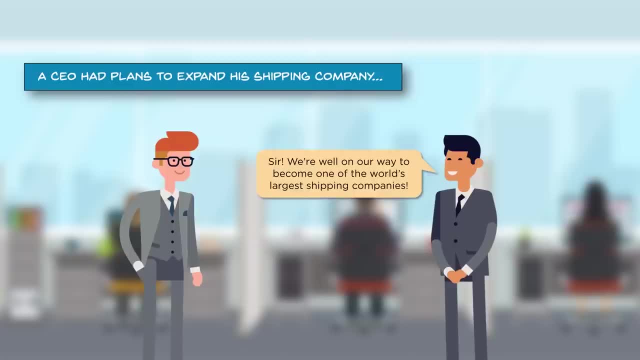 in a city not so far away. a CEO had plans to expand his company globally and called one of his IT personnel for an IT opinion. and this guy has been in the company for a long time, long time, and is very seasoned with the company's infra. and he nicely answered. 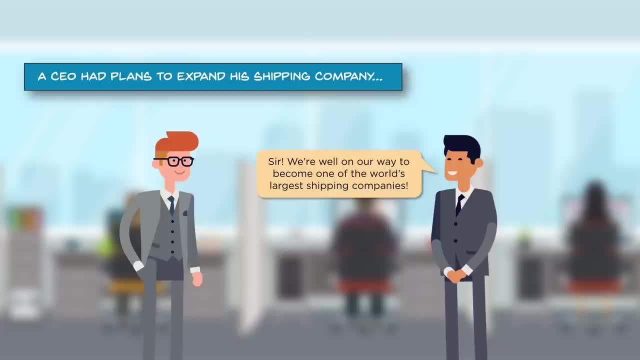 the questions with what he foresaw and he said: I have a good news and a bad news for us to go global. and he starts with the good news. he said, sir, we're well on our way to become one of the world's largest shipping company and the 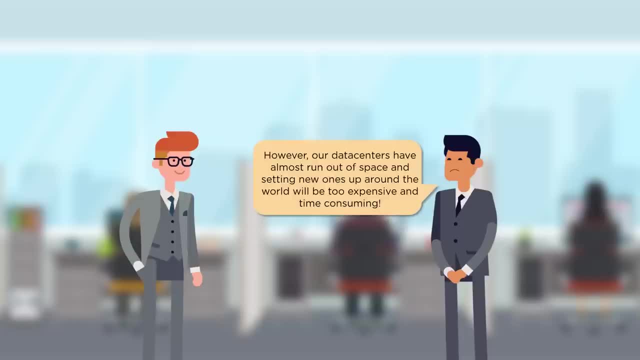 bad news is, however: our data centers have almost run out of space, and setting up new ones around the world would be too expensive and very time-consuming. now the IT personnel- let's call him Mike now. he explains the situation from how he saw it, but the CEO had done some homework about how he was going to do it. 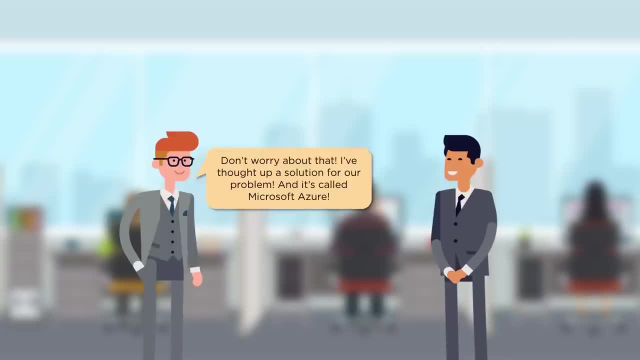 and he answered Mike saying: don't worry about that, Mike, I've come up with a solution for a problem and it's called Microsoft Azure. well, Mike is an hard-working and honest IT professional working for that company, but he did not spend time on learning the latest. 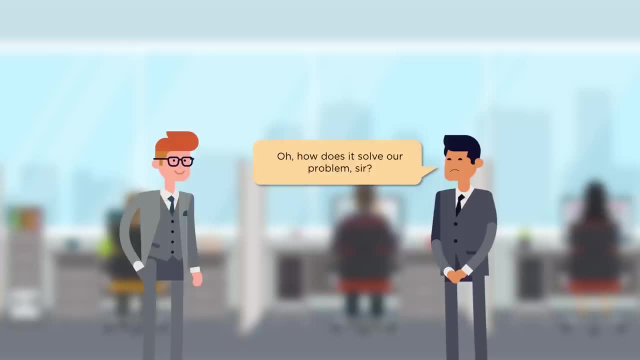 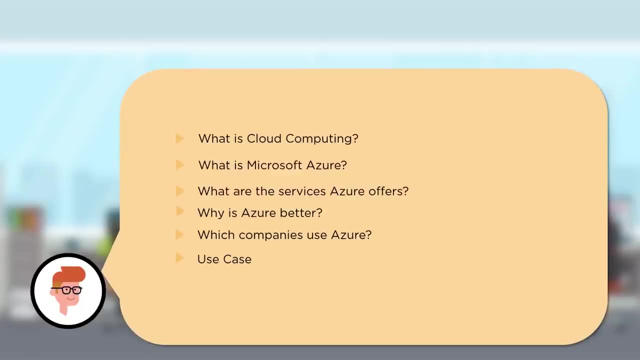 technologies and he asked this question very honestly: oh, how does it solve a problem? and the CEO begins to explain Azure to Mike and he starts with what is cloud computing and then he goes on and talks about Azure and the services offered by Azure and why Azure is better than the other cloud providers and what 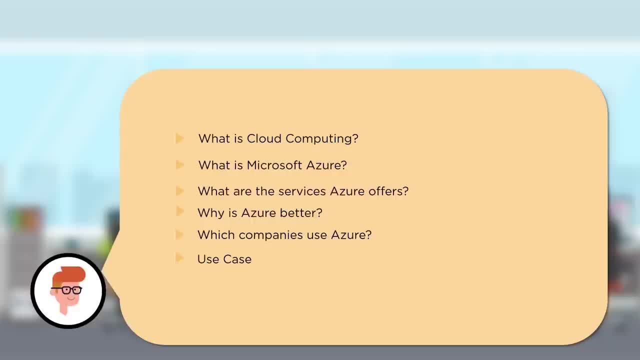 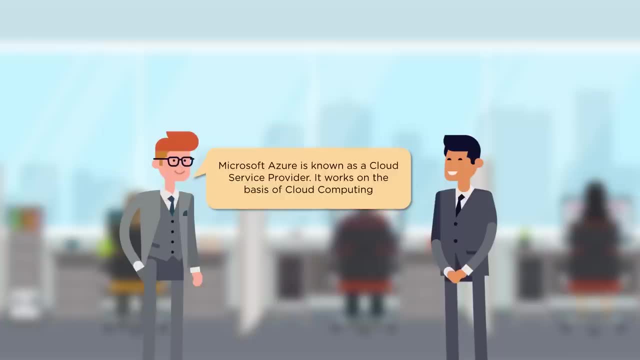 are the great companies that uses Azure and how they got better out of it. and then he winds it all up with the use cases of Azure. so he begins his explanation saying Microsoft Azure is known as the cloud service provider and it works on the basis of cloud computing. now Microsoft Azure is. 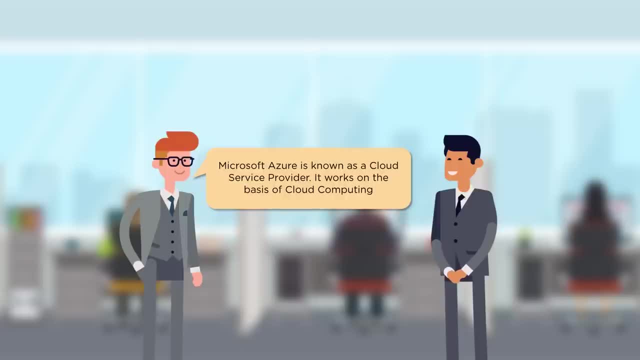 formerly known as Windows Azure, and it's Microsoft's public cloud computing platform. it also provides a range of cloud services, including some of them are compute, analytics, storage and networking. we can always pick and choose from these services to develop and scale our applications, or even plan on running. 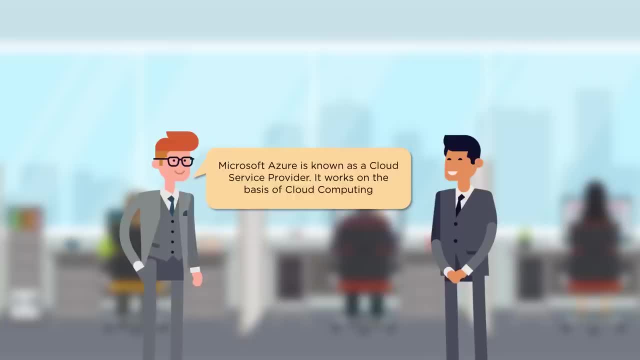 existing applications in the public cloud. Microsoft Azure is both a platform as a service and infrastructure as a service. let's now fit their conversation out and let's talk about what is cloud computing? Azure services offered by Azure. how is Azure leading when compared to other cloud service providers and what? 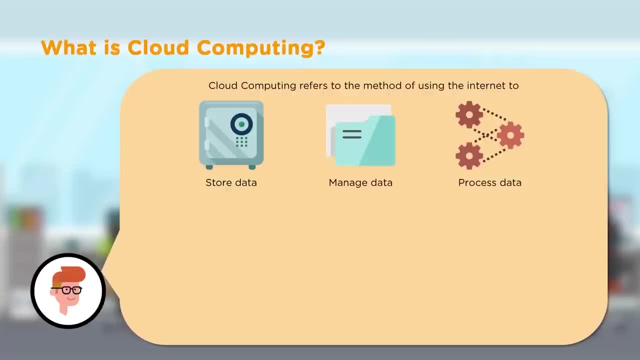 are the companies that are using Azure. let's talk about that in simple terms. cloud computing is being able to access compute services like servers, storage, database networking, software analytics, intelligence and lot more over the internet, which is the cloud, with the flexibility of the resources that we use, like anytime I want a resource, I can use one and it becomes available. 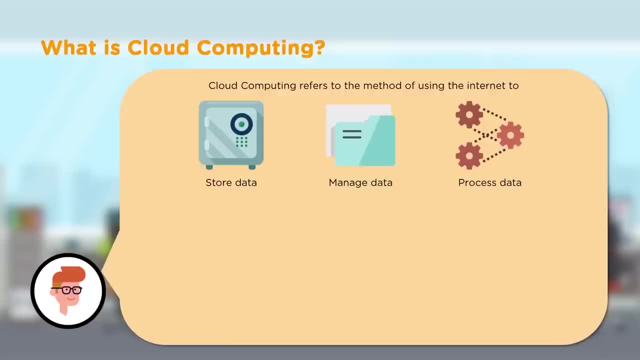 immediately and anytime if I want to retire and resource. I can simply retire a resource and not pay for it, and we also typically pay only for these services that we use and this helps greatly with our operating cost to run our infrastructure more efficiently and scale our environment up or down. 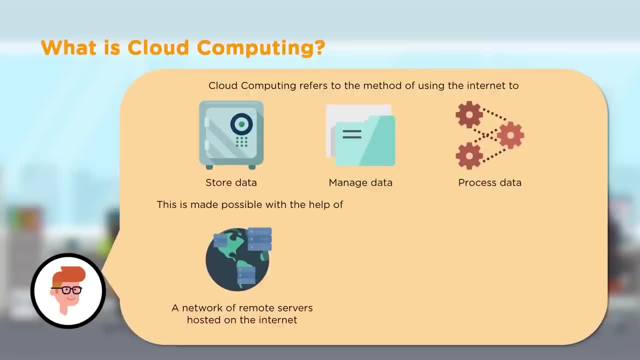 depending on the business needs and changes. and all of these services are available to us and we can use them to run our infrastructure more efficiently and scale our environment up or down, depending on the business needs and changes. and all the servers and storages and databases and networking- all that are accessed. 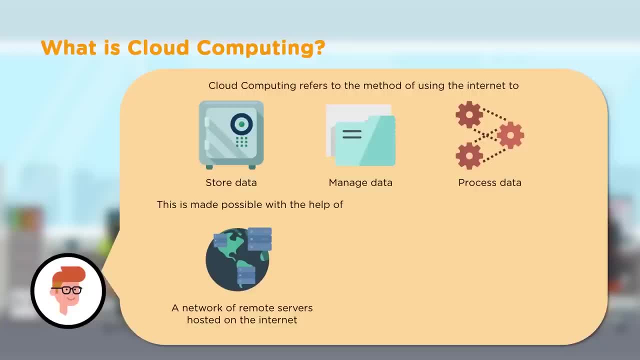 through the network of remote systems or remote computers hosted in the internet, typically in the providers data center, which is Azure in this case. now we don't use any physical server or an on-premises server here. well, we still use physical servers and VMs in a hosted on a. 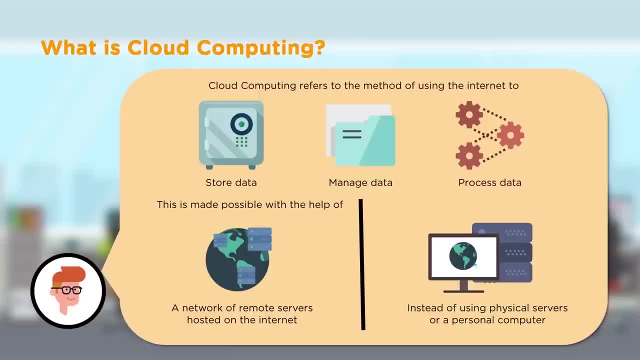 hardware or a physical server, but they're all in the providers environment and none of them sit on-premises or in our data center. we only access them remotely. it looks and feels the same, except for the fact that they are in a remote location. we access them remotely, do all the work remotely. 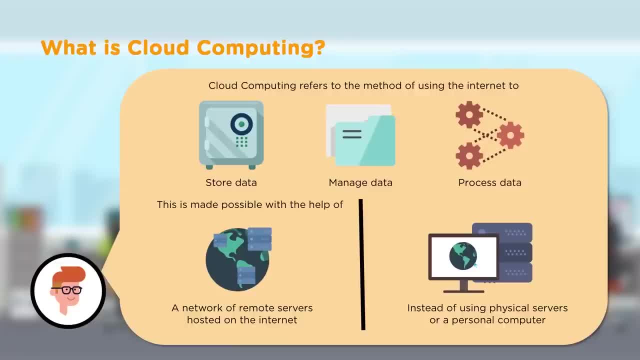 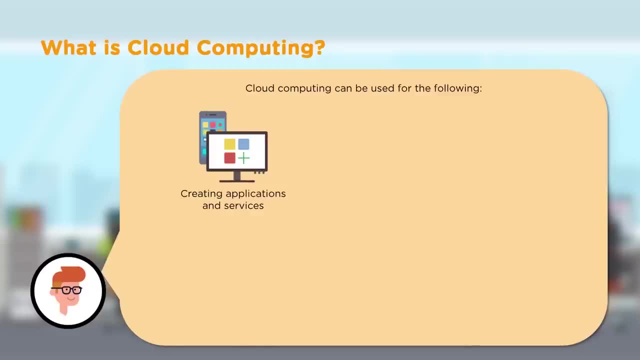 and when we're done, we can shut it down and not pay for them. so some of the use cases, some of the use cases of cloud computing, are creating applications and services. the other use cases are storing or using cloud for storage alone, if there is one thing that ever grows in an organization. 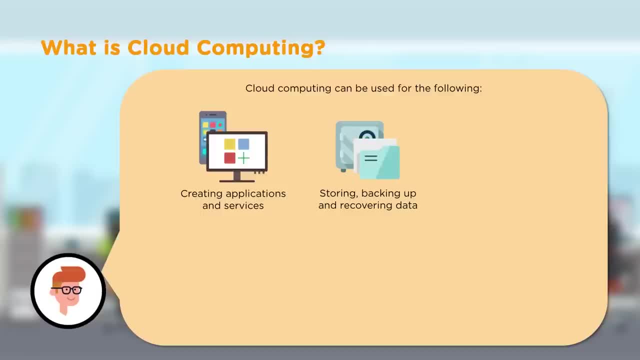 is the storage. every new day there is a new storage requirement and it's very dynamic. it's very hard to predict and if we go out and buy a big storage capacity upfront and till we use the storage capacity fully, the empty storage is. you know we're wasting money on them. so instead I can go for a storage which. 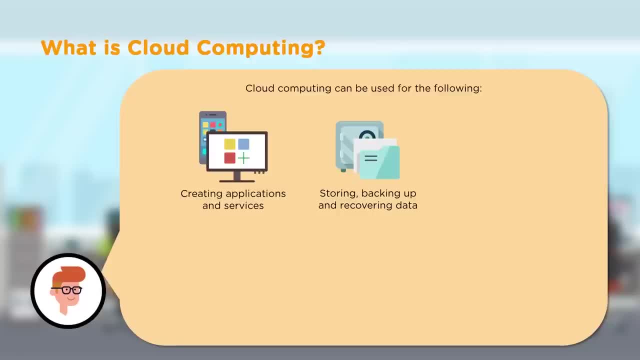 scales dynamically. that's, in the cloud, put storage or put data in the cloud and pay only for what you're storing and for the next month, if you have deleted or flushed out some files or data, pay less for it. so it's a very dynamic storage in. 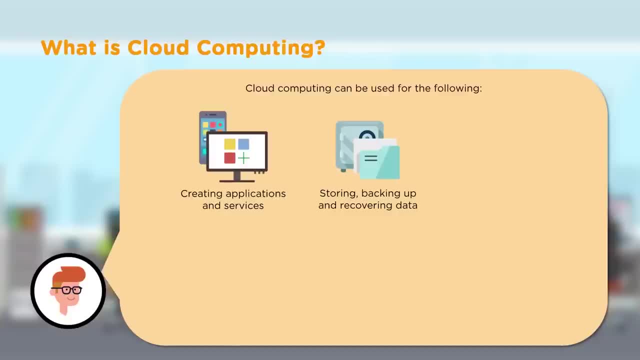 the cloud and a lot of companies are getting benefited from storing data in the cloud because of its dynamic in nature and the cost that comes along with it- the cheap cost that comes along with it and also they give a lot of the providers like Azure. they give data replication for. 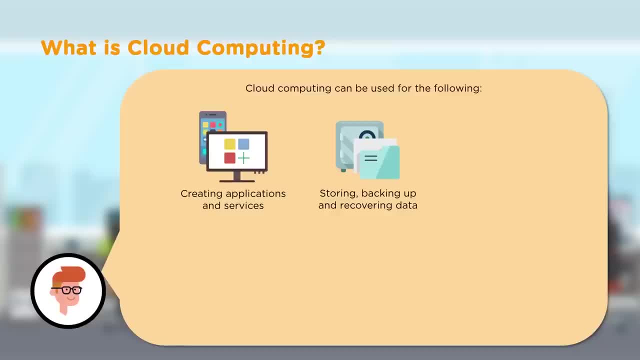 free. they promise an SLA along with the data we store in the cloud, so there's an SLA attached to it, and they also provide data recoveries as well. if, in case, something goes wrong with the physical disk where our data is stored, Azure automatically makes our data available. 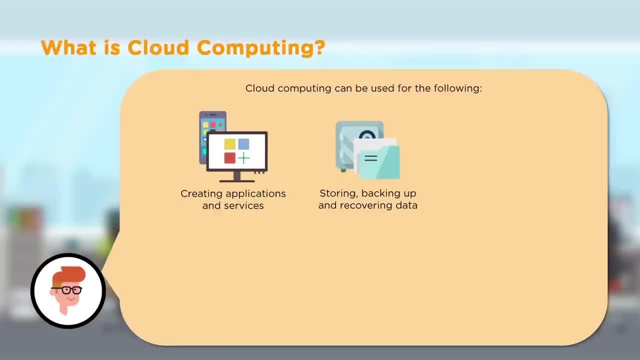 from the redundant or other places where it had stored our data because of the SLA they wanted to keep. the other use case for Azure is hosting websites and running blogs using the compute service. be it storing music and letting your users stream the music, Azure is a good place to store music and stream the 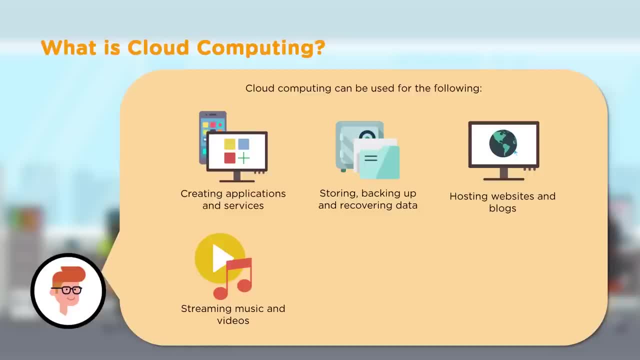 music with the benefit of CDN content delivery network, which allows us to stream a video or audio files with great speed. you know, with that, with Azure, our audio or video application works seamlessly because they are provided to the client with very low latency and that improves the customer experience for our application. as your, 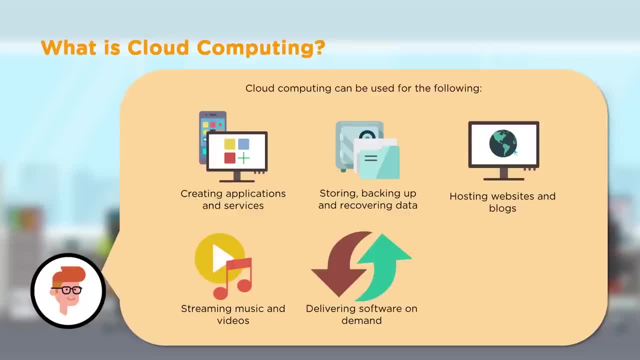 compute service is a good place for delivering software on demand. there are a lot of softwares, embedded software that we can buy using Azure, and everything on a pay-as-you-go service model. so anytime we need a software, we can go out and immediately buy the software. for the next one hour or two hour, let's say, and use them and then. 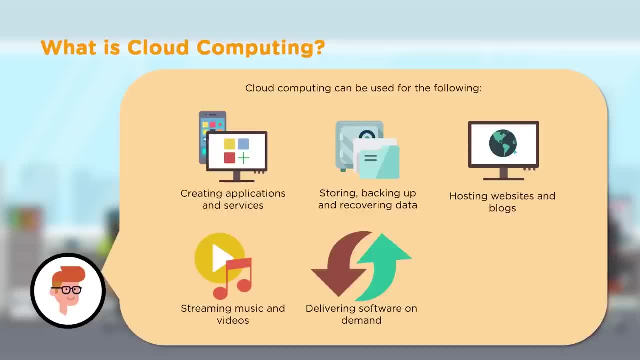 return it back. we're not bound to any yearly licensing cost by that, as your computing services has analytic available for us with which we can analyze, get a good visualization of what's going on in a network. beat logs, beat the performance, beat the metrics you know, instead of looking at logs and searching logs and 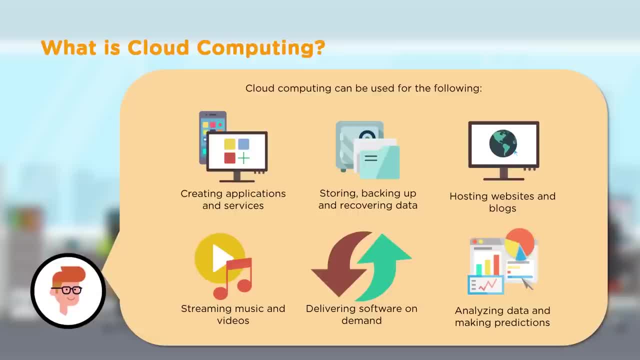 trying to do manual things over the heaps and heaps of logs that we have saved. Azure analytic services helps us to get a good visual off what's going on in the network. where have we dropped? where have we increased? what's causing what's the major driver is the top 10 errors that we get in the server, in the application stuff like that. those can be. 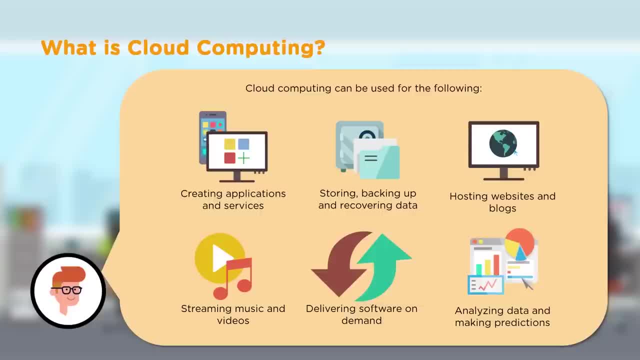 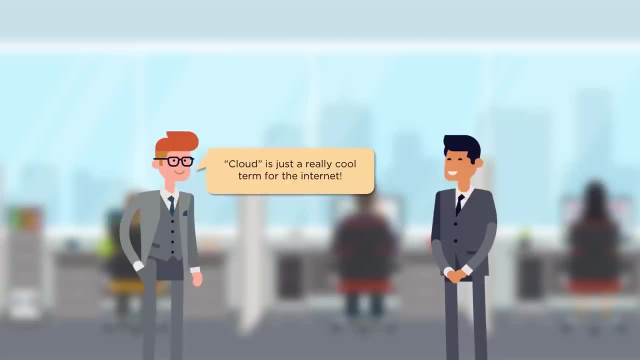 easily gathered from the azure analytic services. now, cloud is really a very cool term for the internet. a good analogy would be looking back. anytime we look at a diagram, when we do not know how things are transferred, we simply draw a cloud right. for example, a mail gets sent from: 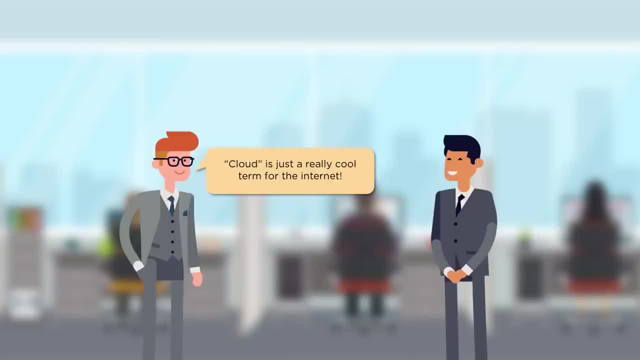 a person in one country to a person in the other country, a lot of things happening in between, from the time you hit the send button and the time the other person hits the read button. right and we. the simple and the easiest way of putting it in a picture is simply draw a cloud and on the one end, 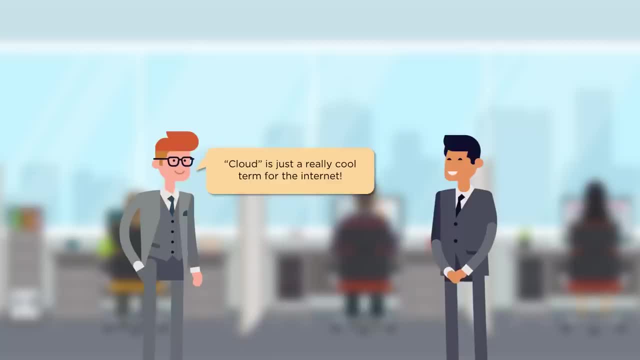 one person will be sending the email and, on the other end, the other person will be reading the email. so a cloud is a really cool term for the internet. now that's some basics about cloud computing. now that we've understood about cloud computing in general, let's talk about microsoft azure as a 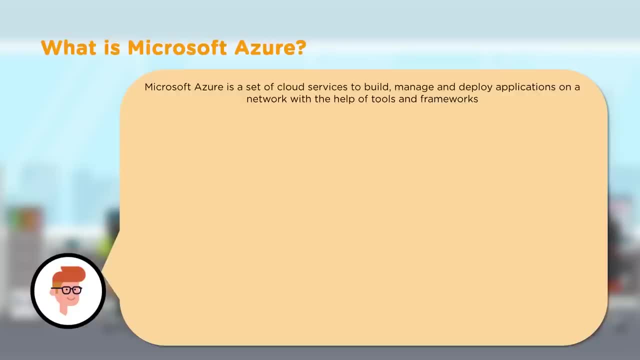 cloud service- now microsoft azure, is a set of cloud services to build, manage and deploy applications on a network with the help of microsoft azure's frameworks. now microsoft azure is a computing service created by microsoft basically for building, testing, deploying and managing applications and services through a global network of microsoft managed data centers- now microsoft. 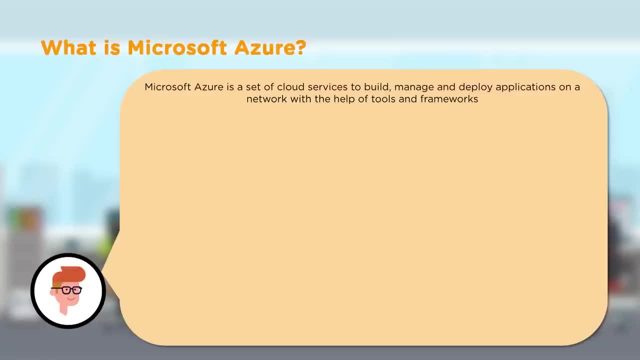 azure provides saas, which is software as a service, and paas, which is platform as a service, and iaas- infrastructure as a service, and they support many different programming languages, tools and framework, and those tools and framework include both microsoft specific and third-party software. now let me pick and talk about a specific service, for example, management azure automation provides. 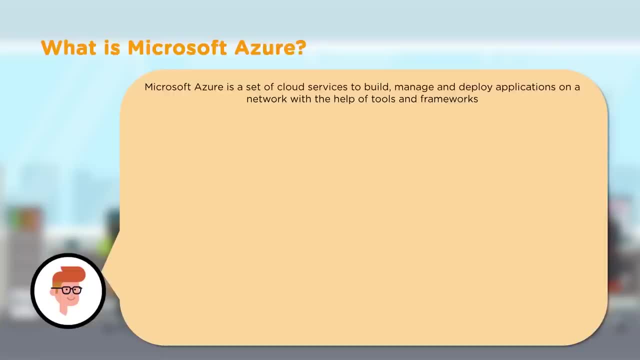 a way for us to automate the manual, long running and frequently repeated tasks that are commonly performed tasks both in cloud and enterprise environment. it saves a lot of time and increases the reliability and it kind of gives a good administrative control and even schedules the task automatically to be performed on a regular basis. so it's a really cool service and it's a 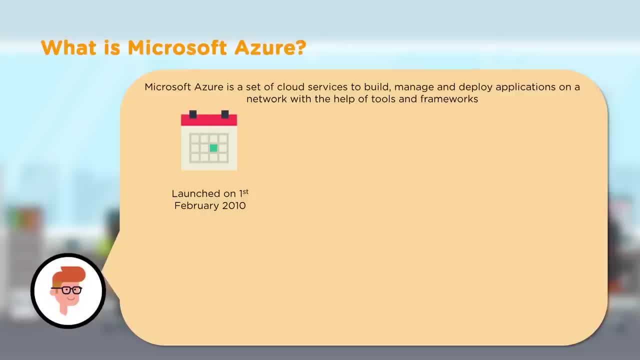 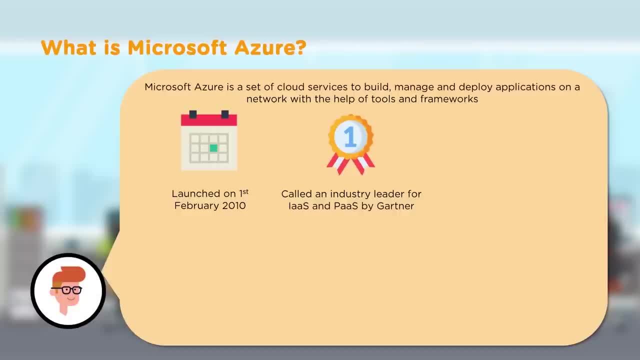 industry leader for infrastructure and platform as a service by a gartner. now gartner is the world's leading research and advisory company. this microsoft azure supports a number of programming languages like c, sharp, java and python. all these cool services we get to use in our work as a. 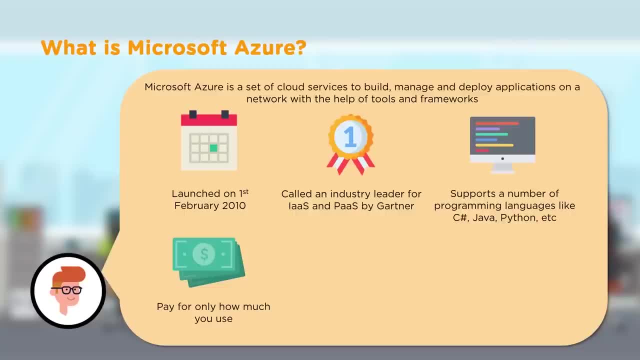 to use and pay only for how much we use. For example, if we use for an hour, we only get to pay for an hour, even the costliest system available. If we use them for an hour, we only pay for that particular hour and then we're done. No more billing on the resource that we have used. 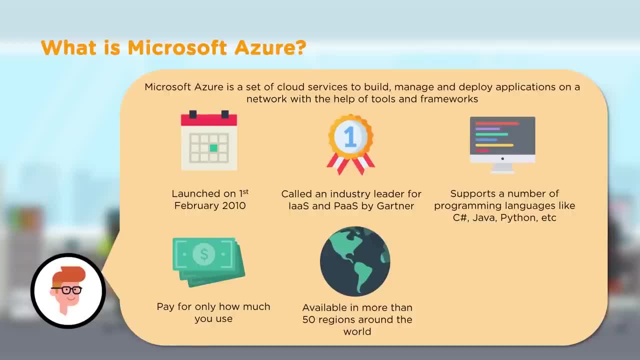 Microsoft Azure has spread itself more than 50 regions around the world, So it's quite easy for us to pick a region and start provisioning and running our applications, probably from day one, because the infrastructure and the tools and technologies needed to run our application are already available. All that we have to do is commit the code in that particular region or 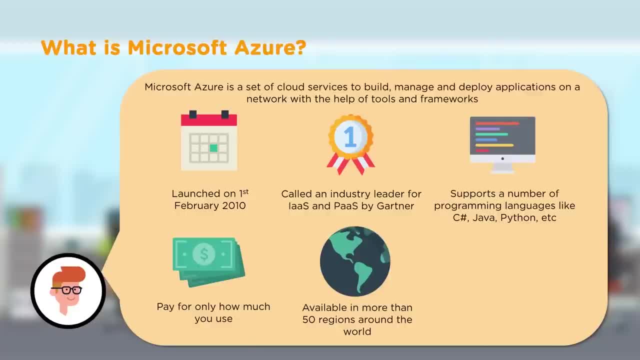 build an application and launch it in that particular region and they become live starting day one. Now, because we have 50 regions around the world, we can very carefully design our environment To provide low latency services to our customers instead of in traditional data center. 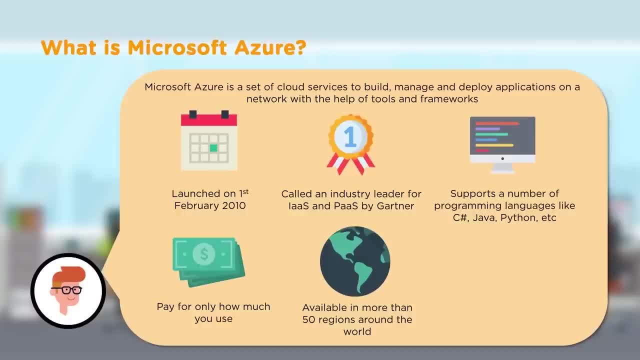 let's say, customers will have to- or their requests will have to- travel all the way around the globe to reach the data center, which lives in the other side of the planet, And this adds more latency to it, and it is really not feasible to build a data center near each customer location. 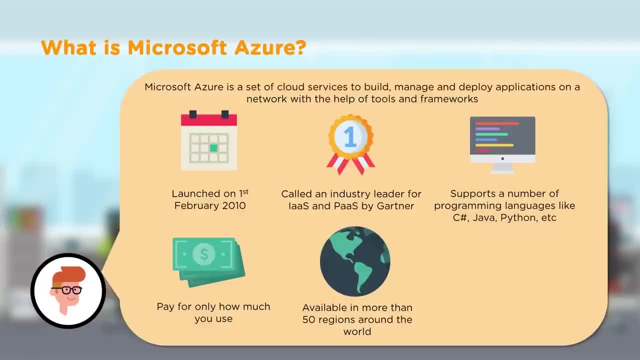 because of the cost involved, But with Azure, it's possible. Azure already has data centers around the world and all that we have to do is just pick a data center, build an environment there. They're available starting day. one number one: 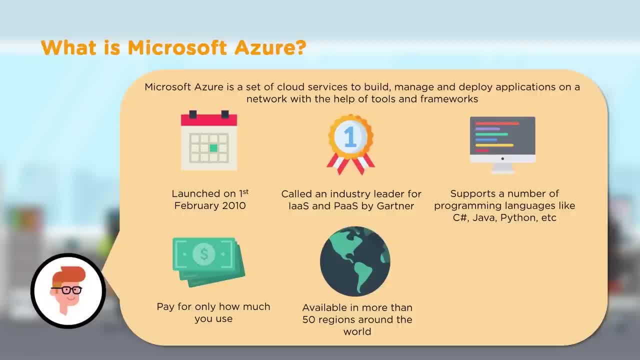 And also the cost is considerably saved because we are using a public cloud instead of an physical infrastructure to serve those customers from a very local location. And the services that Azure is offering is ever increasing. As of now, as we speak, we have like 200 plus services offered and they span through different domain or different platform or different technologies available within the Azure console portal. 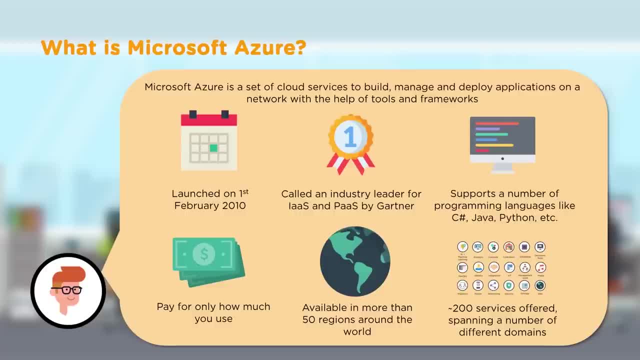 Now, we're going to talk about that later in this section, So hold your breath till we talk about it. But for now, just know that we have like 200 plus services offered by Azure. Let's now talk about different services in Azure, starting with artificial. 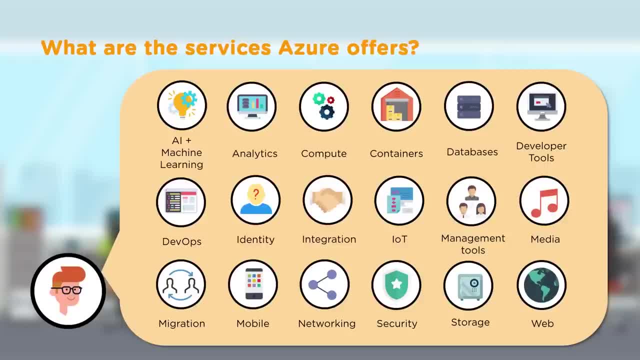 intelligence plus machine learning, where we have a lot of tools and technologies. So the wide variety of services available in Azure includes artificial intelligence plus machine learning plus analytic services to get and or to give us a good visual of how the data or how the application is performing or the type of the category of data stored. 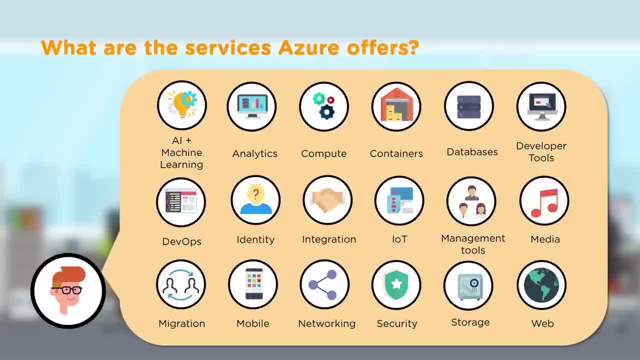 and to read from the logs, And variety of compute services, Different VMs with different size and different operating systems, different containers available, different type of databases available, a lot of developer tools that are available for us and identity service to manage our users in the Azure cloud. 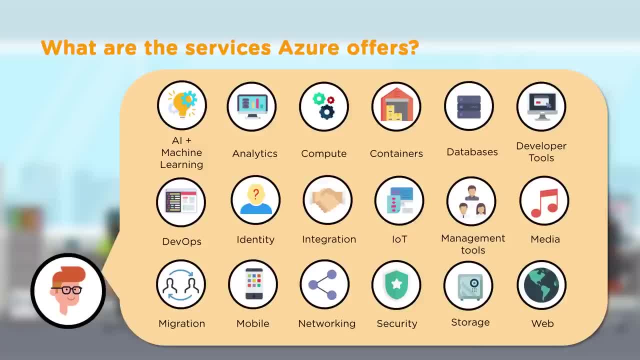 And those users can be integrated or federated with, let's say, Google, Facebook, LinkedIn. So they are some external federation services. They can be used to integrate with the Azure cloud. So they are some external federation services. They can be used to integrate with the Azure cloud. 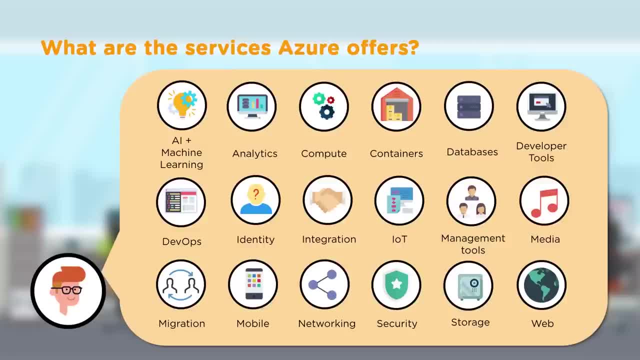 They can be used to integrate with the Azure cloud. So they are some external federation services. They can be used to integrate with our identity system, IoT, IoT services, IoT tools and technologies available And management tools to manage the users you know, creating identities. one. 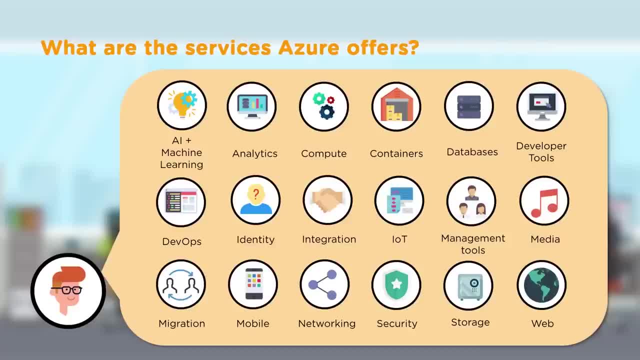 and then managing them on top of it is a totally different thing. And we have tools, technologies to manage the users, Cool services for data migration. Data migration is now made simple. Tools and technologies available for mobile applications, application development And I can plan my own network in the cloud with the networking services. 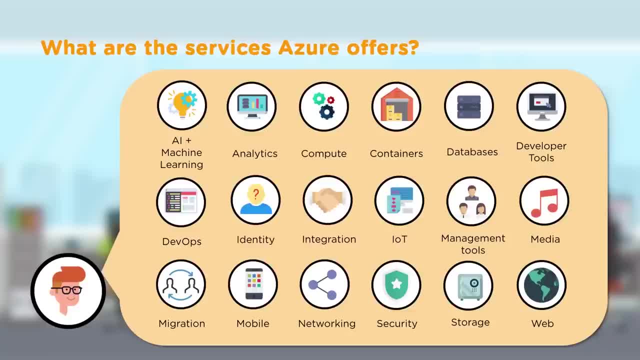 I can implement my own security, both Azure provided and third-party security services, on Azure cloud. That's now possible And a lot of storage options available in the cloud. So these are just a glimpse of the big list of services available in Azure cloud. So that was a glimpse. 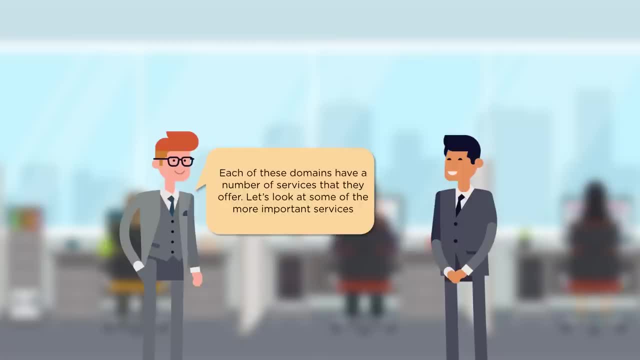 of what's available in the cloud. Let's talk about the services in a specific. Let's take compute, for example. You know, whenever we're building a new application or deploying existing ones, the Azure compute service provides the infrastructure we need to run and maintain. 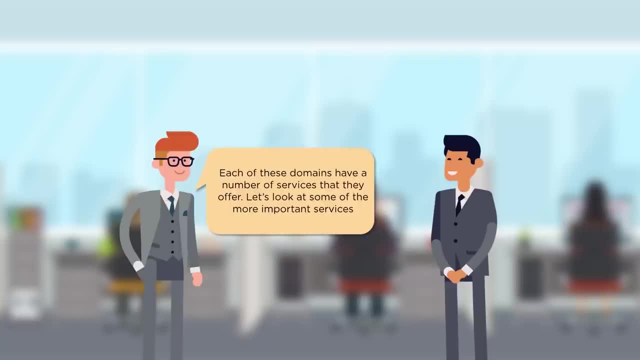 our application. We can easily tap in the capacity that Azure cloud service has and we can scale our compute requirement on demand. We can also containerize our application. We have the option of choosing Windows or Linux VM machine and take the advantage of the flexible options Azure. 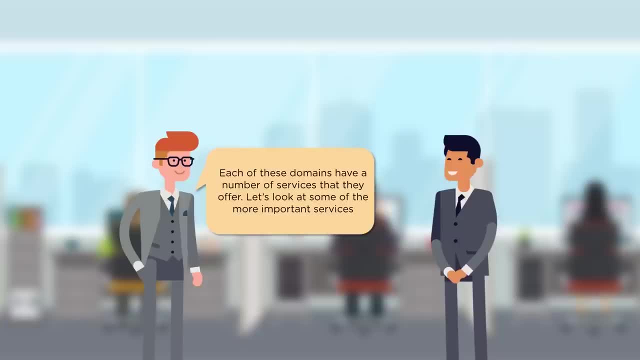 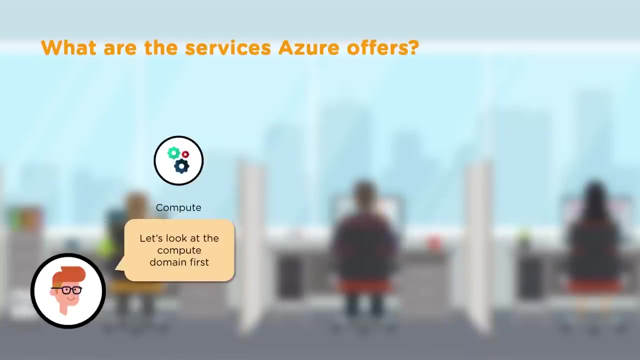 provides for us to migrate our VMs to Azure and lot more. And these compute services also include a full-fledged identity solution, meaning integration with Active Directory in the cloud or an on-premises, and lot more. Let's look at some of the services that this compute domain. 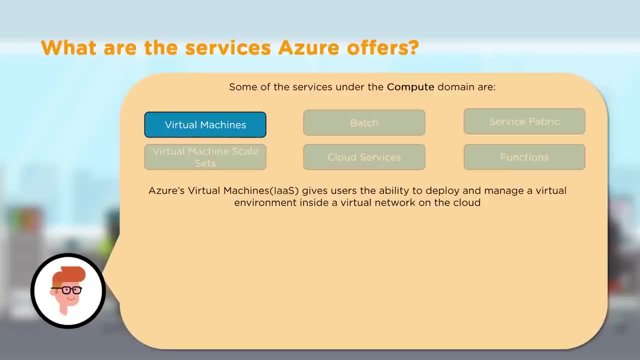 provides. Some of the services the compute domain provides are virtual machines, and this Azure virtual machines gives us the ability to develop and manage a virtual computer environment or a virtualized environment inside Azure's cloud environment- that, too, in a virtual private environment. So let's take a look at some of the services that this compute domain provides. 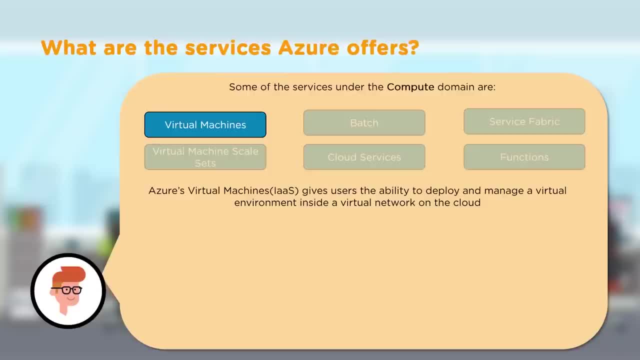 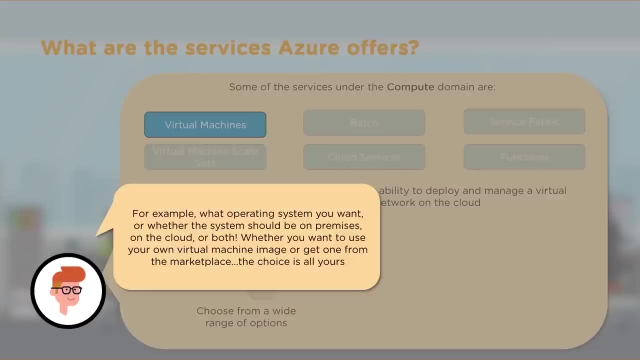 Now. we will talk about virtual private network at a later point, but as of now, just know that there are a lot of services available in Azure compute service that we can get benefited from. We can always choose from a very wide range of compute options, For example. you know. 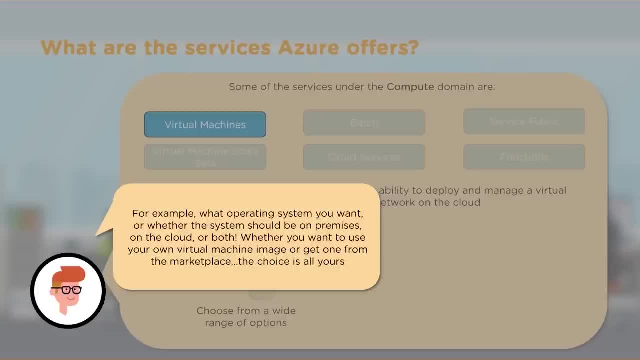 we have an option to choose the operating system. We have the option to choose whether the system should be in on-premises or in the cloud, or do we want to maintain the environment both in on-premises and in the cloud? We have the option of choosing the operating system. 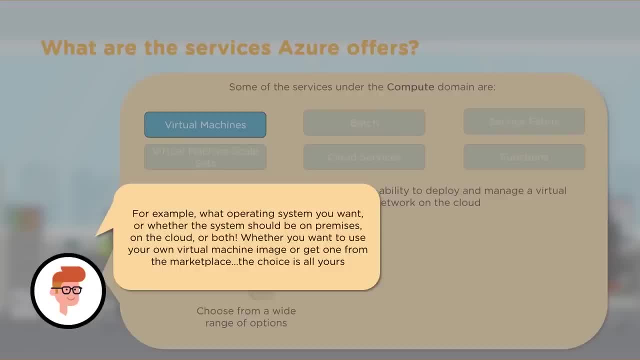 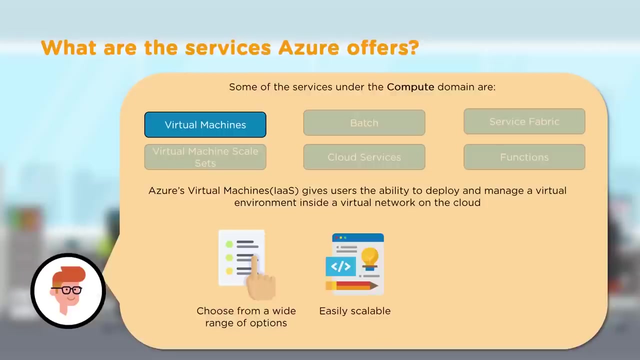 whether we want to use our own operating system with some software attached to it, or do we want to go and buy the operating system from the cloud, from Azure marketplace. And these are just a few of the options available for us when we want to buy the compute environment And these compute. 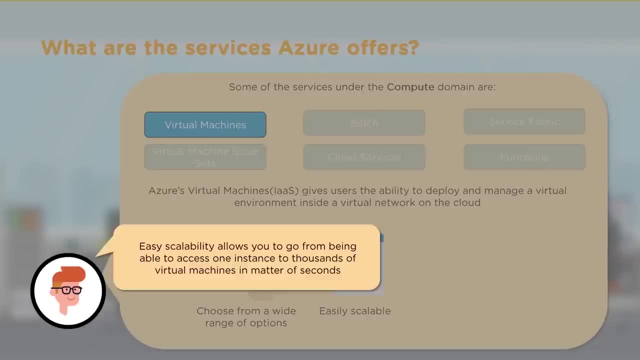 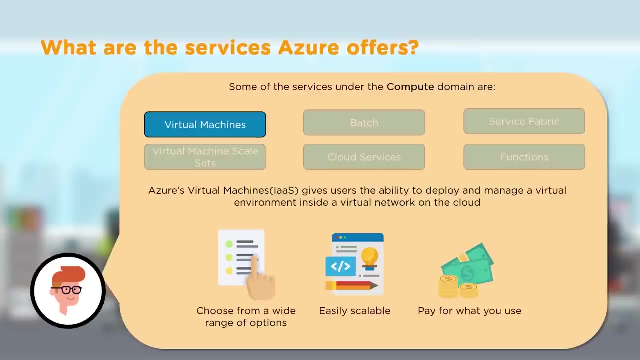 environments are easily scalable, meaning we can easily scale our VM instance from one instance to thousands of virtual machines in a matter of minutes, or simply put in a couple of button clicks, And all these services are available on a pay-for-what-we-use model. 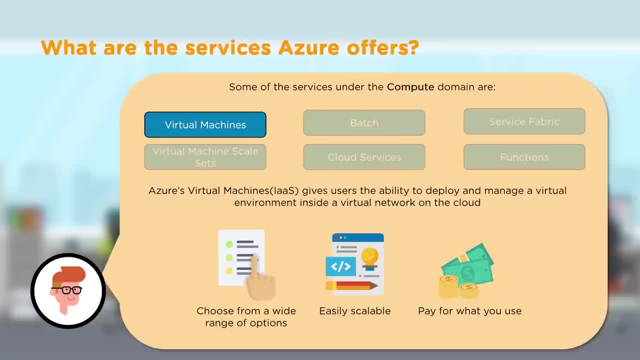 meaning there is no upfront cost. We use the service and then pay for the services that we have used. There's no literal long-term commitment when it comes to using virtual machines in the cloud, And these models are available on a pay-for-what-we-use model, meaning there is no. 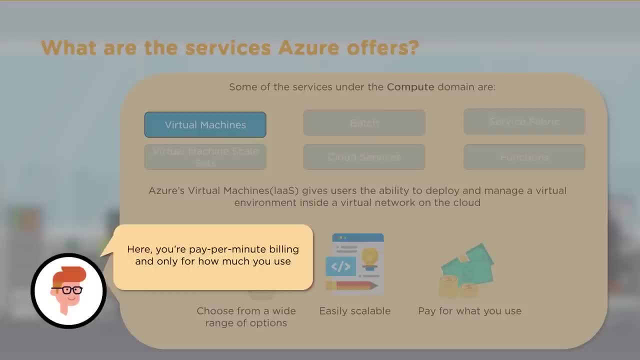 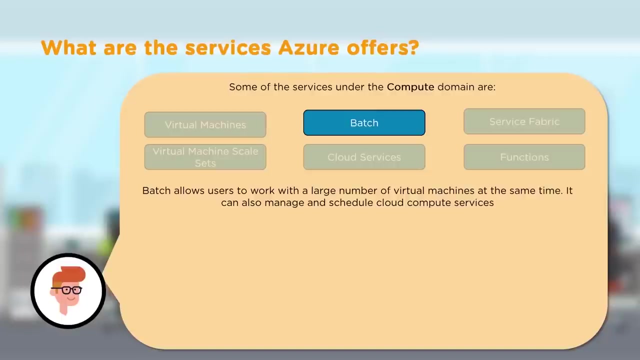 upfront cost. Most of the services are built on a pay-per-minute billing basis, And at no point, because of the pay-per-minute billing model, at no point, we will be overpaying for any of the services. That's attractive, isn't it? Now let's talk about batch service. Now, batch service is. 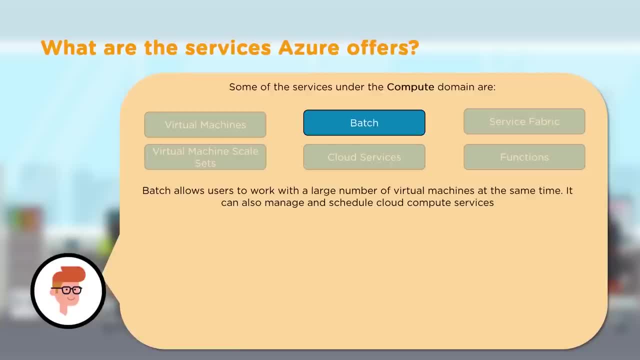 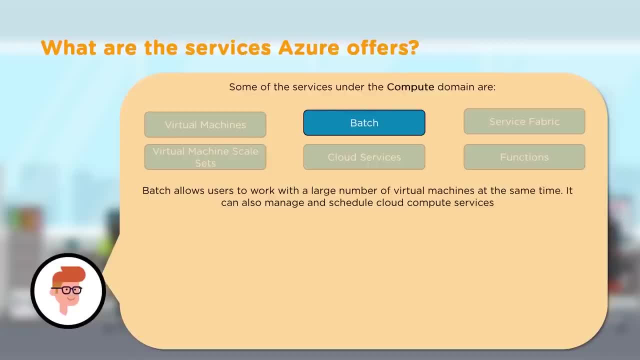 we can take advantage of the services that we have And we can take advantage of the environment's unique features, And not only that. in short, the batch service helps us to manage the whole batch environment And also it helps to schedule the jobs. Now this Azure batch service actually runs. 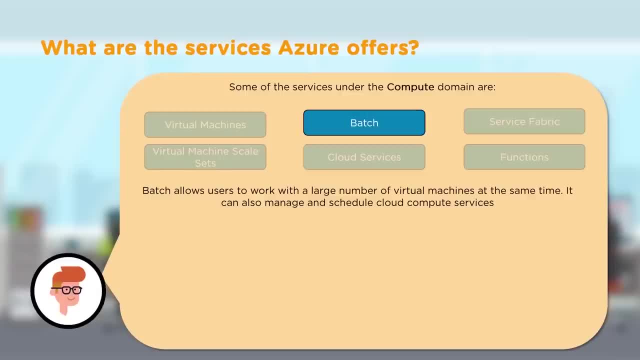 on a large scale, parallel and high-performance computing. Because of that, batch jobs are highly efficient in Azure. And when we run batch services, this Azure batch creates a pool of computer nodes and installs the needed applications that we need to run. And when we run batch services, this Azure. 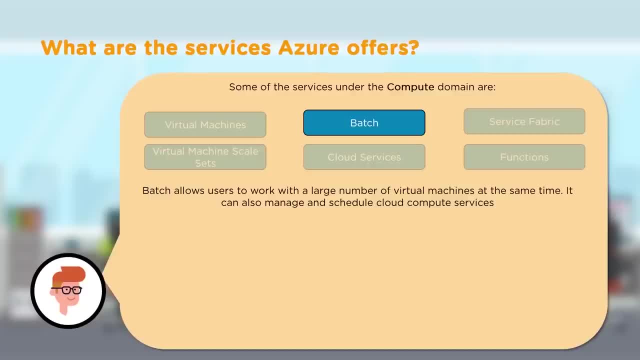 batch has an assignment full to help us schedule the add-ons that we want to run, and then it schedules jobs to those individual nodes in those pools. As a customer, there is no need for us to install a cluster, or there is no need for us to install a software that actually schedules the 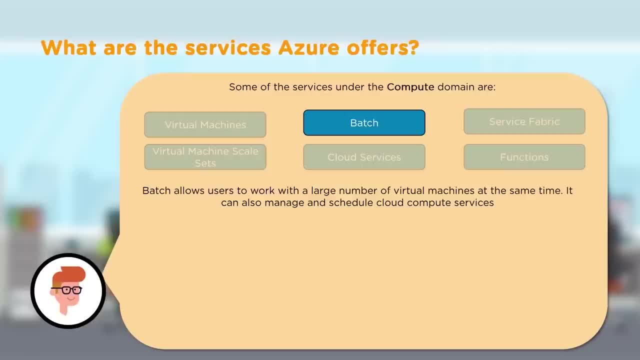 jobs, or even to manage, or even to scale those infrastructure or the software, because everything is managed by Azure And this batch service is a platform as a service. There is no additional for I mean. the only charges that we'll be paying is for the virtual machines. 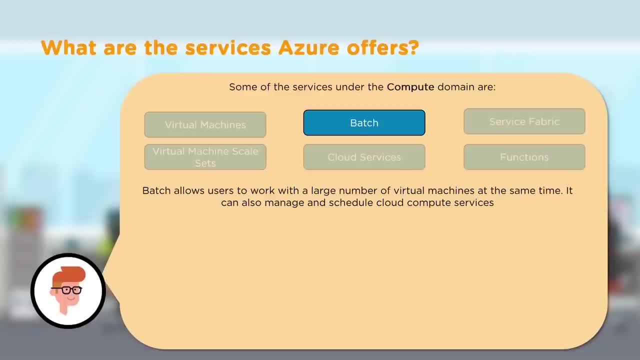 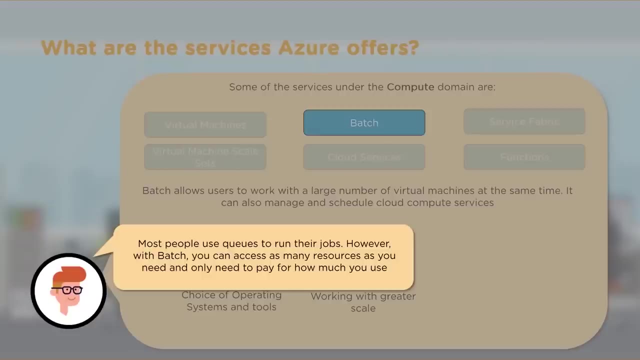 that the service uses and the storage that we will be using, of course, and the networking services that we will be using for this batch service. let's summarize this batch service. we have a choice of operating system that we can pick and use, and it scales by itself. now the alternative for the batch would be: 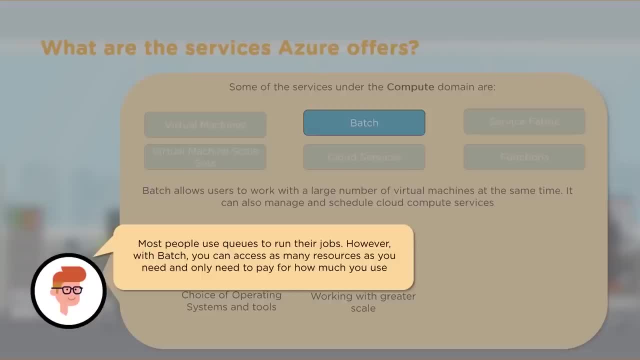 queues. but in queues we'll have to pre provision and pay for the infrastructure even if we're not using it. but with a batch we only pay for what we use and this batch service helps us to manage the application, manage the scheduling as a whole, as if they are just one thing, as next thing in the 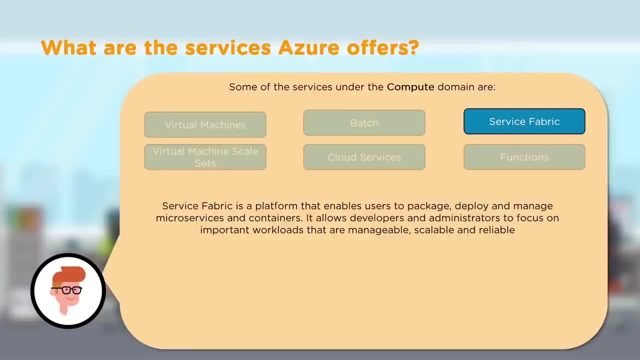 compute domain. let's talk about this fabric service now. this fabric service is actually a distributed system platform that helps us to package, deploy and manage a schedule, scalable and a very reliable microservice and containers. and what does it help? this Azure fabric service helps us or it helps the developers and 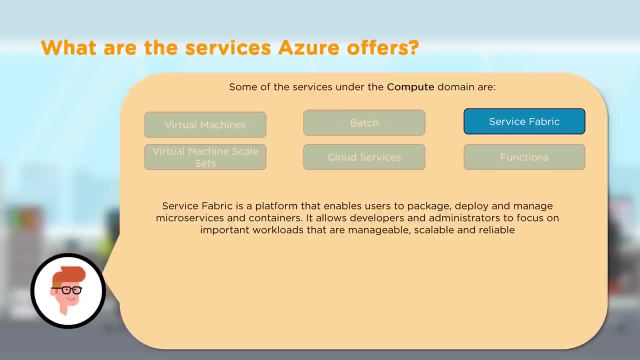 administrators, so they can avoid the complex infrastructure problems and they can focus only on implementing workloads or taking care of their development, taking care of their application, instead of spending time on infrastructure. so what service fabric? service fabric: it provides runtime capabilities and life cycle management, two applications that are composed of micro services. no, 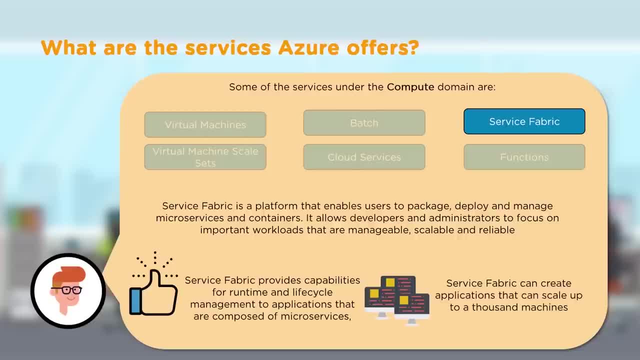 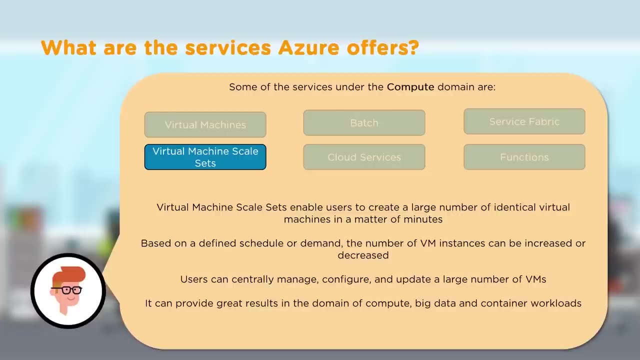 infrastructure management at all, and with service fabric we can easily scale the application to tens or hundreds or even to thousands of machines. here machines represent containers. as next thing in compute domain, let's talk about virtual machine scale set. now, this virtual machine scale set. it lets us to. 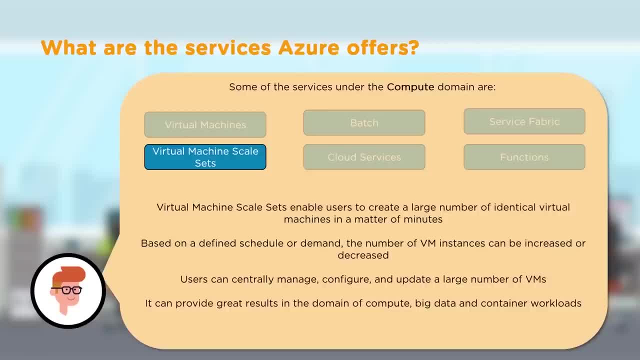 create a group of identical, load-balanced VM's. I just want to mention it again. It helps us to manage a group: identical and load balanced VMs. The number of instances or the number of VM instances in a scale set can increase or decrease in response to the demand or in response to a schedule that we define. 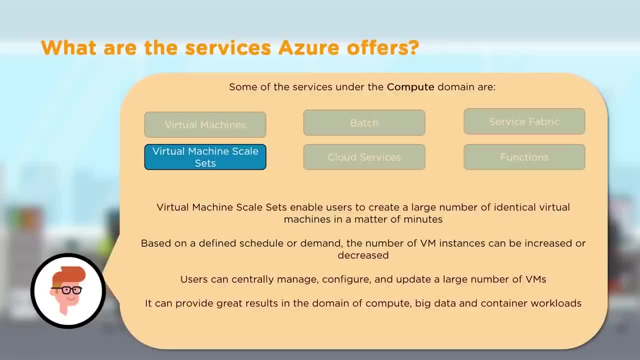 You know, the resources needed on a Monday morning is not the same as that would be required on a Saturday or a Sunday morning. All right, And even within the day, the resources that would be needed in the beginning of the business hour is not the resources that would be needed at noon or, you know, after eight or nine in the evening. 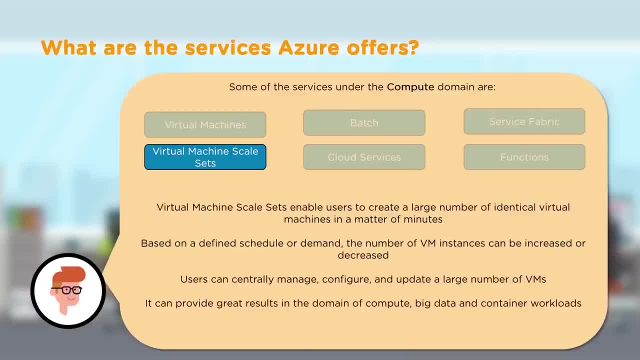 So the demands could actually vary in the environment And this scale set helps us to take care of the varying demand or take care of the different infrastructure requirement at a different schedule: throughout the day, throughout the week, throughout the month, or could be throughout the year as well. 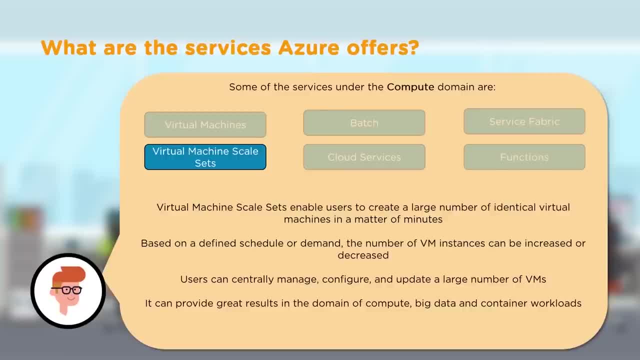 The scale set also allows us to provide high Availability to our applications, and it helps us to centrally manage, configure and update a large number of VMs, as if they they are just one thing. Now you might ask: well, virtual machines are enough. 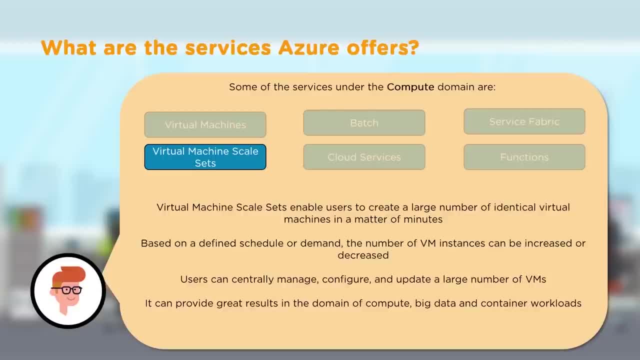 Why would we need a virtual machine scale set? Just like I said, this virtual machine scale set helps us with a greater redundancy and improved performance for our applications, And those applications can be accessed through a load balancer that actually distributes the requests. 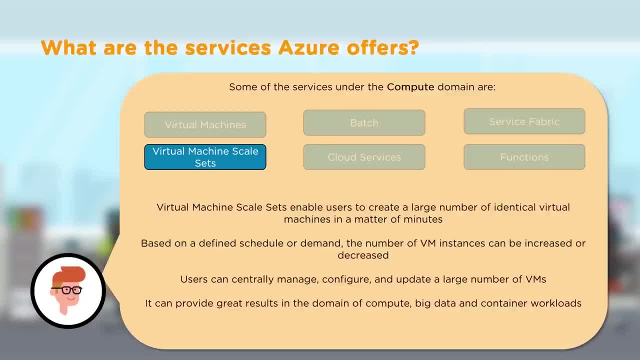 So, in a nutshell, this virtual machine scale set. it helps us to create a large number of identical virtual machines, number one and with scale set, we can increase or decrease the virtual machines. with virtual machine scale set, We can centrally manage and configure and update a big group of VMs and it's a great use case when it comes to big data or container workloads as next thing in compute domain. 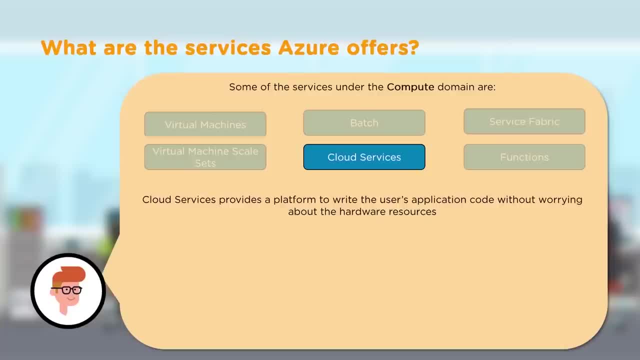 Let's talk about cloud services now. This Azure Cloud service is actually a platform as a service, and it's very friendly. In fact, it is designed for applications that support scalability, or an application that requires scalability or reliability, And, and on top of it, you want them to be very inexpensive to operate. 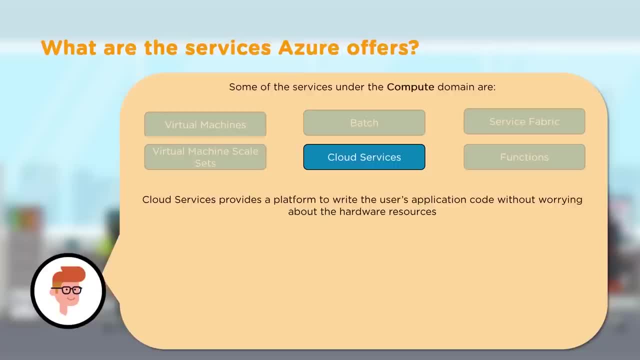 So Azure cloud service provides all these. So where would this cloud service run? Well, it runs on a VM, but it's a platform as a service. VMs are infrastructure as a service And when we run applications on VM through cloud service, it becomes platform as a service. 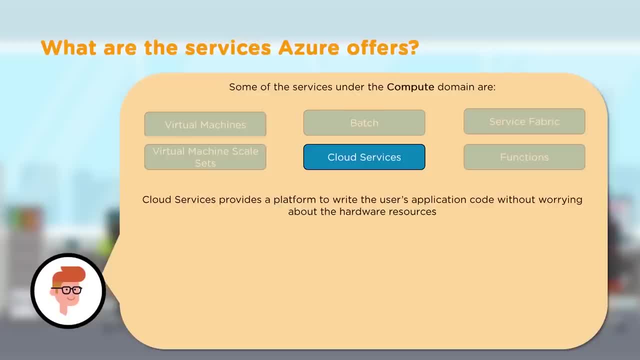 So here is how you got to be thinking. with infrastructure as a service like VMs, We first create and configure the environment and then we run applications on top of it. Let's look at the responsibility. The responsibility for us in VM is that we manage everything end to end, like you know, deploying new patches. 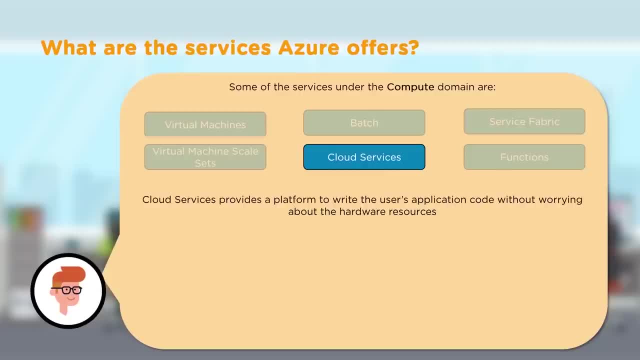 picking the versions of the operating system and making sure they are intact and all that stuff. It's all managed by us, But, on the Contrary, with platform as a service, it's- I mean, it's as if the environment is already ready. 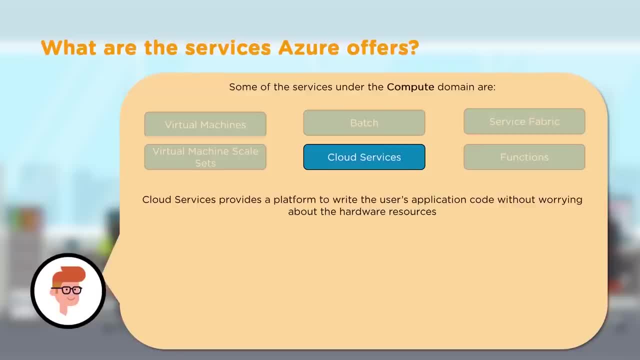 All that you have to do is deploy your application in it and manage the platform. I mean manage the platform not as an administrator, because all the administration is taken care by Azure. like deploying new versions of the operating system, It's all handled by the Azure. 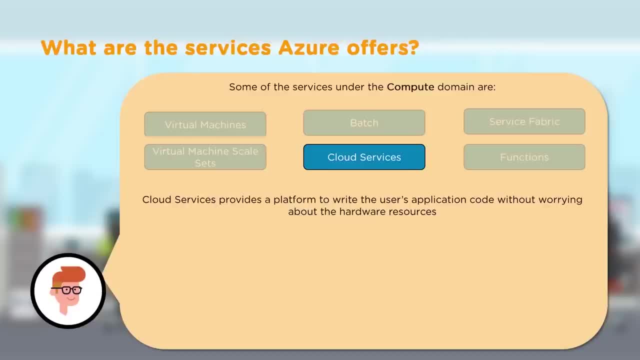 So we deploy the application and we manage the application. That's it. Infrastructure management is handled by Azure. So what does cloud Service provide? This cloud service provides a platform where we can write the application code and we don't have to worry about hardware. 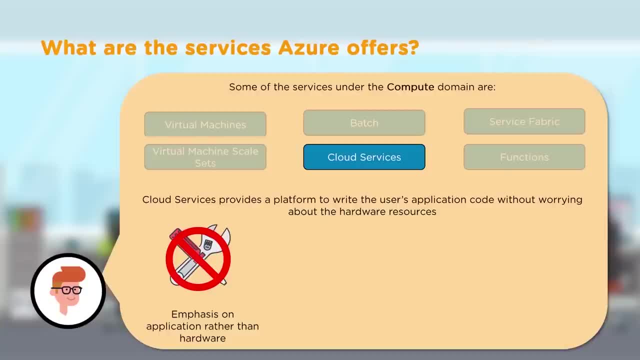 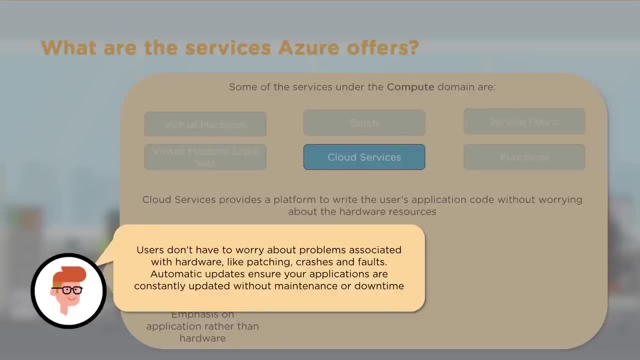 Simply hand over the code and cloud service takes care of it. So no worry on the hardware at all. So responsibilities like patching. What do we do if something crashes? How do I update the infrastructure? How do I manage the maintenance or the downtime in the underlying infrastructure? 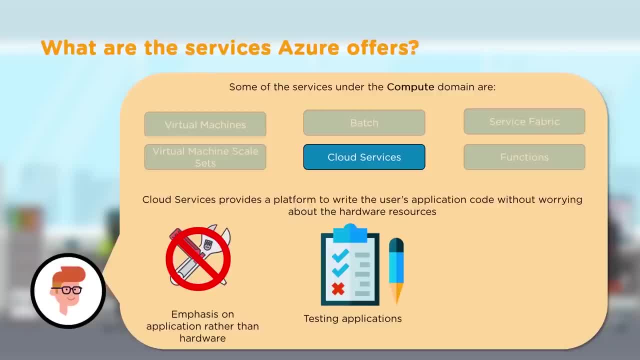 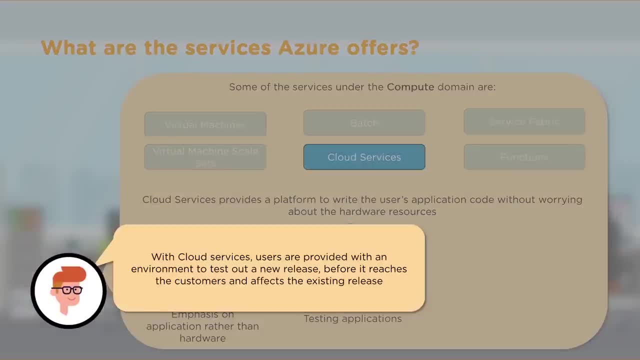 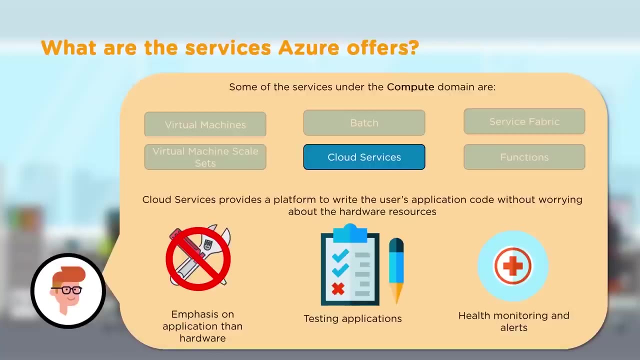 All that is handled by Azure. It also provides and good testing environment for us. You know we can simply run the code, test it before it's actually released to the production. I want to expand a bit on these testing applications. So this Azure cloud service. it actually gives us an staging environment for testing a new release without it affecting the existing release. 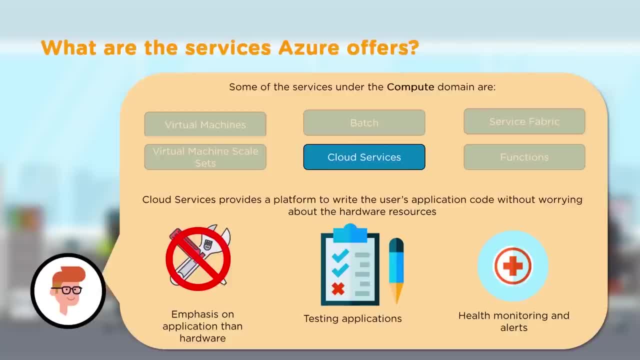 which actually reduces the customer downtime. so we can run the application tested and any time that's ready. So the production engagement is here. All that's needed for us to do to move it to production is simply to swap the staging environment into the production environment. 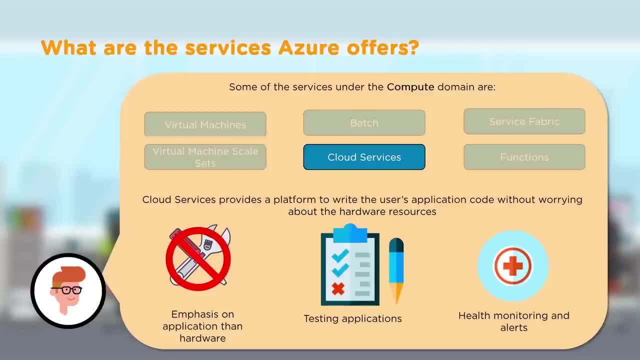 And the old production environment will now become the new staging environment, where we can add more to it and then swap it back at a later point. So it kind of gives us a swappable environment for testing our applications. And not only that, it gives us health monitoring alerts. 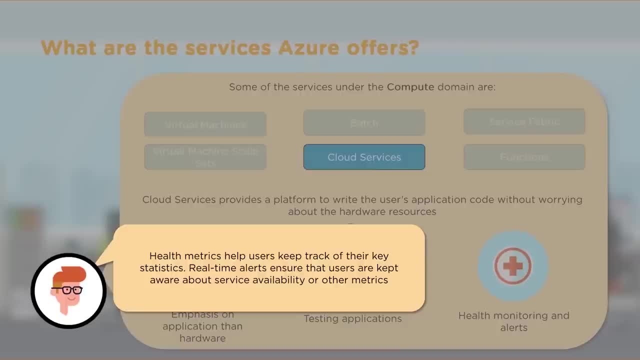 It helps us to monitor the health and availability of all our technical and technical applications, our application- and there is a dashboard we can benefit from when we use azure cloud services and that shows the key statistics all in one place, and we can also set up real-time alerts to one. 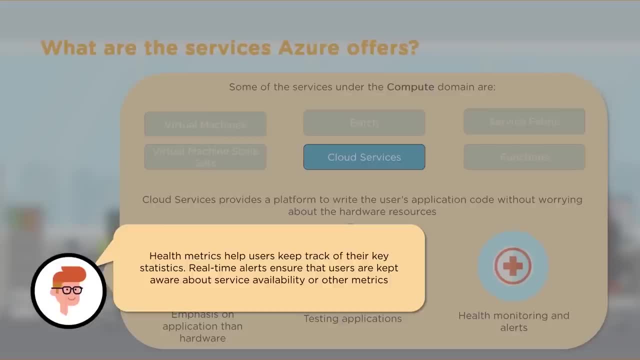 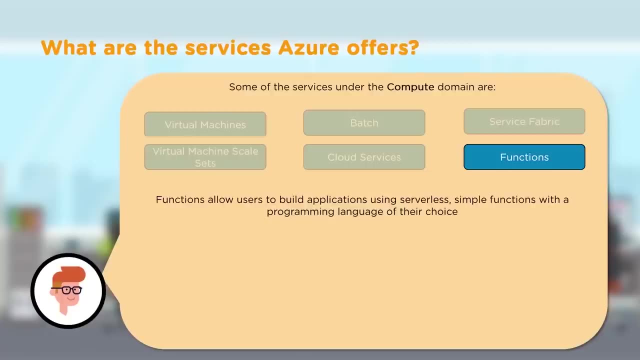 when a service availability or a certain metrics that we are concerned about degrades. as next thing in compute domain, let's talk about functions. now. functions are serverless computing now many time. if you heard about azure being serverless a lot of time they are referencing or the person who's 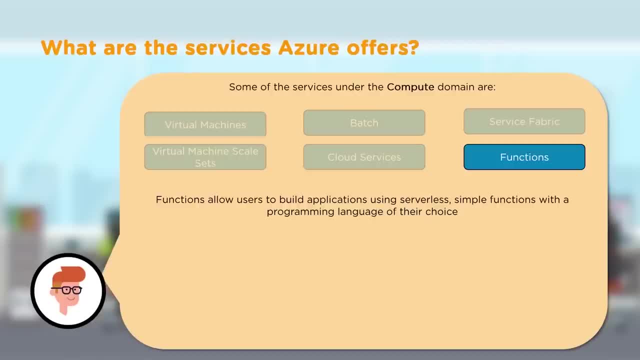 talking to you is referencing to serverless computing or azure functions, which is a serverless computing service hosted on microsoft azure. the main motive of a function is to accelerate and simplify application development functions helps us to run code on demand without we need to pre-provision or manage any azure infrastructure. 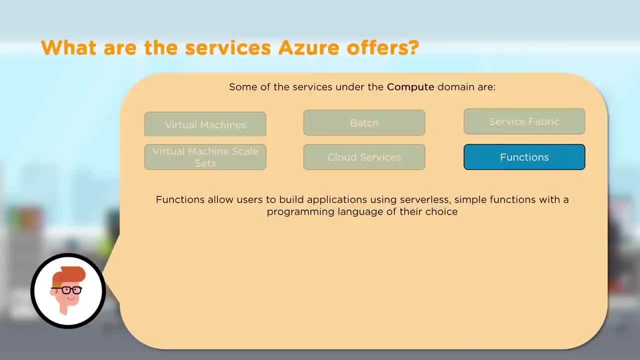 so azure functions are script or a piece of code that gets run in response to an event that you want to handle. so, in short, we can just write a code that you need for a problem at hand without actually worrying about the whole application or the infrastructure that will. 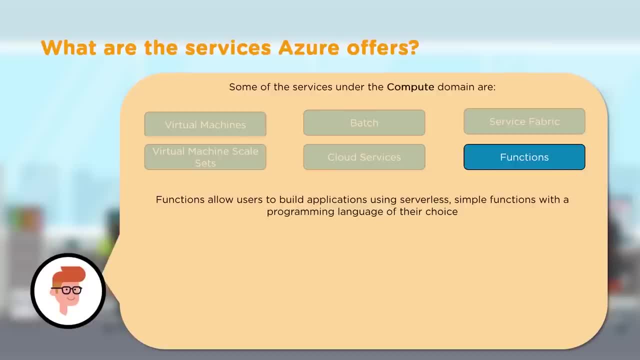 be running that code. and the best of all the best is when we use functions. we only pay for the time that our code runs. so what does functions provide, or what does azure functions provide? azure functions allow users to build applications using serverless, simple functions with the 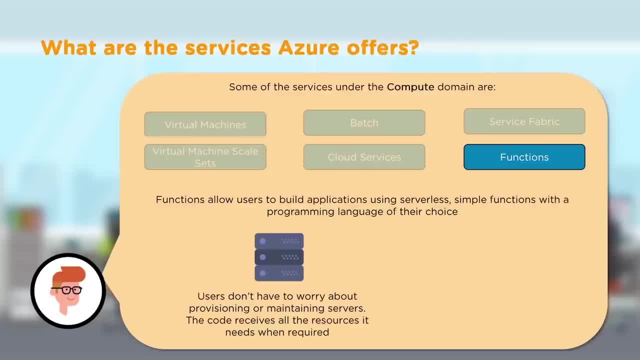 programming language of our charge. so the current programming languages that are supported is c, sharp, f, sharp node, js, the java and php. so here we really don't have to worry about provisioning or maintaining servers. if a code requires more resource, yes, azure functions handles, or it provides the additional resources needed by the court, and the best part is we only pay for. 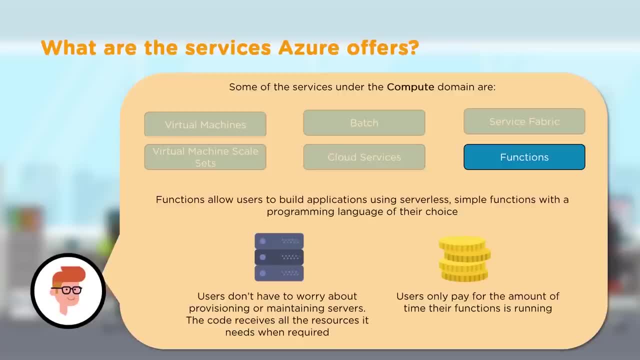 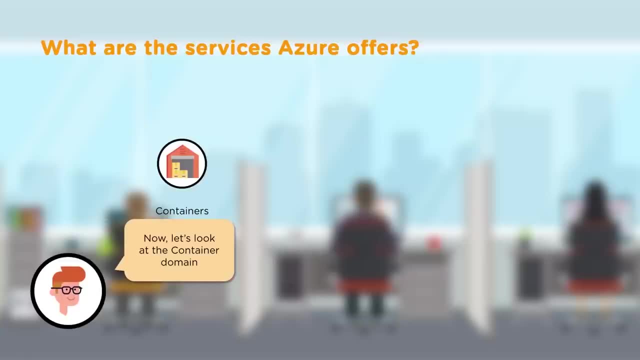 the amount of time the functions are running, not the resources, but the amount of time the function is running. as next thing, and moving to the new domain, let's talk about the container domain in azure now, the container domain or the container service. it allows us to quickly. 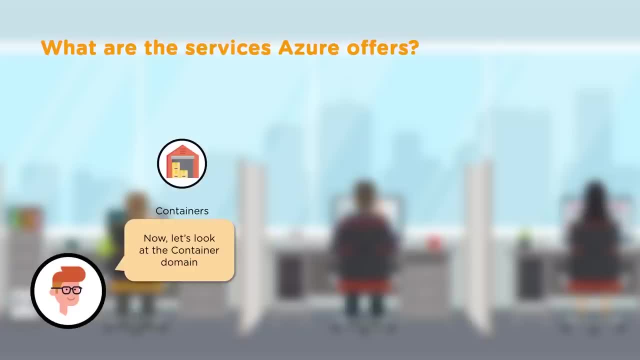 deploy a production ready kubernetes or a docker swarm cluster. now, what's a container? a container is a standard unit of software that packages of code and all its dependencies so the applications run quickly and reliably from one computing environment to another. it could be a testing to staging, to developing development environment, to staging. 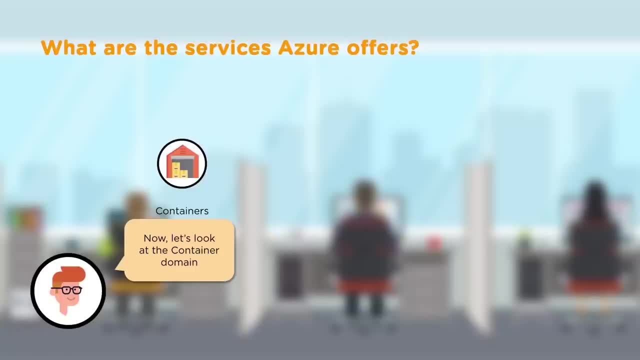 to production, or from one production to another production, or on-premises to cloud, or one cloud to another cloud, vice versa. now imagine we had an option not to worry about the vm and just focus on the application. well, that's exactly what containers helps us achieve. 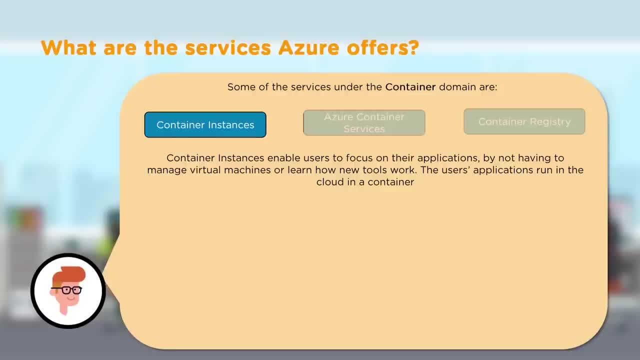 these container instances enable us to focus on applications and not worrying about managing vms or not worrying about the learning, the new tools required to manage the vms or even the deployment and our applications that we create. they run in a container. running in a container is what helps us to achieve all these not being able to manage or not needing to manage. 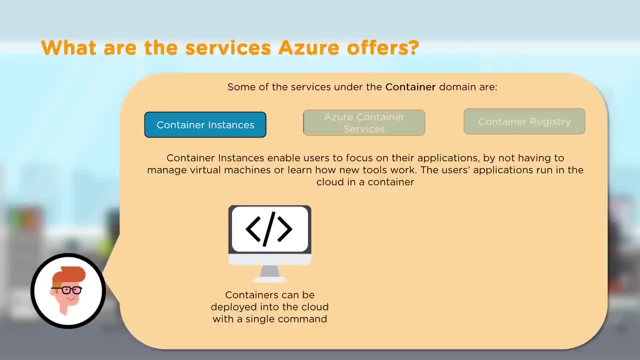 the virtual machines. so these containers, they can be deployed into the cloud using a single command, if using command line interface, and a couple of button clicks if we are using the azure portal, and these containers are kept lightweight, but they are equally secure as virtual machines. let's talk about container services. next thing, the container service, or 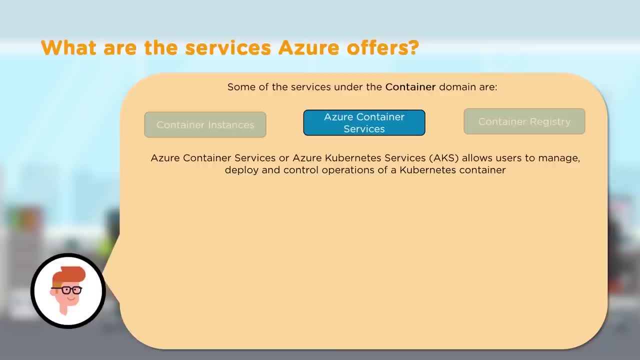 sometimes called as azure kubernetes service. it helps us to manage the containers. container is one thing and a service that's used to manage the container is another thing. at a service or acs, it helps us to manage the containers. so let's expand on this a bit. so this 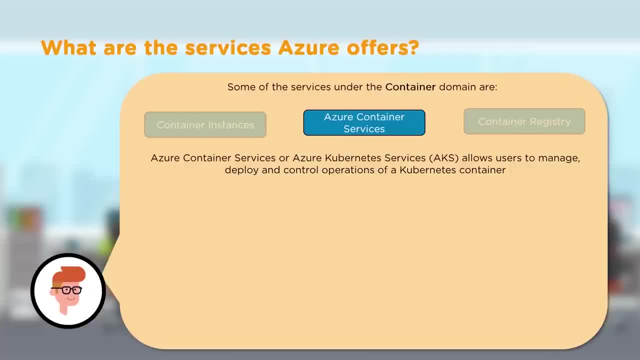 azure container service, or acs it. it actually provides a way to simplify the creation, configuration and management of a cluster of virtual machines that are pre-configured to run containerized applications on top of them and deploying them. deploying these containers might take like 15 to 20 minutes, or deploying the virtual machines that. 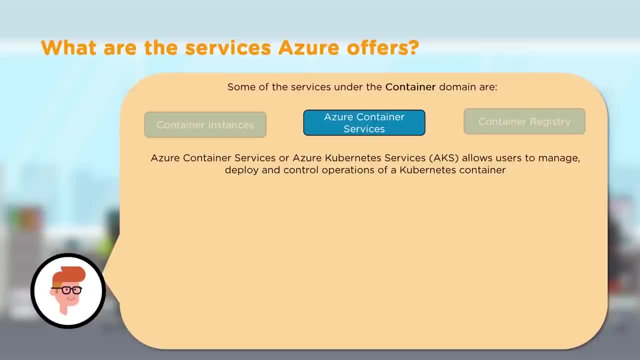 run containers in. it might take 15 to 20 minutes and once they are provisioned we can actually manage them by using simple ssh tunnel into them. and this acs when it runs application. it runs applications from docker images. what does that mean? a docker images? 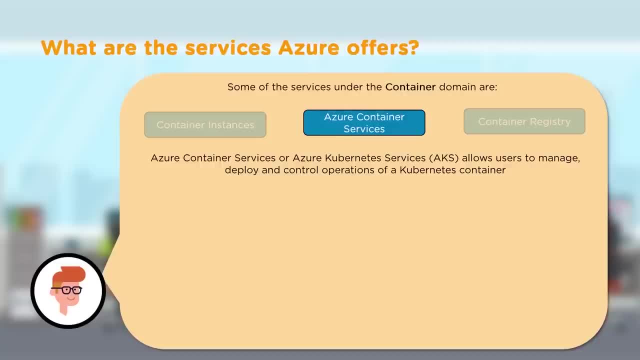 makes sure that the applications the container runs are fully portable, images are portable, and acs also helps us to ask, orchestrate the container environment. not only that, it also helps us to ensure that these applications that we run in containers can be scaled to thousands or even tens of thousands of containers. so, in a nutshell, managing an existing application. 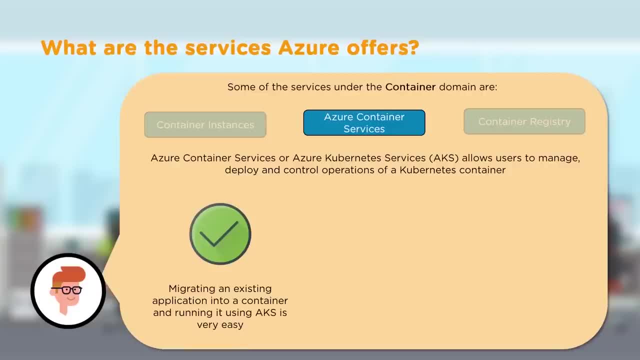 into a container and running it using aks or acs is really easy, or that's what it is all about: to make the application management or migration easy. now managing the container based architecture- and we discussed that containers could be tens or even tens of thousands of containers, so managing them is made simple using this, container services and even training. 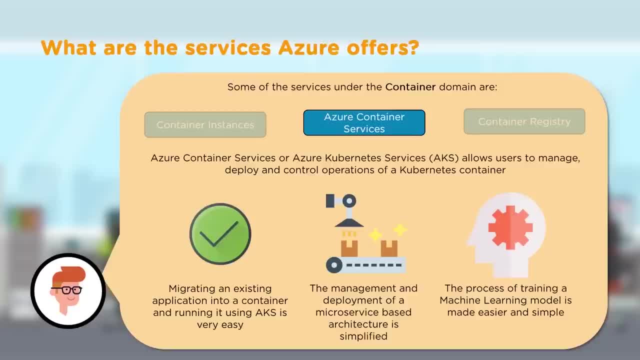 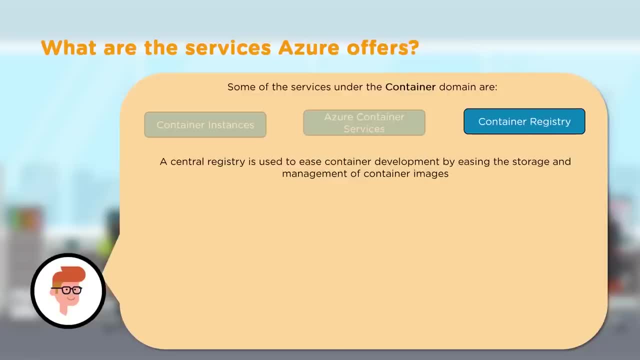 of model using a large data set in a complex and resource intensive environment. this aks helps us to simplify that environment. all right, as next thing in container domain, let's talk about container registry. we spoke about registry a little bit when we spoke about docker images, so 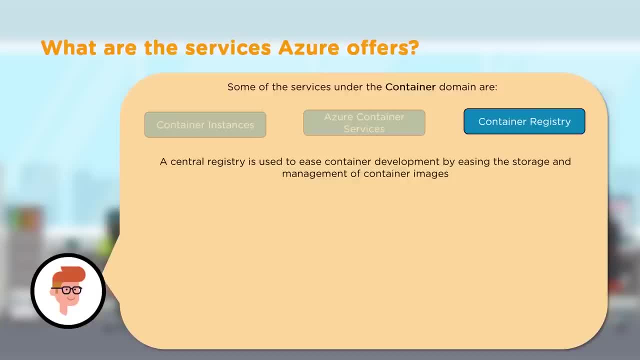 container registry is a single place where we can store our images, which are docker images. when we use, when we use containers, it's it's docker images that we use for our image purposes. so these container images are a central registry that can be used to ease container development by easing the storage and management of container images. so there we can. 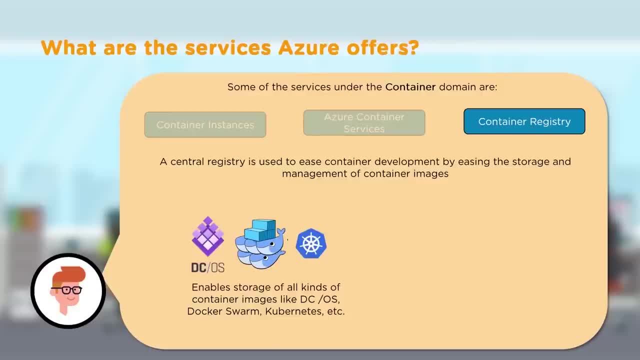 store all kind of images like docker swarm, or the images used in docker swarm are in kubernetes. everything can be stored in container registry in azure now, anytime we store a container image, it provides us an option for geo replication. what that means is that we can efficiently manage a single 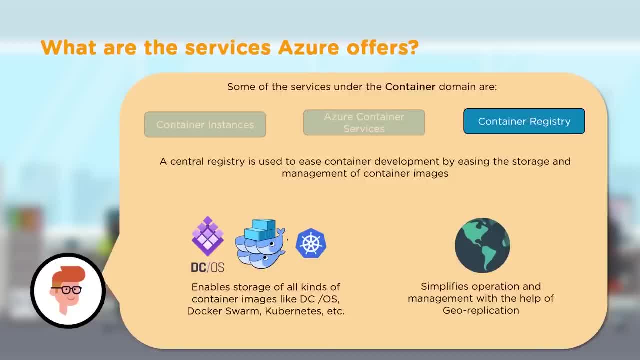 registry replicated across multiple regions. now, these geo replication, it actually enables us to manage global deployments, assuming we are having an environment that requires a global deployment. so it helps us to manage global deployments as one of the major challenges of the docker version. so, entity, because we are geo replicating, we would be updating, we would be editing one image and 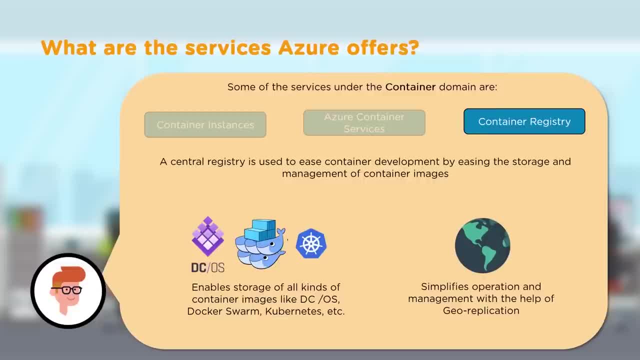 that image gets replicated throughout the global replication centers we would have set up and so just one editing would have actually edited the global images and those global images would have provisioned at the global application. so one edit, replication and then provisioning of the applications global wide. and this replication also helps us to helps us network latency. 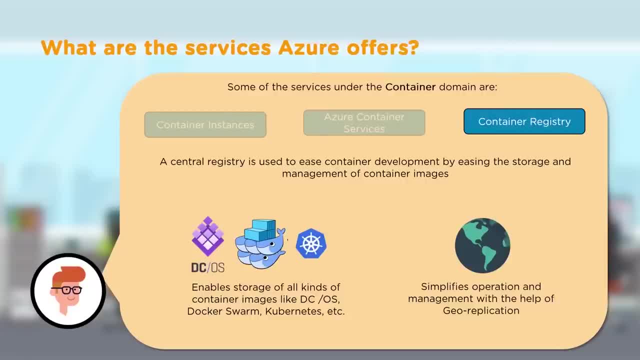 because you know any time an application needs to deploy, it does not have to rely on a single source which which can be reached only through high latency network, because we have global replications around the world. any time the application wants to check back, it would check back the application which is in a very nearby location, for the application itself global. 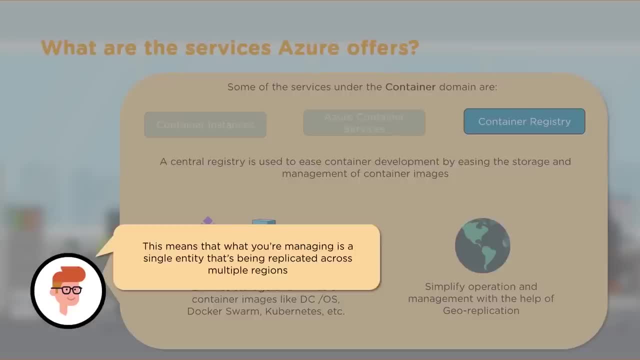 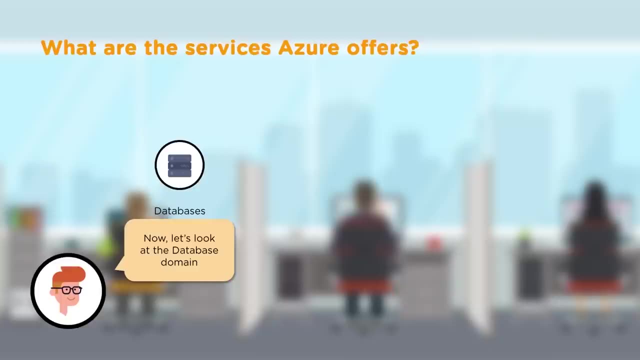 replication. Replication means that we are managing it as a single entity that's being replicated across the multiple regions in the globe. As next thing in a learning, let's talk about Azure databases. Now, these Azure databases are rational. In fact, they have many flavors in them. 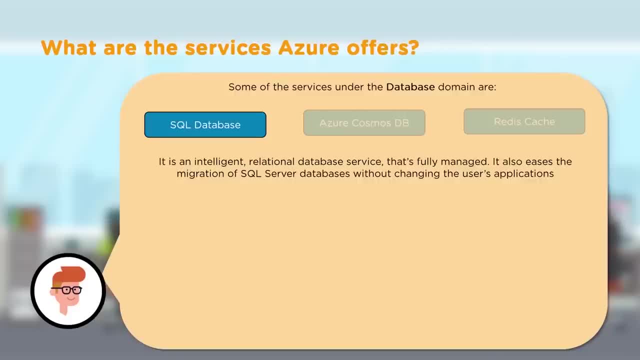 We're going to look at different flavors of SQL, NoSQL cache- type of database that Azure offers. So we're going to learn one at a time or we're going to learn one by one. So this Azure SQL database is a rational database. 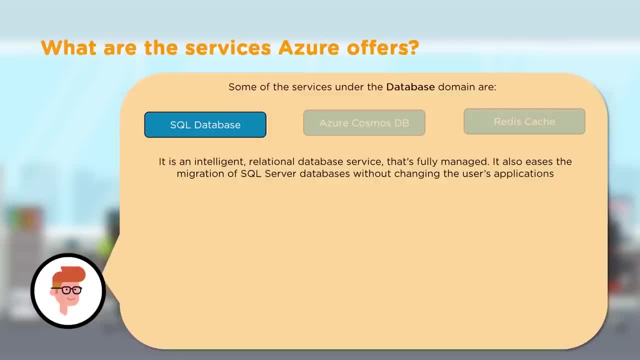 In fact, it's a rational database as a service. It's managed by Azure. We don't get to do a lot of management in it. so it's a rational database as a service based on Microsoft SQL Server Database Engine, And this database is a high-performance database. 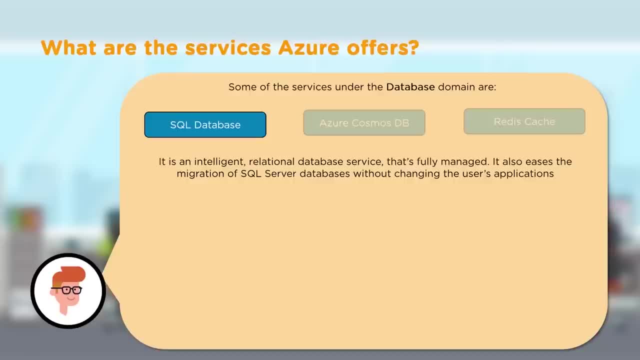 It's very reliable and it's very secure as well. And this high reliability, High performance and for this high security, we really don't have to do anything. It comes along with it and it's managed by Azure, And there are two things that I definitely need to mention about Azure SQL Database. 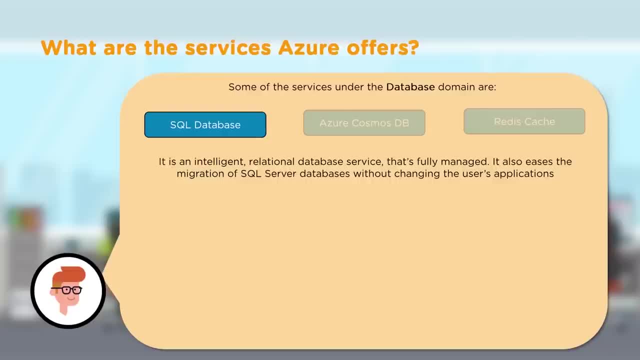 That is, it's an intelligent service Number one. it's fully managed by Azure And it also has this one good thing, which is it has built-in intelligence that learns app patterns and adapts to maximize performance and reliability and data protection. 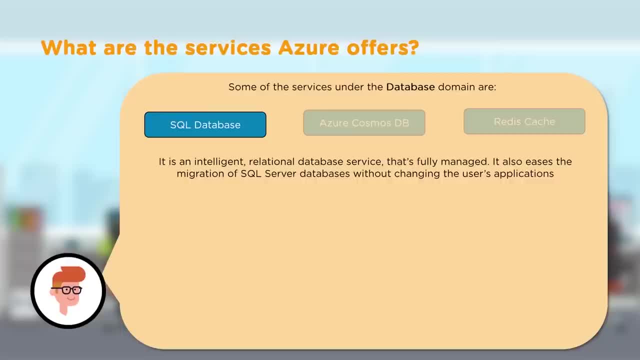 That's something that's not found in many of the other cloud providers that I'm aware of, so I thought I'll mention it. So it uses built-in intelligence to learn about the user's database patterns and helps improve performance and protection, And migration or importing data is very easy when it comes to Azure SQL Database. 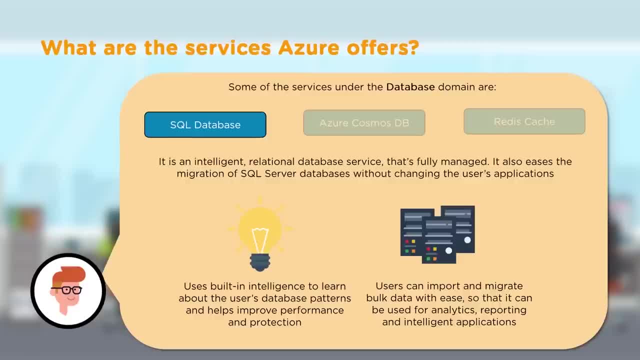 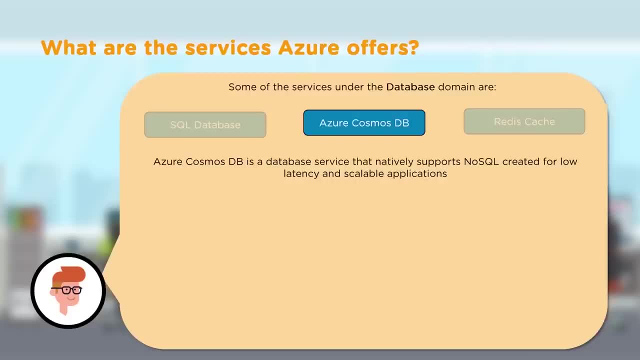 So it can be readily or immediately used for analytic reporting and intelligent reporting. So it can be readily or immediately used for analytic reporting and intelligent reporting. So it can be readily or immediately used for analytic reporting and intelligent reporting. As next thing, let's talk about Azure, Cosmo DB. 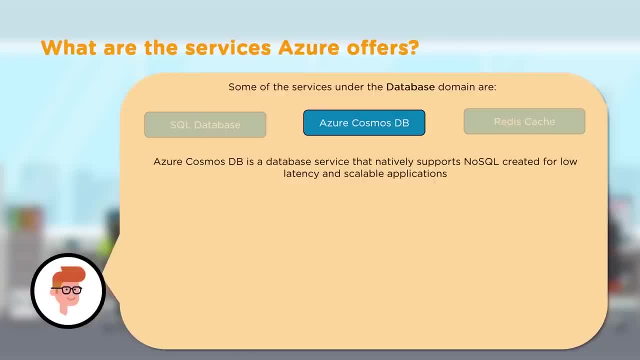 Now Azure Cosmo DB is a database service that is for NoSQL type And it's created to provide low latency and an application that scales dynamically or that scales rapidly. Now this Azure Cosmo DB is a globally distributed service and it's a multi-modal database. 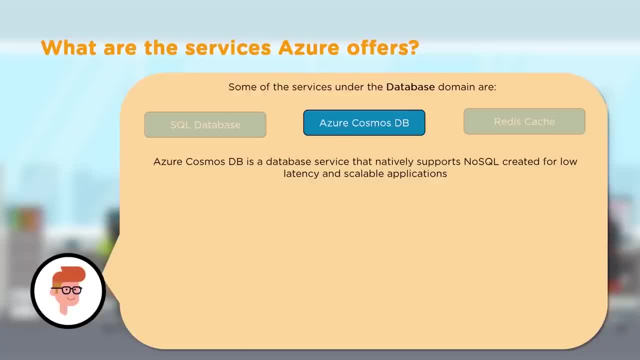 This can be provisioned in a click of a button. That's all we got to do. if we need to provision an Azure Cosmo DB in the Azure, It helps with scaling the database. Now we can elastically and independently scale throughput and storage across this database and in any of the Azure geographic regions. 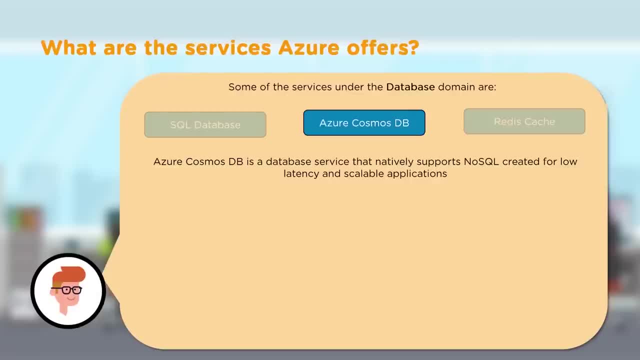 It provides a good throughput, It provides good latency, It provides good availability and it provides- or Azure promises- a comprehensive SLA that no other database can offer. That's the best part about Cosmo DB. So this Cosmo DB was built with global distribution in mind, and it's built with the horizontal scale in mind. 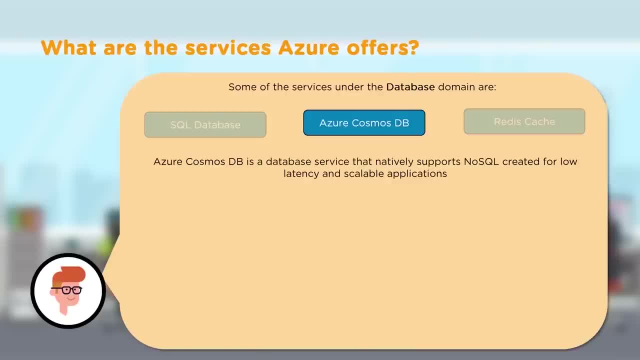 And all this we can use by only paying for what we have used. And remember, the difference between Azure Cosmo DB and the SQL database is that Azure Cosmo DB supports NoSQL, whereas SQL doesn't. All right, A few other things about Azure Cosmo DB, is it? 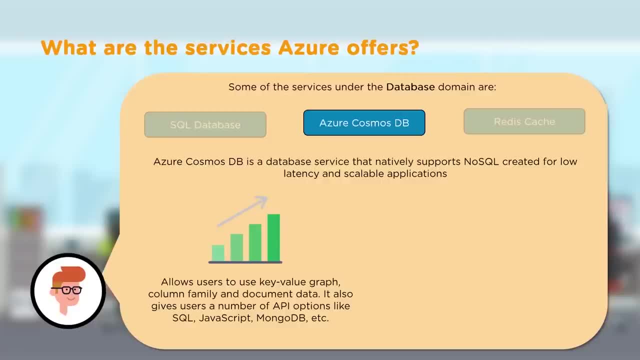 allows users to use key value, graph, a column, family and document data. It also gives users a number of API options like SQL, JavaScript, MongoDB and a few others that you might want to check in the document at the time of reading. 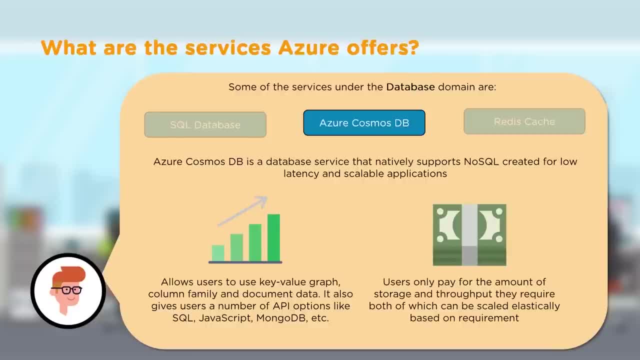 And the best part here is that all that we mentioned we get to use only by paying for the amount of storage and throughput that are required, And the storage and the throughput can be elastically scaled based on the requirement of that. All right, Let's talk about Redis. 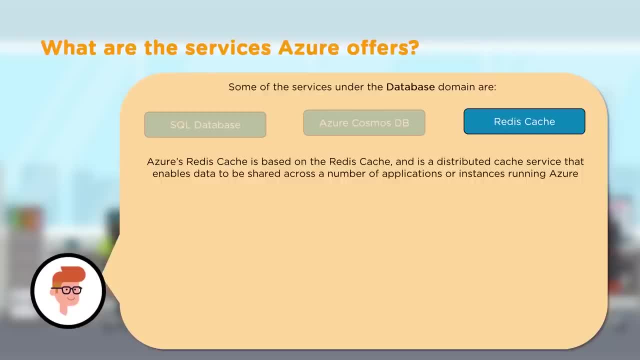 Cache. discussion about Azure database won't be complete without we talking about Redis cache Now, Redis cache is a secure data cache. It's also called- it's also sometimes called- as messaging broker that provides high throughput and low latency access to data for the applications. 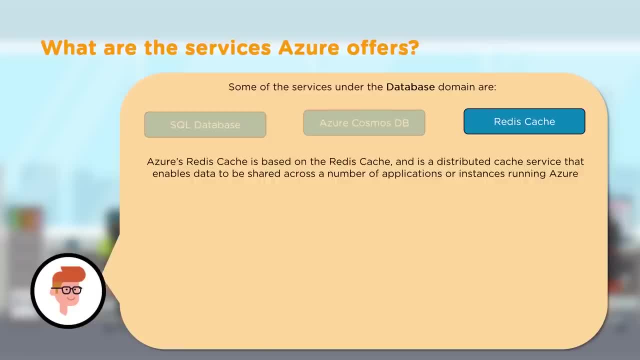 Now, Redis cache is based on a popular open source caching product, which is Redis, sometimes called as Redis cache. Now what's the use case? It's typically used to cache to improve performance and scalability of a system that rely heavily on back end data stores. 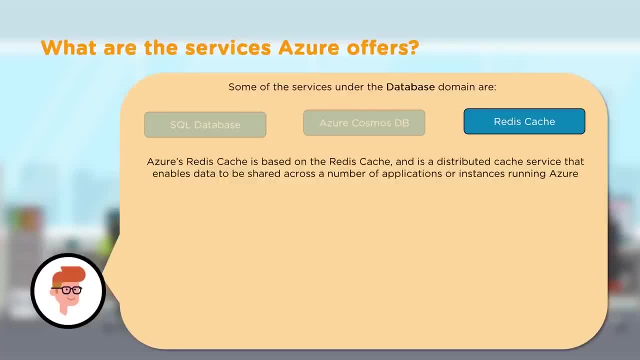 Now performance when we use Redis cache is improved by temporarily copying the frequently accessed data to a fast storage located very close to the application. Now, with Redis cache, this fast storage is located in memory with Redis cache instead of being loaded from the actual disk in the database itself. 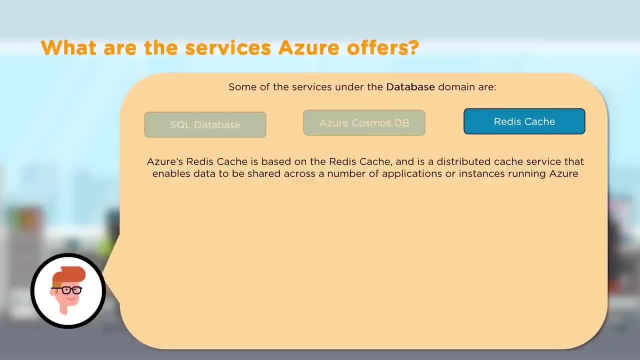 Now this Redis cache can also be used as an in-memory data structure. Not only that, it can be used as a distributed non-relational database and a message broker. So there are a variety of use cases for this Redis cache. And by using Redis cache, the application performance is improved by taking advantage. 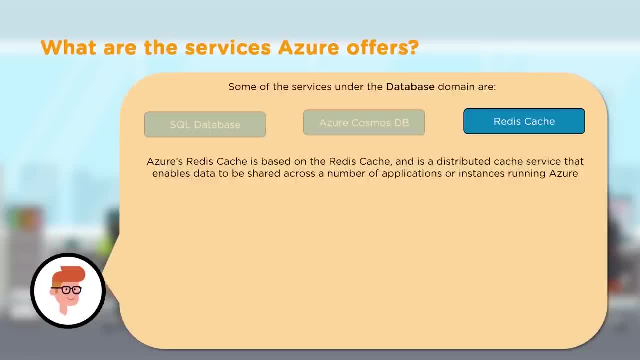 of the low latency and the high throughput performance that this Redis cache engine provides. So to summarize this Redis cache: when we use Redis cache, data is stored in the memory instead of the disk to ensure that there is high throughput and low latency when the application needs to read the data. 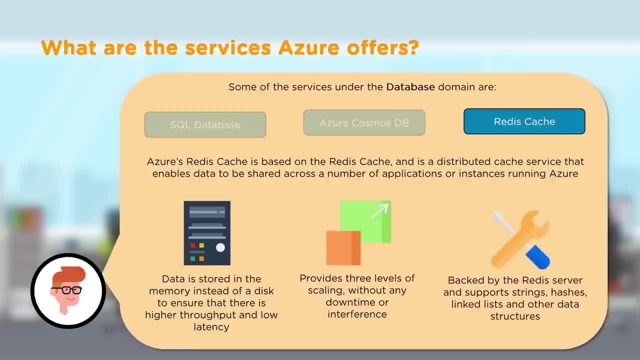 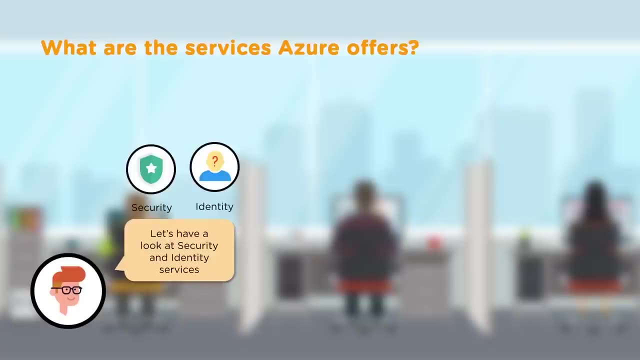 It provides various levels of scaling without any downtime or interference. Now this Redis cache is actually backed by Redis server and it supports a string hashes linked list and various other data structures. Now let's talk about security and identity services. Now, identity management in specific is a process of authenticating first and then. 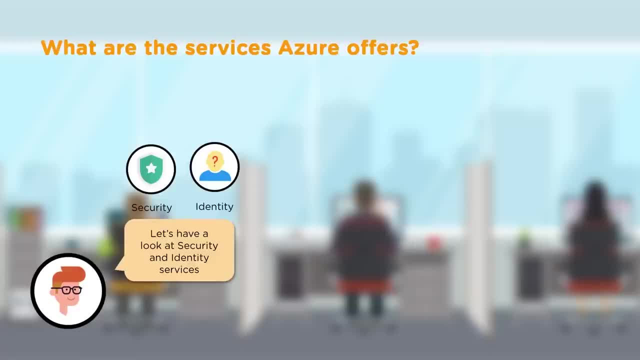 authorizing, using security principles. And not only that: identity management involves controlling information about those principal identities. You might ask now, what's a principal identity? Now, identity or principal identity are services, applications, users, groups and a lot more. 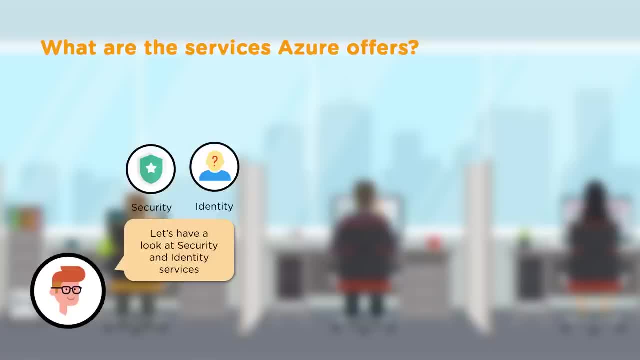 The speciality about this identity management is that it not only helps authenticate and authorize principles in cloud, it also helps authenticate and authorize principles or resources on premises, especially when you run a hybrid cloud environment. So all these services and features that this identity management helps us to get. 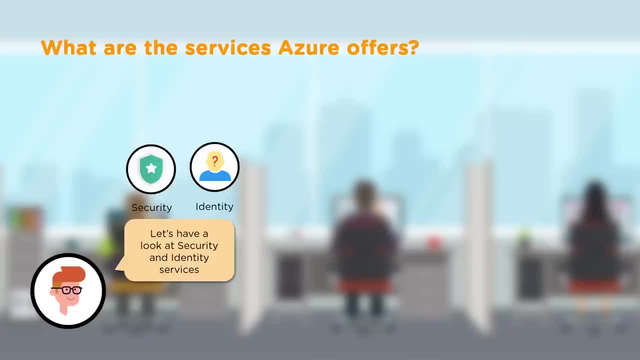 additional level of validation, like identity management, can provide multi-factor authentication. it can provide access policies based on condition- a permit or deny based on condition. It can also monitor suspicious activity, And not only that, it can also report it. It can also help generate alerts for potential security issues and, in a way, 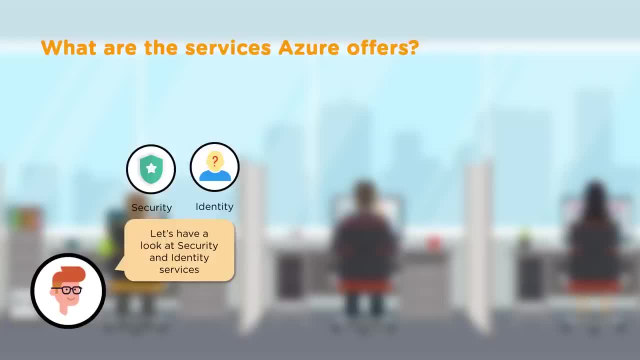 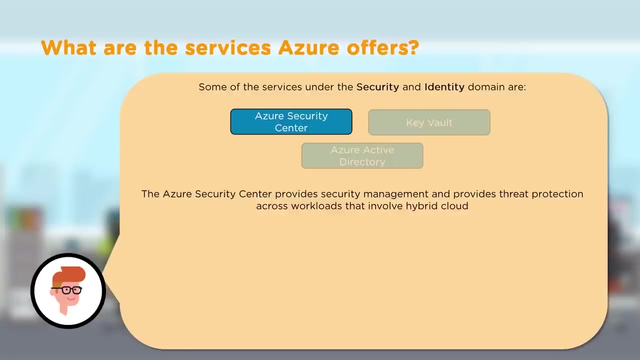 to mitigate. it can send us an alert so we can get involved and prevent a security accident from happening. So let's talk more about identity management. So some of the services under security and identity management are Azure Security Center. Now this Azure security. 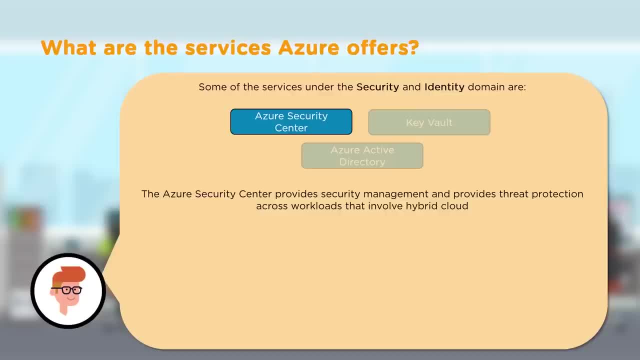 center provides security management and threat protection across the workloads in both cloud and in the hybrid environment. It helps control user access and application control to stop any malicious activity, if present. It helps us to find and fix vulnerabilities before they can be even exploited. It integrates very well with analytic 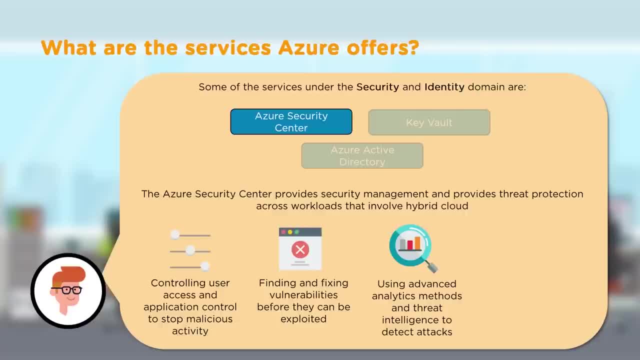 methods that helps us to identify, or it gives us the intelligent tools to identify or detect attacks and prevent them before it can actually happen. And it also works seamlessly with hybrid environments, So you don't have to have one policy for on premises and one policy for the cloud. 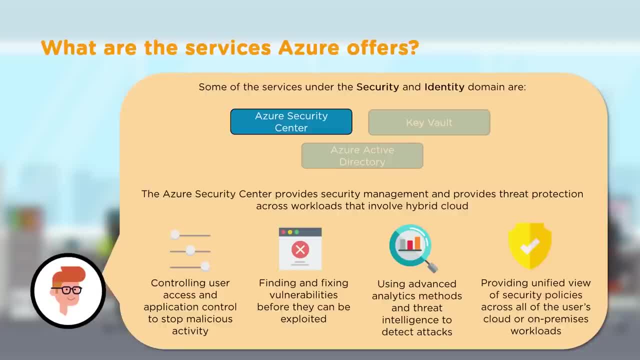 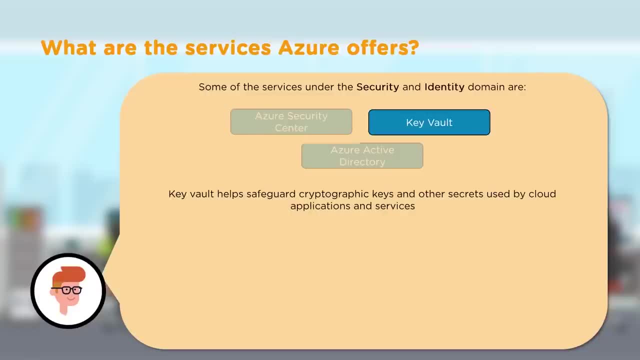 It's now a unified service both for on premises and the cloud. The next service in security and identity would be Key Vault. Now, Key Vault is a service or a feature that helps safeguard the cryptographic keys And any other secrets used by the cloud applications and the services. 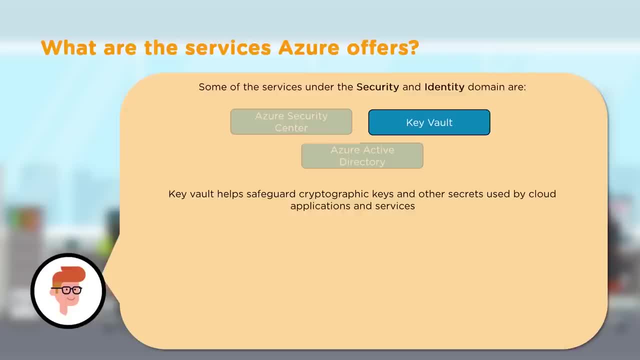 In other words, this Azure Key Vault is a tool for securely storing and accessing the secrets of the environment, I mean the secret keys. Now, a secret is anything that you really want to have a very tight control access like the certificates, like the passwords, stuff like that. 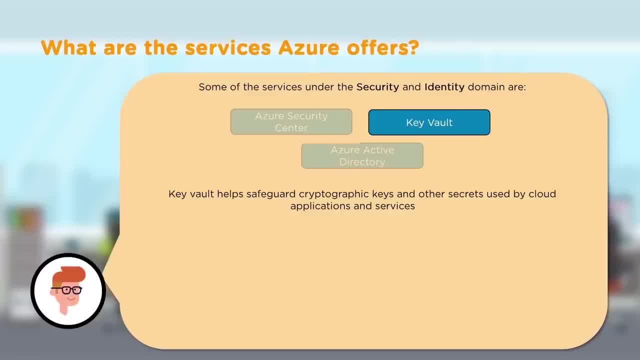 Now, if I tell you what Key Vault actually solves, that would actually explain what Key Vault is Now. Key Vault is used in secrets management. It's helped in securely storing the tokens, the passwords, the certificates. It helps in key management and it really 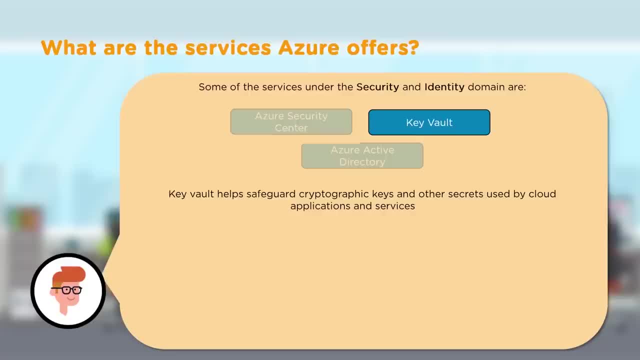 helps in creating and controlling the encryption keys that we would use to encrypt data. It helps in certificate management. Talking about certification management, it helps us to easily provision, manage and deploy public and private SSL TLS certificates. It's in Azure and a lot more. 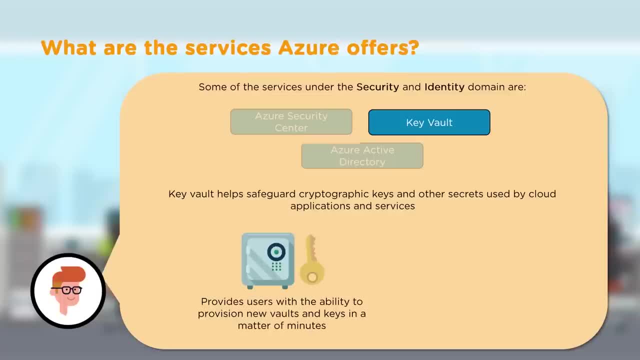 So, in a nutshell, this Key Vault. it provides users the ability to provision new vaults and keys in just a matter of minutes, All that in a single command, or all that in a couple of button clicks. It also helps users to centrally manage their keys, secrets and policies. 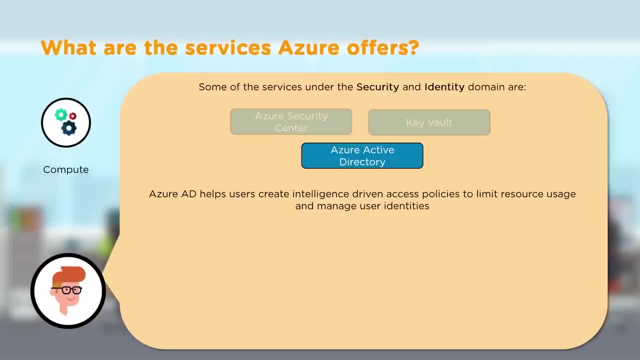 Next in the list, let's talk about Azure Active Directory. Now, Azure Active Directory. it helps us to create intelligent and driven access policies to limit resource usage and manage user identities. But what does that mean? Now, this Azure Active Directory is a cloud. 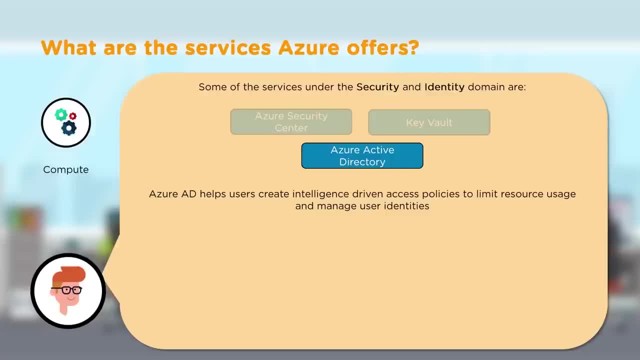 based Active Directory and identity management service. Now Azure Active Directory combines- and it's actually a combination of the core directory services plus application access management, plus identity protection. And one good thing about this Azure- in fact, there are a lot of good things. 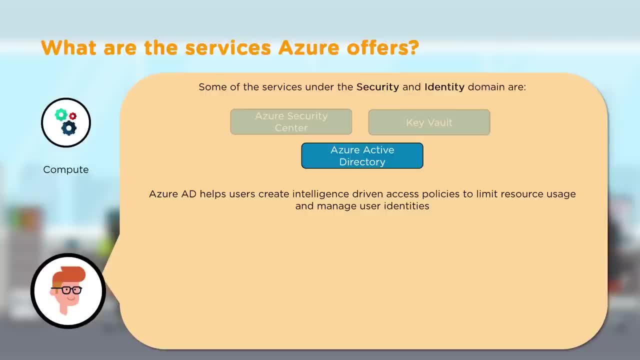 but especially when you're running hybrid environments, you might wonder well how this Azure Active Directory is going to behave. Now, this Azure Active Directory is built to work on on premises and cloud environment as well. Not only that, it also works seamlessly with mobile applications as well. 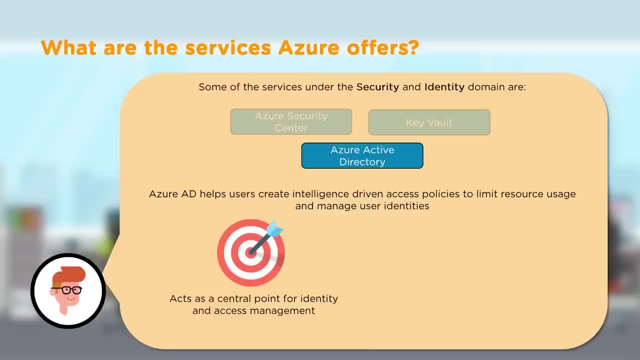 So, in a nutshell, this Azure Active Directory. it acts as a central point of identity and access management for our cloud environment. It also provides good security solutions that protect against unauthorized access of our app and the data. Now that we've discussed about security and identity, 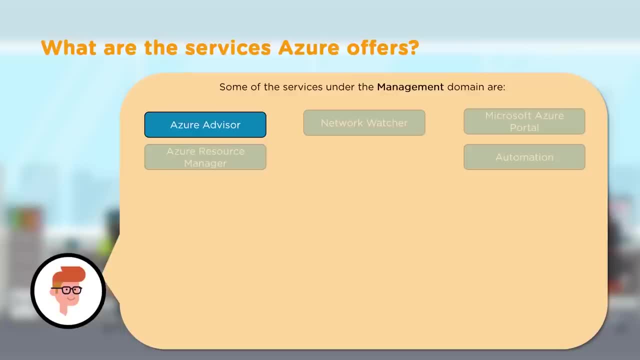 let's talk about the management tools that Azure has to offer. Azure provides built in management and account governance tools that helps administrators and developers, that helps them to keep their resources secure and very compliant And, again, it helps both in on premises and in the cloud environment. 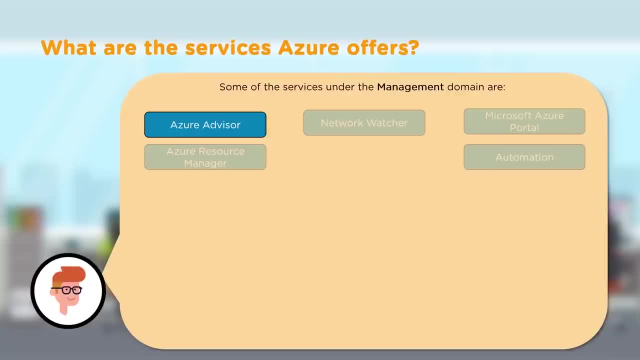 And these management tools help us to monitor the infrastructure, monitor the applications. It also helps in provisioning and configuring resources. It also helps in updating apps. It helps in analyzing threats, taking backup of the resources, build disaster recoveries. It also helps in applying policies and conditions to automate our environment. 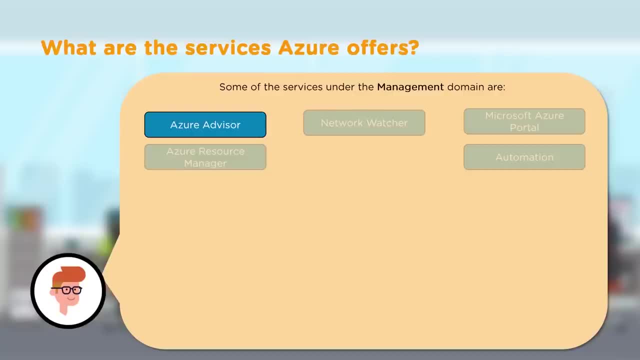 We use Azure management tools and it's also used in cost control methods. So this Azure management plays a wide role across the Azure services And in the management tools. first comes the Azure Advisor, Now this Azure Advisor. it acts as a guide to educate us about Azure best practices. 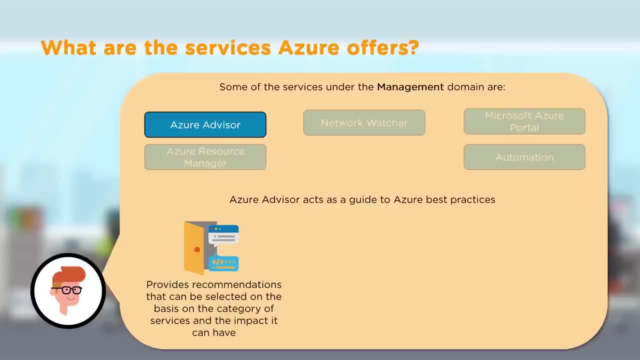 It throws recommendations that we can select on the basis of the category of service And it also provides the impact It can have or the impact that would happen in our environment if we follow the recommendations given. and recommendations- or first one is the recommendations- are kind. 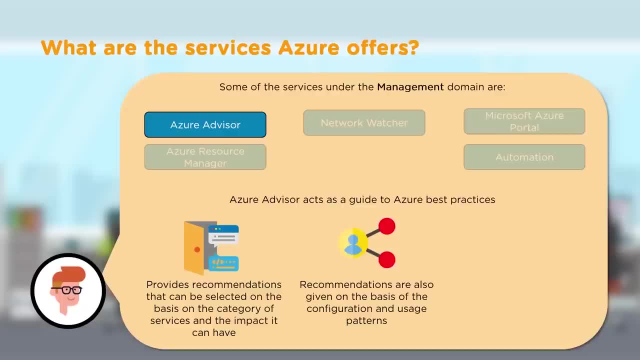 of templatized and it throws the templatized recommendations. Not only that, it also provides customized recommendations on the basis of the configuration, on the basis of our usage patterns, And these recommendations are not hard. It's not like something that it recommends. 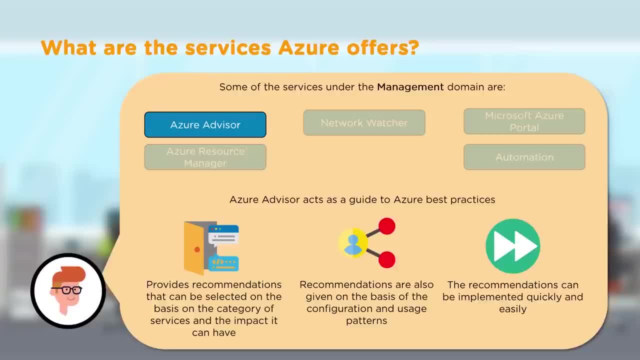 And then just leaves us hanging there. These recommendations provided are very easy to follow, Very easy to implement and see results. You can think of Azure Advisor as an very personalized cloud consultant that helps you to follow best practices to optimize our deployments. It kind of analyzes our resources, our configurations, our usage. 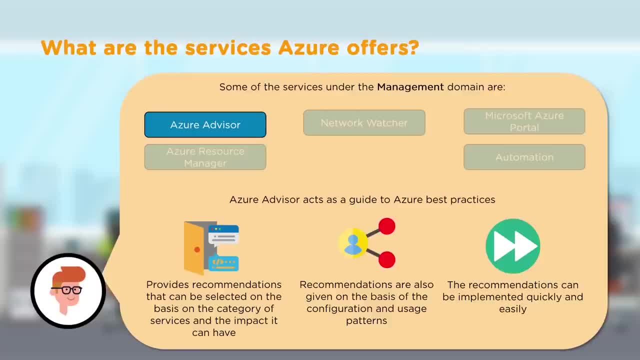 And then it recommends a solution for us that really helps in improving the cost effectiveness, improving the performance, improving high availability and improving security in our Azure environment. So with this Azure Advisor, we can get a proactive, actionable and personalized best practice recommendations. 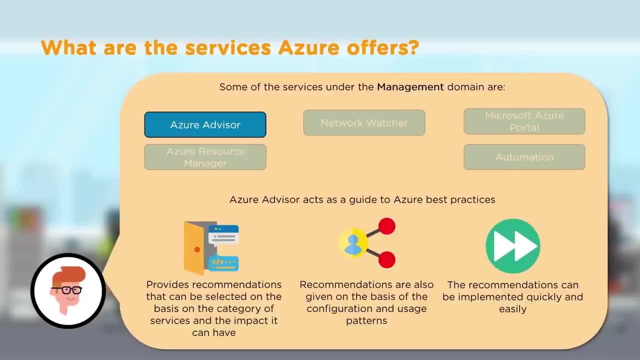 Now you don't have to be an expert. Just follow the Azure Advisor and your environment is going to be good. It also helps and improve the performance, security, high availability, of our environment And also it helps in bringing down the overall Azure spend. 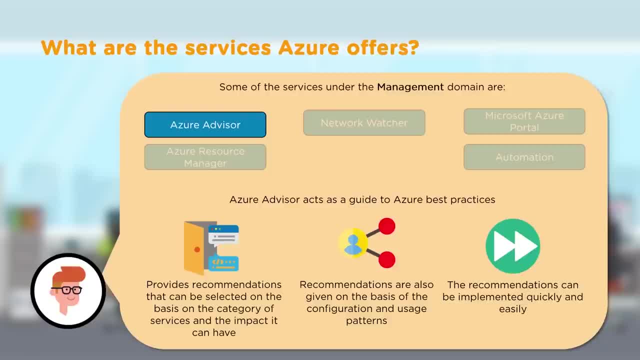 And the best part is it's a free service that analyzes our Azure usage and provides recommendations how we can optimize our Azure resource to reduce cost and reduce cost at the same time, boost the performance, helps in strengthening the security and improve the overall reliability of our environment. 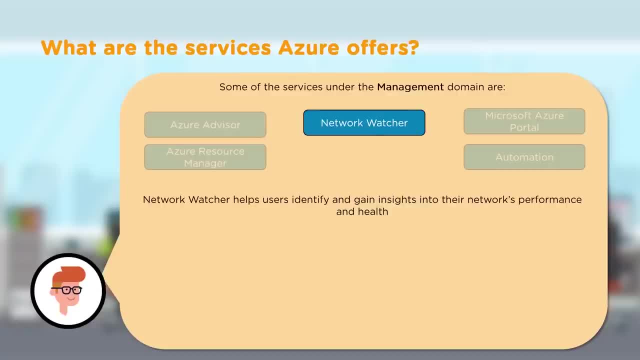 And next in the list would be Network Watcher. Now this Network Watcher helps users identify and gain insights in the overall network performance and the health of the overall environment. Now these Azure Watchers provides enough tools to monitor, to diagnose, to view the metrics and to enable or disable logs. 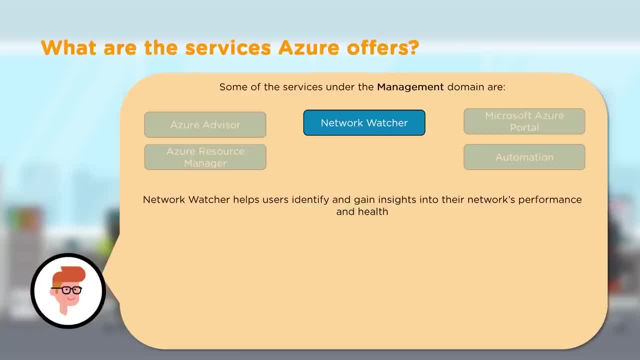 which means to generate and collect the logs for resources in the Azure virtual network. So with Network Watcher, you can monitor and diagnose issues in networking without even logging into the virtual machines. with just the logs, which are real time, we can actually come to a conclusion. what could be wrong in a 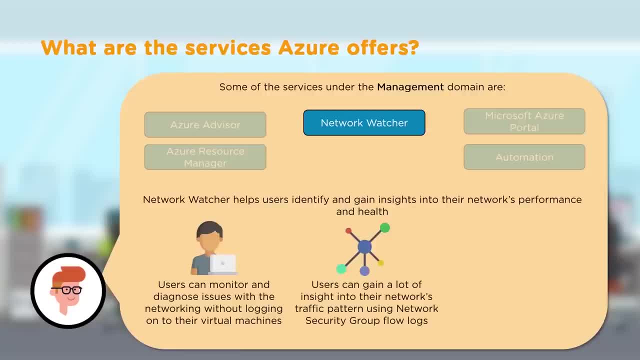 certain resource in a VM or in a database, you know. but just looking at the logs- And not only that, it's used for analytic or to gain some intelligence of what's happening in our network- we can gain a lot of insight to the current network. 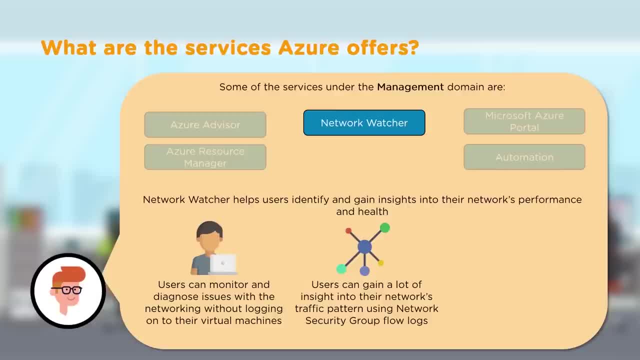 traffic pattern using the security group flow logs that this Network Watcher offers. It also helps in investigating VPN connectivity issues using detailed logs. Now, you might or might not know that you know VPN troubleshooting requires both parties or it involves two parties. you know. 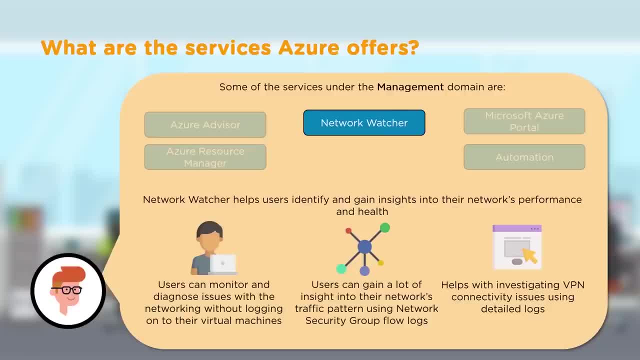 the person- the network administrator on this side and the network administrator on the other side, and they will have to check logs on their end and we'll have to check logs on our end and stuff like that. But with the Network Watcher it kind of takes it to the next level. 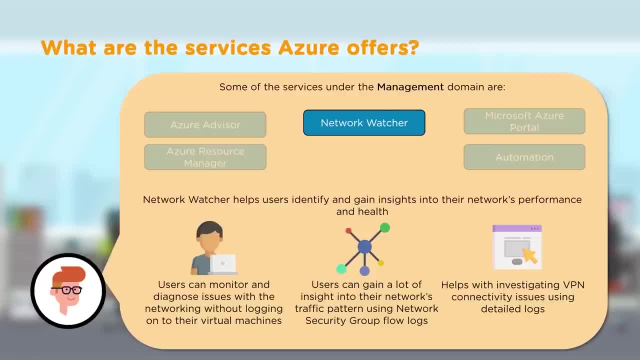 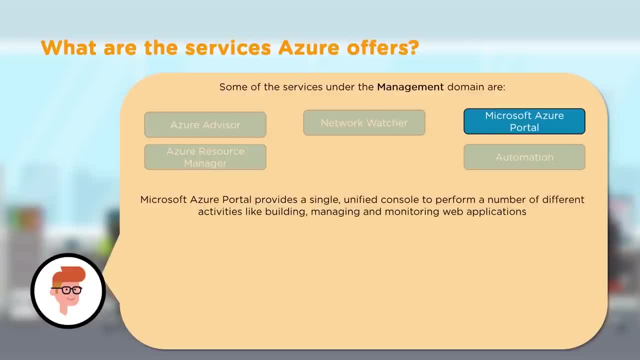 So with the logs itself, we could easily identify which side is having the issue and suggest an appropriate fix. And the next in the list would be Microsoft Azure Portal. Now, this Microsoft Azure Portal: it provides a single unified console to perform various number of activities like building- not only building. 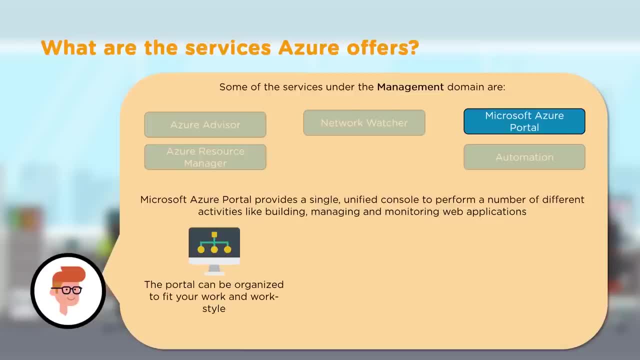 managing and monitoring the web applications that we build. Now this portal can be used to organize our environment, Or the appearance of the environment or the visual of the environment, based on our work style, and, using Azure portal, users can control who gets to manage. 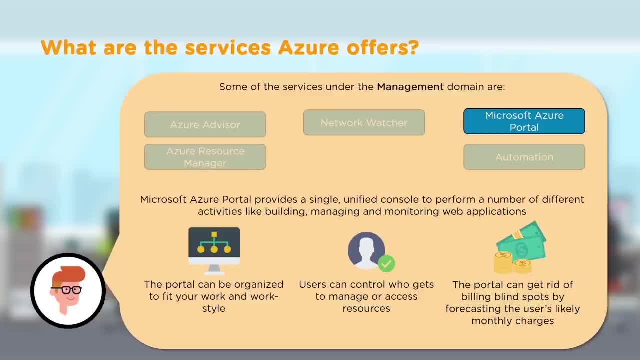 or access the resources all from the Azure portal. And this Azure portal gives a very good visibility on the spends that happen on each resource Right, And, if we can customize it, we can also identify spends based on team, spends based on days, spends based on hours. 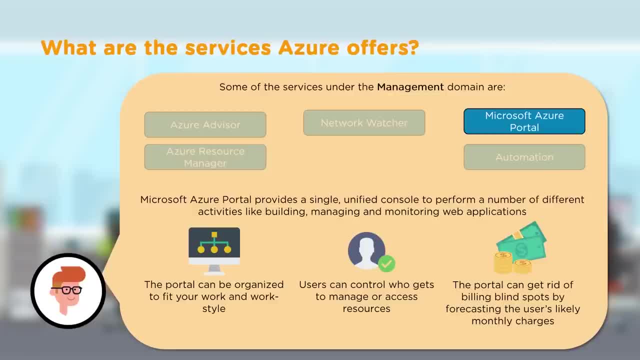 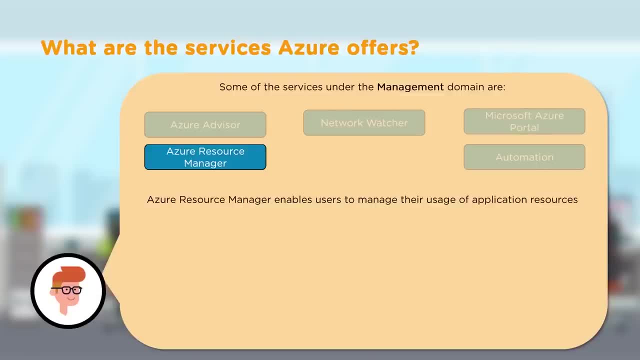 Based on department stuff like that, So it kind of gives us a good visual of where the money is spending or where is the bill consumed within the Azure environment. Next in the list would be Azure Resource Manager. Now, Azure Resource Manager enables us. 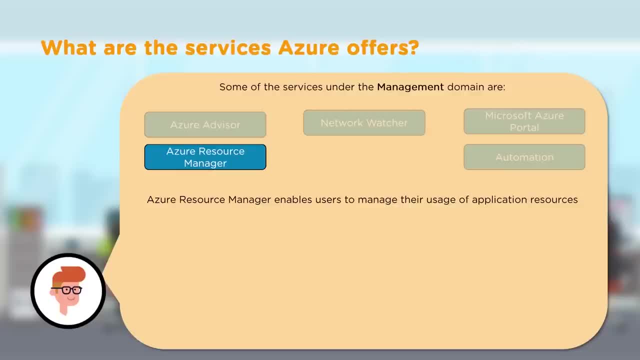 to manage the usage of the application resources. Now we use Resource Manager to deploy, monitor and manage solution resources as a group, as if it's one single entity. Now, the infrastructure of our application is typically made of various components, which includes virtual machine storage, virtual network, web app database servers. 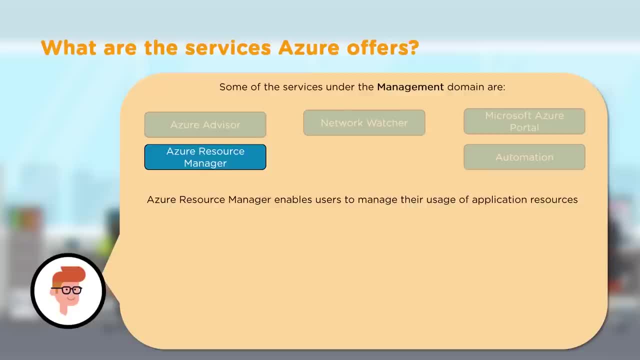 some other third party services that we might use in our environment And they are, by nature, separate services, But with Azure Resource Manager, we don't see them as different components or different entities. Instead, we see them as related to services in a group that supports an application. 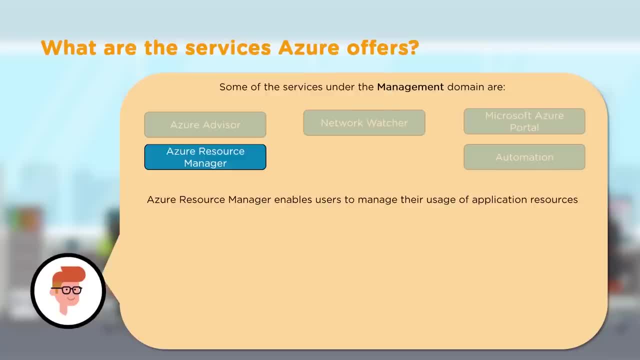 Now we kind of get the relation between them instead of letting them spread. Azure Resource Manager identifies the relation between them and helps us to visually see them all as one or single entity. Not only that Azure Resource Manager helps, or it ensures that the resources 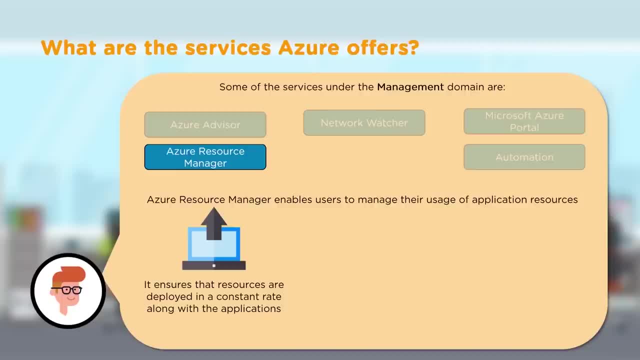 that we provision are deployed at a constant rate. along with the other application, It also helps users to visually see their resources and how they are connected, And that helps in managing the resources a lot better. Resource group also is used to control who can access the resources within. 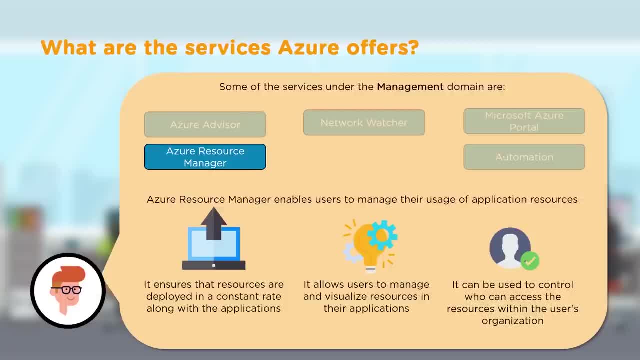 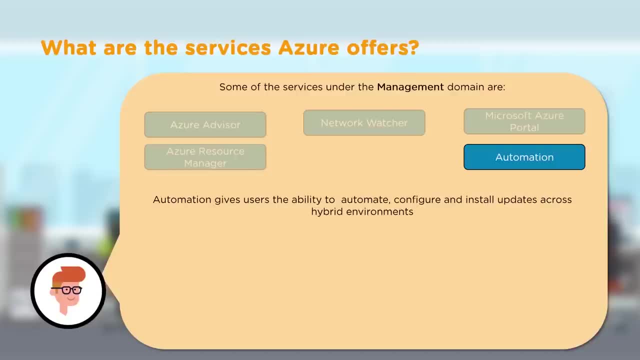 the user's organization kind of gives you the fine grained control over who gets to access and who does not get access. And the last one in the management tools would be automation, And this automation gives us the ability to automate, configure and install upgrades across hybrid environments. 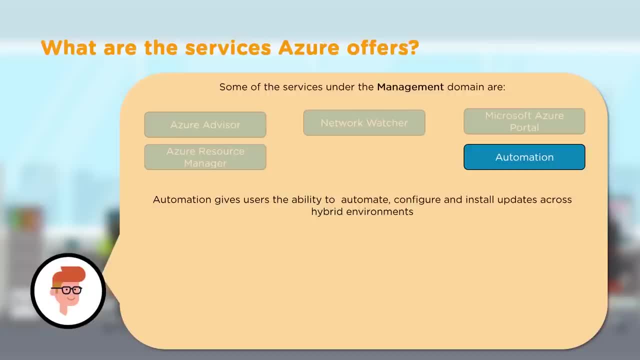 It provides a cloud based automation and configuration service. Not only that, this can be applied for non-Azure environments as well, which is on premises. So some of the automation we could do is process automation, update management, automation, configuration features, automation, stuff like that. 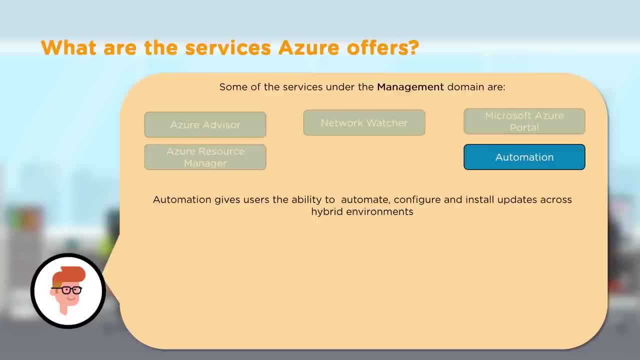 And this Azure automation provides complete control during the deployment automation and also during the decommissioning of the workloads and resources. With automation we can actually automate time consuming or mundane or any task that's error prone because of human errors. Those things can be automated. 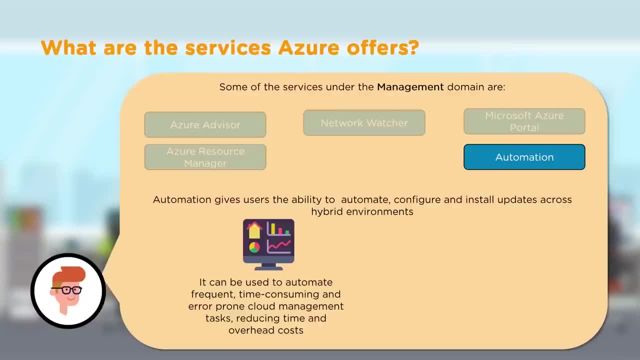 So irrespective of how many times you run it, it's going to run the same way, And that really helps in reducing the overall time and also the overhead cost, because a lot of the things are automated, Which means it's human error free. 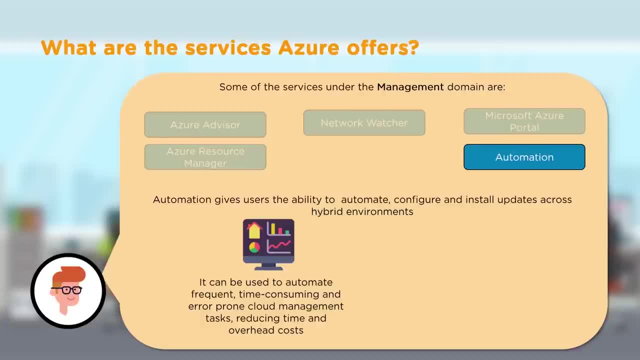 which means the application is not going to break and keep running for a longer time. With automation, we can actually build a good inventory of operating system resources and configuration items all in one place with ease, And this really helps in tracking the changes and investigating the issue. 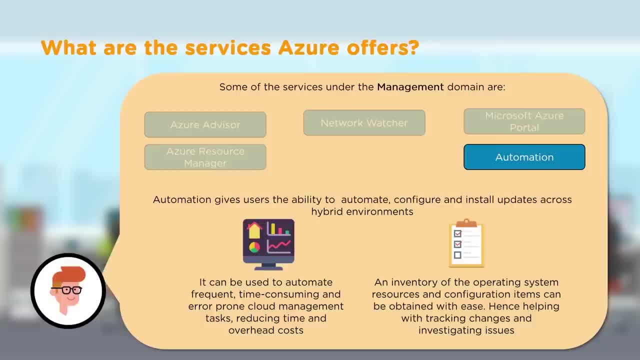 Let's say something happened. because we have automation, because it's logging the configuration changes, It's easy to track, easy to identify, easy to identify what has changed lately that has broken the environment, go back and fix it or kind of roll it back. 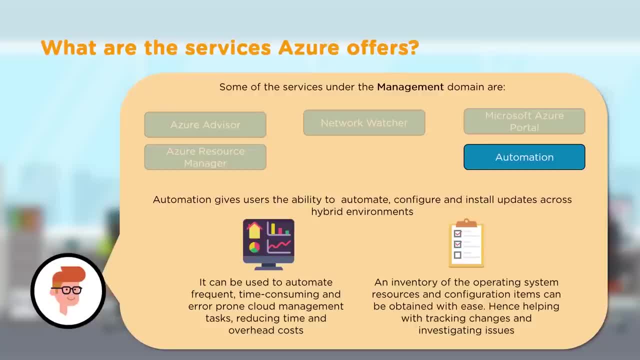 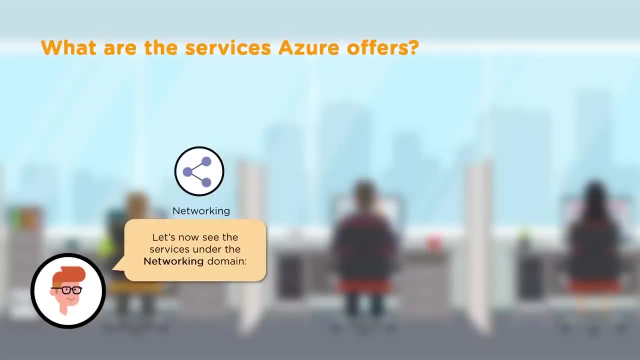 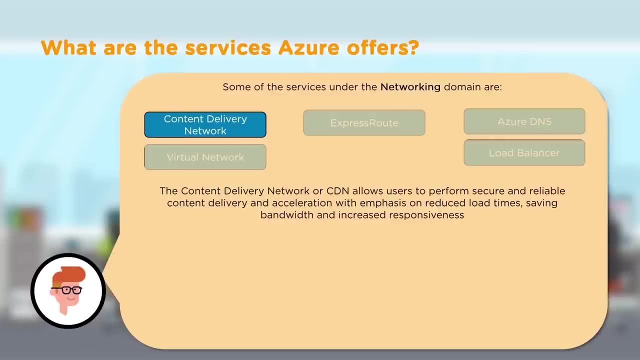 That solves the problem And that actually summarizes the Azure management tools or management services. Now let's talk about the networking tools or the networking services available in Azure. There are a variety of services, especially networking services, that Azure offers, And I'm sure it's going to be an interesting one. 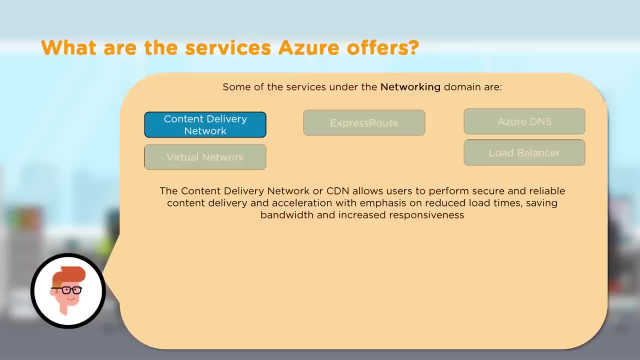 Let's begin Our discussion with content delivery network. Now the content delivery network, in short CDN. it allows us to perform secure and a very reliable content delivery. Not only that, it also helps in accelerating the delivery time, or, in other words, reducing the delivery time, also called as load times. 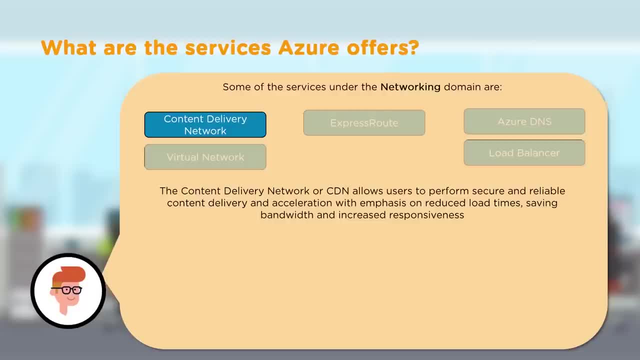 It also helps in saving bandwidth and increases in responsiveness to the application. Let's expand on this. The content delivery network is actually a distributed network of servers that can efficiently deliver web content to users. Now CDNs- we're going to use the word CDN here. 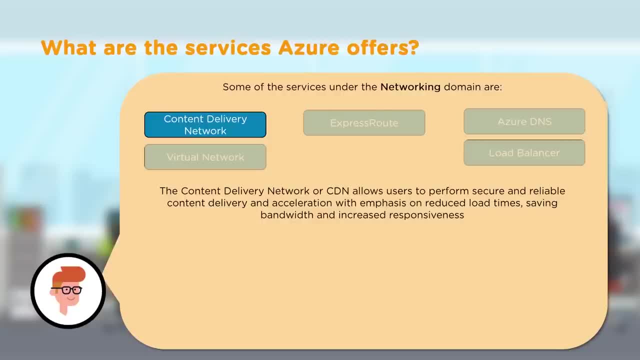 CDNs store cached content on global edge servers, also called as POPs, point of presence- locations that are very close to the end users, So the latency is minimized. It's like taking a copy of the data, or taking a multiple copy of the data and storing it in different parts of the world. 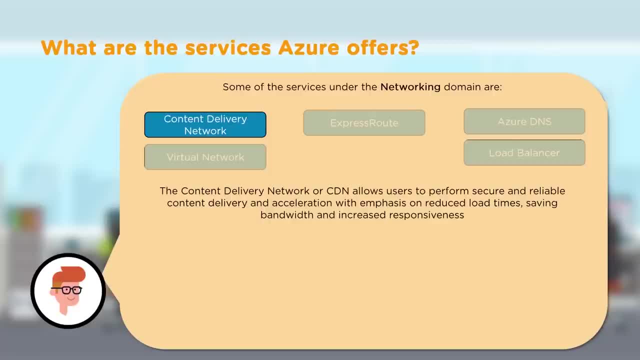 And whoever is requesting it. the data gets delivered to them from a server which is very locally to them. So this CDN offers developers a global solution for rapidly delivering high bandwidth content to users by caching the content in a strategically placed location which is very near to them. 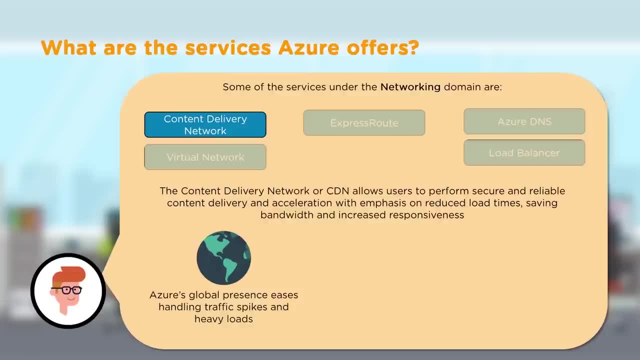 So these content delivery networks. it really helps in handling. That's one advantage You get for content delivery network. That's we can handle spikes and heavy loads very efficiently And we can also run analytic against the logs that gets generated in content delivery network, which helps in gaining good insight. 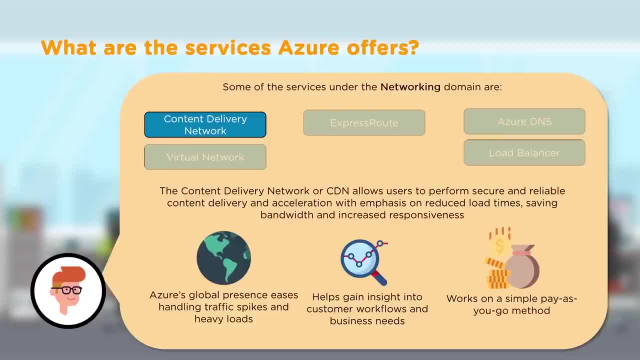 on the workflow and what would be the future business need for that application. And this, just like a lot of other services. this is on a pay as you go type, So you use the resource first and then you only pay for what you have used. 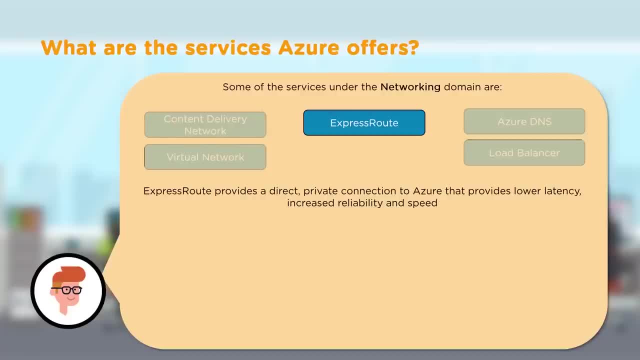 The next one in networking would be ExpressRoute. Now, ExpressRoute is actually a circuit or a link that provides and a direct private connection to Azure And because it's direct, it gives low latency link to Azure. It gives good speed and reliability for the Azure data transfer. 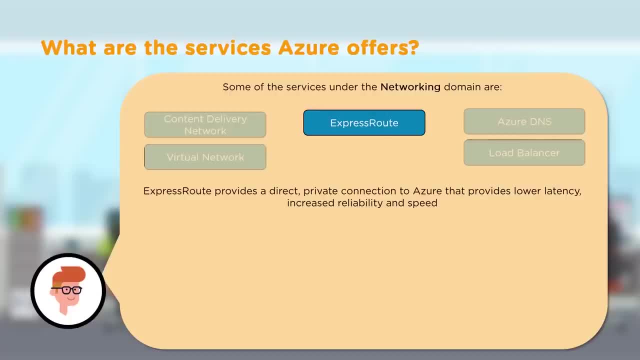 It could be on premises to Azure. So it gives very good speed, It gives increased reliability and low latency for that connection. Let's expand on this a bit. And now this ExpressRoute is a service that actually provides a private connection between Microsoft data center and infrastructure in our premises or 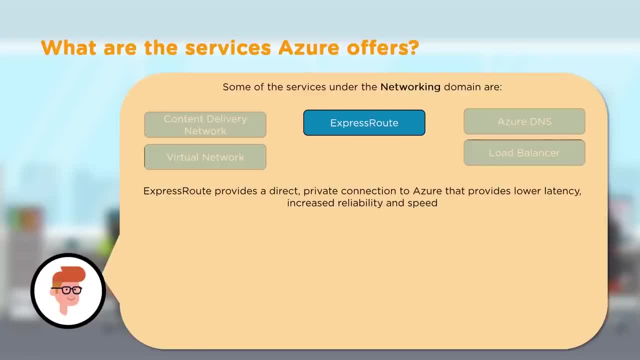 in a different colocation facility that we might have Now. these ExpressRoutes do not go over the public Internet And because they don't go over the public Internet, they offer a high security, reliability and speed and low latency compared to the connections which are in the Internet. 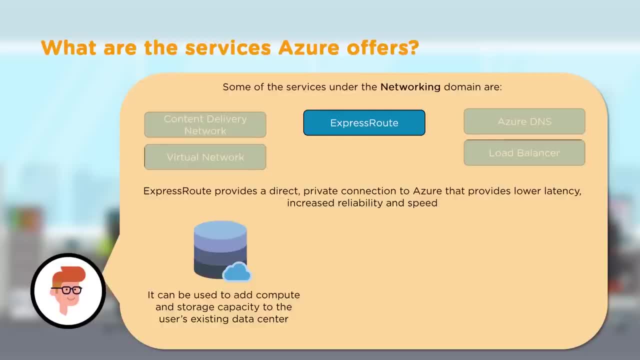 Because it's fast, because it's reliable, because it has low latency. it can be used as an extension of our existing data center. You know users are not going to feel the difference whether they are accessing services from an on premises or in the cloud environment, because latency is. 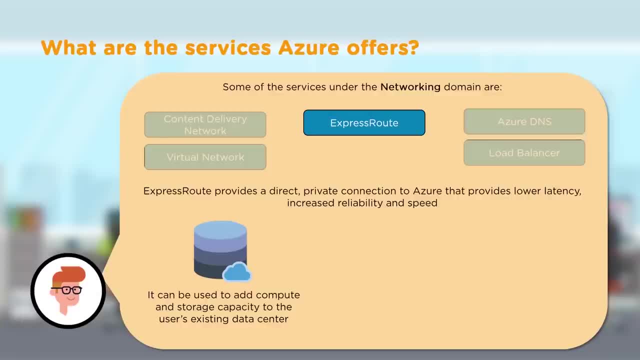 minimized as much as possible. Users are really not going to see the difference. And because it's a private line and not a public Internet line, it can be used to build hybrid applications without compromising privacy or the performance. Now, these virtual private cloud. 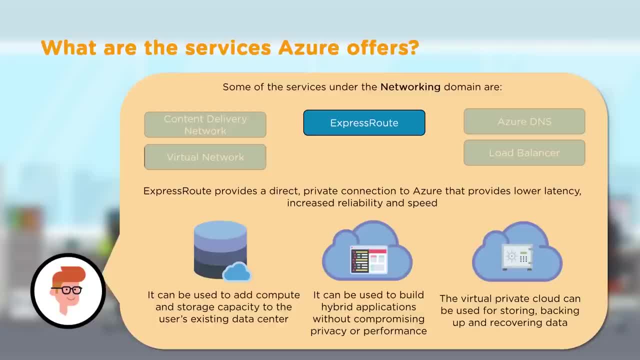 these ExpressRoutes can be used for taking backups. If assume a backup going through the Internet, that would be a nightmare. If you use ExpressRoute for backups, that's going to be fast, And imagine recovering a data through the Internet, from the cloud through the Internet to the on premises. 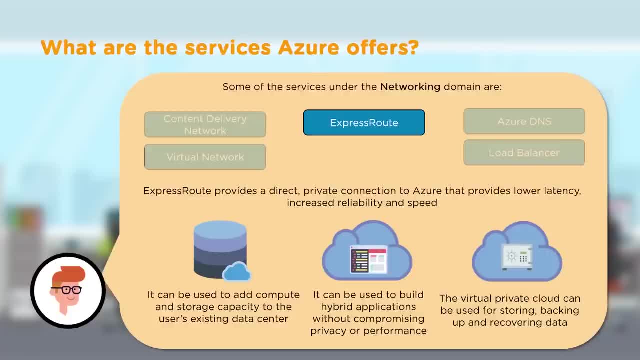 in a time of disaster, that would be the worst nightmare. So these ExpressRoutes can be used not only to backup but also to recover the data, because it provides good speed, low latency. Recovering the data is going to be a lot sooner. 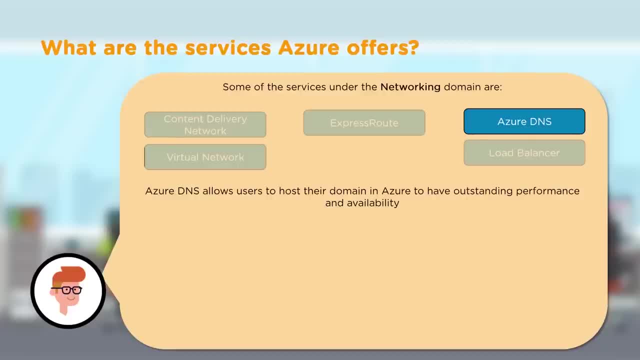 The next product or service we're going to discuss in networking is Azure DNS. Now, Azure DNS allows us to host domain name in Azure, And these domain names come with an exceptional performance and availability. Now Azure DNS is used to set up and manage. 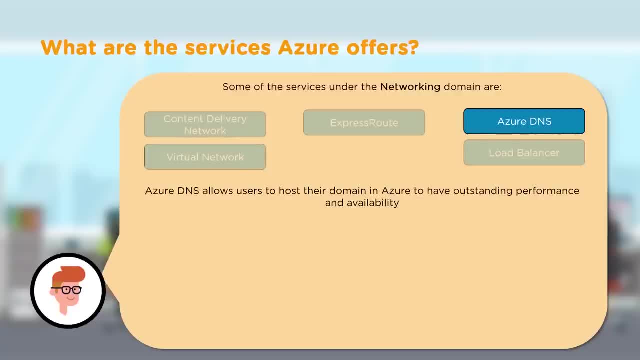 DNS zones and records for our domain name in the cloud. Now this Azure DNS is a service for DNS, just like the name says, And it provides name resolution. by using Azure's infrastructure And by using this domain, we can actually manage the DNS ourselves. 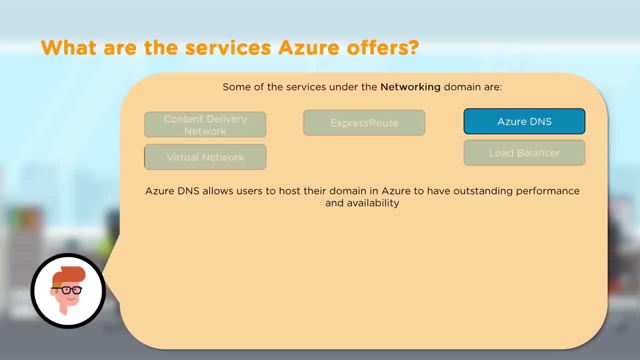 through the Azure portal with the same credential. Imagine having a DNS provider which does not even belong in our IT. Imagine that environment. We would have a separate portal to manage the DNS environment. Those are gone And now we can actually manage the DNS. 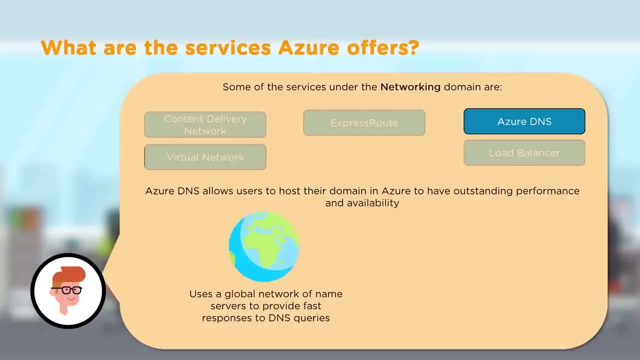 in the very same Azure portal where we use the rest of the other services, And this Azure DNS very much integrates with other DNS service providers. It uses a global network of name servers to provide fast response to DNS queries And these domains are having additional availability compared to the other. 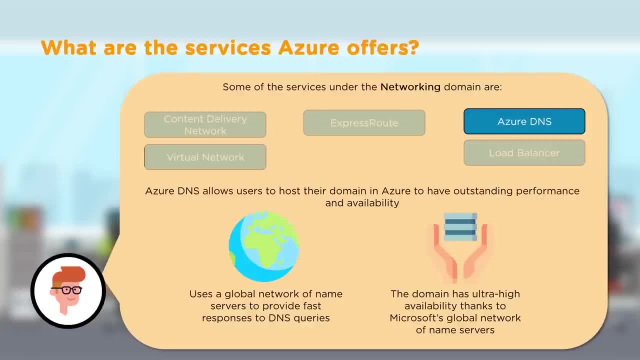 domain service providers: availability promises. These are going to have more availability than the rest because most of the servers are maintained by Microsoft and it helps resolve sooner. It helps resyncing, Let's say a server fails. it kind of helps resyncing with the. 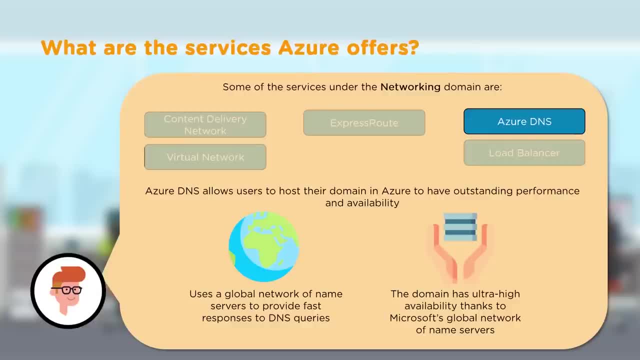 rest of the servers. So all the Microsoft's environment, all the Microsoft's global network of name servers kind of ensures that our domain names are resolved properly. not only properly, but also are available most of the time. Next in the list in networking services is virtual network. 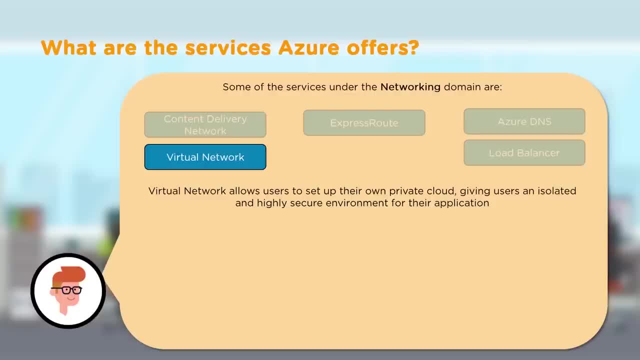 I'm sure this is going to be very interesting and I'm sure you're going to like it. So this networking, or virtual networking, in Azure, it actually allows us to set up a our own private cloud in the public cloud. It gives us an isolated and highly secure environment for our application. 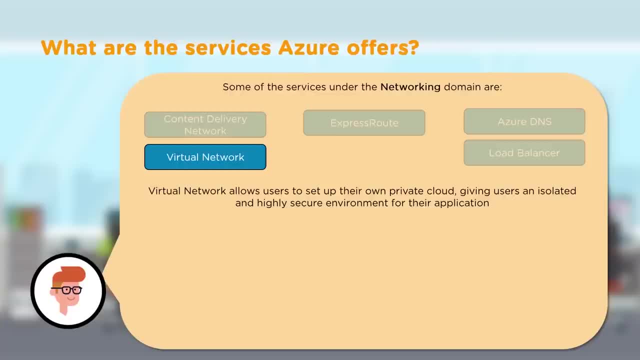 Let's expand on this. This Azure virtual network helps us to provision Azure virtual machines and it helps us to securely communicate with other on premises and Internet networks. It also helps in controlling the traffic that flows through or flows in and out of this virtual network to other virtual networks and to the Internet. 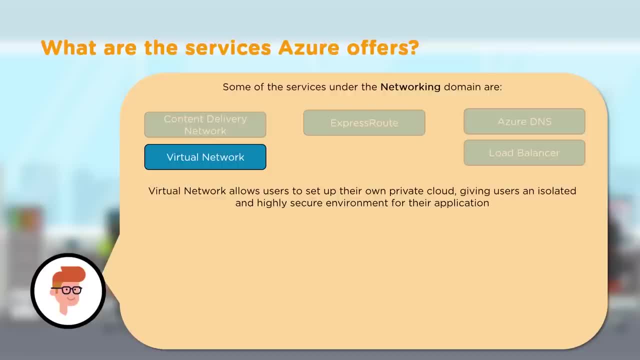 Now this Azure virtual network, sometimes called as VNet, is actually a representation of our own network in the cloud. It's actually a logical isolation of the Azure cloud dedicated to our subscription. All our environments are provisioned in a VNet that is separate from another. 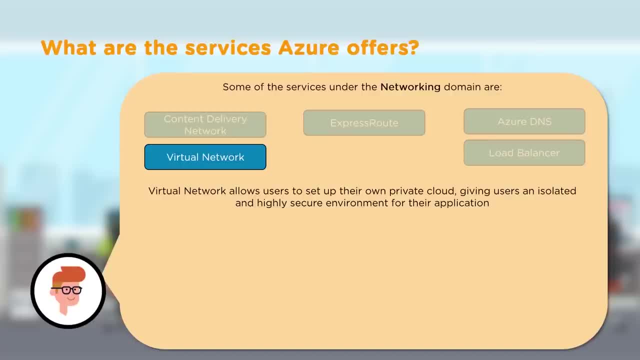 customer's VNet. That way we have that logical separation there. So this virtual network can also be used to provision VPNs in the cloud, so we can connect to the cloud and the on premises infrastructure and a lot more, especially in an environment where we have hybrid environment. 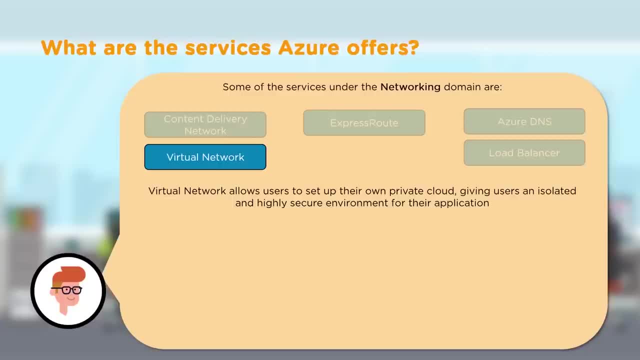 Surely we will be using virtual network, because that's going to require a VPN for secure data transfer in and out of the cloud and in and out of the on premises environment. All right, so it kind of gives us a boundary for all the resources. 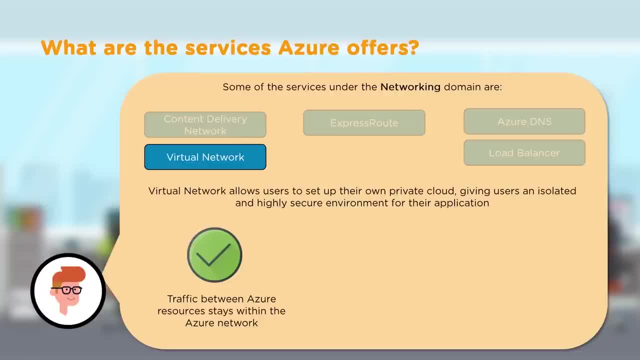 So all the traffic between the Azure resources- they kind of logically stay in between or logically stay within the Azure virtual network, And here we can design the network- is given over to us. You can pick the IP, you can pick the routing, you can pick the subnet and a lot. 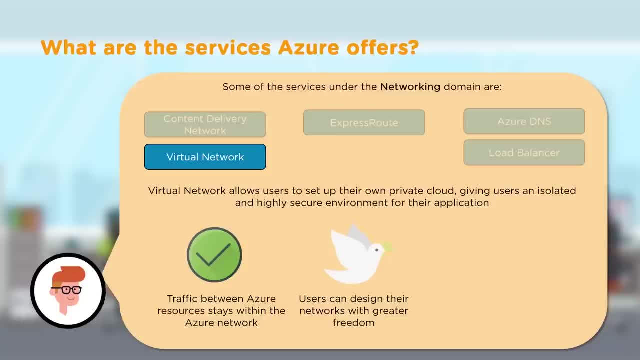 of freedom is given, or I would say a lot of control on how the network is designed. It's not like something that's all already cooked and we only get to use it. No, we can actually build the network from the scratch. We can pick the IP address that we like. 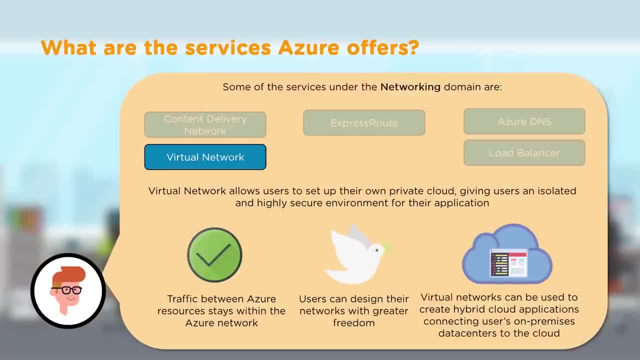 We can pick which subnet needs to communicate with the other subnet- Stuff like that. And, like I said, if you are using hybrid environment, you definitely would be requiring a virtual network, because it helps connect the on premises and the cloud in a secure fashion using VPN. 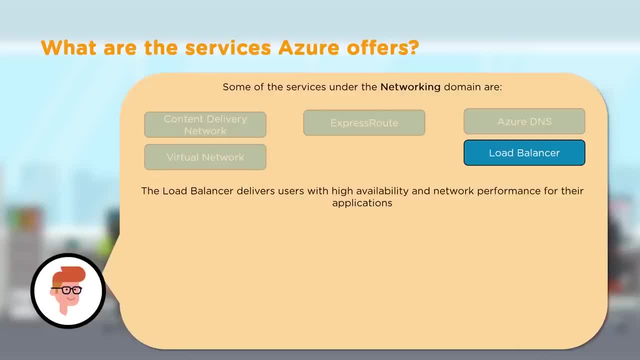 The last product we're going to discuss in networking is a load balancer. This load balancer Actually provides application a good availability and a good network performance. So how does it work? It actually works by load balancing the traffic to and from the virtual machine. 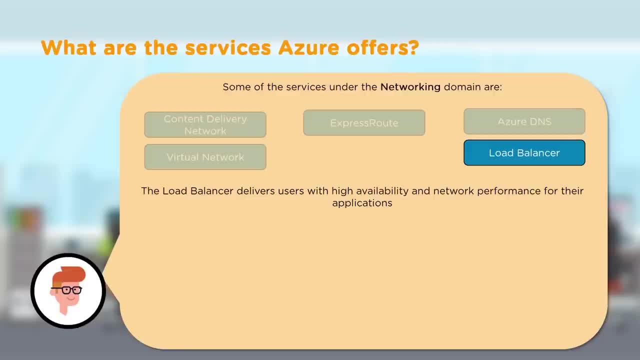 and the cloud resources. not only that, it also load balances between cloud and across premises virtual networks. with Azure load balancer, We can actually scale our application and create high availability for our services, which means our obligation will be available most of the time. 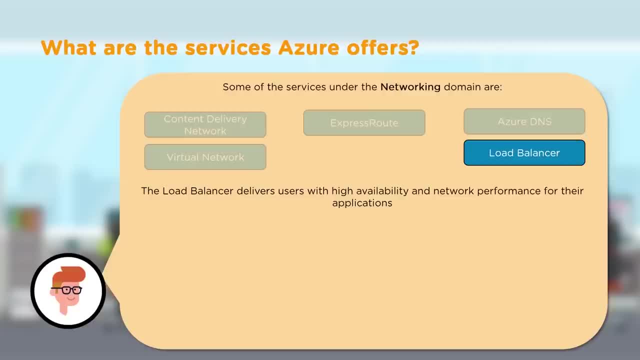 If any of the server goes dead, the server does not get traffic. What happens if the server gets traffic? User is going to experience downtime. What happens if the server does not get traffic? User won't experience any downtime. The connection is shifted to an healthy service. 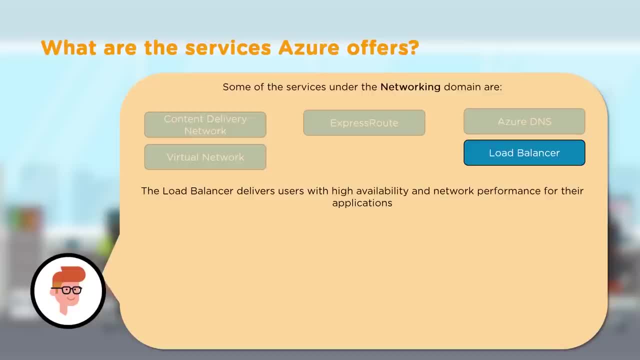 So the user experiences uptime all the time. So this load balancer supports inbound and outbound scenarios and it provides low latency. It gives high throughput of the data transfer And we can actually scale up the flow of the TCP and UDP connections from hundreds to thousands to even millions because we have a load balancer now in between. 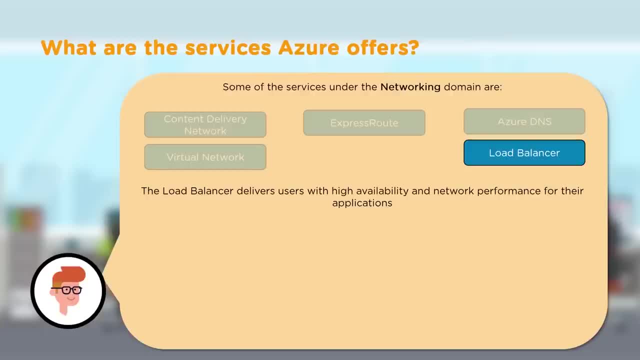 the user and the application. So how does it operate? This load balancer actually receives the traffic and it load balances the traffic to the back end pool of instances connected to it, according to the rule and the help probe that we set. That's how it maintains high availability. 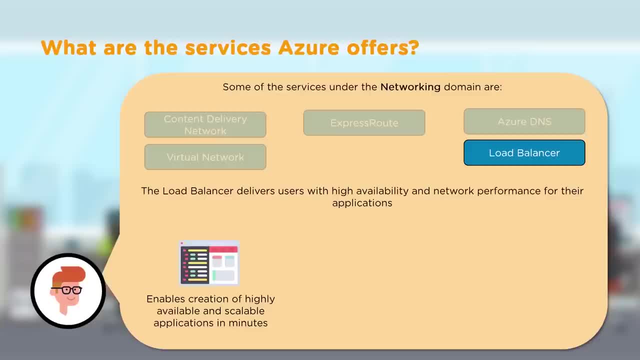 So what does it do? What does load balancer help? It helps in creation of high, available, scalable application in the cloud in minutes. It can be used to automatically scale the environment with the increasing application traffic, And one feature of load balancer is to check the health of the user's application. 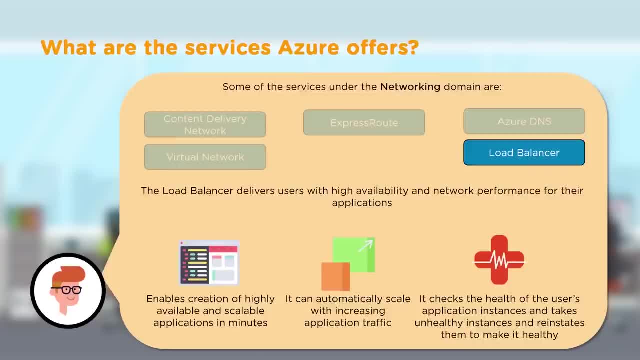 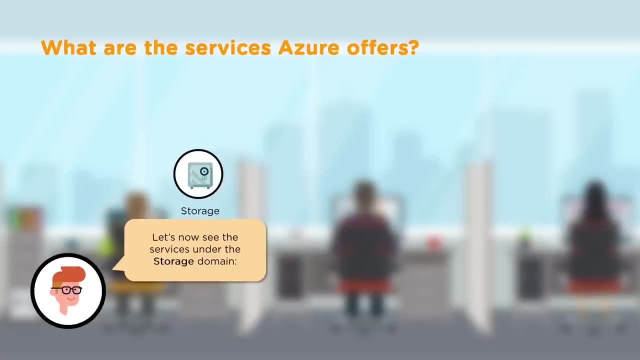 instance and it removes or it stops sending the request to the unhealthy instance and kind of shifts that connection to the healthy instance. That way a user or a connection does not get stuck with an instance that's not healthy. That's all that you need to know about the networking services. 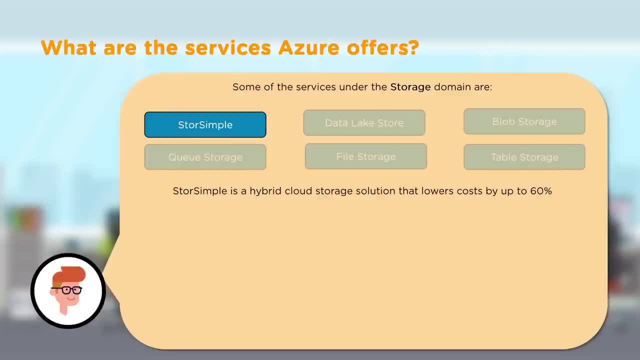 Now let's talk about the storage services, or the storage domain in Azure. Now, Azure storage in general is a Microsoft managed service providing cloud storage which, basically, is highly available, secure, durable, scalable and redundant because it's all managed by Azure. 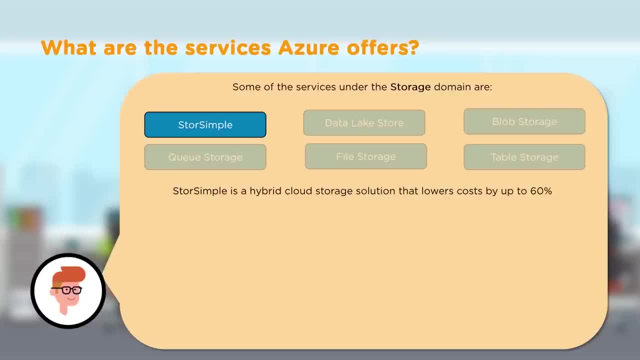 We don't get to manage a lot of it. And these Azure storages are a group of storage services. They cater to different needs and the storage products include Azure Blobs, which is actually an object storage. it includes Azure Data Lake. it includes Azure Files, as you see, it includes Azure Queues. 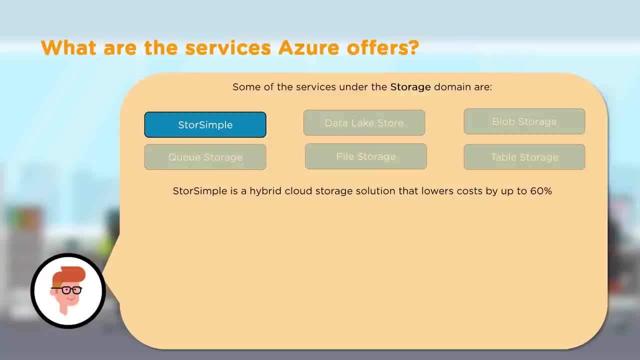 it includes Azure Tables and a lot more, But let's start our discussion with Azure Store Simple. Azure Store Simple is an hybrid cloud storage solution that actually lowers the cost of storage to nearly 60 percent Of how much you would be actually spending without using it. 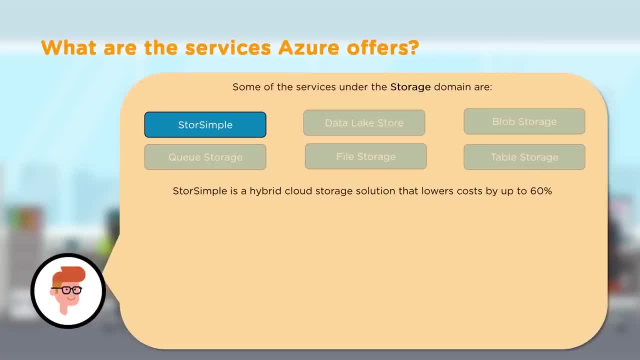 So Azure Simple Storage or Store Simple, is an integrated storage solution that manages the storage task between on premises and the cloud storage. What I really like about Azure is that it's built around a hybrid environment in mind. There are a lot of other cloud providers. 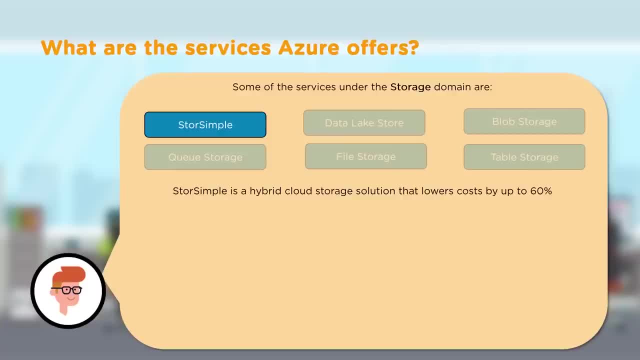 that are there where running an hybrid environment is a big challenge. Now it has some compatibility. You won't be able to find a hybrid or on premises and cloud solution for your need- stuff like that- But with Azure, especially when it comes to storage a lot of the things that we're 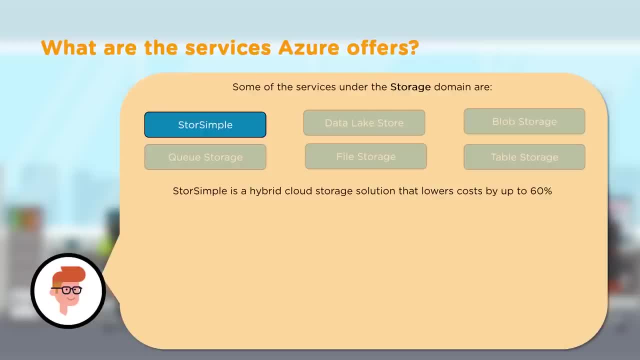 going to see it clearly is designed with hybrid environment in mind. All right, So let's come back and talk about Store Simple. So Store Simple is a very efficient, cost effective and a very easily manageable SAN storage area networking solution in the cloud. I thought I'll throw in this information. 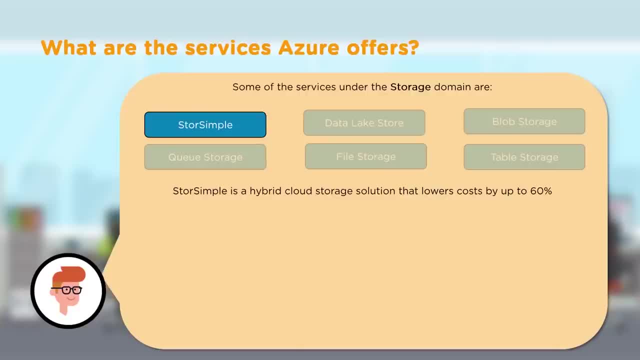 The reason why it got Store Simple is really because it uses Store Simple 8000 series devices which are used in Azure data center, And this Store Simple or Simple Storage. it comes along with storage sharing to manage the stored data across the various storage media. 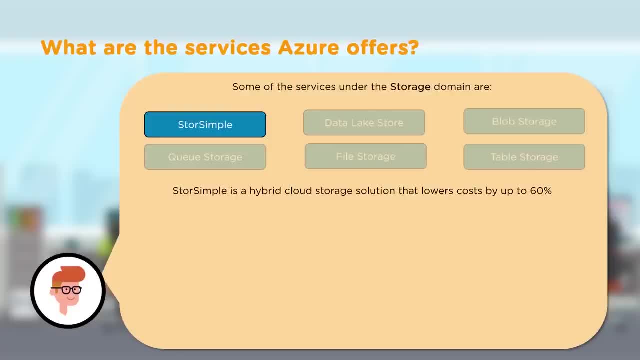 So the current, the very current data is actually stored in on premises, on solid state drives, and data that is used less frequently is stored in HDDs or hard disk drives And the data that requires archived or that needs to be archived- very old data, let's say less frequently. 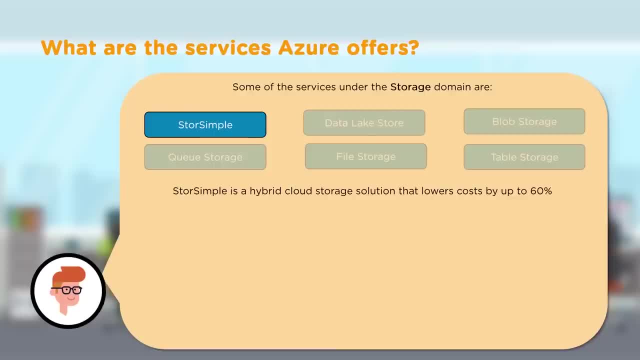 used data candidate for archive, they are actually pushed to the cloud. So you see how this storage tearing automatically happens in Store Simple. And one another cool feature of Store Simple is that it enables us to create an on demand and scheduled backups of data and then store the data locally or in the cloud. 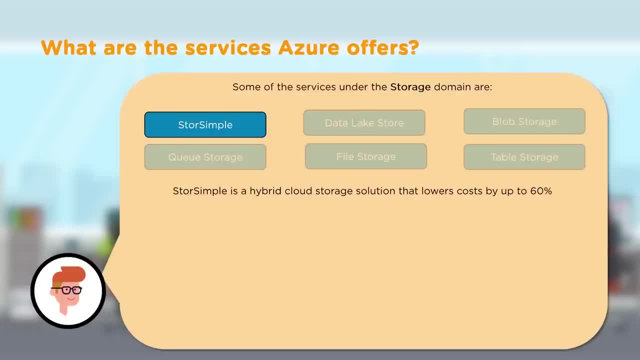 And these backups are actually taken in the form of incremental snapshot, which means that they can be created and restored quickly. It's not a complete backup, it's an incremental backup. And these cloud snapshots, they can be critically important when there is a disaster and when there is a disaster recovery scenario, because these snapshots- 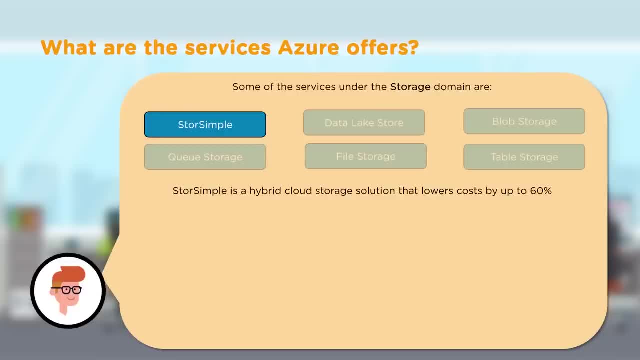 can be called in and they can be put on storage systems and then they become the actual data. So recovering is faster if you have proper scheduled backups or if you have frequent backups And this storage simple, it really helps in easing our backup mechanism, which means it kind 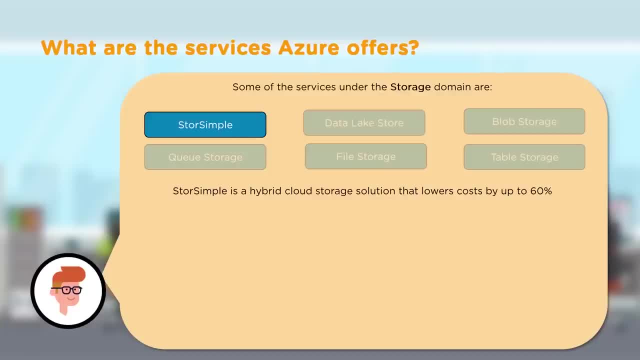 of eases our disaster recovery steps or procedures as well. So the Store Simple. it can be used to automate data management, data migration, data movement, data tearing across the enterprise, both in cloud and on premises. It actually improves the compliance and accelerates the disaster recovery for our environment. 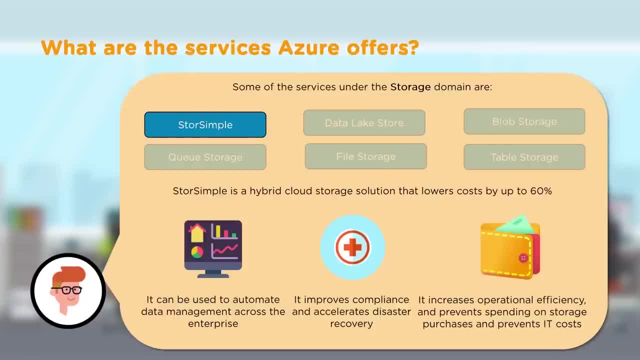 And if there is one thing that's increasing every new day in our environment, that would be storage, And this Store- Simple- addresses that need And we really don't have to preplan or think in deep or having a proper storage, because now we have a simple storage available in the cloud. 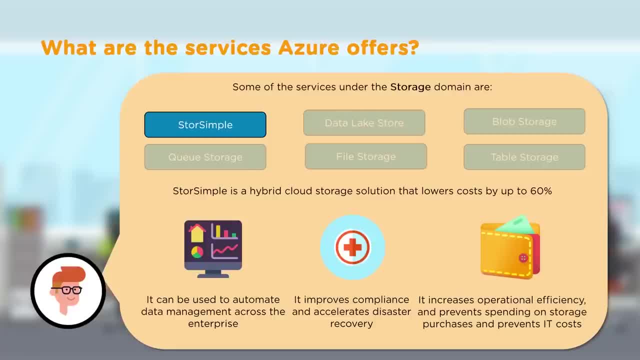 And, moreover, it's on a pay as you go type, So not much preplanning on storage is needed. Yes, there will be a need, but not as much as I would without the cloud or without the simple storage, And the next service under storage that we would like to discuss is the 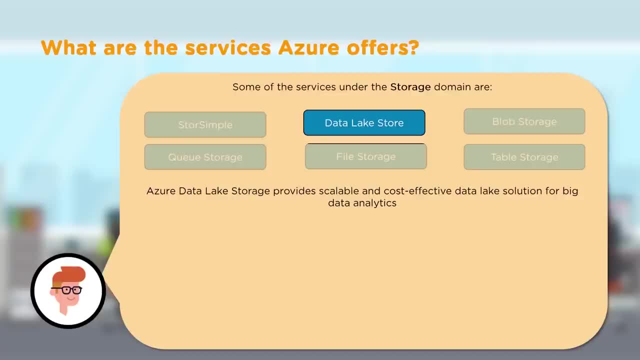 Data Lake Store. This Data Lake Store or storage. it's a cost effective solution for big data analytics in specific, So let's expand this. So this Data Lake Storage is an enterprise wide repository for big data analytic workload. That's the major service that's dependent on this Data Lake Store. 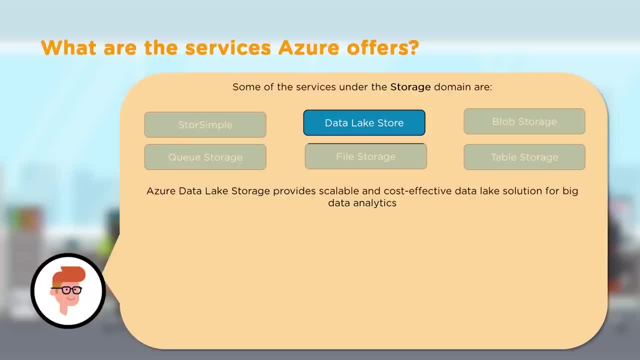 And this Data Lake enables us to capture data of any size, of any type and of any ingestion speed, And it kind of collects them in one single space or in one single place for operational efficiency- I mean operational efficiency- and for analytic purpose. 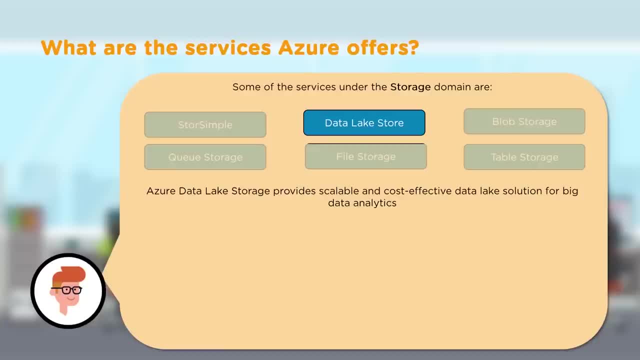 Hadoop in Azure is very dependent on this Data Lake Storage And this Data Lake Store is designed with performance for analytics in mind. So any time you think of, or any time you're using analytic in the cloud or any time you're using Hadoop in the cloud in Azure, 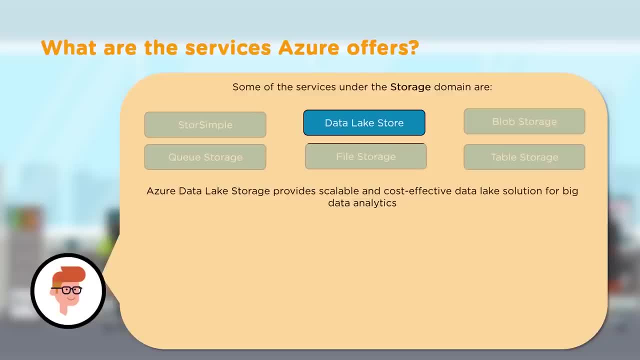 We are definitely using or we will be, to the most part, or the normal procedure or the right storage to pick would be Data Lake Store in Azure. It's designed with security in mind, So any time we use Azure storage, we can be rest assured that we are using storage. 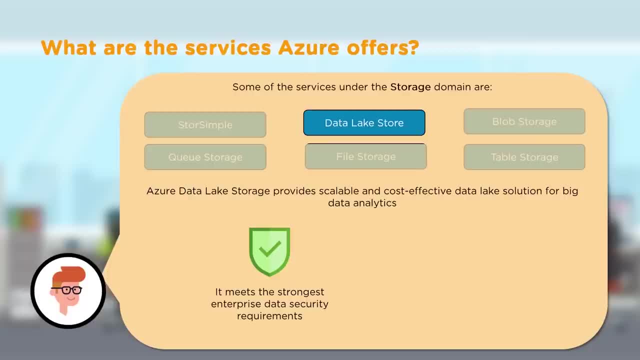 from within a data center which has, or which was built, with security in mind. So this data store also uses Azure blob storage behind the scenes for global scale, durability and for performance. Let's talk about blob storage. A blob storage provides large amount of storage and scalability. 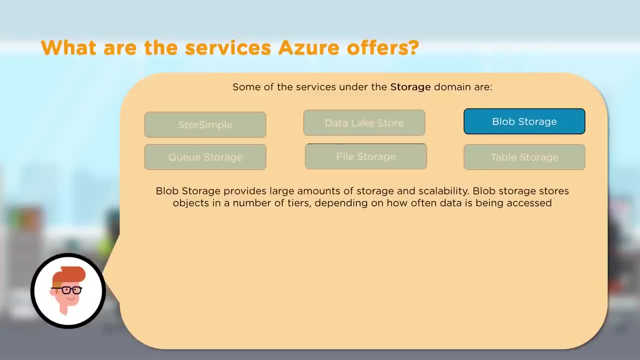 Now this blob storage is the object storage solution for Azure cloud. Let's expand a bit on blob storage. Azure blob storage is Microsoft offering for object storage. Now this blob storage is optimized for storing massive amount of unstructured data, which could be text or binary data. 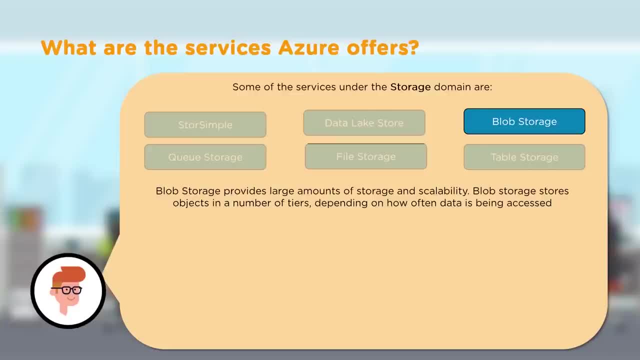 It's designed and it's optimized for rapid reads. If I explain to you on what scenarios we would be using blob storage, that might help you get a good understanding of what blob storage is. So it's helped or it's designed as of now. it's being used in many IT. 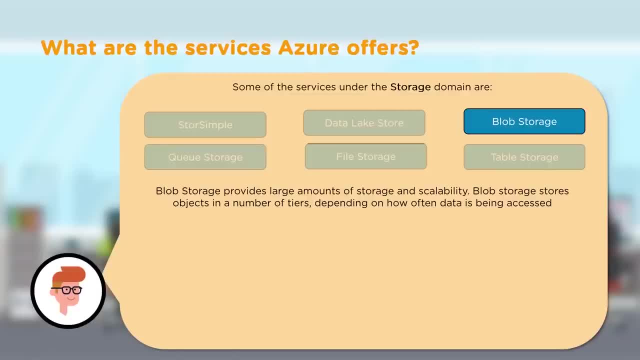 environments to serve images or documents directly to the browser. It helps in storing files for distributed access. A lot of fetches can fetch data from Azure blob storage and it currently is helping users stream video and audio. It's currently being used for writing log files. 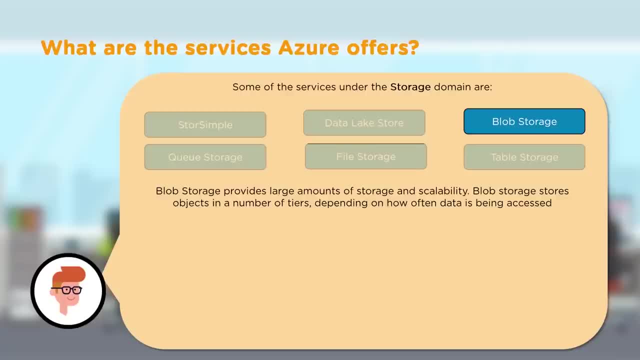 It's currently being used to store data as backup and restore at a later point in times of disaster recovery. It also is used as an archiving storage in a lot of cloud IT environments. It's widely used in storing analytic data- not only storing. 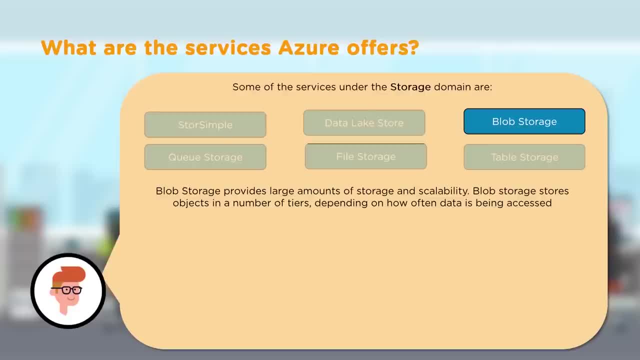 but also running analytic query against the data stored in it. So that's a wide use case for blob storage. Not only that, in addition to all that we mentioned, it also supports versioning, So anytime somebody updates and data, a new version gets created. 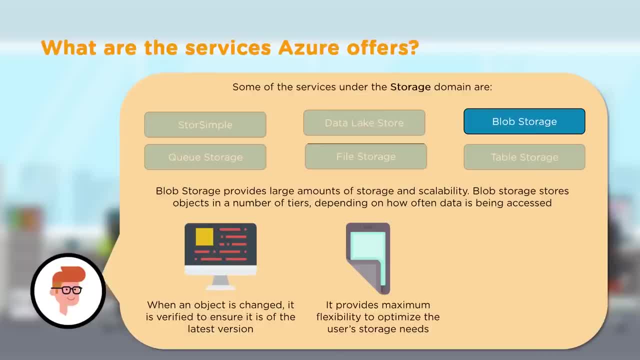 which means at any point I can roll back as and when needed, And it provides a lot of flexibility on optimizing the user's storage need. It also supports tiering of the data, So based on need, when I actually explore, I would find a lot of options I can pick. 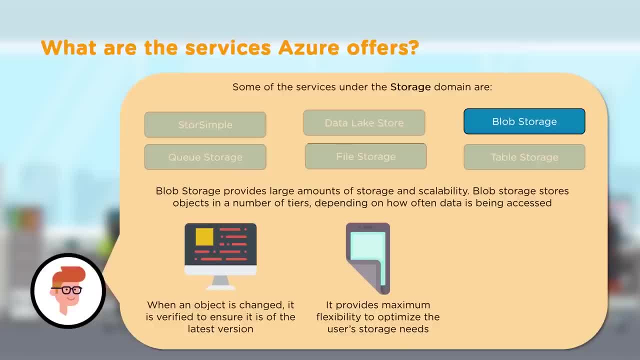 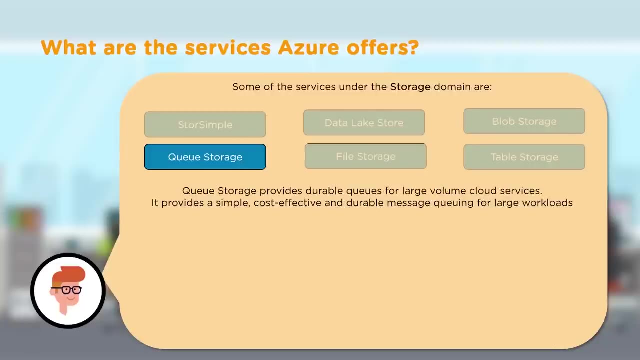 from that. So you know, suits to my unique storage environment or unique storage need And, like I said, it stores unstructured data and this unstructured data is available for customers through REST based object storage environment. The next product and storage service would be queue storage. 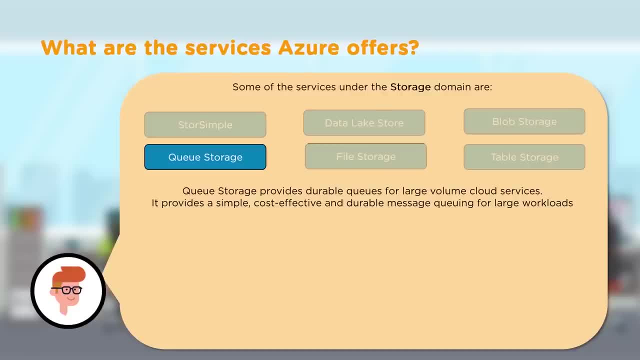 Now. queue storage provides durable queues for large volume cloud services. It's a very simple and a cost effective durable messaging queue for large workloads. Let's expand this queue storage for a moment Now. this queue storage is a service for storing large amount of messages that can. 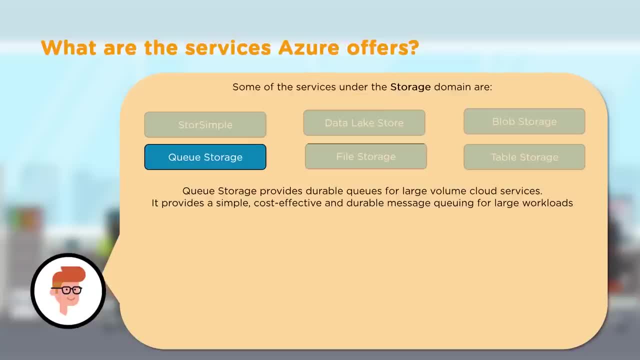 be accessed from anywhere in the world through HTTP and HTTPS calls. A single queue or a single queue message can be up to like 24 KB in size, and a single queue can contain millions of such 24 KB in size messages. And how much can it hold? 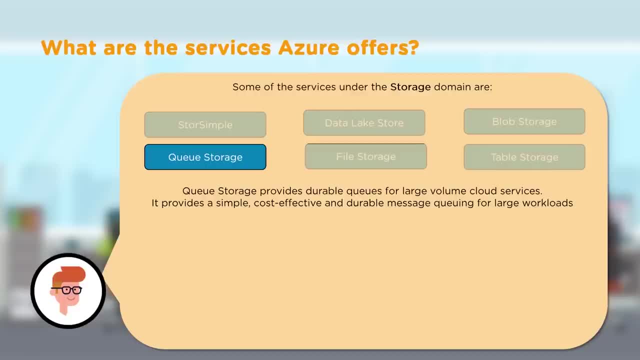 It can hold up to the total capacity of the storage account itself. so that's kind of easy to translate. How much would it hold? And this Azure queue storage. it provides an messaging solution between applications and components in the cloud. What does it help? It helps in designing an application for scale. 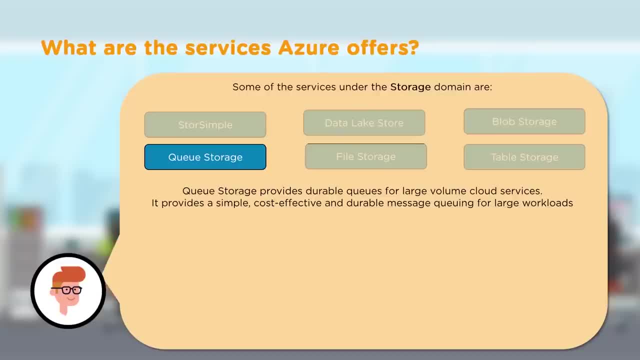 It helps in decoupling the application. So you know, it's not very dependent, or sometimes it's not at all dependent- on the other application, because now we have a queue in between which kind of translates or which kind of connects or which kind of decouples both. 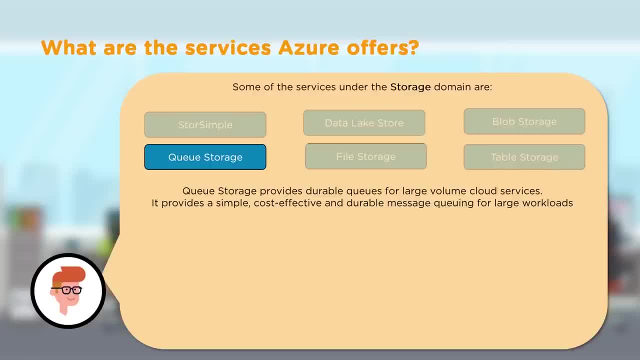 the environment. Now we have a queue in between Both the environment can scale up or scale down independently. The next in the storage service would be file storage. Let's talk about file storage Now. these Azure files provide secure, simple and managed cloud file shares. 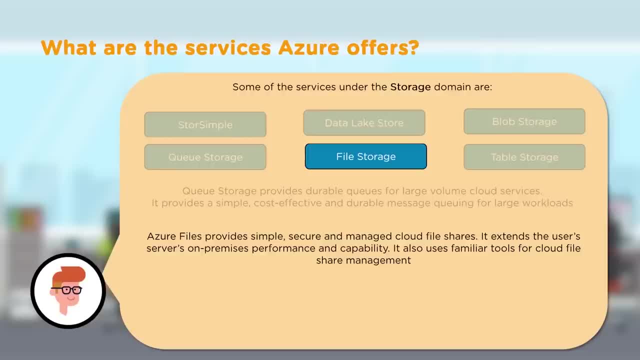 Now, with file share in the cloud, it actually extends the user servers on premises performance and capacity, and a lot of familiar tools for the cloud file share management can be used along with the file storage that we're talking about. So let's expand a bit on file storage. 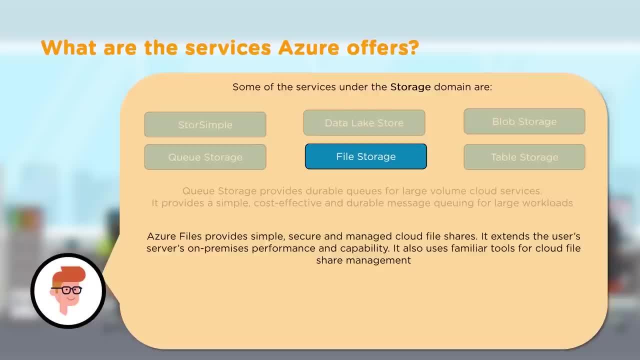 Now this Azure files or Azure file storage offers a fully managed file shares in the cloud that can be accessed via the SMB protocol server message block protocol. Now this Azure file shares can be mounted concurrently By cloud or in on premises deployments. a lot of operating systems are compatible. 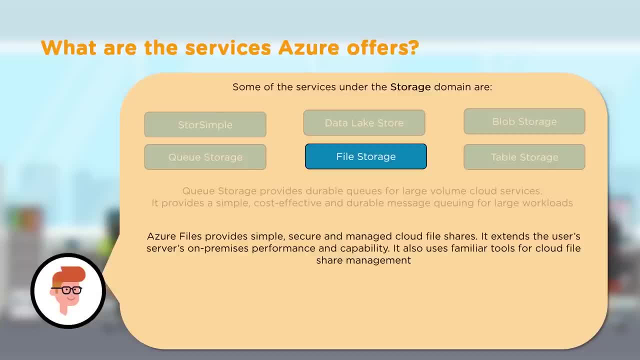 with it. Windows are compatible, Linux is compatible, Mac OS is compatible. In addition to all these- being able to run on on premises and on the cloud, or being able to access from on premises and on the cloud- it can also offer cache for caching. 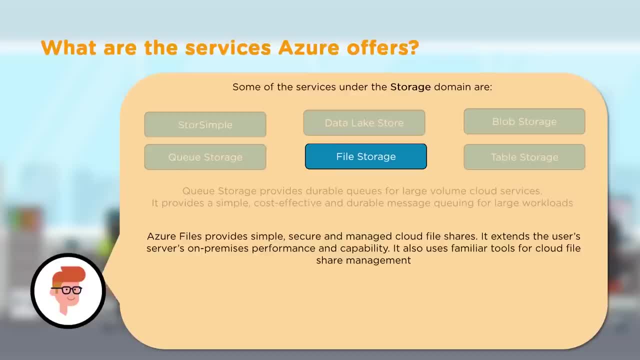 the data and keeping it locally so it's immediately available when needed. So that's some additional feature. I would say That's some advanced feature that it offers compared to the other file shares available in the market. Let's talk about table storage. 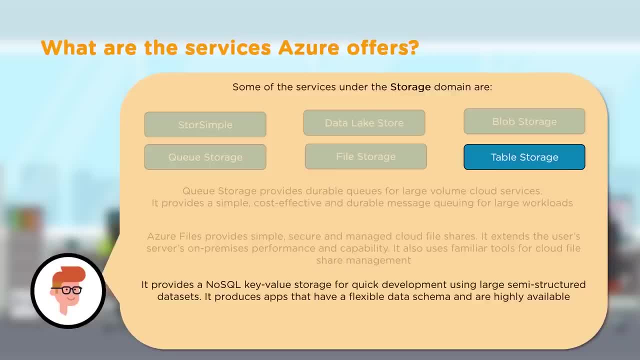 Let's talk about table storage Now. table storage is a NoSQL key value pair storage for quick deployments with large semi-structured data sets. The difference between one important thing to note with table storage is that it has a flexible data schema and also it's highly available. 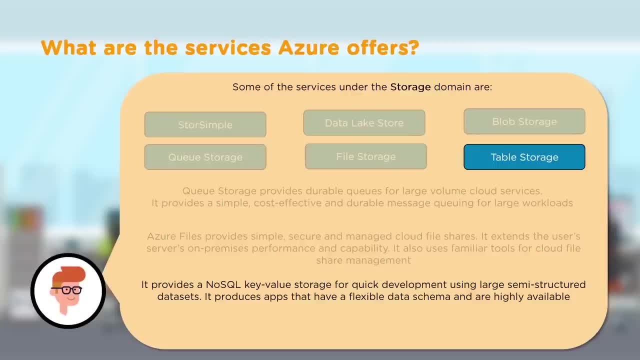 Let's expand a bit on table storage. So anytime you want to pick a schemaless, a NoSQL type table storage is the one we'll end up picking. It provides a key pair attribute storage with a schemaless design. This table storage is very fast and very 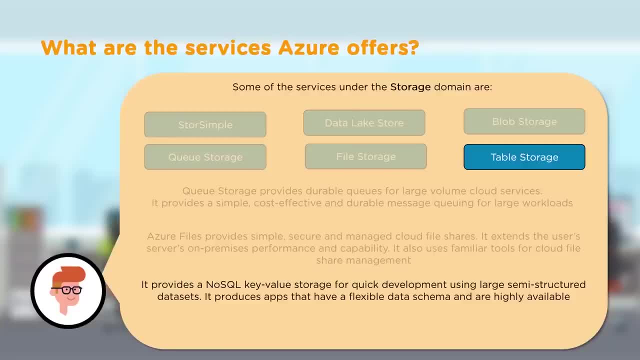 cost effective for many of the applications and for the same amount of data. It's a lot cheaper when you compare it with the traditional SQL data or data storage. So some of the things that we can store in the table storage are, of course they're going to be- flexible data sheets. 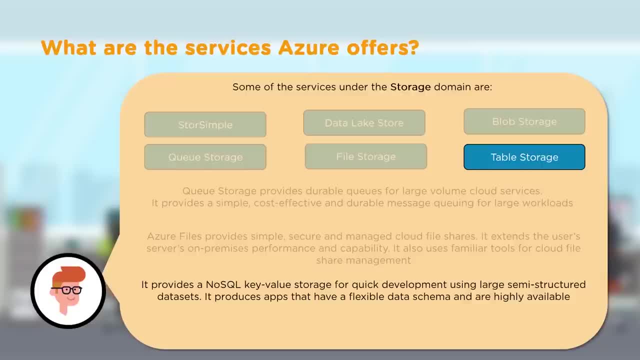 such as user data for web application address books, device information and other types of metadata for our service requirements, And it can have any number of tables up to the capacity limit of the storage account, And this is not possible with SQL. This is only possible with NoSQL, especially with table storage in Azure. 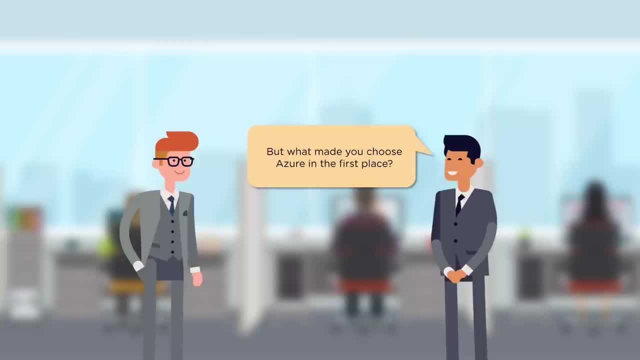 Explanation of storage really concluded the length and breadth of the explanation this CEO was giving his IT personal. but this IT personal is not done with it yet. He still has a question, even after this lengthy discussion, And his question was: well, there are a lot of other cloud providers available. 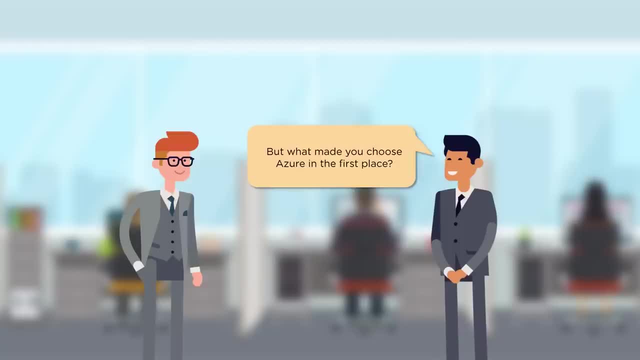 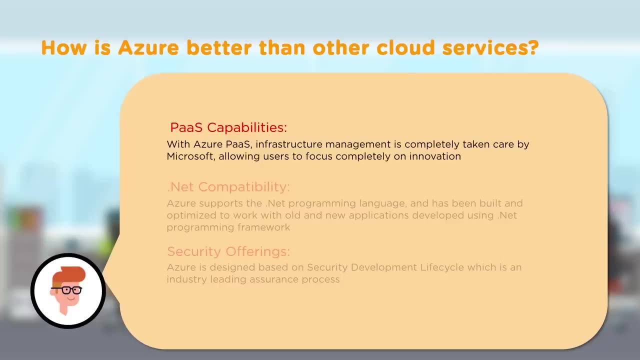 What made you specifically choose Azure. I mean, from the kind of question that he asked, we can say that he is very curious and he definitely had asked and very thoughtful question. So his CEO went on and started to explain about the other capabilities of Azure or how it kind of outruns the rest of the cloud providers. 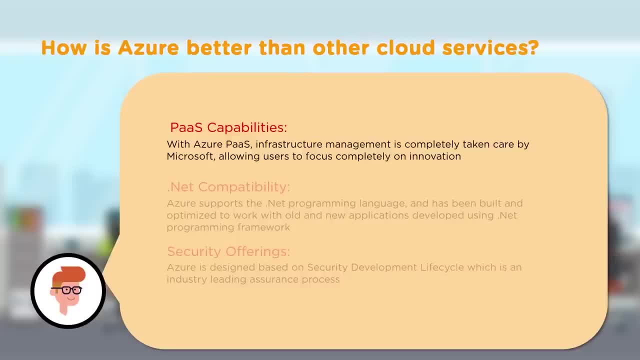 So he started- or he again started, his discussion, but from a different angle now. So he started to explain what are the capabilities or how Azure is better than the competitors. So he started with explaining the platform as a service capabilities, And I'm going to tell you 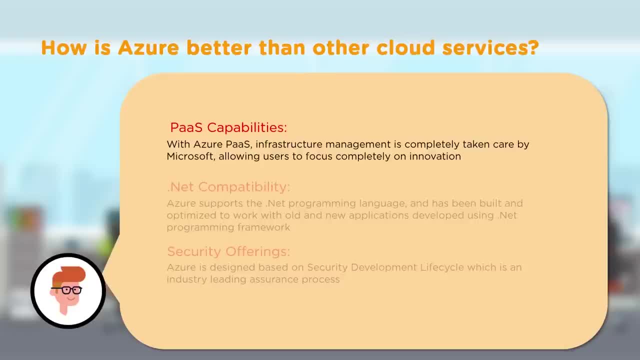 what the CEO told his IT person. So this platform as a service or in platform as a service, the infrastructure management is completely taken care by Microsoft, allowing users to focus completely on the innovation. No more infrastructure management responsibilities. Go and focus on innovation. 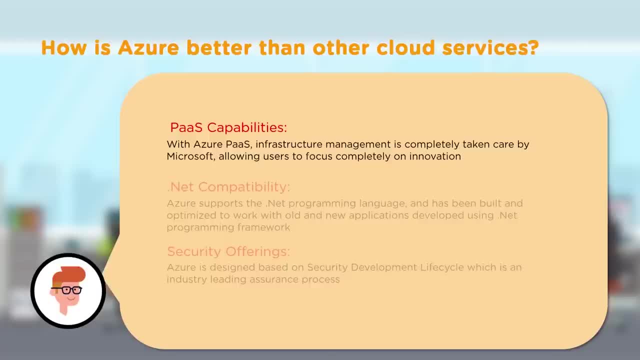 That's. that's a fancy way of saying it. When we buy platform as a service, that's what we get. We can contribute our time on innovation and not just maintaining the infrastructure, And Azure, especially, is NET friendly. Azure supports the NET programming language and it has or it is built or 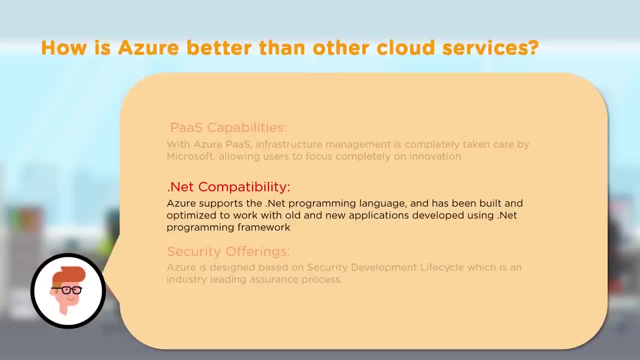 designed or it is optimized to work with old and the new applications deployed using NET programming framework. So if your application is NET, most of the time you would end up picking Azure. I mean, if you try to compare, most of the time you would end up picking Azure as your. 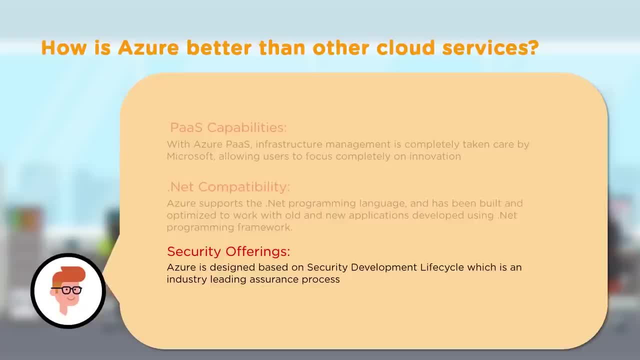 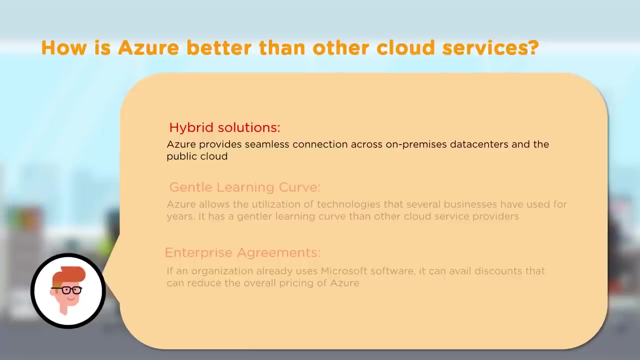 service provider and the security offerings that Azure offers is it's designed based on the security development lifecycle, which is an industry leading assurance process. When we buy services from Azure, it assures that the environment is designed based on security development lifecycle And, like I mentioned many times in the past and I would like to mention it again, 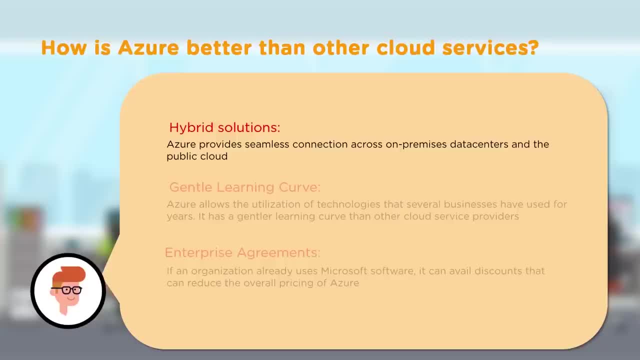 Azure has well thought about the hybrid environments, which a lot of other cloud providers have failed. So it's very easy to set up a hybrid environment to migrate the data or not to migrate the data and still run a hybrid environment. They work seamlessly with Azure because Azure provides seamless connection. 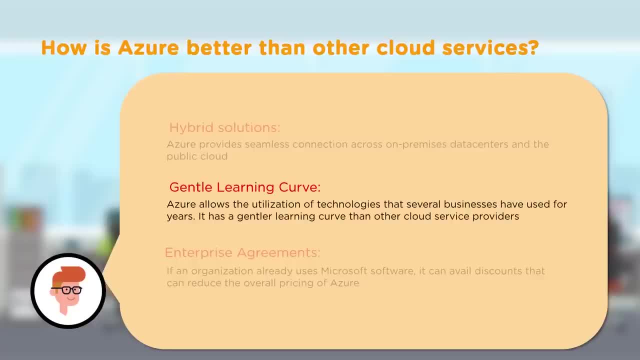 across on premises, data centers and the public cloud. It also has a very gentle learning curve. If you look at the documentation, it's picture rich and the documentations are neat and clear. It would encourage you to learn more. It would encourage you to think and imagine and try easily get a grasp of how services work. 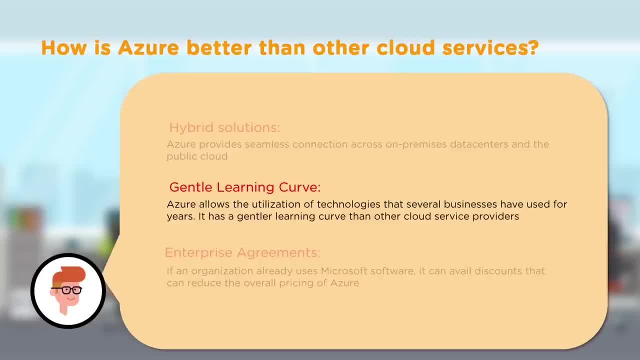 So it has a very gentle learning curve. Azure allows the utilization of technologies that several business have used for years, So there is a big history behind it. It has a very gentle learning curve that the certifications, the documentations, the stage by stage certification levels- it's all very gentle learning curve, which is 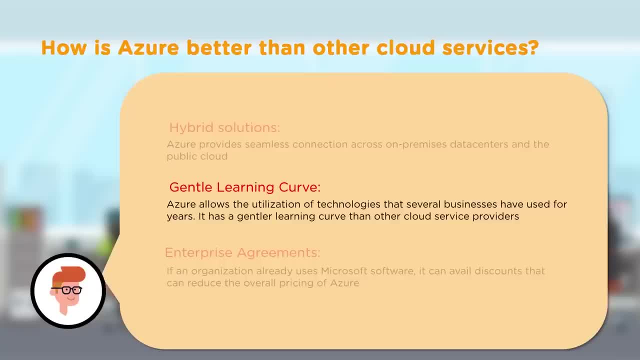 generally missing in other cloud service providers. Now this would really impress the CTOs or people working in finance and budgeting. If an organization is already using Microsoft software, they can definitely go and avail, or be bold and ask for a discount that can reduce the overall Azure. 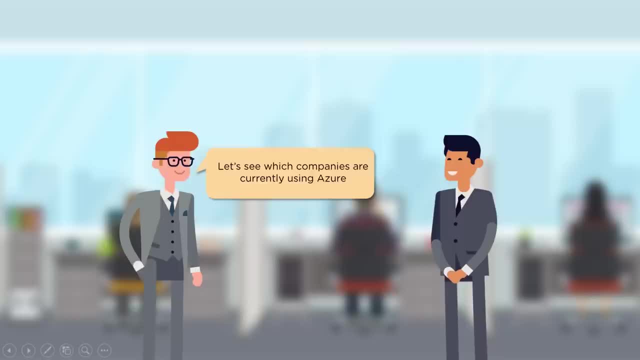 spending, in other words, overall pricing of the Azure. So that's what helped, or they are the information that helped, the CEO pick Azure as his cloud service provider. And then the CEO goes on and talks about the different companies that are currently using Azure. 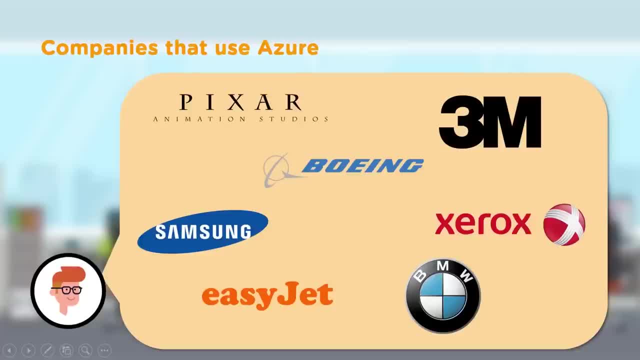 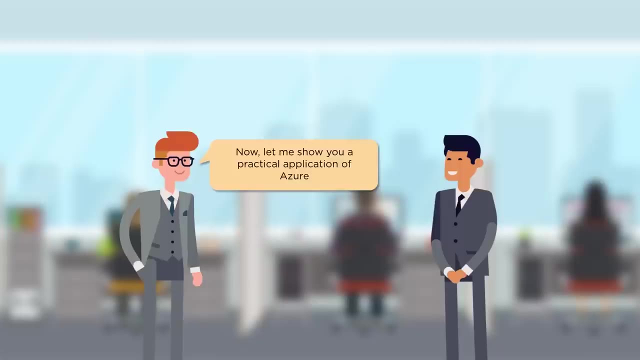 And they are definitely using Azure for a reason. like Pixar, Boeing, Samsung, EasyJet, Xerox, BMW, 3M- They are major multinational, multibillion companies. They rely run, operate their IT in Azure, And this CEO has a thought that his IT person is still not very convinced, unless 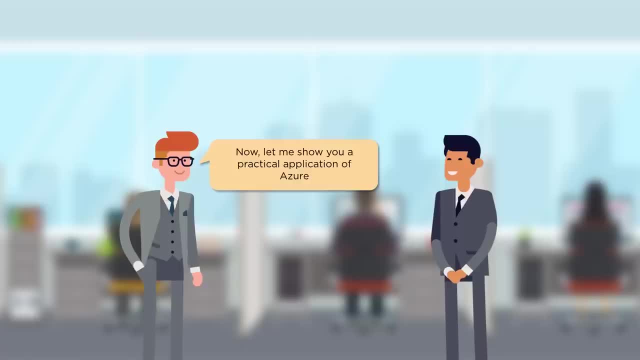 and until he shows him a visual of how easy things are in Azure. So he goes on and explains about a practical application of Azure, which is what exactly I'm going to show you as well. All right, A quick project on building an Azure app. 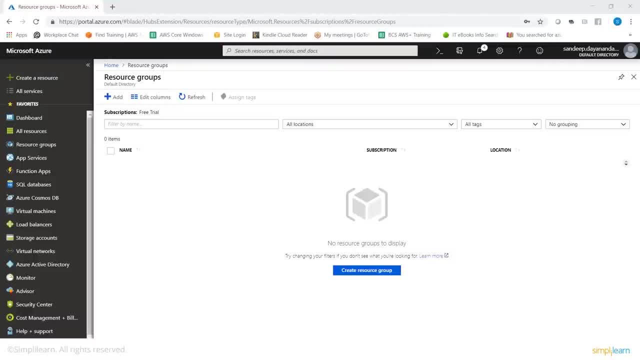 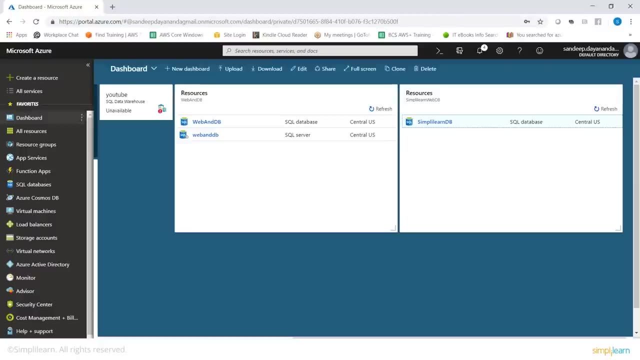 using or building a NET application in Azure web app and making it connect to an SQL database will solidify all the knowledge that we have gained so far. So this is what we're going to do. I have an Azure account open, as you see, logged in and everything is fresh here. 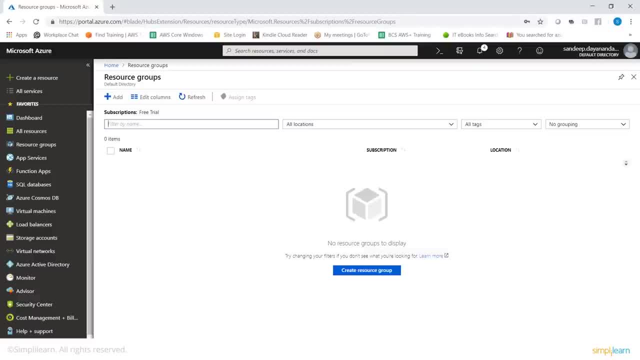 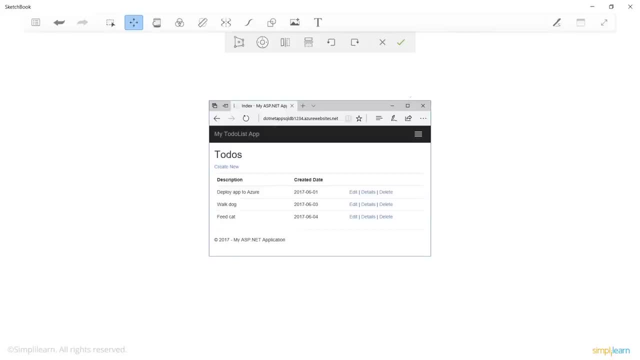 Let me go to resource group. There's nothing in there. It's it's kind of fresh. All right, I'm logged in and this is what we're going to do. So we're going to create an application like this, which is nothing but an to do application: a to do list application. 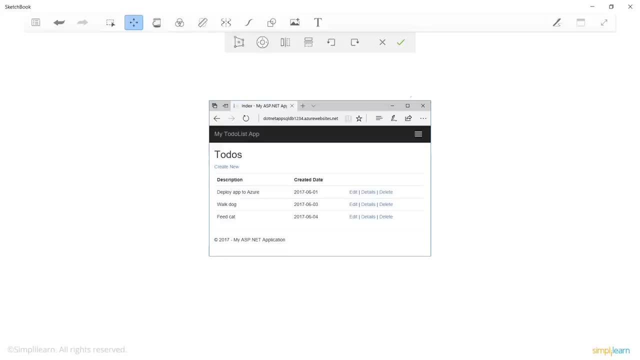 which is going to run from the web app, get information from us and save it in the database that's connected to it. so you can already see it's a secure application, web and DB. All right, So let me go back to my Azure account. 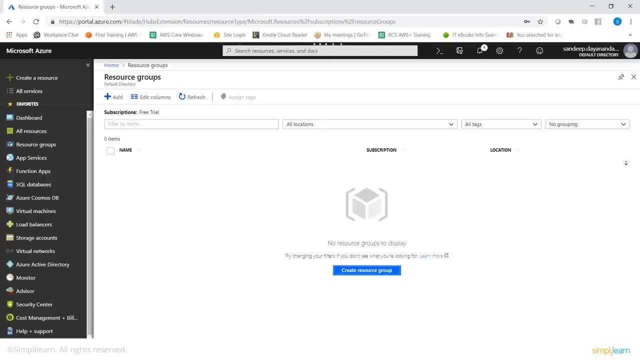 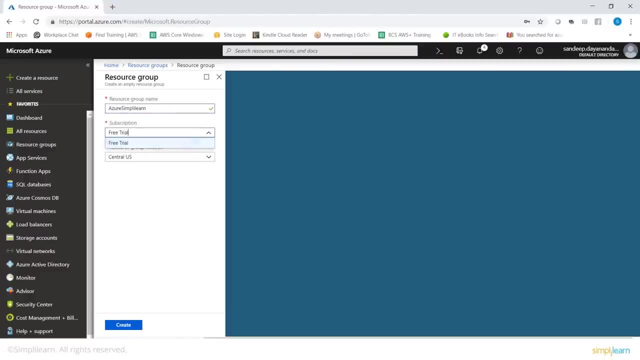 The first thing is to create an resource group. Let's give it a meaningful name. Let's call it Azure. Simply Learn. All right, And it's going to be a free trial. and the location: Pick one that's nearest to you or wherever you want to launch your application. 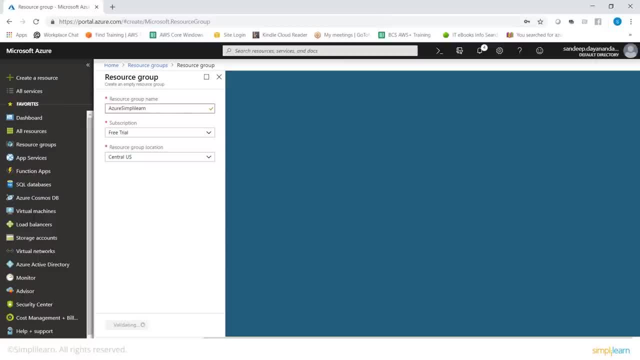 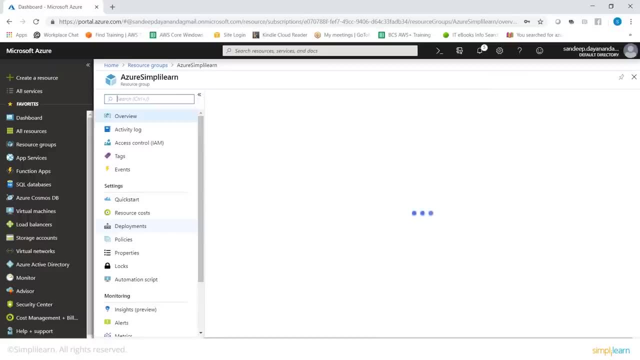 Now for this use case. I'm going to pick Central US And create. It's going to take a while to get created. There you go, It's created. It's called Azure. Simply Learn Now what do we need? 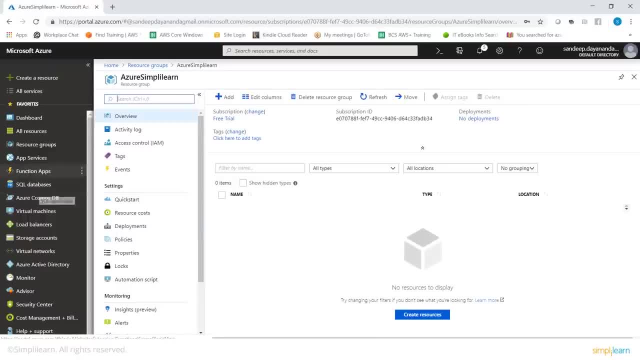 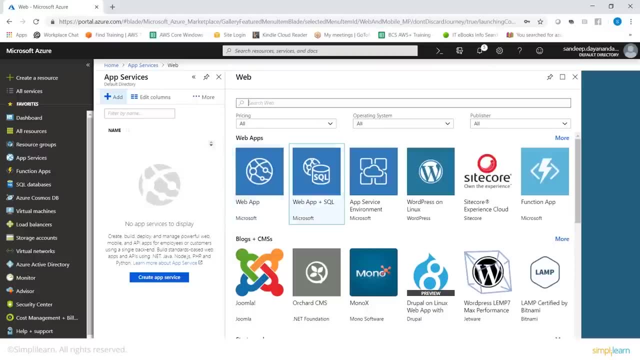 We need a web app and a separate SQL database. Let's first get our web app running, So go to app services and then click on add. It's not the web app plus SQL that we want. We want a web app alone for this example. 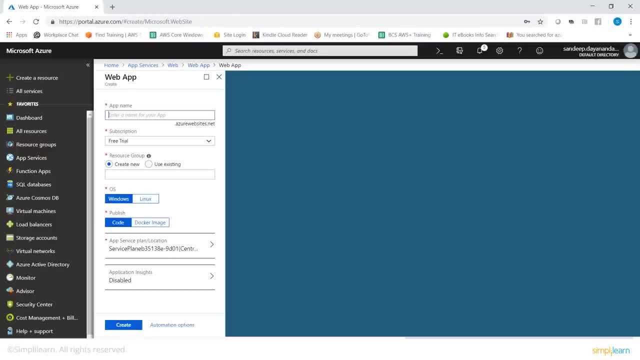 So let's create a web app, give it a quick name. Let's call it Azure, Simply Learn. The subscription is free trial and I'm going to use my existing resource group, a resource group that we created some time back. It's going to run out of Windows and we're going to publish the code. 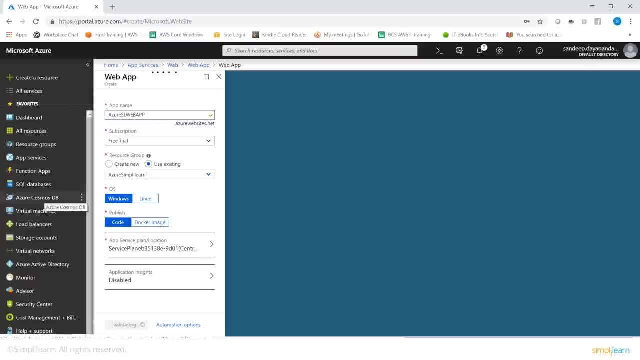 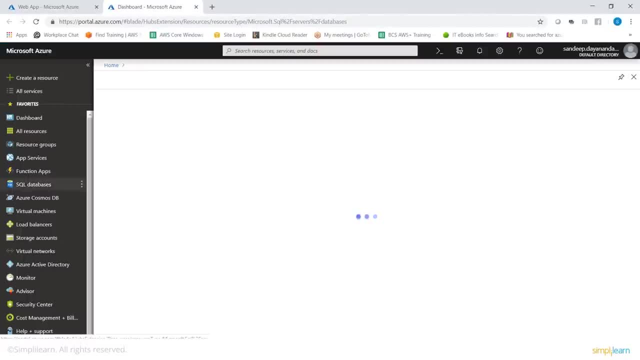 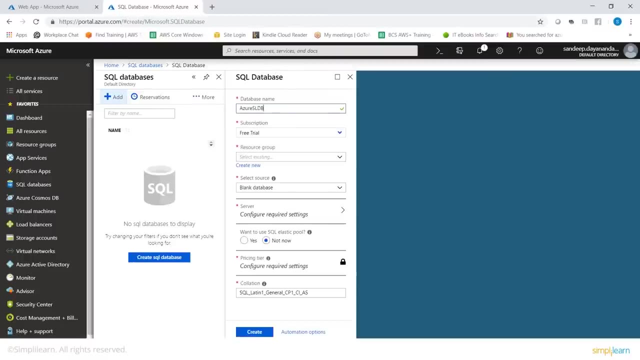 All set, We can create it. All right, While this is running, let me create my database. Right SQL database. create a database, Give it a name. Let's call it Azure. Simply Learn DB. Put it in our existing resource group that we created. 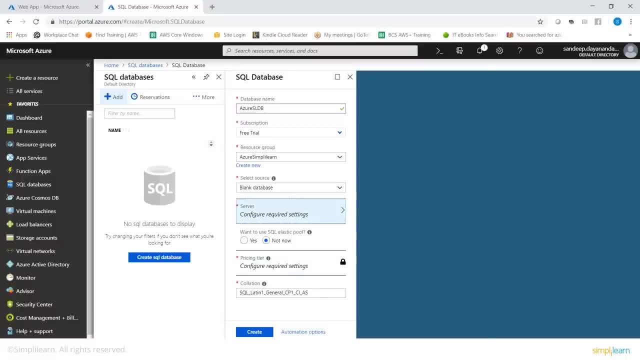 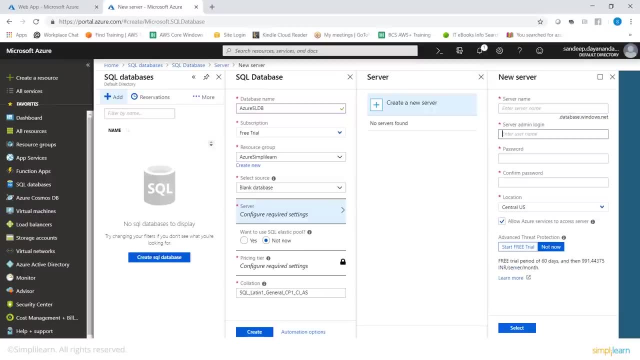 It's going to be a blank database, All right, And it's going to require some settings like the name of the server and the admin login, the password that goes along, and in which location this is going to be created. The server name is going to be Azure- Simply Learn DB. 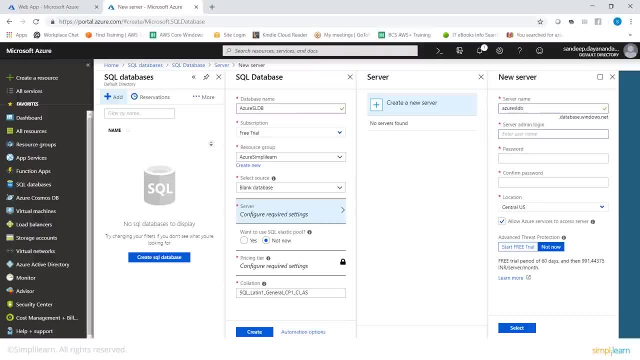 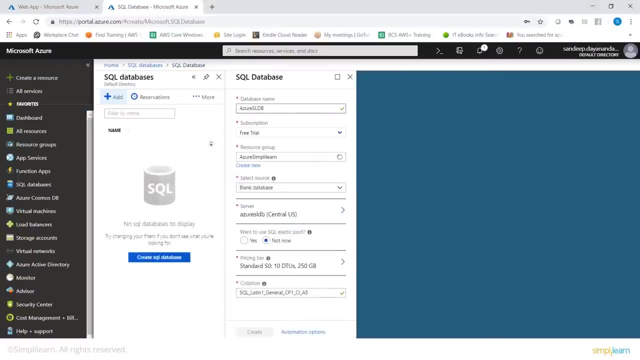 That's the server name The admin login can be. what can be the admin login name? Let's see. So let's call it. Simply Learn: That's my admin login name And let me pick a password, Click on create. So what have we done so far? 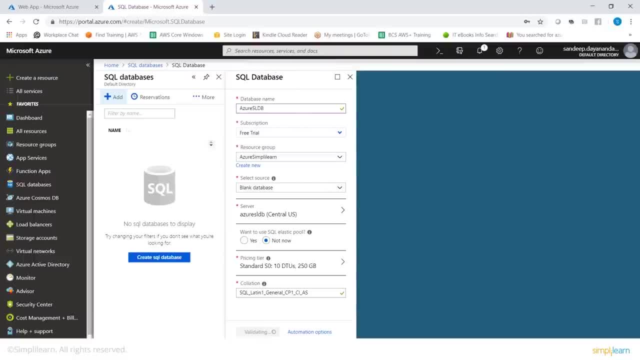 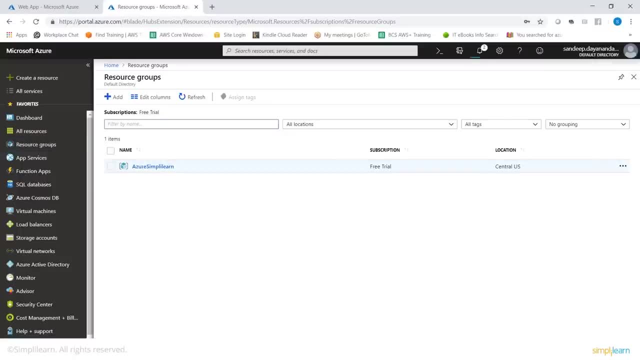 We have created a web app and we have created a database in the resource group that we have created. so if I go to resource group, it's going to take some time before things show up. So if I go to my resource group, I only have one resource group as of now. 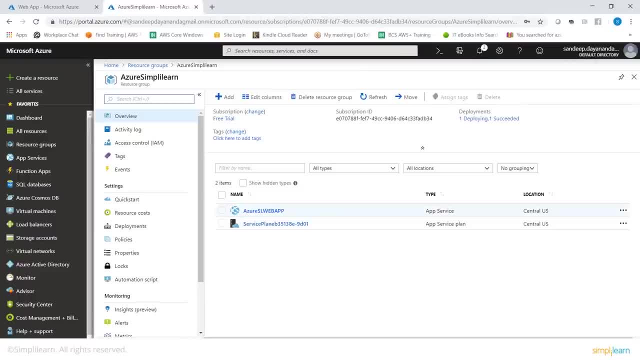 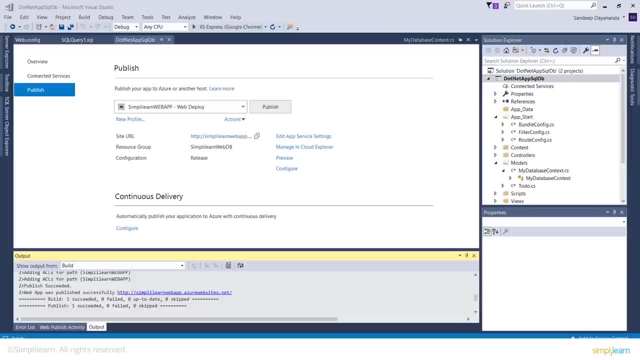 Azure Simply Learn, And there I have a bunch of resources being created and it's still being created. All right. In the meantime, I have my application right here That's running out of, or that's in, Visual Studio as of now, Right, So once the infrastructure is set and ready in the Azure console. 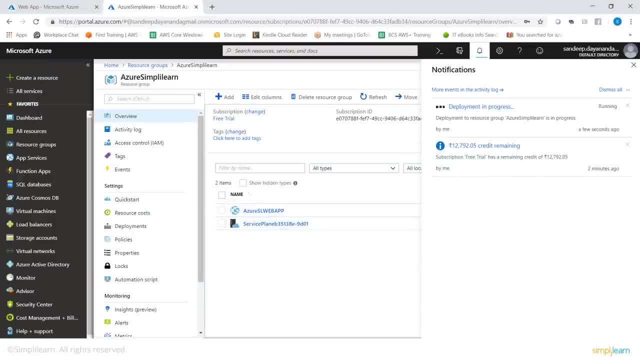 we're going to go back to Visual Studio, feed these inputs in the Visual Studio. So the code knows what the database is, the, the credentials to log into the database, stuff like that. So we're going to feed those information in Visual Studio. 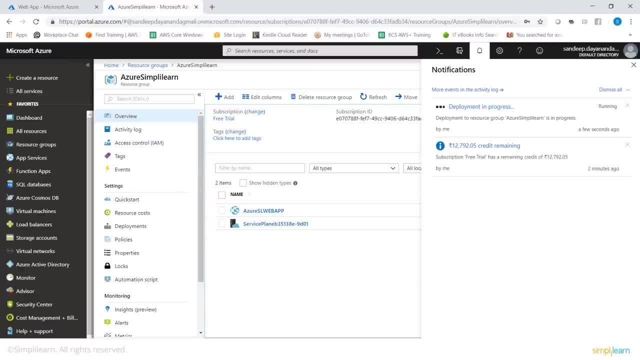 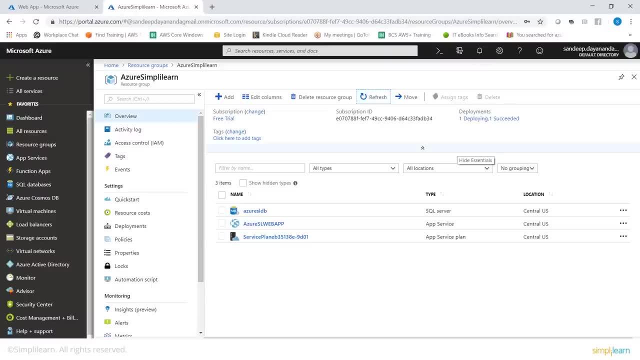 By that we're actually feeding it into the application and then we're going to run it from there. Deploying this application takes quite a while. We really got to be patient. right now We have all the resources that we need for For the application to run. 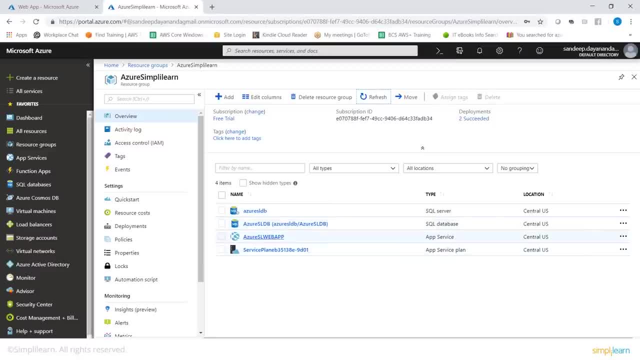 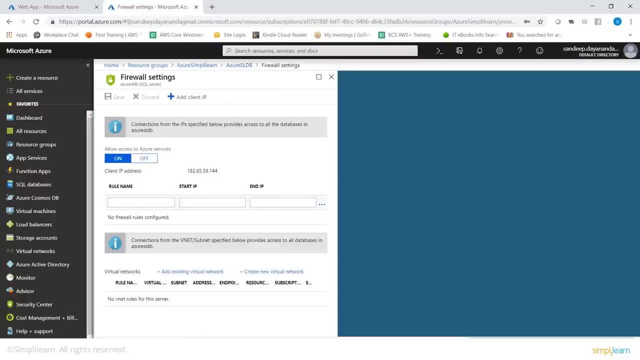 Here's my database and here is my app service. There's one more thing we need to do, that is create and firewall exception rule. So one more thing needed is to create and firewall exception rule, Right? So the application is going to run from my local desktop and it's going to connect to the database. 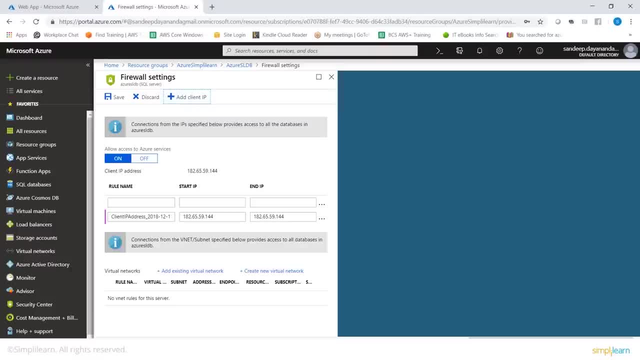 Right, So let's add an exception rule by simply adding the client IP. It's going to pick My IP, the IP of laptop I'm using as of now, and it's going to create an exception to access the database. So that's done. 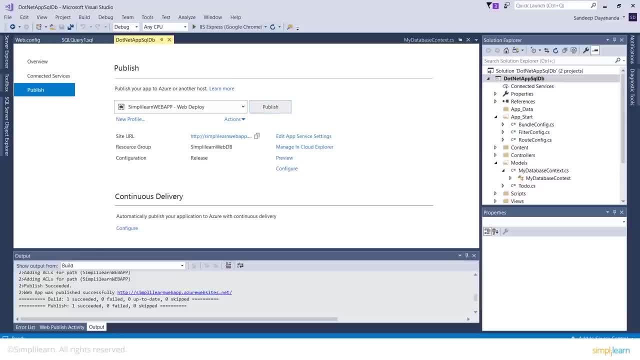 Now we can go back to our Visual Studio. I already have a couple of apps running or a couple of configurations pushed from a Visual Studio. I'm going to clean that up. If you're doing it for the first time, you may not need to do this. 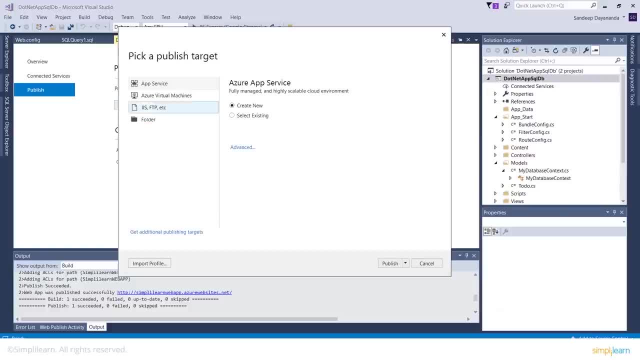 All right, So let's start from scratch. This is very similar to how you would be doing in your environment, Right? So we're going to select an existing Azure app service. Now, before that, I have logged in. As you can see, I have logged in with my credentials. 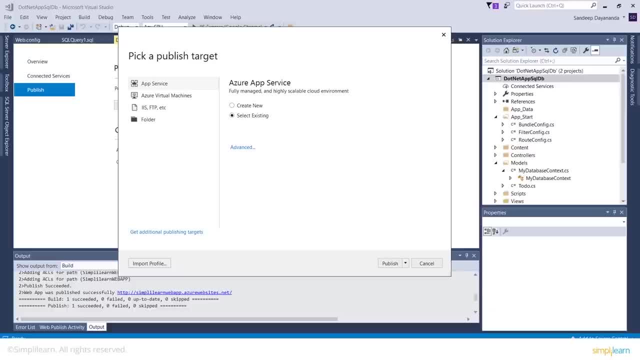 It's going to pull a few things automatically from my Azure account, So in this case I'm going to use an existing Azure app, So select existing and then click on Publish. All right, If you recall, these are the very same resources that we created a while back. 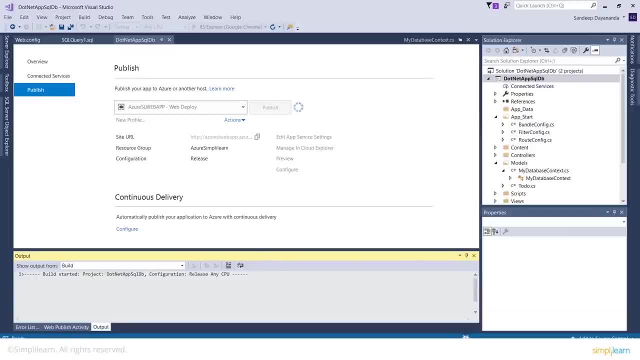 So I'm going to use this one. So I'm going to use this one. So I'm going to use this one. All right, We have clicked on save and it's running kind of validating the code and it's going to come up with an URL. 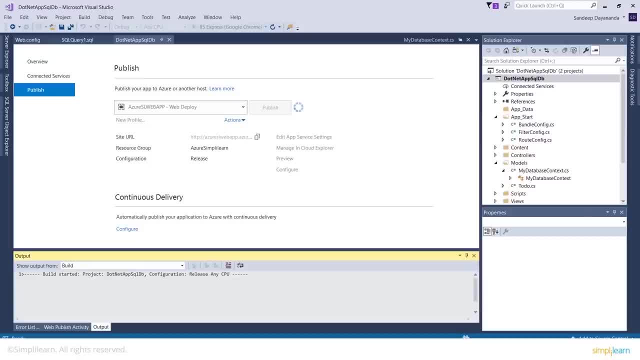 Now, initially, the URL is not going to work because we haven't mapped the application to the database. that would be the next thing. All right, So the app has been published and it's running from my web app. As of now, it's going to throw an error. like you see, it's throwing an error. 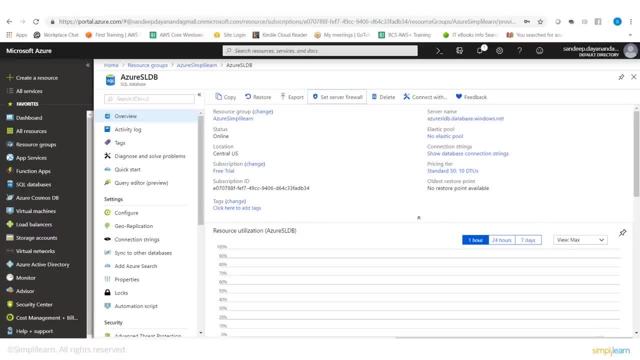 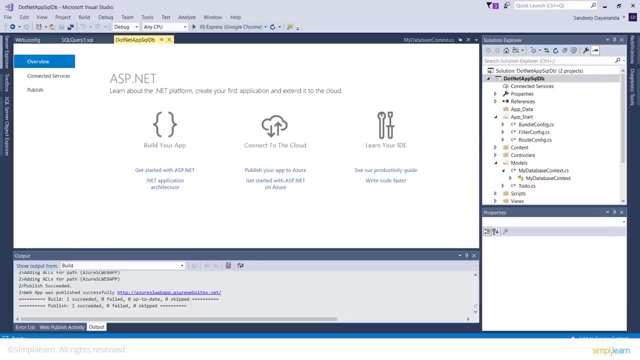 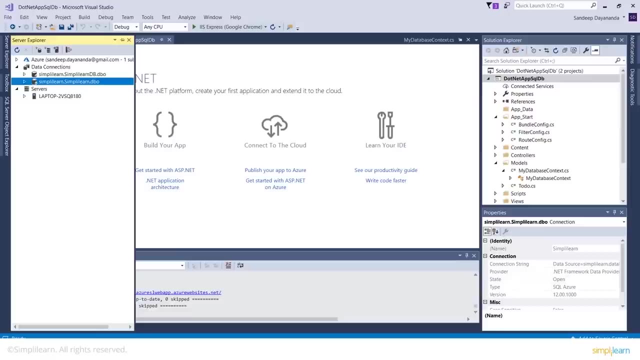 That's because we haven't mapped the app and the DB together, So let's do that. All right, let's do that. So let's go to Server Explorer. This is where we're going to see our databases that we have created. 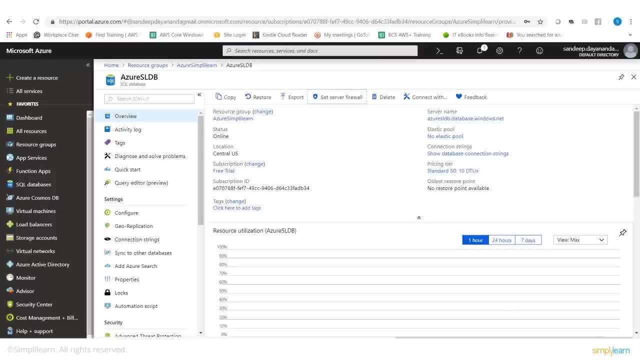 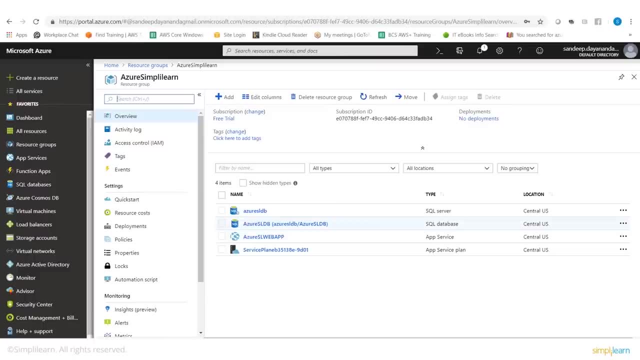 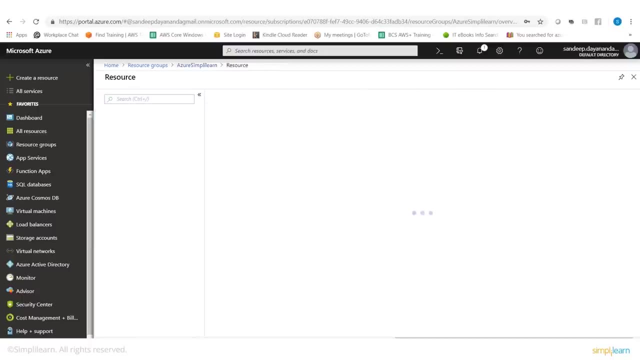 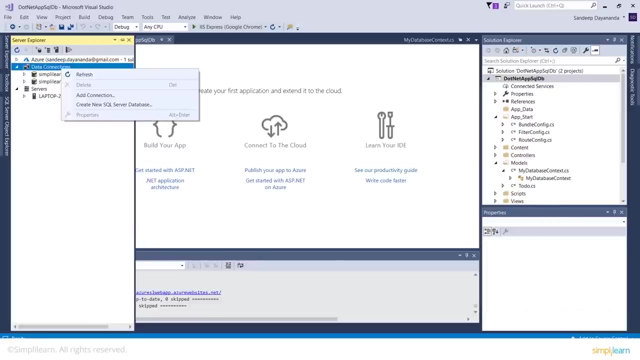 Now let's quickly verify that. Go back to the resource group: Right Appropriate resource group, which is right here And here I have my database: Azure- Simple, Simply learn database. Right. it has some issues connecting to my database. 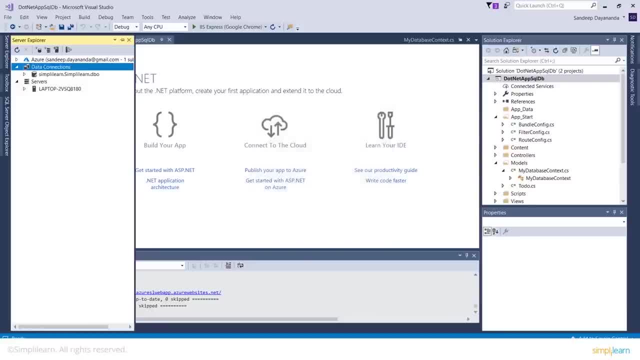 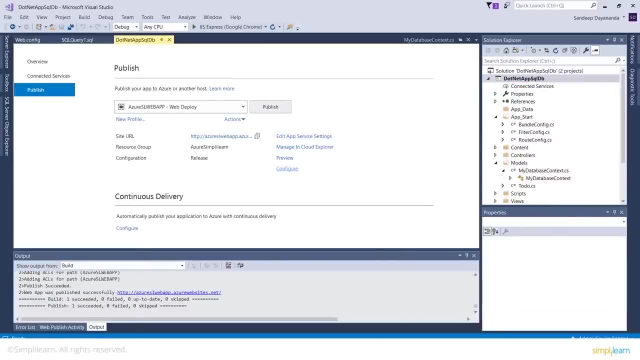 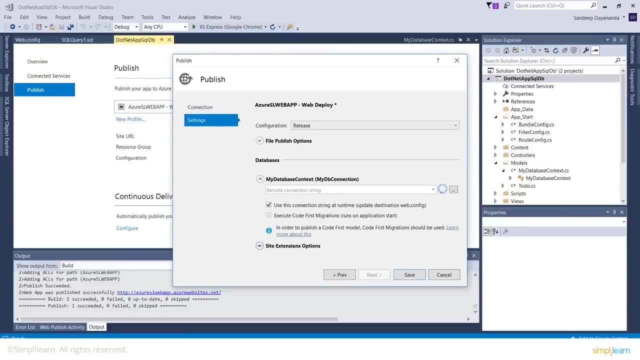 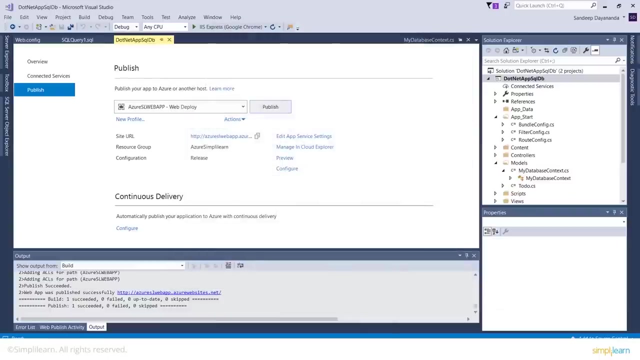 Give me a quick moment. Let's fix it, All right. All right, So we'll have to map the database into this application. All right, So let's go to the Solution Explorer, Click on Publish and a page like this gets shown: 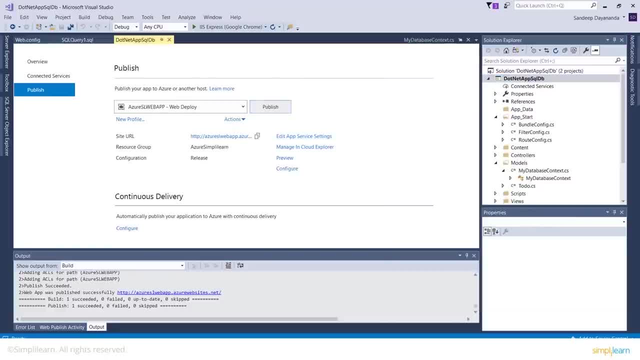 And from here we can go to configure. Here is our web app, All right With all its credentials. Let's go to the Solution Explorer And here we can see that we have a database. We can see that we have a database. 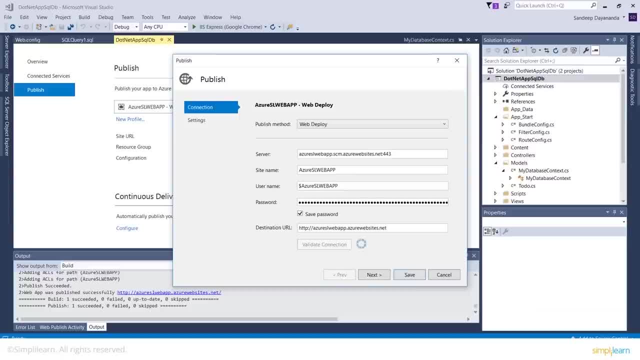 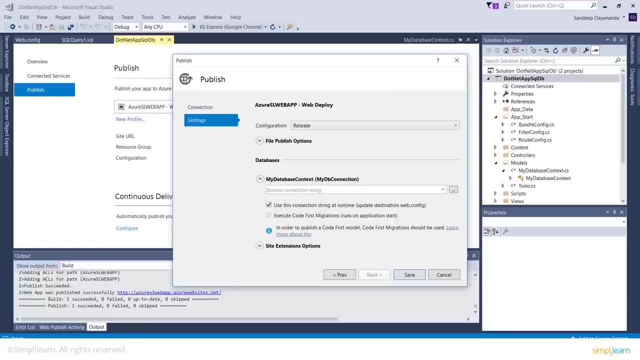 We can see that we have a database. We can see that we have credentials. Let's validate the connection Number one, All right, And then click on next. This is my DB connection string, All right, Which the app is going to use to connect to my DB. 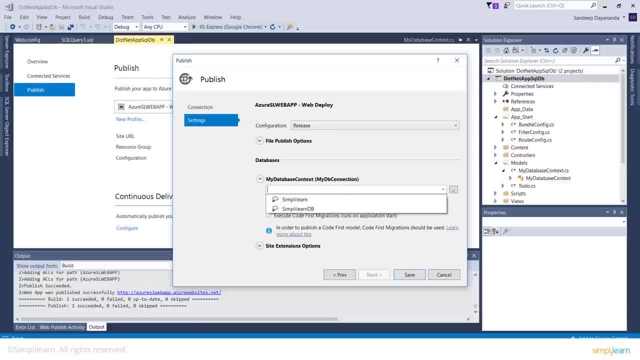 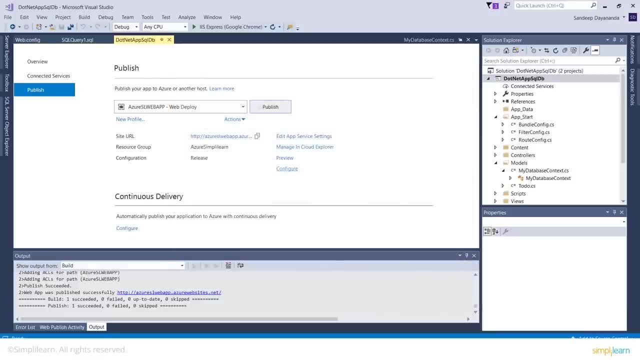 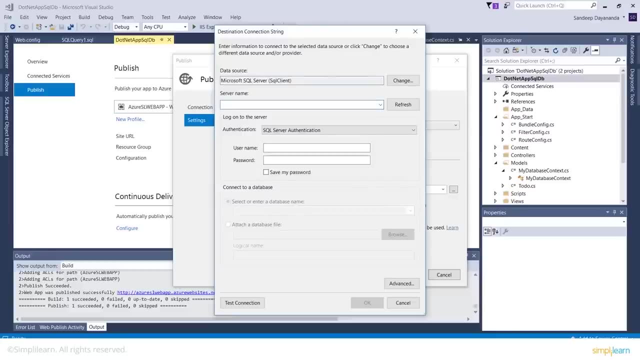 Now, if you recall, our DB was Azure- Simply learn DB- And that's not being shown here. So let's fix that Right. So let's fix that. Click on configure And here let's put our DB servers URL. 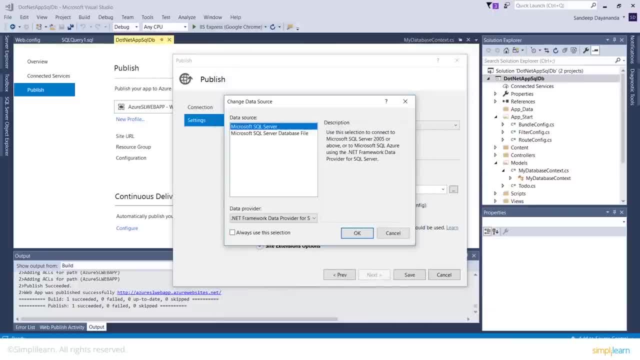 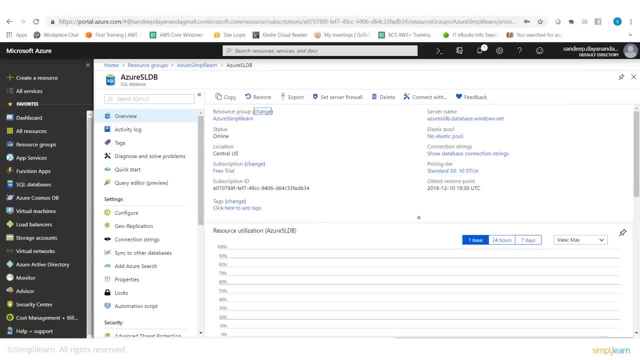 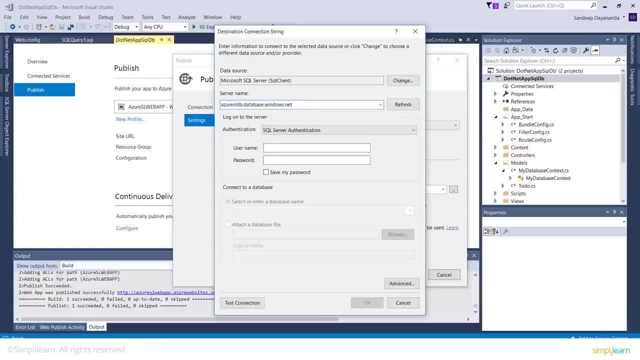 Now, before that, let's change this to SQL server, All right, And then in here put the DB's URL. So go back to Azure. Here is my DB or server's name. Put that here Right: The user name to connect to the server. 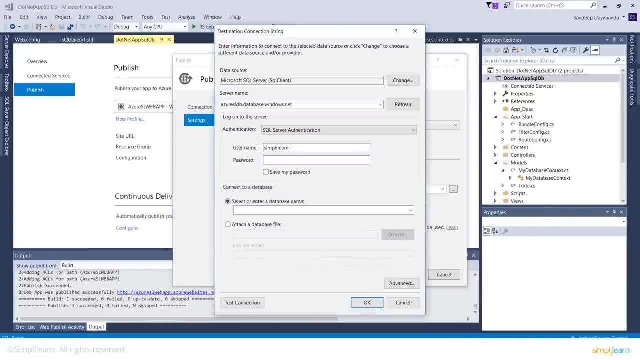 That's right here. Put that in. And the password to connect to the server. Let's put that in Right. It's trying to connect to our Azure portal or the Azure infrastructure. And here is my database. If you recall, it's Azure SLDB. 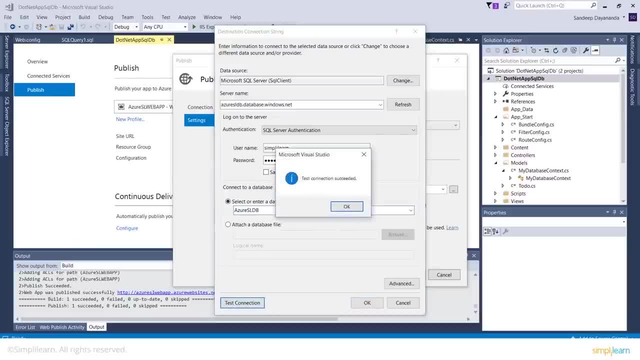 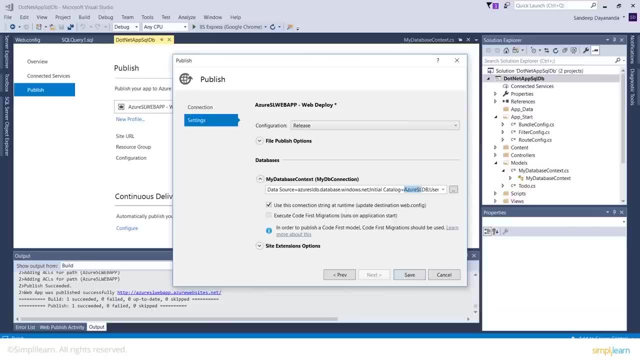 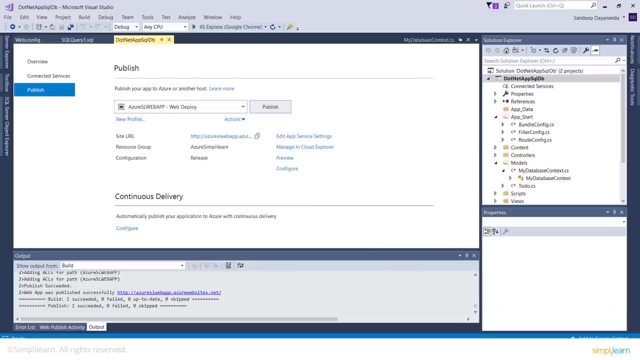 That's the name of the database. Let's test. the connection. Connection is good. Click on OK. So now it's showing up correctly. Azure Simply Learn DB. That's the name of the database that we created. Now it's configured. 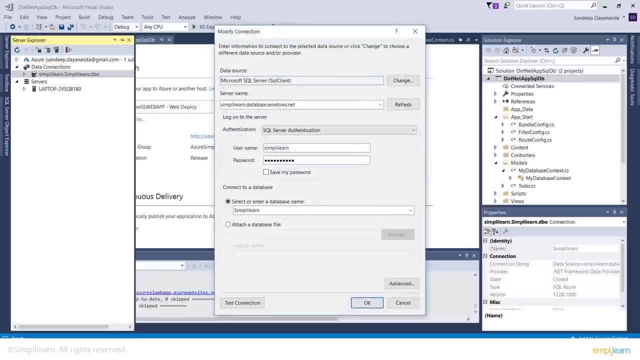 All right, Let's modify the data connections. Let's map it to the appropriate database again. All right, So our name of the database is Azure, Simply Learn DB, And then it's going to be All right. So we're going to change the name of the database. 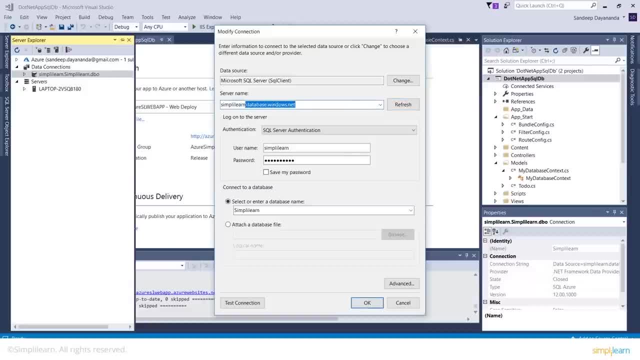 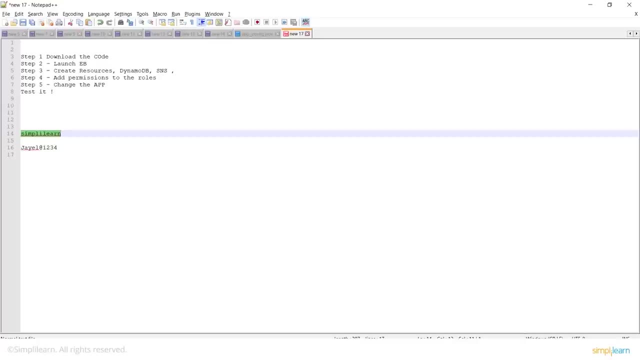 We're going to change the name of the database to Azure Simply Learn DB And then it's going to be SQL Server. That's the data source. The username is Simply Learn And the password is what we have given in the beginning. 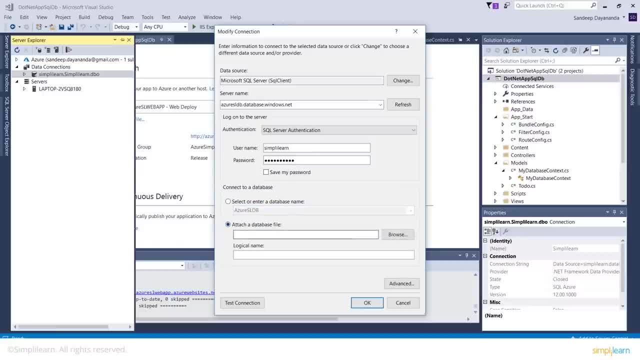 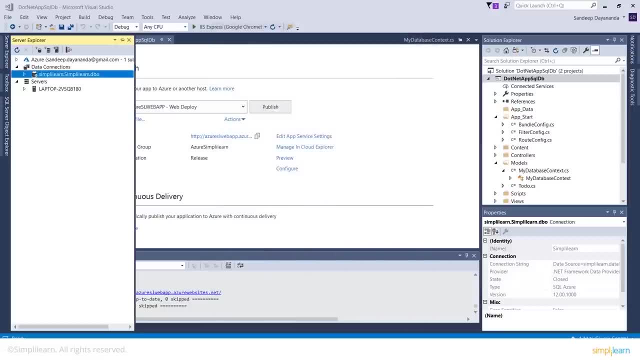 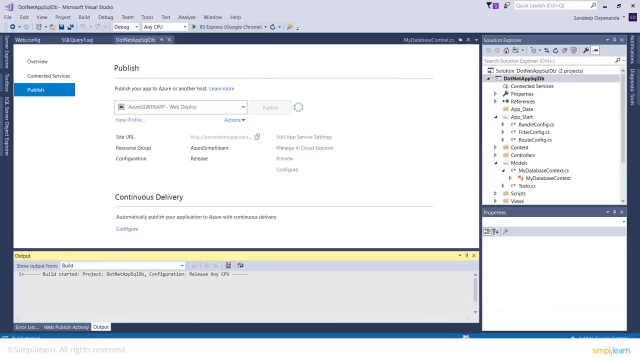 All right, Let's validate the connection. It's good. Click OK. Now we're all set and ready to publish Our application again. Now the application knows how to connect to the database. We have educated it with the correct connection strings. 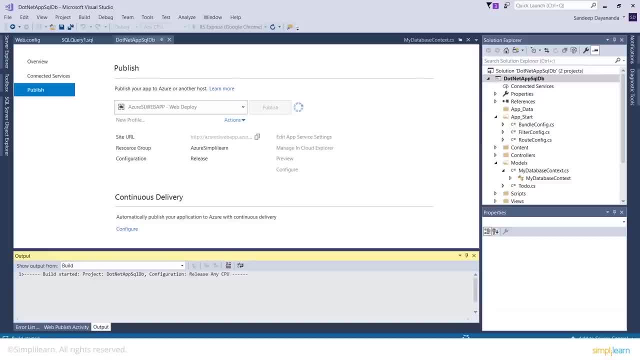 The DNS name, the username and the password for the application to connect to the database. So Visual Studio is building this project And once it is up and running we'll be prompted with an URL to connect And Any time we put or we give inputs to the URL that's going to receive the input and save it in the database. 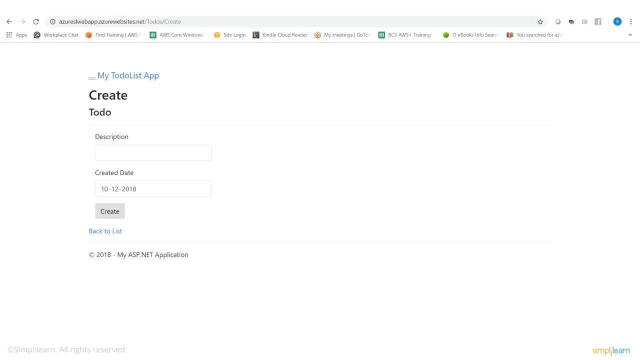 All right, So here is my to do list app and I can start creating to do list For myself. All right, I have the items already listed. I can create an entry and these entries get stored in the in the database. I can create another entry. 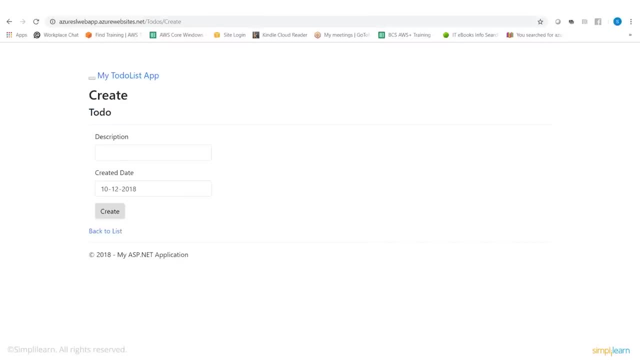 Take the dog for a walk. That's going to get stored. I can create another entry book- tickets for scientific exhibition- And that's going to receive and put that in the database. And that concludes our session. So through the session we saw how I can use Azure services to create a web app. 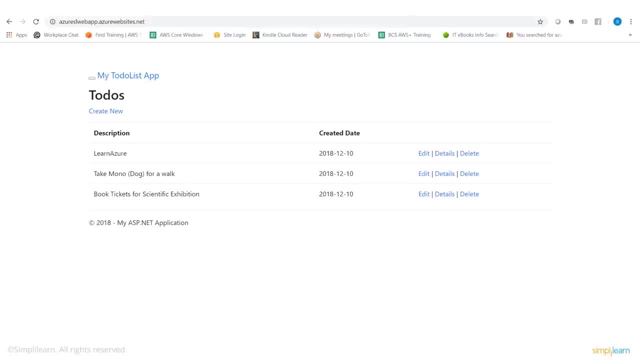 and connect that to the DB instance, and how those two services which are decoupled by default, which are separate by default, how I can use the connection strings to make connection between the app server and the database and be able to create an working app. 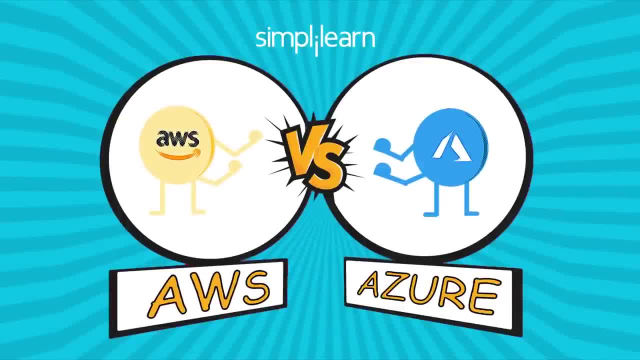 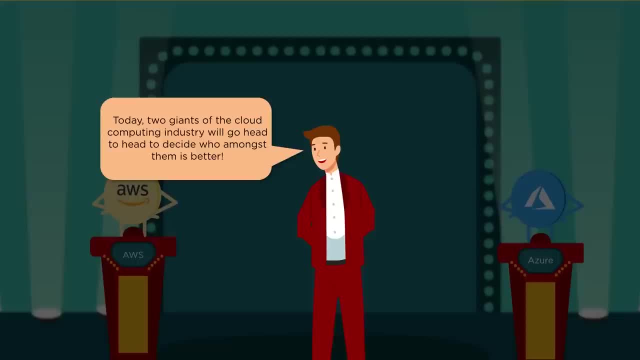 Hi guys, I'm Raul from Simply Learn, And today I'd like to welcome you all to the greatest debate of the century. Today, I'm joined by two giants of the cloud computing industry. They'll be going head to head with each other to decide who amongst them is better. 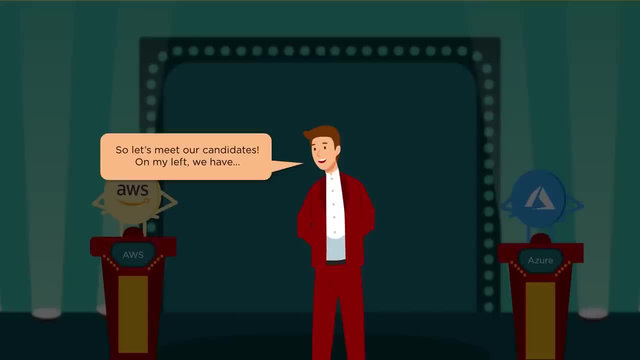 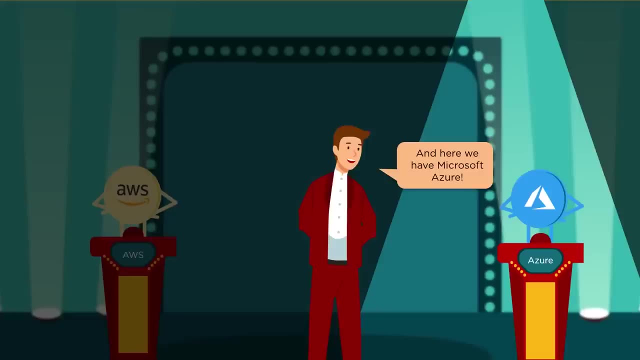 It's going to be one hell of a fight. Now let's meet our candidates. On my left, we have AWS, who's voiced by Apeksha Hi guys. And on my right, we have Microsoft Azure, who's voiced by Anjali. 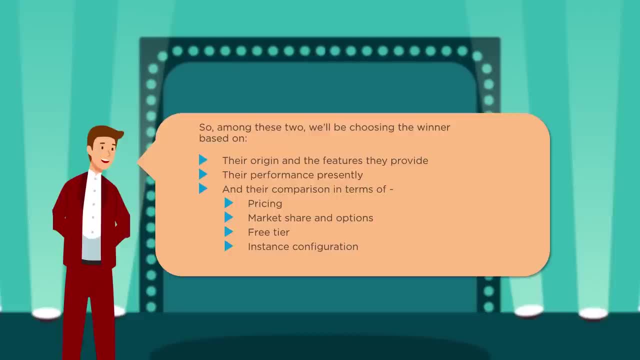 Hey there. So today we'll be deciding who's better on the basis of their origin and the features they provide, their performance in the present day, and comparing them on the basis of pricing, market share and options, free tier and instance configuration. Now let's listen to their opening statements. 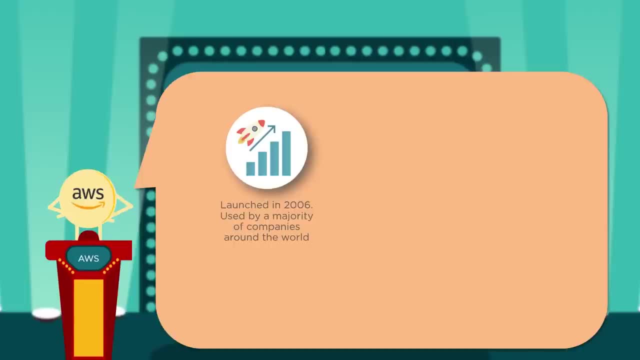 Let's start with AWS. Launched in 2006,, AWS is one of the most commonly used cloud computing platforms across the world. Companies like Adobe, Netflix, Airbnb, HTC, Pinterest and Spotify have put their faith in AWS for their proper functioning. 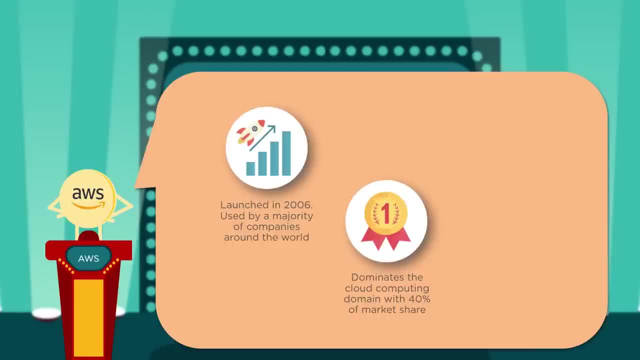 It also dominates the cloud computing domain With almost 40% of the entire market share. So far, nobody's even gotten close to beating that number. AWS also provides a wide range of services that covers a great number of domains- Domains like compute, networking, storage, migration and so much more. 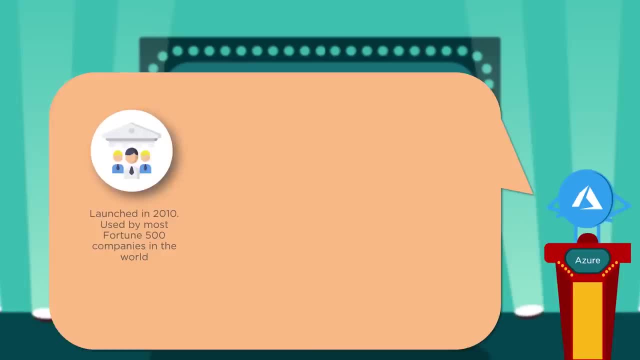 Now let's see what Azure has to say about that. Azure was launched in 2010 and is trusted by almost 80% of all Fortune 500 companies. The best of the best companies in the world Choose to work only with Azure. 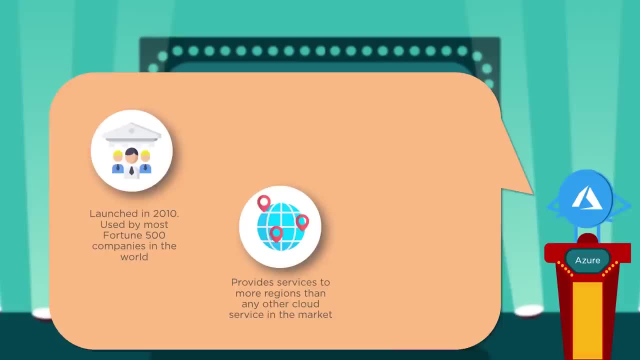 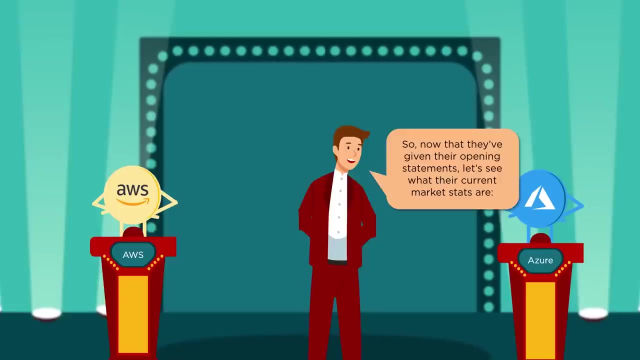 Azure also provides its services to more regions than any other cloud service provider in the world. Azure covers 42 regions already, and 12 more are being planned to be made. Azure also provides more than 100 services spanning a variety of domains. Now that the opening statements are done, let's have a look at the current market status of each of our competitors. 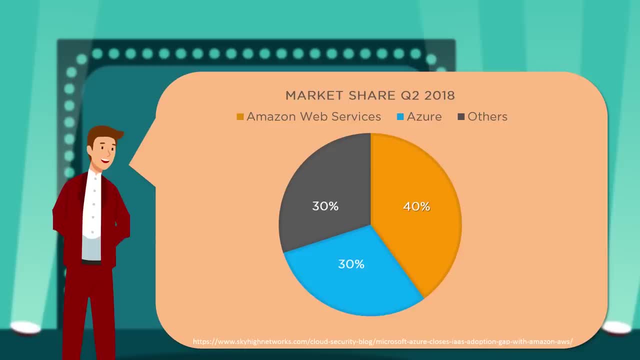 This is the performance round. Here we have the stats for the market share of AWS, Azure and other cloud services. This is for the early 2018 period. Amazon Web Services takes up a whopping 40% of the market share, Closely followed by Azure at 30% and other cloud services adding 30%. 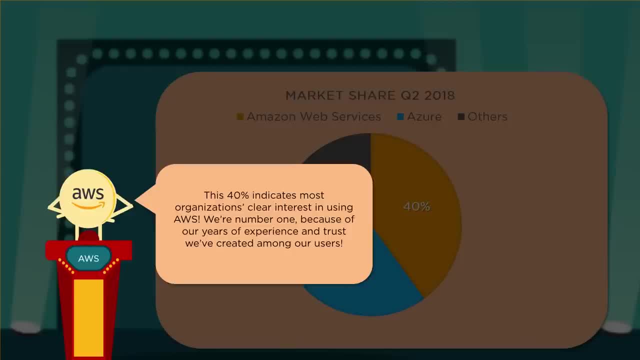 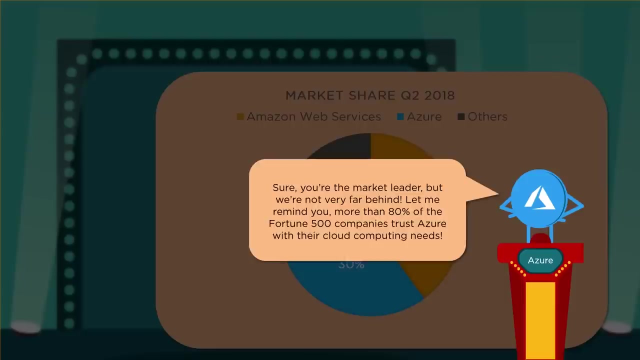 This 40% indicates most organizations' clear interest in using AWS. We are number one because of our years of experience and trust we've created among our users. Sure, you're the market leader, but we're not very far behind. Let me remind you, more than 80% of the Fortune 500 companies trust Azure with their cloud computing needs. 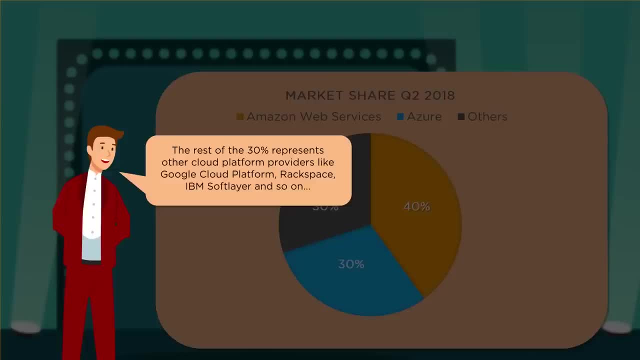 So it's only a matter of time before Azure takes the lead. The rest of the 30% that is in AWS or Azure accounts to the other cloud service providers like Google Cloud Platform, Rackspace, IBM, SoftLayer and so on. Now for our next round, the comparison round. First we'll be comparing pricing. We'll be looking at the cost of a very basic instance, which is a virtual machine of two virtual CPUs and 8GBs of RAM. For AWS. this will cost you approximately $0.0928 per hour. 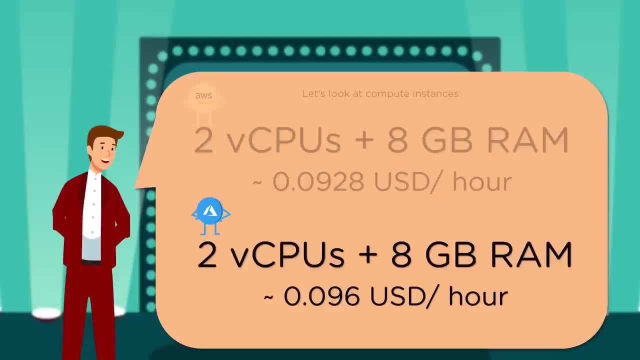 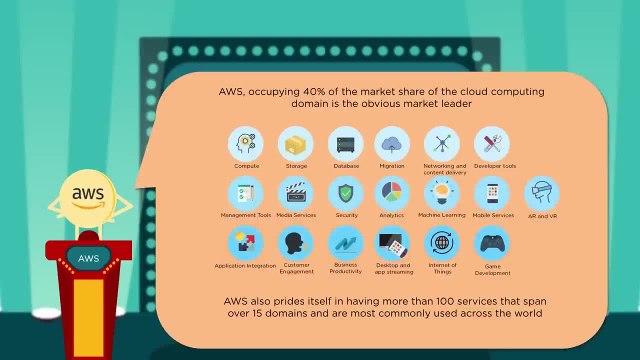 And for the same instance in Azure. it'll cost you approximately $0.096 per hour. Next up, let's compare market share and options. As I mentioned before, AWS is the undisputed market leader when it comes to the cloud computing domain, taking up 40% of the market share. 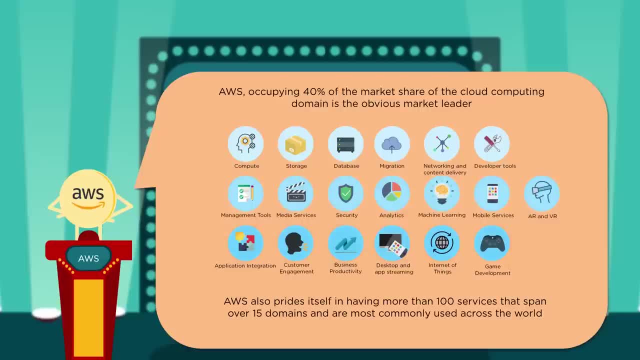 By 2020,, AWS is also expected to produce twice as much of its current revenue, which comes close to $44 billion. Not to mention, AWS is constantly expanding its already strong roster of more than 100 services to fulfill the shifting business requirements of organizations. 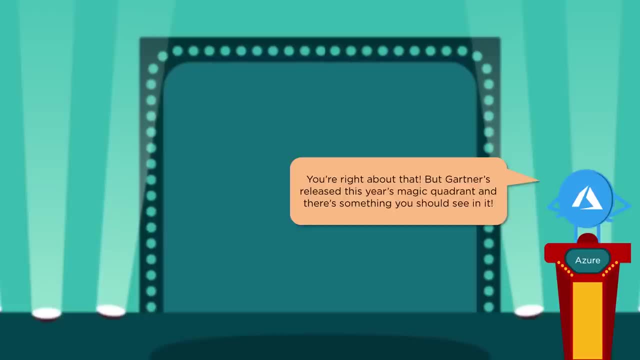 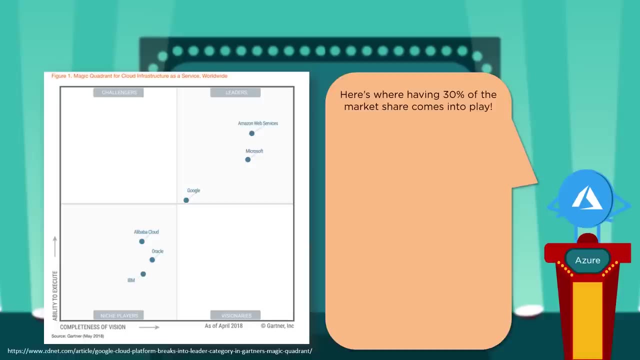 All that is great, really good for you, But the research company Gartner has released a magic quadrant that you have to see. You see, the competition is now neck-to-neck between Azure and AWS. It's only a matter of time before Azure can increase from its 30%. market share and surpass AWS. This becomes more likely considering how all companies are migrating from AWS to Azure to help satisfy their business needs. Azure is not far behind AWS when it comes to services as well. Azure's service offerings are constantly updated and improved on to help users. 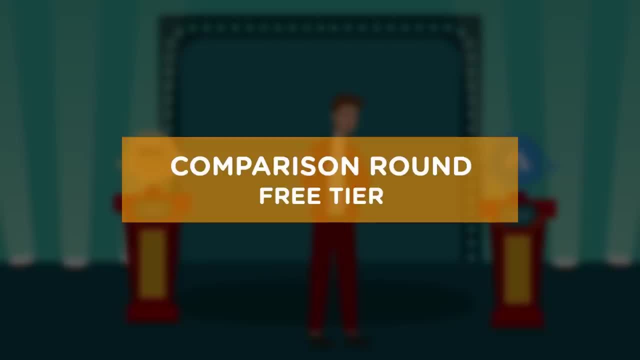 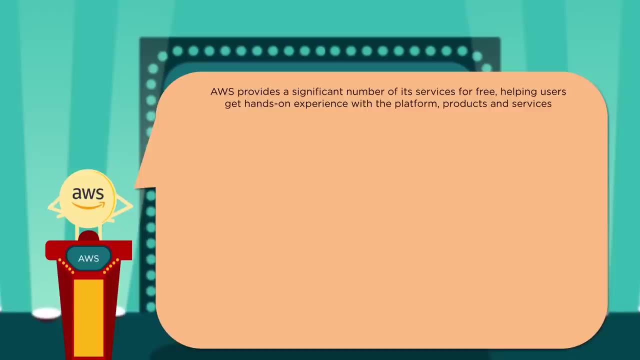 satisfy their cloud computing requirements. Now let's compare AWS and Azure's free offerings. AWS provides a significant number of its services for free, helping users get hands-on experience with the platform products and services. The free tier services fall under two categories. services that will remain free forever and the others that are valid only for one year. The always free category offers more than 20 services, for example, Amazon, SNS, SQS, CloudWatch, etc. And the valid for a year category offers approximately 20 services. 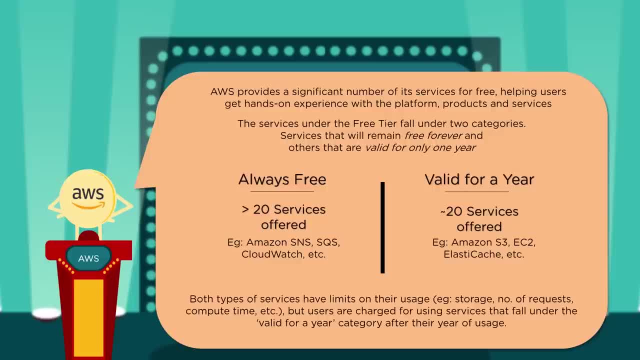 such as Google, Amazon S3, EC2, ElastiCache, etc. Both types of services have limits on their usage, for example, storage, number of requests, compute time, etc. But users are only charged for using services that fall under the valid for a year category. 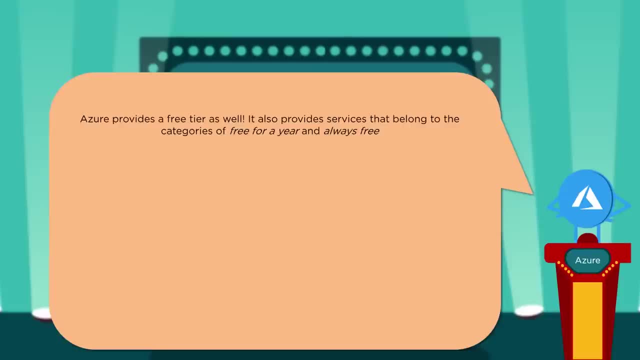 after a year of their usage, Azure provides a free tier as well. It also provides services that belong to the categories of free for a year and always free. There are about 25 plus always free services provided by Azure. These include App Service Functions, Container Service, Active Directory and lots more. 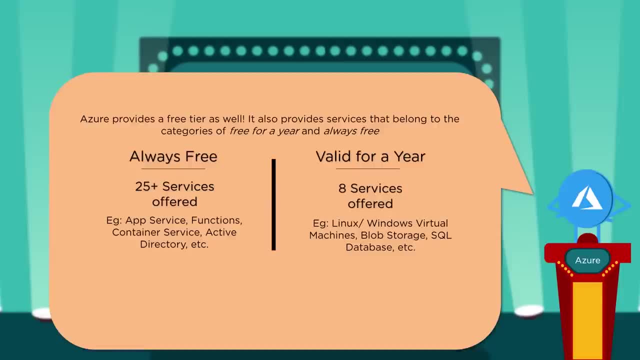 And as of the valid for a year. there are 8 services offered. There's Linux or Windows, Virtual Machines, Blob Storage, SQL Database and few more. Azure also provides the users with credits of $200 to access all their services for 30 days. 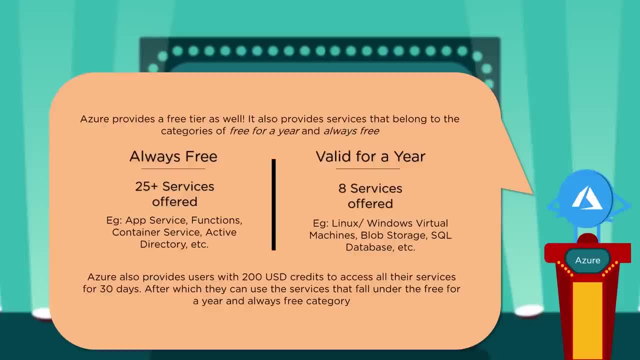 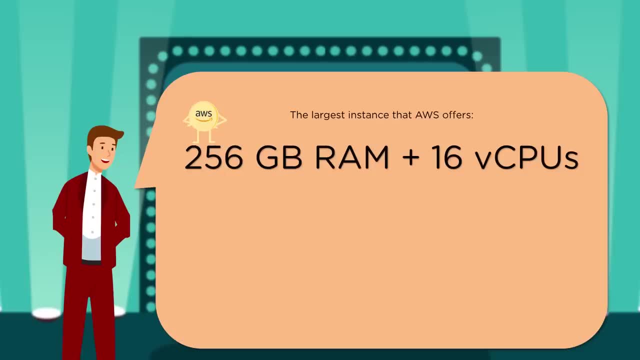 Now, this is a unique feature that Azure provides, where its users can use their credits to utilize any service of their choice. Now let's compare instance configuration. The largest instance that AWS offers is that of a whopping 256GB of RAM and 16 virtual CPUs. 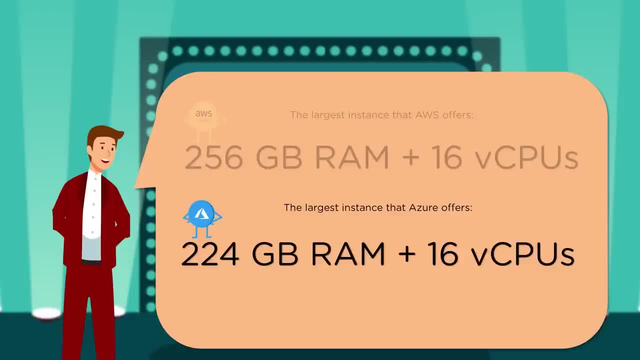 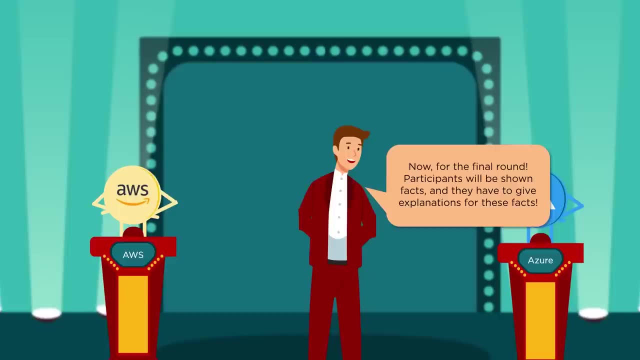 The largest that Azure offers isn't very far behind either: 224GB of RAM and 16 virtual CPUs. And now for the final round. Now, each of our contestants will be shown facts and they have to give explanations for these facts. 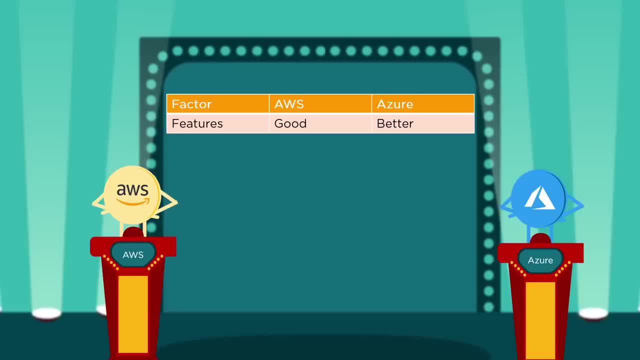 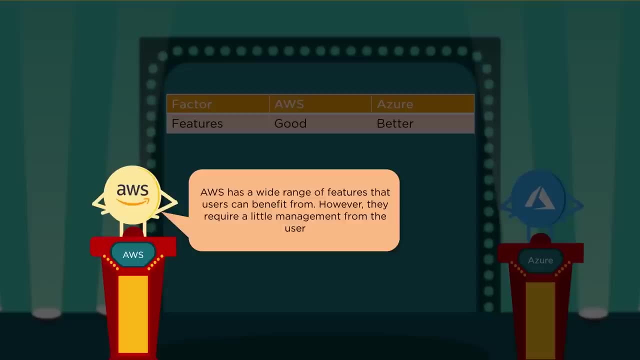 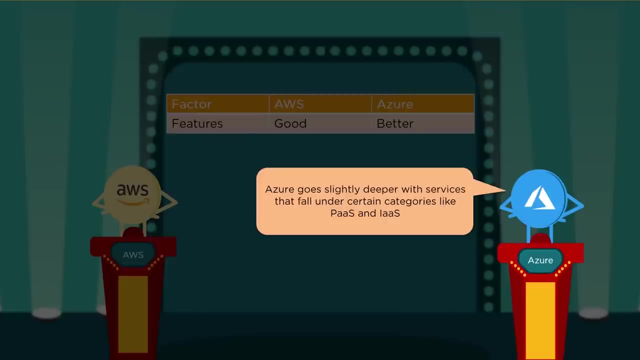 We call it the rapid fire round. First, we have features in which AWS is good and Azure is better. AWS does not cut down on the features it offers its users. However, it requires slightly more management on the user's part. Azure goes slightly deeper with the services that fall under certain categories. 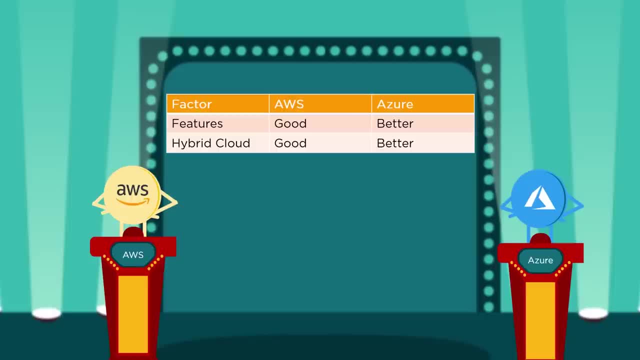 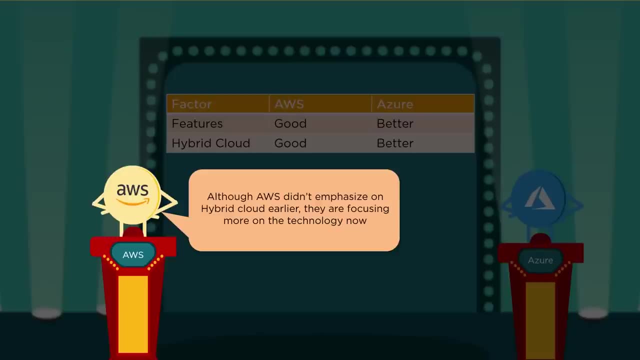 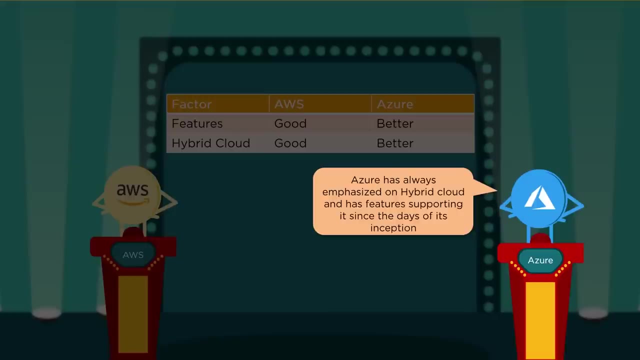 like platform as a service and infrastructure as a service. Next, we have hybrid cloud, where AWS is good and Azure is better. Okay, although AWS did not emphasize on hybrid cloud earlier, they are focusing more on technology now. Azure has always emphasized on hybrid cloud. 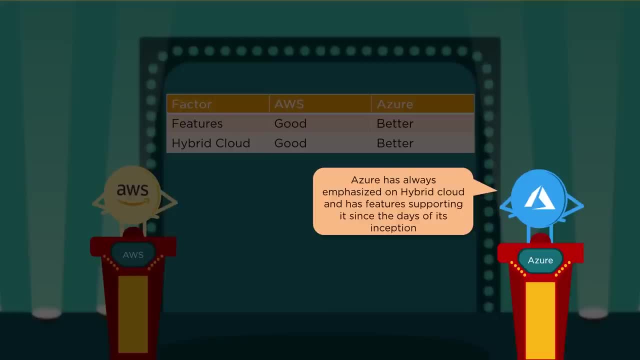 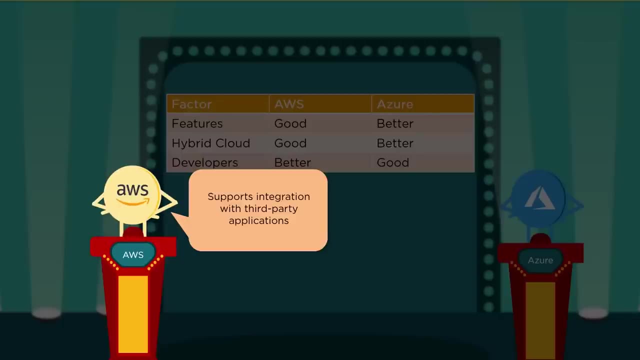 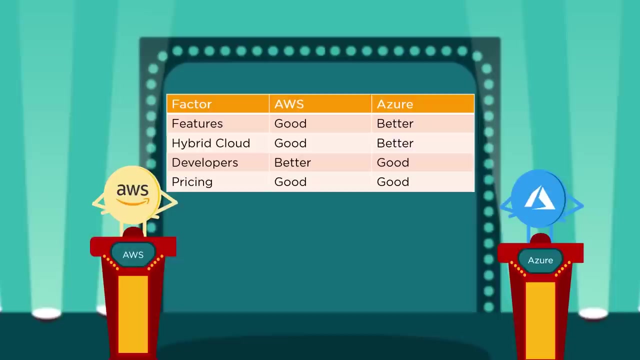 and has features supporting it since the days of its inception. For developers, AWS is better and Azure is good. Of course, it's better because AWS supports integration with third-party applications. Well, Azure provides access to data centers that provide a scalable architecture. For pricing, both AWS and Azure are at the same level. It's good for AWS because it provides a competitive and constantly decreasing pricing model, And, in the case of Azure, it provides offers that are constantly experimented upon to provide its users with the best experience. 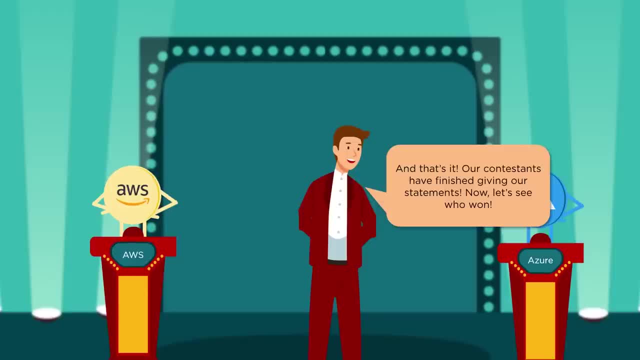 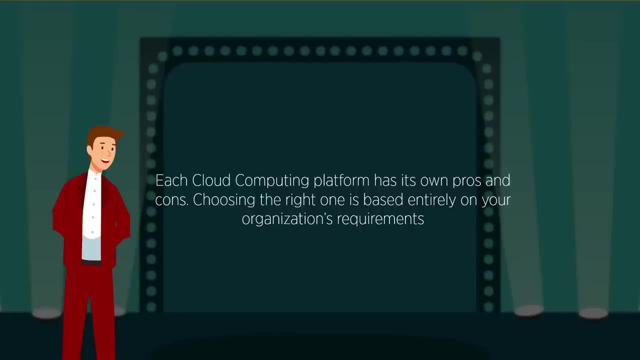 And that's it. Our contestants have finished giving their statements. Now let's see who won. Surprisingly, nobody. Each cloud computing platform has its own pros and cons. Choosing the right one is based entirely on your organization's requirements, Hi guys. 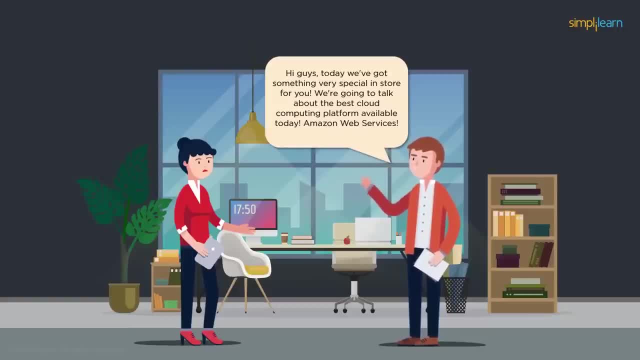 We've got something very special in store for you. We're going to talk about the best cloud computing platform available: Amazon Web Services. Uh, Rahul, I think you said something wrong here. The best cloud computing platform is obviously Google Cloud Platform. 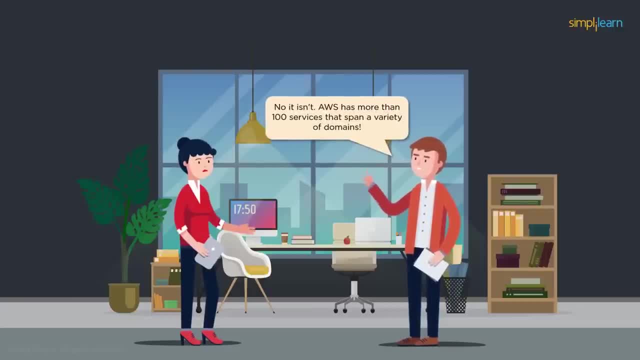 No, it isn't. AWS has more than 100 services that span a variety of domains- Alright, but Google Cloud Platform has cheaper instances. What do you have to say about that? Well, I guess there's only one place we can actually discuss this. 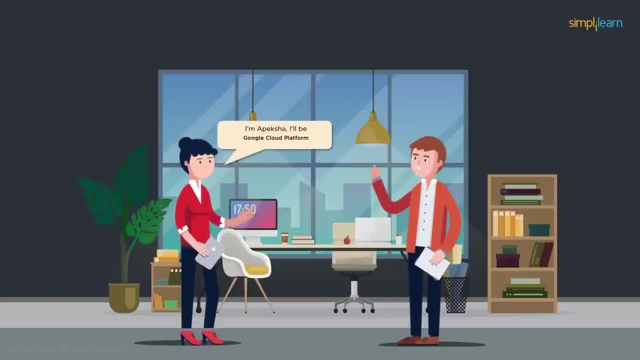 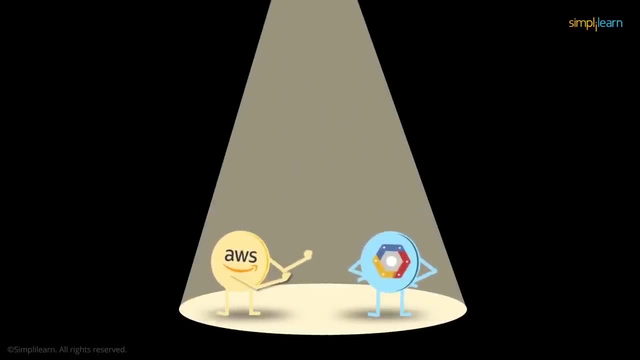 a boxing ring. So, guys, I'm Apeksha and I will be Google Cloud, And I'm Rahul, I'll be AWS. So welcome to Fight Night. This is AWS versus GCP. The winner will be chosen on the basis of their origin and the features they provide. 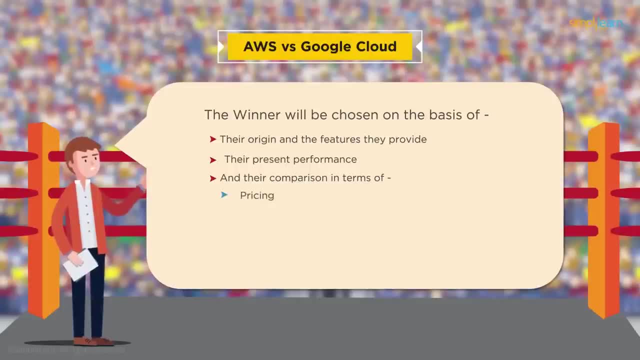 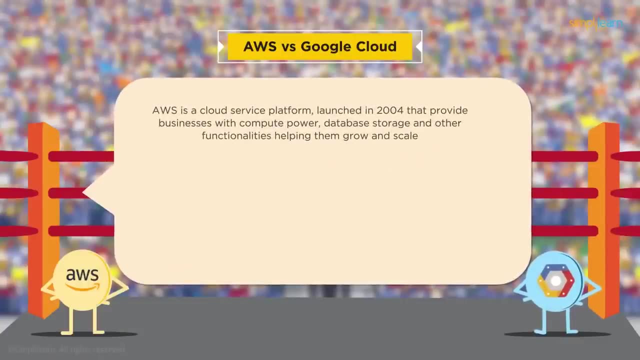 their performance in the present day and comparing them on the basis of pricing, market share and options- the things they give you for free- and instance configuration. Now, first let's talk about AWS. AWS was launched in 2004 and is a cloud service platform. 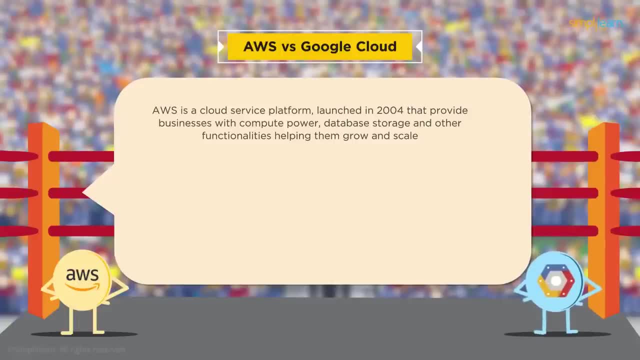 that helps businesses grow and scale by providing them services in a number of different domains. These domains include compute, database storage, migration, networking and so on. A very important aspect about AWS is its years of experience. Now AWS has been in the market a lot longer than any other cloud service platform. 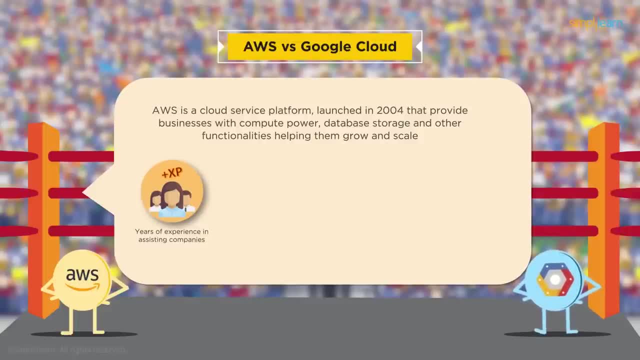 which means they know how businesses work and how they can contribute to the business growing. Also, AWS has over $5.1 billion of revenue in the last quarter. This is a clear indication of how much faith and trust people have in AWS. They occupy more than 40% of the market, which is a significant chunk of the cloud computing market. 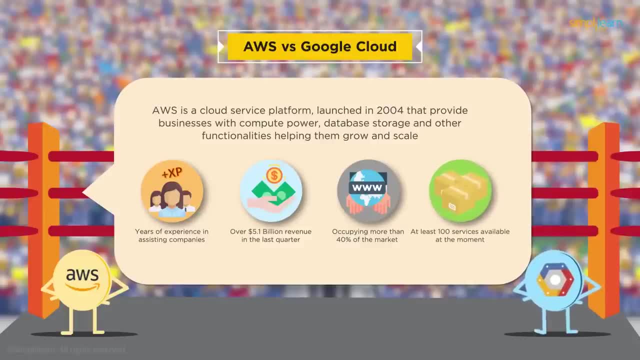 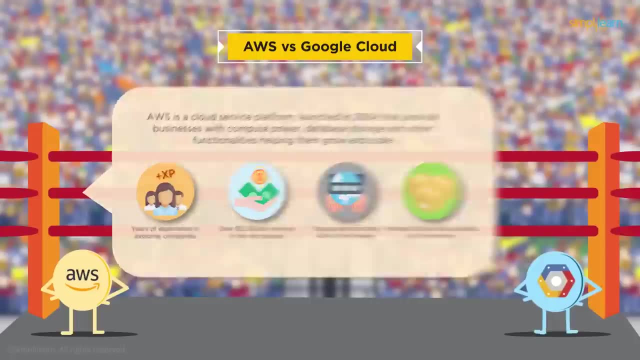 They have at least 100 services that are available at the moment, which means just about every issue that you have can be solved with an AWS service. Now, that was great, but now can we talk about GCP. I hope you know that GCP was launched very recently, in 2011. 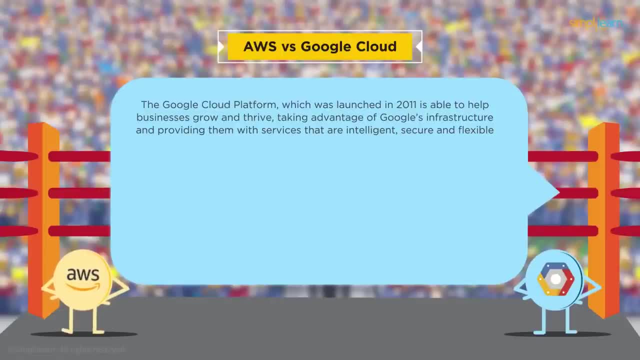 and it is already helping businesses significantly with a suite of intelligent, secure and flexible cloud computing services. It lets you build, deploy and scale applications, websites, services on the same infrastructure as Google. The intuitive user experience that GCP provides- with dashboards, wizards, is way better in all the aspects. 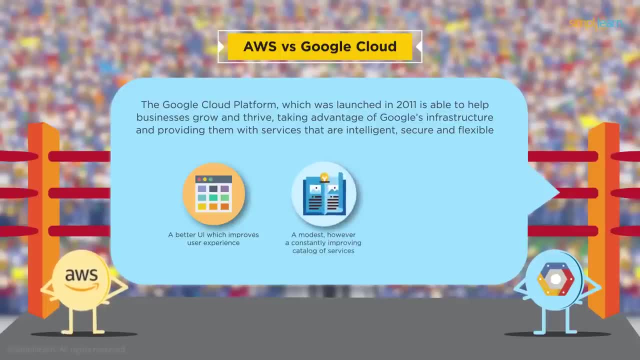 GCP has just stepped in the market and it is already offering a modest number of services And the number is rapidly increasing. And the cost for a CPU instance or regional storage that GCP provides is a whole lot cheaper And you also get a multi-regional cloud storage. 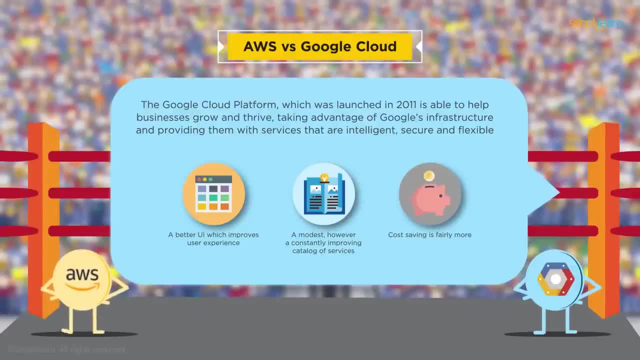 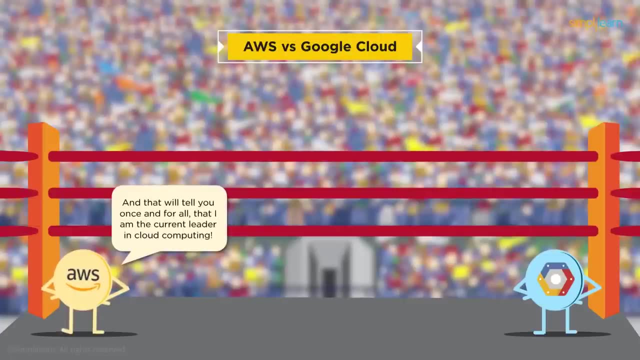 Now, what do you have to say on that? I'm so glad you asked. Let's look at present day, In fact, let's look at the cloud market share of the fourth quarter of 2017.. This will tell you once and for all that AWS is the leader when it comes to cloud computing. 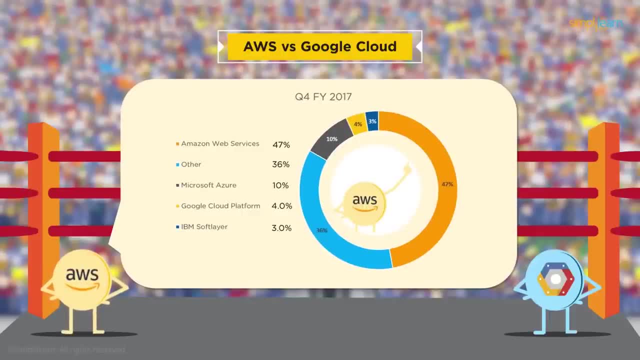 Amazon Web Services contributes 47% of the market share. Others like Rackspace or Verizon Cloud contribute 36%. Microsoft Azure contributes 10%, The Google Cloud Platform contributes 4% And IBM Software contributes 3%. 47% of the market share is contributed by AWS. 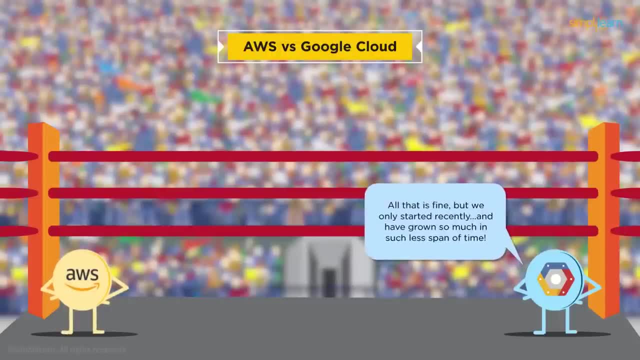 Do you need me to convince you anymore? Wait, wait, wait. All that is fine, But we only started a few years back and have already grown so much In such a less span of time. Haven't you heard the latest news? 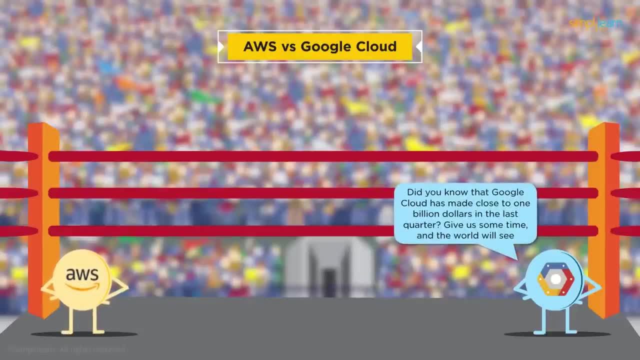 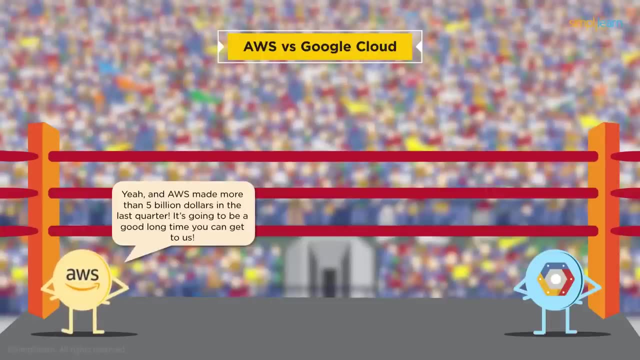 Our revenue is already a billion dollars per quarter. Wait for a few more years and the world shall see. And AWS makes 5.3 billion dollars per quarter. It's going to take a good long time before you can even get close to us. 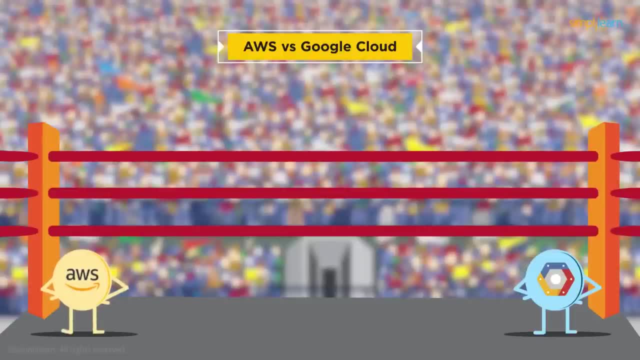 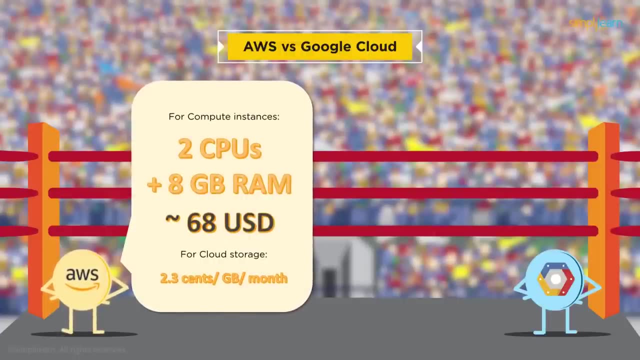 Yes, yes, We'll see. Now let's compare a few things. For starters, let's compare prices. For AWS, a compute instance of 2 CPUs and 8 GB RAM costs approximately 68 US dollars. Now, a compute instance is a virtual machine. 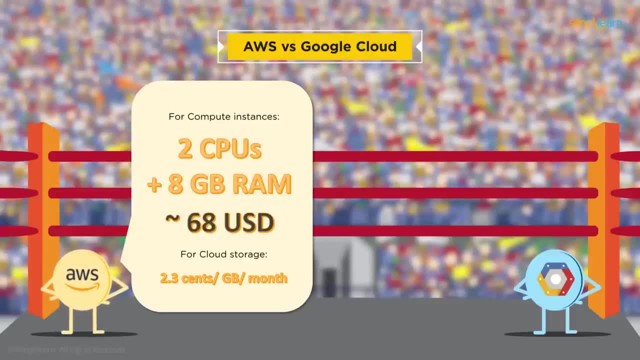 in which you can specify what operating system, RAM or storage you want to have For cloud storage. it costs 2.3 cents per GB per month with AWS. You really want to do that Because GCP wins this hands down. Let's take the same compute instance of 2 CPUs with 8 GB RAM. 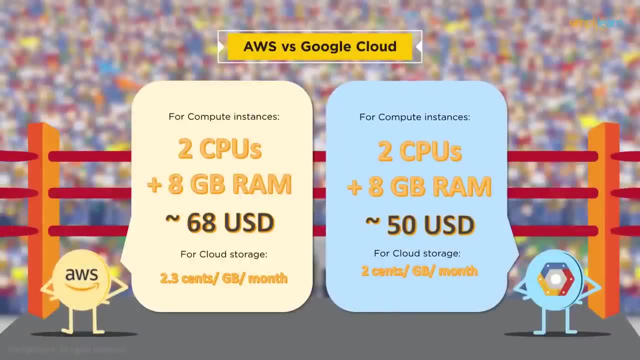 It will cost approximately 50 dollars per month with GCP And, as per my calculations, that's a 25% annual cost reduction when compared to AWS. Talking about cloud storage costs, it is only 2 cents per GB per month with GCP. 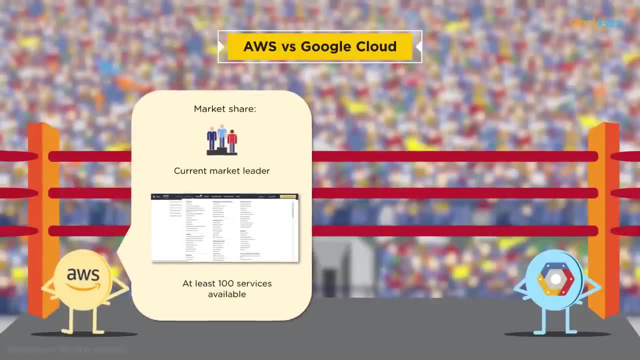 What else do you want me to say? Let's talk about market share and options. Now, AWS is the current market leader when it comes to cloud computing. Now, as you remember, we contribute at least 47% of the entire market share. 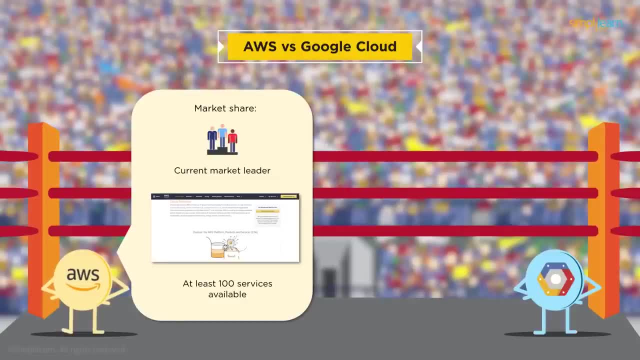 AWS also has at least 100 services available at the moment, which is a clear indication of how well AWS understands businesses and helps them grow. Yeah, that's true, But you should also know that GCP is steadily growing. We have over 60 services that are up and running. 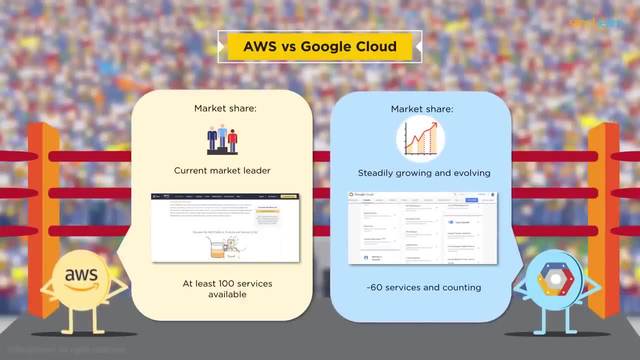 as you can see here, and a lot more to come. It's only a matter of time when we will have as many services as you do. Many companies have already started adopting GCP as their cloud service provider. Now let's talk about things you get for free. 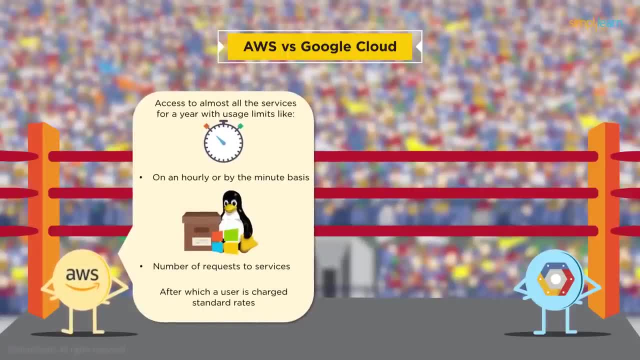 With AWS, you get access to almost all the services for an entire year with usage limits. Now, these limits include an hourly or by-the-minute basis. For example, with Amazon EC2, you get 750 hours per month. You also have limits on the number of requests to services. 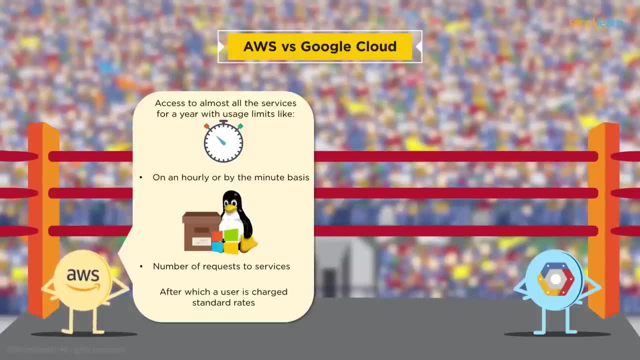 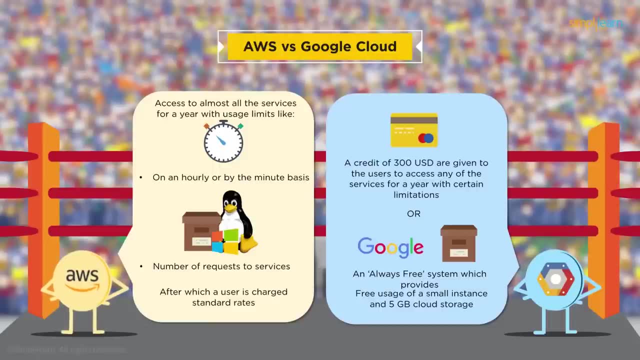 For example, with AWS Lambda, you have 1 million requests per month. Now, after these limits are crossed, you get charged standard rates. With GCP, you get access to all cloud platform products like Firebase, Google Maps API and so on. 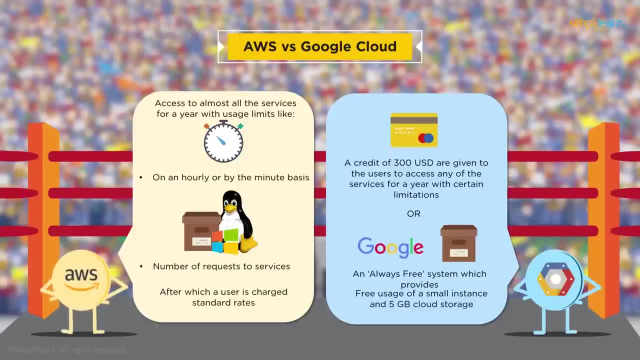 You also get $300 in credit to spend over a 12-month period on all the cloud platform products And, interestingly, after the free trial ends, you won't be charged unless you manually upgrade to a paid account. Now there is also the always free version. 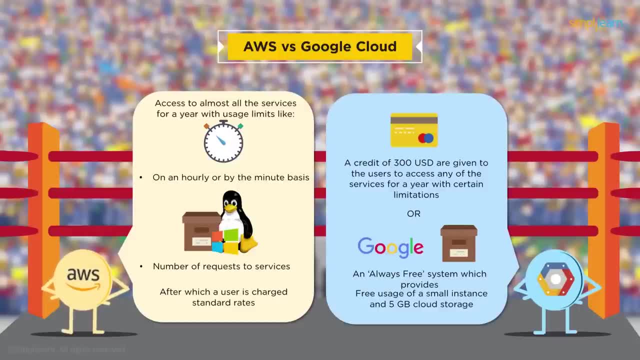 in which you will need an upgraded billing account. Here you get to use a small instance for free and 5GB of cloud storage. Any usage above this- always free usage limits will be automatically billed at standard rates. Now let's talk about how you can configure instances. 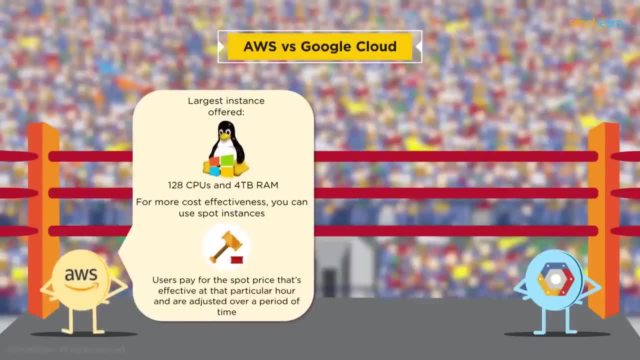 With AWS, the largest instance that's offered is of 128 CPUs and 14GB of RAM. Now, other than the on-demand method, like I mentioned before, you can also use spot instances. Now, these are for situations where your application is more fault tolerant. 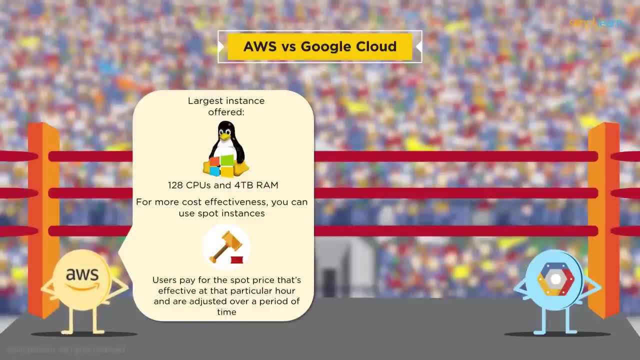 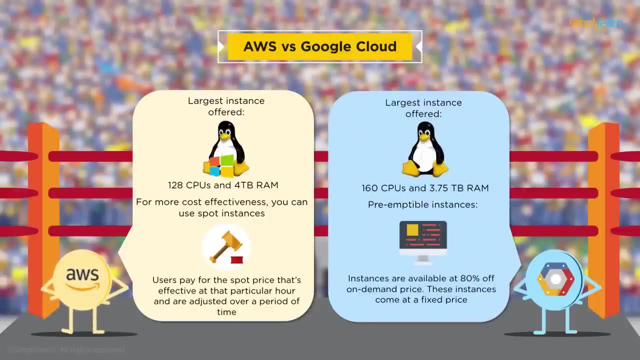 and can handle an interruption. Now you pay for the spot price which is effective at a particular hour. Now these spot prices do fluctuate, but are adjusted over a period of time. The largest instance offered with Google Cloud is 160 CPUs and 3.75 TBs RAM. 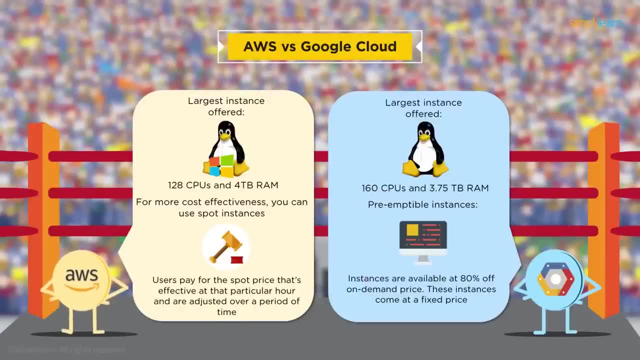 Like spot instances of AWS. Google Cloud offers short-lived compute instances suitable for bad jobs and fault tolerant workloads. They are called as preemptable instances, So these instances are available at 80% off on-demand price, Hence they reduce your compute engine costs significantly. 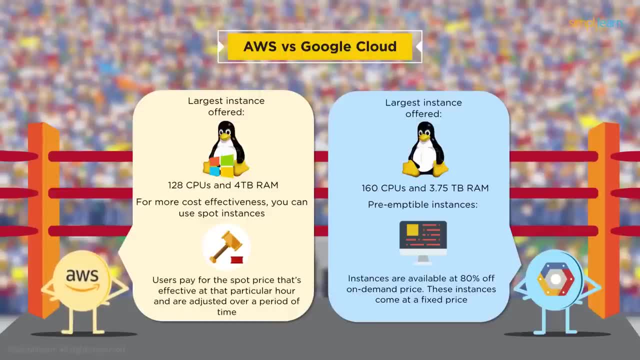 And, unlike AWS, these come at a fixed price. Google Cloud Platform is a lot more flexible when it comes to instance configuration. You simply choose your CPU and RAM combination. Of course, you can even create your own instance types this way. Before we wrap it up, let's compare on some other things as well. 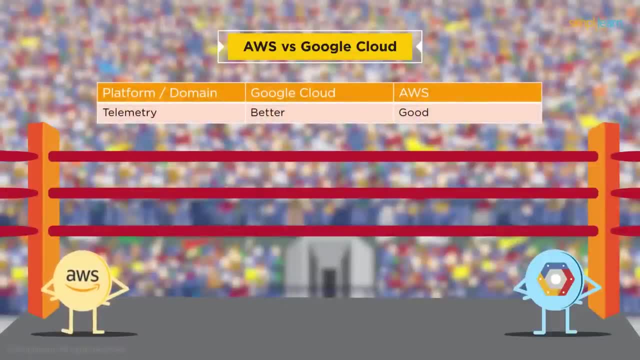 Telemetry. It's a process of automatically collecting periodic measurements from remote devices, For example GPS. GCP is obviously better because they have superior telemetry tools which help in analyzing services and providing more opportunities for improvement. When it comes to application support, AWS is obviously better. 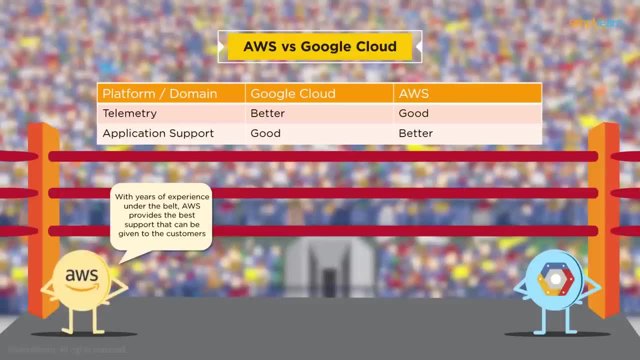 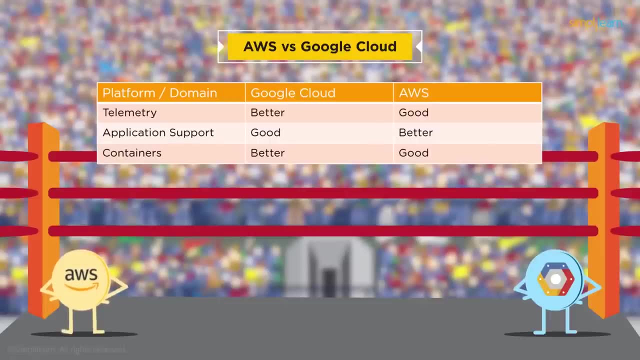 since they have years of experience under their belt. AWS provides the best support that can be given to the customers. Containers are better with GCP. A container is a virtual process running in user space. As Kubernetes was originally developed by Google, GCP has full native support for the tool. 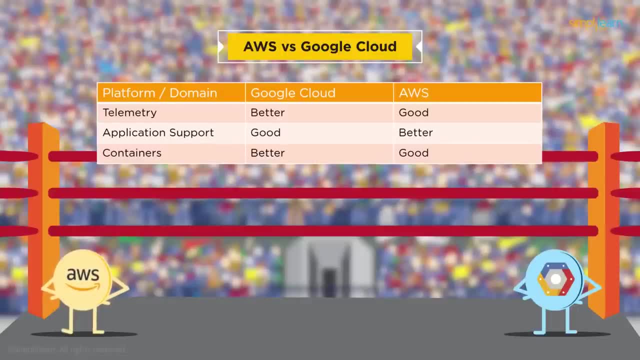 Other cloud services are just fine-tuning and providing a way to provide Kubernetes as a service. Also, the containers help with abstracting applications from the environment they originally run in. The applications can be deployed easily, regardless of their environment. When it comes to geographies, AWS is better, since they have a head start of a few years. 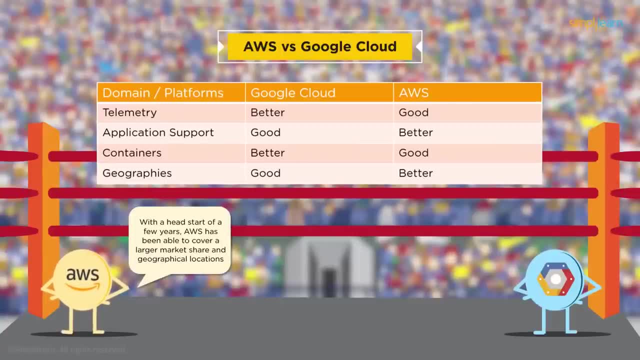 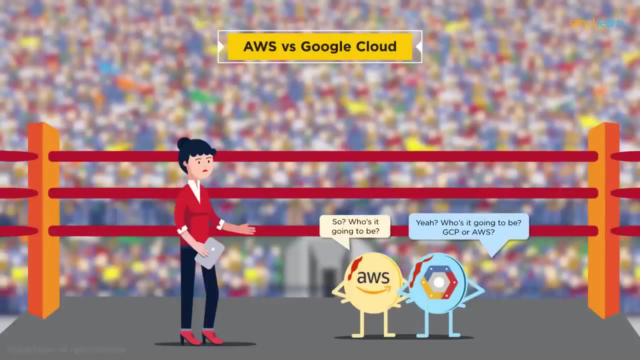 AWS, in this span of time, has been able to cover a larger market share and geographical locations. Now it's time for the big decision. So who's it going to be? Yeah, who is it going to be GCP or AWS? 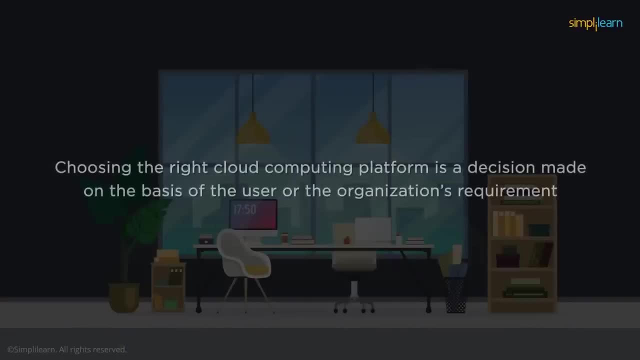 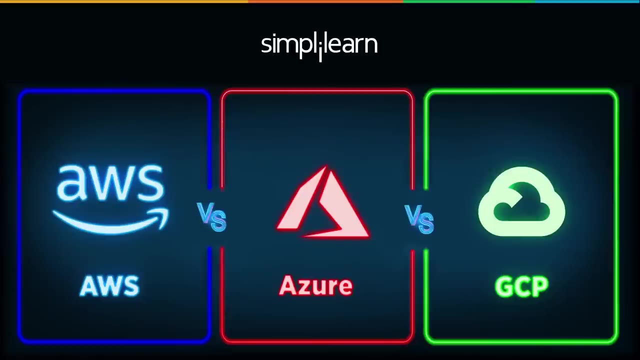 I think I'm going to go for. Choosing the right cloud computing platform is a decision that's made on the basis of the user or the organization's requirement. AWS, Azure and GCP are three of the world's largest cloud service providers, But how are they different from each other? Let's find out. 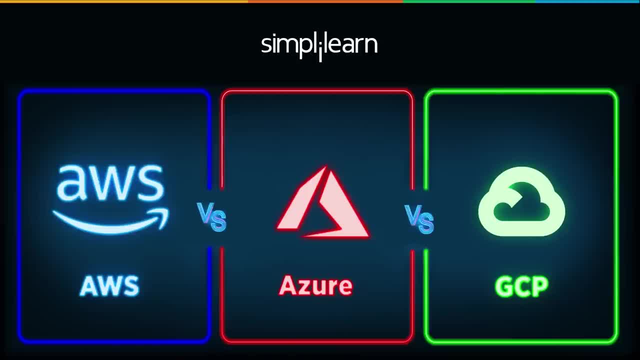 Hey guys, I'm Rahul and I'll be representing Amazon Web Services. I'm Chinmai and I'll be representing Microsoft Azure, And I'm Shruti and I'll be representing Google Cloud Platform. So welcome to this video on AWS vs Azure vs GCP. 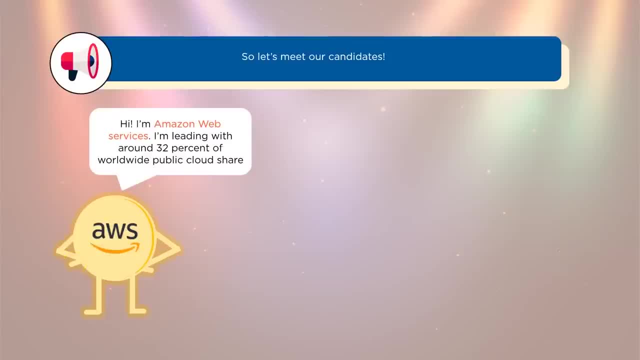 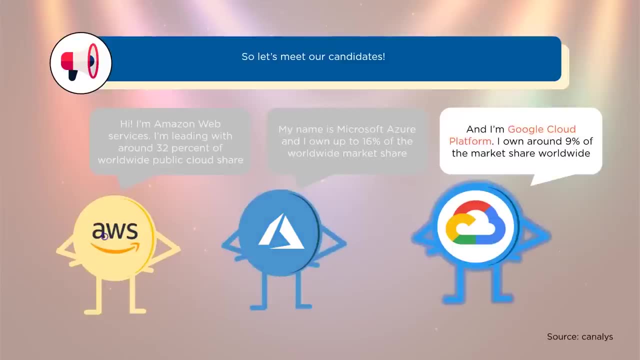 Talking about market share, Amazon Web Services leads with around 32% of the worldwide public cloud share. Azure owns up to 16% of the worldwide market share And GCP owns around 9% of the world's market share. Let's talk about each of these service providers in detail. 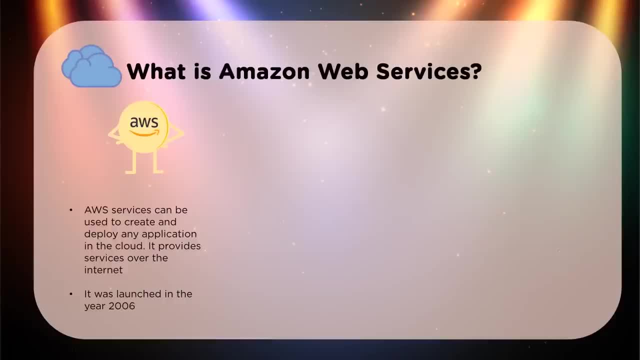 AWS provides services that enable users to create and deploy applications over the cloud. These services are accessible via the internet. AWS, being the oldest of the lot, was launched in the year 2006.. Azure launched in 2010.. GCP is a computing platform that offers a wide range of services to build, manage and deploy applications on the network using tools and frameworks. 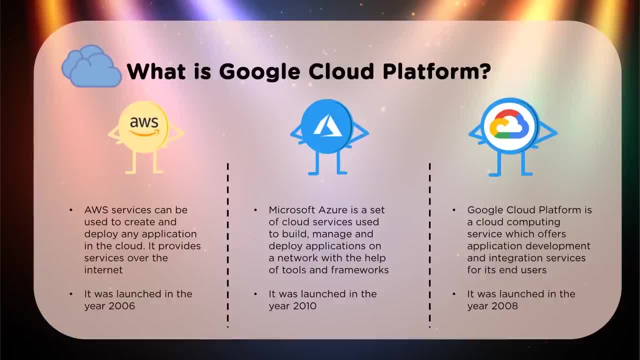 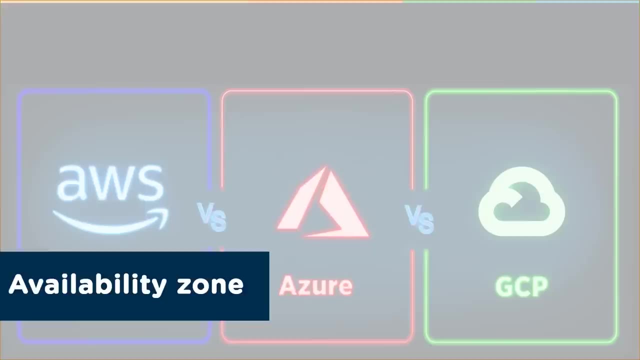 Launched in the year 2008,. GCP offers application development and integration services for its end users. In addition to cloud management, it also offers services for big data, machine learning and IoT. Now let's talk about availability zones. These are isolated locations within data center regions from which public cloud services originate and operate. 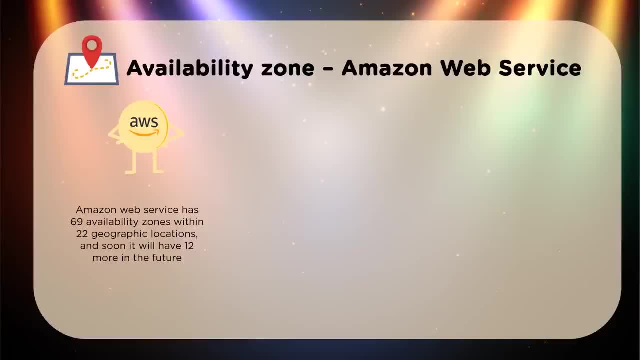 Talking about AWS, they have 69 availability zones within 22 geographical regions. This includes regions in the United States, South America, Europe and Asia Pacific. They are also predicted to have 12 more editions in the future. Azure, available in 140 countries, has over 54 regions worldwide grouped into 6 geographies. 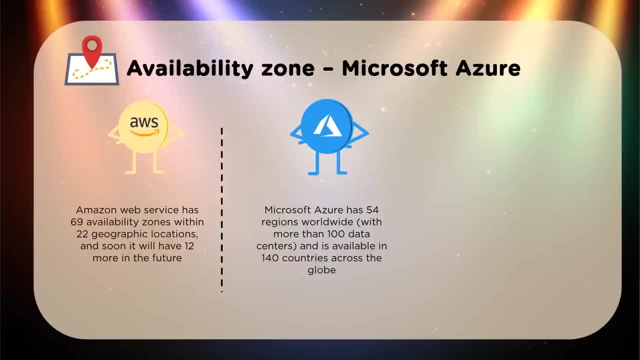 These geographical locations have more than 100 data centers. GCP is available in 200 plus countries across the world. As of today, GCP is present in 61 zones and 20 regions, With Osaka and Zurich being the newly added regions. 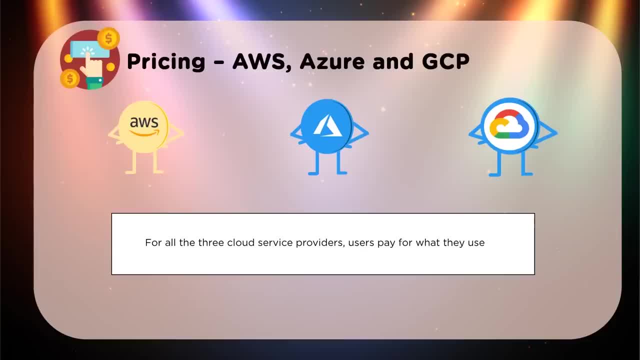 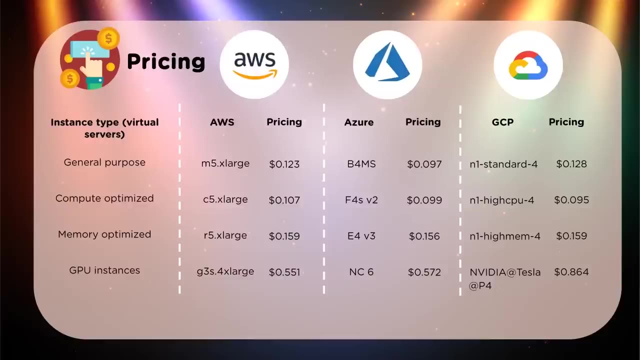 Now let's talk about pricing. These services follow the pay-as-you-go approach: You pay only for the individual services you need for as long as you use them, without requiring long-term contracts or complex licensing. Now, on screen, you can see the pricing for each of these cloud service providers with respect to various instances, like general purpose compute, optimized memory optimized and GPU. 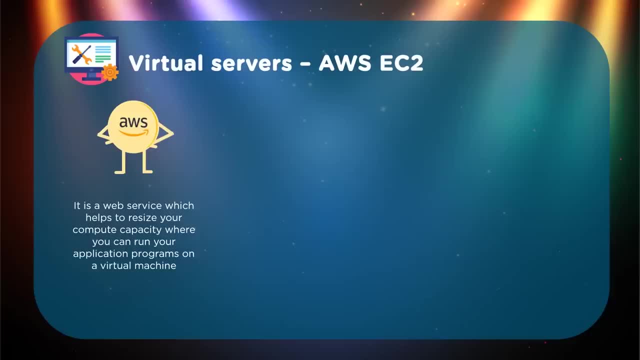 Now let's talk about the compute services offered. First off, we have virtual servers For AWS. we have EC2.. It is a web service which eliminates the need to invest in hardware so that you can develop and deploy applications in a faster manner. 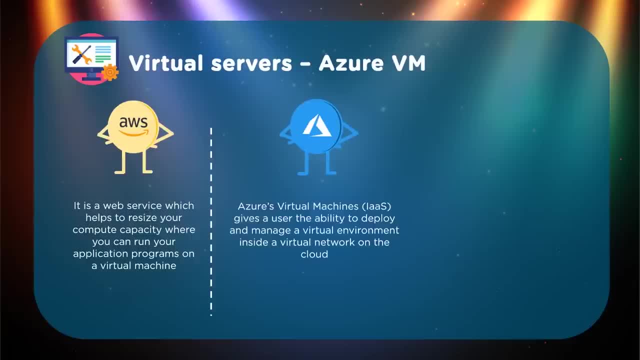 It provides virtual machines in which you can run your applications. Azure's virtual machines is one of the several types of computing resources that Azure offers. Azure gives the user the flexibility to deploy and manage a virtual environment inside a virtual network. GCP's VM service enables users to build, deploy and manage virtual machines. 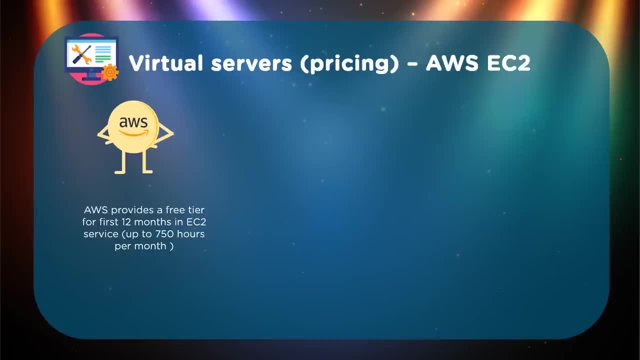 To run workloads on the cloud. Now let's talk about the pricing of each of these services. AWS EC2 is free to try. It is packaged as part of AWS's free tier that lasts for 12 months and provides 750 hours per month of both Linux and Windows virtual machines. 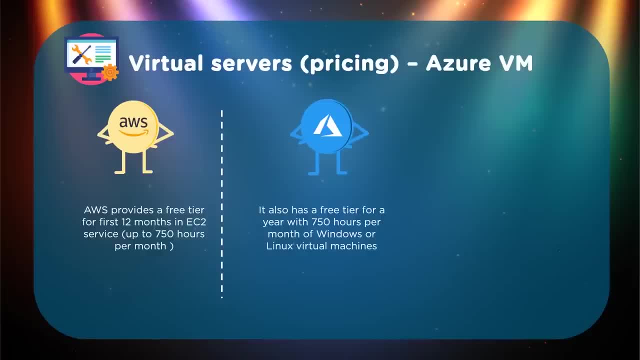 Azure virtual machine service is a part of the free tier that offers this service for about 750 hours per month for a year. The user gets access to Windows and Linux virtual machines. GCP's VM service is a part of a free tier that includes micro-instance per month. 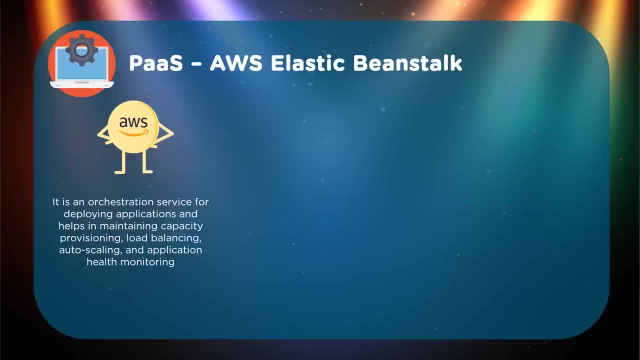 For up to 12 months. Now let's talk about Platform as a Service, or PaaS services. For AWS, Elastic Beanstalk is an easy to use service for deploying and scaling web applications and services developed with Java, NET, NodeJS, Python and much more. 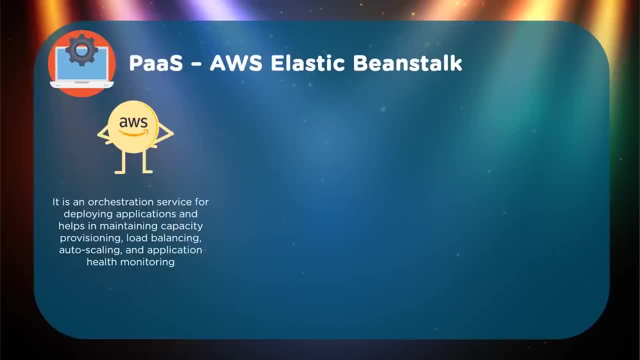 It is used for maintaining capacity provisioning, load balancing, auto scaling and application health monitoring. The PaaS backbone utilizes virtualization techniques. where the virtual machine is independent of the actual hardware that hosts it, The user can write application code without worrying about the underlying hardware. 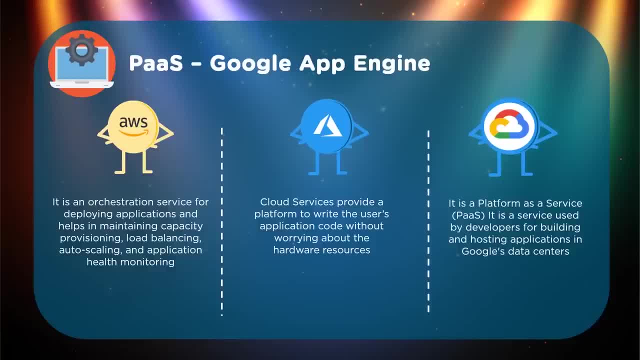 Google App Engine is a cloud computing platform as a service which is used by developers for hosting and building apps in Google data centers. The App Engine requires the apps to be written in Java or Python and store data in Google Bigtable and use the Google Query language for this. 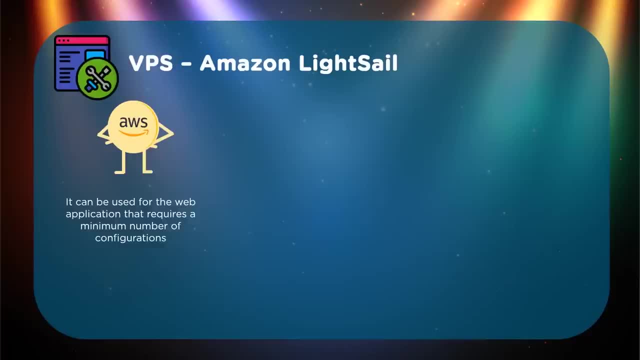 Next, let's talk about Virtual Private Server Services. AWS provides LightSail. It provides everything you need to build an application or a website, along with the cost-effective monthly plan and minimum number of configurations. In simple words, VM Image is a more comprehensive image for Microsoft Azure Virtual Machines. 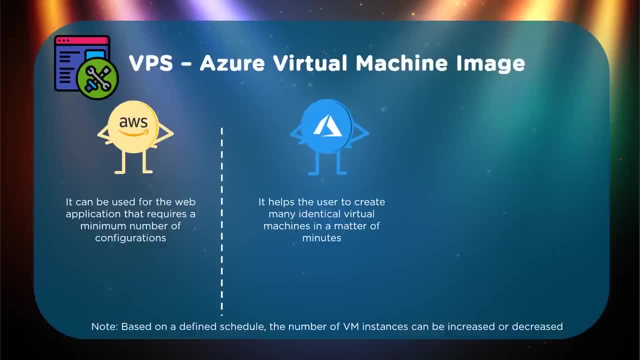 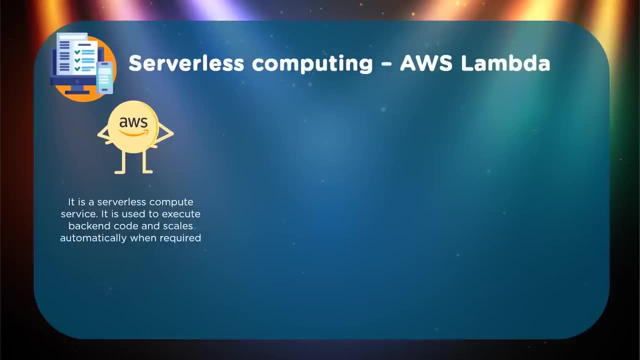 It helps the user create many identical virtual machines in a matter of minutes. Unfortunately, GCP does not offer any similar service. Next up, we have Serverless Computing Services. AWS has Lambda. It is a serverless compute service that lets you run your code without facilitating and managing servers. 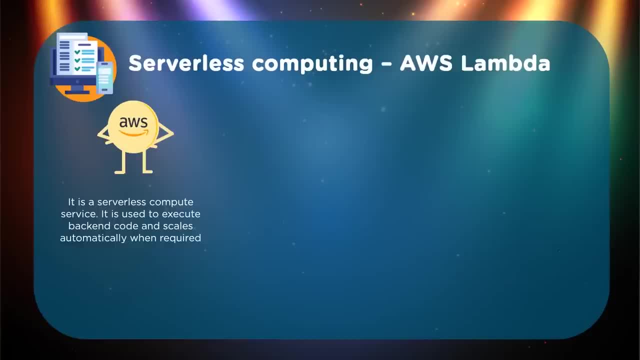 You only pay for the compute time you use. It is used to execute backend code and scales automatically when required. Azure Functions is a serverless compute service that lets you run event-triggered code without having to explicitly provision or manage infrastructure. This allows the users to build applications using serverless, simple functions with the programming language of their choice. 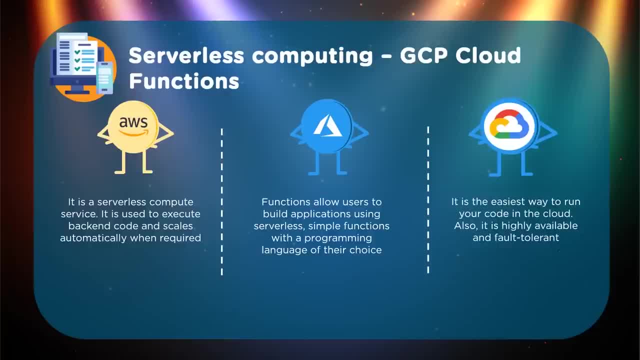 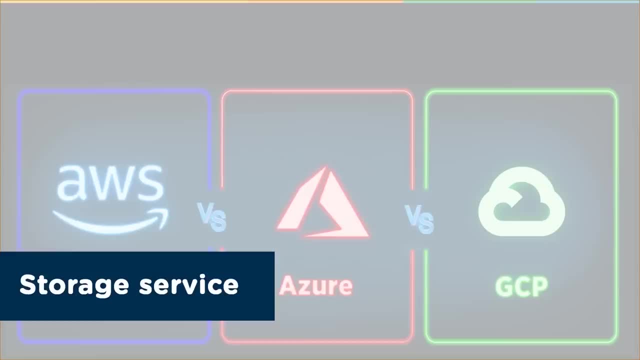 GCP Cloud Functions make it easy for developers to run and scale code in the cloud and build event-driven, serverless applications. It is highly available and fault-tolerant. Let's talk about storage services offered by each of these service providers. First off, we have Object Storage. 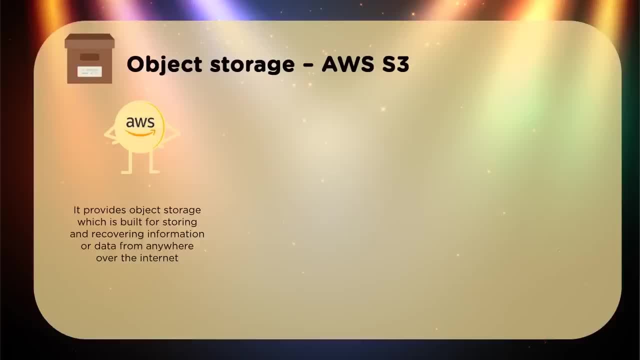 AWS provides S3. It is an object storage that provides industry-standard scalability, data availability and performance. It is extremely durable and can be used for storing as well as recovering information or data from anywhere over the internet. Blob Storage is an Azure feature that lets developers store unstructured data in Microsoft's cloud platform. 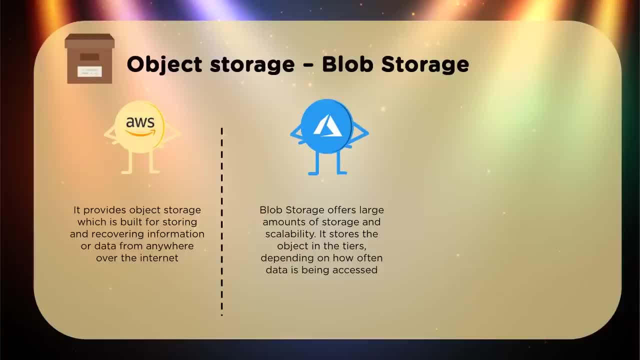 Along with storage, it also offers scalability. It stores the data in the form of tiers, depending on how often data is being accessed. Google Cloud Storage is an online storage web service for storing and accessing data on Google Cloud Platform infrastructure. Unlike the Google Drive, Google Cloud Storage is more suitable for enterprises. 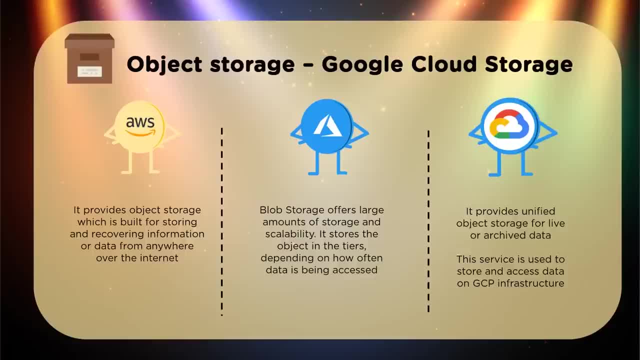 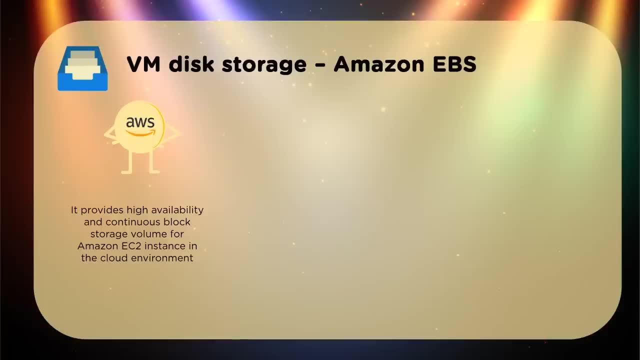 It also stores objects that are organized into buckets. Amazon provides EBS or Elastic Block Store. It provides high-performance block storage and is used along with EC2 instances for workloads that are transaction or throughput intensive. Azure Managed Disk is a virtual disk. 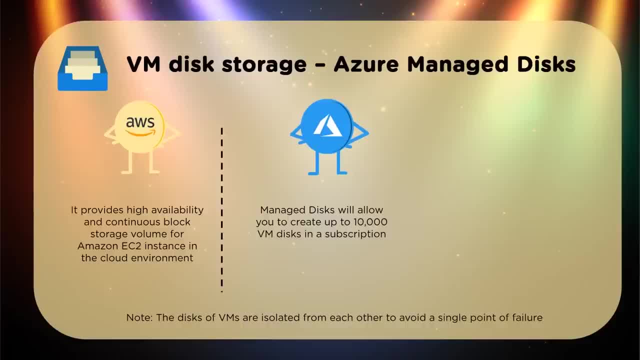 You can think of it like a physical disk in an on-premises server, but virtualized. These managed disks allow the users to create up to 10,000 VM disks in a single subscription. Persistent Storage is a data storage device that retains data after power to the device is shut off. 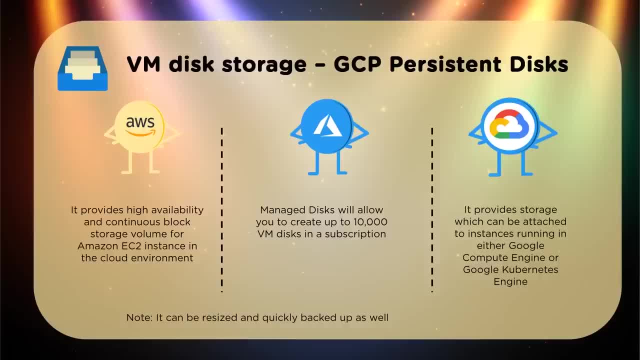 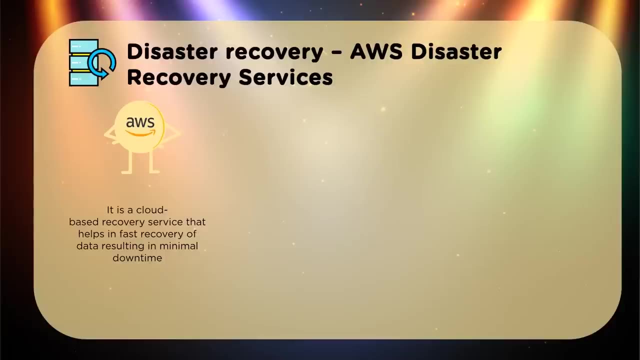 Google Persistent Disk is durable and high-performance. block storage for GCP Persistent Disk provides storage which can be attached to instances running in either Google Compute Engine or Kubernetes Engine. Next up, we have Disaster Recovery Services. AWS provides a cloud-based recovery service that ensures that your IT infrastructure and data are recovered. 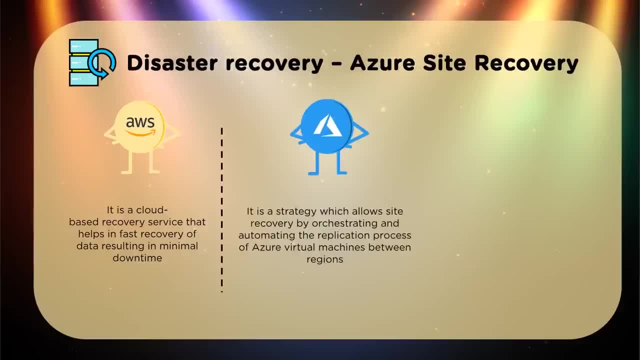 while minimizing the amount of downtime that could be experienced. Site Recovery helps ensure business continuity by keeping business apps and workloads running during outages. It allows recovery by orchestrating and automating the replication process of Azure virtual machines between regions. Unfortunately, GCP has no disaster recovery service. 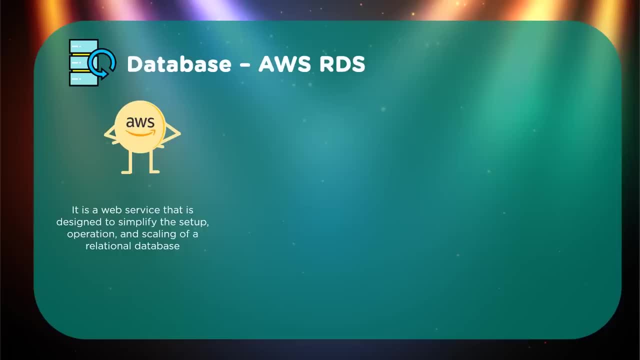 Next, let's talk about Database Services. First off, for AWS, we have RDS, or Relational Database Service. It is a web service that's cost-effective and automates administration tasks. Basically, it simplifies the setup, operation and scaling of a relational database. 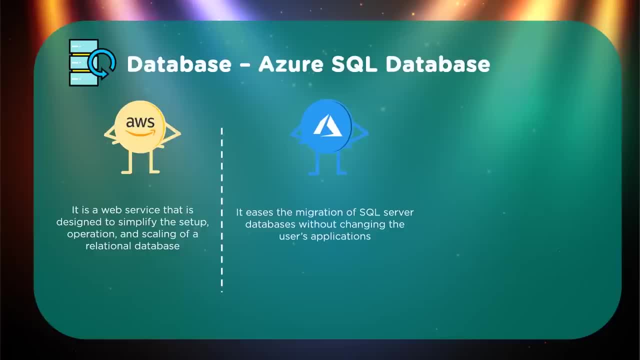 Microsoft Azure SQL Database is a software-as-a-service platform that includes built-in intelligence that learns app patterns and adapts to maximize performance, reliability and data protection. It also eases the migration of SQL Server databases without changing the user's applications. Cloud SQL is a fully managed database service which is easy to set up, maintain and administer. 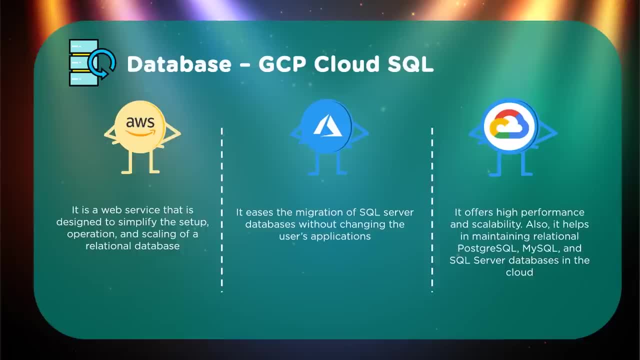 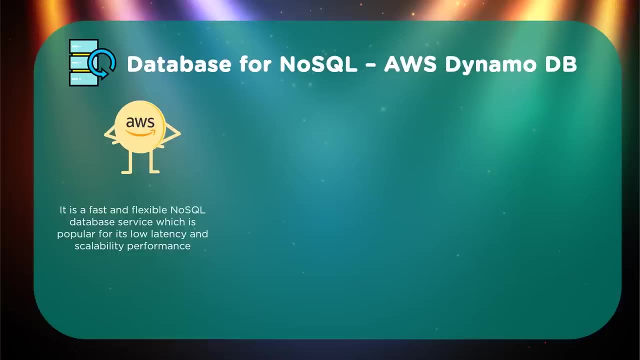 relational PostgreSQL, MySQL and SQL Server databases in the cloud, Hosted on GCP Cloud. SQL provides a database infrastructure for applications running anywhere. Next, we have NoSQL Database Services. AWS provides DynamoDB, which is a managed, durable database that provides security, backup and restore. 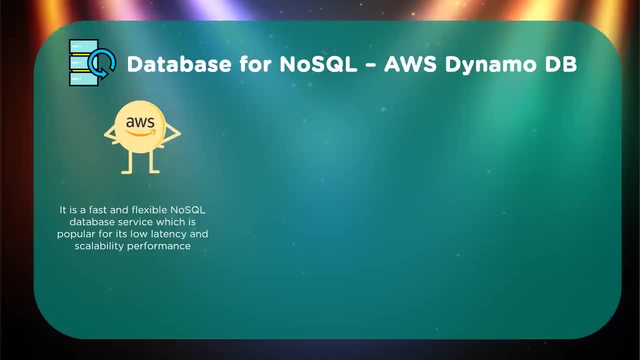 and in-memory caching for applications. It is well known for its low latency and scalable performance. Azure Cosmos DB is Microsoft's globally distributed multi-model database service. It natively supports NoSQL created for low latency and scalable applications. GCP Cloud Datastore is a NoSQL database service offered by Google on the GCP. 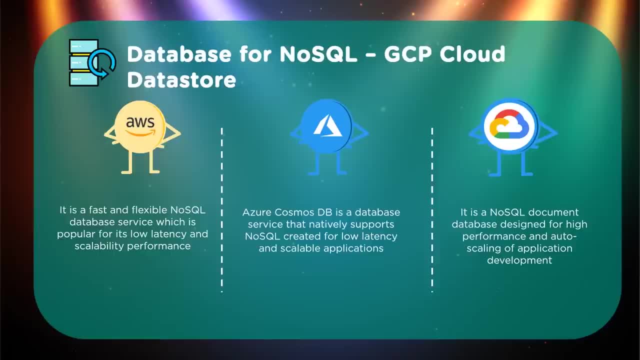 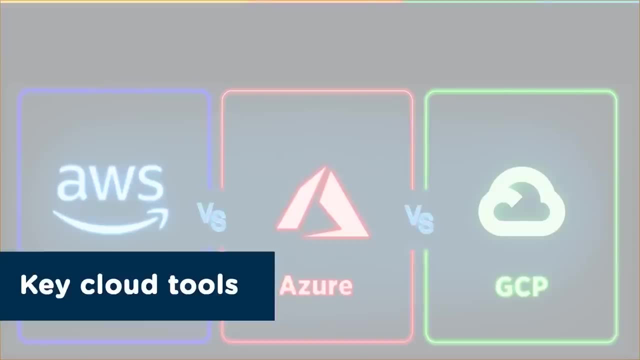 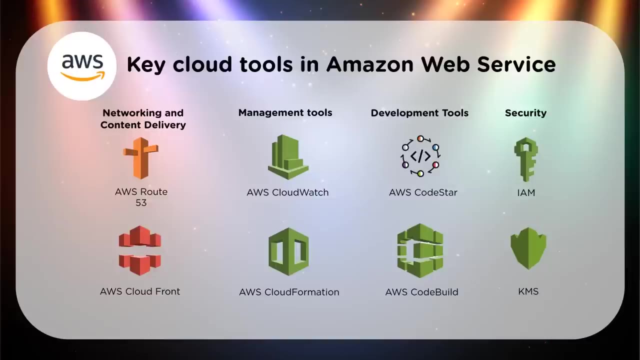 It handles replication and scales automatically to your application's load. With Cloud Datastore's interface, data can easily be accessed by any deployment target. Now let's talk about the key cloud tools for each of these service providers. For AWS in Networking and Content Delivery, we have AWS Route 53 and AWS CloudFront. 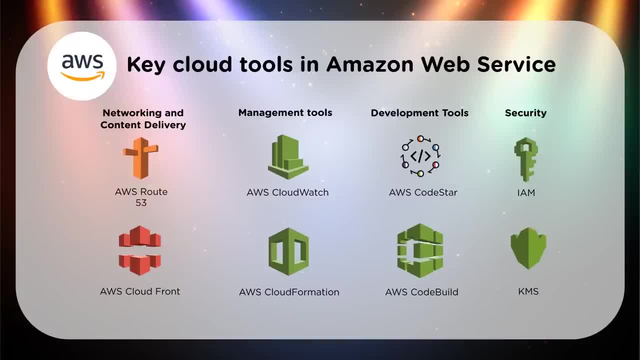 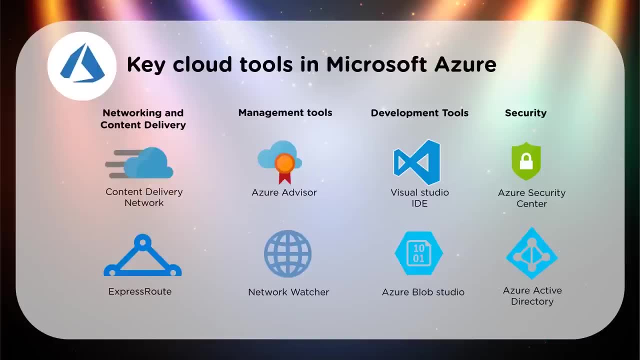 For Management, we have AWS CloudWatch and AWS CloudFormation. For Development, we have AWS CodeStart and AWS CodeBuild. For Security, we have IAM and Key Management Service. For Microsoft Azure. Networking and Content Delivery: we have Content Delivery Network and ExpressRoute. 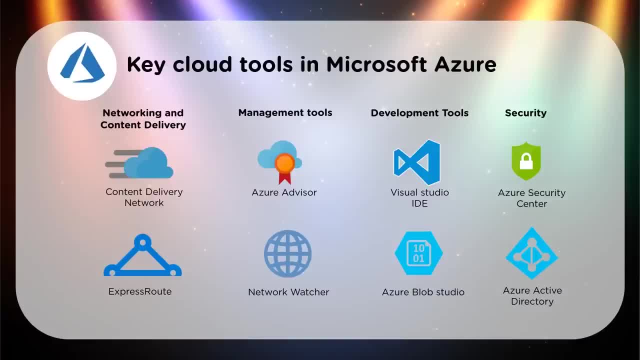 For Management Tools, we have Azure Advisor and Network Watcher. For Development Tools for Management, we have Azure Advisor and Network Watcher. For Development, we have Visual Studio IDE and Azure Blob Studio. For Security, we have Azure Security Center and Azure Active Directory. 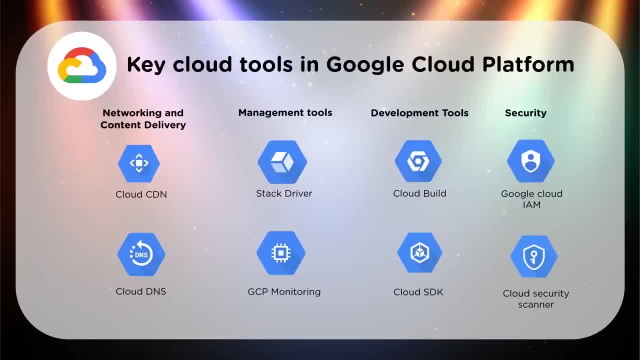 For GCP, we have the following tools: For Networking and Content Delivery, we have Cloud CDN and Cloud DNS. For Management, we have Stackdriver and GCP Monitoring. For Development, we have Cloud Build and Cloud SDK. And finally, for Security, we have Cloud Security. 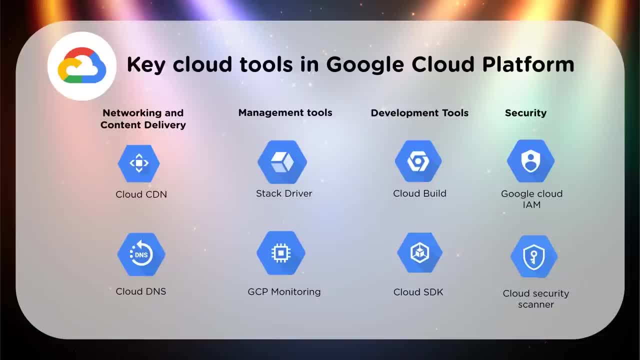 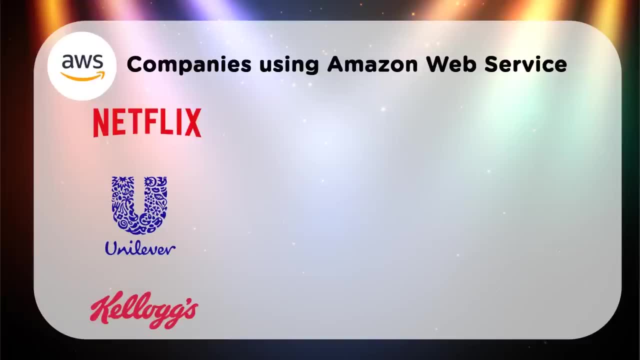 Finally, for Security, we have Google Cloud, IAM and Google and Cloud Security Scanner. Now let's talk about the companies using these cloud providers. For AWS, we have Netflix, Unilever, Kellogg's, NASA, Nokia and Adobe. 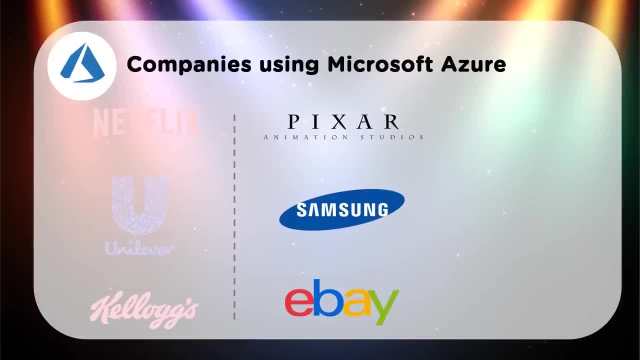 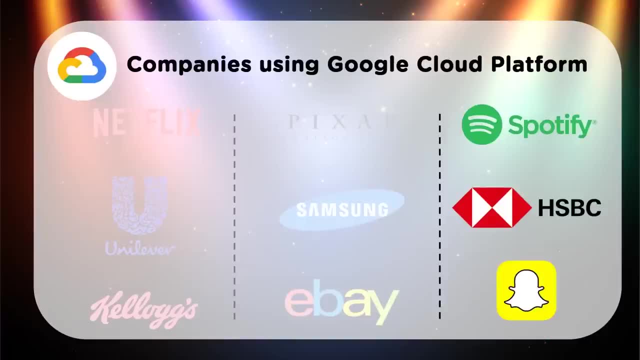 Pixar, Samsung, eBay, Fujitsu, EMC and BMW, among others, use Microsoft Azure. So, as seen on your screens, the companies that use GCP are Spotify, HSBC, Snapchat, Twitter, PayPal and 20th Century Fox. Let's talk about the advantages of each of these services. 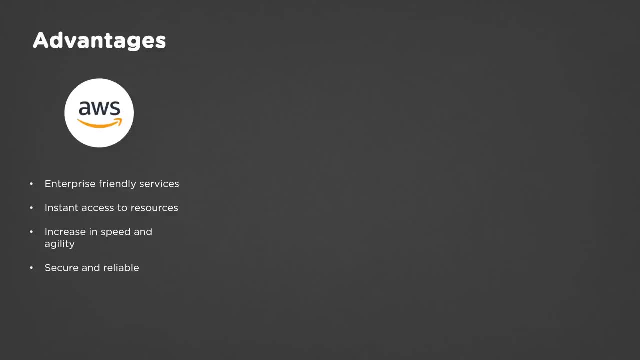 Amazon provides enterprise-friendly services. You can leverage Amazon's 15 years of experience delivering large-scale global infrastructure, And it still continues to hone and innovate its infrastructure management skills and capabilities. Secondly, it provides instant access to resources. AWS is designed to allow application providers, ISVs and vendors to quickly and securely host your applications. 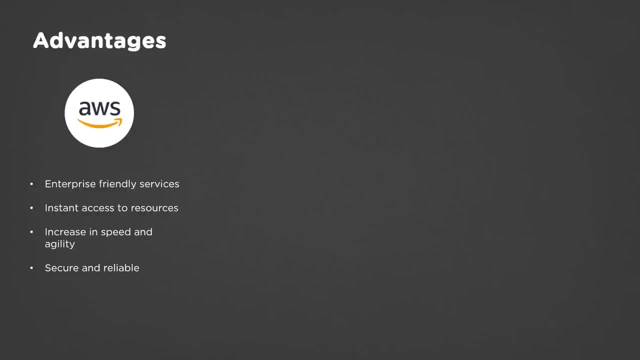 whether an existing application or a new SaaS-based application, Speed and Agility AWS provides you access to its services within minutes. All you need to select is what you require and you can proceed. You can access each of these applications anytime you need them. 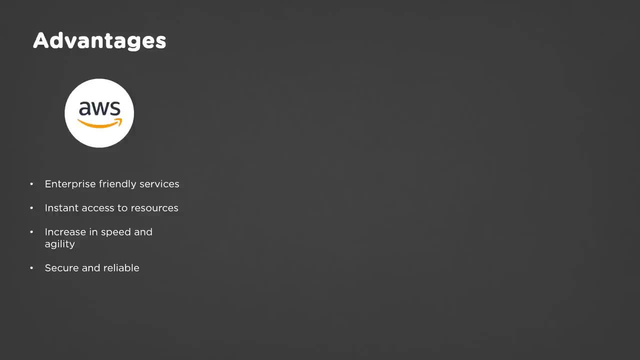 And finally, it's secure and reliable. Amazon enables you to innovate and scale your application in a secure environment. It secures and hardens your infrastructure. More importantly, it provides security at a cheaper cost than on-premise environments. Now talking about some of the advantages of Azure. 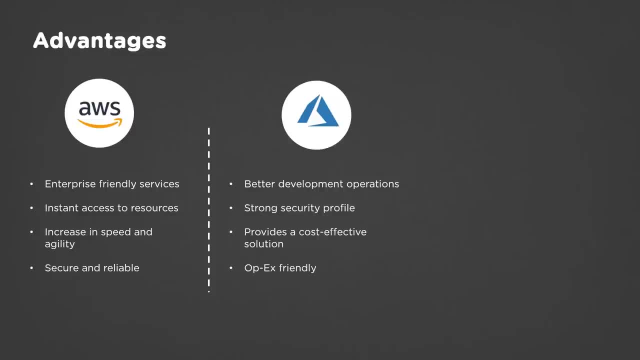 Microsoft Azure offers better development operations. It also provides strong security profile. Azure has a strong focus on security, Following the standard security model of detect, assess, diagnose, stabilize and close. Azure also provides a cost-effective solution. The cloud environment allows businesses to launch both customer applications and internal apps in the cloud. 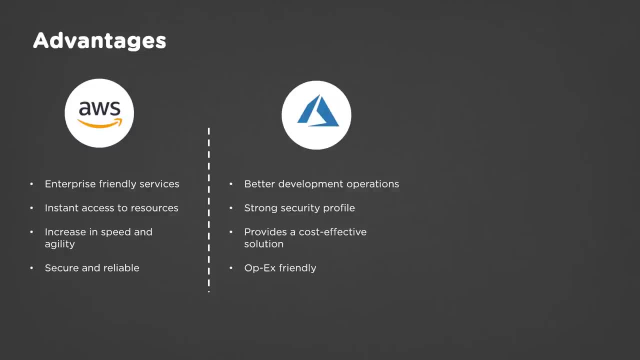 which saves on IT infrastructure costs. Hence it's OPEX friendly. Let's now look at the advantages of GCP. Google builds in minute-level increments, so you only pay for the compute time you use. They also provide discounted prices for long-running workloads. 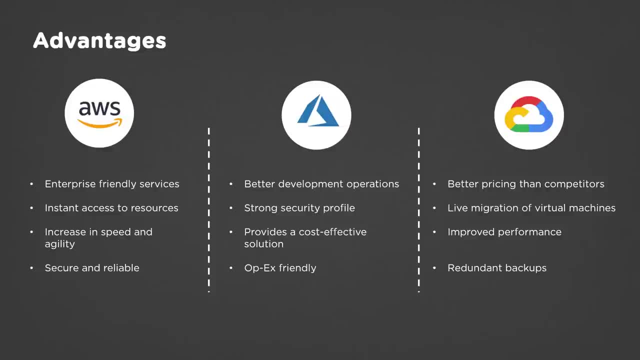 For example, in Google, you use the VM for a month and get a discount. GCP also provides live migration of virtual machines. Live migration is the process of moving a running VM from one physical server to another without disrupting its availability to the users. 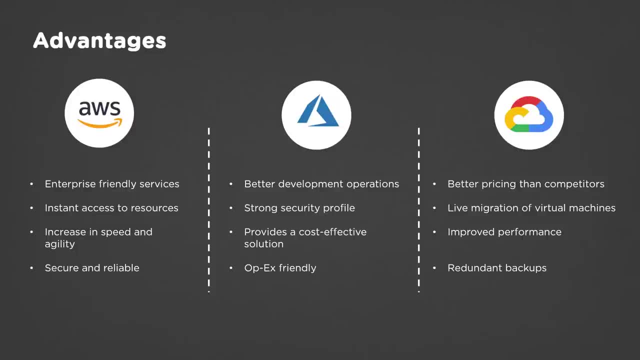 This is a very important differentiator for Google Cloud compared to other cloud providers. GCP provides automatic scalability. This allows a site's container scale to as many CPUs as needed. Google Cloud Storage is designed for 99.9% durability. It creates server backup and stores them in an user-configured location. 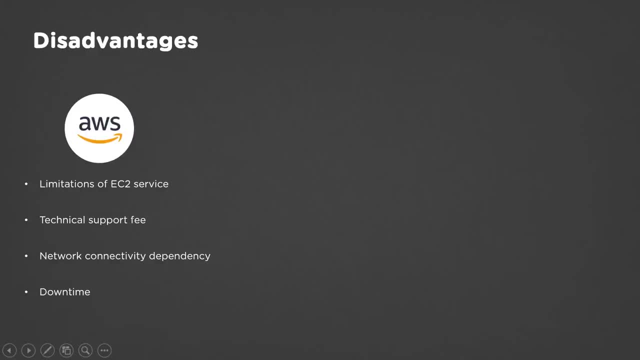 Let's talk about the disadvantages of each of these services. For AWS, there's a limitation of the EC2 service. AWS provides limitations on resources that vary from region to region. There may be a limit to the number of instances that can be created. 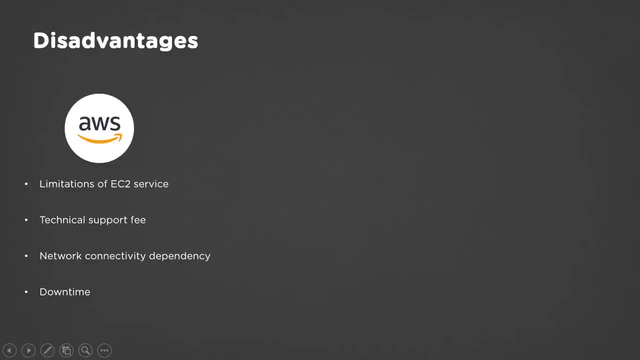 However, you can request for these limits to be increased. Secondly, they have a technical support fee. AWS charges you for immediate support and you can opt for any of these packages: Developer, which costs $29 per month. Business, which costs more than $100. 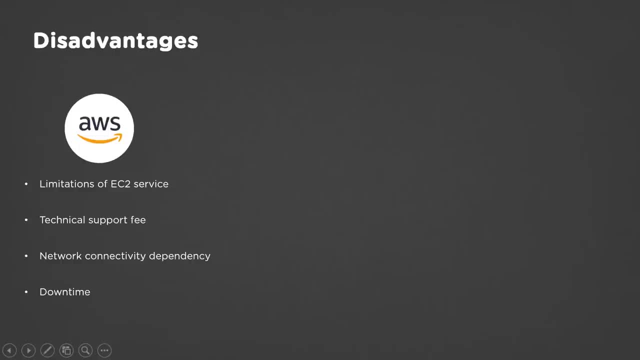 And Enterprise that costs more than $15,000.. It has certain network connectivity issues. It also has general issues when you move to the cloud, like downtime, limited control, backup protection and so on. However, most of these are temporary issues and can be handled over time. 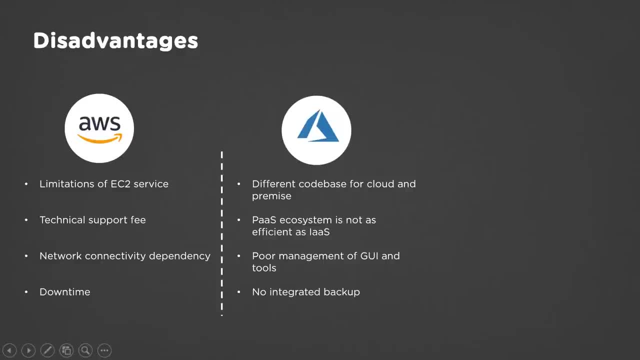 Talking about some of the disadvantages of Microsoft Azure. Codebase is different when working offline and it requires modification when working on the cloud. PaaS ecosystem is not as efficient as IaaS. Azure Management Console is frustrating to work with. It is slow to respond in a batch. 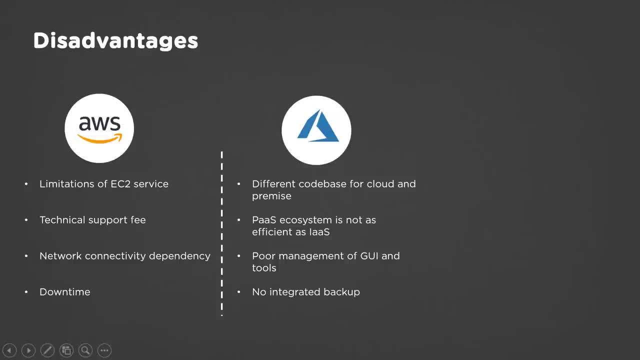 It requires an update and requires far too many clicks to achieve simple tasks. Azure Backup is intended for backing up and restoring data located on your on-premises servers to the cloud. That's a great feature, but it's not really useful for doing bare-metal restores of servers in a remote data center. 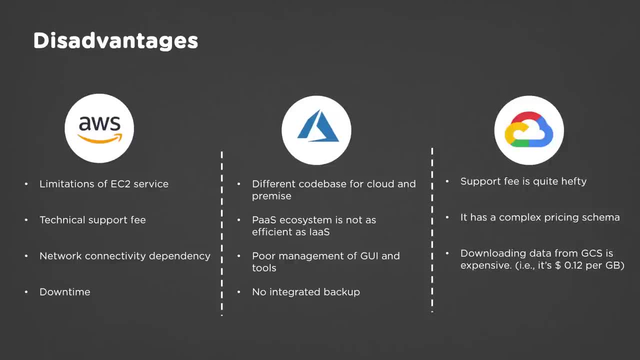 Let's now look into the disadvantages of GCP. So when it comes to cloud providers, the support fee is very minimal, But in the case of GCP, it is quite costly. It is around $150 per month for the most basic service. 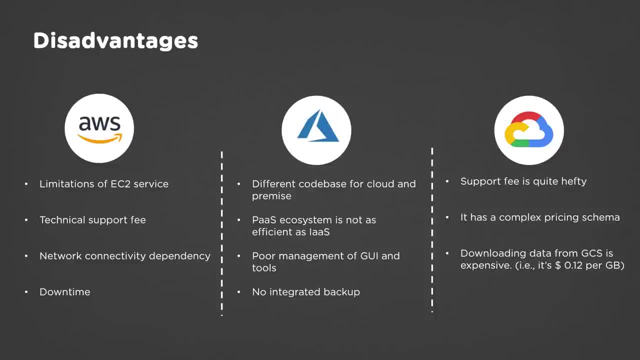 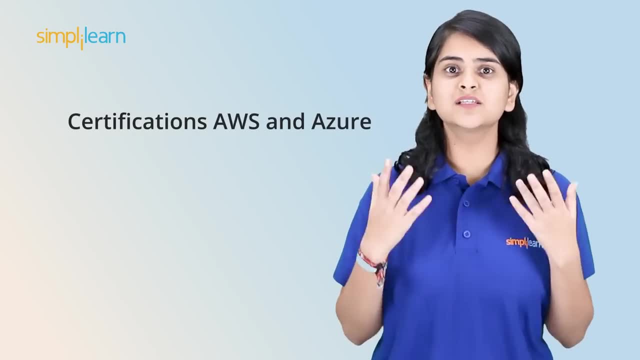 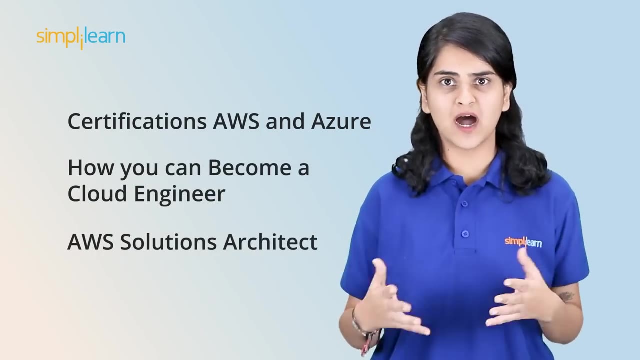 Similar to AWS S3, GCP has a complex pricing schema. Also, it is not very budget-friendly when it comes to downloading data from Google Cloud Storage. Now let us see the certifications that are available for AWS and Azure and how you can become a cloud engineer and an AWS solutions architect. 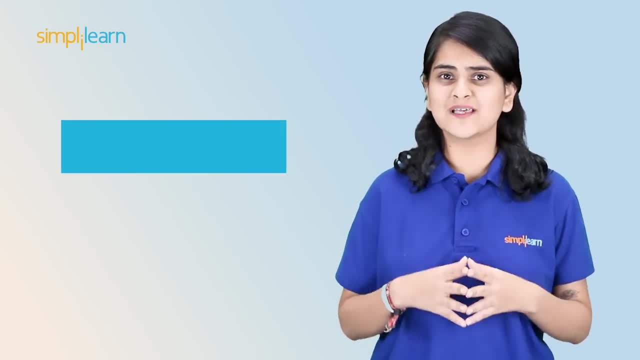 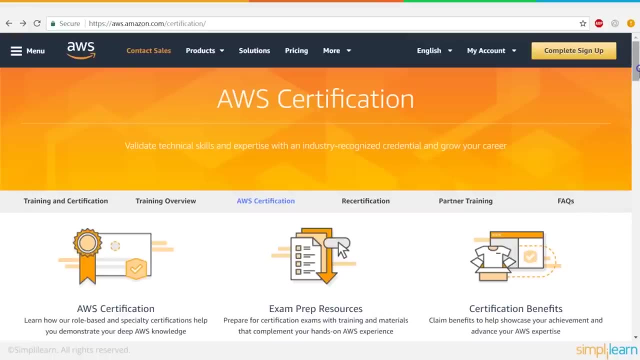 Rahul will talk about these topics. We'll also cover some important AWS and Azure interview questions. Right now we're in the AWS certification website, whose link will be in the description, And now we're going to talk about the types of AWS certification. 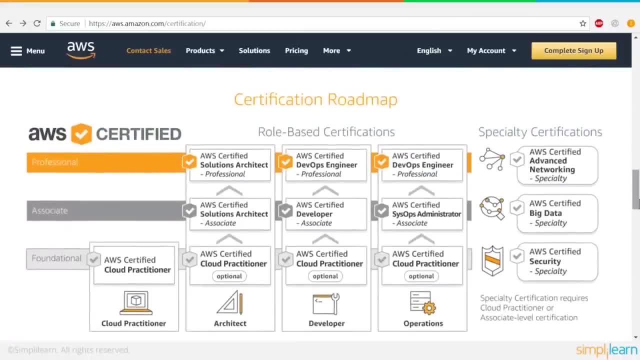 As you can see here, there are three levels of AWS certification. There's the foundational level, associate level and professional level certification. Now, the foundational level certification only requires you to have a basic understanding of how the AWS cloud works. The AWS Certified Cloud Practitioner is optional for the architect path, developer path and operations path. 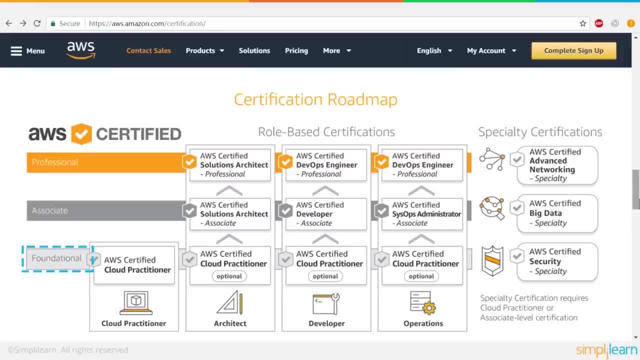 It is mandatory for the specialty certifications like the advanced networking, big data and security certifications. Now the associate level certifications are mid-level certifications for a technical role. Now a professional certification is the highest level of certification that you can have for a technical role. 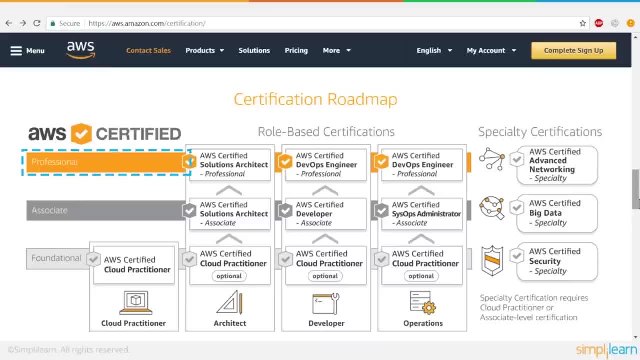 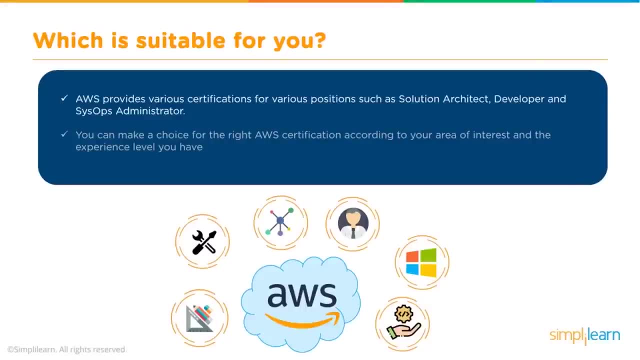 Now you have the solutions architect for the architect path and the DevOps engineer certification for both the developer and operations path. So how do you decide which of these certifications is suitable for you? So you've seen here that AWS provides various certifications for a number of job roles. 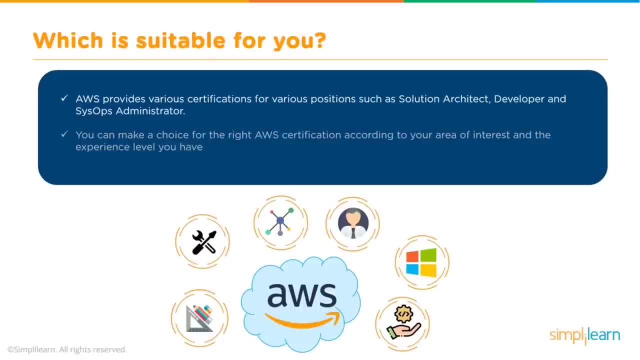 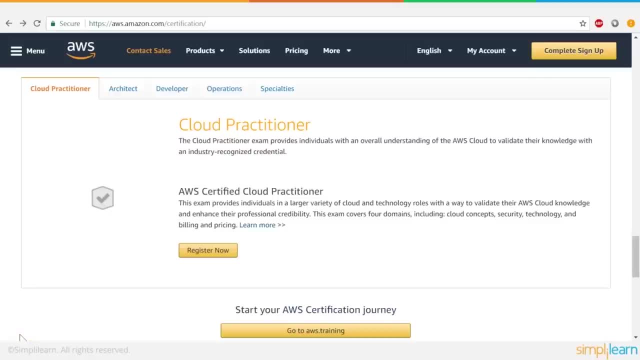 access ops administrator, solution architect, developer. So you need to make the right choice, taking into consideration the areas of your interest and the experience level that you have. Now we're going to talk about each of these certifications in detail. 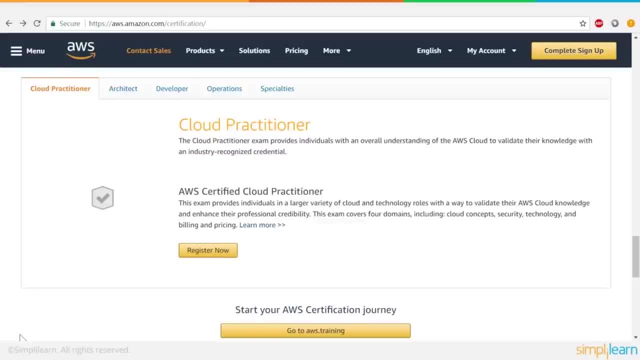 So first let's talk about the AWS Certified Cloud Practitioner. Now we all understand that AWS is a widely recognized product in the market, So this certification helps you validate how well you know the AWS cloud. So this is just the basic understanding. 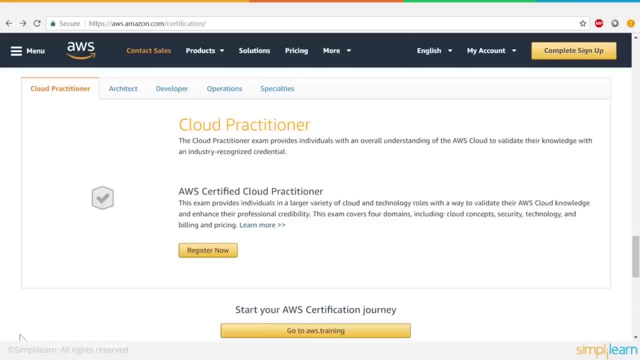 Now it is optional for the developer path and the operations path. I would suggest it's a good idea to start here, because it forms a solid bedrock on all the other things that you're going to learn soon. Now, more importantly, it does not require any technical knowledge of other roles, such as development, architecture, administration. 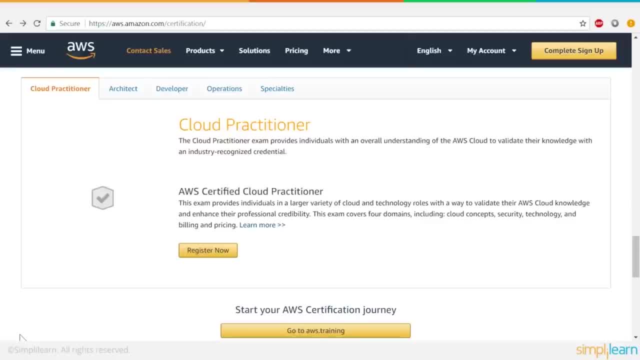 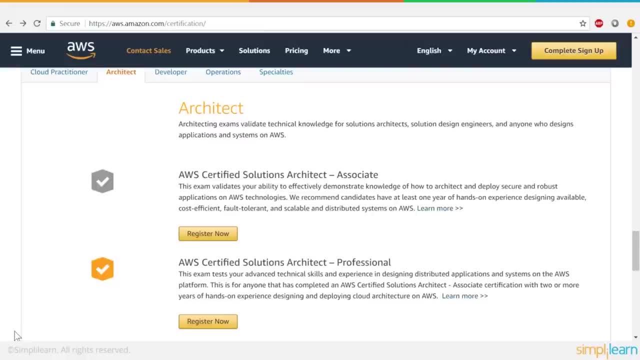 and so on. So it's a great place to start for newcomers. Now you have the architect role certifications. Now this is for you if you're interested in becoming a solutions architect or a solution design engineer or someone who just works with designing applications or systems on the AWS platform. 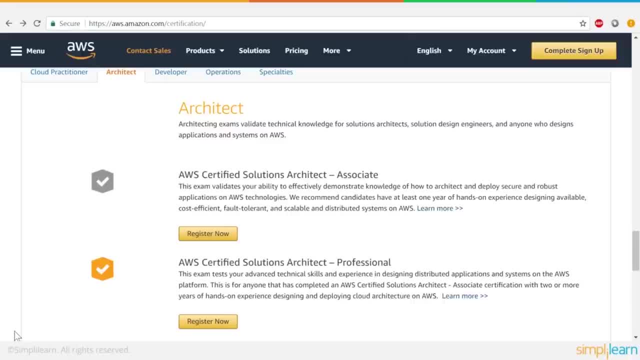 Now. first, we have the AWS Certified Solutions Architect Associate Level Certification. Now this certification is for you if you want to show off how well you can architect and deploy applications on the AWS platform. Now it is recommended that you have at least a year of experience. 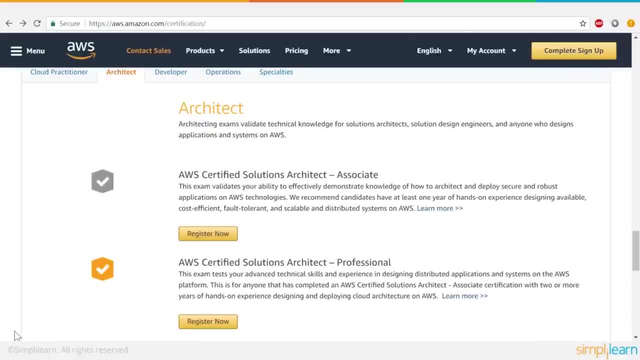 working with distributed systems on the AWS platform. At the same time, it's also required that you understand the AWS services and be able to recommend a service based on requirements. You need to be able to use architectural best practices and you need to estimate the AWS cost and how you can reduce them. 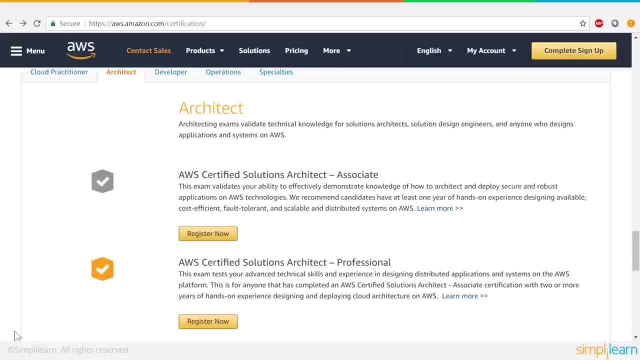 Next up you have the AWS Certified Solutions Architect Professional Level Certification. Now you will not get the certification unless you're done with the AWS Certified Solutions Architect Associate Level Certification. This is a show of your technical skills and experience in designing distributed solutions. 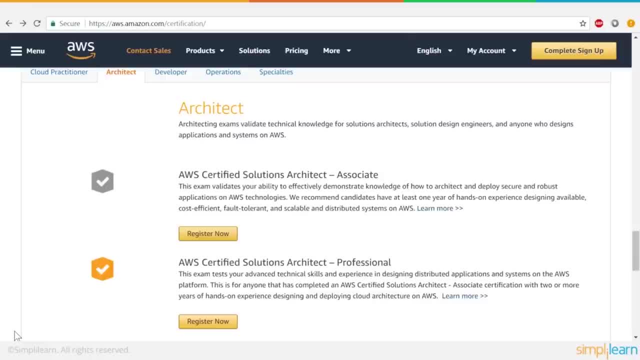 Now the AWS Certified Solutions Architect. Professional Level Certification is for you if you want to develop and maintain applications on the AWS platform. Now. this does require you to have two years of experience working with cloud architecture on AWS. At the same time, it also requires you to be able to evaluate requirements and then make architectural recommendations. 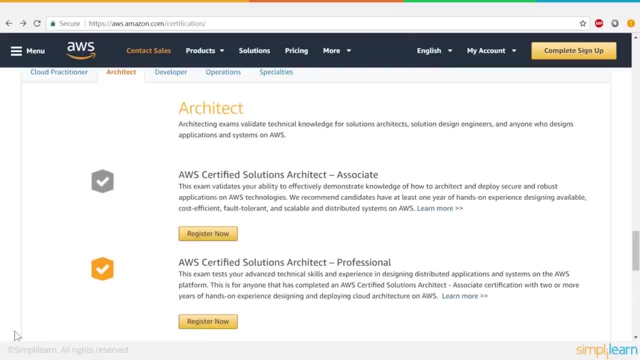 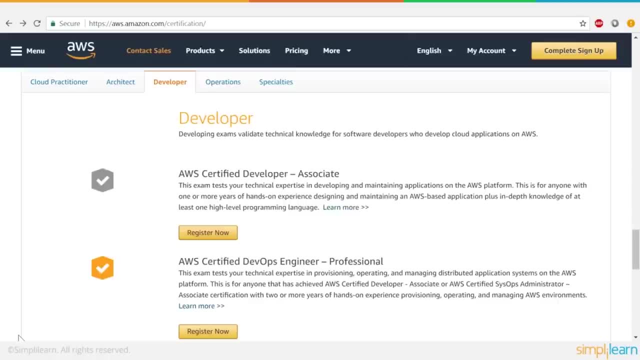 You also need to provide guidance on the best practices on architectural design across a number of different platforms. The developer level certifications are for you if you're interested in becoming a software developer Now. the AWS Certified Developer Associate Certification is to test how well you know how to develop and maintain applications on the AWS platform. 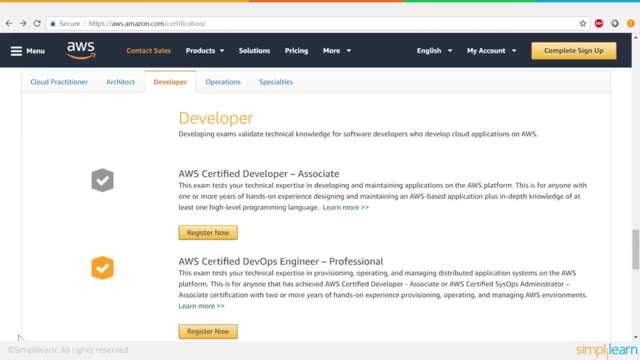 It does require you to have a year or more of hands-on experience to design and maintain AWS-based applications. Like any software developer role, it is necessary that you know in depth at least one high-level programming language. It's also necessary that you understand the core of AWS services uses and basic architectural best practices. 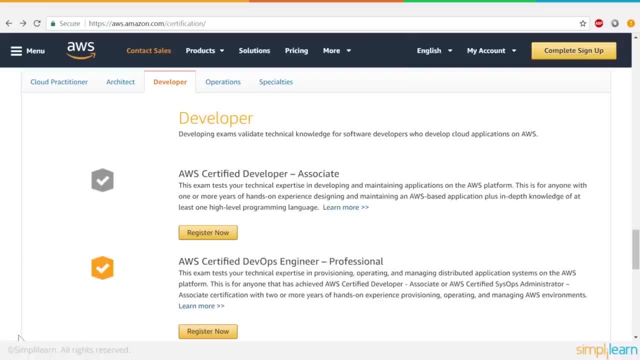 You need to be able to design, develop and deploy cloud-based solutions on the AWS platform, And you need to understand how applications can be created. You need to have experience in developing and maintaining applications For a number of AWS services. you need to be able to design, develop and deploy cloud-based solutions on the AWS platform. 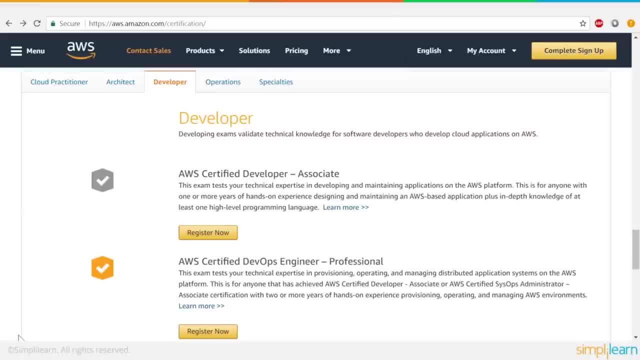 You need to have experience in developing and maintaining applications. Now for the AWS Certified DevOps Engineer Professional Level Certification. Note here that this certification is exactly the same as the one you have under the Operations role, So both of them are the same thing. 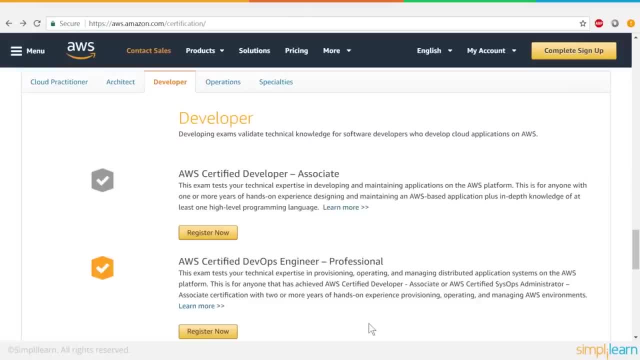 So here it tests your ability to create, operate and manage distributed applications on the AWS platform. Now it is necessary or it is mandatory to have the AWS Certified Developer Associate Certification or the AWS Certified SysOps Administrator Certification, with two or more years of hands-on experience in doing the same in the AWS environment. 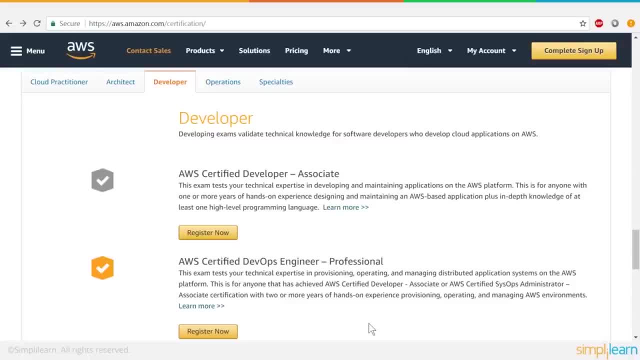 It requires you to be able to develop code in at least one high-level language. You need to be able to automate and test applications via scripting and programming, and to understand Agile or other development processes. The Operations Certifications are for you if you want to become a SysOps Administrator. Systems Administrator. 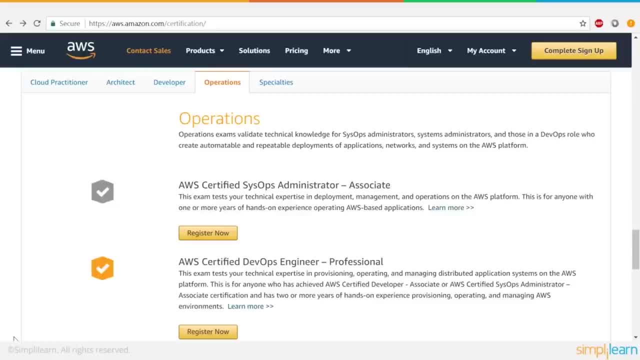 or someone in the DevOps role who wants to deploy applications, networks and systems in an automatable and repeatable way. The AWS Certified SysOps Administrator Associate Certification tests your knowledge in deployment, management and operations on the AWS platform. Now you need to have one or more years of hands-on experience in AWS-based applications. 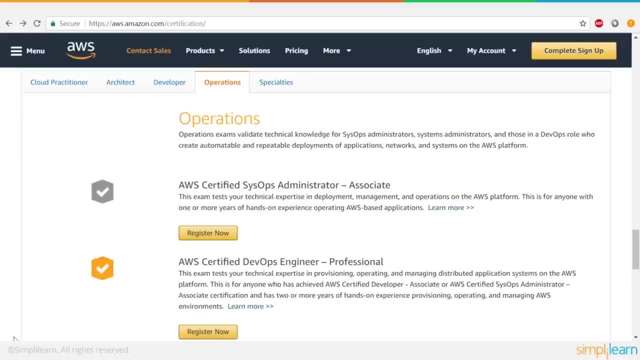 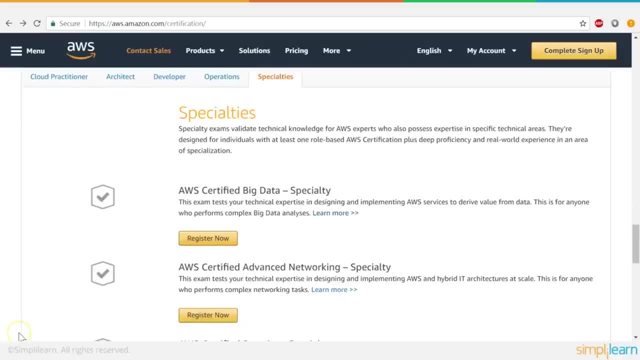 You need to be able to identify and gather requirements, then define a solution to be operated on AWS. You need to be able to provide guidance for the best practices through the lifecycle of a project as well. Now the Specialty Certifications are for you if you are well-versed in AWS. 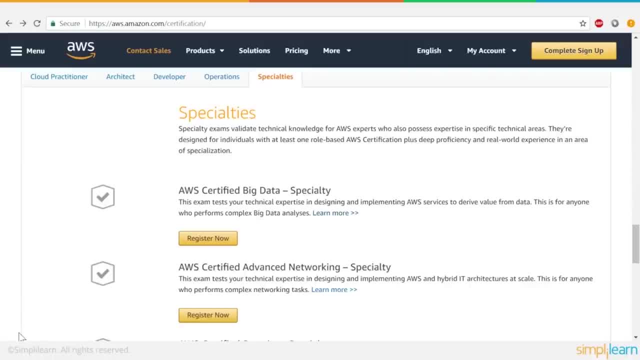 and want to showcase your expertise in other technical areas. The AWS Certified Big Data Certification showcases your ability to design and implement AWS services, which can help derive value from a large amount of complex data. You are, however, required to have completed the Foundational or Associate Level Certification before you can attempt this. 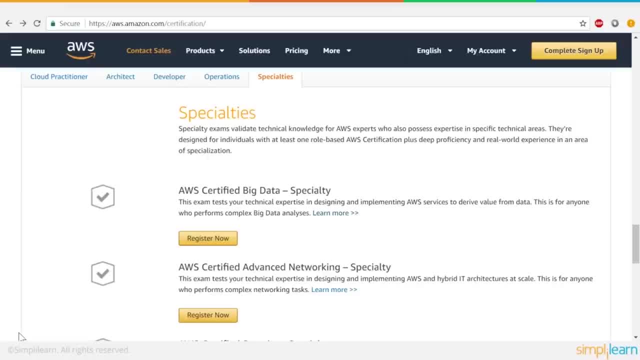 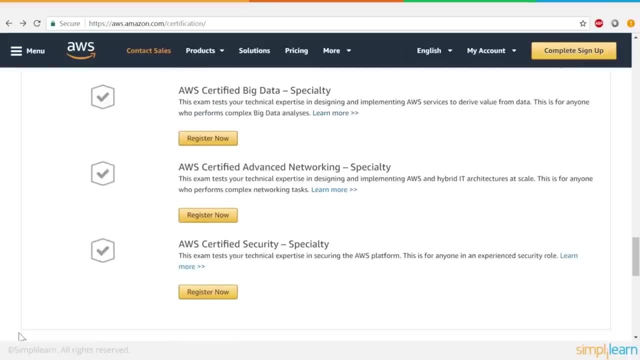 You need a minimum of 5 years of hands-on experience in the data analytics field as well. Next, we have the AWS Certified Advanced Networking Certification. This validates your ability to design and implement AWS solutions, as well as other hybrid IT network architectures, at scale. 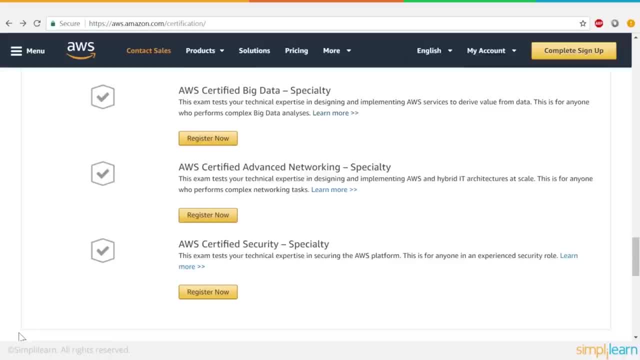 This also requires you to have completed the Foundational or Associate Level Certification. You need to have a minimum of 5 years of hands-on experience in the data analytics field as well. Lastly, we have the AWS Certified Security Certification. It helps showcase your ability to secure the AWS platform. 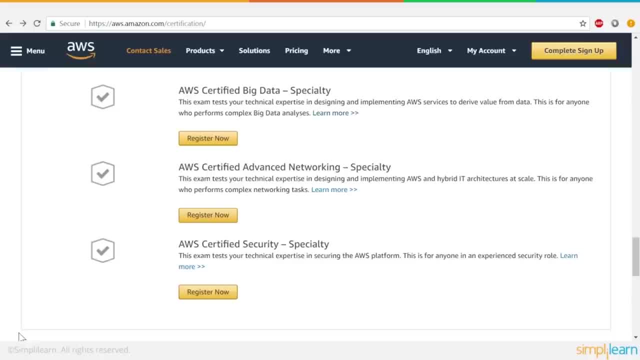 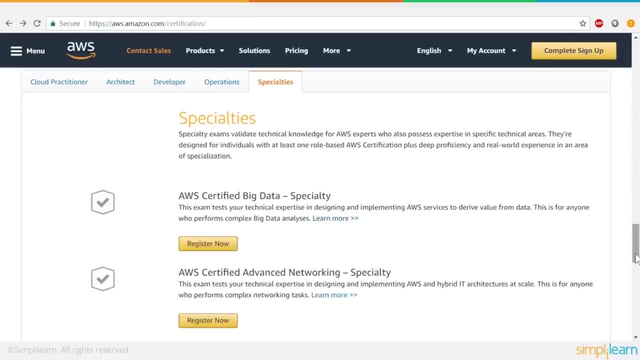 You are required to have an Associate or Crowd Practitioner level of certification, a minimum of 5 years of IT security experience and 2 years of hands-on experience securing AWS workloads. Now say I wanted to schedule an examination. So, for example, I want to do the Solutions Architect Certification. 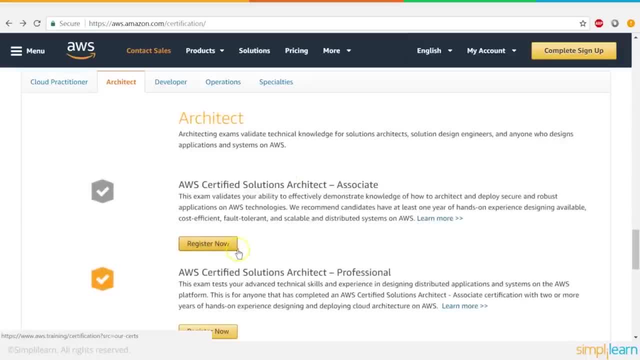 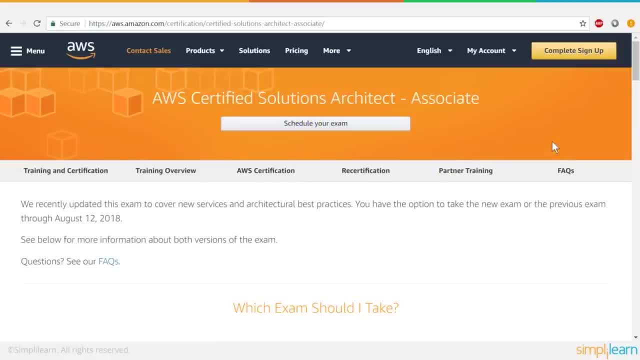 So first I would go there Now. here I can click on Register Now and the process continues, or I can click on Learn More Doing this again. I can schedule the examination here. I can also get access to other data, like the number of questions available. 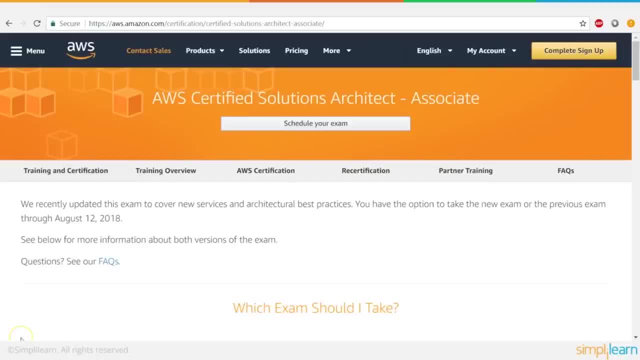 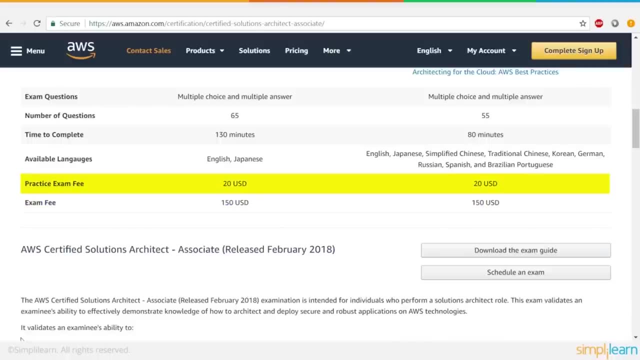 the cost of an examination, the portions I need to study, and so on. Now let's talk about Solutions Architect Certification with a little more detail. Now, this certification exam costs $150 and the practice exam costs $20.. Now here I can schedule the examination or download the exam guide. 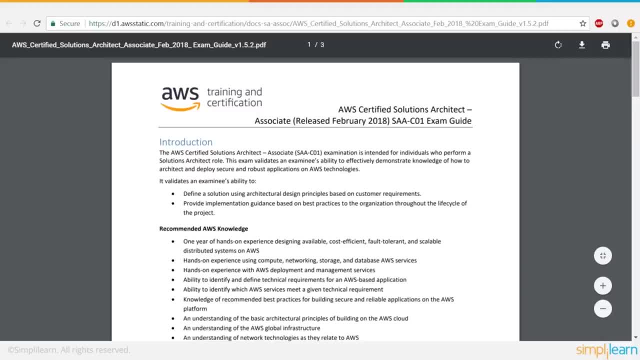 I've already downloaded the exam guide, and here it is Now. this exam guide tells you about what you need to learn and what is expected from you Here. they want you to define a solution based on requirements and provide guidance in its implementation. 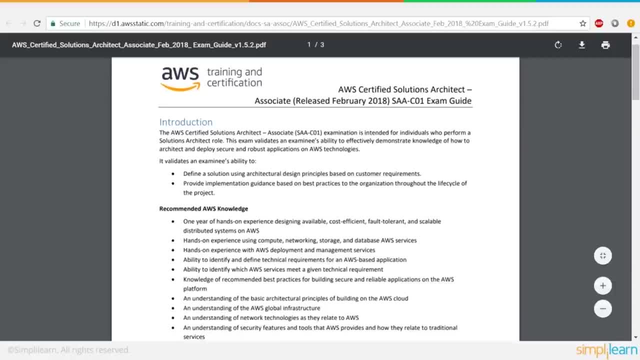 It is also recommended that you know about how the AWS services work: 1 years of hands-on experience with distributed systems on AWS to identify and define technical requirements and so on. The rest is available in the exam guide And, most importantly, they tell you the main content domains and their weightages. 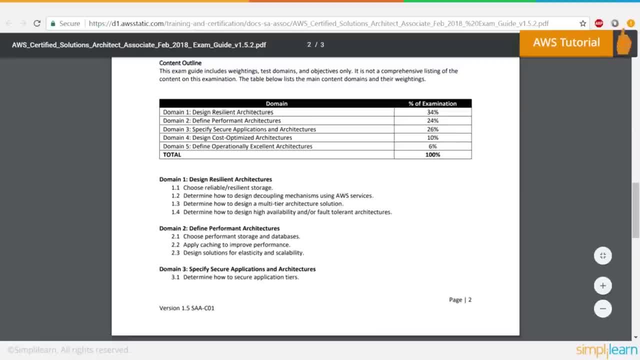 Now we have 5 domains. First domain is to design resilient architectures, which cost 34% of weightage. In domain 2, you have to define performant architectures. 3 is to specify secure applications and architectures, cost-optimized architectures. and 5 to define operationally excellent architectures. 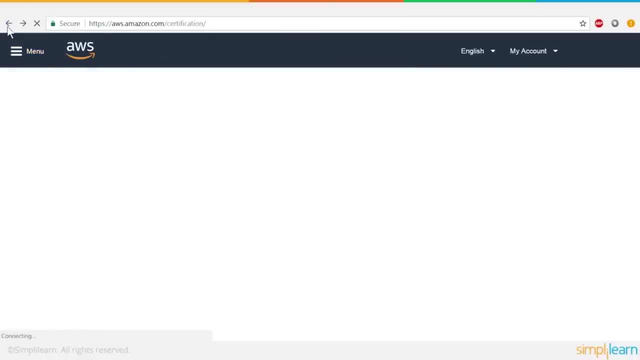 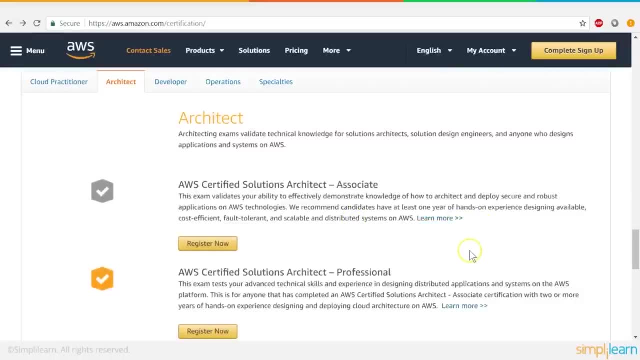 Now, like you've seen here, you've selected one certification and learnt it in detail. You can do the same for any of these other certifications. You can press learn more and download their exam guide and learn everything that you need to know. Hi guys, I'm Rahul from Simply Learn, and today we will be talking about Azure certifications. 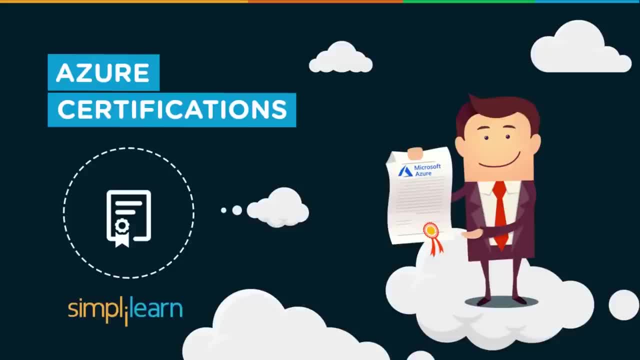 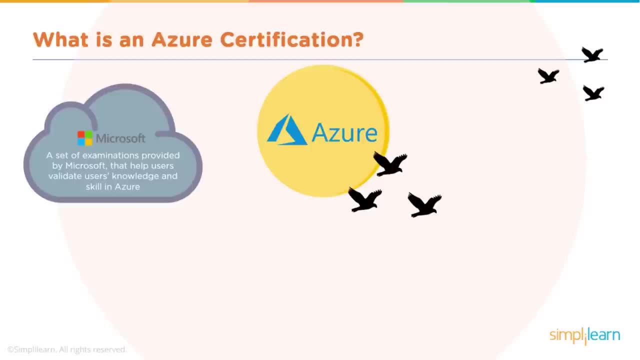 Now, before we go into a little bit of detail, let's first talk about what exactly is an Azure certification? So the Azure certifications are actually examinations that are provided by Microsoft. These help you validate how well you understand the concepts of Azure and how well you can work with it. 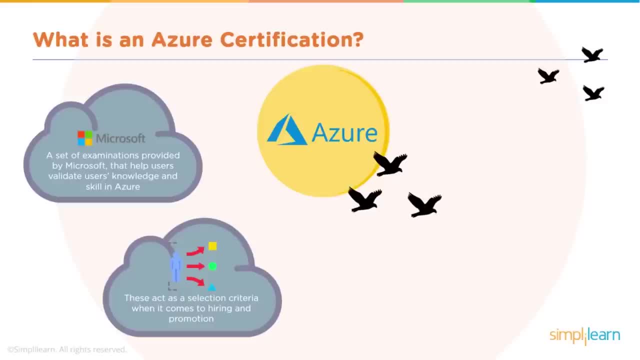 These are basically badges of honor that you can show off. These also play a very important role when it comes to hiring or promotion. You're obviously more likely to be selected if you're a certified professional. Now, these certifications cover a wide range of domains, and these certifications also work towards a specified role. 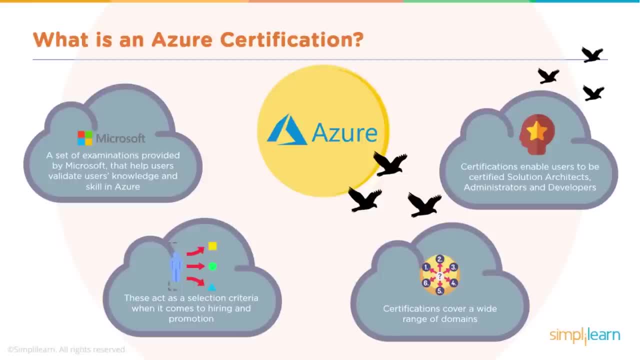 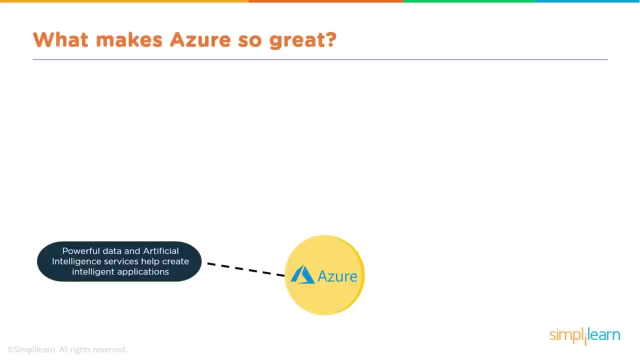 For example, you have certifications that help you become a solutions architect or an Azure administrator or an Azure developer. Now, if you need a little more convincing as to why you should be taking up an Azure certification, here are a few more. Azure provides powerful data and artificial intelligence services that help create intelligent applications. 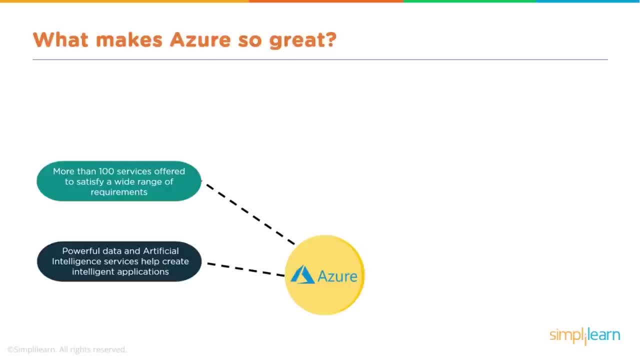 Azure has more than 100 services that span a wide range of domains. They also help satisfy a great number of requirements. More than 80% of the Fortune 500 companies use Microsoft Azure. Azure provides a wide range of cloud services, including Microsoft Azure, for their cloud computing requirements. 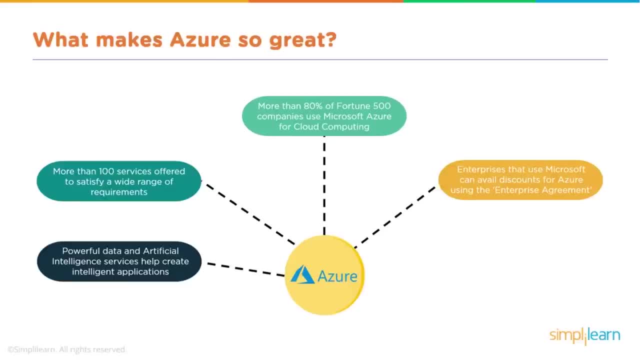 Not to mention, these organizations that use Microsoft products can actually avail an enterprise agreement that gives them discounts on Azure services. And finally, Azure provides services across 42 regions in the world, which is more than any other cloud service provider does in the market right now. 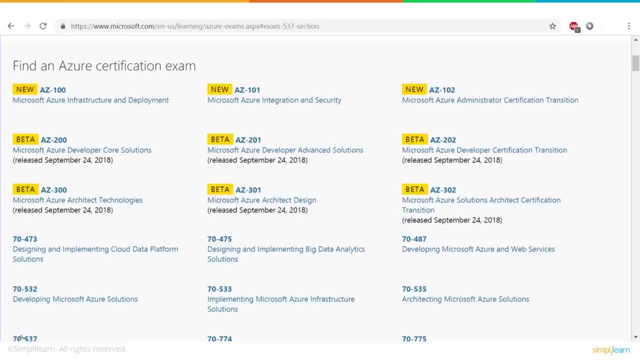 Now let's talk about Azure certifications. So it's highly likely that you've heard of Microsoft's more popular certifications: the 70532, 70533, and 70535.. But Microsoft is changing its approach towards certifications. Microsoft's new certifications aim to make the individual fall into a particular role. 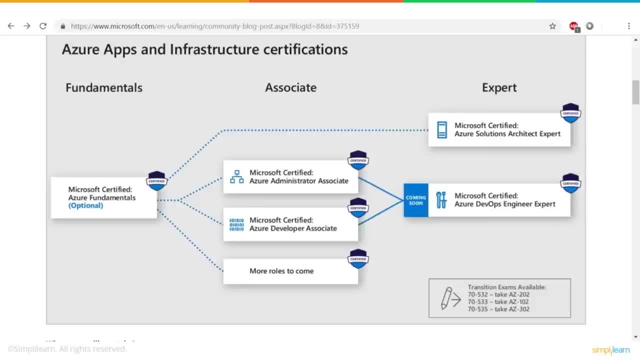 For example, the Azure Administrator Associate, Azure Developer Associate, Azure Solutions Architect and the Azure DevOps Engineer Expert. This is what Microsoft introduced in the Ignite conference that took place on September 24th. There, Microsoft introduced new certifications that fall under the AZ category. 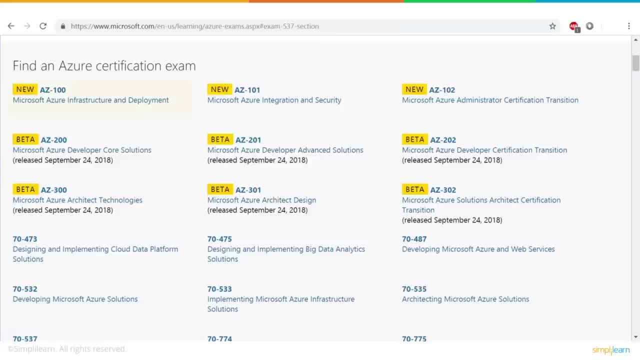 Now, to become an Azure Administrator Associate, you'll have the AZ-100 certification, or the Microsoft Azure Infrastructure and Deployment, and the AZ-101, or Microsoft Azure Integration and Security. To become an Azure Developer, you need the AZ-200, which is the Microsoft Azure Developer Core Solutions certification. 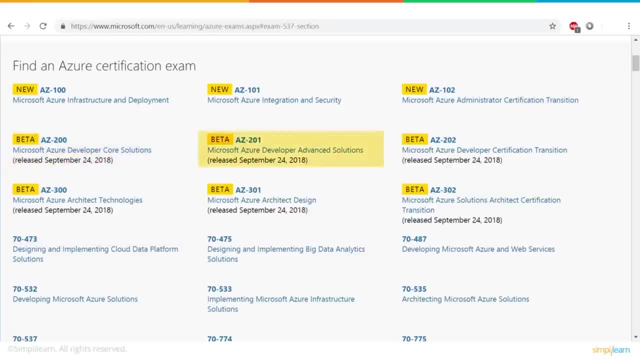 and AZ-201, or the Microsoft Azure Developer Advanced Solutions certification. Finally, to become a Solutions Architect, you'll need the AZ-300, or the Microsoft Azure Architect Technologies, and the AZ-301, or the Microsoft Azure Architect Design. Now, these were all introduced on September 24th when the Ignite conference took place. 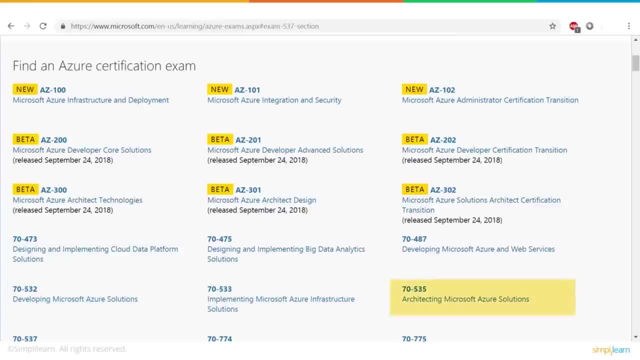 Now the old certifications- the 532,, 533, and 535, will be discontinued from the 31st of December 2018.. So what happens to the people who've actually done it? That's why Microsoft introduced the AZ-102,, 202, and 302 transition certifications. 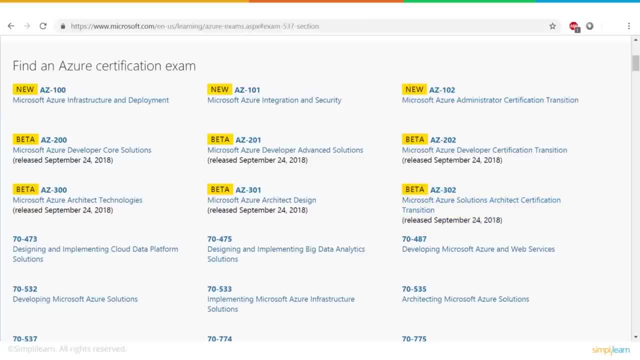 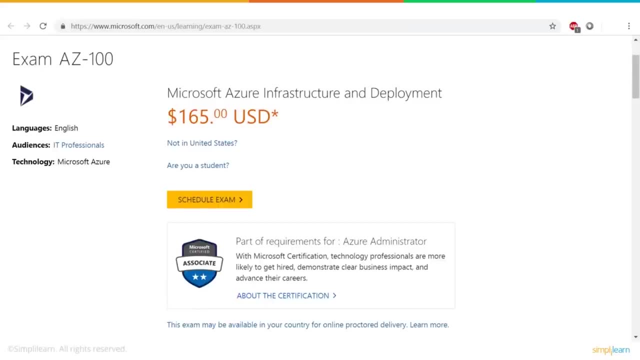 Now we'll talk about that in a little bit. So now let's go into all of the new certifications in detail. So now let's talk about Exam AZ-100, or the Microsoft Azure Exchange Certification. Now let's talk about the Microsoft Azure Exchange Certification. 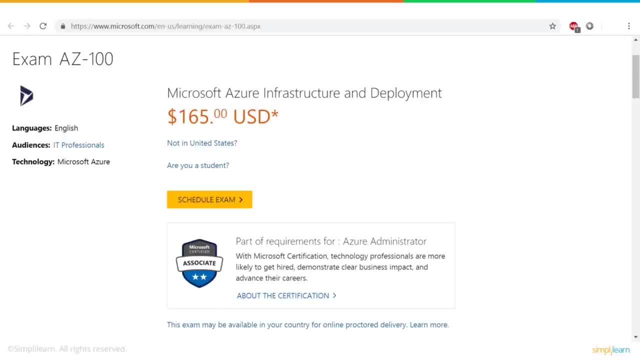 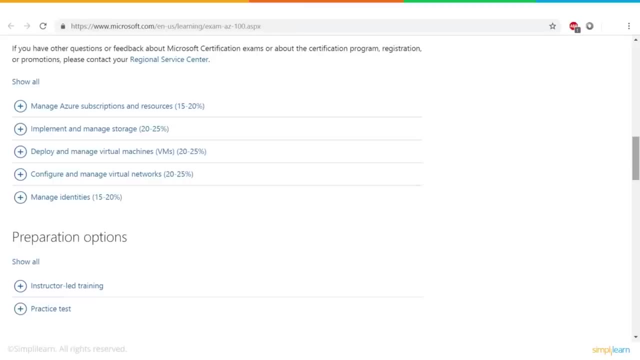 So this is basically part one of two when it comes to becoming an Azure administrator. This costs $165 US dollars. Now let's have a look at the syllabus for this exam, some of the domains that you need to prepare for and their approximate weightages. 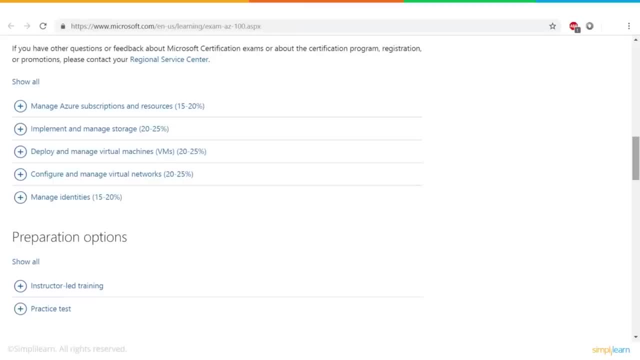 So, first off, you need to know how you can manage Azure subscriptions and resources. This involves managing subscriptions, analyzing how resources are being used and how they're consumed, and managing other resource groups. Secondly, you have implementing and managing storage. You need to know how you can create and configure storage accounts. 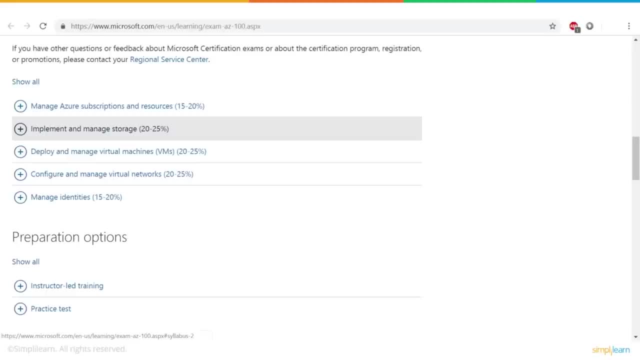 how you can import and export data to Azure, configure Azure files and how you can implement Azure backup. Then you have deploying and managing virtual machines. You need to know how you can create and configure virtual machines for Windows or Linux. You need to know how you can automate deployment of virtual machines. 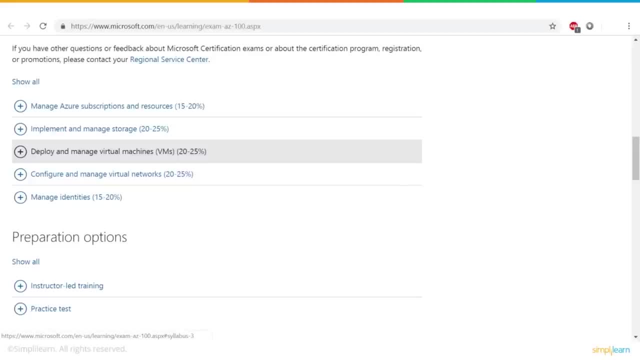 You need to know how you can manage Azure virtual machines and manage virtual machine backups. Then you need to know how you can configure and manage virtual networks. You need to be able to create connectivity between virtual networks. how you can implement and manage virtual networking. 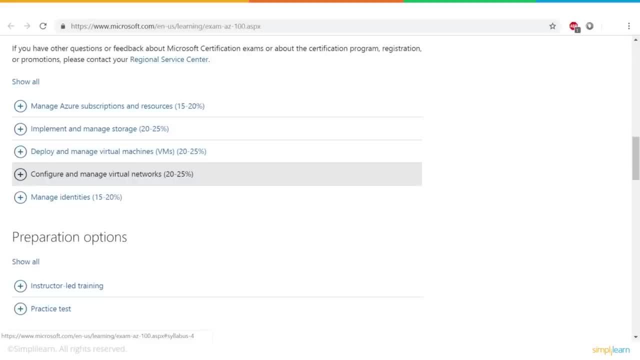 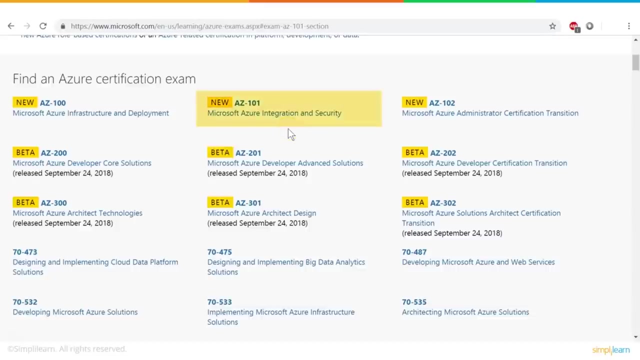 configure name resolution groups. Finally, you need to know how you can manage identities. You need to be able to manage Azure Active Directories and you need to know how you can implement and manage hybrid identities. The next step in becoming an Azure administrator is to do the AZ-101 or the Microsoft Azure Integration and Security Certification. 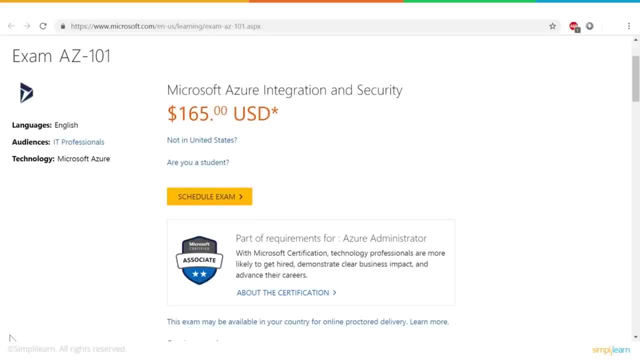 The AZ-101, or the Microsoft Azure Integration and Security Certification, goes into a little more detail when it comes to becoming an Azure administrator. This certification costs $165.. Now let's have a look at some of the important topics that you need to know for this examination. 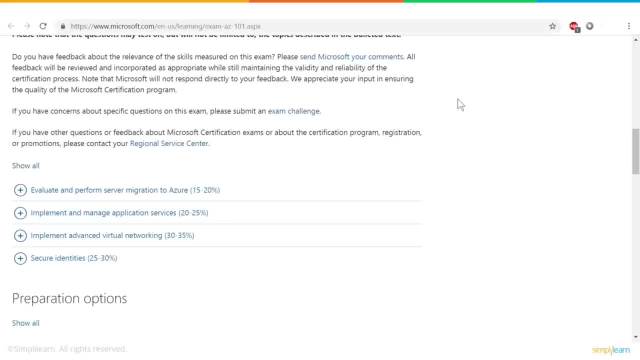 So let's have a look at some of the portions that you need to be well-versed with to perform well in this examination. First up, we have evaluating and performing server migrations to Azure. Then we have implementing and managing application services. 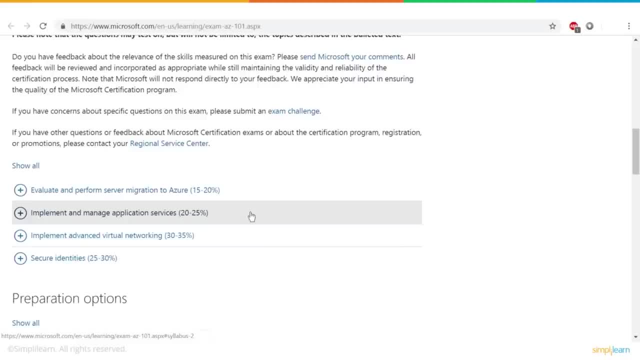 which involves configuring serverless computing, managing app service plans and managing app services. Then you have implementing advanced virtual networking. that involves implementing application load balancing, implementing Azure Load Balancer, monitoring and managing networking, integrating the on-premise network with the Azure network, and so on. 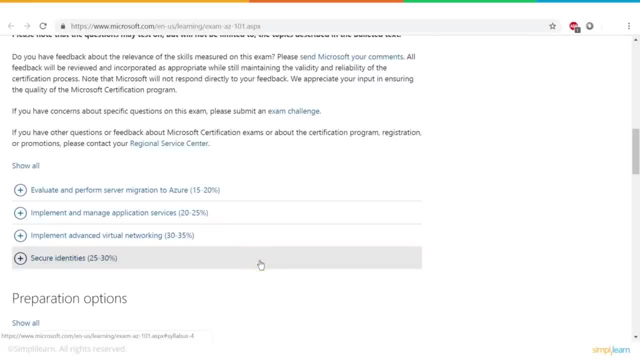 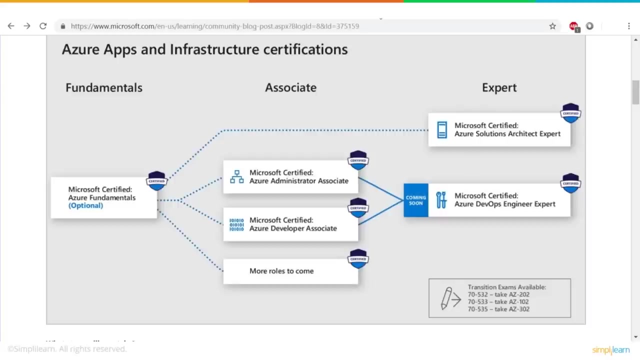 And, finally, securing identities. You need to be able to implement a multi-factor authentication, manage a role-based control system, implementing Azure Active Directories and privilege identity management. So, after you're done with AZ-100 and 101, you become a Microsoft Certified Azure Administrator Associate. 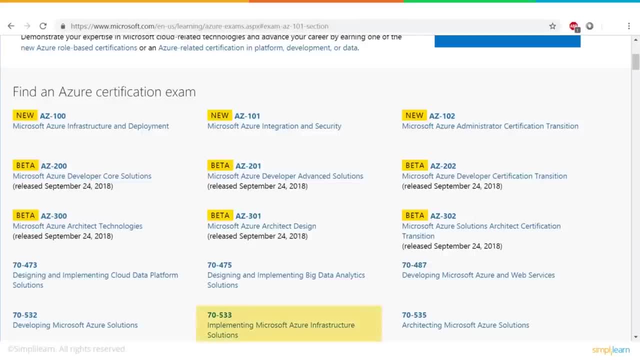 Now what happens to the people who've already done the Implementing Microsoft Azure Infrastructure Solutions Certification or the 70533?? It's for these people that Microsoft has the AZ-102 or the Microsoft Azure Administrator Certification Transition. Now this examination that costs 99 US dollars. 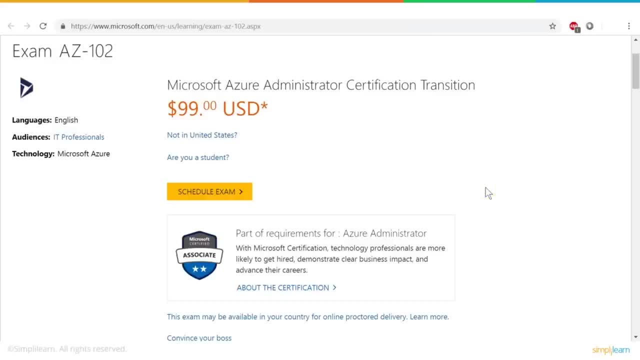 contains concepts from both AZ-100 and AZ-101.. And this exam is only valid for people who've already completed the 70533 certification. Now, if you have completed the 70533, I suggest you do this transition certification immediately, as this will be discontinued by Microsoft by the 31st of March 2019.. 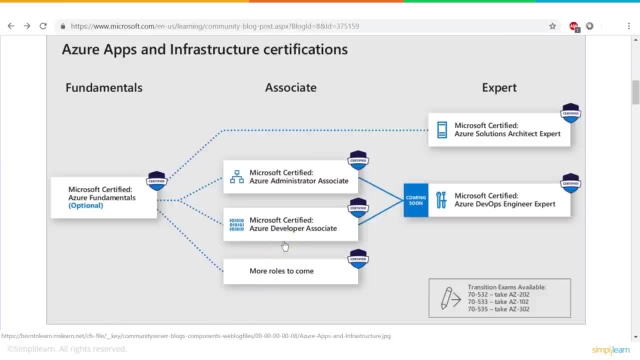 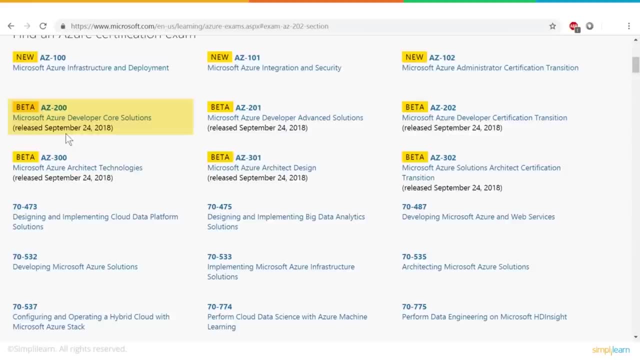 Now let's have a look at how you can become a Microsoft Certified Azure Developer Associate. To do this, you need to complete two certifications: The AZ-200, or the Microsoft Azure Developer Co-Solution certification, and the AZ-201, or the Microsoft Azure Developer Advanced Solutions certification. 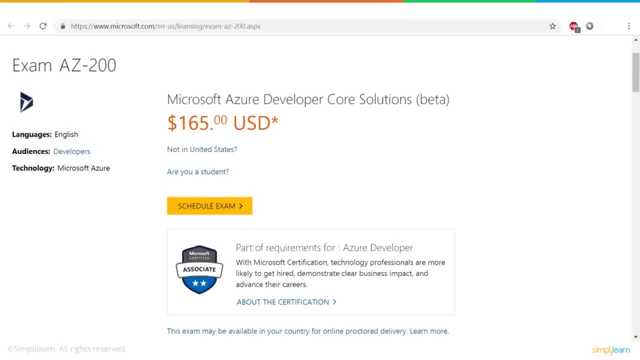 So now let's have a look at the AZ-200.. Now, this certification is part 1 of 2 when it comes to becoming an Azure Developer Associate. It costs 165 US dollars. Now this examination is in its beta phase. 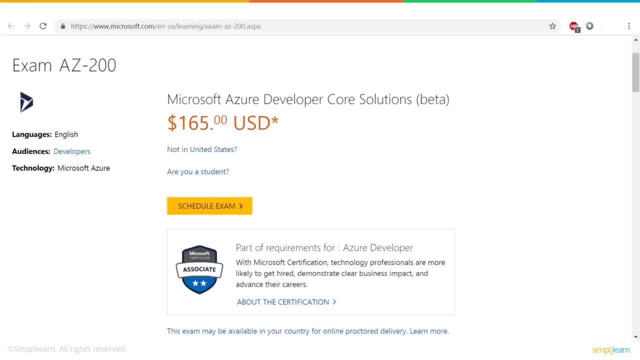 which means that, unlike normal examinations, where you get your results as soon as you finish the examination, this exam will take at least one or two weeks before you can get your result. The questions are still being worked on and improved upon. There's also a limitation to how many people can take the exam at the moment. 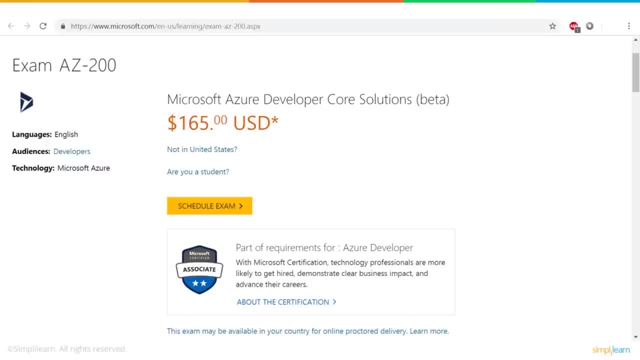 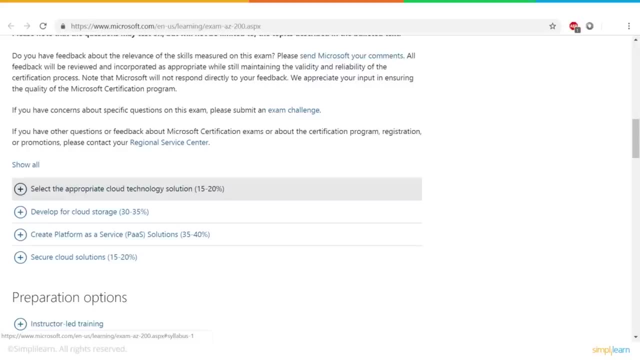 Now let's have a look at some of the portions that you need to prepare for for this examination. You need to be able to select an appropriate cloud technology solution based on your requirements. This may involve a compute solution, integration or a storage solution. 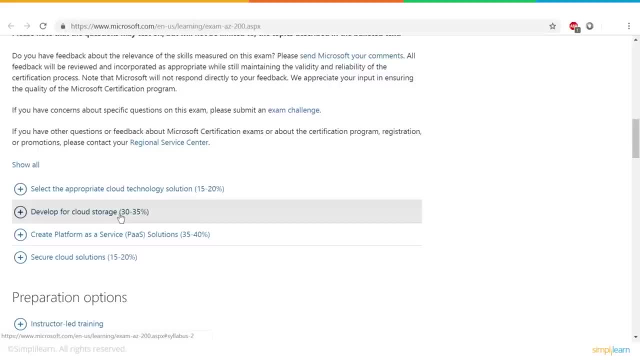 Next, you need to be able to develop for cloud storage, which involves developing solutions that involve storage tables, file storage, relational databases and so much more. You need to be able to create platform as a service solutions, which involves creating web applications, mobile applications, app services. 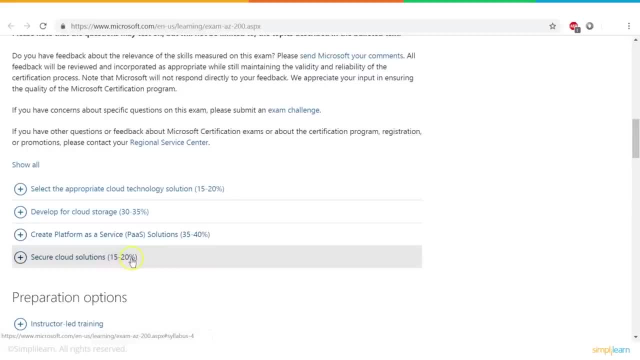 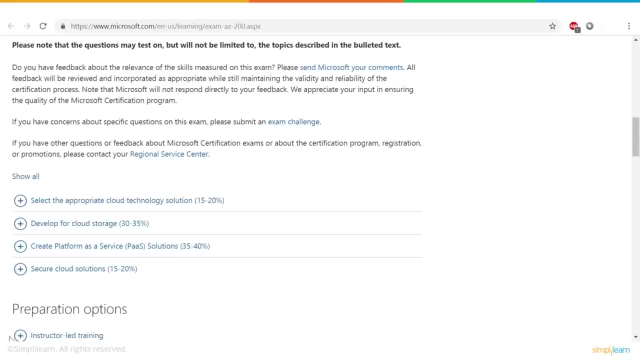 serverless functions and so much more. And finally, you need to be able to secure cloud solutions. You need to implement authentication, access control and secure data solutions. Now Microsoft recommends that you have at least a year of experience working with Microsoft Azure, creating applications with Azure tools and technologies. 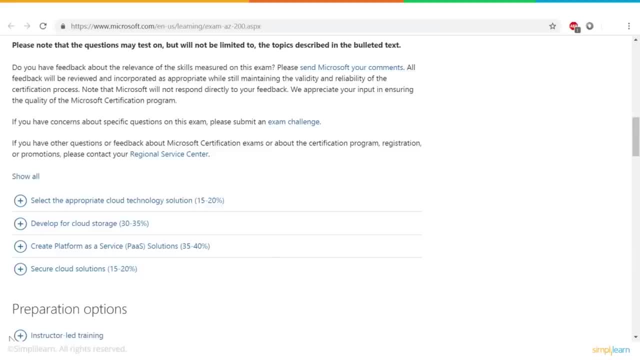 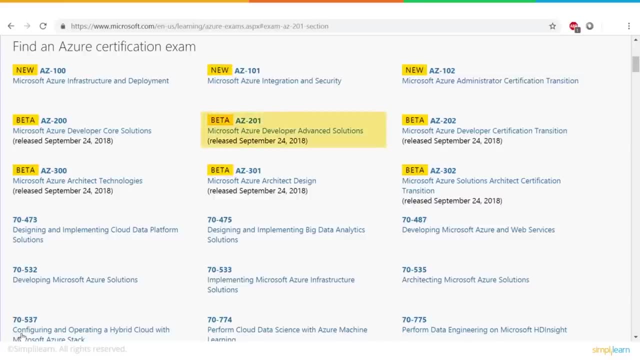 while at the same time having a solid understanding of all the phases of software development. Now let's have a look at the next step to becoming a Microsoft Azure developer. You need to do the AZ-201 or the Microsoft Azure Developer Advanced Solutions Certification. 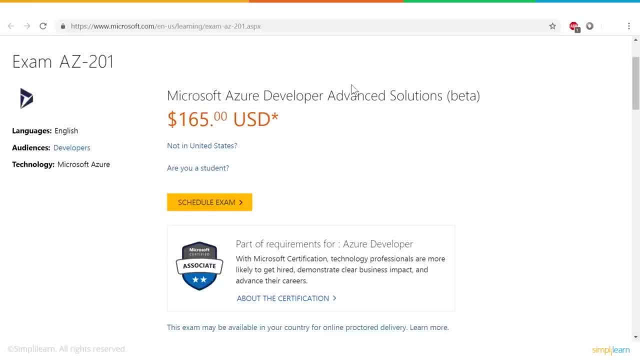 Now let's have a look at that. Now, this examination is also in its beta phase and will move to its final version in the next few months. As of now, it costs $165.. Now let's have a look at some of the portions. 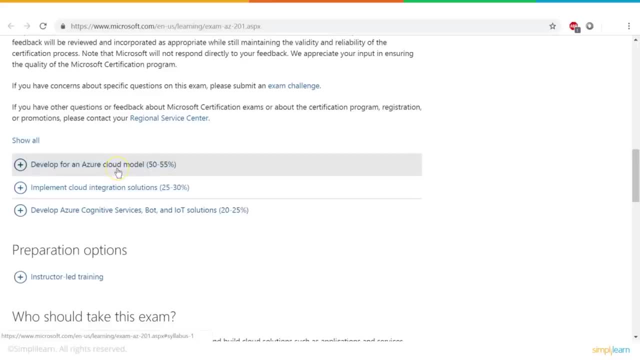 that you need to prepare for for this examination. You need to know how you can develop for an Azure cloud model. You need to develop for auto-scaling, develop for long-running tasks, distribute a transaction and so much more. You need to know how you can implement cloud integration solutions. 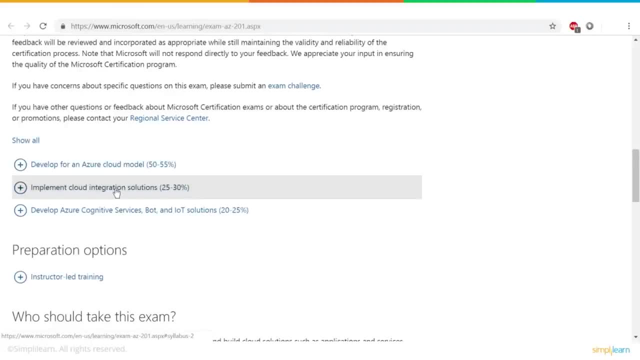 like managing APIs using API management, configure a message-based integration architecture to develop an application message model, and so much more. And finally, you need to know how you can develop Azure's cognitive services, bot and IoT solutions. You need to be able to create and integrate bots. 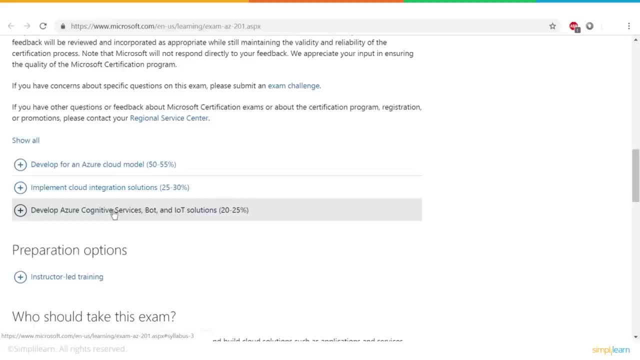 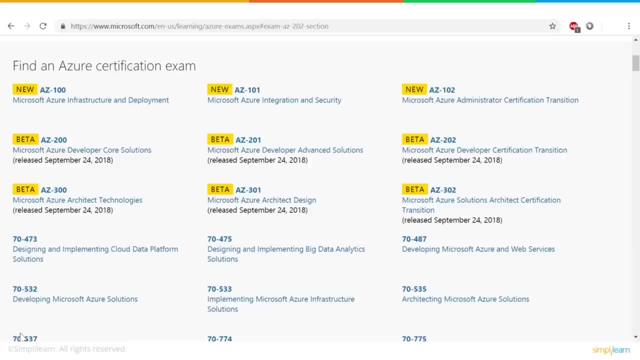 create and implement IoT solutions and to integrate the Azure cognitive services in an application. After you're done with all of this, you become a Microsoft-certified Azure Developer Associate. Now let's talk about AZ-202.. Now, this is a transition examination. 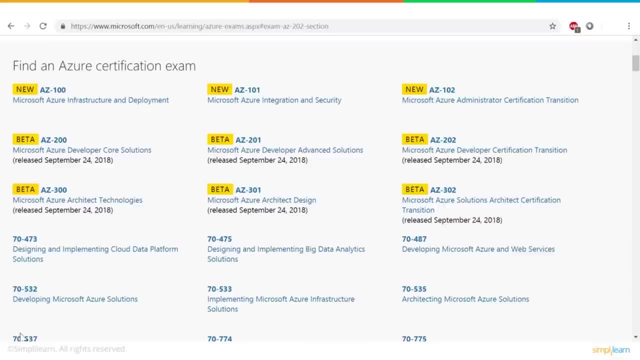 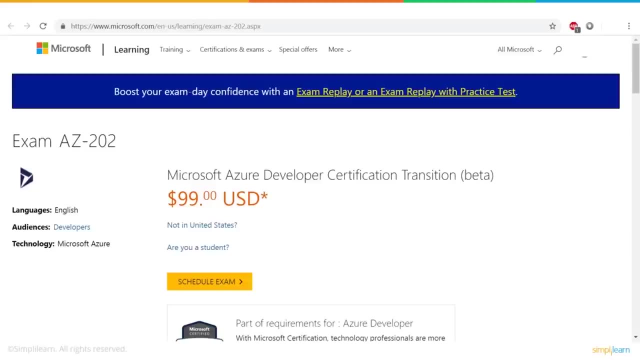 for anyone who's done 70532 or developing Microsoft Azure Solutions Certification. Now, just like the other transition certification, this costs 99 US dollars and it is in its beta phase Now. this is accessible for only people who have done the 70532. 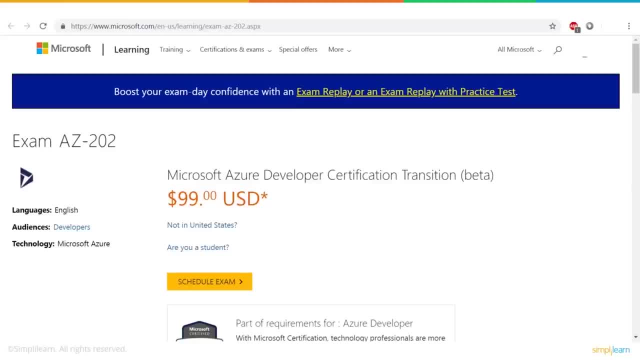 and is available only for a limited period of time. This will be discontinued from the 31st of March 2019.. Now this has concepts that have been included in both AZ-200 and AZ-201.. Concepts like developing for cloud storage. 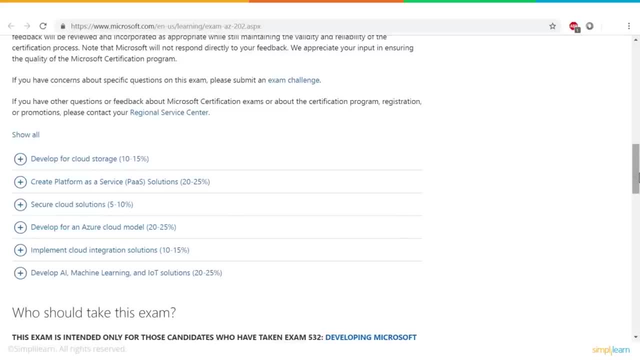 creating platform as a service solutions, securing cloud solutions, developing for an Azure cloud model, implementing cloud integration solutions, developing AI, machine learning and IoT solutions. Now, after you're done with this, you can become a Microsoft-certified Azure Developer Associate. 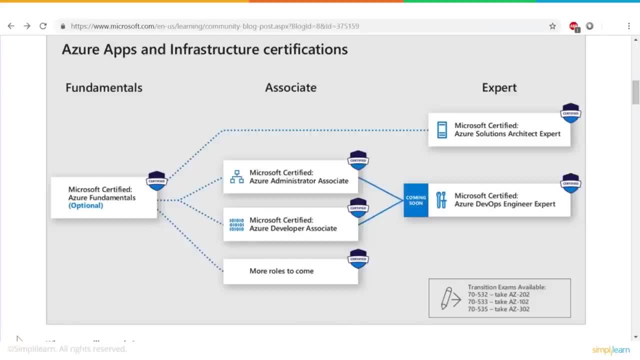 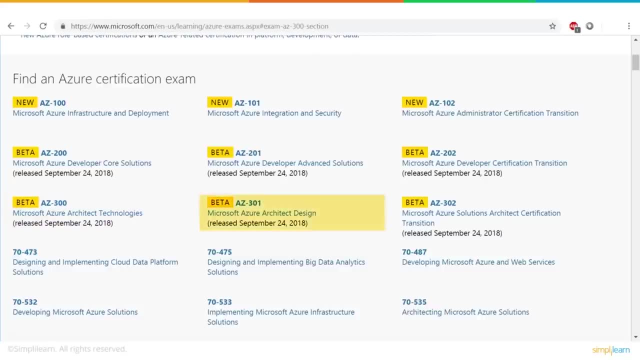 Now let's find out how you can become a Microsoft-certified Azure Solutions Architect Expert. For this, you need to do two certifications: the AZ-300 and the AZ-301.. Now let's have a look at AZ-300,. 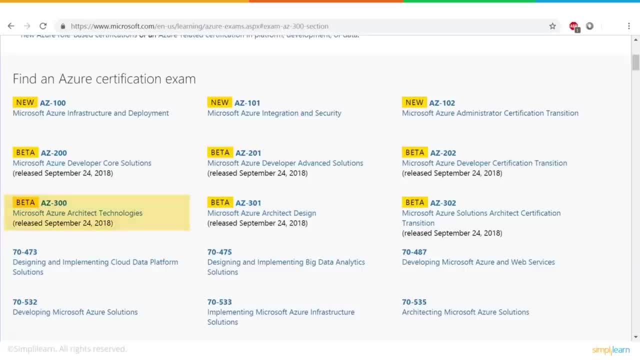 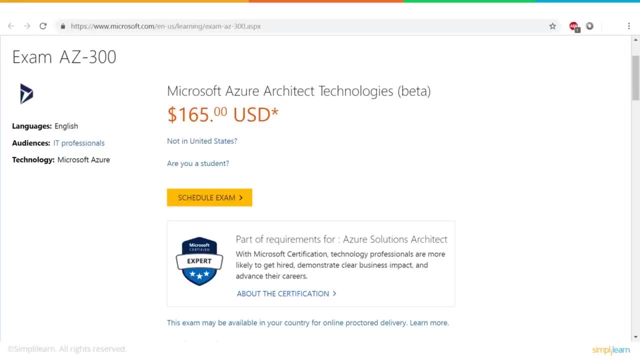 which is the Microsoft Azure Architect Technologies certification. Now the AZ-300 is still in its beta phase and costs $165.. This is part one of two for becoming a Microsoft-certified Azure Solutions Architect Expert. Now let's talk about some of the topics. 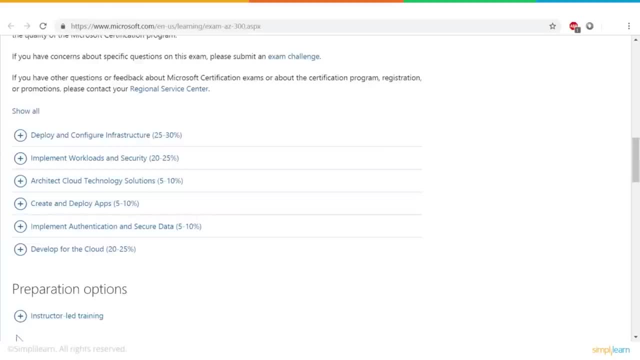 that you need to prepare for for this examination. You need to know how you can deploy and configure infrastructure, which involves analyzing resource utilization consumption, creating and configuring storage accounts, creating and configuring virtual machines for Windows and Linux, automating deployment of virtual machines and so much more. 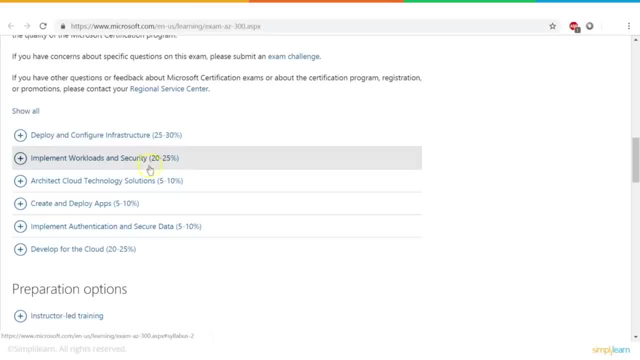 Then you need to know how you can implement workloads and security, like migrating servers to Azure, configure serverless computing, implementing application load balancing, managing role-based access control, implementing multi-factor authentication, and so on. Then you need to architect cloud technology solutions. 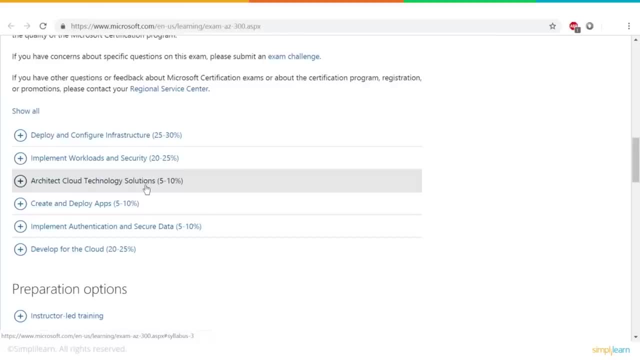 You need to be able to select appropriate compute solutions, integrate solutions, storage solutions. You need to be able to create and deploy applications, like, for example, creating web applications using PaaS. create an application or service that runs on Service Fabric. 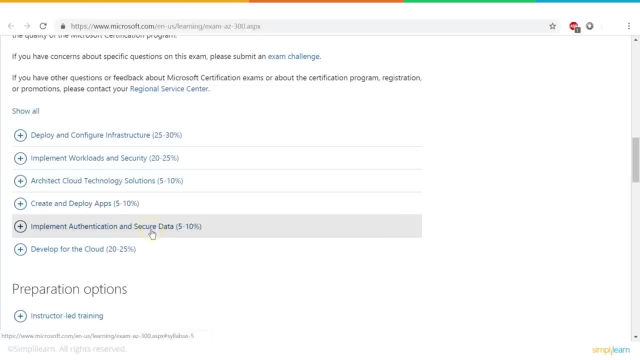 design and develop applications that run in containers and so on. Then you need to implement authentications and secure data And, finally, you need to develop for the cloud, which means you need to know how you can develop long-running tasks, configure message-based integration, develop for auto-scaling. 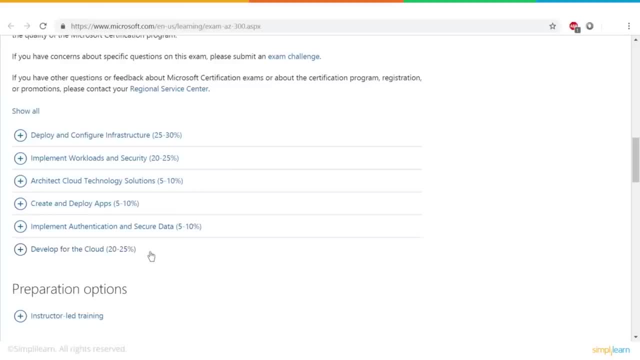 implement distributor transactions and so on. Now, this certification does require you to be having expert-level skills in at least Azure administration, Azure development or DevOps. You also need to have experience with the various steps in IT operations, like networking, virtualization, security and so on. 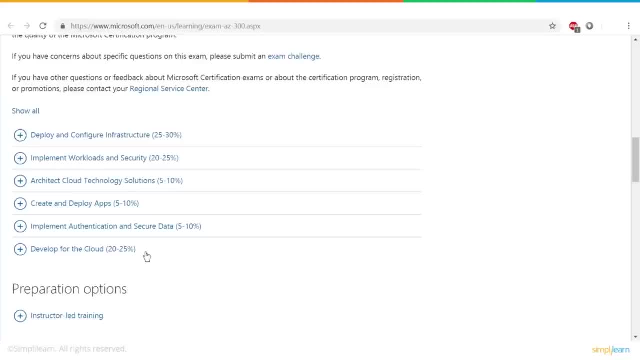 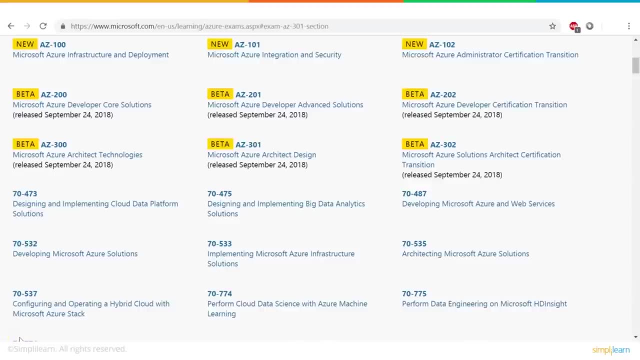 This is because the Azure Solutions Architect play a very important role of advising stakeholders to convert their requirements into scalable, secure and reliable solutions. So now the next step is to do the AZ-301, or the Microsoft Azure Architect Design certification. Now let's have a look at that. 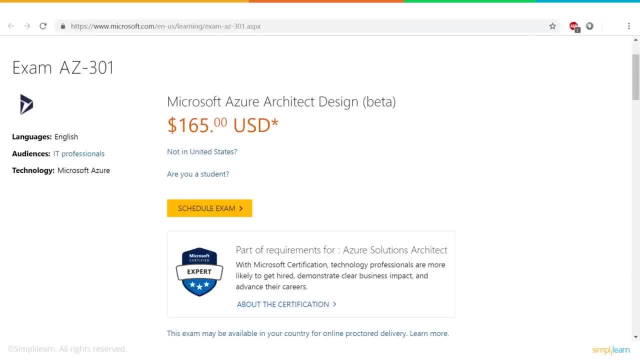 Now, like all the other certifications, this costs $165 and is still in its beta phase. This is the final step in becoming an Azure Solutions Architect expert. Now let's have a look at some of the topics that you need to prepare for for this certification. 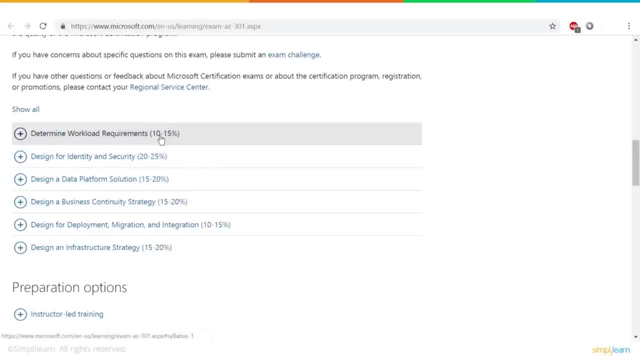 Firstly, you need to know how you can determine workload requirements. You need to know how to gather information and requirements to optimize the consumption strategy and to design an auditing and monitoring strategy. You need to design for identity and security, like design, identity management, design authentication, authorization. 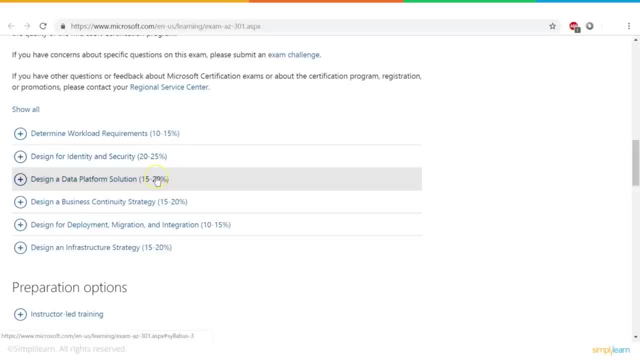 and a monitoring strategy for identity and security. Then you need to know how you can design a data platform solution. You need to design a data management strategy, a data protection strategy, document, data flows and so on. Then you need to design a business continuity strategy. 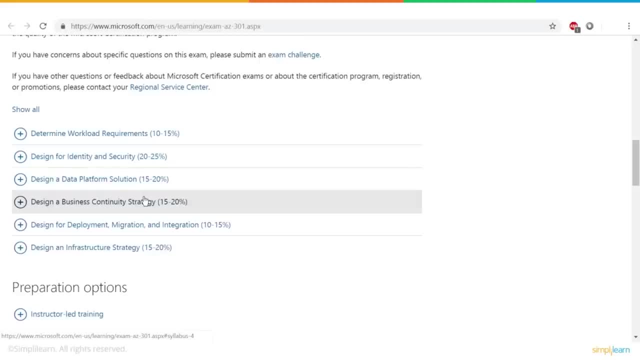 For example, to design a site recovery strategy, ensure that there's high availability, design a disaster recovery strategy and to design a data archiving strategy. Then you need to design for deployment, migration and integration. You need to design deployments, design migrations. 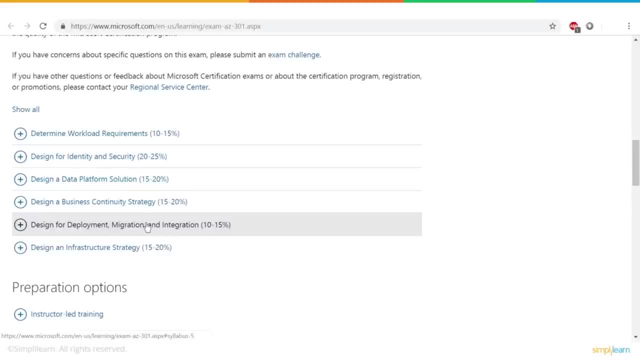 and design an API integration strategy. And finally, you need to know how you can design a storage strategy, a compute strategy, networking strategy and so on. After you're done with all of this, you become a Microsoft-certified Azure Solutions Architect expert. 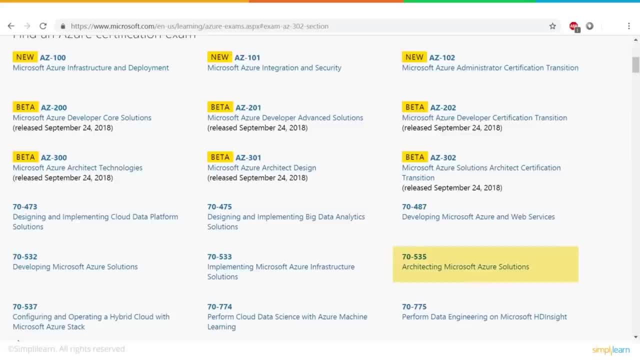 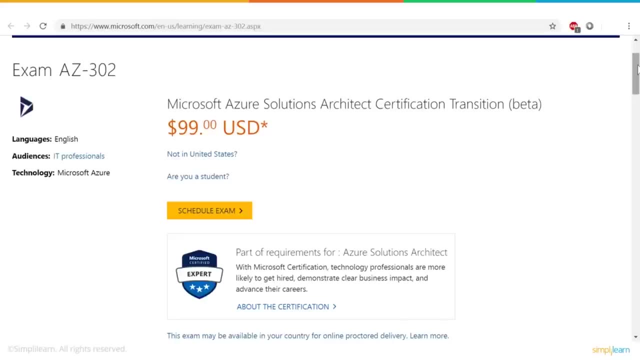 So what about those people who've already done the 70535 or the architecting Microsoft Azure Solutions certification? That's where the AZ302 comes in Now. the AZ302 is a transition certification which costs 99 US dollars. This acts as a replacement for anyone who's done the. 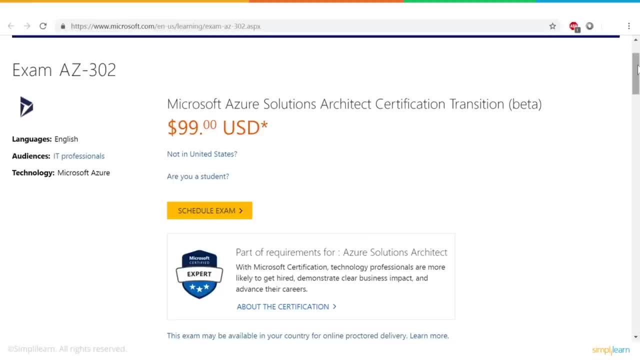 70535 certification. Now, this is again in its beta phase, but will last only till March 31st 2019.. Now, if you finish the certification, you get to become an Azure Solutions Architect expert. Now this consists of topics included in both AZ300 and 301.. 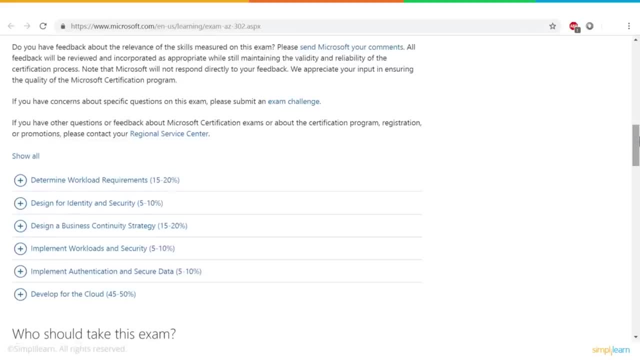 Concepts like determining workload requirements, designing for identity and security, designing a business continuity strategy, implementing workloads and security, implementing authentication and securing data, and developing for the cloud. Now, what we've mentioned in this video are the most important Azure certifications. Now there are older certifications, but we've not covered them because we'll be focusing on the more important role-based examinations that have been introduced recently. The cloud tech services market is expected to grow 17.3% in the span of 2018 to 2019,. 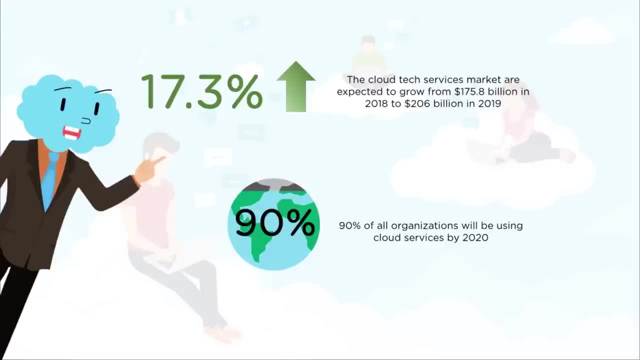 which means there's a growth from $175.8 billion to a whopping $206 billion in 2019.. As of 2020, it's expected that 90% of all organizations in the world would be using cloud services, Not to mention several organizations around the world. 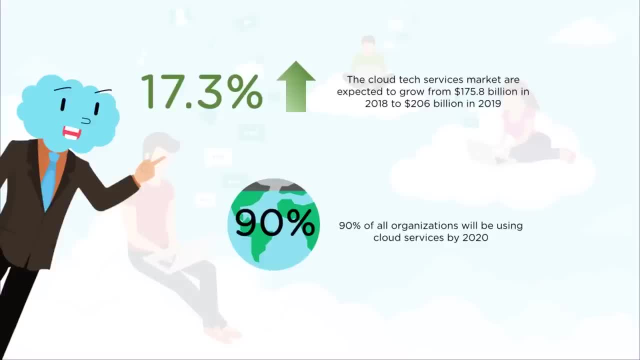 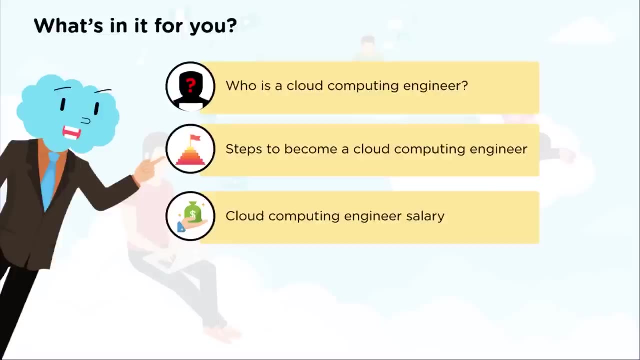 suggest that using cloud computing services has enabled their employees to experiment a lot more with technologies like machine learning and artificial intelligence. So here's what we'll be going through today. Firstly, we'll be talking about who is a cloud computing engineer, the steps you need to take to become a cloud computing engineer. 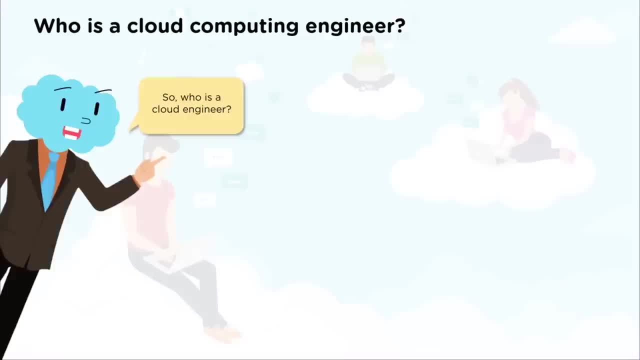 and the cloud computing engineer salaries. First off, who is a cloud computing engineer Now? a cloud computing engineer is an IT professional who takes care of all the technical aspects of cloud computing, be it design, planning, maintenance and support. Now a cloud computing engineer can take up a number of different career paths. 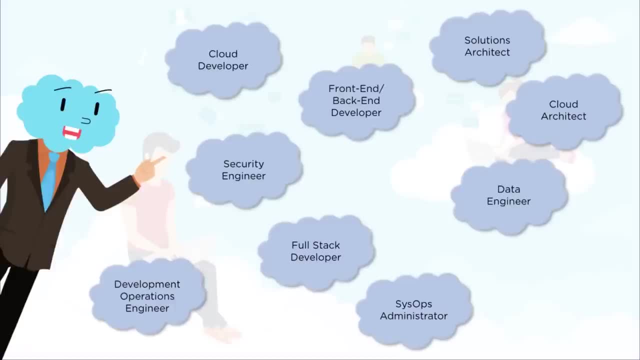 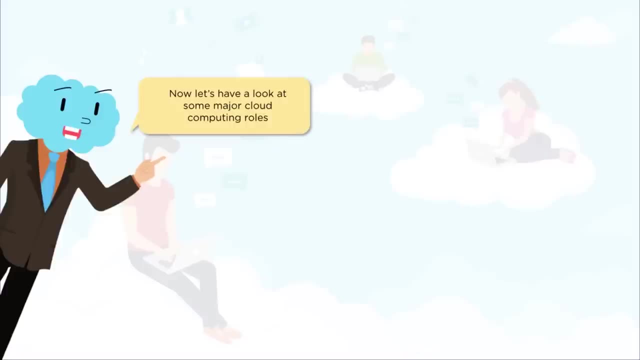 This could be that of a cloud developer, security engineer, a full-stack developer, SysOps administrator, solutions architect, cloud architect, and so much more. Now let's have a look at some of the major cloud computing roles. First off, we have solutions architect. 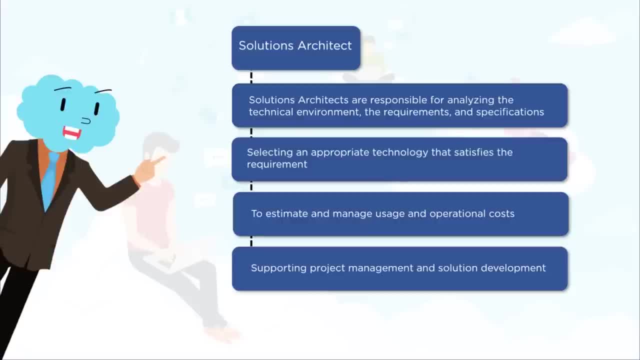 Now, these are individuals who are responsible for analyzing the technical environment in which they are going to produce the solutions, the requirements and the specifications. Secondly, they are required to select an appropriate technology that satisfies said requirements. They need to estimate and manage the usage. 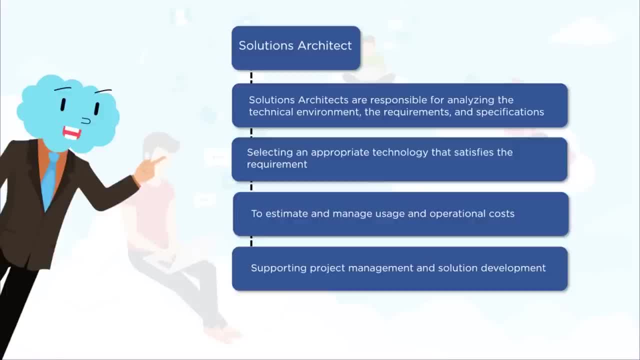 and the operational costs of the solutions they provide, and they need to support project management as well as solution development. Next, we have SysOps administrators. They are involved in deploying, managing and operating highly scalable and fault-tolerant systems. They need to select an appropriate service based on compute. 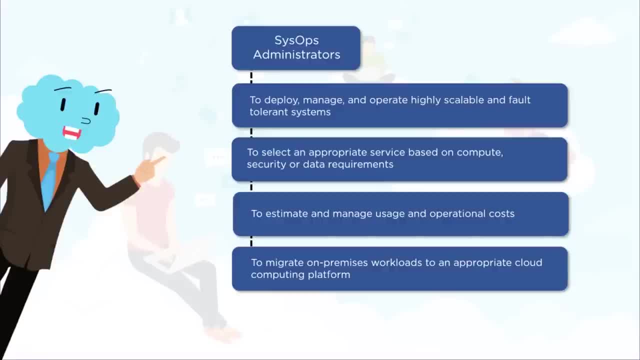 security or data requirements. They need to estimate and manage usage and operational costs, and they need to be able to migrate on-premises workloads onto an appropriate cloud computing platform. So, among both of these roles, there are certain requirements that are remaining constant. 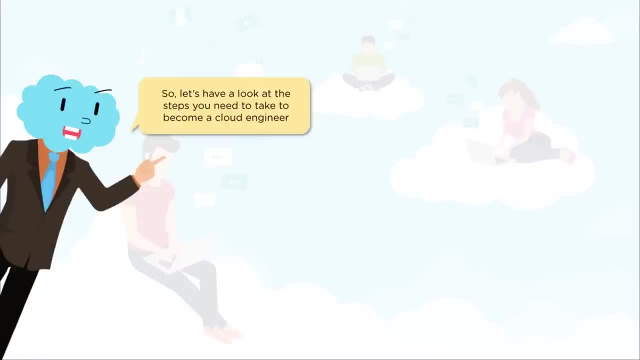 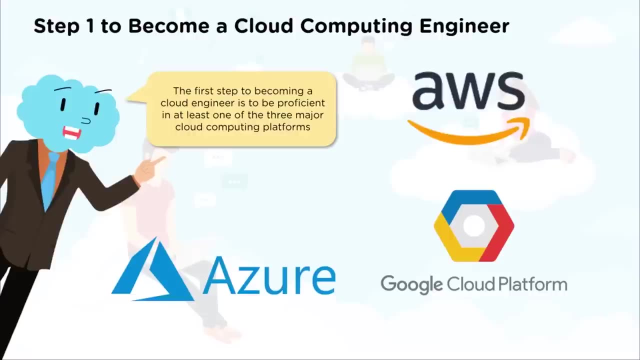 Now let's have a look at the steps you need to take to become a cloud computing engineer. Your first step is to gain proficiency in a cloud computing platform. Now the first step is to become proficient in at least one of the three major cloud computing platforms. 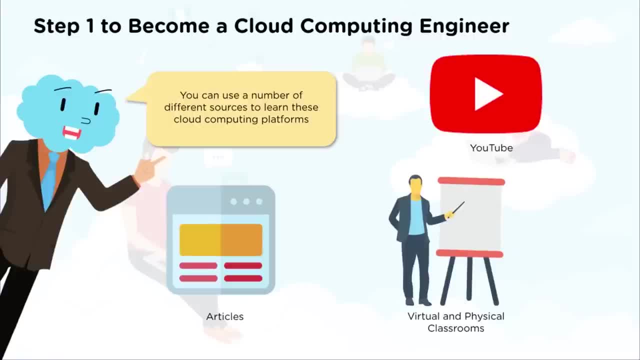 be it AWS, Azure or the Google Cloud Platform. Now there are a huge number of resources that you can find on the internet. It could be YouTube videos, articles, virtual or physical classrooms, and so much more. Now, after you're done learning, 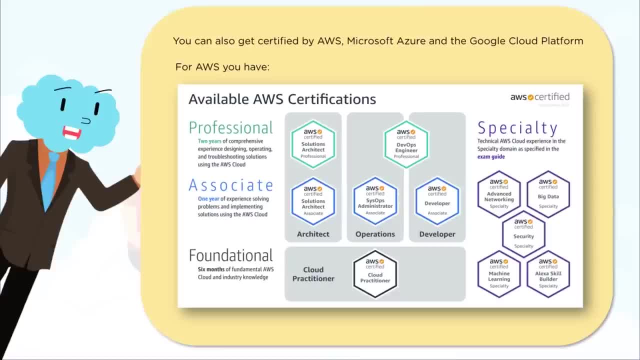 you can get certified by Microsoft Azure, AWS or the Google Cloud Platform. Now, for AWS, you have a number of different certifications, which can be divided into three categories, which are the foundational, which is just the basics. the associate level certifications. 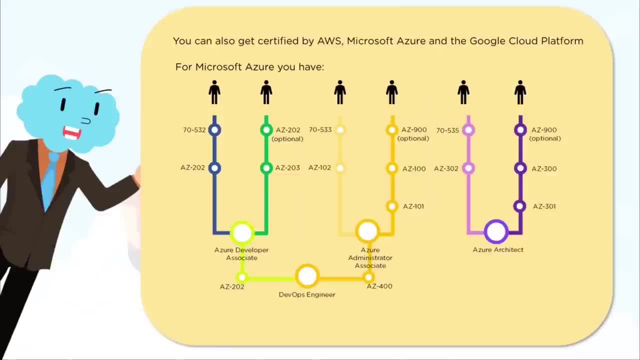 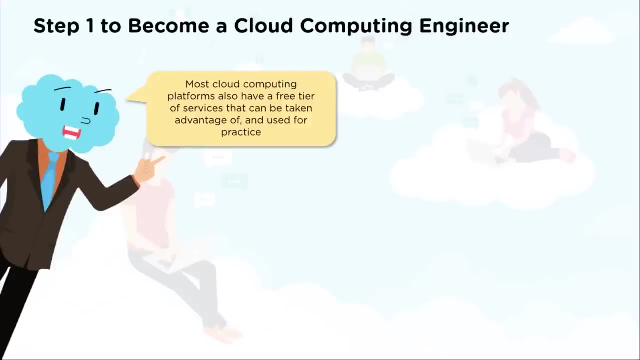 the professional level certifications and the specialty certifications. Similarly, with Microsoft Azure, you have certifications that enable you to become an Azure Developer Associate, an Azure Administrator Associate, an Azure Architect Professional and a DevOps Engineer. Now, most cloud computing platforms. 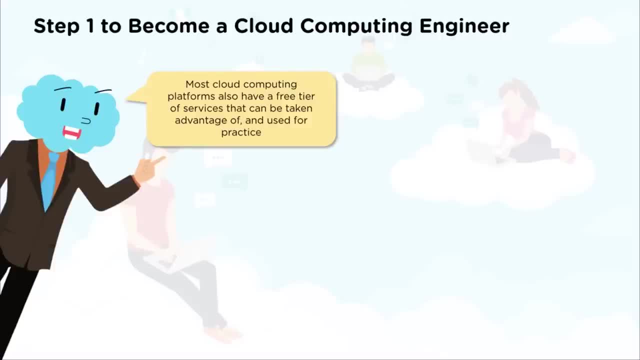 have a free tier that you can take advantage of. These provide a number of free services for a period of time, some of which are free forever. Use these platforms to your advantage and do as much practice as you can on them Now if you want to learn more about cloud computing. 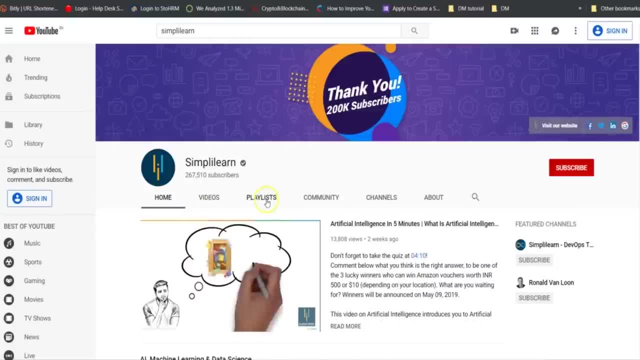 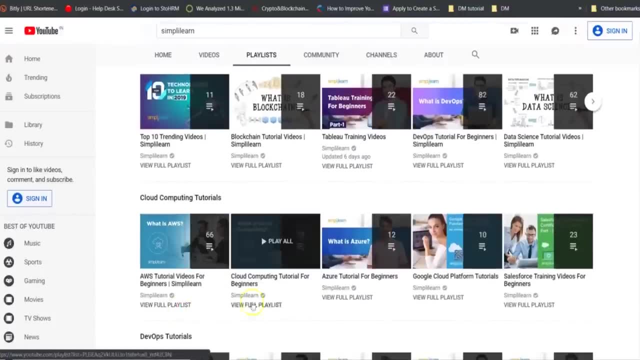 you can also check out Simply Learn's YouTube channel. Then you can go on to the playlist section right here and you can find comprehensive videos on a number of different cloud computing platforms: AWS and Microsoft Azure. Our AWS tutorial videos talk about what exactly is AWS. 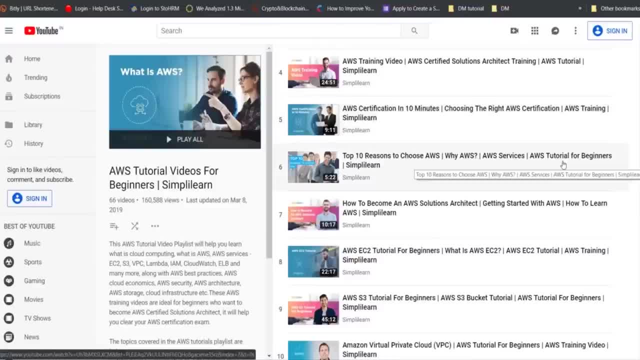 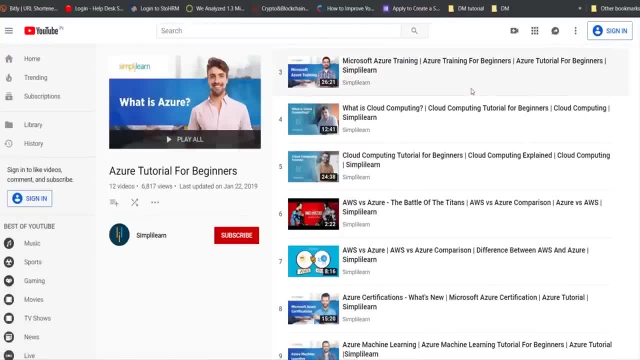 how you can become an AWS Solutions Architect, Amazon EC2, S3,, some of the other services and so much more. We also have detailed tutorials on Azure, which talks about what exactly is Azure, the certifications provided by Azure, some of the services like Machine Learning. 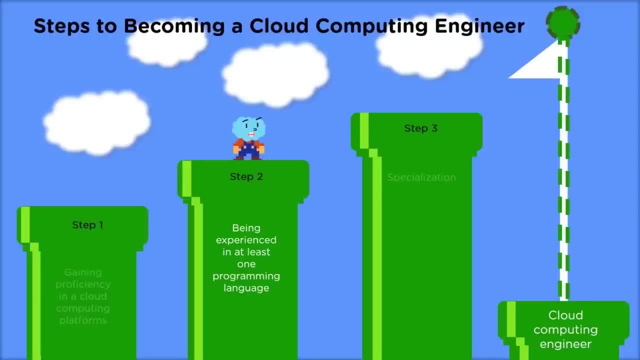 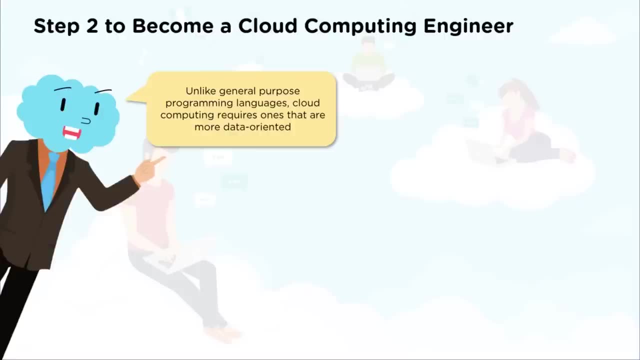 Azure, Active Directory and so much more. And now we're at step two, being experienced in at least one programming language. Unlike general purpose programming languages like C, C++, C, Sharp and so on, cloud computing requires ones that are a lot more data-oriented. 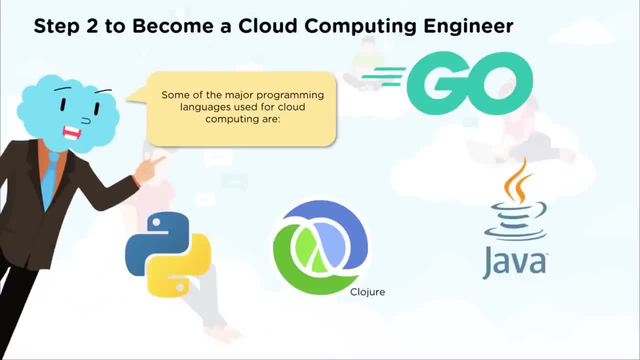 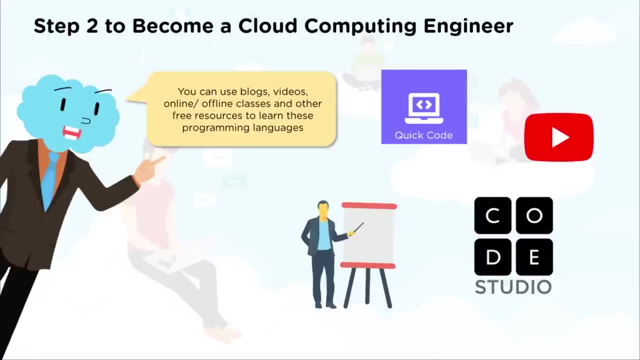 Now, some of the major programming languages that are used in cloud computing are Go, Python, Clojure and Java. Now, as I said before, there is a wealth of resources that you can learn from. There are free websites that you can practice your code on. 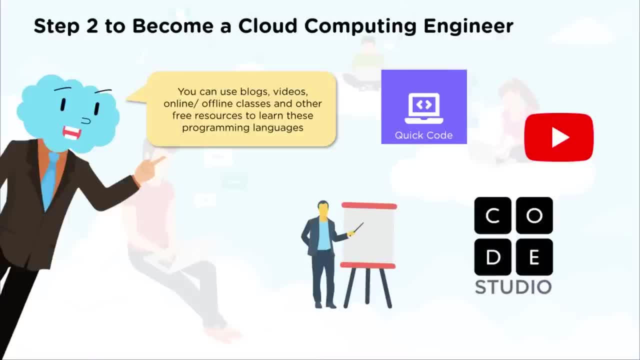 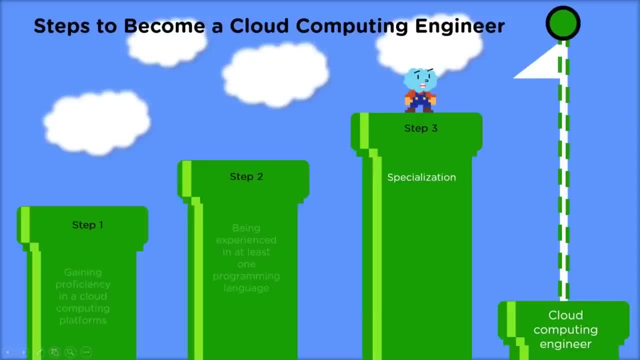 like Quick Code, Code Academy and several others. There's also resources like YouTube videos as well, as there's the option of online or offline classes. Now we're at step three, specialization. You'll also need to be well-versed with a number of key concepts. 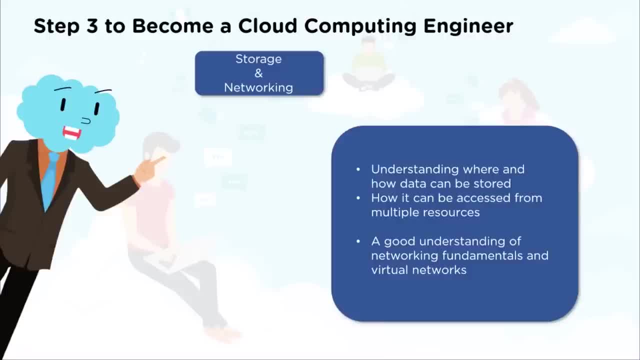 These are storage and networking. Now, with storage, you need to know how data can be stored and where it can be accessed from. You need to know how it can be accessed from multiple different resources. You'll also need to have some experience with the services provided by Azure and AWS. 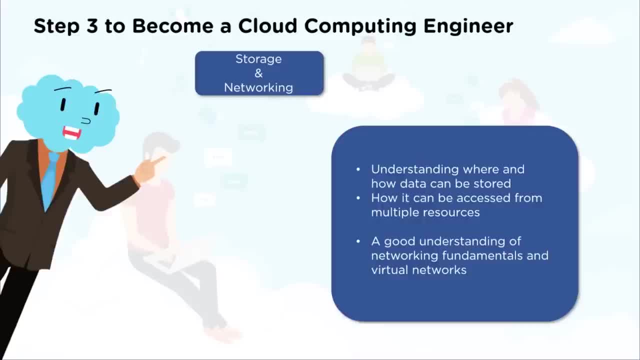 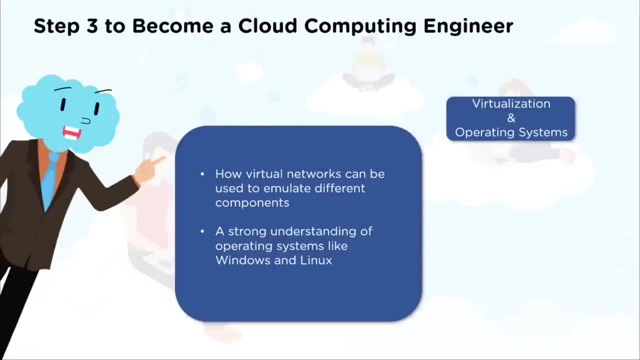 like the Amazon S3 in AWS and the appropriately named Azure Storage from Microsoft Azure. With networking, you need to have a strong understanding of the networking fundamentals, as well as virtual networks. Next up, we have virtualization and operating systems. With virtualization, you need to know how virtual networks 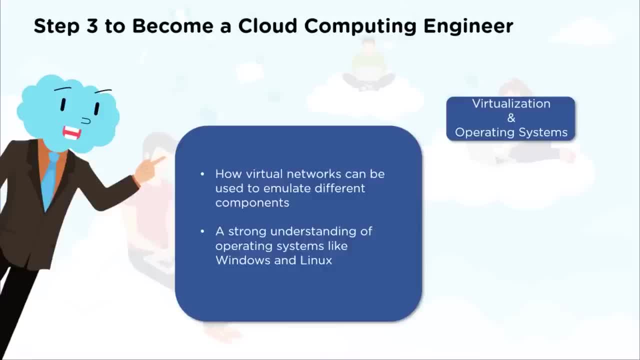 which are just a combination of different virtual machines, can be used to emulate different components in a particular system With operating systems. you need to have a very strong understanding of operating systems like Windows and Linux. Next up we have security and disaster recovery. 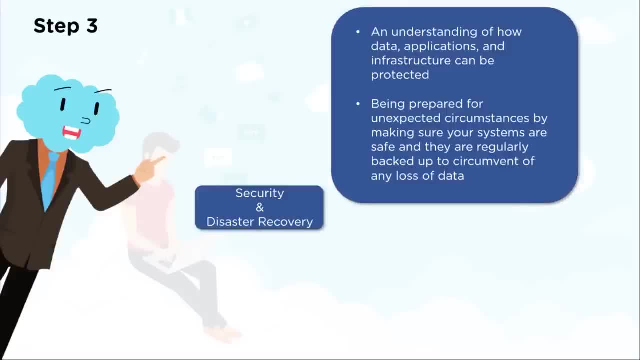 Now you need to understand how data application, as well as infrastructure, can be protected from malicious attacks. With disaster recovery, you need to be prepared for any unexpected circumstance by making sure your systems are always safe and are regularly backed up to prevent any sort of loss of data. 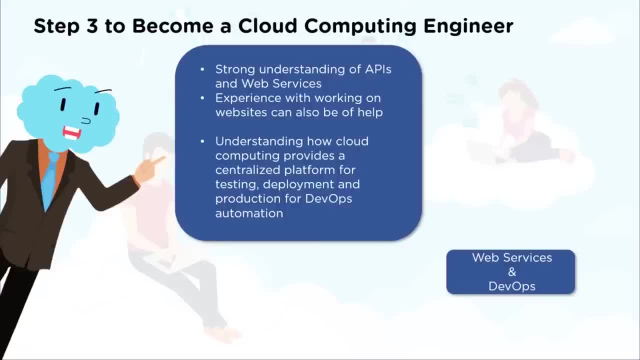 Then we have web services and DevOps. Now you need to have a strong understanding of APIs or application program interfaces and web services. Some amount of experience with web design also can be of great help. With DevOps, you need to have a strong understanding. 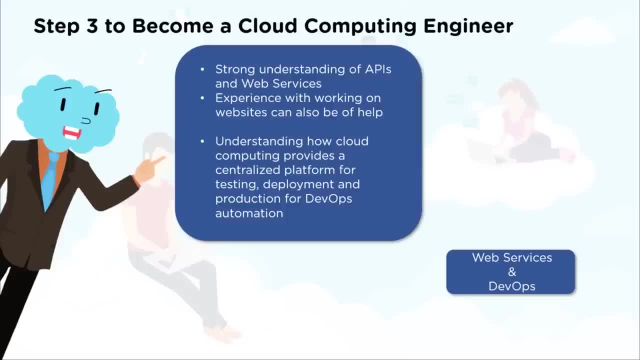 of how cloud computing is able to provide a centralized platform on which you can perform testing, deployment and production for DevOps automation. Moreover, with DevOps, you understand the synergy that the operations as well as the development teams have with each other and for the success of any project. 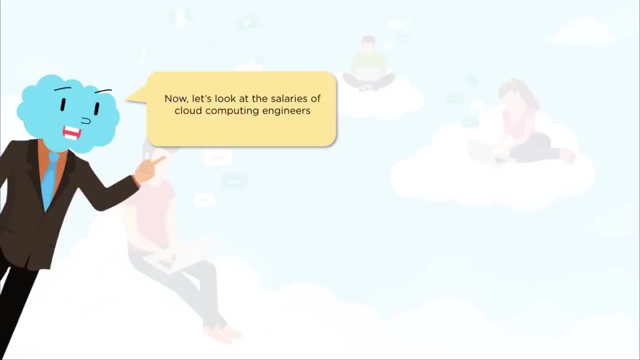 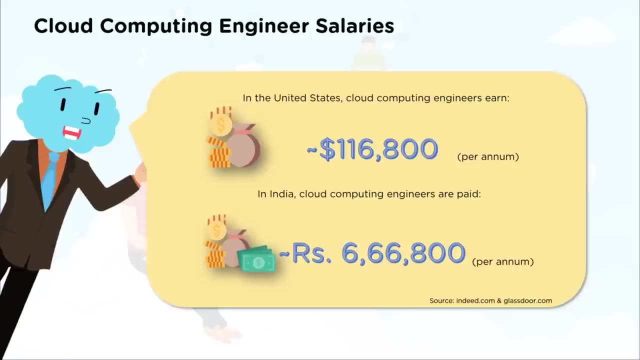 And finally, you're a cloud computing engineer. Now let's have a look at the salaries of cloud computing engineers. In the United States, cloud computing engineers earn around $116,000 per annum. In India, a cloud computing engineer is paid approximately 6,66,000 rupees per annum. 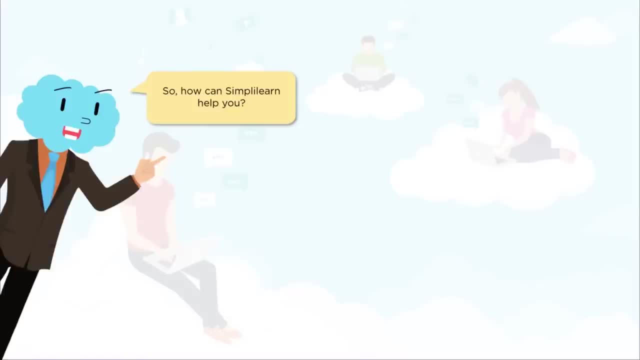 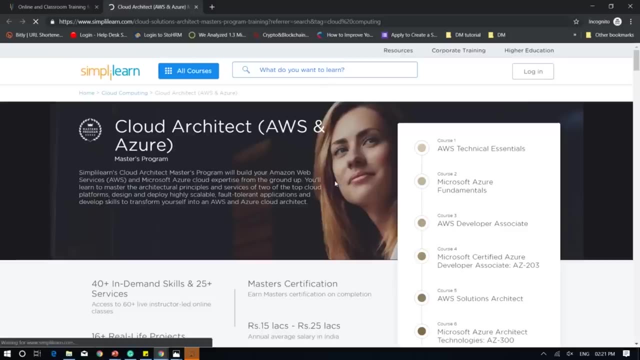 Now, how can Simply Learn help you become a cloud computer? So let's head on to Simply Learn's website. Here we have the Cloud Architect Master's program. Now this deals with a number of different courses, all of which can help you get started in your journey. 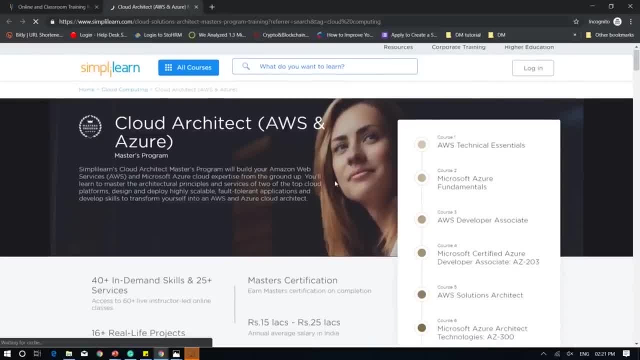 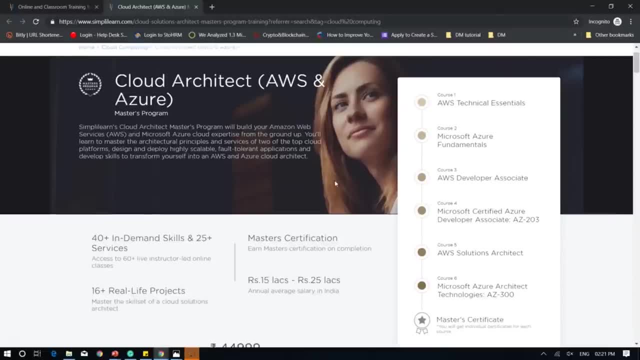 to becoming a cloud computing engineer. This master's program covers a number of different courses like AWS Technical Essentials, Microsoft Azure Fundamentals, AWS Developer Associate and so much more. It provides you 40-plus in-demand skills and 25-plus services. 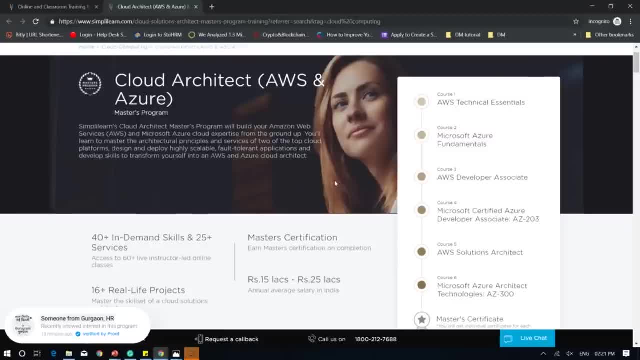 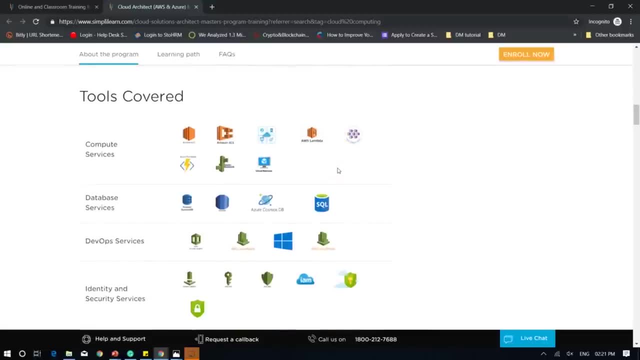 provides you a master's certification, it has 16-plus real-life projects and helps you get a salary that ranges between 15 to 25 lakh rupees per annum. It also covers a variety of tools like Amazon EC2, Azure Data Factory, virtual machines and so much more. 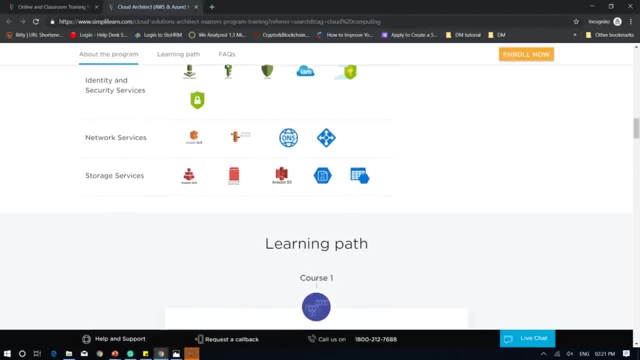 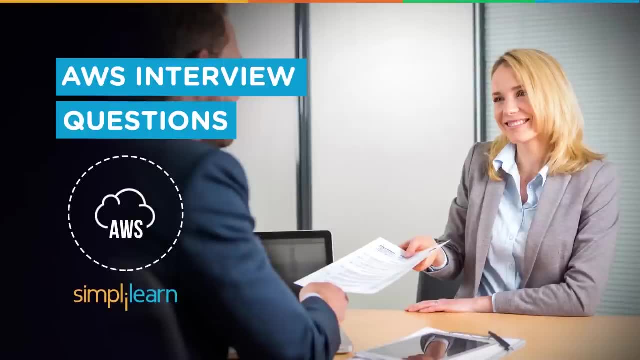 So why don't you head on to simplylearncom and get started on your journey to getting certified and getting ahead? I'm here to walk you through some of the AWS interview questions which we find are important, And our hope is that you would use this material in your interview preparation. 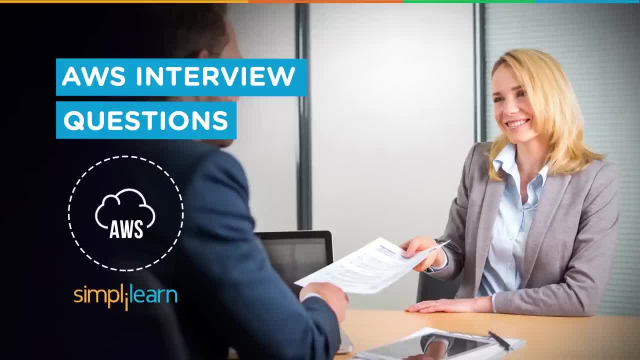 and be able to crack that cloud interview and step into your dream cloud job. By the way, I'm a cloud technical architect trainer and an interview panelist for cloud network and DevOps, So as you progress in watching, you're going to see that these questions are practical, scenario-based questions. 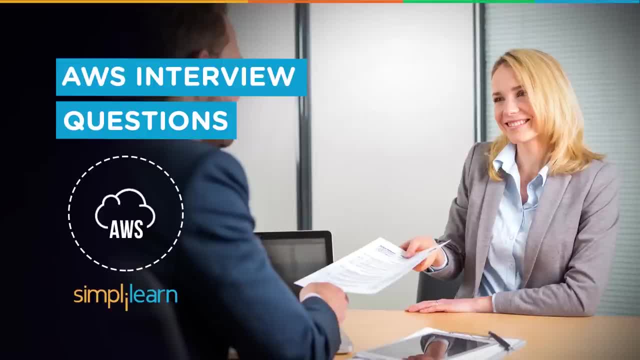 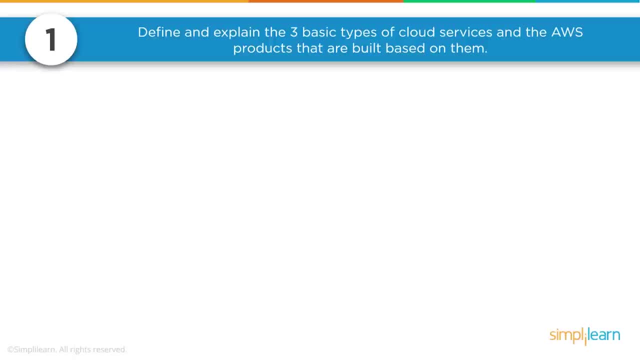 that test the depth of the knowledge of a person in a particular AWS product or in a particular AWS architecture. Why wait, Let's move on. So in an interview, you would find yourself with a question that might ask you, define and explain the three basic types of cloud services. 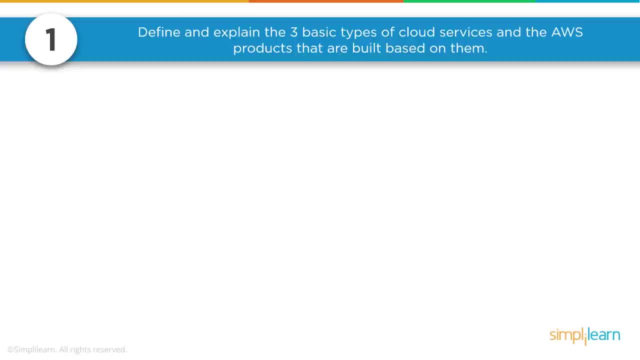 and the AWS products that are built based on them. See here, it's a very straightforward question. Just explain three basic types of cloud service, And when we talk about basic type of cloud service, it's compute. obviously that's a very basic service. 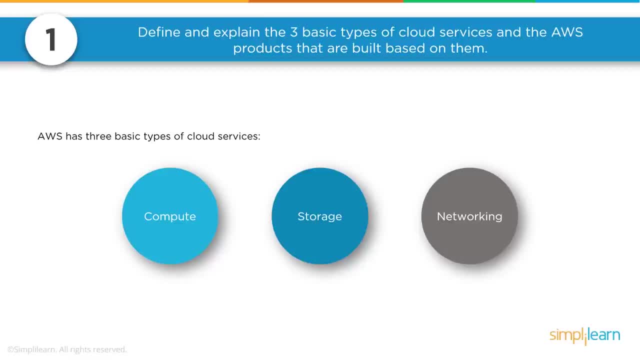 storage- obviously because you need to store your data somewhere, and networking, that actually connects a couple of other services to your application. These basic will not include monitoring. These basic will not include analytics, because they are considered as optional. They are considered as advanced services. 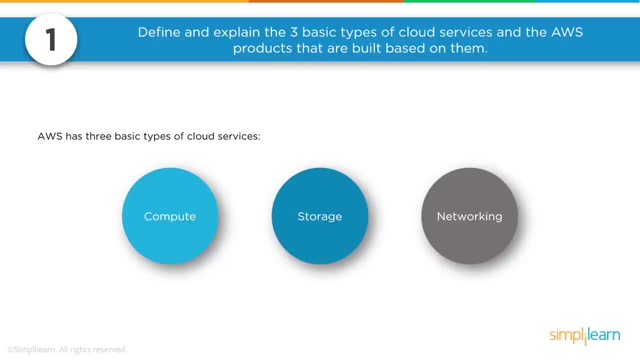 You could choose a non-cloud service or a product for monitoring and for analytics, So they're not considered as basic. So when we talk about basics, they are compute, storage and networking. And the second part of the question says: 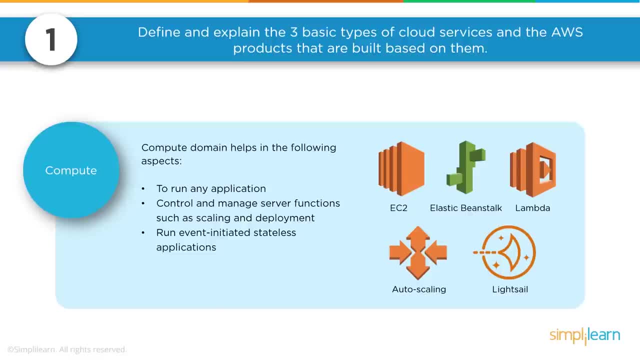 explain some of the AWS products that are built based on them. Of course, compute EC2 is a major one. That's the major share of the compute resource. And then we have platform as a service, which is Elastic Beanstalk, And then function as a service, which is Lambda. 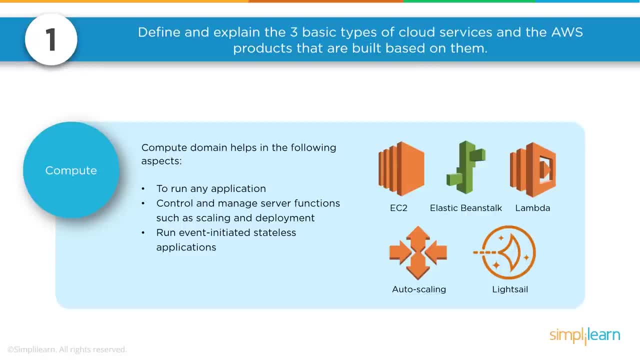 Autoscaling and LightSail are also part of compute services. So the compute domain, it really helps us to run any application And the compute service helps us in managing the scaling and deployment of an application. Again, Lambda is a compute service. 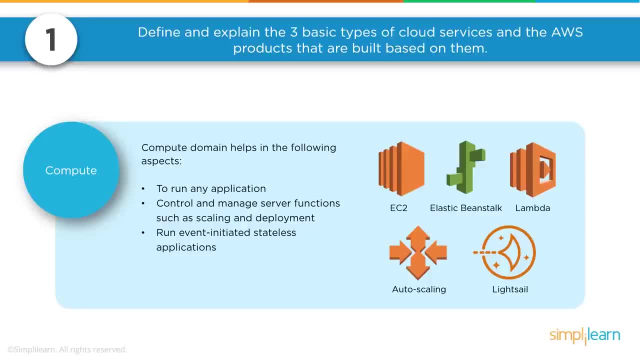 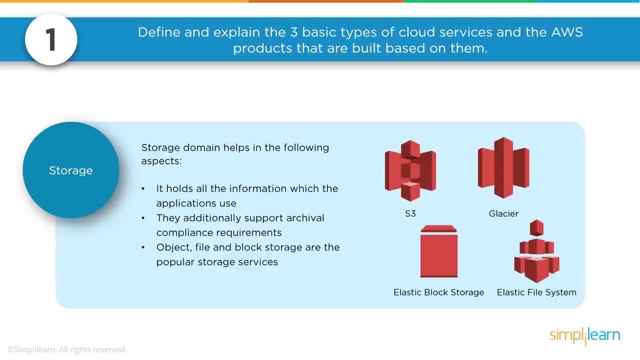 So the compute service also helps in running event-initiated stateless applications. The next one was storage. A lot of emphasis is on storage these days, because if there's one thing that grows in a network on a daily basis, that's storage. 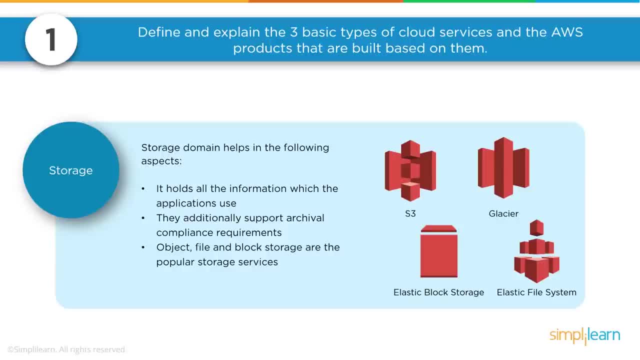 Every new day we have new data to store, process manage. So storage is again a basic and an important cloud service, And the products that are built based on the storage services are S3, object storage- Glacier for archiving. 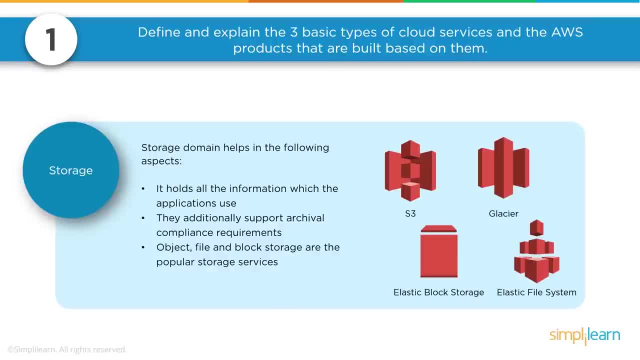 EBS elastic block storage as a drive attachment for the EC2 instances And EFS file share for the EC2 instances. So the storage domain helps in the following aspects: It holds all the information that the application uses. It holds all the application data. 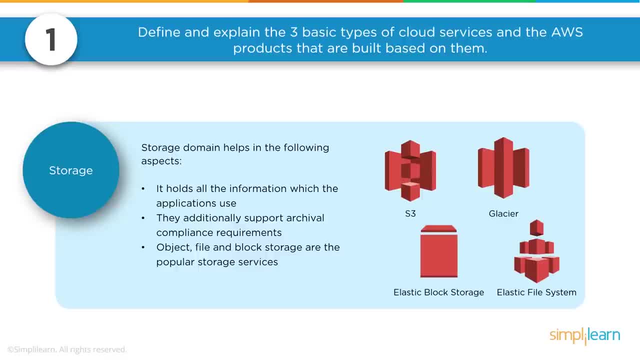 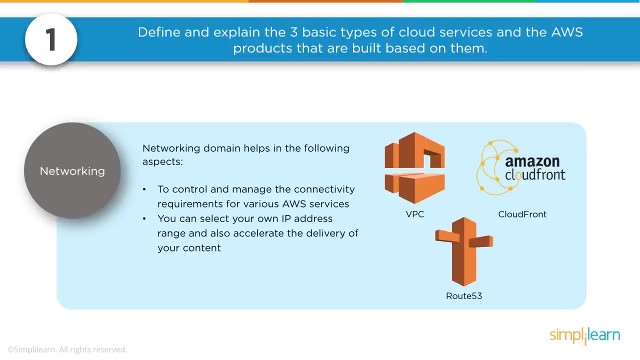 And we can also archive old data using storage which would be Glacier, And any object files and any requirement for block storage can be met through elastic block store and S3, which is again an object storage. Talking about networks, it's just not important to answer the question with the name of the services. 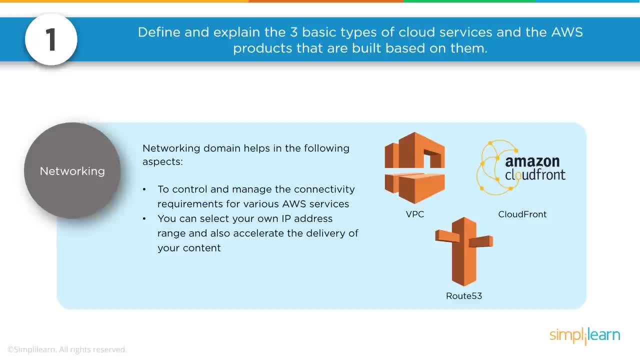 and the name of the product. It'll also be good if you could go in depth and explain how they can be used, So that actually proves you to be a person knowledgeable enough in that particular service or product. So, talking about networking domain, VPC networking- 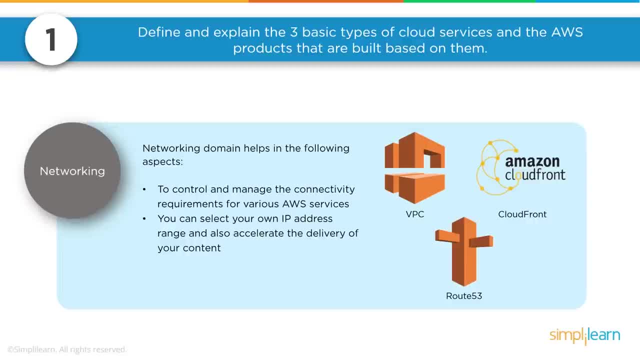 Can't imagine networking without VPC in a cloud environment, especially in AWS cloud environment. And then we have Route 53 for domain resolution or for DNS. And then we have CloudFront, which is an edge caching service That helps customers get or customers to read their application with low latency. 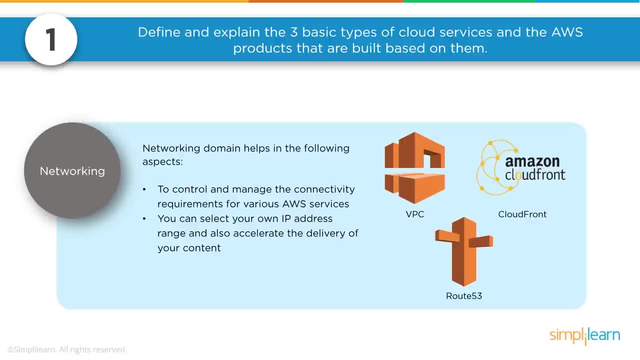 So networking domain helps with some of the following use cases. It controls and manages the connectivity of the AWS services within our account And we can also pick an IP address range If you're a network engineer or if you are somebody who works in networks or are planning to work in network. 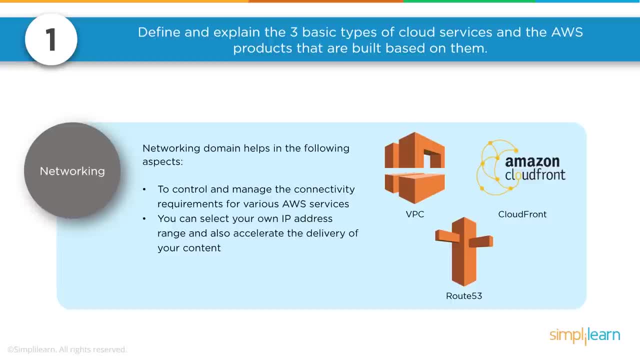 you will soon realize the importance of choosing your own IP address range For easy remembering. So having an option to have your own IP address in the cloud, own range of IP address in the cloud, it really helps, really really helps in cloud networking. 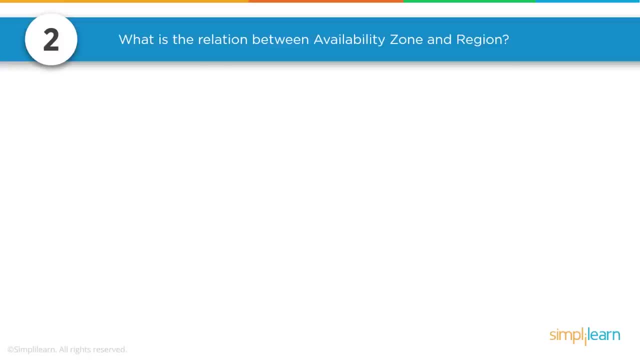 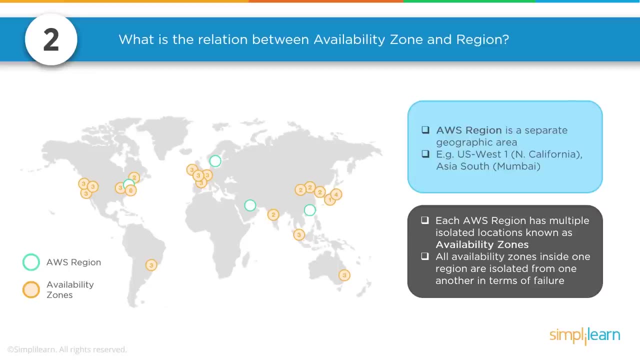 The other question that gets asked would be the difference between the availability zone and the region. Actually, the question generally gets asked to test how well you can actually differentiate and also correlate the availability zone and the region relationship. So a region is a separate geographic area, like the US to S1,. 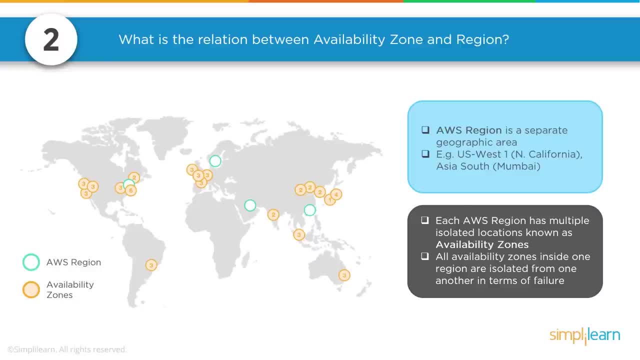 which represents North California, or the AP South, which represents Mumbai. So regions are a separate geographic area. On the contrary, availability zone resides inside the region. You shouldn't stop there. You should go further and explain about availability zones, And availability zones are isolated from each other. 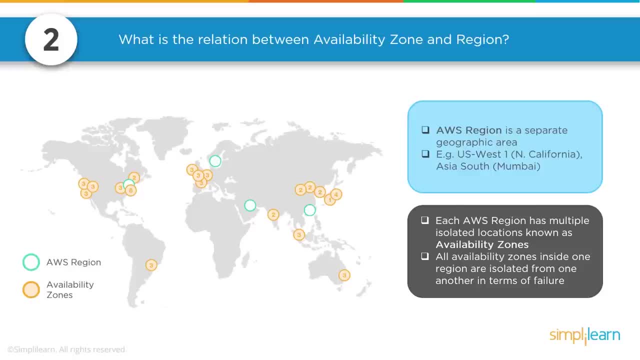 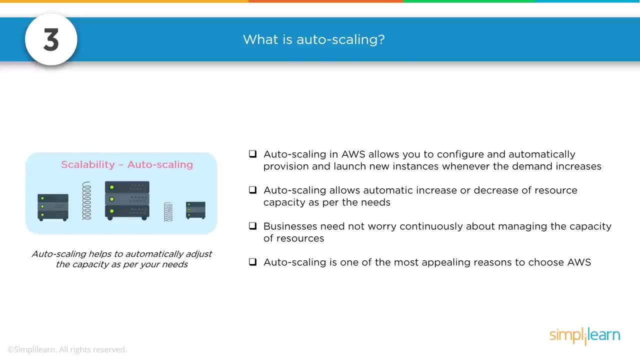 And some of the services will replicate themselves within the availability zone. So availability zone does replication within them, but regions- they don't generally do replication between them. The other question you could be asked is: what is auto scaling? What do we achieve by auto scaling? 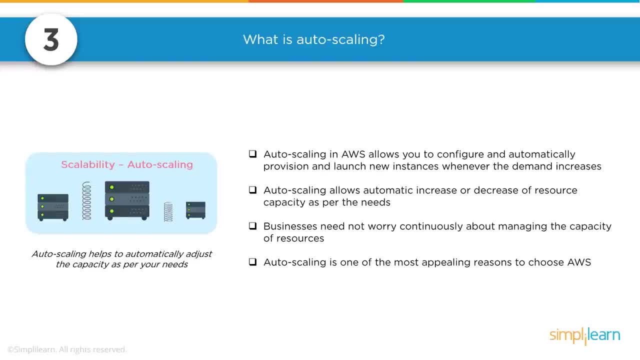 So, in short, auto scaling. it helps us to automatically provision and launch new instances whenever there is a demand. It not only helps us meeting the increasing demand, it also helps in reducing the resource usage when there is low demand. So auto scaling also allows us to decrease the resources. 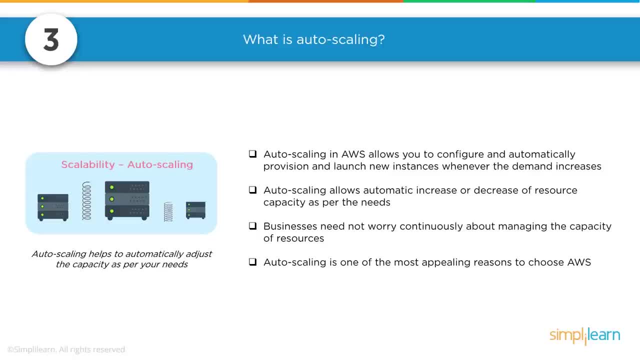 or resource capacity as per the need of that particular arc. Now, this helps business in not worrying about putting more effort in managing or continuously monitoring the server to see if they have the needed resources or not, because auto scaling is going to handle it for us. 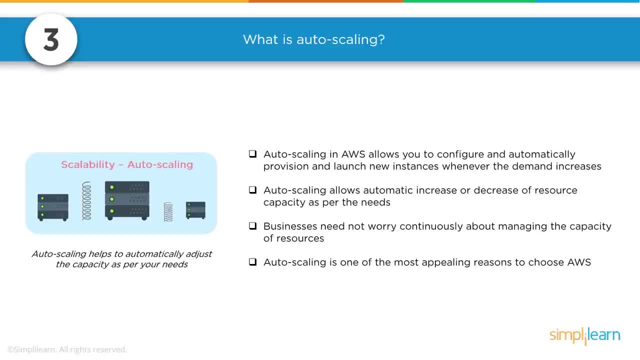 So business does not need to worry about it. And auto scaling is one big reason why people would want to go and pick a cloud service, especially an AWS service. The ability to increase and shrink based on the need of that arc- That's how powerful is auto scaling. 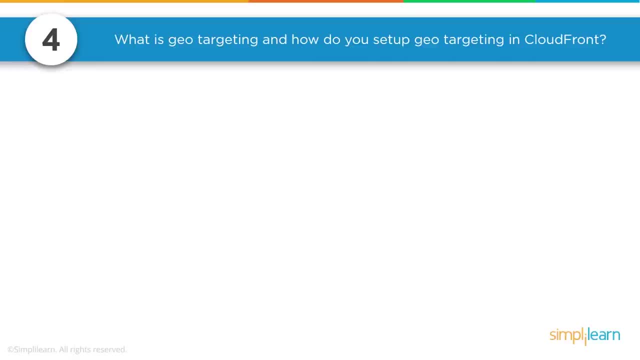 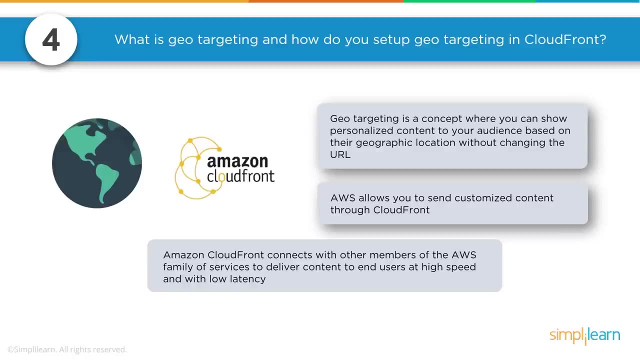 The other question you could get asked is: what's geo-targeting in CloudFront? Now we know that CloudFront is caching and it caches content globally in the Amazon caching servers global wide. The whole point is to provide users worldwide access to the data. 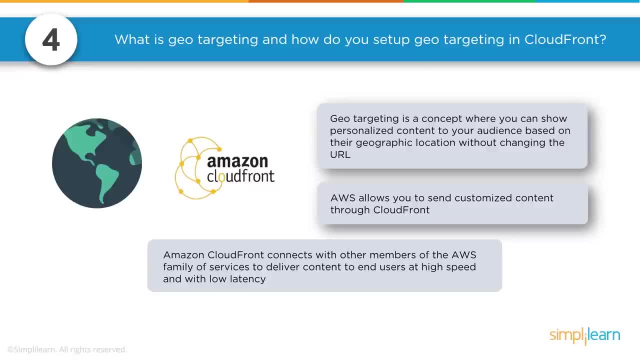 from a very nearest server possible. That's the whole point in using or going for CloudFront. Then what do you mean by geo-targeting? Geo-targeting is showing customer and specific content Based on language. we can customize the content. 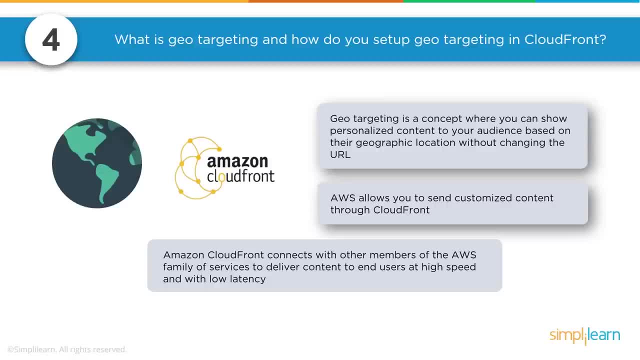 Based on what's popular in that place. we can actually customize the content. The URL is the same, but we could actually change the content a little bit. Not the whole content, otherwise it would be dynamic, but we can change the content a little bit. 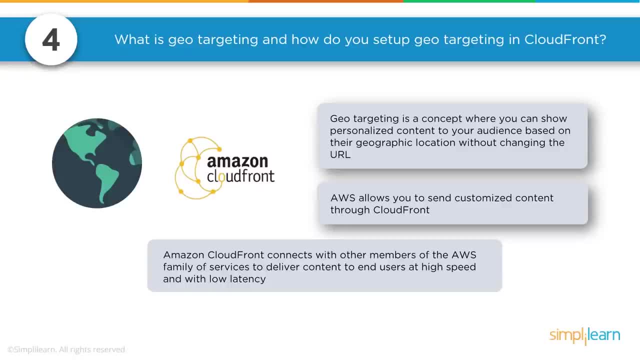 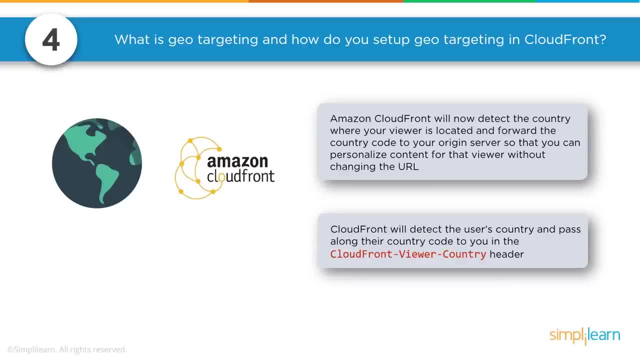 a specific file or a picture or a particular link in a website and show customized content to users who will be in different parts of the globe. So how does it happen? CloudFront will detect the country where the viewers are located and it will forward the country code. 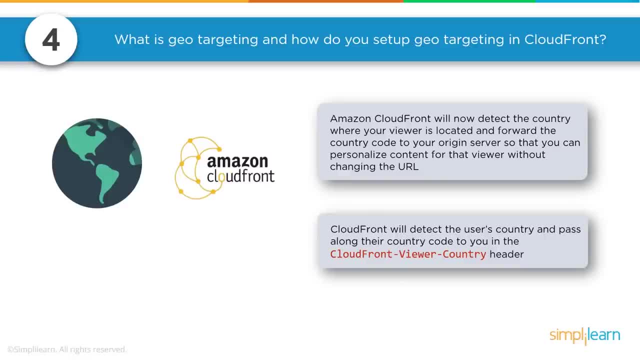 to the origin server. Once the origin server gets the specialized or specific country code, it will change the content and it will send to the caching server and it gets cached there forever. The user gets to view a content which is personalized for them for the country they are in. 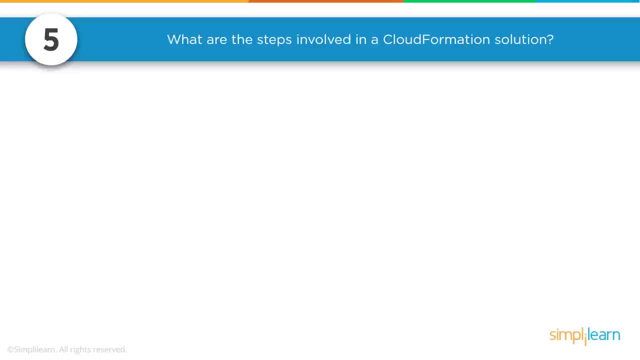 The other question you could get asked is the steps involved in using CloudFormation or creating a CloudFormation or backing up an environment with a CloudFormation template. We all know that if there is a template, we can simply run it and it provisions the environment. 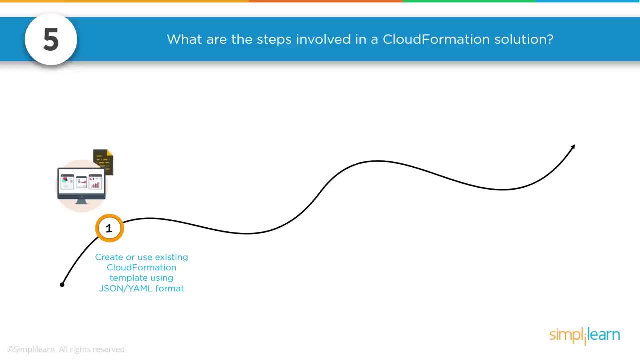 but there is a lot more going into it. So the first step in moving towards infrastructure as a code is to create the CloudFormation template, which, as of now, supports JSON and YAML file format. So first create the CloudFormation template and then save the code in an S3 bucket. 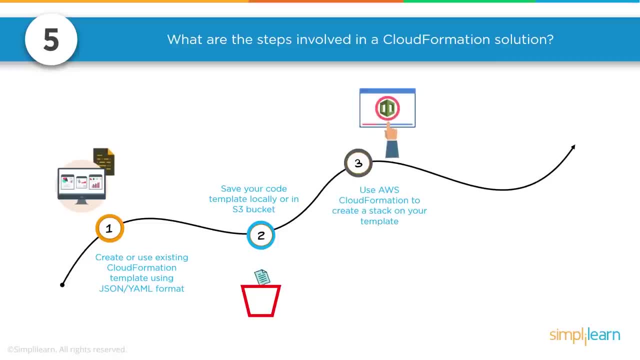 S3 bucket serves as the repository for our code and then, from the CloudFormation, call the file in the S3 bucket and create a stack. And now CloudFormation uses the file, reads the file, understands services that are being called, understands the order. 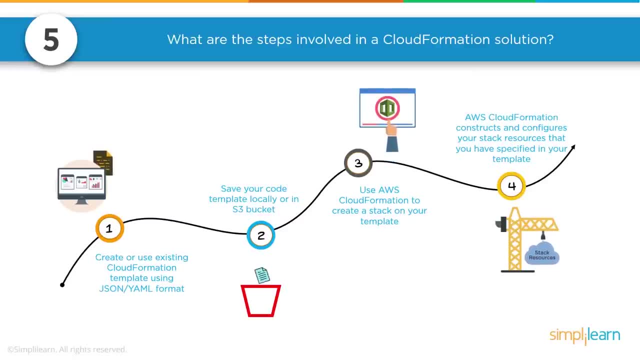 understands how they are connected with each other. CloudFormation is actually an intelligent service. It understands the relation based on the code. It would understand the relationship between the different services and it would set an order for itself And then would provision the services, one after the other. 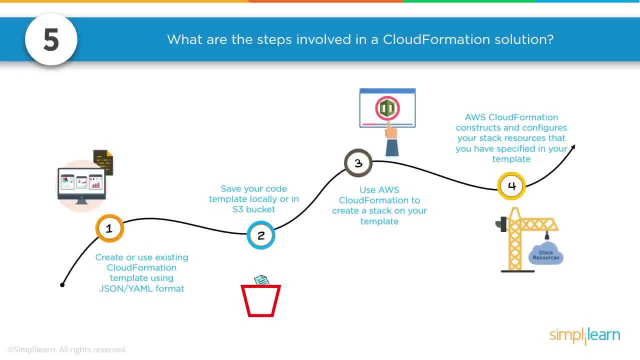 Let's say, a service has a dependency and the dependent service the other service, which this service, let's say service A and B. Service B is dependent on service A. let's say, CloudFormation is an intelligent service. It would provision the resource A first. 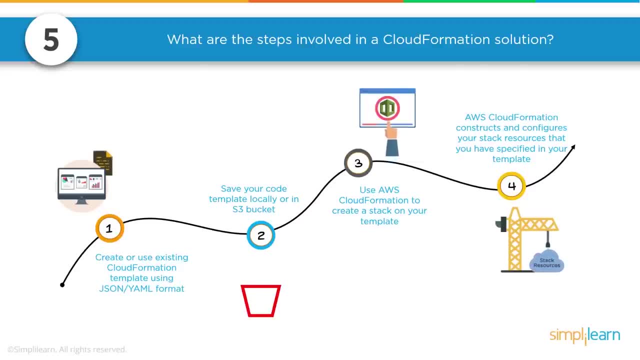 and then would provision resource B. What happens if we inverse the order? If we inverse the order, resource B first gets provision and because it does not have dependency, the CloudFormation's default behavior is that if something is not provisioned properly, if something is not healthy, it would roll back. 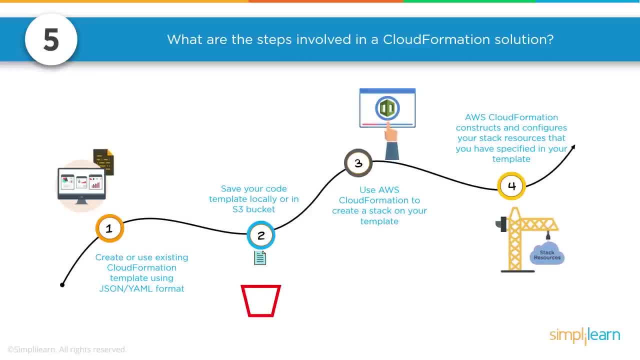 Chances that the environment provisioning will roll back. So to avoid that, CloudFormation first provisions all the services that has or that's dependent on, that's dependent by another service, So it provisions those services first and then provisions the services that has dependencies. 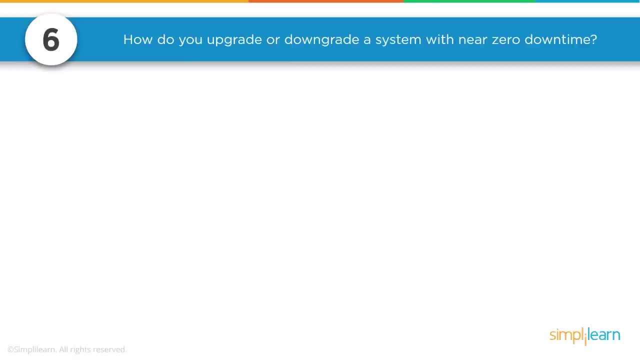 And if you are being hired for a DevOps, or if the interviewer wanted to test your skill on systems side, this definitely would be a question in his list. How do you upgrade or downgrade a system with near zero downtime? Now everybody's moving towards zero downtime. 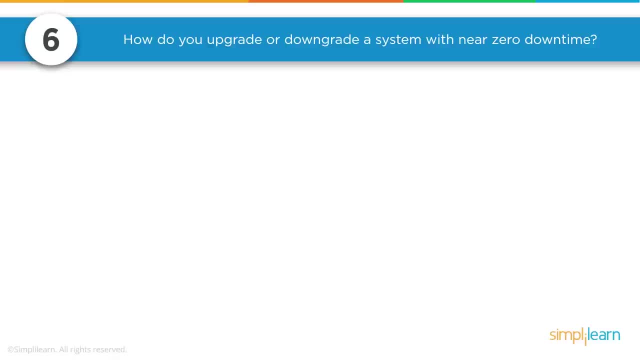 or near zero downtime. All of them want their application to be highly available. So the question would be: how do you actually upgrade or downgrade a system with near zero downtime? Now I don't know that I can upgrade an EC2 instance to a better EC2 instance by changing the instance type. 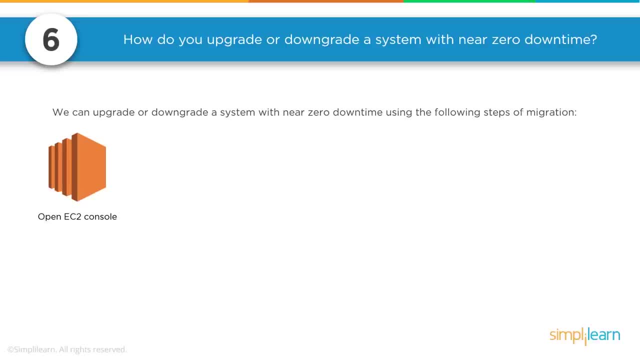 stopping and starting, But stopping and starting is going to cause a downtime, right? So that's you shouldn't be answering or you shouldn't be thinking in those terms, because that's wrong answer. Specifically, the interviewer wants to know how do you upgrade a system with zero downtime? 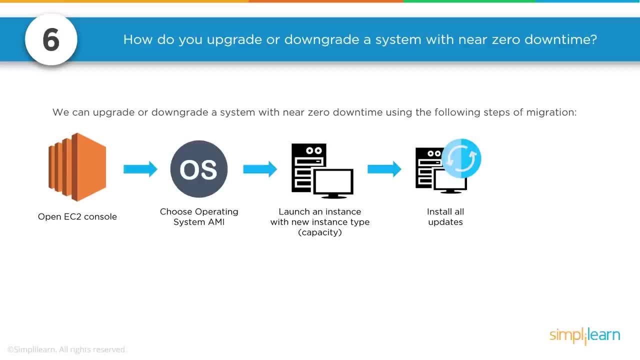 So upgrading system with zero downtime. it includes launching another system paralleling with the bigger EC2 instance type over the bigger capacity and install all that's needed. If you are going to use an AMI of the old machine, well and good, you don't have to go through. 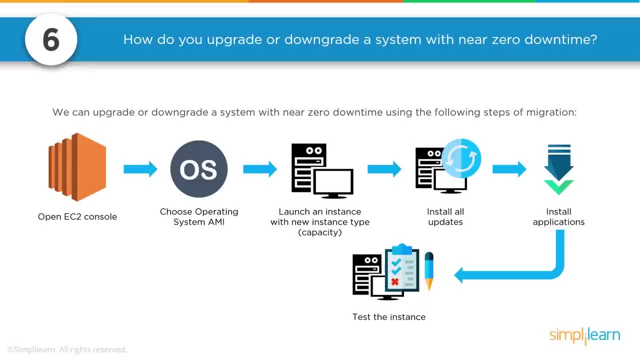 installing all the updates and installing all the application From the AMI. once you've launched it in a bigger instance, locally test the application to see if it is working. Don't put it on production yet. Test the application to see if it is working. 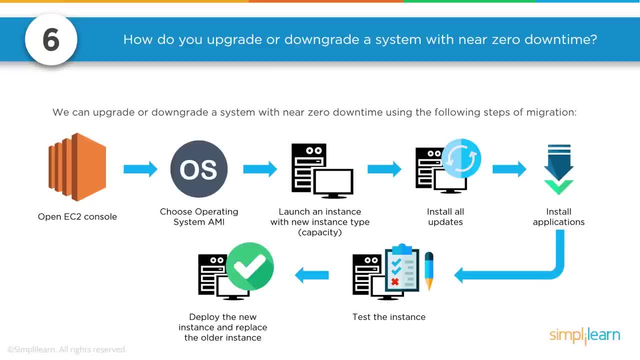 And if the application works, we can actually swap. If you are starting, if your server is behind, and behind Route 53, let's say all that you could do is go to Route 53, update the information with the new IP address. 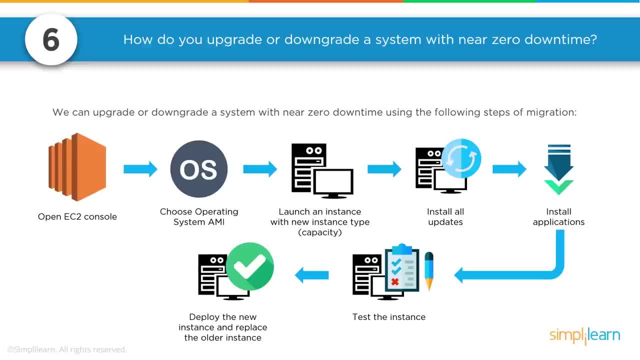 new IP address of the new server and that's going to send traffic to the new server now. So the cutover is handled. Or, if you're using static IP, you can actually remove the static IP from the old machine and assign it to the new machine. 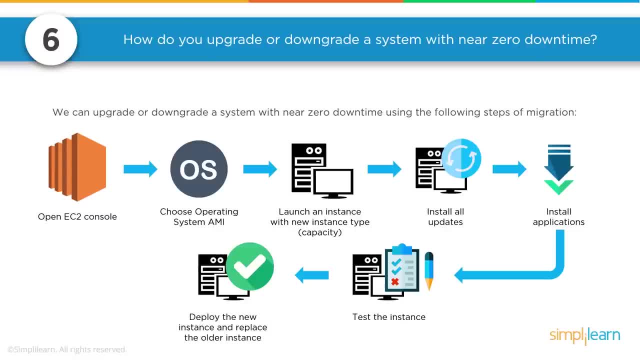 That's one way of doing it. Or if you are using elastic NIC card, you can actually remove the NIC card from the old machine and attach the NIC card to the new machine. So that way we would get near zero downtime. If you're hired for an architect level, 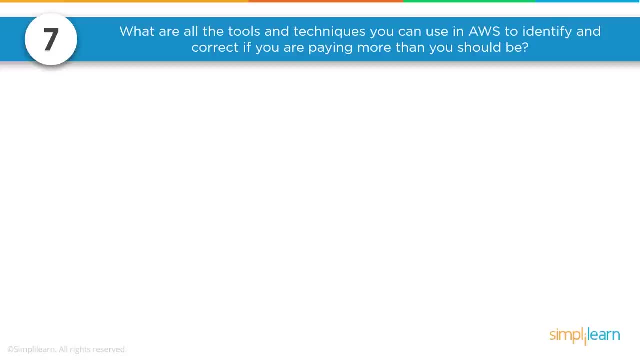 you should be worrying about cost as well, along with the technology, And this question would test how well you manage cost. So what are the tools and techniques we can use in AWS to identify and correct? identify and know that we are paying the correct amount? 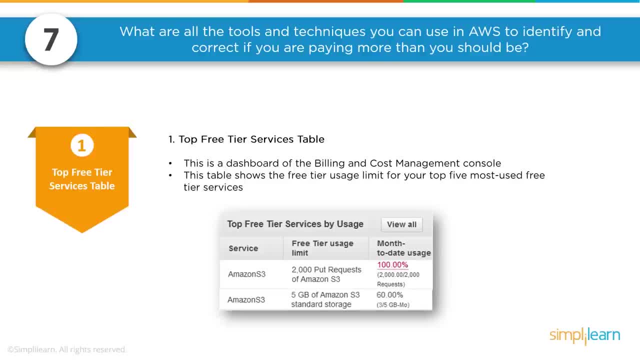 for the resources that we are using, Or how do you get visibility of your AWS resources running? One way is to check the billing. There's a place where you can check the top services that were utilized. It could be free and it could be paid service as well. 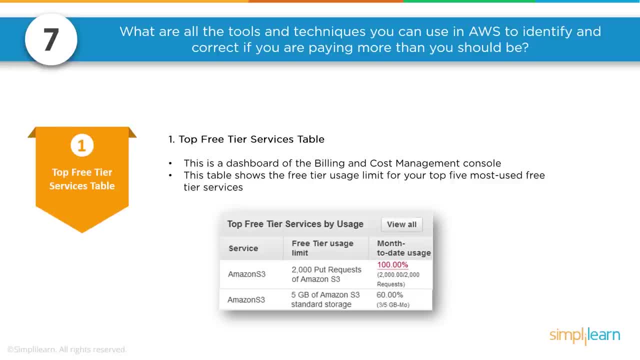 Top services that can be utilized. It's actually in the dashboard of the cost management console, So that table here shows the top five most used services. so looking at it, you can get it All right. so I'm using a lot of storage. 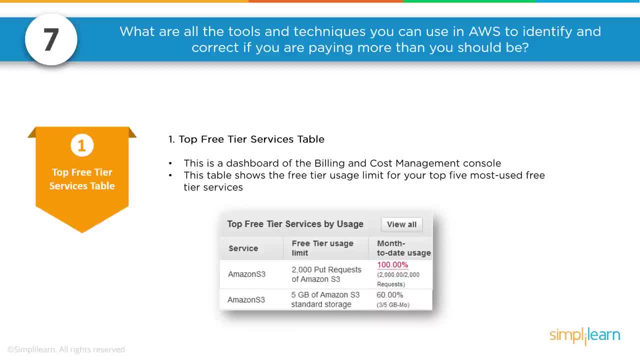 I'm using a lot of EC2.. Why is storage high? You can go and try to justify that and you will find if you are storing things that shouldn't be storing and then clean it up. Why is compute capacity so high? Why is data transfer so high? 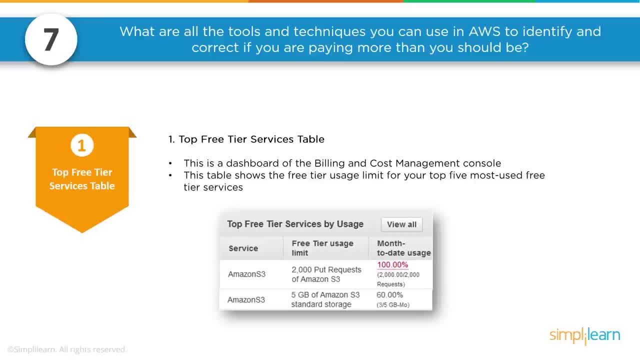 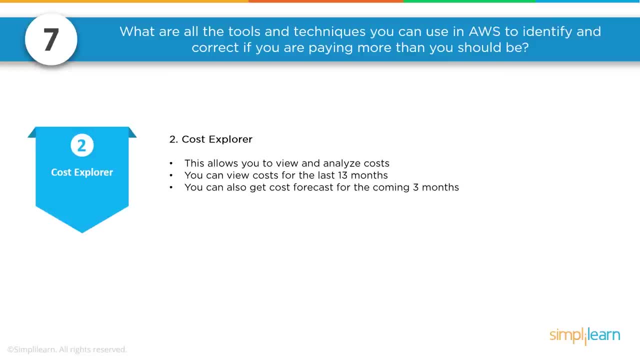 So if you start thinking in those levels, you'll be able to dig in and clean up unnecessary and be able to save your bill. And there are cost explorer services available which will help you to view your usage pattern or view your spending for the past 13 months or so. 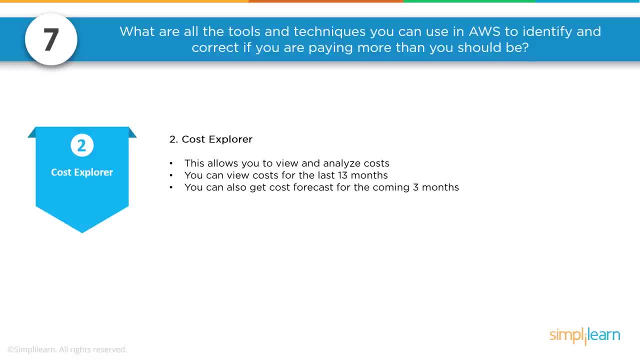 And it will also forecast for the next three months. Now, how much will you be using if your pattern is like this? That will actually help and will give you a visibility on how much you have spent. how much you will be spending if the trend continues. 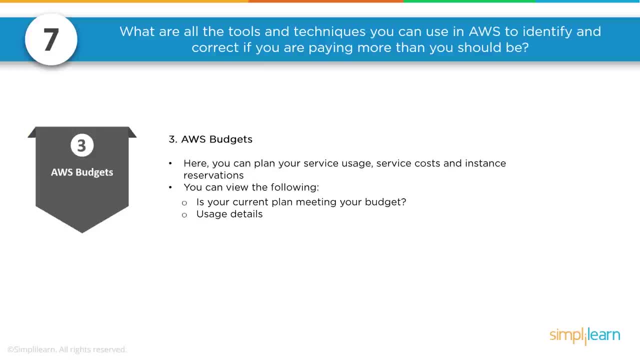 Budgets are another excellent way to control cost. You can actually set a budget: That's how much I am willing to spend for this application, for this team, or for this month for this particular resource. So you can actually put a budget mark. 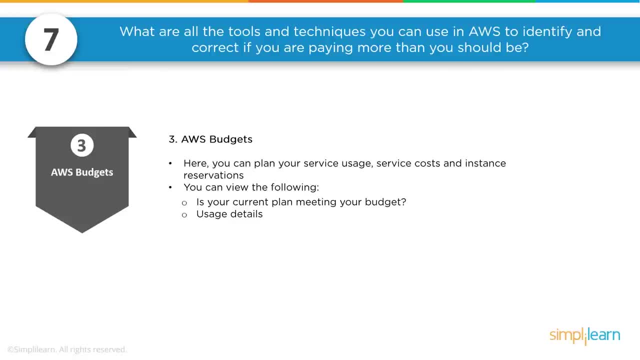 and anytime it exceeds, anytime it's nearing, you would get an alarm saying that well, we're about to reach the allocated budget amount, stuff like that. That way you can go back and know, and you know that, how much the bill is going to be for that month. 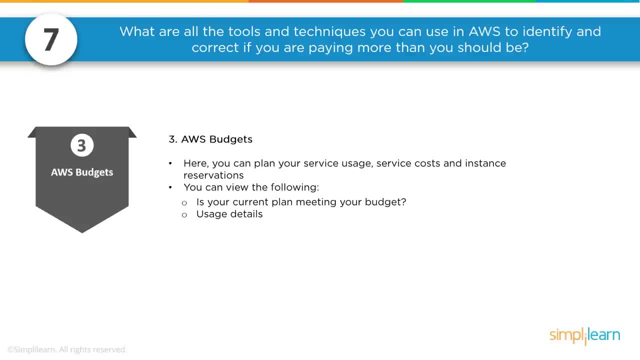 or you can take steps to control bill amount for that particular month. So this budget is another very good tool that you could use. Cost allocation tags helps in identifying which team or which resource has spent more in that particular month, Instead of looking at the bill as one list. 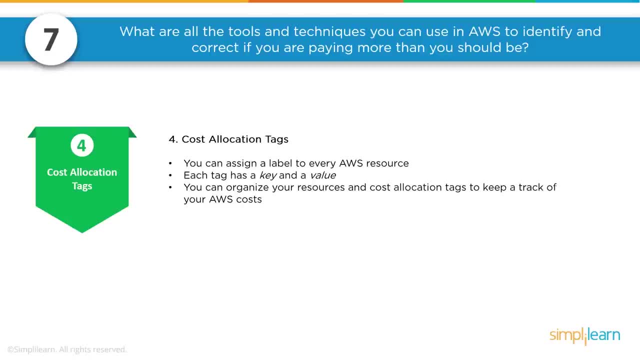 with no specifications into it and, looking at it as an expenditure list, you can actually break it down and tag the expenditure to the teams with cost allocation tags. The dev team has spent so much. The production team has spent so much. The training team has spent more. 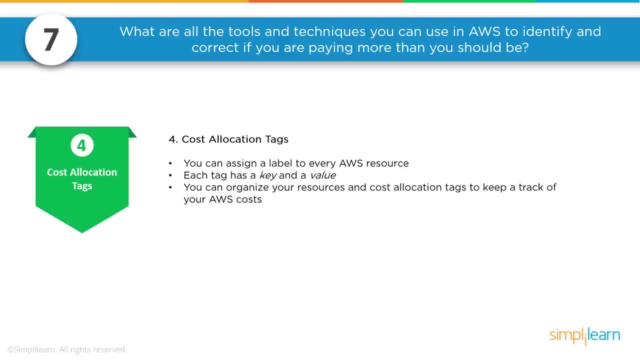 than the dev and the production team. Why is that? You'll be able to think in those levels only if you have cost allocation tags. Now, cost allocation tags are nothing but the tags that you would put when you create a resource, So for production services. 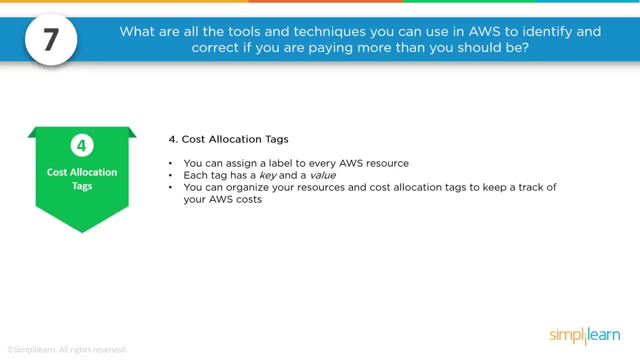 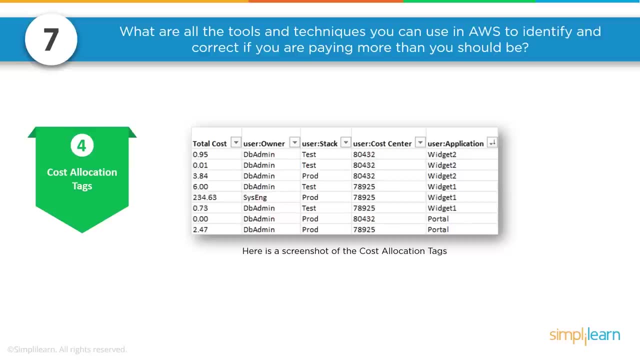 you would create a production tag and you would associate that resources to it And at a later point, when you actually pull up your bill, that's going to show a detailed list of: this is the owner, this is the group and this is how much they have used in the last month. 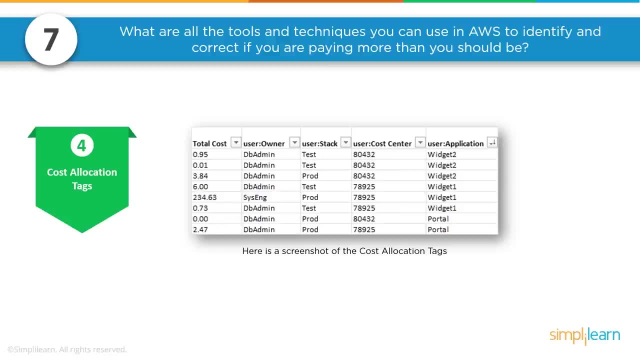 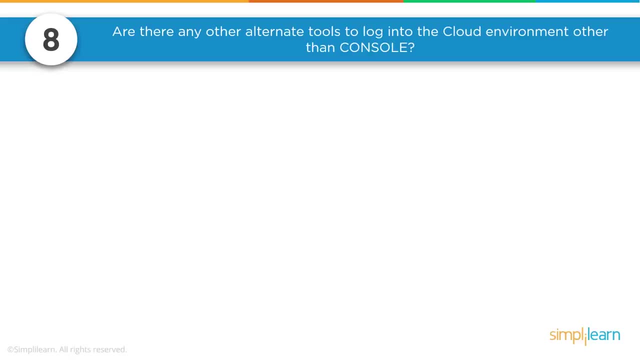 And you can move forward with your investigation and encourage or stop users using more services with the cost allocation tags. The other famous question is: are there any other tools or is there any other way of accessing AWS resource other than the console Console? is GUI right? 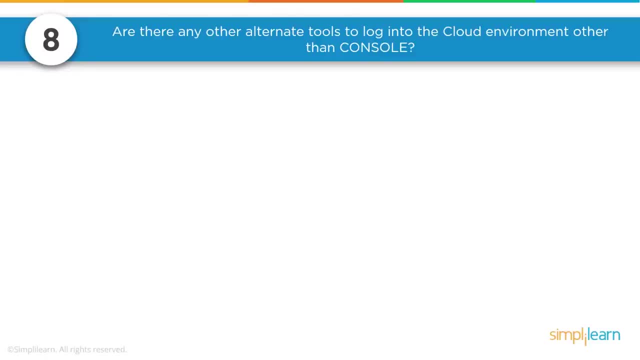 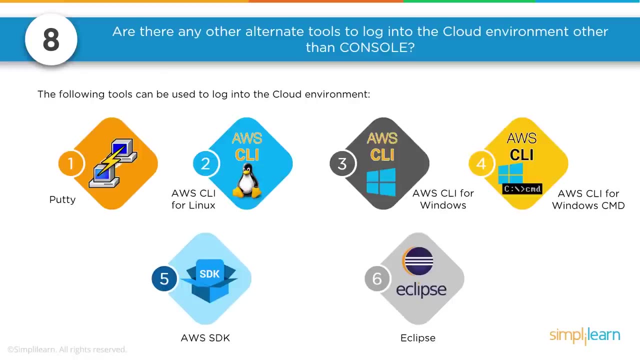 So, in other words, other than GUI, how would you use the AWS resource and how familiar are you with those tools and technologies? The other tools that are available that we can leverage and access the AWS resource are, of course, PuTTY. You can configure PuTTY to access the AWS resources. 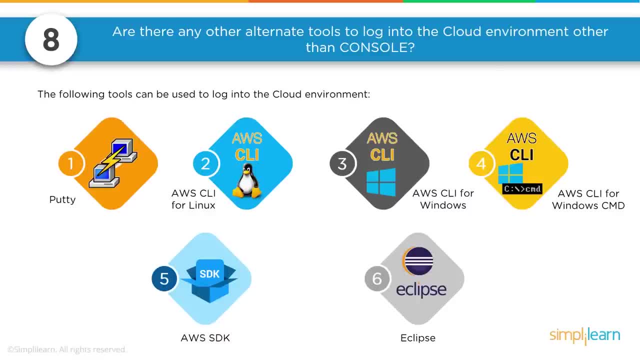 like log into an EC2 instance. An EC2 instance does not always have to be logged in through the console. You could use PuTTY to log into an EC2 instance and like the jump box, like the proxy machine and like the gateway machine. 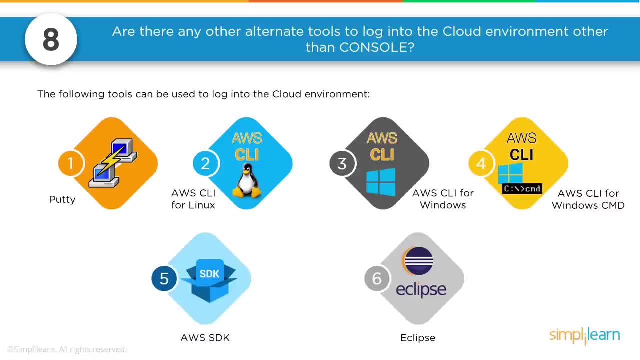 And from there you can actually access the rest of the resources. So this is an alternative to the console And of course we have the AWS CLI. in any of the Linux machines or Windows machines We can install. So that's point two, three and four. 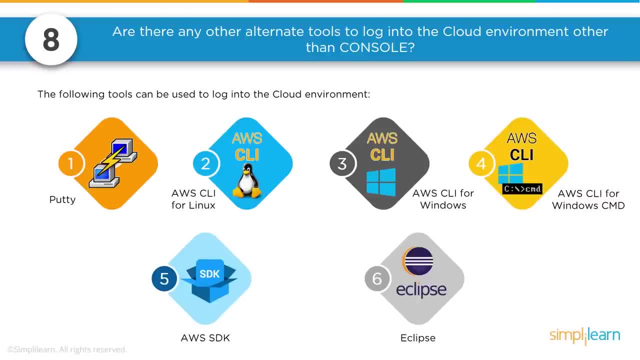 We can install AWS CLI for Linux, Windows, also for Mac, So we can install them And from there, from your local machine, we can access, run AWS commands and access provision, monitor the AWS resources. The other ones are: we can access the AWS resource programmatically. 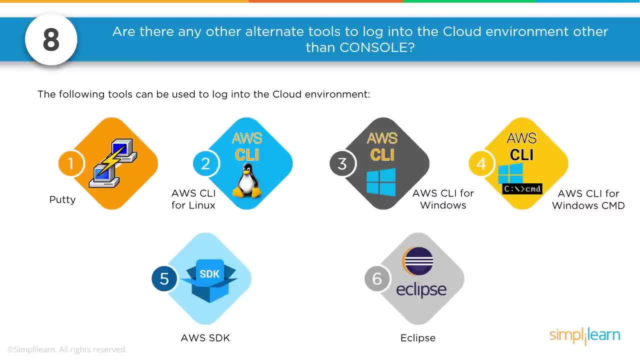 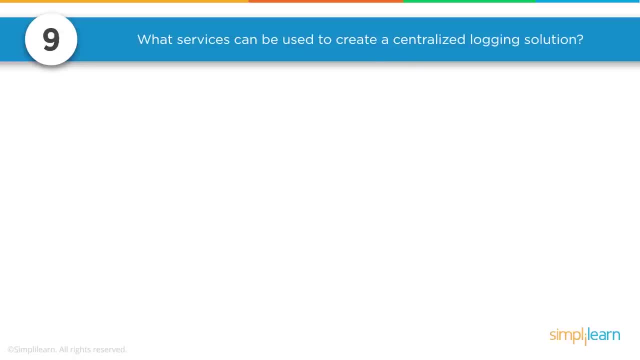 using AWS SDK and Eclipse. So these are a bunch of options. we have to use the AWS resource other than the console If you're interviewed in a company or by a company that focuses more on security and want to use AWS native services for their security. 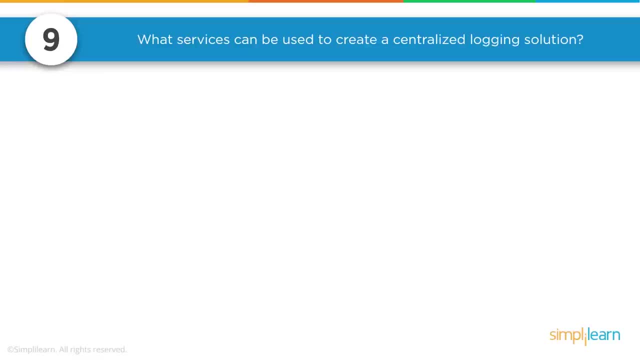 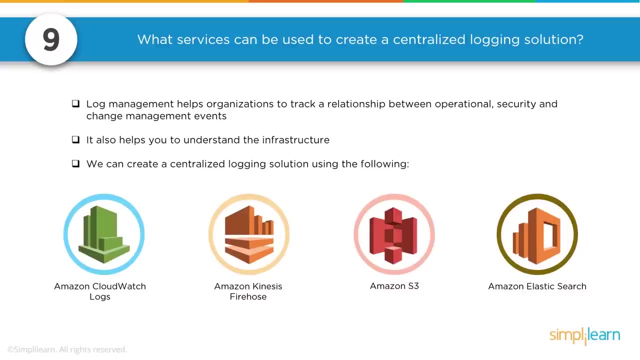 then you would come across this question: What services can be used to create a centralized login? The basic services we could use are CloudWatch logs, store them in S3, and then use Elasticsearch to visualize them and use Kinesis to move the data from S3 to Elasticsearch. 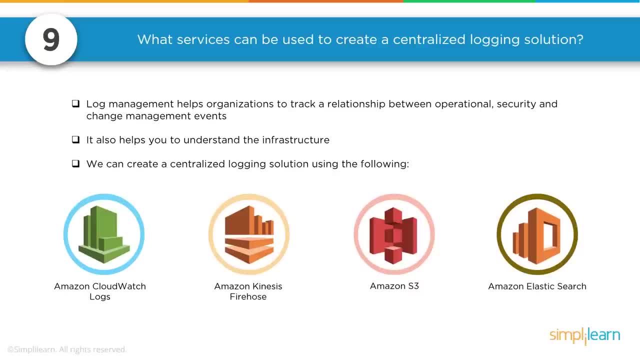 So log management- it actually helps organizations to track the relationship between operational and security changes and the events that got triggered based on those logs. Instead of logging into an instance or instead of logging in to the environment and checking the resources physically, I can come to a fair conclusion by just looking at the logs. 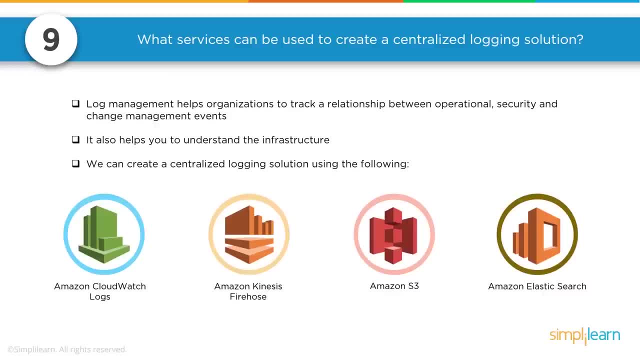 Every time there's a change the system would scream and it gets tracked in the CloudWatch and then CloudWatch pushes it to S3.. Kinesis pushes the data from S3 to Elasticsearch and I can do a time-based filter and I would get a fair understanding. 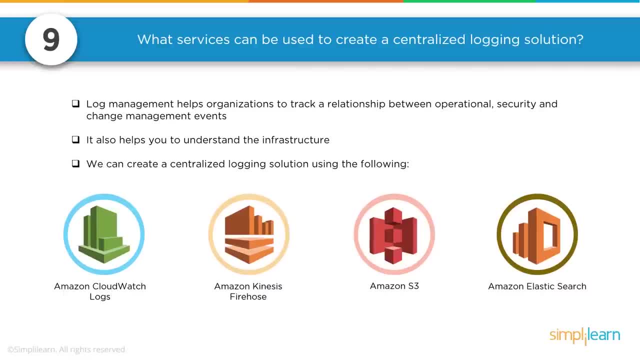 of what was going on in the environment for the past one or whatever the time window that I wanted to look at. So it helps I'm getting a good understanding of the infrastructure as a whole. All the logs are getting saved in one place. 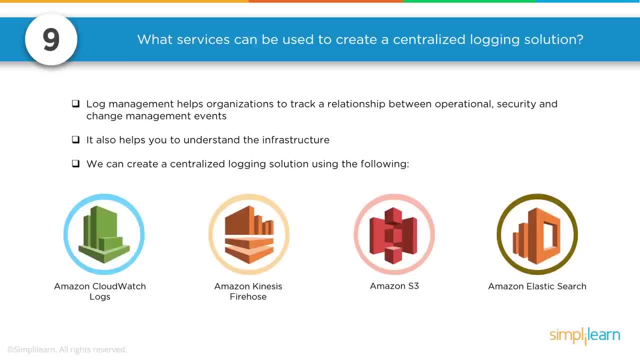 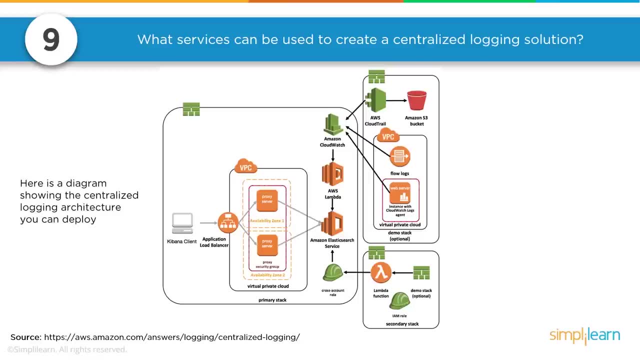 So all the infrastructure logs are getting saved in one place, So it's easy for me to look at it in an infrastructure perspective. So we know the services that can be used- and here are some of the services and how they actually connect to each other. 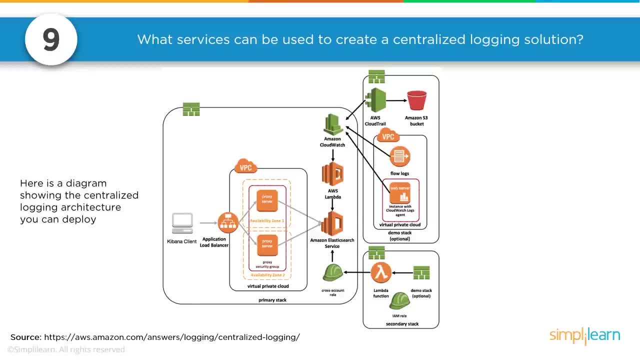 It could be logs that belongs to one account. It could be logs that belongs to multiple accounts, It doesn't matter. You know those three services are going to work fairly good and they're going to inject or they're going to like suck logs from the other accounts. 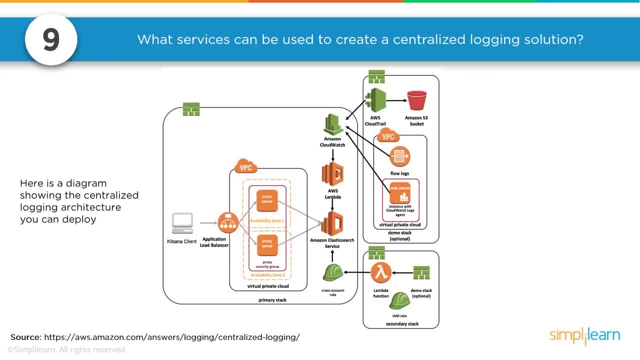 put it in one place and help us to monitor. So, as you see, you have CloudWatch here that actually tracks the metrics. You can also use CloudTrail. if you want to log API calls as well, push them in an S3 bucket. 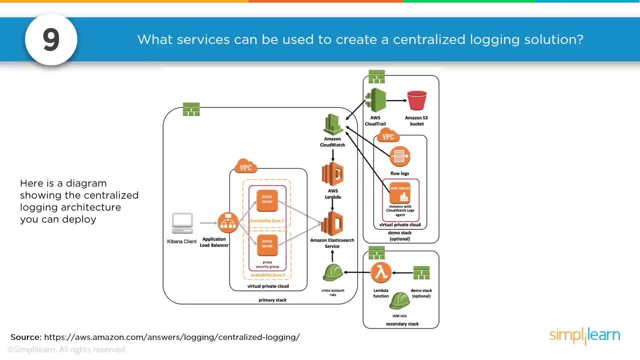 So there are different types of logs. Flow logs are getting captured in an instance, Application logs are getting captured from the same VPC, from a different VPC, from the same account, from a different account, and all of them are analyzed using Elasticsearch. 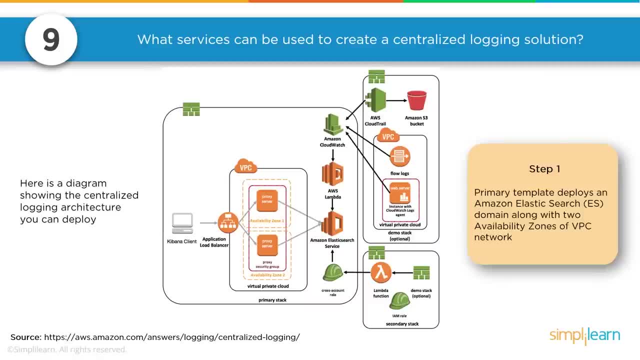 using the Kibana client. So step one is to deploy the ECS cluster. Step two is to restrict access to the ECS cluster because it's valid data. You don't want anybody to put their hands and access their data, So restrict access to the ECS dashboard. 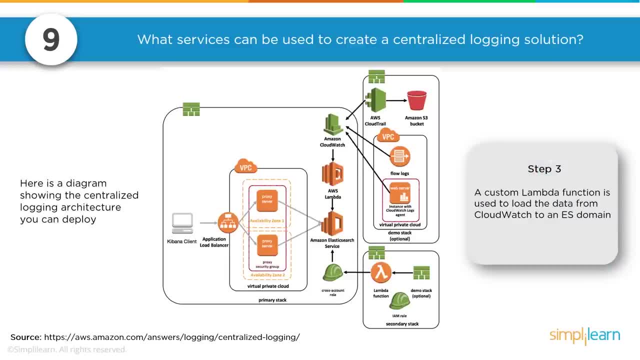 and we could use Lambda also to push the data from CloudWatch to the Elasticsearch domain. And then Kibana is actually the graphical tool that helps us to visualize the logs, Instead of looking at log as just statements or in a bunch of characters. 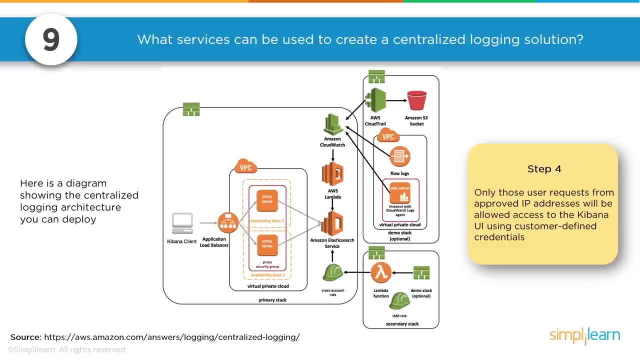 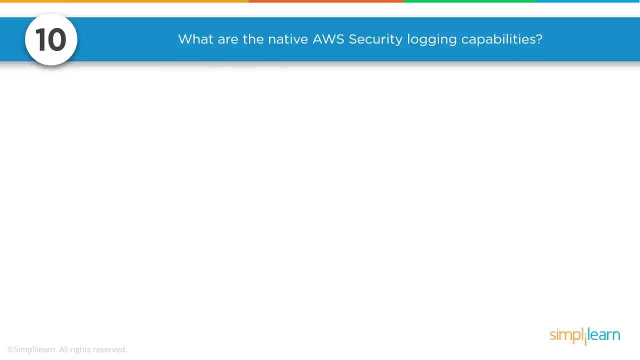 a bunch of files. Kibana helps us to analyze the logs in a graphical or a chart or a bar diagram format. Again, in an interview, the interviewer is more concerned about testing your knowledge on AWS security products, especially on the logging monitoring. 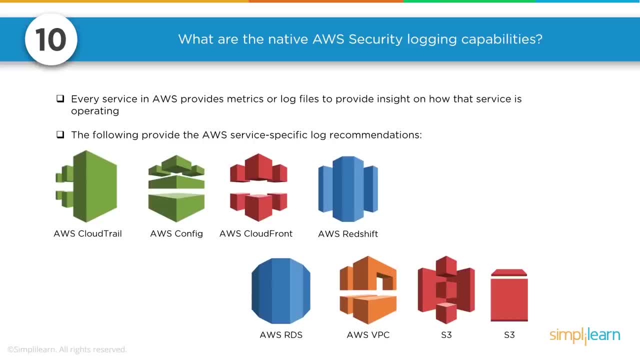 event management or incident management. Then you could have a question like this: What are the native AWS security logging capabilities? Now, most of the services have their own logging in them. like have their own logging, like S3, S3 has its own login. 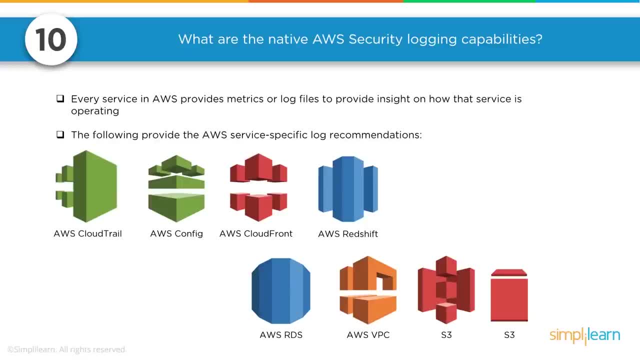 and CloudFront has its own logging, DS has its own logging, VPC has its own logging. In additional there are account level logins like CloudTrail and AWS Config Services. So there are a variety of logging options available in the AWS like CloudTrail, Config, CloudFront, Redshift logging. 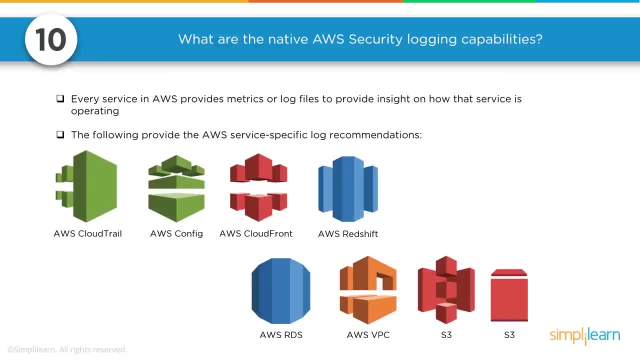 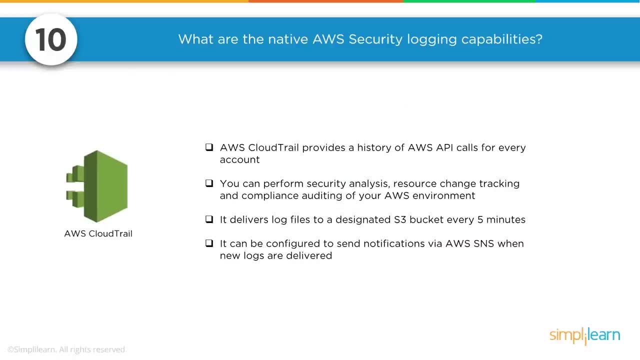 RDS logging, VPC flow logs, S3 object logging, S3 access logging, stuff like that. So we're going to look at two servers in specific: CloudTrail. Now this CloudTrail, the very first product in that picture we just saw. 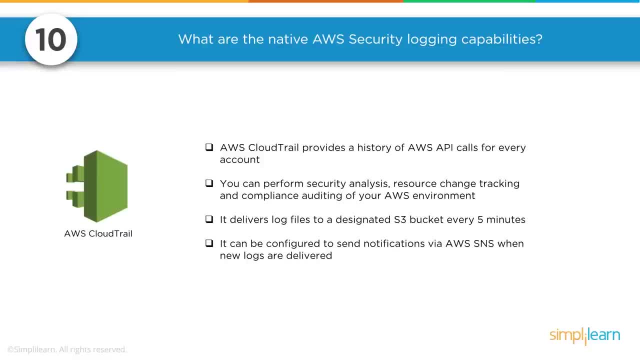 the CloudTrail provides a very high level history of the API calls for all the account And with that we can actually perform a very good security analysis, a security analysis of our account, And these logs are actually delivered to. you can configure it. 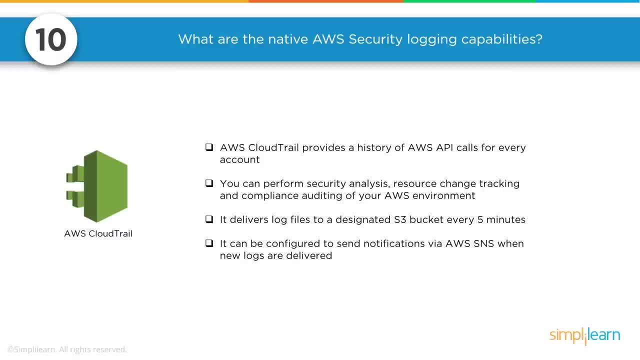 they can be delivered to S3 for long time archivals And based on a particular event. it can also send an email notification to us saying: hey, just got this error, thought I'll let you know stuff like that. The other one is Config Service. 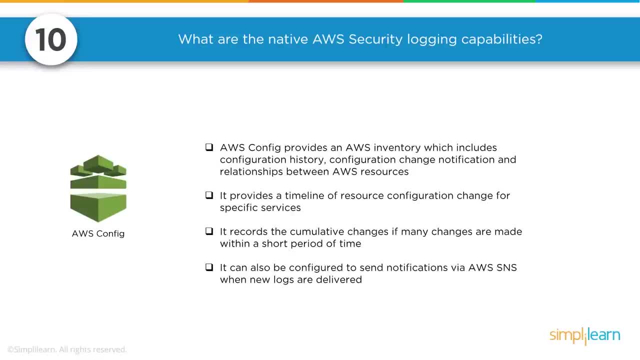 Config Service helps us to understand the configuration changes that happen in our environment And we can also set up notifications based on the configuration changes. So it records the cumulative changes that are made in a short period of time. So if you want to go through the lifetime of a particular resource, 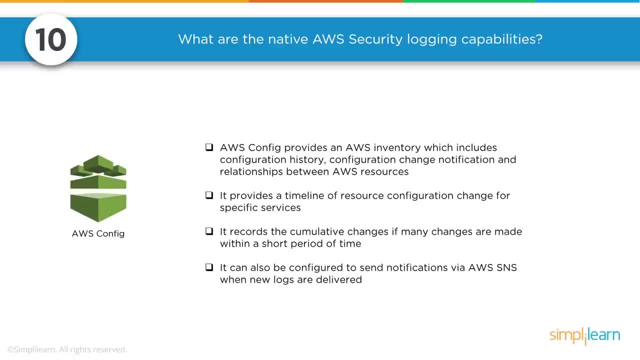 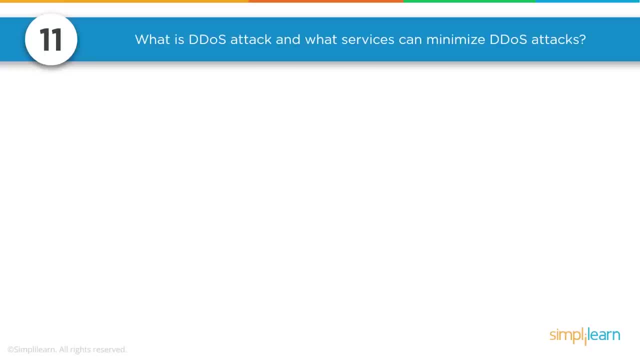 what are the things that happened? What are the things that went through? They can be looked at using AWS Config, All right, The other question you could get asked is if you know your role includes taking care of cloud security as well. 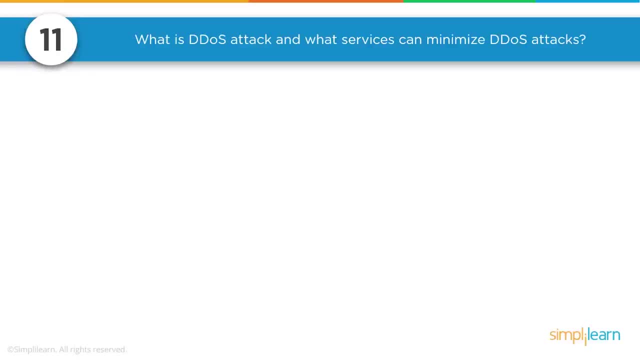 then the other question you could get asked is the native services that Amazon provides to mitigate DDoS, which is denial of service. Now, not all companies would go with Amazon native services, but there are some companies which want to stick with Amazon native services. 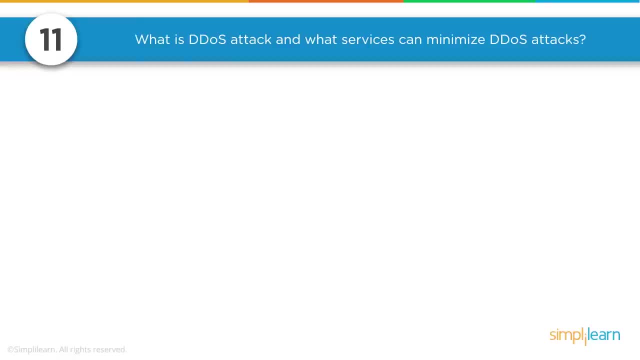 just to save them from the headache of managing the other softwares or bringing in another tool, a third party tool, into managing DDoS. They simply want to stick with Amazon proprietary Amazon native services And a lot of companies are using Amazon service to prevent DDoS. 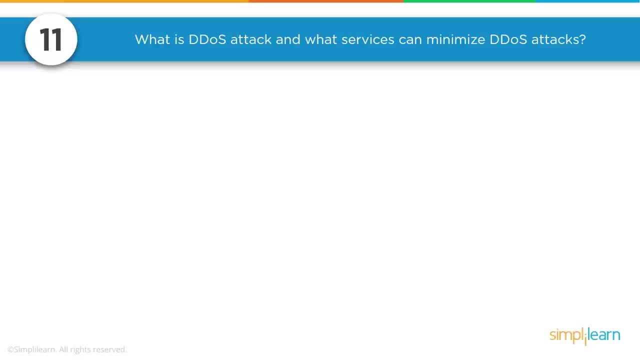 denial of service. Now, denial of service is. if you already know what denial of service is, well and good. If you do not know, then let's know it now. Denial of service is a user trying to, or maliciously making attempt to, access a website or an application. 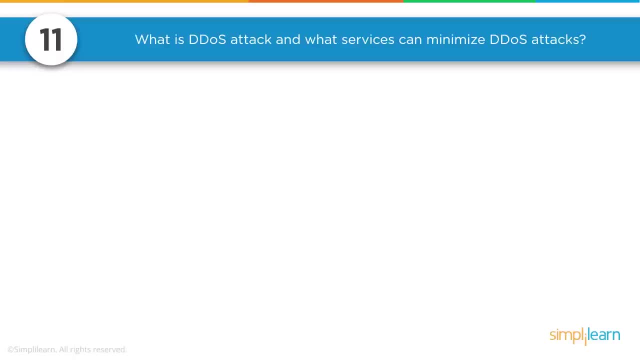 The user would actually create multiple sessions And he would occupy all the sessions And he would not let legitimate users access the servers. So he's, in turn, denying the service for the user. A quick picture review of what denial of service is Now look at it. 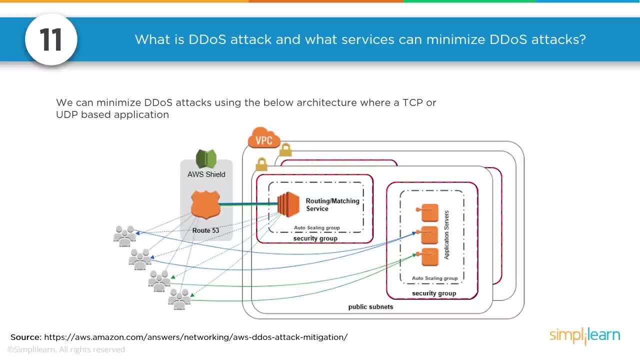 These users. instead of making one connection, they are making multiple connections, And there are cheap software programs available that would actually trigger connections from different computers in the internet with different MAC addresses. so everything kind of looks legitimate for the server And it would accept those connections. 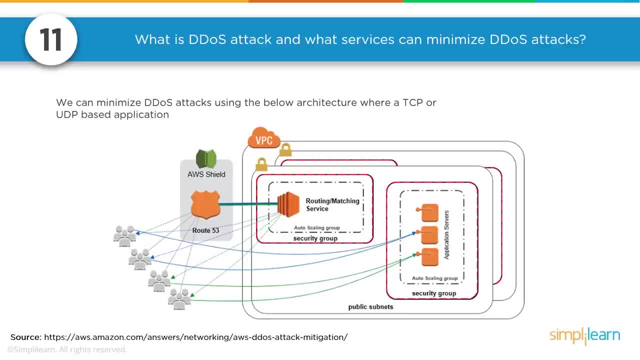 And it would keep the sessions open. The actual users won't be able to use them. So that's denying the service for the actual users. Denial of service- All right, And distributed denial of service is generating attacks from multiple places, you know, from a distributed environment. 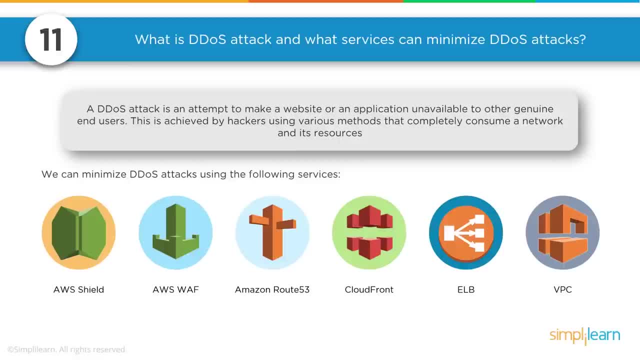 So that's distributed denial of service. So the tools, the native tools that helps us to prevent the denial of service attacks in AWS is Cloud Shield and Web Access Firewall, AWS, WAF. Now they are the major ones. They are designed to mitigate a denial of service. 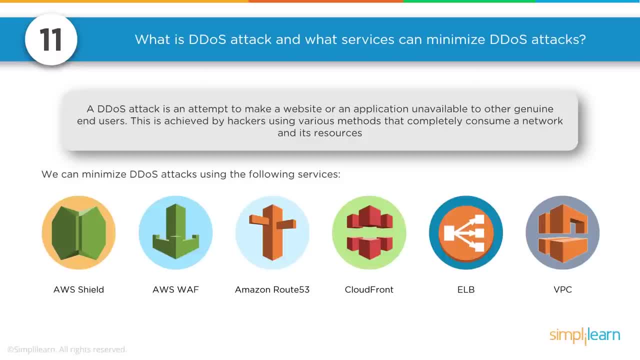 If your website is often bothered by denial of service, then we should be using AWS Shield or AWS WAF, And there are a couple of other tools that also does. when I say that also does, denial of service is not their primary job. 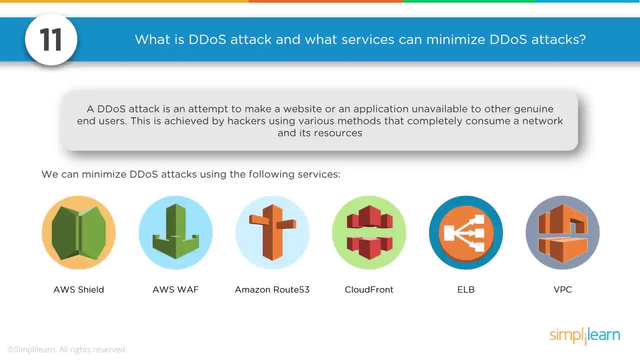 but you could use them for denial of service. Route 53's purpose is to provide DNS. Outfront is to provide caching. Elastic Load Balancer- ELB's work is to provide load balancing. VPC is to create a secure virtual private environment. 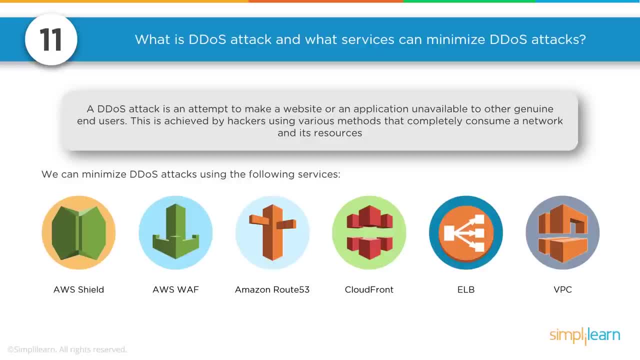 But they also support mitigating denial of service, but not to the extent you would get in AWS Shield and AWS WAF. So AWS Shield and WAF are the primary ones, but the rest can also be used to mitigate distributed denial of service. 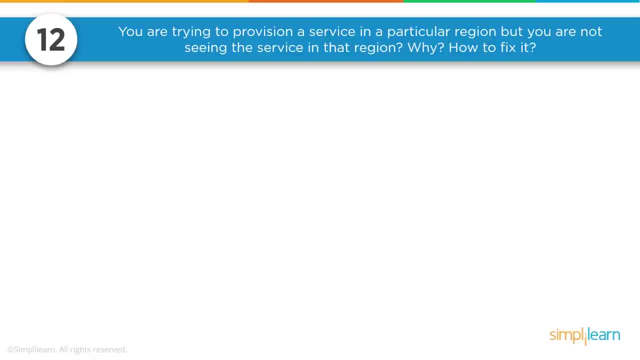 The other tricky question is: this actually will test your familiarity with the region and the services available in the region. So when you're trying to provision a service in a particular region, you're not seeing the service in that region. How do we go about fixing it? 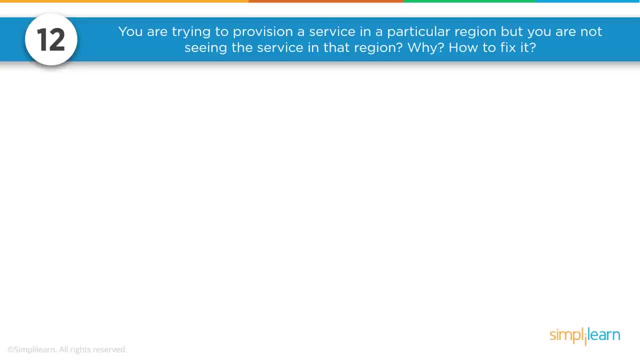 Or how do we go about using the service in the cloud. It's a tricky question And if you have not gone through such situation, you can totally blow it away. You really need to have a good understanding on regions, the services available in those regions. 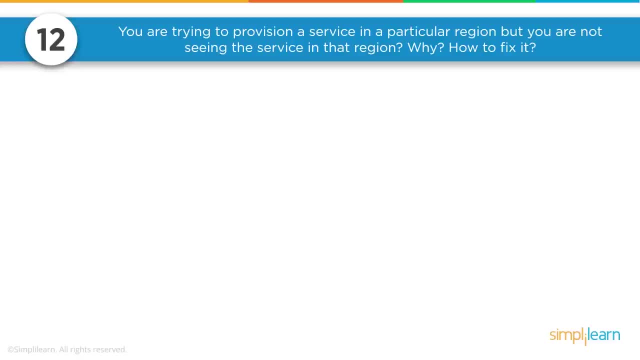 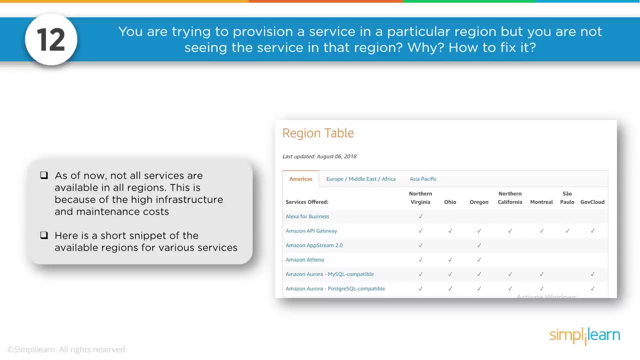 and what if a particular service is not available? how to go about doing it? The answer is: not all services are available in all regions. Anytime Amazon announces a new service, they don't immediately publish them on all regions. They start small and as and when the traffic increases. 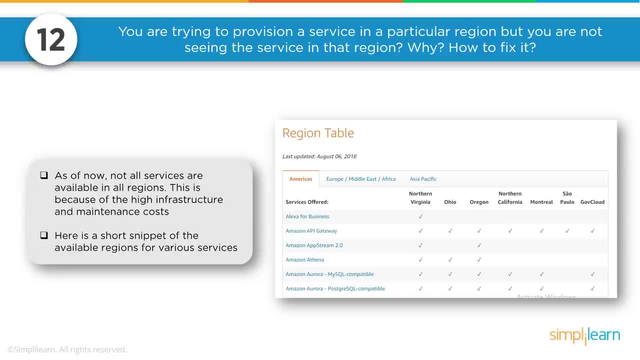 as and when it becomes more likable to the customers, they actually move the service to different regions. So, as you see in this picture, within America, North Virginia has more services compared to Ohio, compared to North California. So, within America itself, North Virginia is the preferred one. 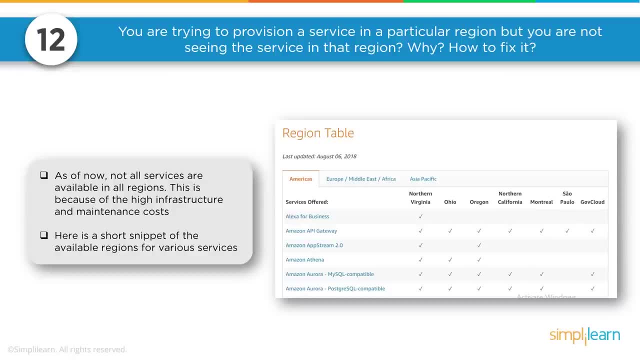 So similarly, there are preferred regions within Europe, Middle East and Africa and preferred regions within Asia Pacific. So anytime we don't see a service in a particular region, chances that the service is not available in that region yet. we got to check the documentation and find the nearest region. 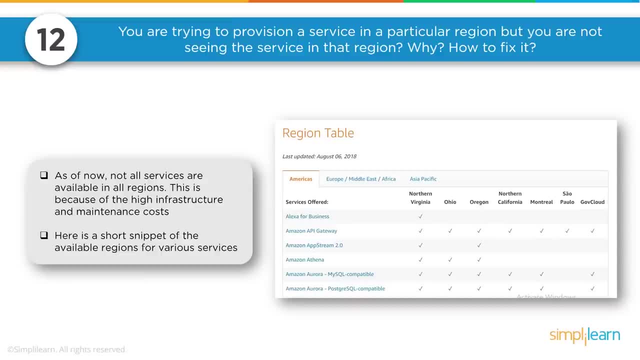 that offers that service and start using the service from that region. Now you might think: well, if I'm looking for a service in Asia, let's say in Mumbai, and if it is not available, why not simply switch to North Virginia and start using it? 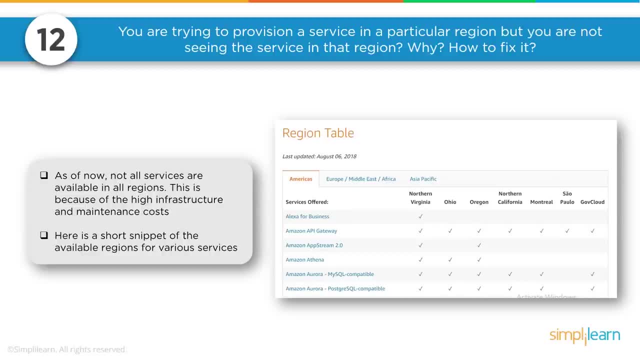 You could, but that's going to add more latency to your application. So that's why we need to check for application, which is check for region, which is very near to the place where you want to serve your customers, and find nearest region instead of always going back to North Virginia. 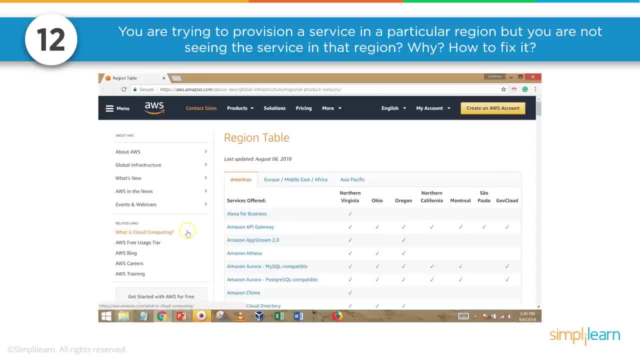 and deploying an application in North Virginia. Again, there's a place, there's a link in AWS that you can go and look for services available in different region- And that's exactly what you're seeing here- And if your service is not available in a particular region, 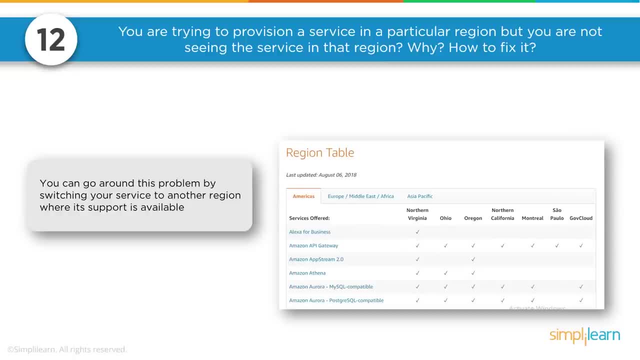 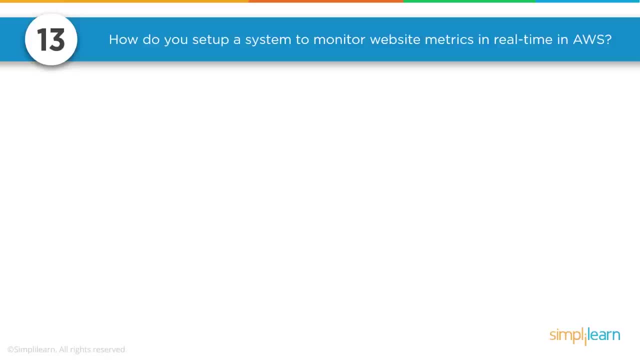 switch to the other region that provides your service, the nearest other region that provides that service, and start using service from there. With the coming up of cloud, a lot of companies have turned down their monitoring team. Instead, they want to go with the monitorings that cloud provides. 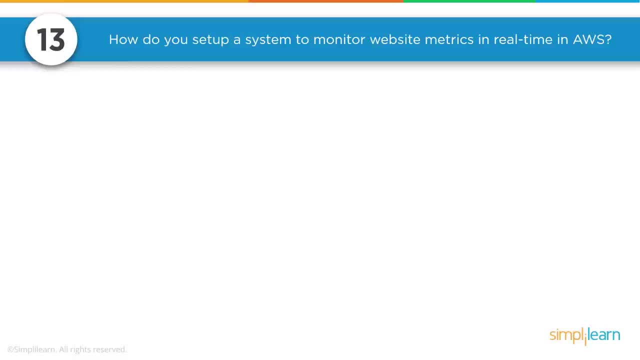 You know nobody wants to, or at least many people don't want to- go through the hassle of at least new startups and new companies that are thinking of having a monitoring environment, that they don't want to go with traditional NOC monitoring. Instead they would like to leverage AWS monitorings available. 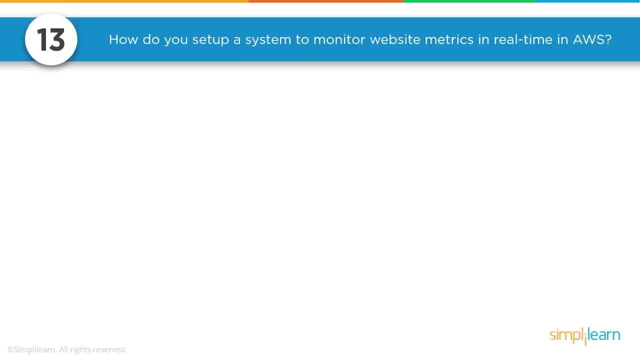 because it monitors a lot of stuff, not just the availability, but it monitors a lot of stuff like failures, errors. It also triggers emails, stuff like that. So how do you actually set up a monitor to website? How do you set up a monitor to monitor the website metrics in real time in AWS? 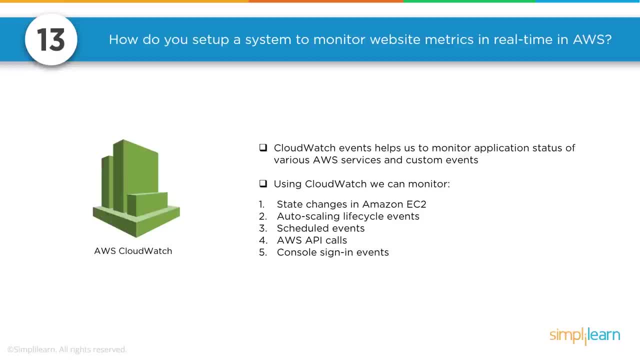 The simple way. anytime you have a question about monitoring, CloudWatch should strike your mind, because CloudWatch is meant for monitoring, is meant for collecting metrics, is meant for providing graphical representation of what's going on in a particular network at a particular point of time. 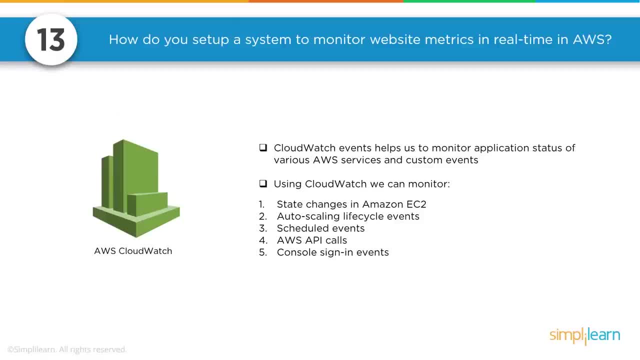 So CloudWatch. CloudWatch helps us to monitor applications and using CloudWatch, we can monitor the state changes, not only the state changes. the auto-scaling life cycle events Anytime. there are more services added. there is a reduction in the number of servers because of less usage. 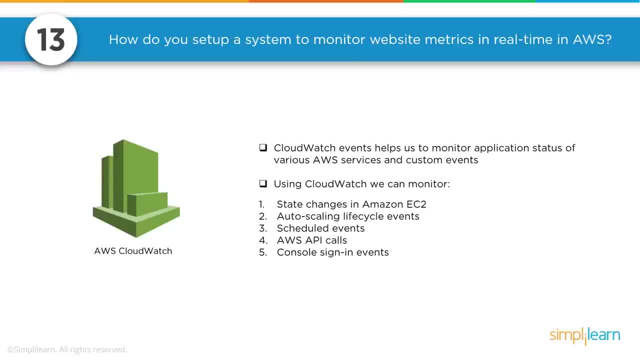 Very informative messages can be received through CloudWatch. CloudWatch can now support scheduled events. If you want to schedule anything, CloudWatch has an event that would schedule an action. schedule a trigger- time-based, not incident-based. You know anything happening and then you get an action happening. 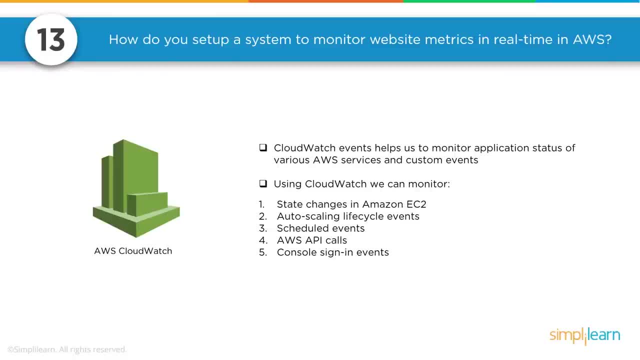 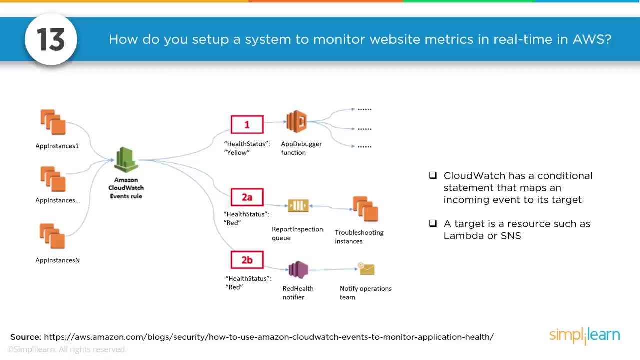 that's incident-based. On the other hand, you can simply schedule a few things on time-based, So that's possible with CloudWatch. So this CloudWatch integrates very well with a lot of other services like notifications for notifying the user or for notifying the administrator about it. 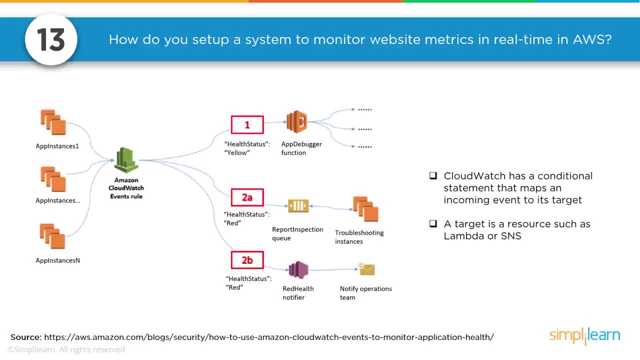 and it can integrate well with Lambda. So the trigger and action anytime you're designing an auto-healing environment. this CloudWatch can actually monitor and send an email if we are integrating it with SNS simple notification service or this CloudWatch can monitor and based on what's happening. 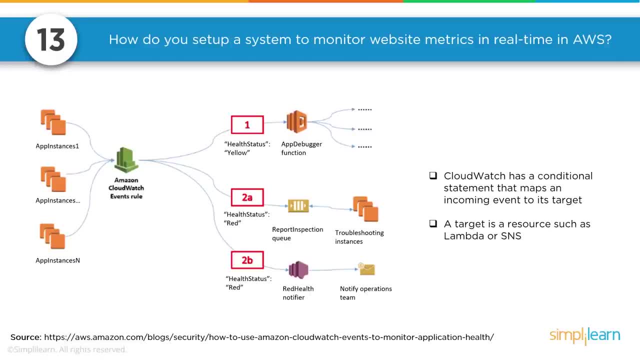 it can trigger an event in Lambda and that would in turn run a function till the environment comes back to normal. So CloudWatch integrates well with a lot of other AWS services. All right, so CloudWatch has three statuses: Green when everything is going good. 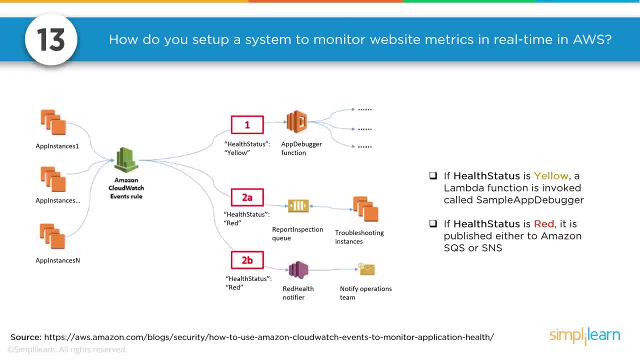 Yellow when the service is degraded And red when the service is not available. Green is good, so we don't have to do anything about it, But anytime there's an yellow, the picture that we're looking at- it's actually calling a Lambda function. 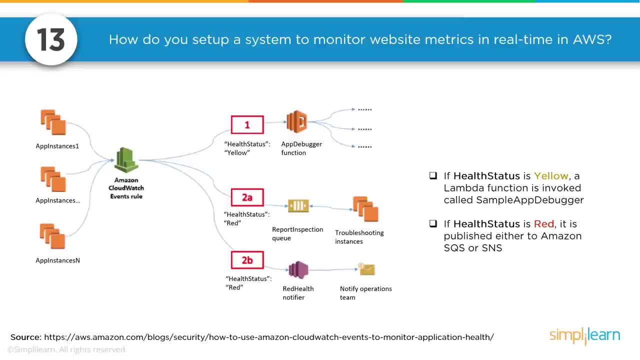 to debug the application and to fix it. And anytime there's a red alert, it immediately notifies the owner of the application about: well, the service is down. and here is the report that I have. Here is the metrics that I've collected about the service, stuff like that. 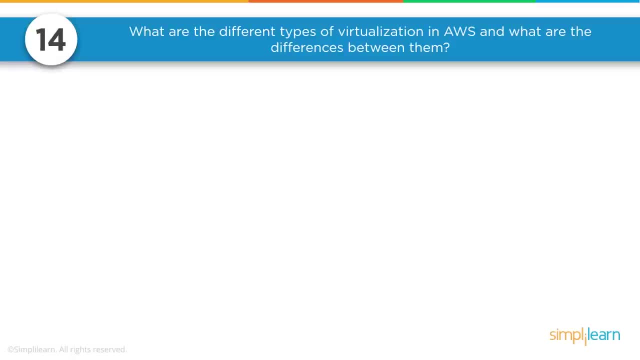 If the job role requires you to manage the servers as well. there are certain job roles which are on the system side. There are certain job roles which is development plus system side. Now you're responsible for the application and the server as well. So if that's the case, 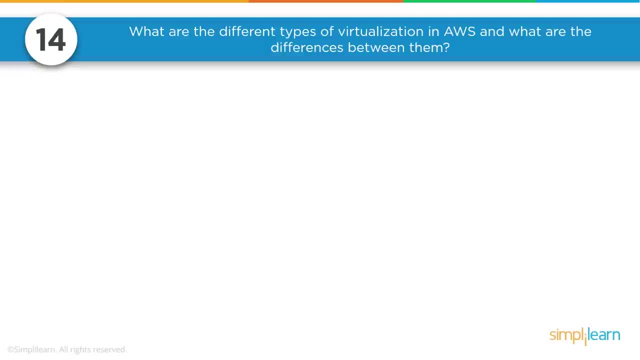 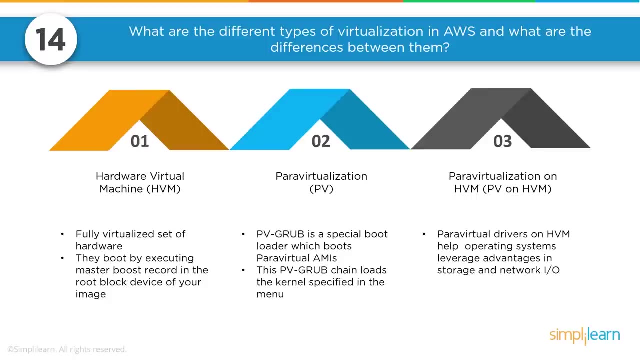 you might be tested with some basic questions like the different types of virtualization and AWS and what are the difference between them. All right, the three major types of virtualization are HVM, which is Hardware Virtual Machine. The other one is PV, Para Virtualization. 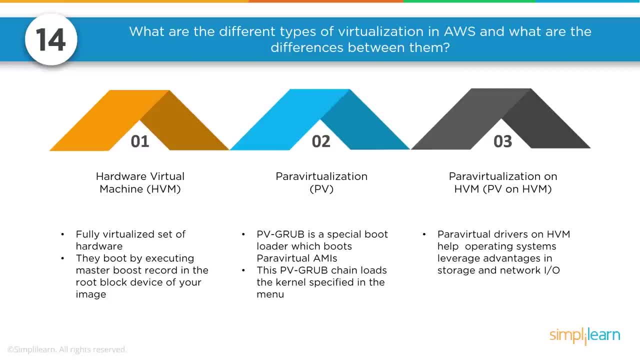 And the third one is PV on HVM, Para Virtualization, on Hardware Virtual Module. All right, the difference between them, or actually describing them, is actually the difference between them. HVM, it's actually a fully virtualized hardware, You know, the whole hardware is virtualized. 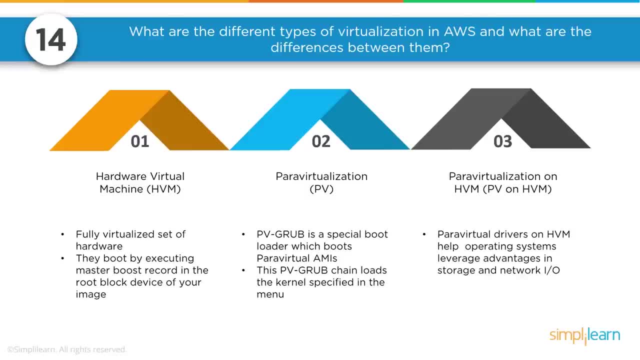 and all virtual machines act separate from each other And these VMs are booted by executing master boot record in the root block. And when we talk about Para Virtualization, Para Grub is actually the special boot loader which boots the PV AMIs. 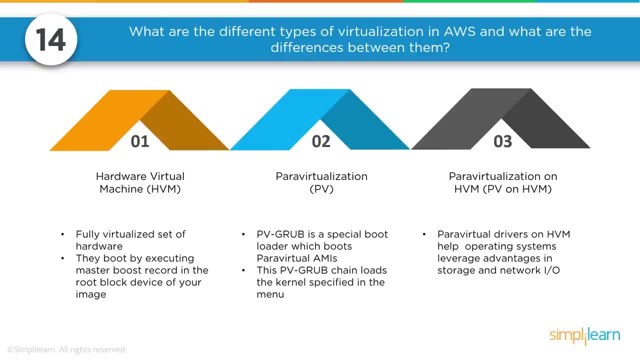 And when we talk about PV on HVM, it's actually the marriage between HVM and PV And this Para Virtualization on HVM, in other words PV on HVM. it actually helps operating system take advantage in storage and the network input output available through the host. 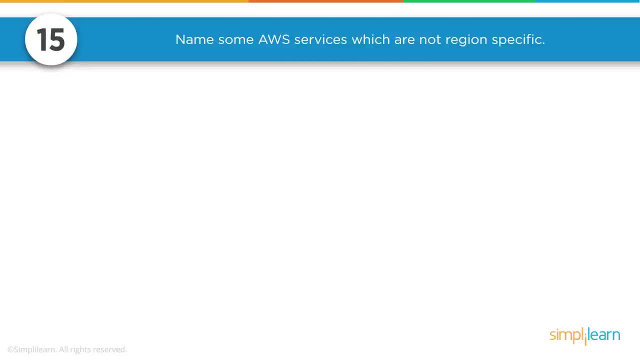 Another good question is name some of the services that are not region specific. Now you've been taught that all services are within a region and some services are within an availability zone. For example, EC2 is within an availability zone. EBS is within an availability zone. 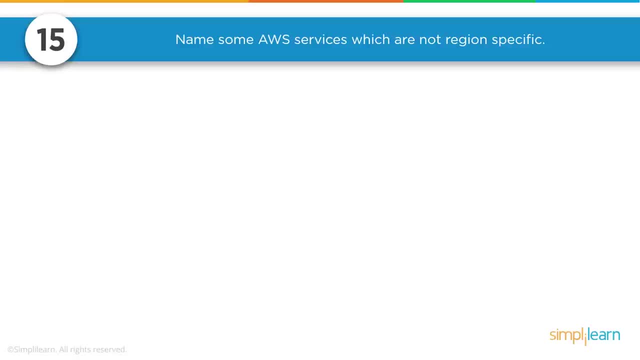 S3 is region specific. DynamoDB is region specific Stuff like that. VPC is both availability and region specific, meaning subnets are availability zone specific and VPC is region specific stuff like that. So you might have thought you might have learned in that combination. 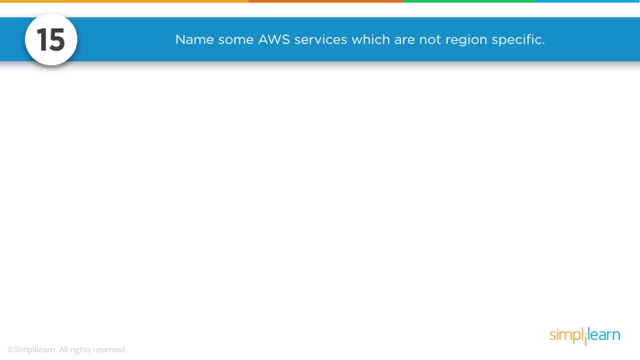 But there could be some tricky questions that test you How well you have understood the region, non-region and availability, non-availability services. I should say there are services that are not region specific. That would be IAM. So we can't have IAM for every availability zone and for every. 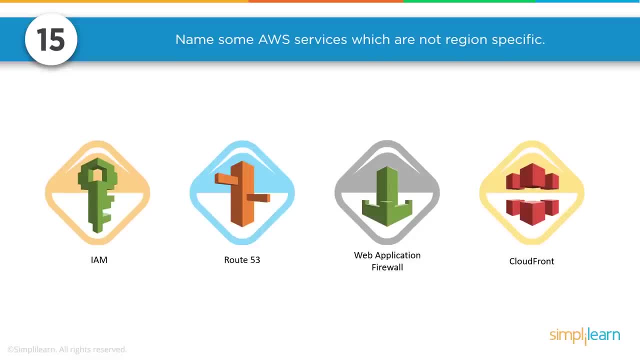 region, which means, you know, users will have to use one username and password for one region And any time they switch to another region, they will have to use another username and password. that that's more work And that's not a good design as well. 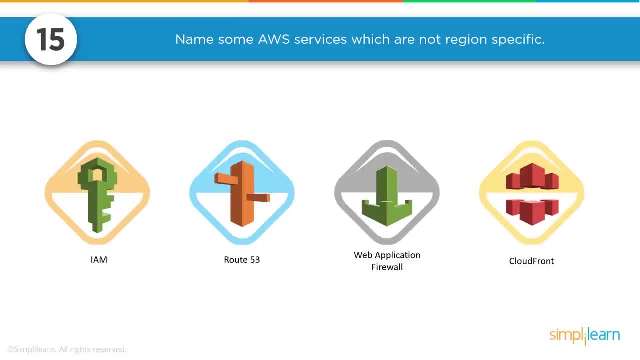 Authentication has to be global, So IAM is a global service and which means it's not region specific. On the other hand, Route 53 is again a regional specific, So we can't have Route 53 for every region. Route 53 is not a region specific service. 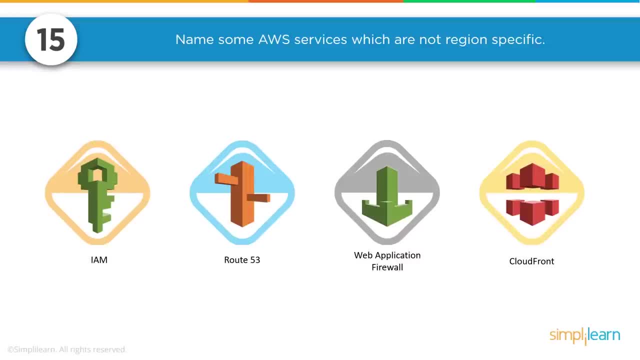 It's a global service and it's one application. Users access from everywhere or from every part of the world, So we can't have one URL or one DNS name for each region. if your application is a global application And then Web Application Firewall works well with CloudFront. 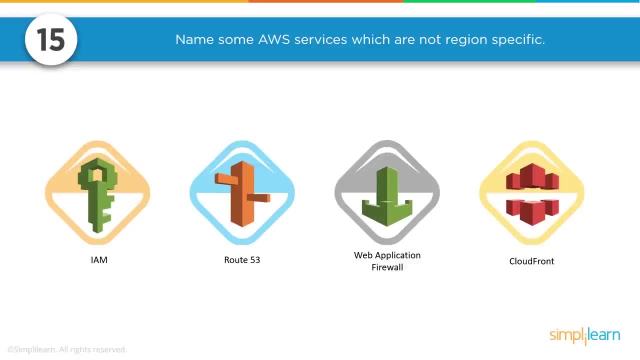 Then CloudFront is a region based service. So the Web Application Firewall, it's not region specific service, It's a global service. And CloudFront is again a global service, though you can, you know, cache content on a continent and country basis. 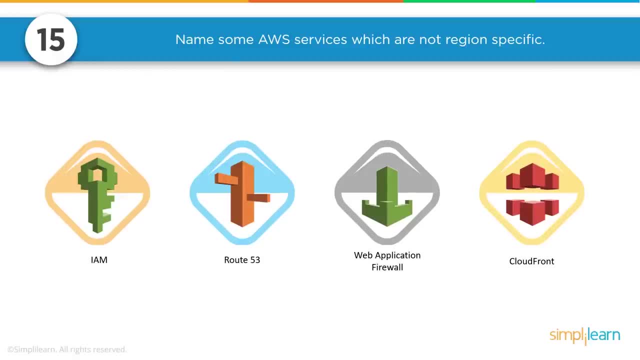 It's still considered a global service right. It's not bound to any region. So when you activate CloudFront, you're activating it away from region or availability zone. So when you're activating Web Application Firewall, because it's not a region specific service, 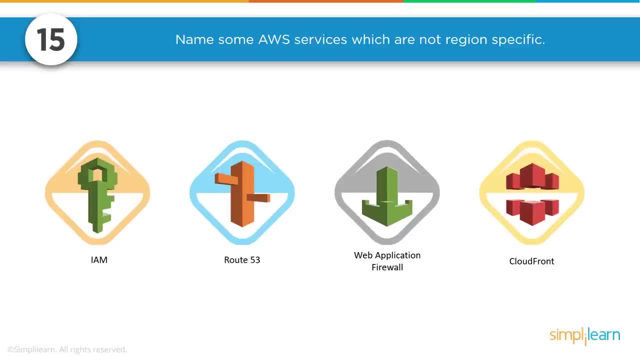 you're activating it away from availability zone and regions. So a quick recap: IAM, users, groups, roles and accounts. They are global services. They can be used globally. Route 53 services are offered at edge locations and they are global as well. 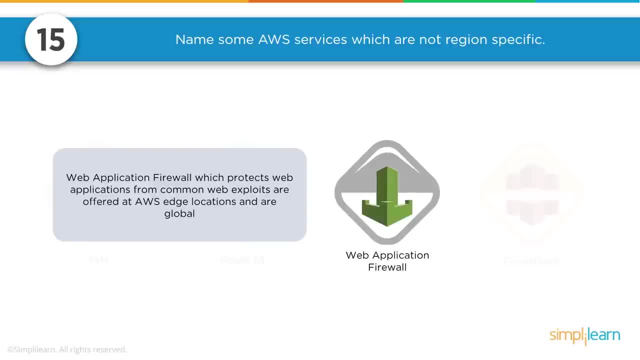 Web Application Firewall, a service that protects our web application from common web exploits. They are global service as well, CloudFront. CloudFront is Global Content Delivery Network, CDN, and they are offered at edge locations, which are a global service, In other words, non region specific service. 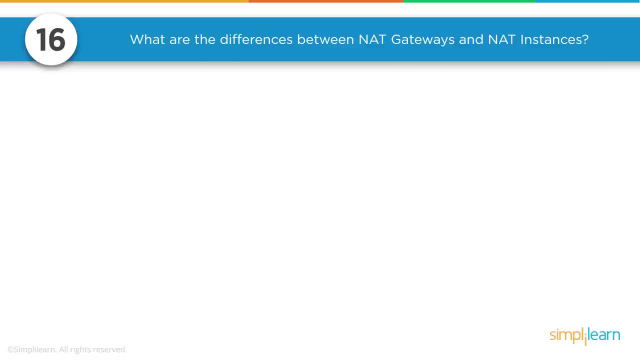 Beyond region service. All right, this is another good question as well In the project that you are being interviewed: if they really want to secure their environment using NAT or if they are already securing their environment using NAT by any of these two methods, like NAT Gateway or NAT Instances. 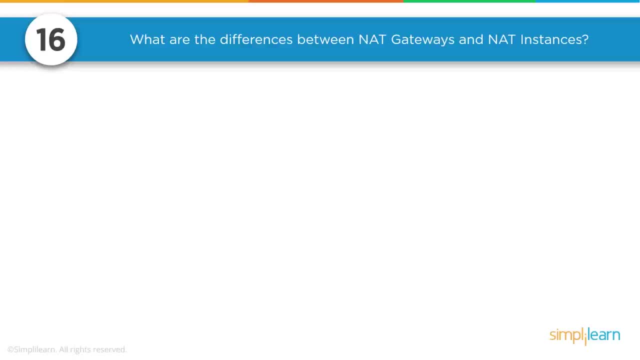 you can expect this question: What are the difference between a NAT Gateway and NAT Instances? Now, they both serve the same thing, right? They're not two different services. They're trying to achieve two different things. They both serve the same thing. but still they do have differences in them. right On a high level, they both achieve providing NATing for the service behind it, But the difference comes when we talk about the availability of it. NAT Gateway is a managed service by Amazon, whereas NAT Instance is managed by us. 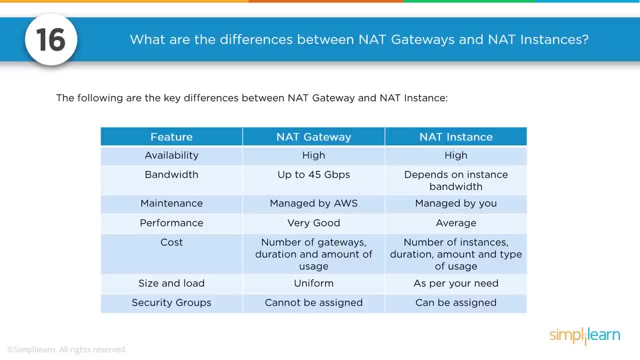 Now I'm talking about the third point: maintenance. here NAT Gateway is managed by Amazon, NAT Instance is managed by us And availability of NAT Gateway is very high. And availability of NAT Instance is less compared to the NAT Gateway because it's managed by us. 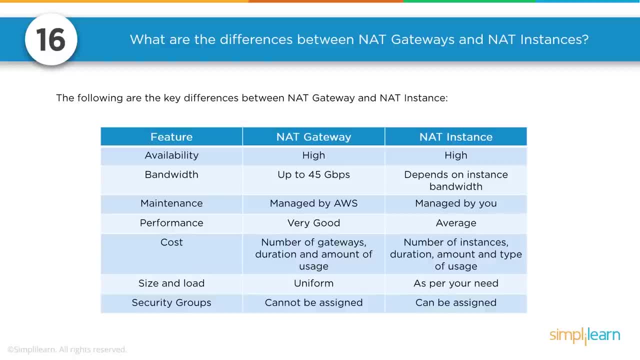 You know it's on an EC2 instance which could actually fail, And if it fails we'll have to relaunch it. But if it is NAT Gateway, if something happens to that service, Amazon would take care of reprovisioning it. 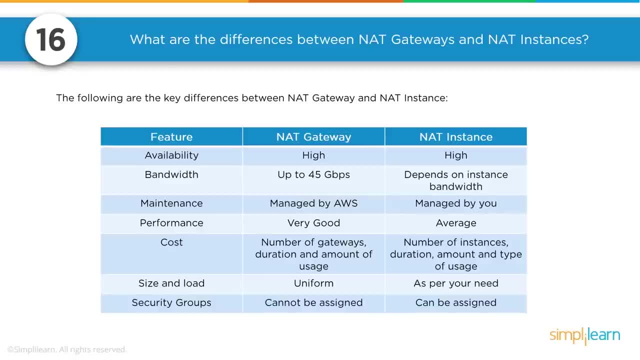 And talking about bandwidth, it can burst up to 75 gigabits. Now, traffic through the NAT Gateway can burst up to 75 gigabits, But for NAT Instance it actually depends on the server that we launch, And if we are launching a T2 Micro, it barely gets any bandwidth. 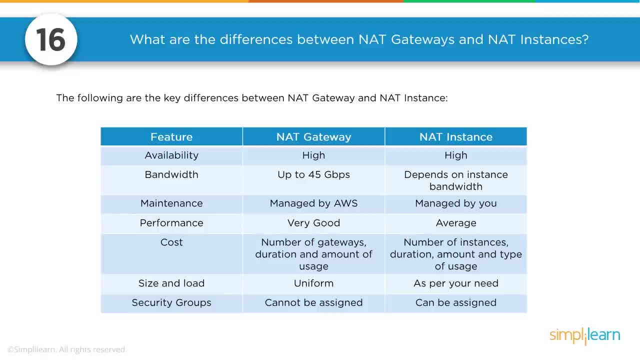 So there's a difference there. And the performance because it's highly available. because of the bigger pipe, 75 gigabits, the performance of the NAT Gateway is very high, But the performance of the NAT Instance is going to be average. 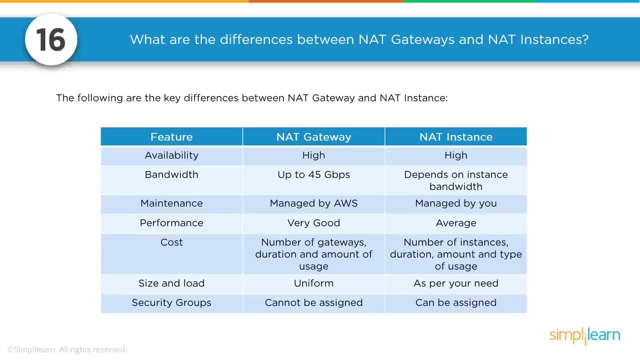 Again, it depends on the size of the NAT Instance that we pick And billing. billing for NAT Gateway is the number of gateways that we provision and the duration for which we use the NAT Gateway. But billing for NAT Instance is number of instance and the type of instance that we use. 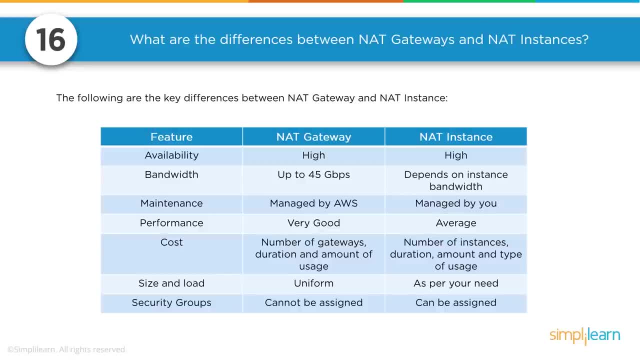 Of course number of instance, duration and the type of instance that we use. Security in NAT Gateway cannot be assigned, meaning it already comes with full packed security. But in NAT Instance security is a bit customizable. I can go and change the security because it's a server managed by me or managed by us. 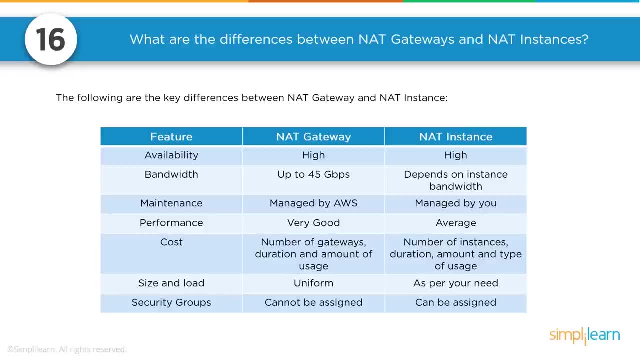 I can always change the security. Well, allow this, allow, don't allow this stuff. like that. Size and load of the NAT Gateway is uniform, But the size and the load of the NAT Instance changes as per. a NAT Gateway is a fixed product. 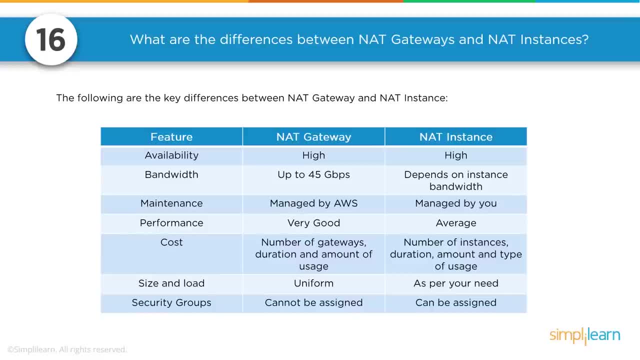 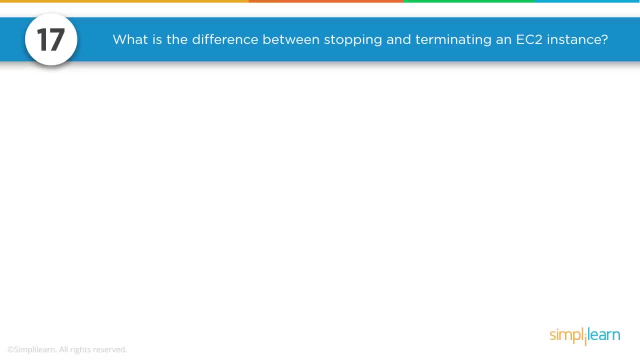 But NAT Instance can be small instance can be a big instance, So the size and the load through it varies. The other question you could get asked is: what is the difference between stopping and terminating an EC2 instance? Now you will be able to answer only if you have worked on environments. 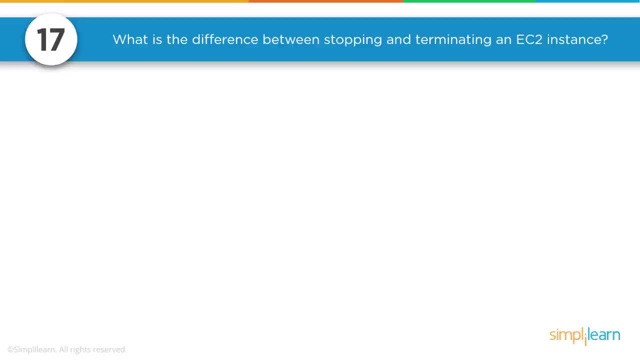 where you have your instance stopped and where you have your instance terminated. If you have only used lab and are attending the interview, chances are that you might be always lost when answering this question. It might look like both are the same. Well, stopping and terminating both are the same, but there is a difference in it. 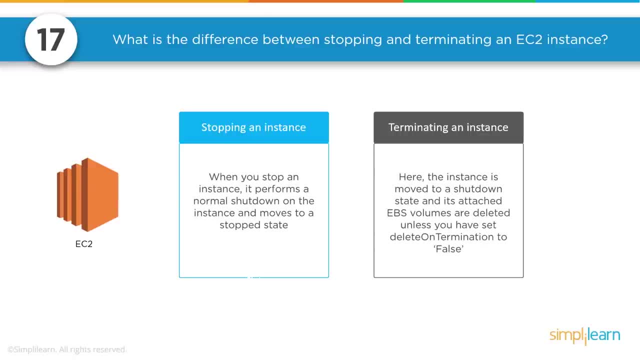 So when you stop an instance, it actually performs a normal shutdown on the instance and it simply moves the instance to the stopped state. But when you actually terminate the instance, the instance is moved to this stopped state. The EBS volumes that are attached to it are deleted and removed. 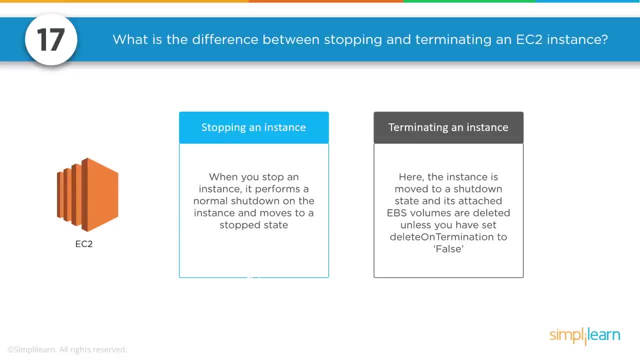 and we'll never be able to recover them again. So that's a big difference between stopping and terminating an instance. If you're thinking of using the instance again, along with the data in it, you should only be thinking of stopping the instance, but you should. 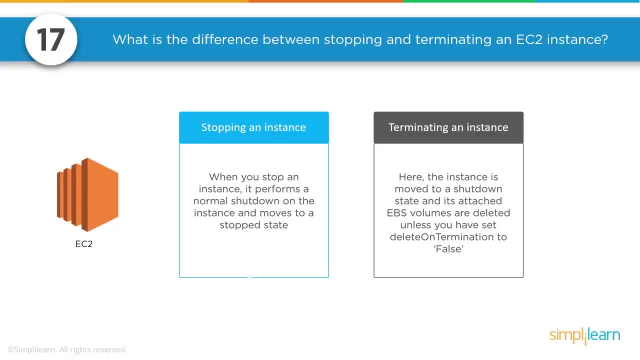 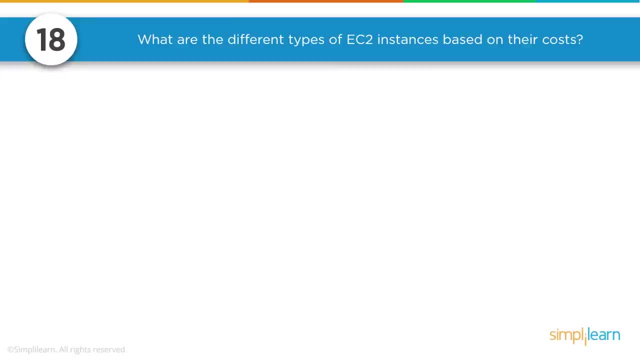 be terminating the instance only if you want to get rid of that instance forever. If you are being interviewed for an architect level position or a junior architect level position, or even a cloud consultant level position, or even in an engineering position, this is a very common question that gets asked. 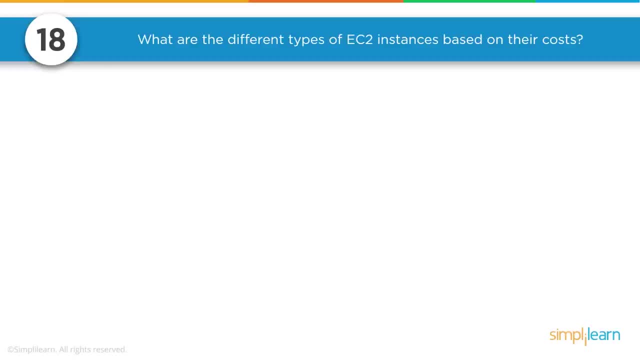 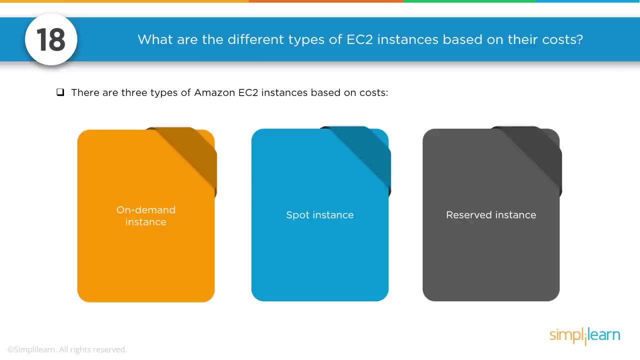 What are the different types of EC2 instances? based on their cost or based on how we pay them? They're all compute capacity. For example, the different types are on demand instances, spot instances and reserved instances. It kind of looks the same. 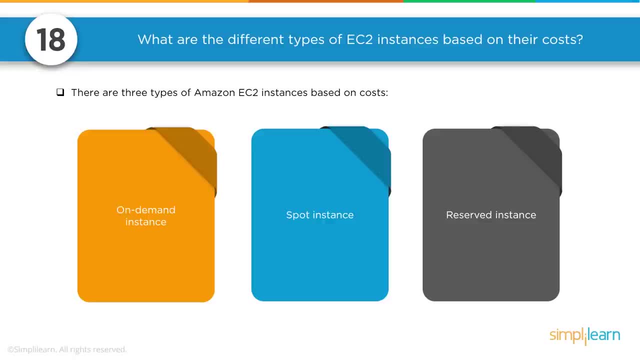 They all provide the compute capacity, They all provide the same type of hardware for us. But if you are looking at cost saving or optimizing cost in our environment, we got to be very careful about which one are we picking. We might think that well, I'll go with on demand instance, because 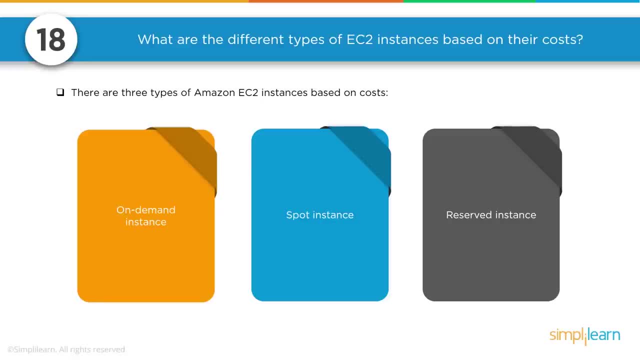 I pay on a per hour basis, which is cheap. I can use them anytime I want, and anytime I don't want I can simply get rid of it by terminating it. You're right, But if the requirement is to use the service for one year, the requirement is. 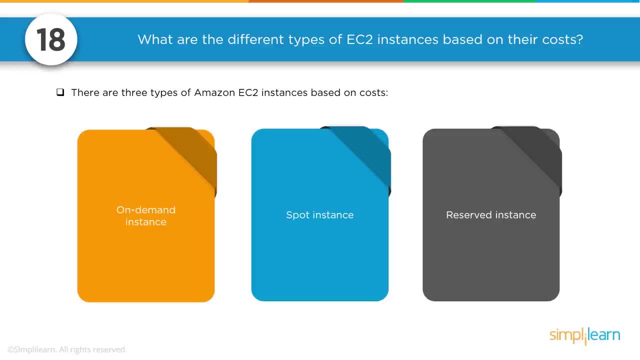 to use the service for three years, then you'll be wasting a lot of money buying on demand instances. you'll be wasting a lot of money paying on an hourly basis. Instead, we should be going for reserved instance, where we can reserve the capacity. 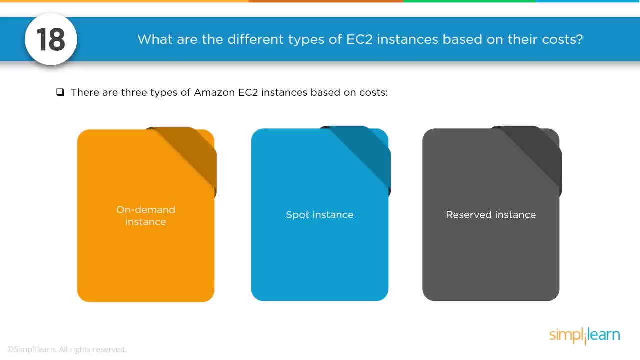 for the complete one year or complete three years and save a huge amount in buying reserved instances. All right, So on demand is cheap to start with, You're only planning to use it for a short while, but if you're planning to run it, 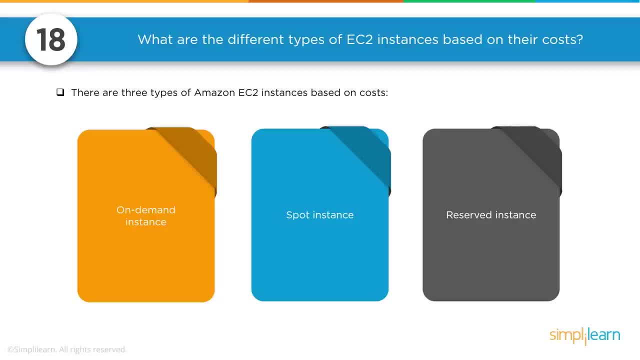 for a long while, then we should be going for reserved instance. That is what is cost efficient. So spot instance is cheaper than on demand instance, And there are different use cases for spot instance as well. So let's look at one after the other. 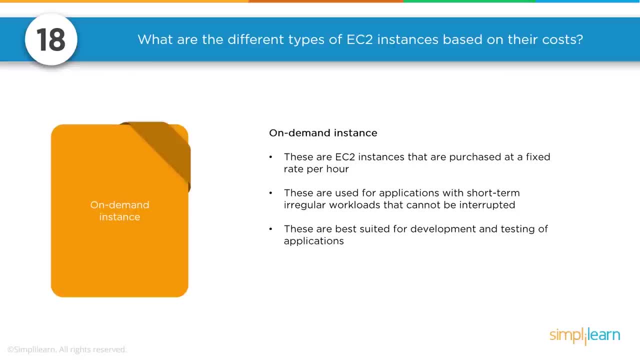 The on demand instance. the on demand instance is purchased at a fixed rate per hour. This is very short term and irregular workloads and for testing for development on demand instance is a very good use case We should be using on demand for production. 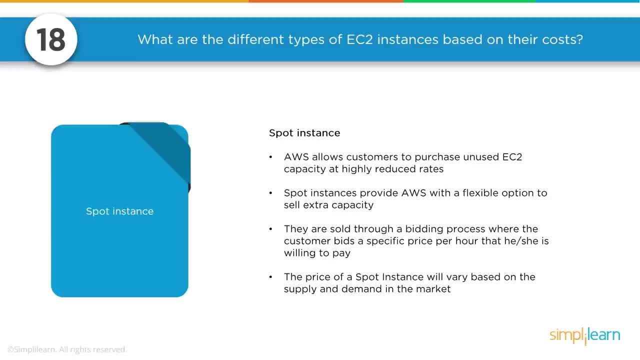 Spot instance. spot instance allows users to purchase EC2 at a reduced price And any time we have more instances, we can always go and sell it in spot instances. I'm referring to any time we have more reserved instances, we can always sell them in spot instance catalog. 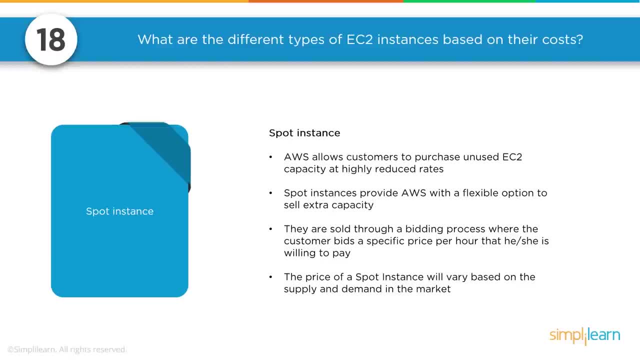 And the way we buy, spot instance, is we actually put a budget. This is how much I'm willing to pay. All right, Would you be able to give service within this cost? So, any time the price comes down and meets the cost that we have put in will be. 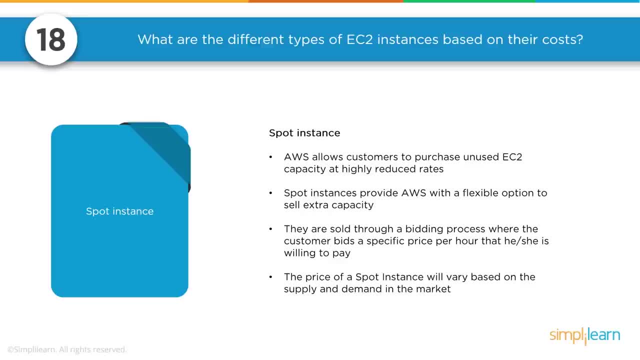 assigned an instance and any time the price shoots up the instance will be taken away from us. But in case of on demand instances, we have bought that instance for that particular hour and it stays with us. But with spot instances it varies based on the price. 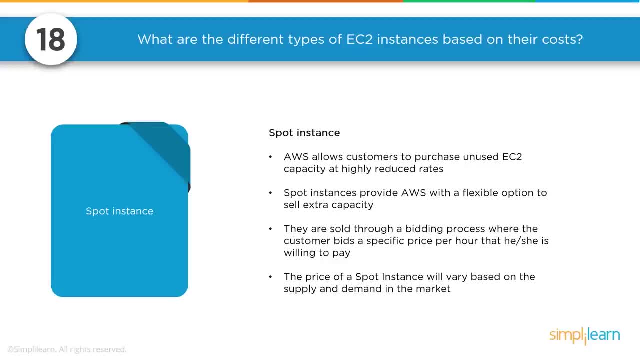 If you meet the price, you get the instance. If you don't meet, the price goes away to somebody else And the spot instance availability is actually based on supply And demand in the market. There's no guarantee that you will get spot instance at all time. 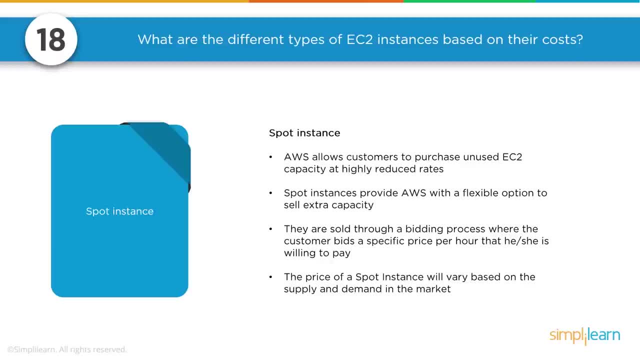 All right. So that's a caveat that you should be familiar with. That's a caveat that you should be aware when you are proposing somebody, that we can go for spot instance and save money. It's not always going to be available If you want your spot instance to be. 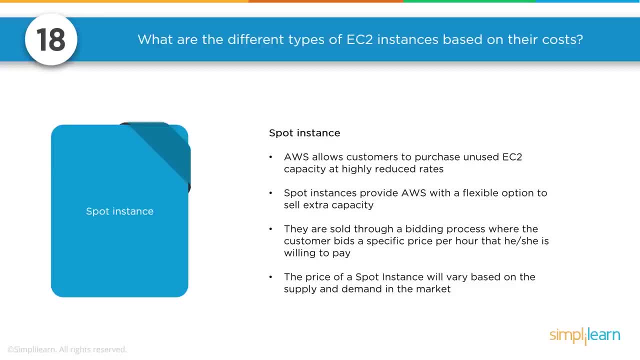 available to you, then we need to carefully watch the history of the price of the spot instance Now. how much was it last month and how much was it? How much is it this month? So how can I quote? How much can I quote Stuff like that? 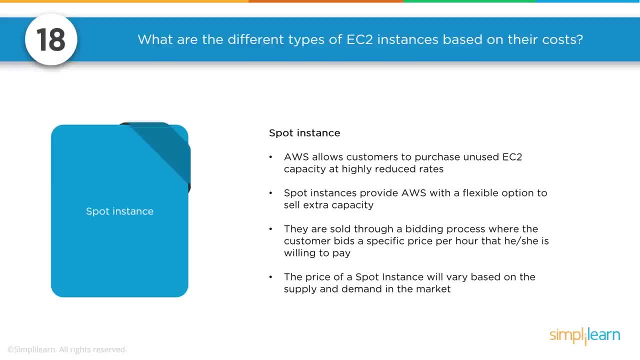 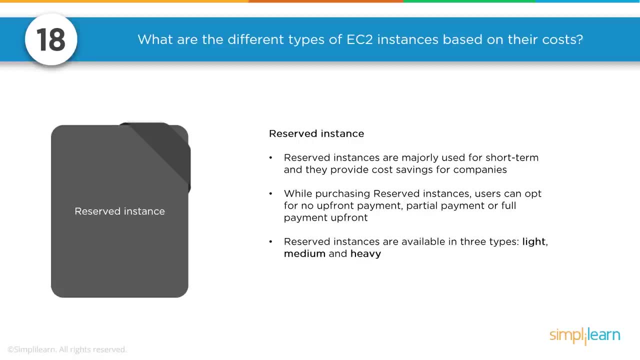 So you got to look at those history before you propose somebody that well, we're going to save money using spot instance. On the other hand, reserved instance provide cost savings for the company. We can opt for reserved instances for, you know, one year or three years. 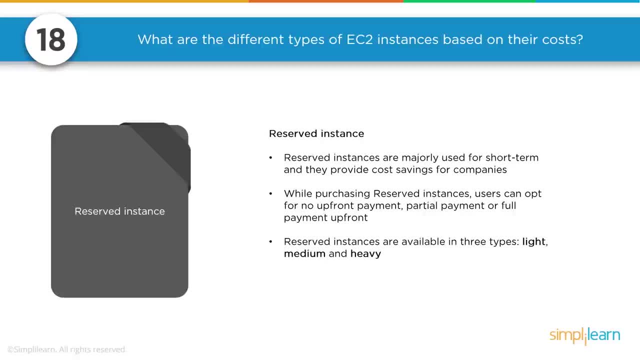 There are actually three types of reserved instances: light, medium and heavy reserved instances. They are based on the amount that we would be paying and cost benefit. The cost benefit also depends with reserved instance. The cost benefit also depends based on: are we doing all upfront or no upfront or 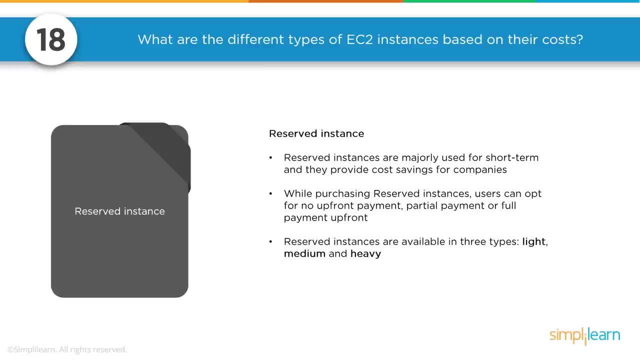 partial payment, then split the rest as monthly payments. So there are many purchase options available. But overall, if you're looking at using an application for the next one year and three years, you should not be going for on demand instance. you should be going for reserved instance. 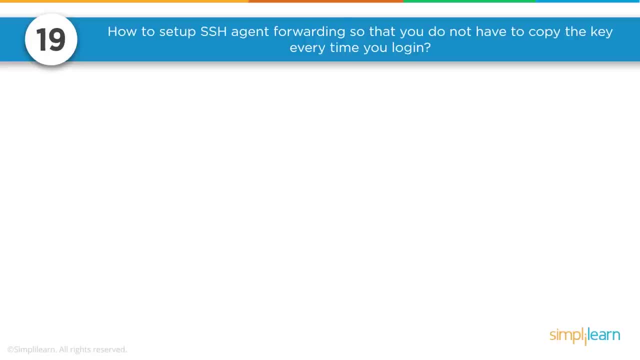 And that's what gives you the cost benefit. And in an interview you might be asked how you interact with the AWS environment. Are you using CLI, Are you using console? And depending on your answer- whether console or CLI- the panelist put a score. 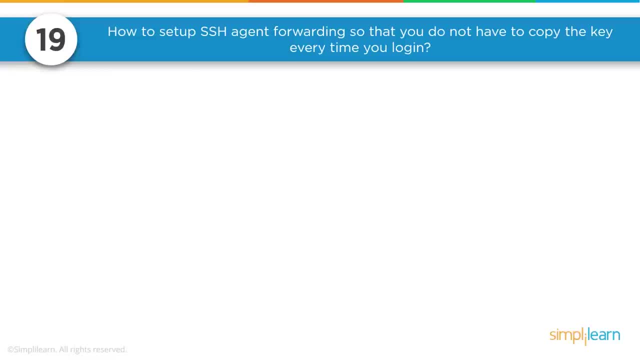 OK, this person is CLI specific, This person is console specific, or this person has used AWS environment through the SDK, stuff like that. So this question tests whether you are a CLI person or a console person. And the question goes like this: How do you set up SSH agent forwarding so that you do not? 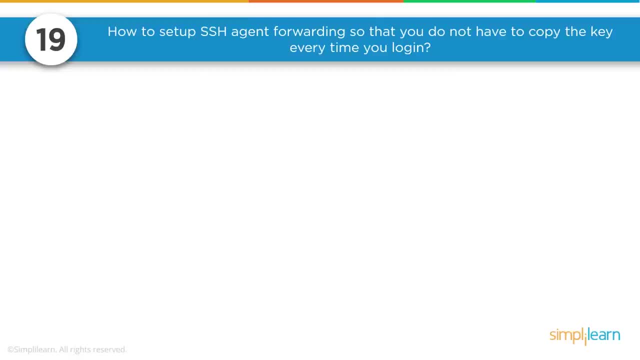 have to copy the key every time you log in If you have used Puri any time. if you want to log into an EC2 instance you will have to put the IP and the port number Along with that. you will have to map, or we will have to map the key in the Puri. 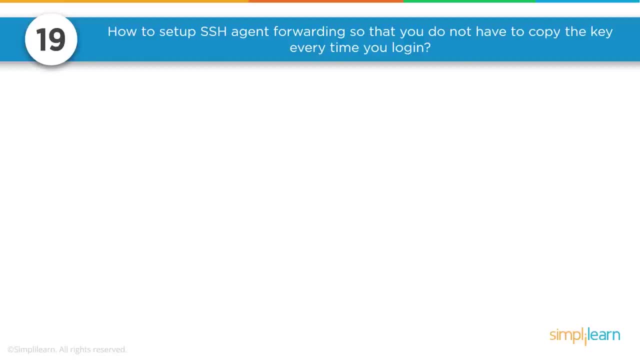 And this has to be done every time. That's what we would have done in our lab environments, Right, But in production environment, using the same key or mapping the same key again and again every time, it's actually a hassle. it's considered as a blocker. 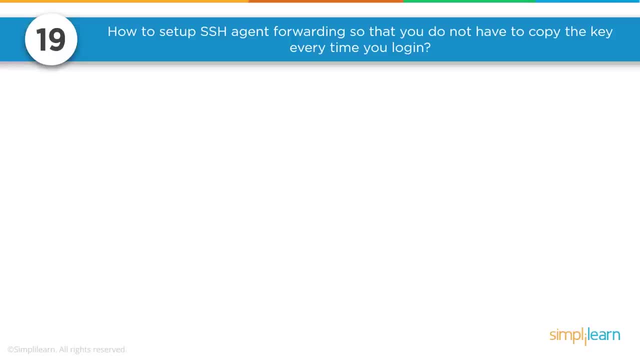 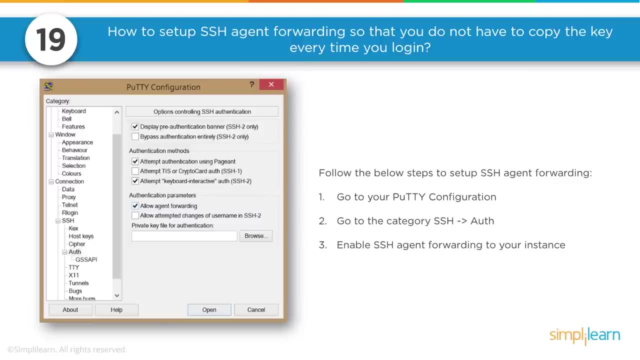 So you might want to cash it, you might want to permanently add it in your Puri session so you can immediately log in and start using it. So here, in the place where you would actually map the private key, there's a quick button that actually 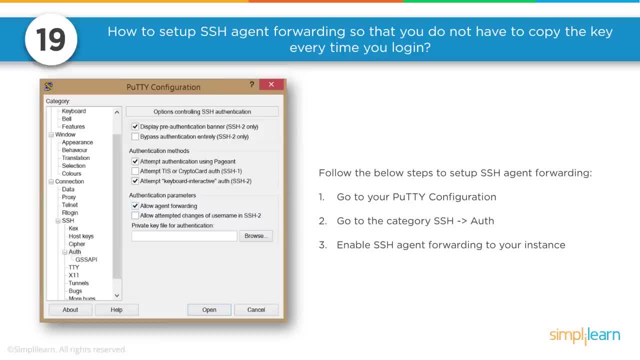 fixes or that actually binds your SSH to your Puri instance So we can enable SSH agent forwarding. that will actually bind our key to the SSH And next time when we try to log in you don't have to always go through mapping the key and trying to. 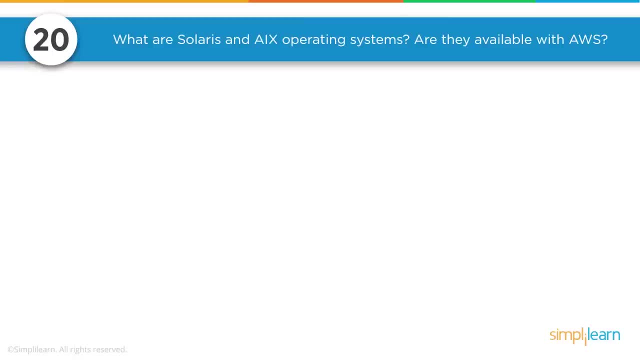 log in again or at this question: what are Solaris and AX operating systems? Are they available with AWS? That question generally gets asked to test: How familiar are you with the AMIs available? How familiar are you with EC2? How familiar are you with the EC2 hardwares available? that basically test that. 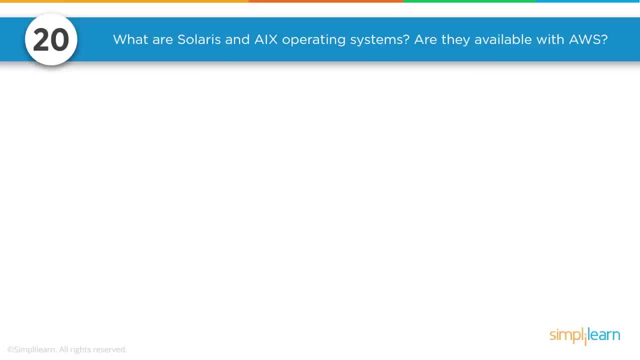 Now the first question or the first thought that comes to your mind is: well, everything is available with AWS. I've seen Windows, I've seen Ubuntu, I've seen Red Hat, I've seen Amazon, AMIs, And if I don't see my operating system there, I can always go to marketplace and try them. 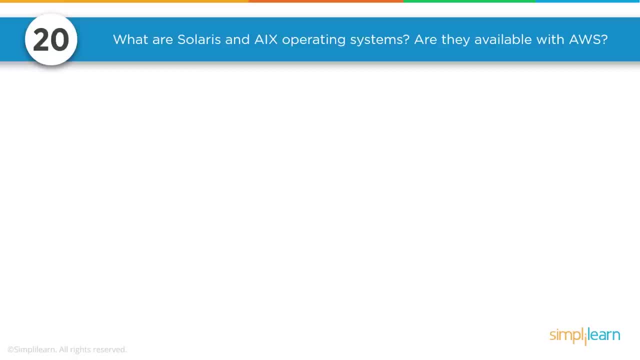 If I don't find a marketplace, I can always go to community and try them. So there are a lot of AMIs available. There are a lot of operating systems available. I will be able to find Solaris and AX, but that's not the case. 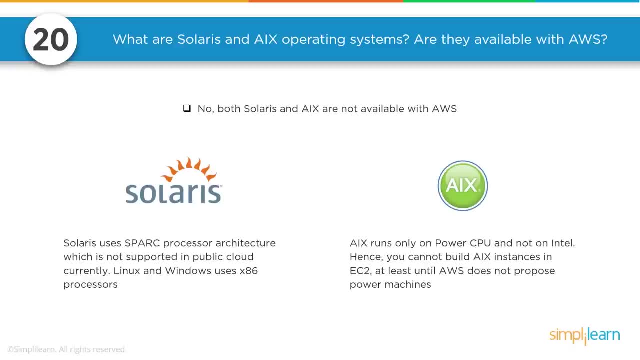 Solaris and AX are not available with AWS. That's because Solaris uses a different. I mean, Solaris does not support the architecture, does not support public cloud currently. The same goes for AX as well, And they run on power CPU and not on Intel. 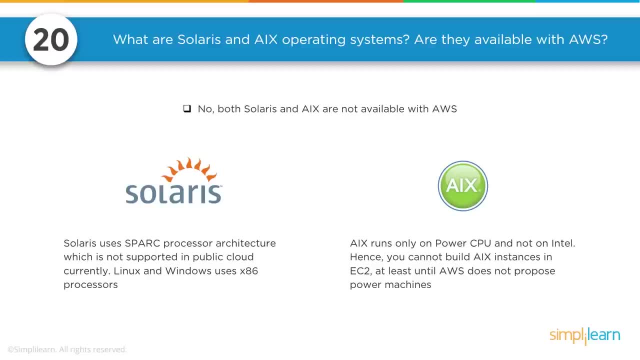 And, as of now, Amazon does not provide power machines. This should not be confused with HPC, which is high performance computing. Should not be confused with that. Now, these are different hardwares, different CPU itself that the cloud providers do not provide yet. 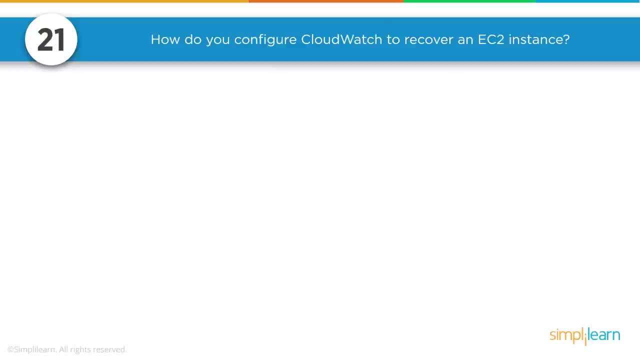 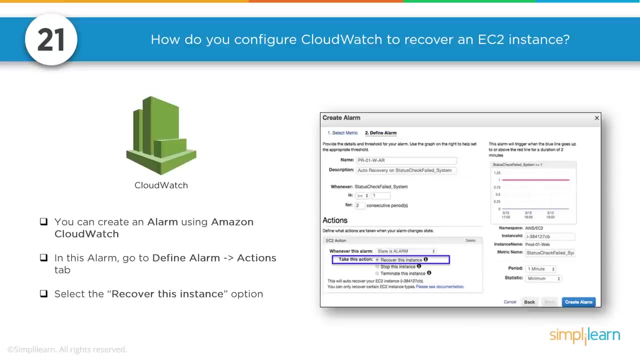 Another question you could get asked in organizations that would want to automate their infrastructure using Amazon native services would be: how do you actually recover an EC2 instance or auto recover an EC2 instance when it fails? Well, we know that EC2 instances are considered as immutable, meaning irreparable. 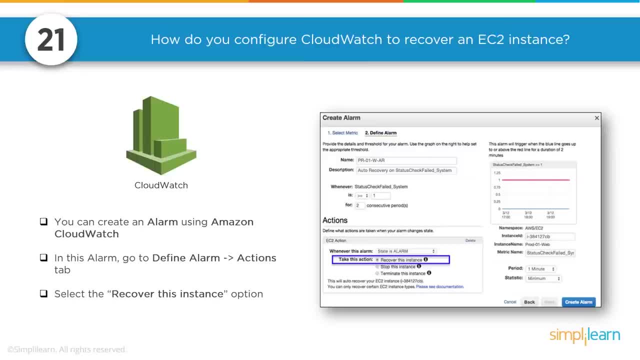 We don't spend time fixing bugs in an OS stuff like that. You know, once an EC2 instance crashes like it goes on an OS panic or there are various reasons why it would fail, We don't have to really worry about fixing it. 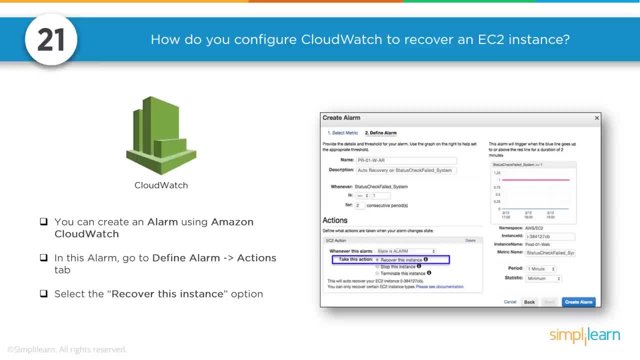 We can always relaunch that instance and that would fix it. But what if it happens at two o'clock in the night? What if it happens that during a weekend, when nobody's in office looking or monitoring those instances? So you would want to automate that, not only on a weekend or during midnights. 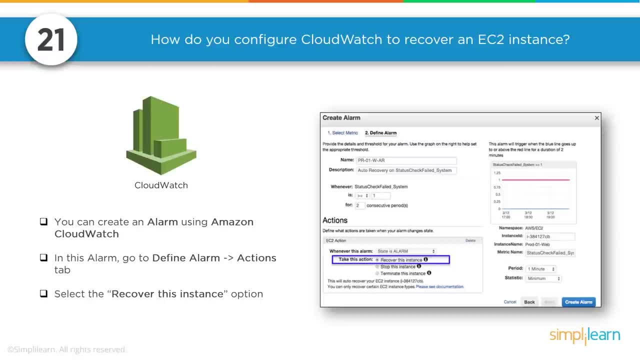 but it's general practice good to automate it. So you could face this question: How do you actually automate an EC2 instance once it fails? And the answer to that question is: using CloudWatch, we can recover the instance. So, as you see, there is an alarm threshold, a set in CloudWatch. 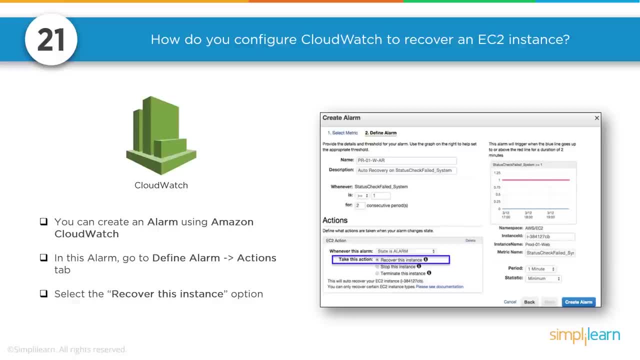 And once the threshold is met, meaning if there is an error, if there is a failure, if the EC2 instance is not responding for a certain while, we can set an alarm. And once the alarm is met, let's say the CPU utilization stayed high for five- 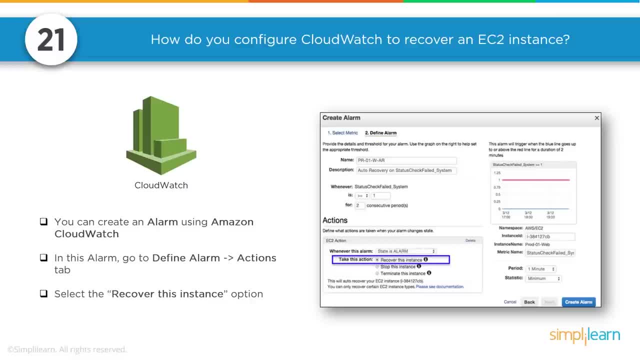 minutes. right, it's not taking any new connections, or the instance is not pinging for five minutes, Or in this case it's two minutes. It's not pinging so it's not going to respond connection. So in those cases you would want to automatically recover that EC2 instance. 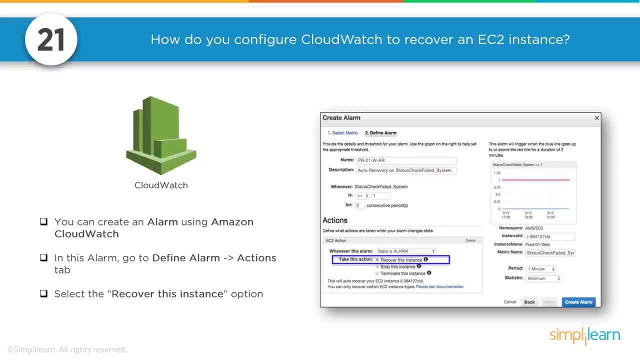 by rebooting the instance. All right, Now look at this. Take this action section under the action. So there we have a bunch of options like recover this instance, meaning reboot the instance. So that's how we would recover. The other two options are beyond the scope of the question. 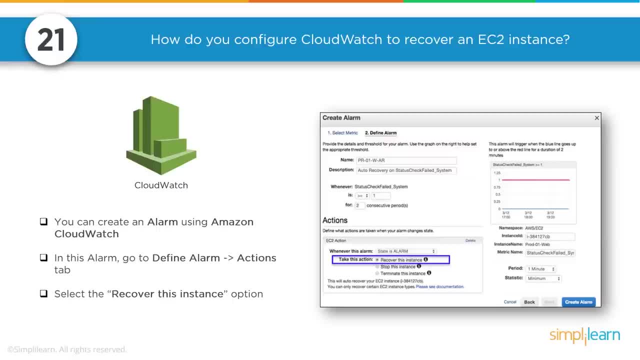 But still you can go ahead and fly, just like I'm going to do it. So the other option is: stop the instance. That's very useful when you want to stop instances that are having low utilizations. Nobody's using the system as of now. 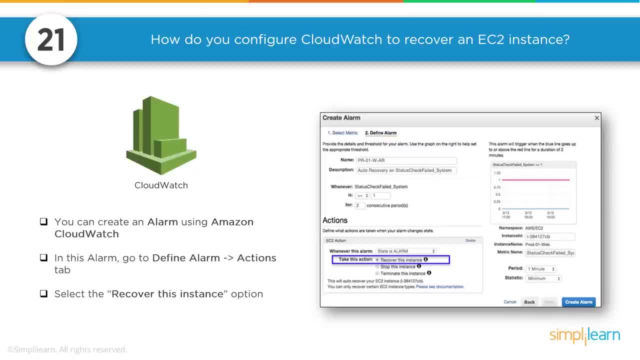 You don't want them to be running and wasting the cloud expenditure So you can actually set an alarm that stops the EC2 instance that's having low utilization. So somebody was working in an instance and they left it without or they forgot to shut down that instance. 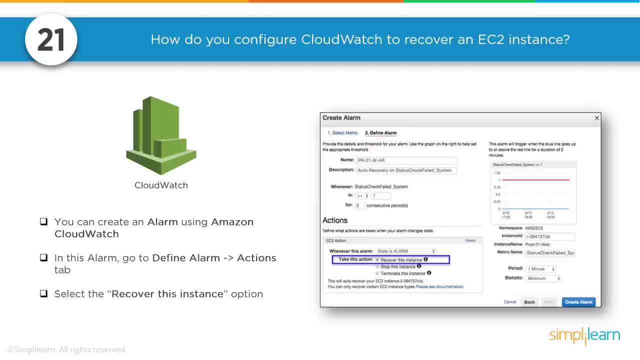 And it gets. I mean they will only use it again the next day morning. So in between there could be like 12 hours that the system is running idle, nobody's using it and you're paying for it. So you can identify such instances and actually stop them when the CPU 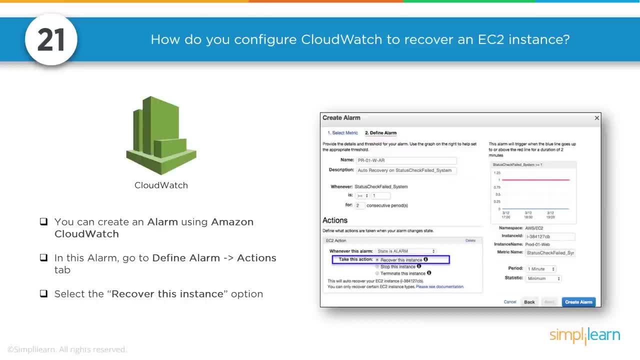 utilization is low, meaning nobody is using it. The other one is to terminate. Let's say you want to give system to somebody temporarily and you don't want them to hand the system back to you. All right, This is actually an idea. 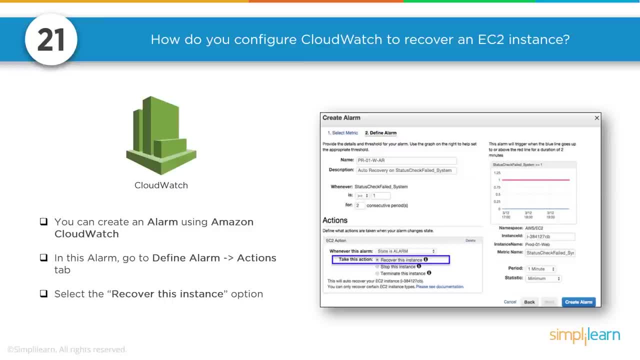 In other words, this is actually the scenario. So you hand over the system to somebody And when they're done, they're done. We can actually terminate the system. So you could instruct the other person to terminate the system when they're done. 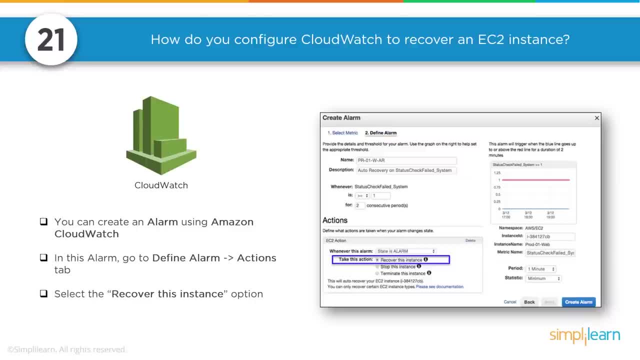 and they could forget and the instance could be running forever. Or you can monitor the system after the specified time is over and you can terminate the system. Or, best part, you can automate the system termination, So you assign a system to somebody and then turn on this CloudWatch action. 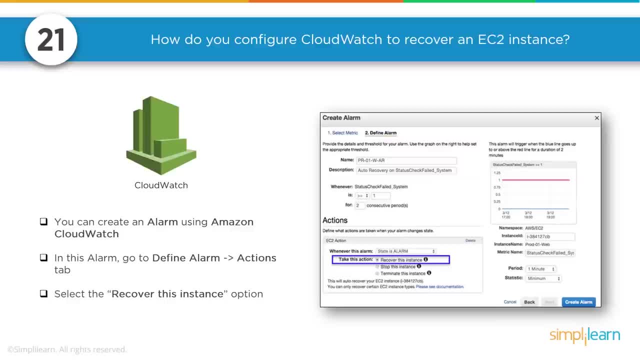 to terminate the instance when the CPU is low for like two hours, meaning they've already left, or CPU is low for 30 minutes, meaning they've already left, stuff like that. So that's possible. And if you're getting hired for a system side architect, or even on the sysop side, 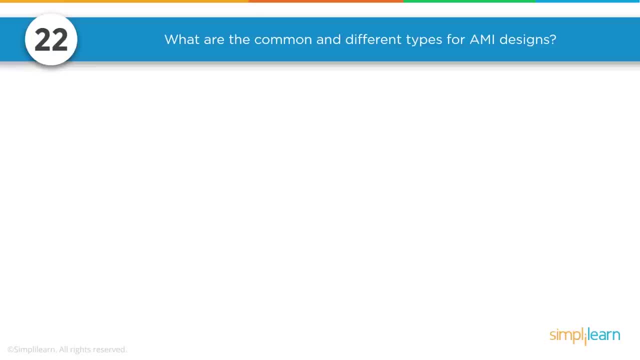 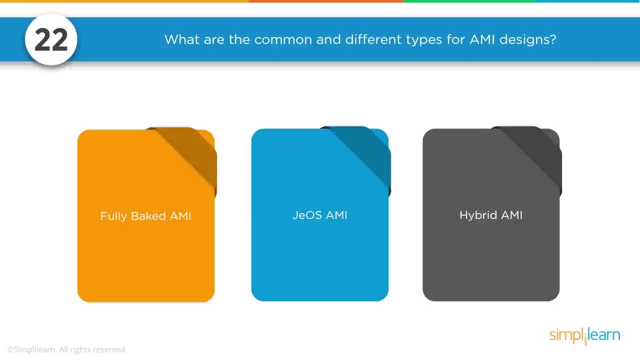 you could face this question: what are the common and different types of AMI designs? There are a lot of AMI designs. The question is the common ones and the difference between them. So the common ones are the full back AMIs and the other one is just enough. 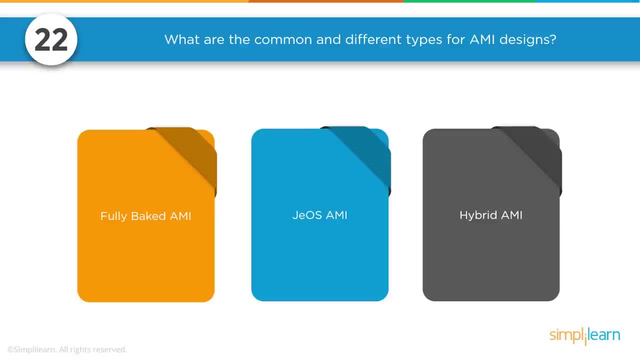 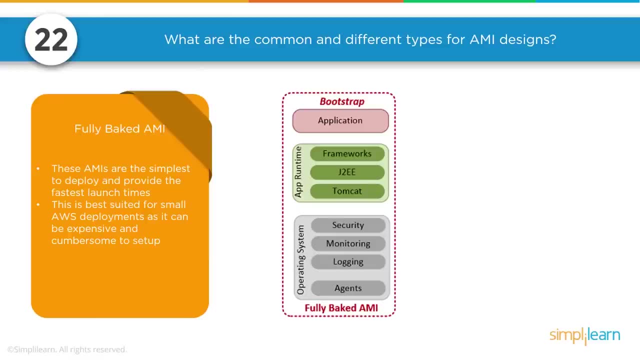 OS AMI, JE OS AMI, and the other one is hybrid type AMIs. So let's look at the difference between them. The full back AMI, just like the name says, it's fully baked. It's ready to use AMI. 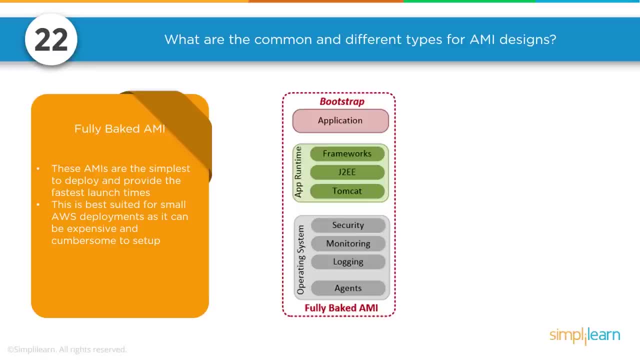 This is the simplest AMI to deploy, Can be a bit expensive. It can be a bit cumbersome because you'll have to do a lot of work beforehand. You could use the AMIs. a lot of planning, a lot of thought process will go into it and the AMI is ready to use. 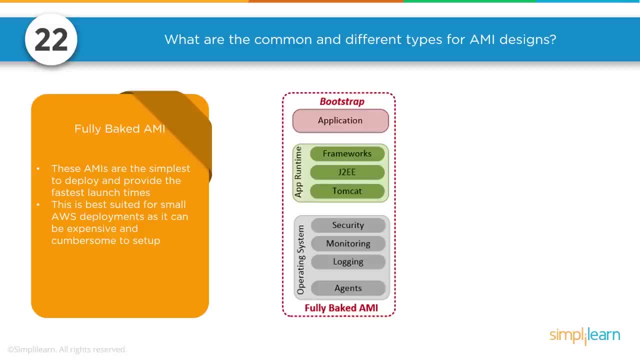 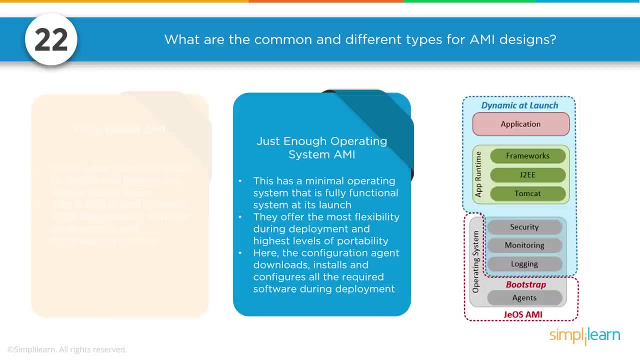 You hand over the AMI to somebody and it's ready to use. or if you want to reuse the AMI, it's already ready for you to use. So that's full baked AMI. The other one is just enough: operating system AMI, just like the name says. 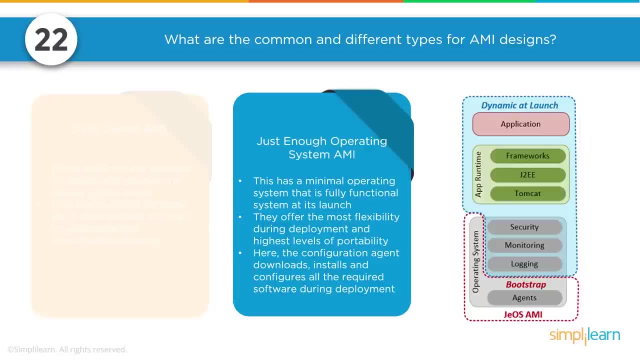 It has. I mean, as you can also see in the diagram or in the picture, it covers a part of the OS. all bootstraps are already packed properly and the security, monitoring, logging and the other stuff are configured at the time of deployment. 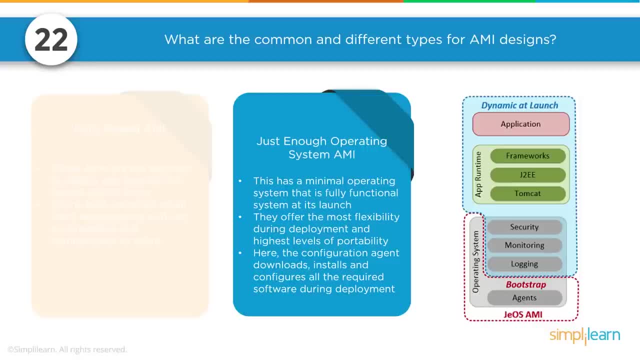 Or at the time you would be using it. So not much thought process will go in here. The only focus is on choosing the operating system and what goes the operating system- specific agents or bootstraps. that goes into the operating system. That's all we worry about. 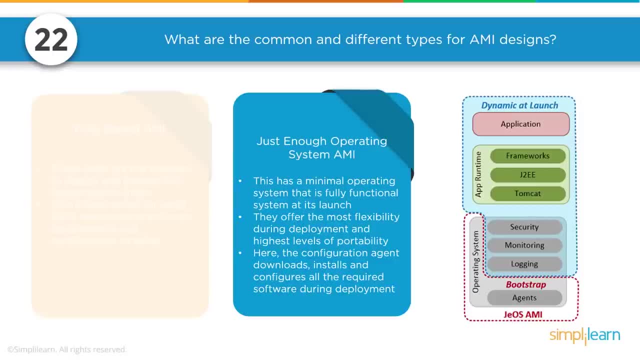 The advantage of this is it's flexible, meaning you can choose to install additional software at the time of deploying. But that's going to require an additional expertise on the person who will be using the AMI. So that's another overhead there. But the advantage is that it's kind of flexible. 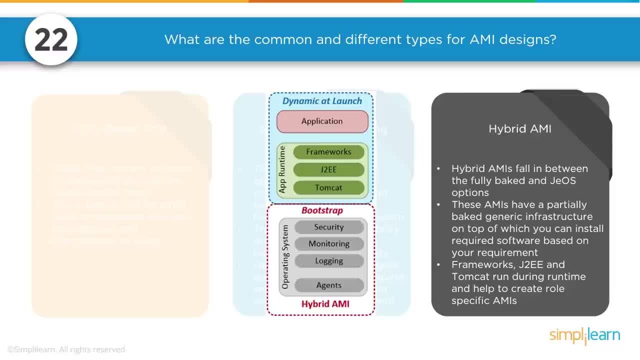 I can change the configurations during the time of deployment. The other one is a hybrid AMI. Now, the hybrid AMI actually falls in between the fully baked AMI and just enough operating system options. So these AMIs have some features of the baked type and some features of the just enough OS type. 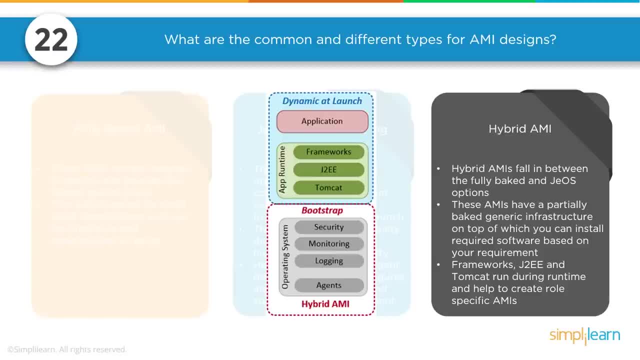 So, as you see, the security monitoring logging are packed in that AMI And the runtime environments are installed during the time of deployment. So this is where the strict company policies would go into the AMI. Company policies like, you got to log this, you got to monitor this. 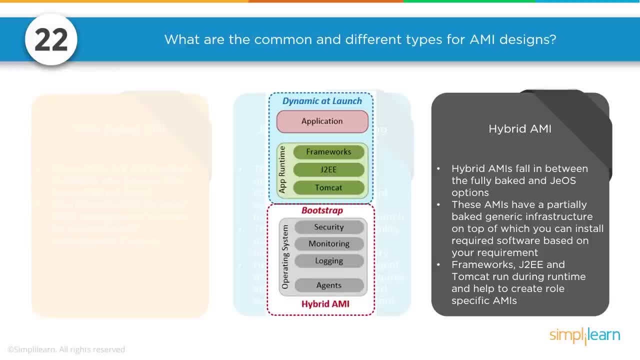 These are the ports that generally gets open in all the systems, stuff like that. So they strictly go into the AMI and sits in an AMI format and during deployment you have the flexibility of choosing the different runtime and the application that sits in an EC2 instance. 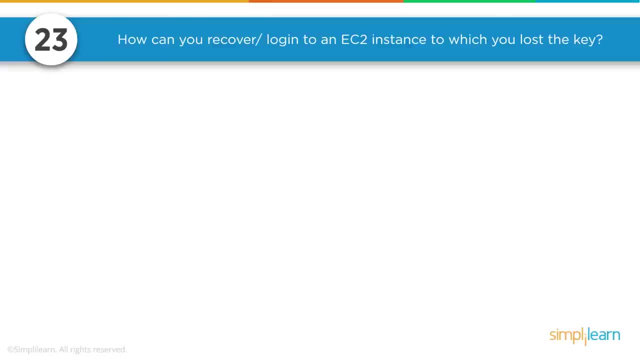 Another very famous question you would face in an interview is: how can you recover login to an EC2 instance to which you lost the key? Well, we know that if the key is lost, we can't recover it. There are some organizations that integrate their EC2 instances with an AD. 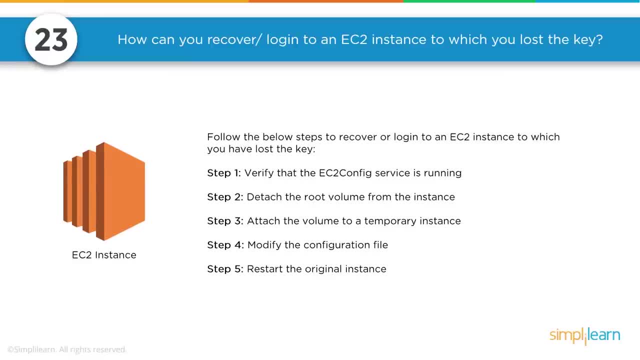 That's different. All right, So you can go and reset the password in the AD and you will be able to log into the new password. But here the specific, tricky question is: you are using a key to log in And how do you recover if you have lost the key? 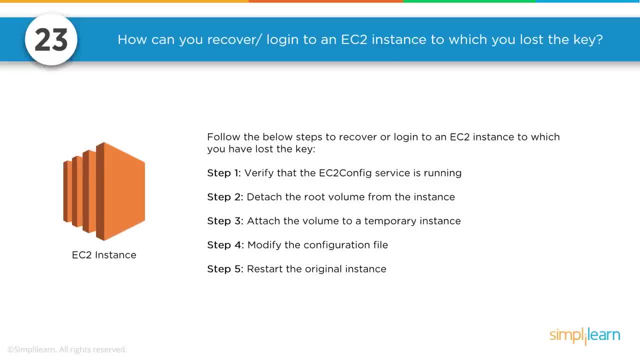 Generally companies would have made a backup of the key so we can pick from the backup. But here the specific question is: we have lost the key, Literally no backups on the key at all. So how can we log in? And we know that we can't log into the instance without the key present with us. 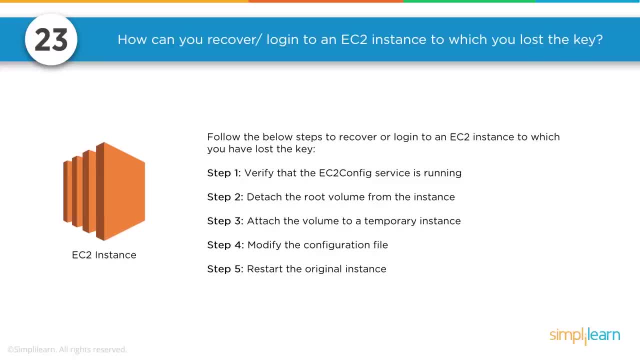 So the steps to recover is that make the instance use another key and use that key to log in. Once the key is lost, it's lost forever. We won't be able to recover it. You can't raise a ticket with Amazon, Not possible. 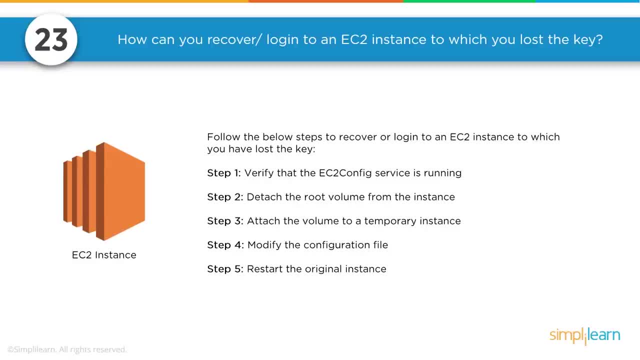 They're not going to help. It's beyond the scope, So make the instance use another key. It's only the key that's the problem. You still have valid data in it. You ought to recover the data. It's just the key that's having the problem. 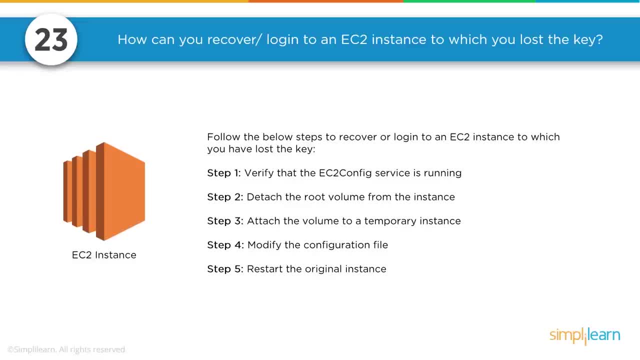 So we can actually focus on the key part alone and change the key, and that will allow us to log in. So how do we do it? Step by step procedure. So first verify the EC2 config service is running in that instance. If you want, you can actually beforehand install the EC2 config in that service, or 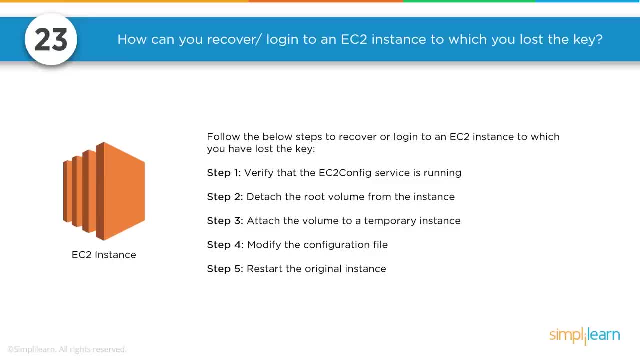 you can actually make the EC2 config run through the console. just a couple of button clicks and that'll make the EC2 config run in that EC2 instance and then detach the root volume for that instance. Of course it's going to require a stop and start. 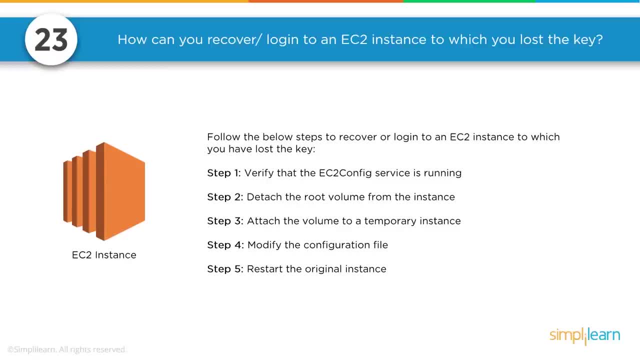 To detach the root volume from the instance. attach the root volume to another instance as a temporary volume- or it could be a temporary instance that you've launched only to fix this issue- and then log in to that instance and to that particular volume and modify the configuration file. 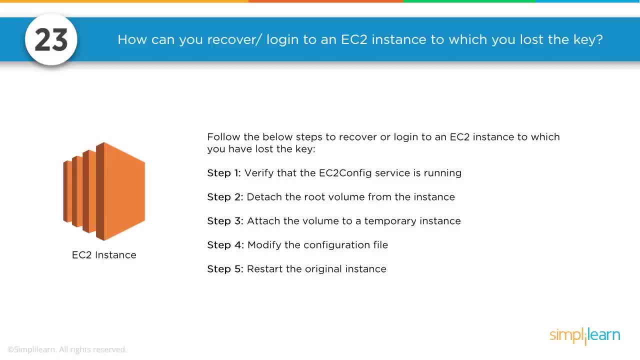 Modify it to use the new key and then move the root volume back to its original position and restart the instance. and now the instance is going to have the new key and you also have the new key with which you can log in. So that's how we go ahead and fix it. 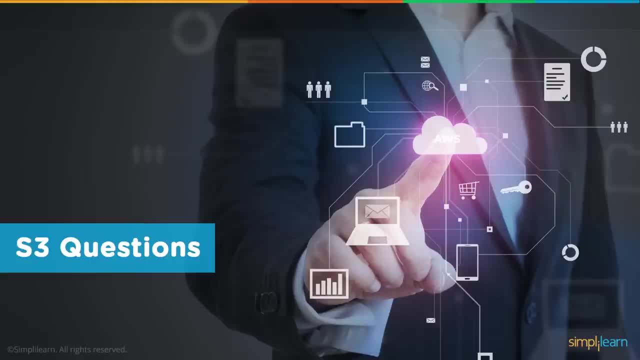 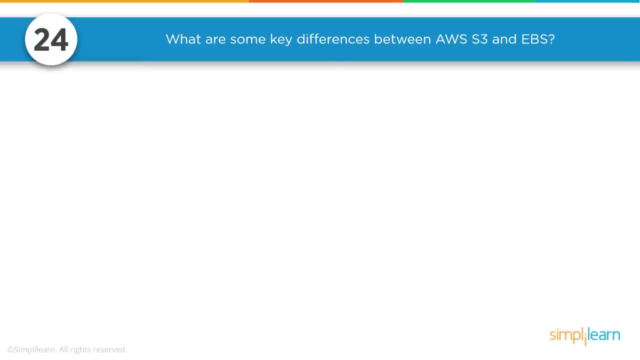 Now let's move on to some product specific or S3 product specific questions. A general perception is S3 and EBS can be used interchangeably and the interviewer would want to test What is your knowledge on S3 and EBS. Well, EBS uses S3. 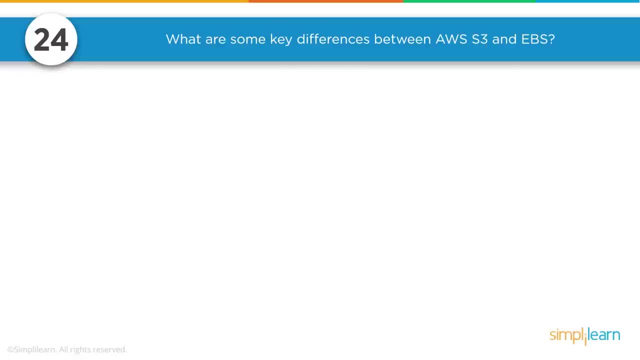 That's true, but they can't be interchangeably used. So you might face this question: What are some key differences between AWS, S3 and EBS? Well, the differences are: S3 is an object store, meaning you can't install anything. 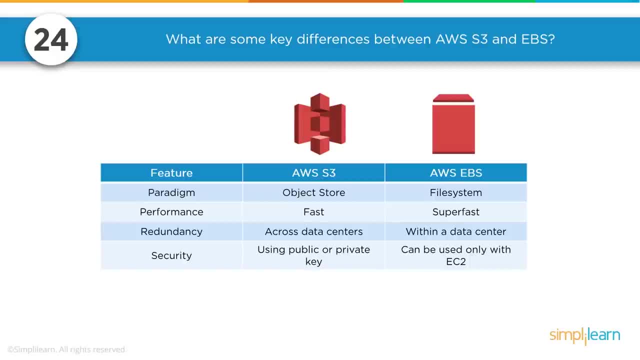 in it You can store drive files, but you can't actually install in it. It's not a file system, but EBS is a file system. You can install services- I mean install applications- in it, and that's going to run. 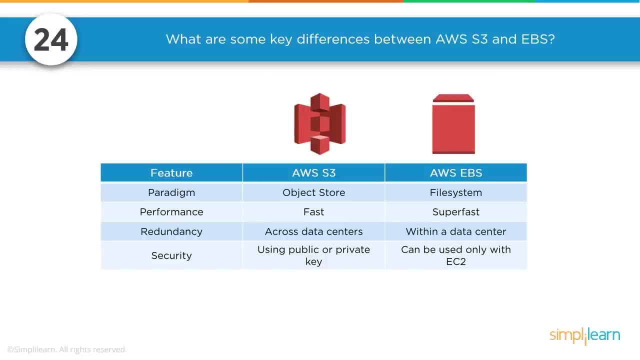 stuff like that. And talking about performance, S3 is much faster and EBS is super faster when accessing from the instance, because from the instance, if you need to access S3, you'll actually have to go out through the Internet and access the S3 or S3 is an external service, a very external. 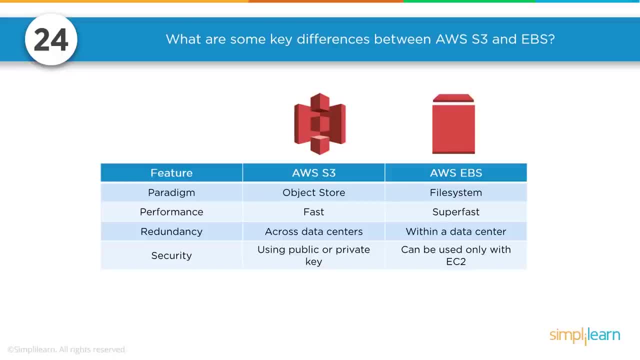 service that you'll have to go through or you'll have to go outside of your VPC to access S3.. S3 does not come under a VPC, but EBS comes under a VPC. It's on the same VPC. 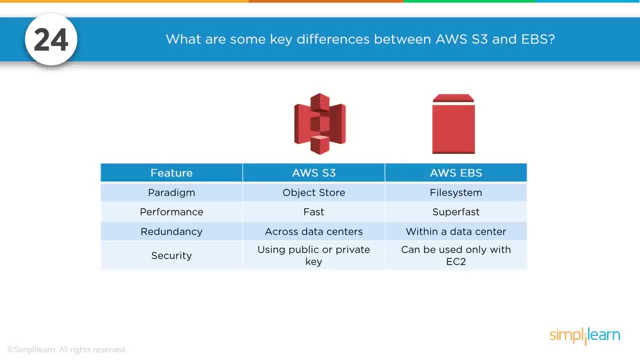 So you would be able to use it kind of locally compared to S3. EBS is very local, so that way it's going to be faster And redundancy. talking about redundancy of S3 and EBS, S3 is replicated. The data in S3 is replicated across the data centers, but EBS is replicated. 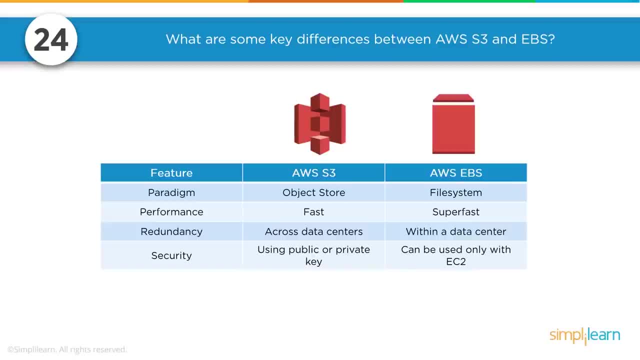 within the data center, meaning S3 is replicated across availability zones. EBS is within an availability zone, so that way redundancy is a bit less in EBS. In other words, redundancy is higher in S3 than EBS. And talking about security of S3, S3 can be made private as well as public. 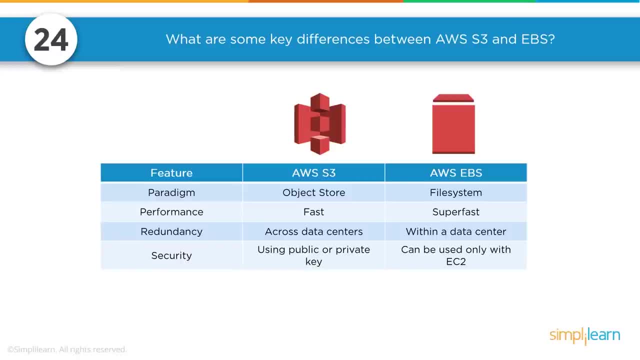 meaning anybody can access S3 from anywhere in the Internet. That's possible with S3. But EBS can only only be accessed when attached to an EC2 instance. Just one instance can access it, whereas S3 is publicly directly accessible. 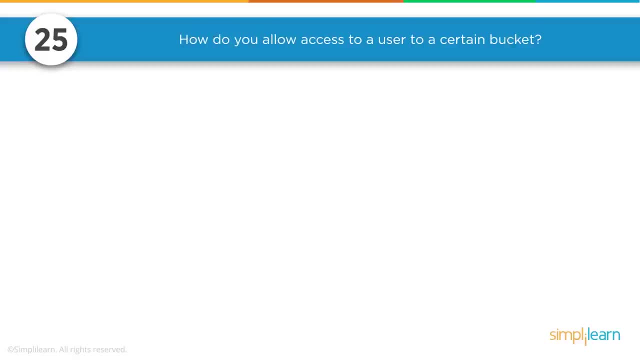 The other question related to S3 security is: how do you allow access to a user to a certain a user to a certain bucket, which means this user is not having access to S3 at all, but this user needs to be given access to a certain bucket. 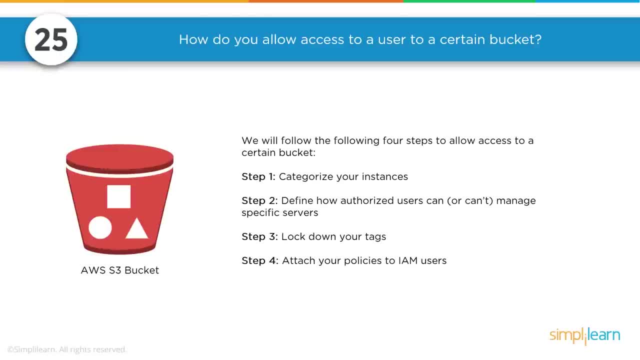 How do we do it? The same case applies to servers as well. In a few cases there could be an instance where a person is new to the team and you actually don't want them to access the production service. Now he is in the production group and by 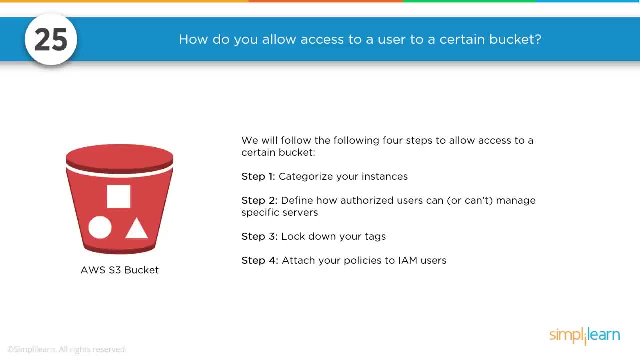 default, he or she is granted access to that server, But you specifically want to deny access to that production server till the time he or she is matured enough to access or understand the process, understand the do's and don'ts before they can put their hands on the production server. 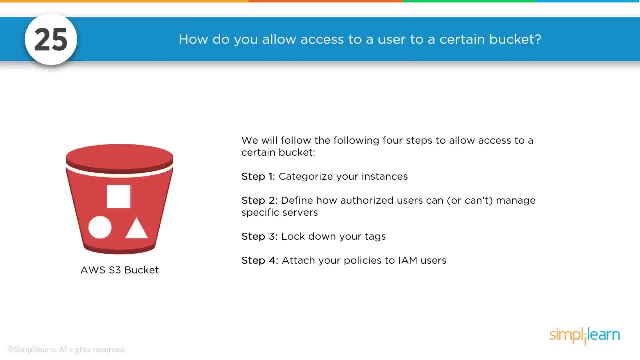 So how do we go about doing it? So first we would categorize our instances- Well, these are critical instances, These are normal instances, and we would actually put a tag on them. That's how we categorize. So you put a tag on them, put a tag saying: well, they are highly critical. 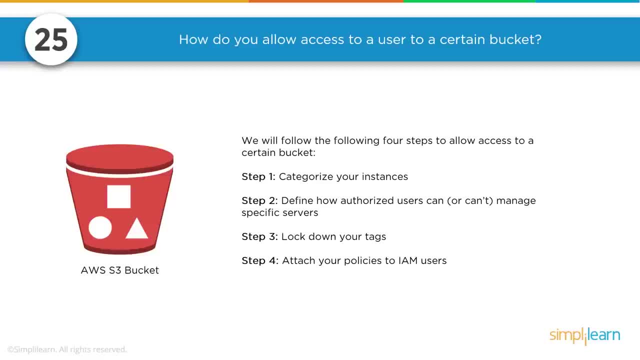 They are medium critical and they are not critical at all. Still they're in production Stuff like that- And then you would pick the users- who wants to or who should be or should not be given access to a certain server And you would actually allow the user to. 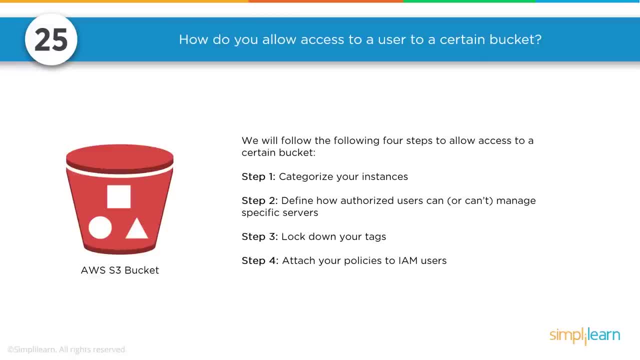 access or not access servers based on a specific tag. In other words, you can use actually tags. In the previous step we put tags on the critical server Right, So you would define that this user is not going to use this tag. 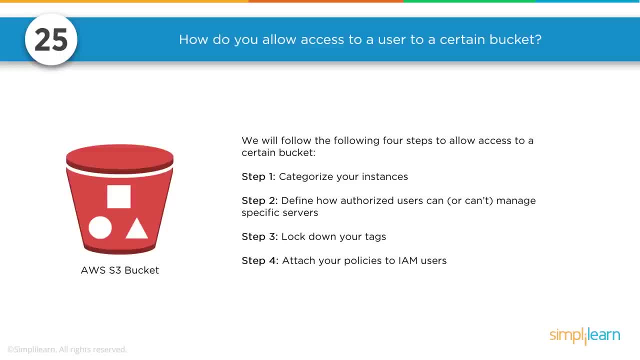 This user is not allowed to use the resources with this tag. So that's how you would make your step forward. So you would allow or deny based on the tags that you have put. So in this case, he or she will not be allowed to servers which are tag critical servers. 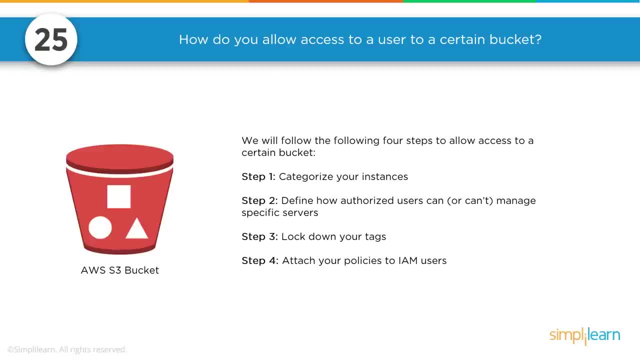 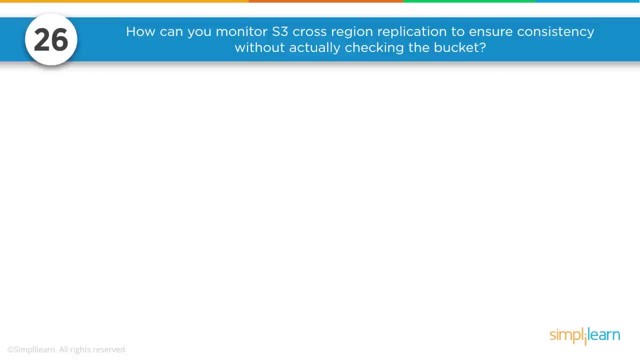 So that's how you allow, deny access to them, And the same goes for bucket as well. If an organization is excessively using S3 for their data storage because of the benefit that it provides, the cost and the durability, you might get asked this question, which is organizations would replicate. 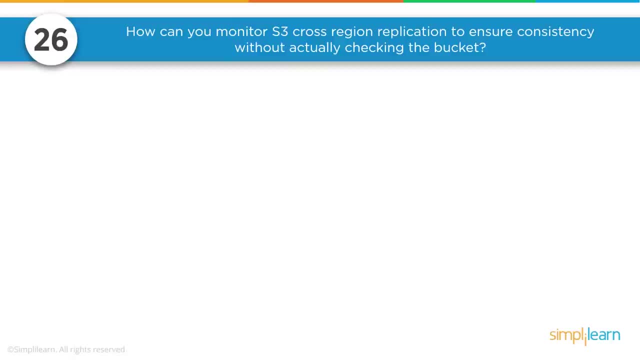 the data from one region to another region for additional data durability and for having data redundancy. not only for that, they would also do that for DR purposes, for disaster recovery. if the whole region is down, you still have the data available somewhere else and you can pick and use it. 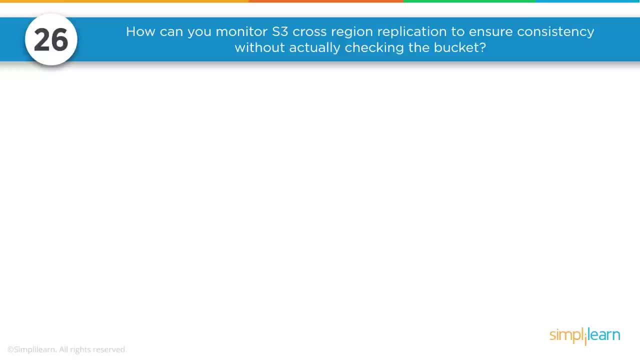 Some organizations would store data in different regions for compliance reasons, to provide low latency access to their users who are local to that region, Stuff like that. So when companies do replication, how do you make sure that there is consistency in the replication? how do you make sure that the replication 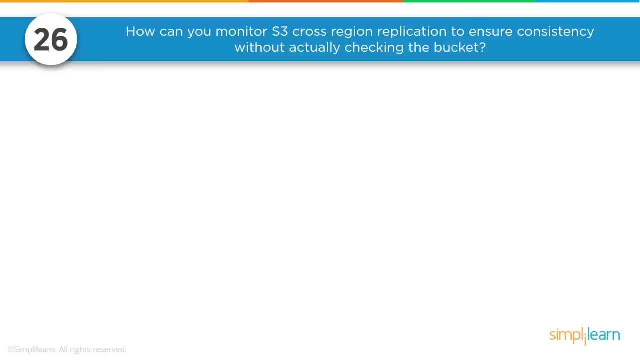 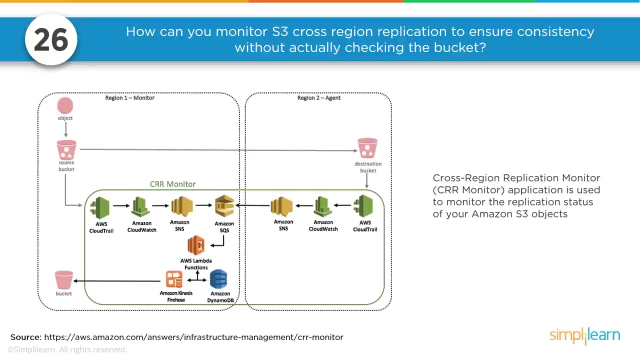 is not failing and the data gets transferred for sure, And there are logs for that replication. This is something that the companies would use where they are excessively using S3 and they're fully relying on the replication in running their business. And the way we could do it is we can set up a replication monitor. 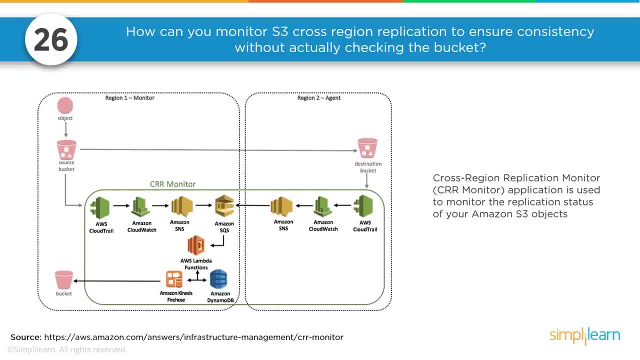 It's actually set of tools that we could use together to make sure that the cloud replication- region level replication- is happening properly. So this is how it happens now on this side: on the left hand side we have the region one and on the right hand side we have region two and region. 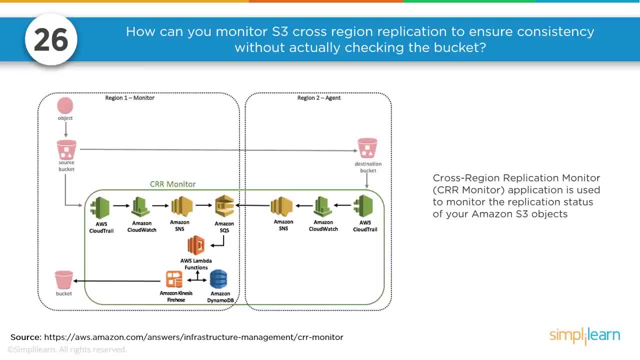 one is the source bucket and region two is the destination bucket Right. So object is put in the source bucket and it has to go directly to the region two bucket or made a copy in the region two bucket. And the problem is sometimes it fails and there is no. 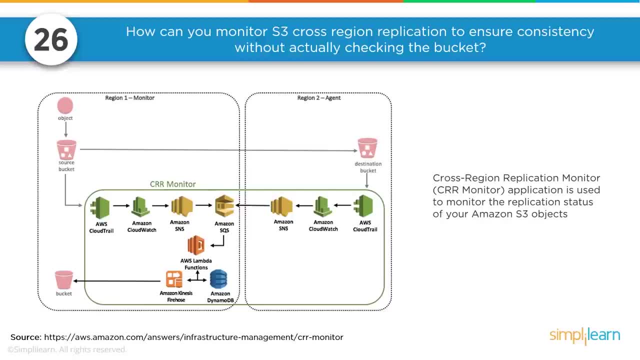 consistency between them. So the way you would do it is connect these services together and create an cross replication or cross region replication monitor that actually monitors, that actually monitors your environment. So there are cloud watch that make sure that the data is moved. No data is failing. 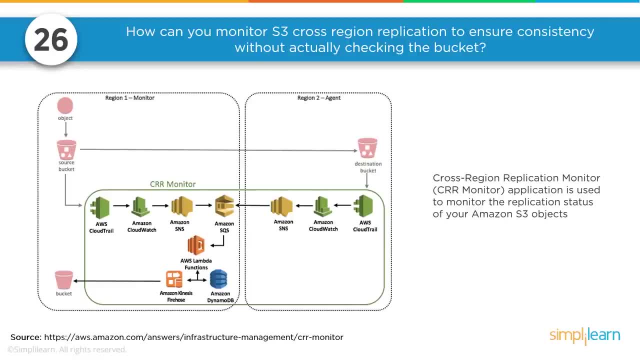 Again, there's cloud watch on the other end. Make sure that the data is moving, And then we have the logs generated through CloudTrail and that's actually written in DynamoDB And if there is an error, if something is failing, you get notified. 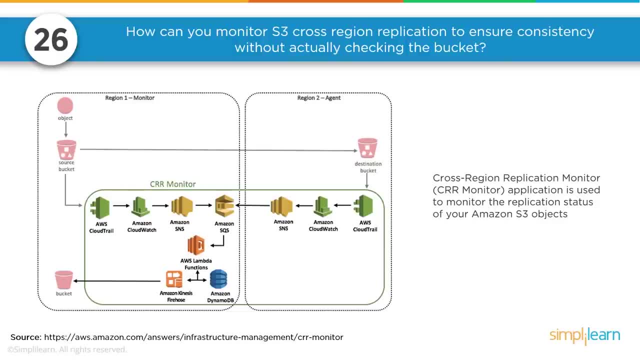 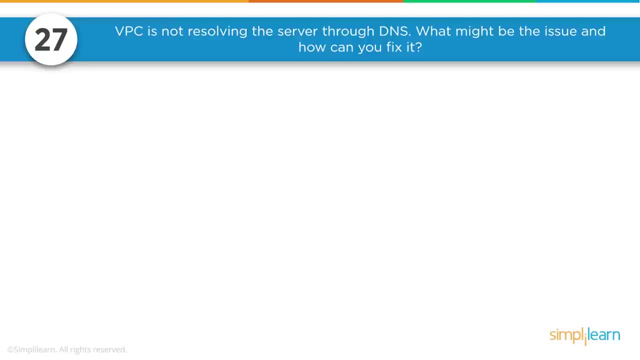 through an SMS or you get notified through an email using the SNS service. So that's how we could leverage these tools and set up and cross region replication monitor that actually monitors your data replication. Some common issues that company companies face in VPC is that we all know that. I 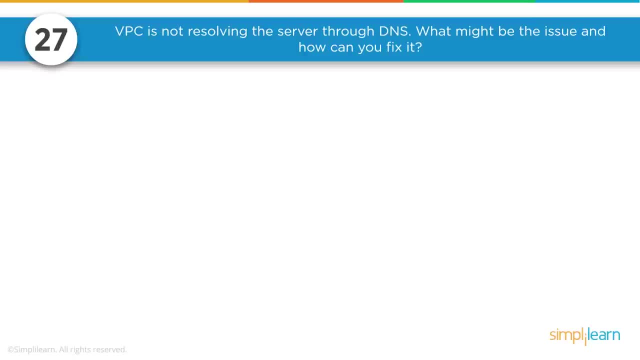 can use Route 53 to resolve an IP address externally from the Internet, But by default the servers won't connect to the other servers using our custom DNS name. That does not do that by default, So it's actually a problem. There are some additional things that as 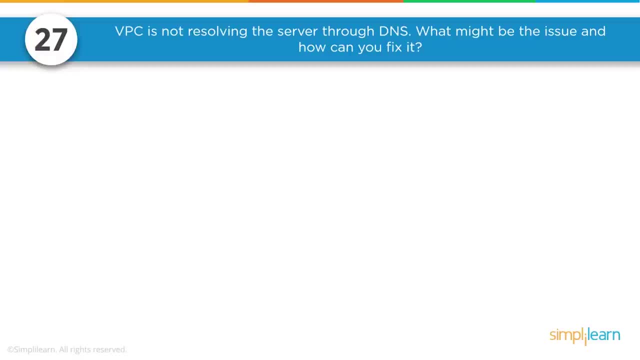 an administrator or as an architect or as a person who uses it, you will have to do, And that's what we're going to discuss. So the question could be: VPC is not resolving the server through the DNS. You can access it through the IP, but not through the DNS name. 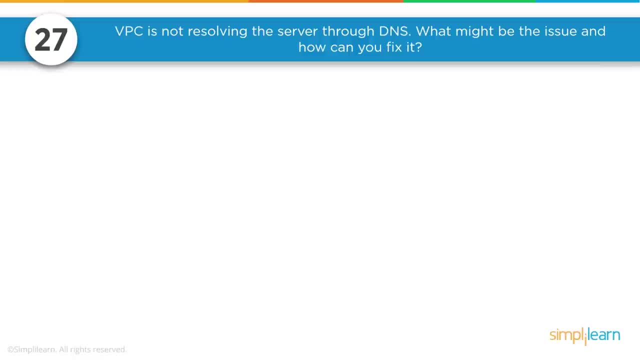 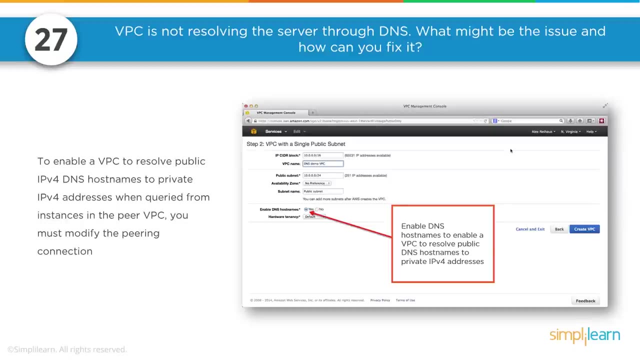 And what could be the issue and how do you go about fixing it. And you will be able to answer this question only if you have done it already. It's a quick and simple step. By default, VPC does not allow. that's the default feature. 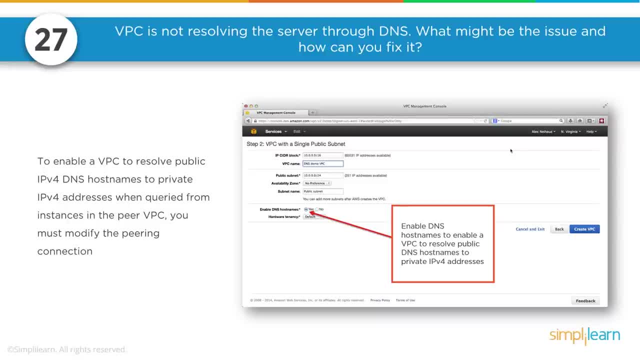 And we will have to enable the DNS host name resolution before Now. this is for the custom DNS, not for the default DNS that comes along. This is for the custom DNS, So we will have to enable the DNS host name resolution. So we'll have to enable the DNS host name resolution. 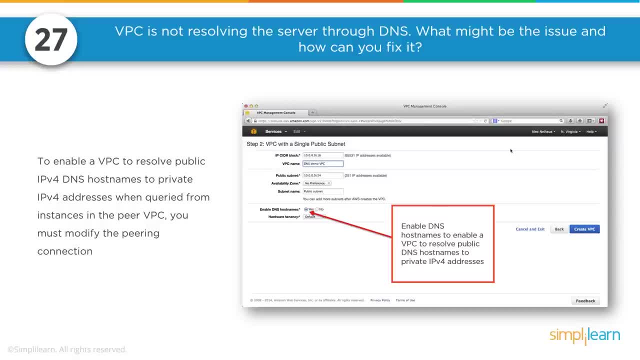 So they actually resolve. Let's say I want to connect to a server one dot simply learn dot com. by default It's not allowed, But if I enable this option, then I will be able to connect to server one simply learn dot com. 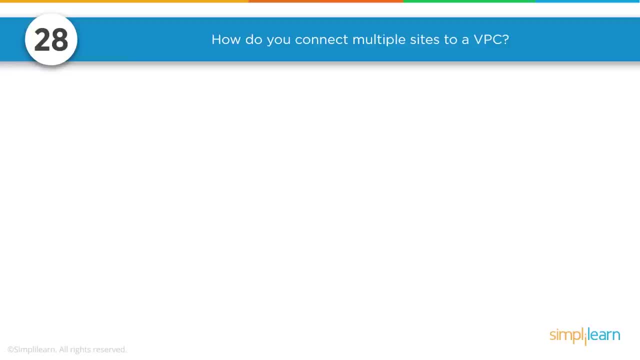 If a company has VPCs in different regions and they have a head office in a central place and the rest of them are branch offices and they are connecting to the head office for access or, you know, for saving data or for accessing certain files or certain data or storing data. 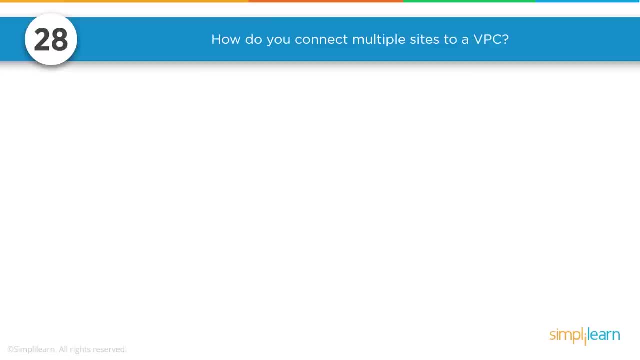 All right. So they would actually mimic the hub and spoke topology where you have the VPC which is centrally in an accessible region, a centrally accessible region, And then you would have a local VPCs or branch offices in different other regions and they get connected to the VPC in the central location. 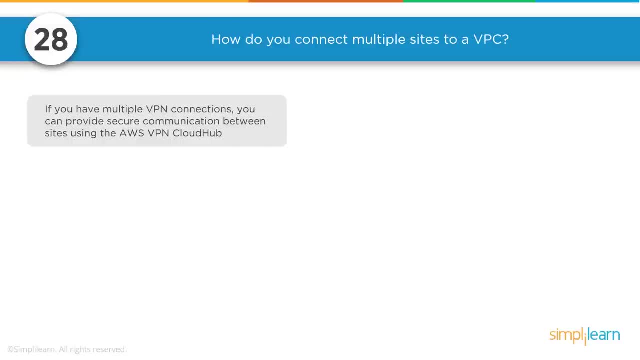 And the question is: how do you actually connect the multiple sites to a VPC and make communication happen Between them? By default, it does not do that. We know that VPCs- they need to be paired between them in order to access the resources. 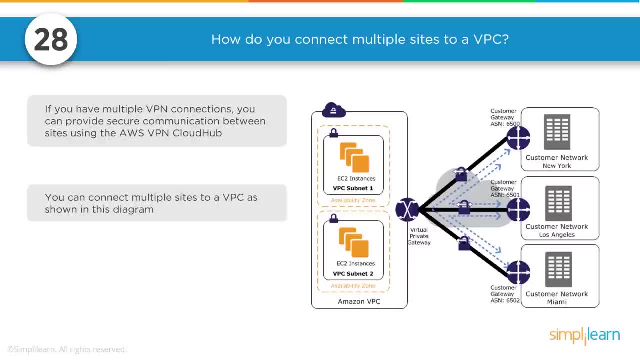 Let's look at this picture. So I have like a customer network or branch offices in different parts and they get connected to a VPC. that's fine. So what we have achieved is those different offices, the remote offices. they are connecting to the VPC and they're talking, but they can't connect, or they. 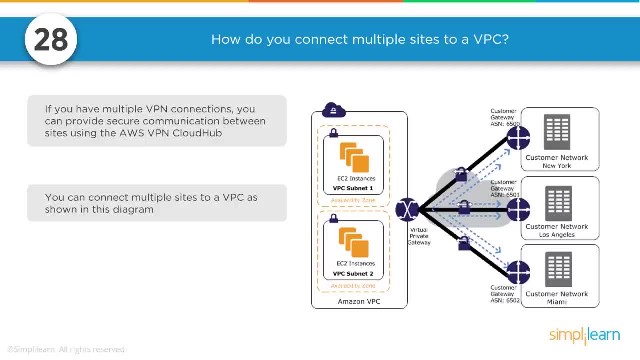 can't talk to each other. That's what We have built, But the requirement is the traffic needs to, or they should be able to talk to each other, but they should not have a direct connection between them, which means that they will have to come and hit the VPC and then reach the other. 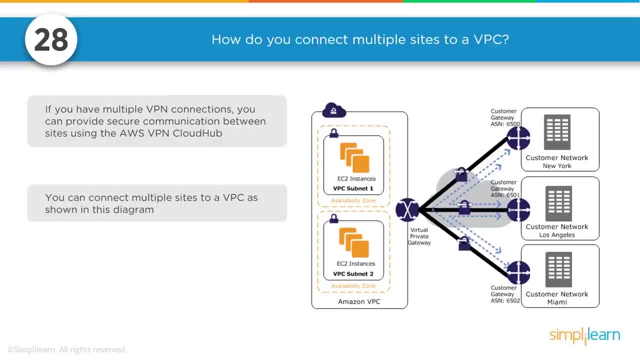 customer network which is in Los Angeles or which is in New York. That's the requirement, So that's possible with some architecting in the cloud. So that's using VPN Cloud Hub- You look at this dotted lines- which actually allows customers or 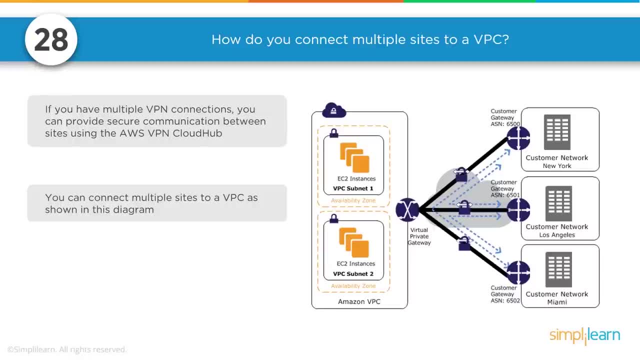 which actually Allows the corporate networks to talk to each other through the VPC. Again, by default, it doesn't happen. Cloud Hub is an architecture that we should be using to make this happen, And what's the advantage of it as a central office or as the headquarters? 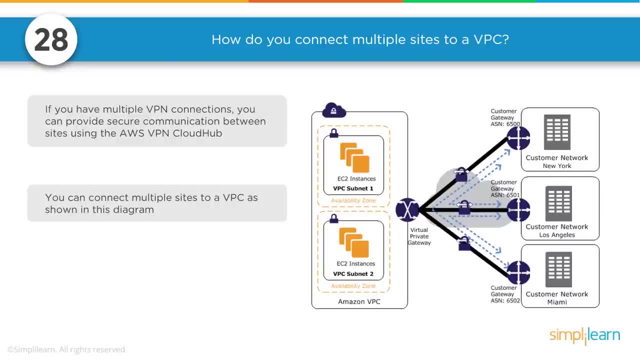 office, which is in the VPC, or headquarters data center, which is in the VPC. You have control, or the VPC has control, on who talks to who and what traffic can talk to and what traffic can be routed to the other head office, stuff like that. 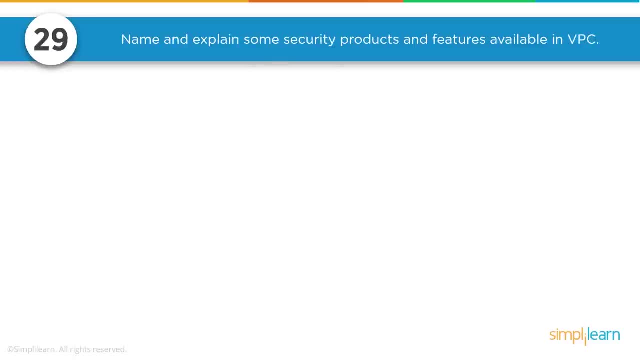 That centralized control is on the VPC. The other question you could get asked is name and explain some security products and features available in the VPC. Well, VPC itself is a security service. It provides security service to the application. But how do you actually secure the VPC itself? 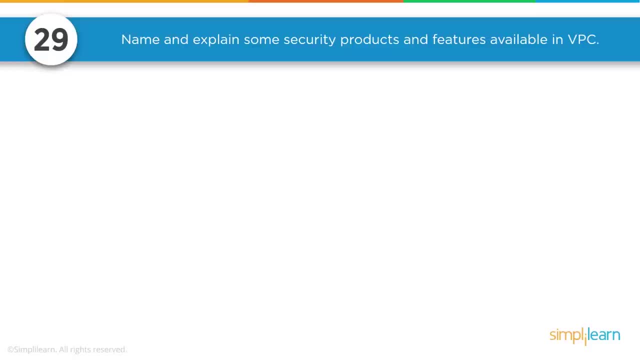 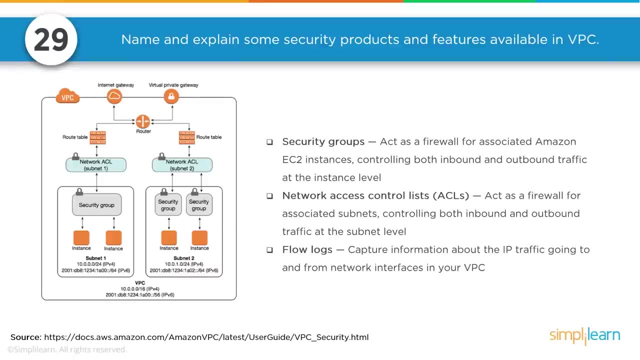 That's the question. And yes, there are products that can actually secure the VPC, or the VPC delivers these products to secure the application. Access to the VPC is restricted through a network access control list, Right, So that's a security product in VPC. 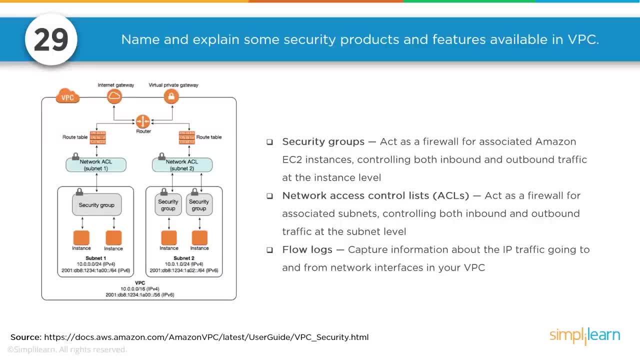 And a VPC has security groups that protects the instances from unwanted inbound and outbound traffic. A network access control list protects the subnets from unwanted inbound and outbound access And there are flow logs we can capture in VPC. that captures incoming and outgoing traffic through a VPC which will be used for later analysis, as in what's. 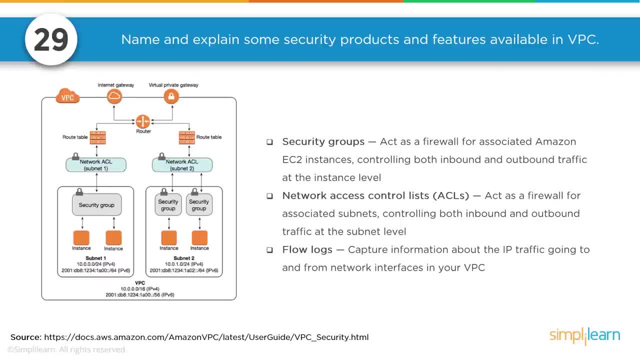 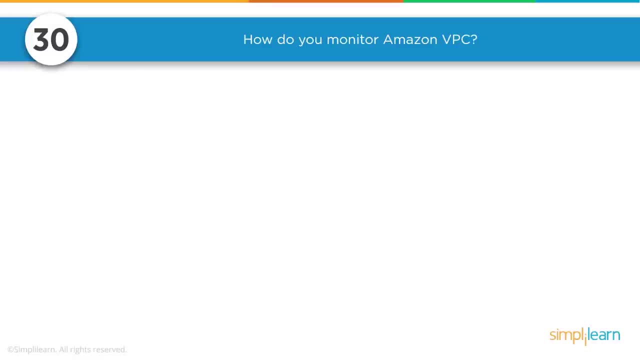 the traffic pattern, what's the behavior of the traffic pattern, stuff like that. So there are some security products and features available in VPC. Now how do you monitor VPC? VPC is a very important concept, very important service as well. 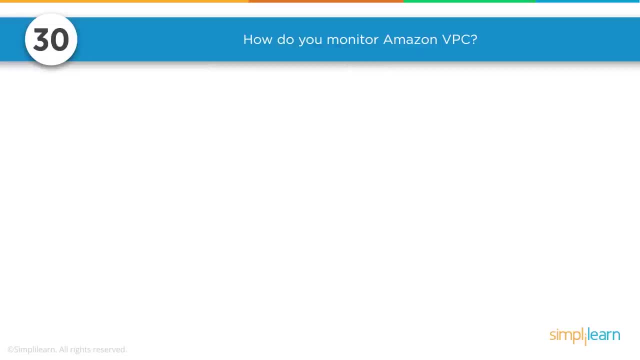 Everything sits in a VPC. Most of the service sits in a VPC, except for Lambda and S3 and DynamoDB and a couple of other services. Most of them sit in a VPC For security reasons. So how do you monitor your VPC? 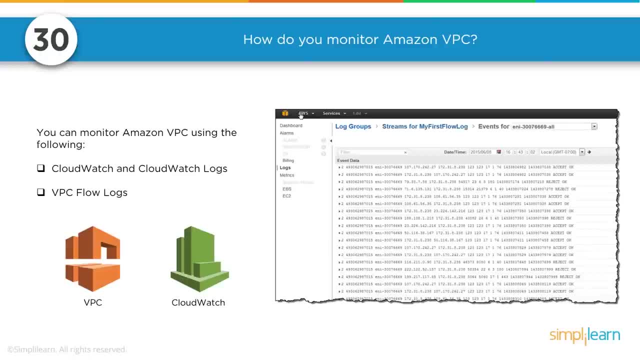 How do you gain some visibility on your VPC? Well, we can gain visibility on a VPC using VPC flow log. That's the basic service. As you see, it actually captures what's allowed, what's not allowed, stuff like. 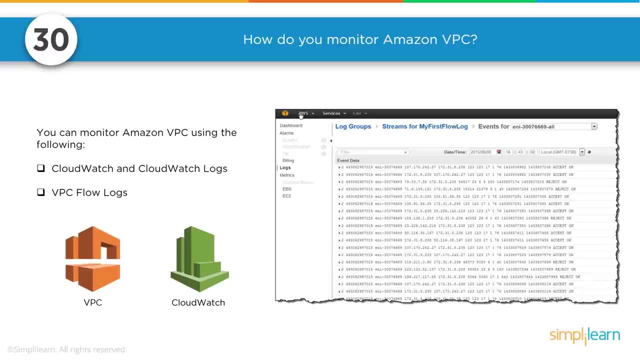 that which IP is allowed, which IP is not allowed, stuff like that. So we can gather it and we can use that for analysis. And the other one is CloudWatch, and CloudWatch logs The data transfer that happens. So this is who gets allowed and who does not get allowed. 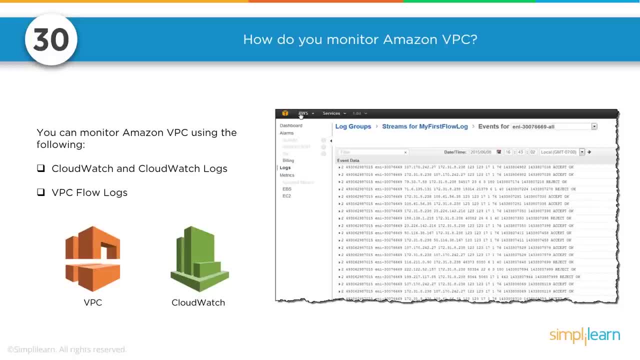 I mean the flow logs is who is allowed and who is not allowed, That kind of detail. And CloudWatch gives information about the data transfer. How much data is getting transferred. We can actually pick unusual data transfers if there is a sudden hike in the graph. 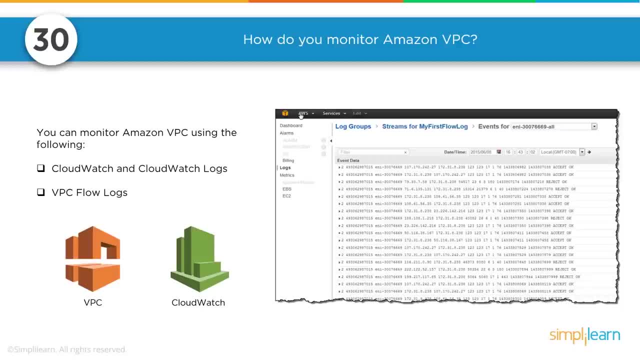 There's a sudden hike and something happens at 12 on a regular basis and you weren't expecting it. There's something suspicious. It could be valid backups. It could be a malicious activity as well. So that's how you know by looking at CloudWatch logs and CloudWatch dashboard. 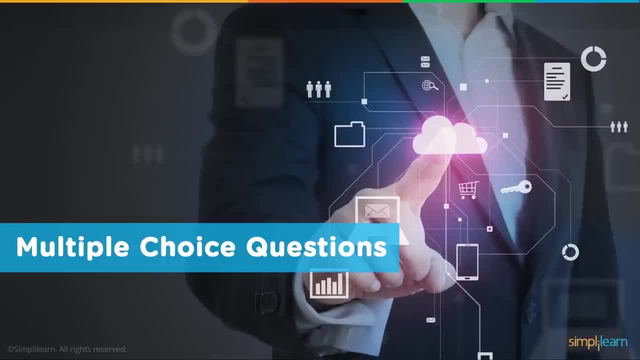 Now let's talk about multiple choice questions. When going for an interview, you might sometimes find yourself that the company is conducting an online test. based on the score, They can put you to a panelist and then they would take it forward. So we thought we'll also include multiple 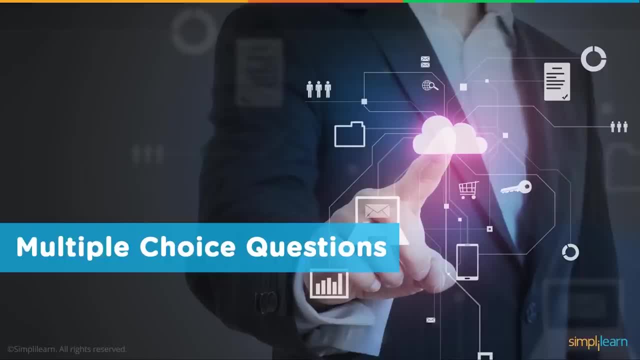 choice questions to help you better handle such situation, if you come across All right. So in order to understand yourself in such a situation, the key to clear them is to understand the question properly. read between the lines. That's what they say. You know there can be like a big paragraph with three lines or ten lines. 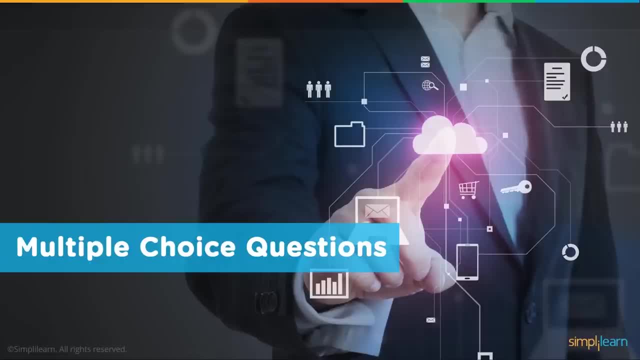 You really got to understand what the question is about and then try to find an answer for that question. So that's rule number one. And then the second rule is: try to compare and contrast the services mentioned, or try to compare and contrast the answers you can easily read out. 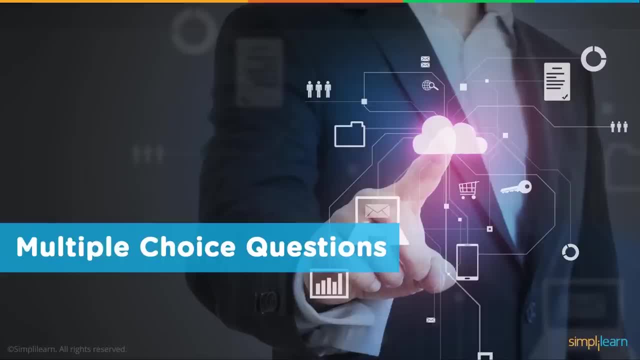 one or two answers and then you'll be left with only two answers to decide from. So that also helps you with time and that also helps you with some precision in your answer. So number one: read between the lines. number two: compare and contrast the services. 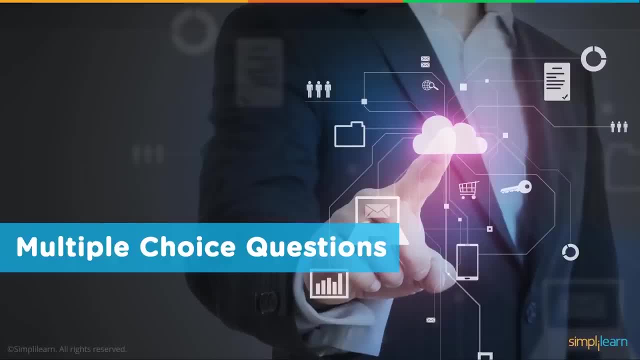 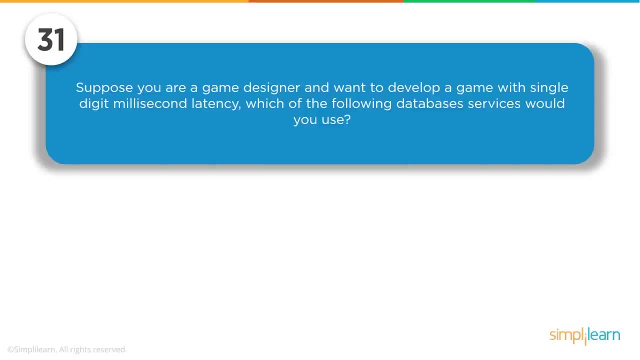 and you'll be able to easily weed out the wrong ones. So let's try answering this question. Suppose you are a game designer and you want to develop a game with a single digit millisecond latency. Which of the following database services would you choose? So we know that the following are database: 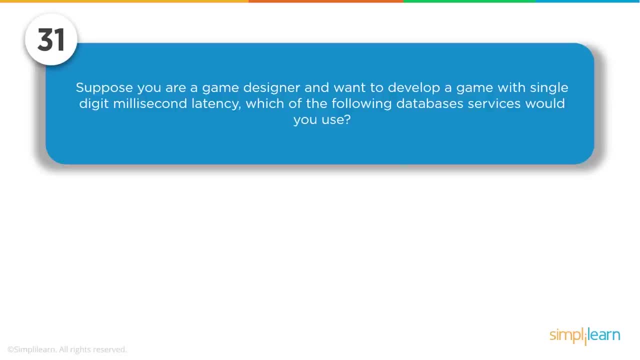 services. Good enough, All right. and it talks about millisecond latency. That's a key point. and the third thing is: it's a game, Could be a mobile game. It's a game that you are trying to design and you need a millisecond latency, and it has to be a database, All right. so let's talk about 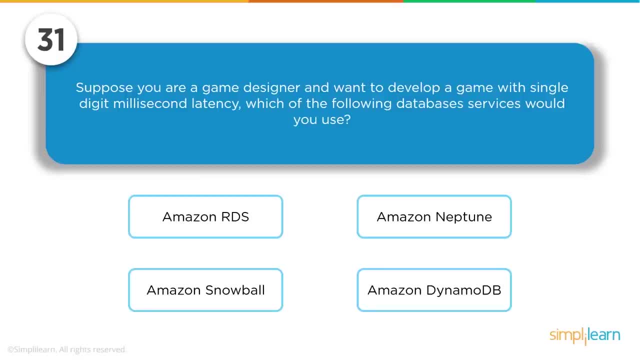 the options available. RDS: RDS is a database, for sure. Is it good for game design. We'll come back to that. Neptune: Neptune is a graph database service in Amazon, So that's kind of out of the equation, and Snowball is actually. 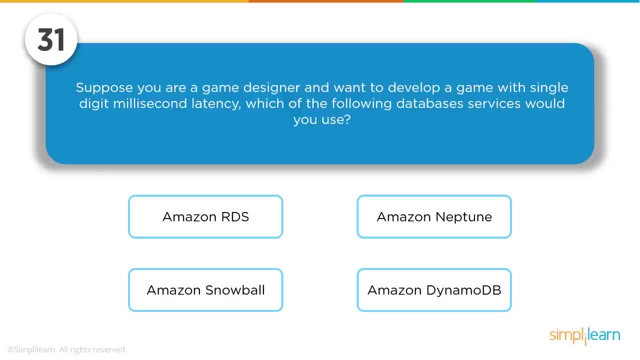 a storage, All right it's. it's a transport medium, I would say. So that's again out of the equation. So the tie is between RDS and DynamoDB If we need to talk about RDS. RDS is a platform as a service. It provides cost-efficient. 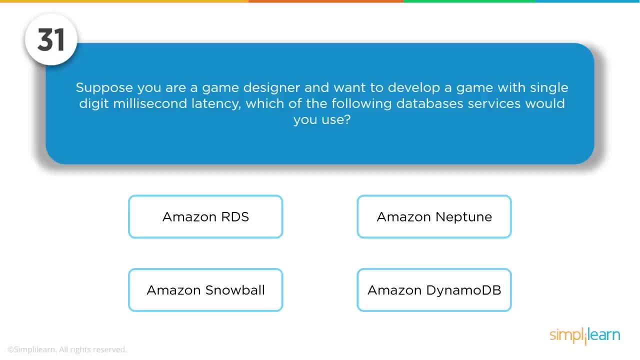 resizable capacity. RDS is a platform as a service. It provides cost-efficient resizable capacity But it's an sequel database, Meaning the tables are kind of strict. I know it's good for banking and other type of applications, but not really good for. 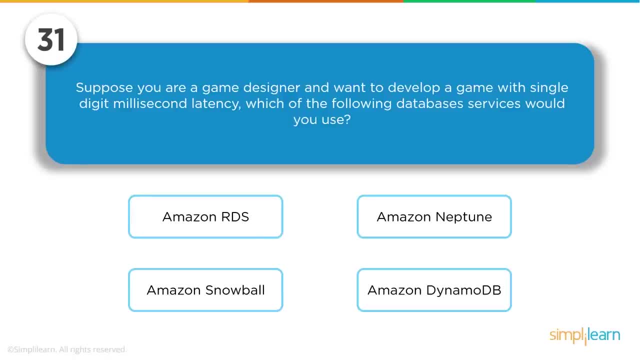 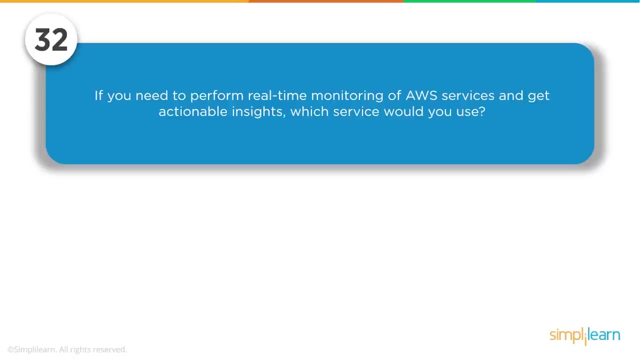 anything that has to do with gaming. So the only option left is DynamoDB. Again, it's right answer. DynamoDB is actually a fast and flexible NoSQL database service and it provides a single digit millisecond latency at any scale, and- And it's a database at the same time, It's a key value store model database. So the right answer is DynamoDB. All right, let's look at the next question. If you need to perform real time monitoring of AWS services and get actionable insights, which service would you use? 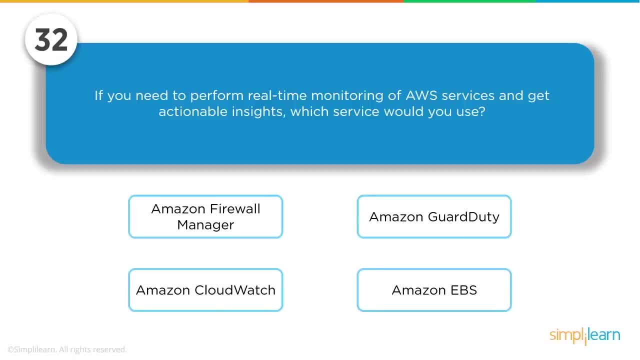 All right, let's list the services. So it talks about real time monitoring. A firewall manager. What does it provide? Now, firewall manager is not really a monitor, just like the name says. It's a manager. It manages multiple firewalls And AWS GuardDuty is a threat detection service. It does monitoring. It does continuously monitor our environment, but it monitors for threats. 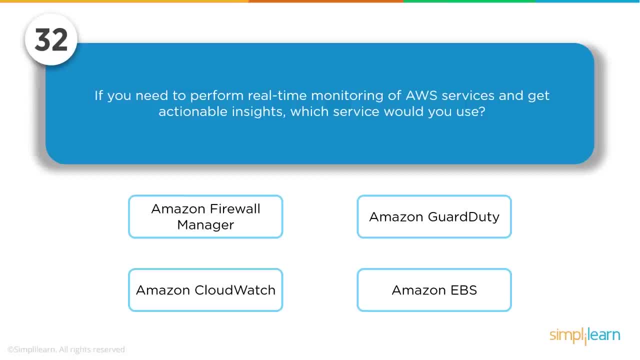 All right, Only threats. Now let's talk about CloudWatch. CloudWatch is a service that helps to track metrics. It's a service that is used to monitor the environment and give us a system wide visibility, And also it helps us to store logs. So at the moment it kind of looks like that could be the right answer. We don't know that yet, But I mean we have one more option left. That's EBS. So what's EBS? EBS is a block storage. 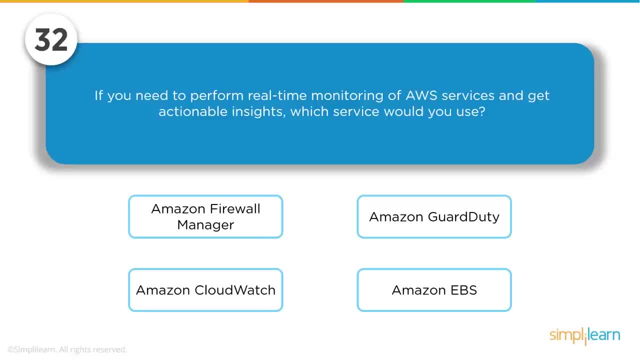 Elastic block Store. If we abbreviate EBS, it's elastic block store. So all three of them are easily out of the question. The first one is to manage. Second one is to find threats. Of course it does. monitoring So there's. I mean, if there is one relation between CloudWatch and GuardDuty, that's monitoring. So easily we can actually find ourselves slipped towards picking GuardDuty, But know that GuardDuty is only for gaining security insight, but not about gaining AWS service insight. 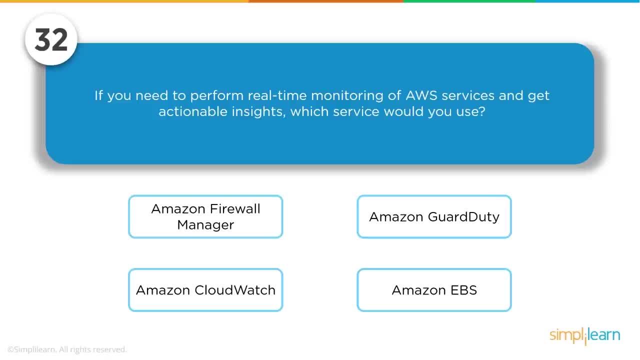 So CloudWatch is a service that helps us to get a system wide, or an AWS wide or an account wide. It has a number of metrics we can monitor and get a very good insight of how a service is performing, be it CPU, be it RAM, be it network utilization, be it connection failures. CloudWatch is a service that helps us perform a real time monitoring and get some actionable insights on the services. 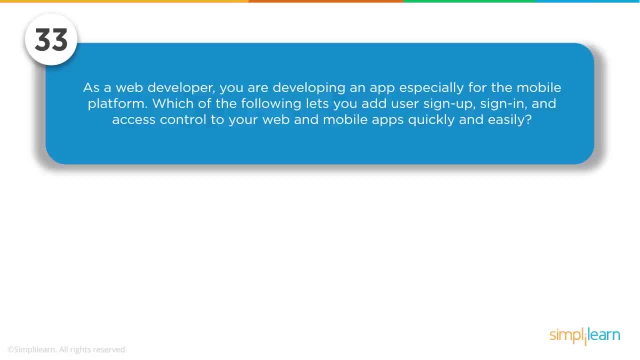 All right, let's talk about this 33rd question. All right, so we have like four options here. So we have like four options here. So we have like four options here. So let's try to weed out services which are not relevant to it. 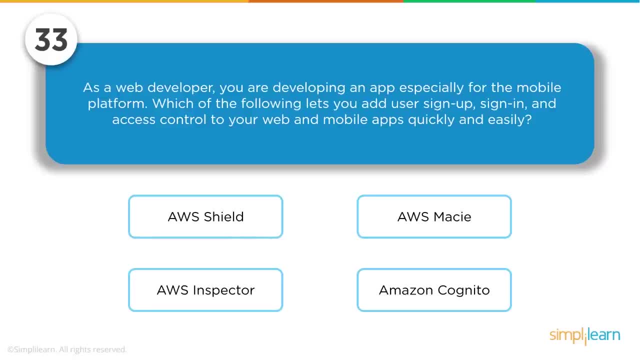 So what's AWS Shield? AWS Shield is actually a service that provides a DDoS mitigation or DDoS protection- denial of service protection. It's in security feature. Let's talk about the second option. AWS Massey is again a security service that uses machine learning to automatically discover and classify. 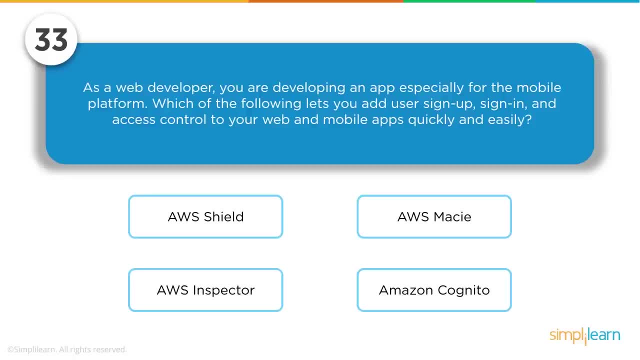 It again talks about security, and this security is all about encrypting or saving the data. It does not come close with signing up a mobile platform. All right, let's talk about the other one, AWS Inspector. Now AWS Inspector has something to do with apps. 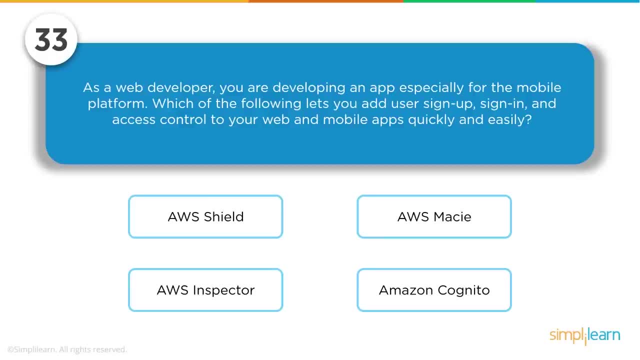 It definitely has something to do with apps. So it kind of looks like that's relevant as of now. So it actually helps with improving the security and compliance of the apps That we deploy in the cloud. So kind of looks like it could be because it has to do with apps. 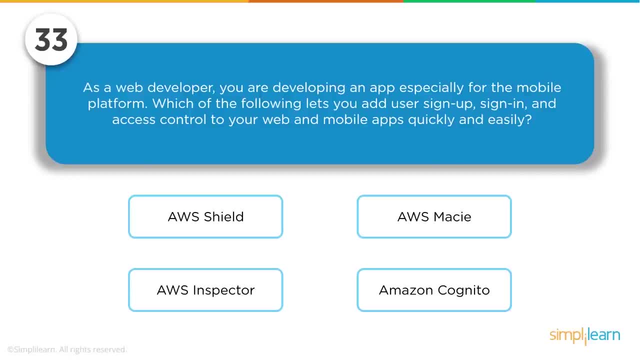 The last one, Cognito. Now, Cognito is a service that actually lets the administrator to have control access over web and mobile apps, And it's a service that helps us to sign up and sign in to a mobile and web app, So that very much looks like we found the answer. 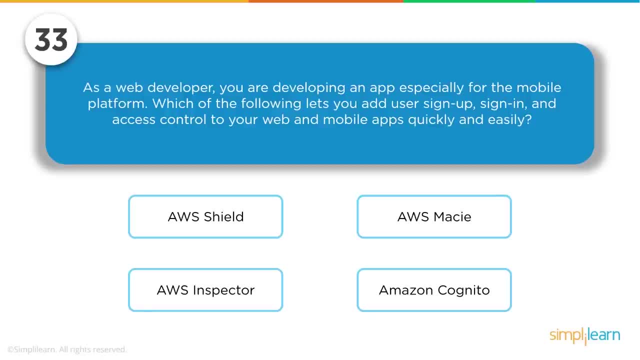 So Cognito is a service that helps web app and mobile app For sign up and signing in and also gives the administrator to have control over who has access- control over the web and the mobile app. Pretty much we found it. So it's Cognito. 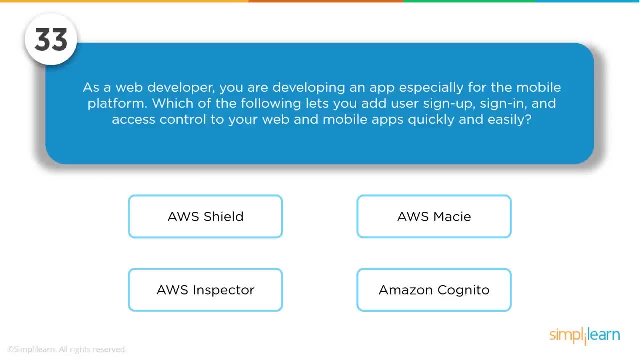 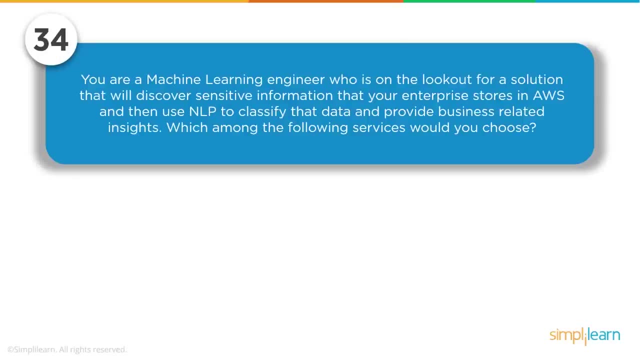 Cognito is a service that helps us to set up, sign up, sign in and have access control over the users who would be using our mobile and web app. All right, how about this question? You are an ML engineer or a machine learning engineer who is on the lookout for a solution that will discover sensitive information. 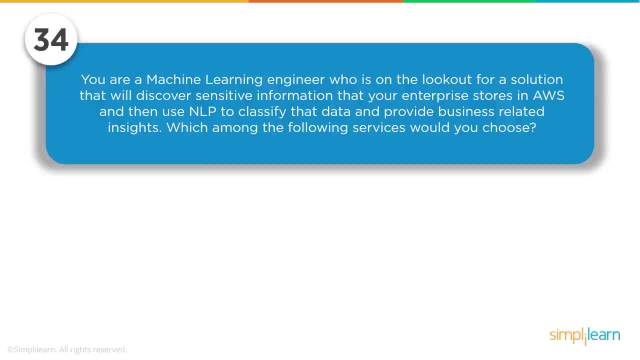 That your Enterprise stores in AWS and then uses NLP to classify that data and provide business related insights. which among the following services would you choose? So we have a bunch of services that's going to help us achieve- or one of it is going to help us achieve- the above requirement. 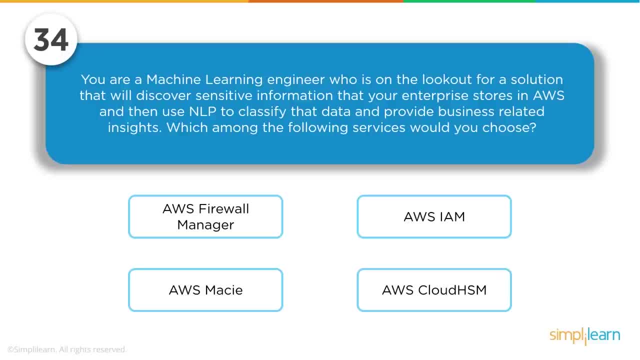 So it's a service that deals with machine learning. You're a machine learning engineer who's looking for a service that will help you to discover information That your enterprise store. So we're talking about storage: discover information in store and then classify the data depending on severity, sensitivity. classify the data. 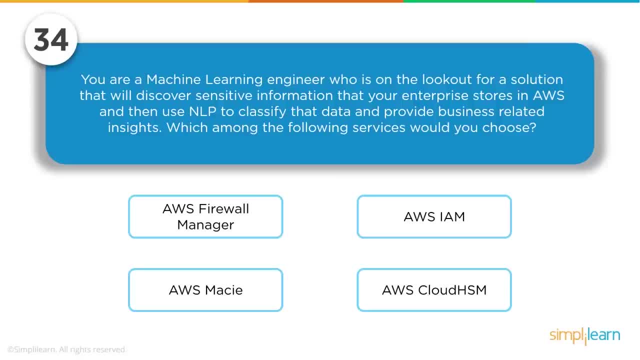 So which service is that? So firewall manager, just like the name says, it's a manager, and the AWS IAM. If we abbreviate it, it's identity and access management. So it's identity and access management, Nothing to do with identifying sensitive data and managing it. 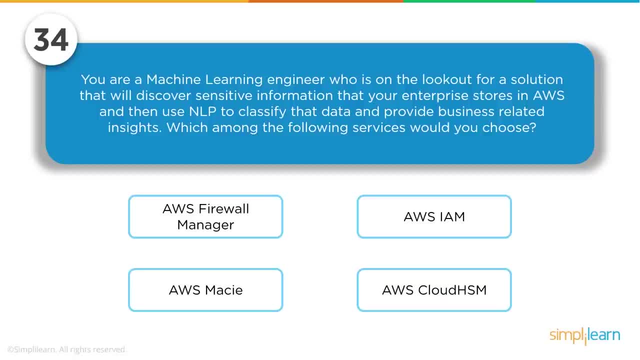 So the first two is already out of the equation. Then the AWS Massey. we already had a quick definition description for AWS Massey- that it's actually a security service that uses machine learning kind of looks like it could be it. It's a security service that uses machine learning and it discovers and classifies the sensitive information. 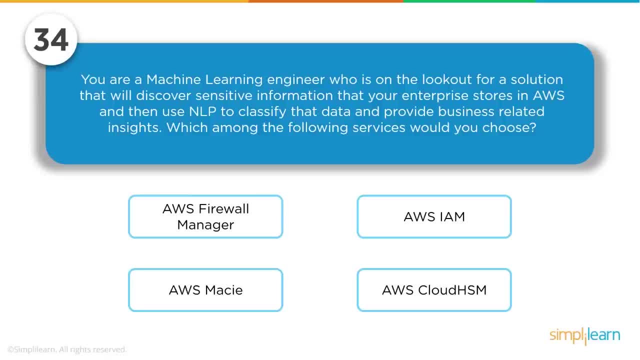 Not only that, it does not stop there. It goes beyond and protects the sensitive data. AWS Massey kind of looks like. but we still have one more option. Okay, One more option to look at, which is cloud HMS. Cloud HMS is also a security service. 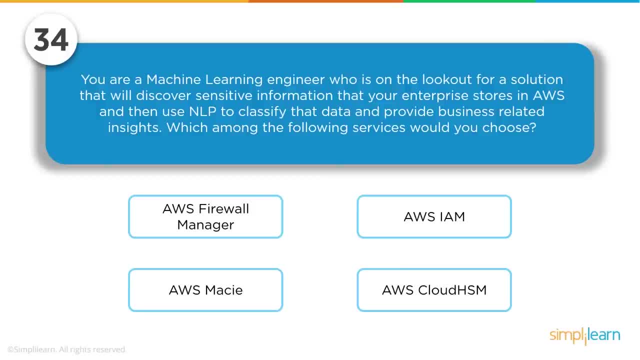 Kind of looks like that could be the answer as well, And it enables us to generate encryption keys and save the data. So kind of 50% of it is a security service. It encrypts, helps us protect the data. but AWS Massey is right on spot. 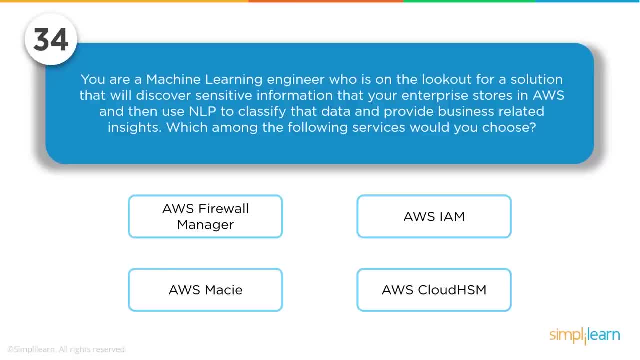 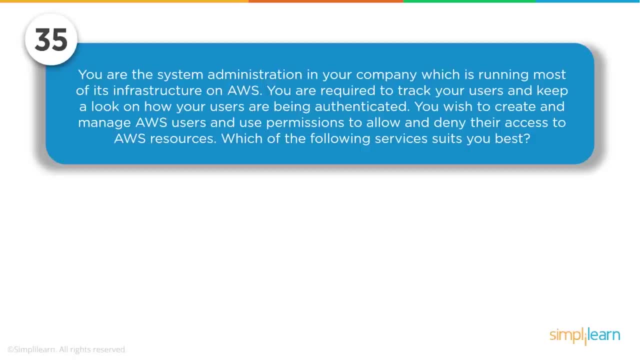 It's a machine learning service. It helps us to classify the data and also to protect the data. So the answer for this question would be AWS Massey. So hope you kind of get it how this is going. So first we apply the thumb rule, identify the question that's being asked. read between: 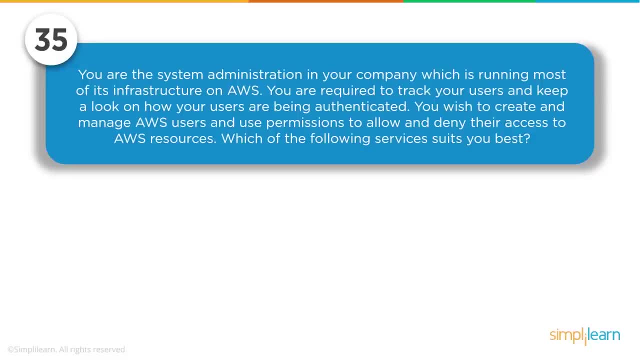 the lines and then try to find the service that meets your requirement. and finding the service is by first reading out the wrong ones. recollect everything that you've learned about the service and see how well that matches with those hints that you have picked up. 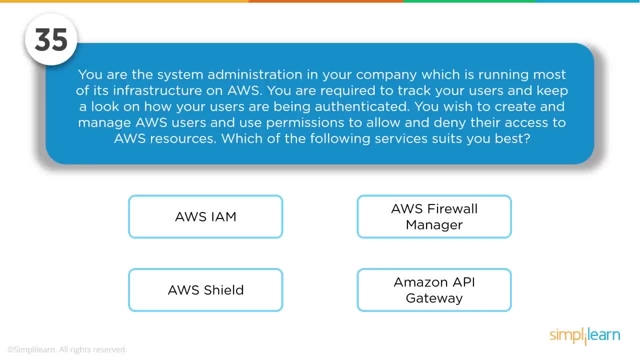 And if that doesn't match weed that out, then you'll end up with two, just two, to decide from at some point, And then it becomes easy for you to decide: Click on the question, submit it and then move on to the other question in your interview. 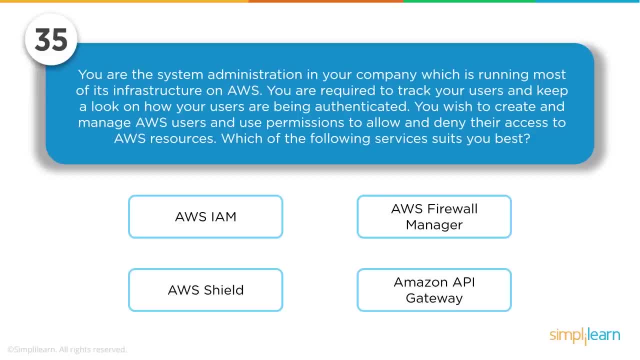 All right. So how about this one? You are a system administrator in a company which is running most of its infrastructure on AWS. You are required to track your users and keep a look on how your users are being authenticated. All right, So this is where the problem statement starts. 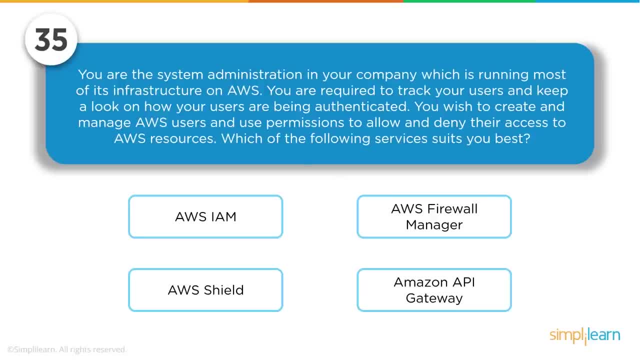 You need to keep track of how your users are being authenticated and you wish to create AWS users and use permissions to allow and deny their access to the AWS resources. You are to give them permission number one. And then I mean, if we put them in the right order, first giving them permissions and then 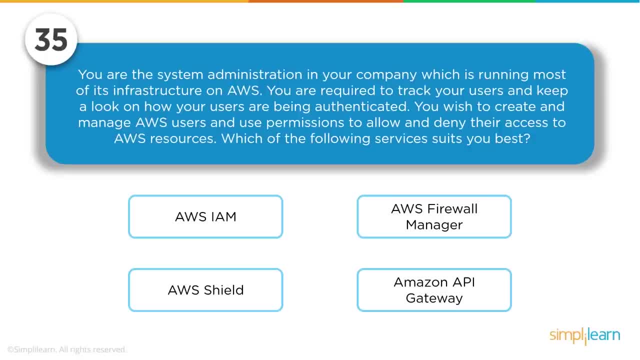 tracking their usage. Let's see which of the service will help us achieve it. IAM is a service that helps us to looking at the permissions. we can actually predict whether the user or the group will have service or not. So that helps us to get a track of who is able to use, who is not able to use certain. 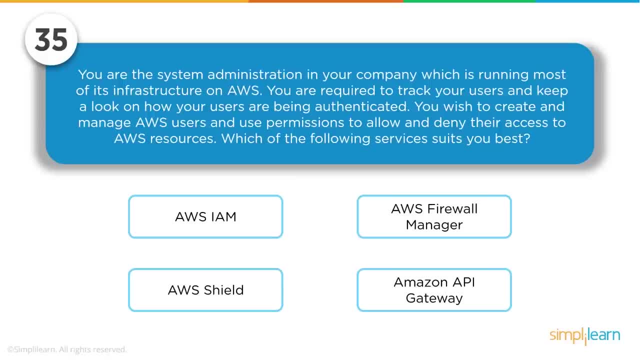 service and all that stuff. So it kind of looks like, but we have other three options left. Let's look at AWS Firewall Manager. just like the name says, It's actually a firewall manager. It helps us to manage multiple firewalls. simple as that. 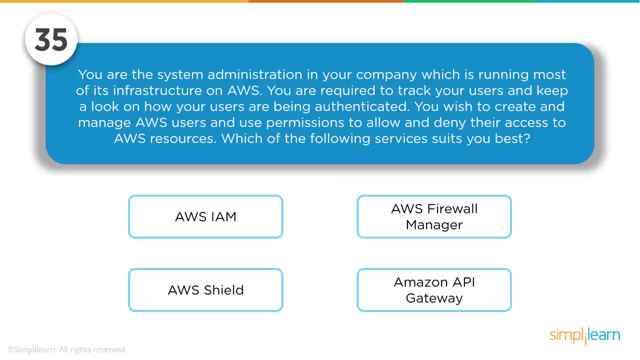 And Shield is a service. It's a service that's used to protect denial of service or distributed denial of service, And API Gateway is a service that makes it easy for developers to create, publish, maintain and monitor And secure API. So I mean it's completely on the API side, very less on user and how you authenticate. 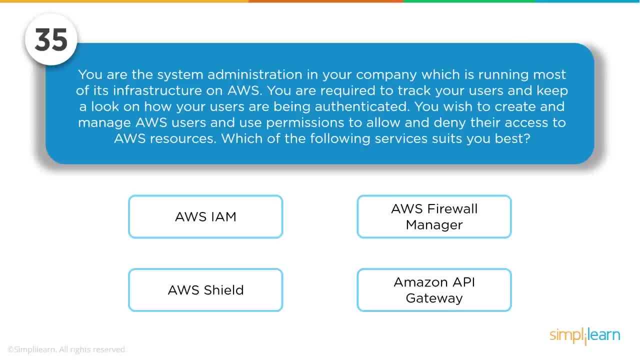 your user. We can get that by looking at the name itself. right, If we abbreviate it or if you try to find a definition for the name API Gateway, you would get it. It has to do with API. But if we abbreviate AWS, IAM, it's identity and access management pretty much meets the 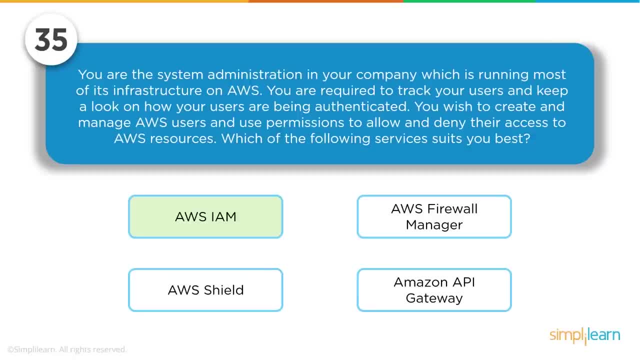 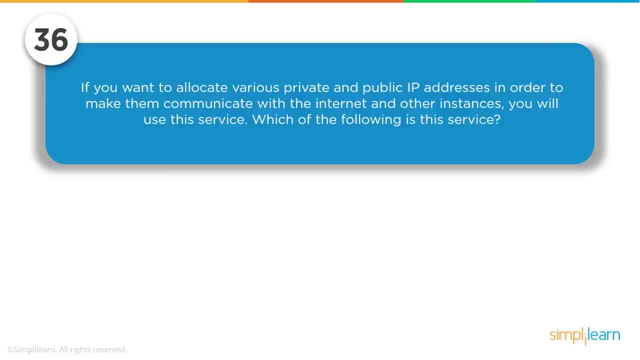 requirement for the problem statement about It's AWS, IAM, It's identity and access management. That's the right answer. All right, Let's look at this one. If you want to allocate various private and public IP address in order to make them communicate, 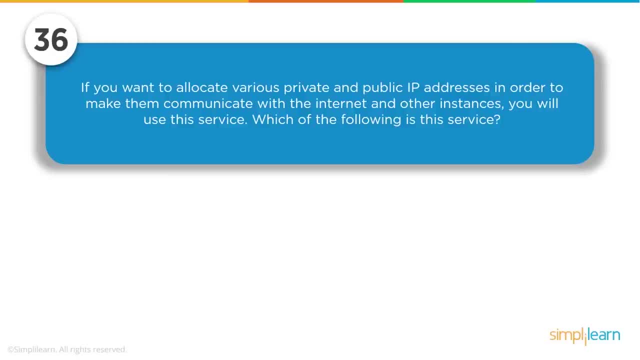 with the internet and other instances, you will use this service. Which of the following is this service? So it talks about using public and private IP address. So this service uses IP address. And then this service helps us to allow and deny connections to the internet and to the. 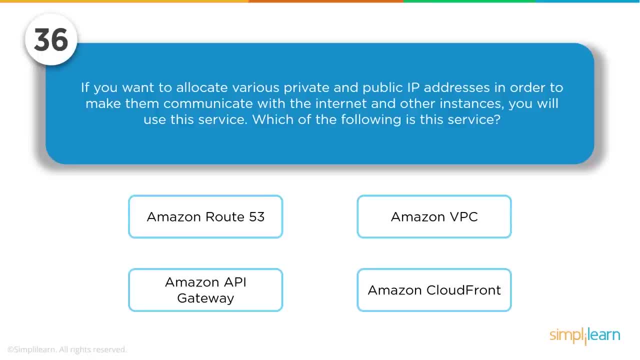 other instances. So you get the question: is it? Let's pick the service that helps us achieve it? Route 53.. Route 53 is actually a DNS service, right? It's not a service that's used to allow or deny. 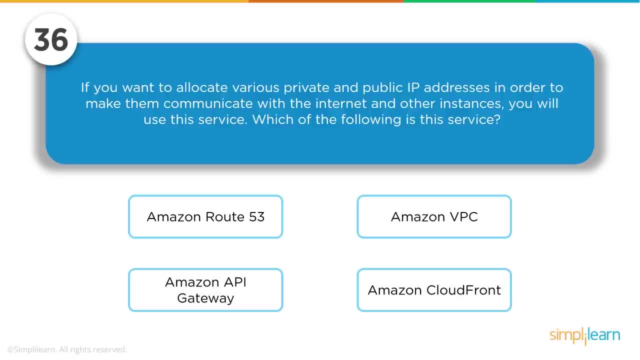 No, it does not do that VPC. VPC uses public and private IP address. Yes, So kind of looks like a VPC helps us to allow. I mean the security in VPC, the security group, the network access control list in a VPC, the routing table in a VPC. that actually 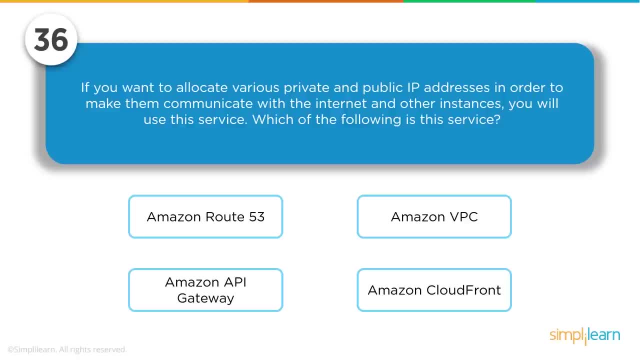 helps us to allow or deny a connection to a particular IP address or to a particular service within the VPC or outside of the VPC. So as of now it kind of looks like it could be. but let's look at the other services. 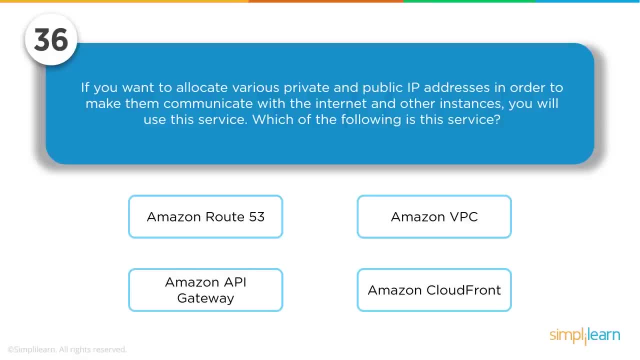 What if? if we find a service that closely matches to the above requirement than the Amazon VPC Gateway, API Gateway? We know that it's a managed service that makes it easy for developers to create, publish, maintain and monitor APIs and secure API. so that has completely do with API, not with IP. 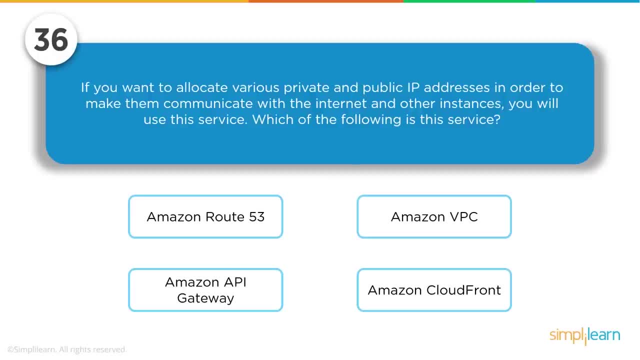 CloudFront. We know about CloudFront that it's an content delivery network and it provides global distribution of servers where our content can be cached. It could be video or bulk media or anything else. They can be cached locally so users can easily access them and download them easily. 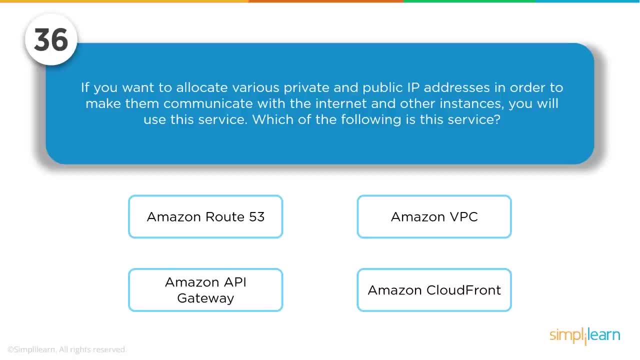 All right, So that's CloudFront. Now, at this point, after looking at all four, It looks like VPC is the right answer, and in fact, VPC is the right answer. VPC has public IP address. VPC can help us with a private IP address. VPC can be used. 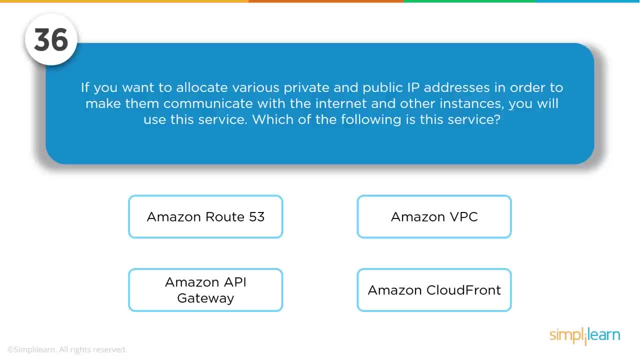 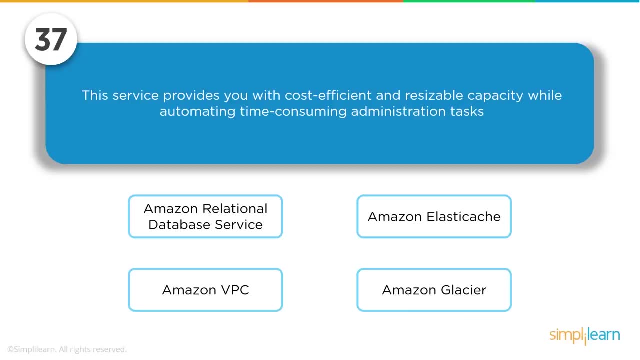 to allow deny connection based on the security group access control list and routing table it has. So that's right answer. is VPC? All right? How about this one? This platform as a service or platform as a DB service provides us with a cost efficient. 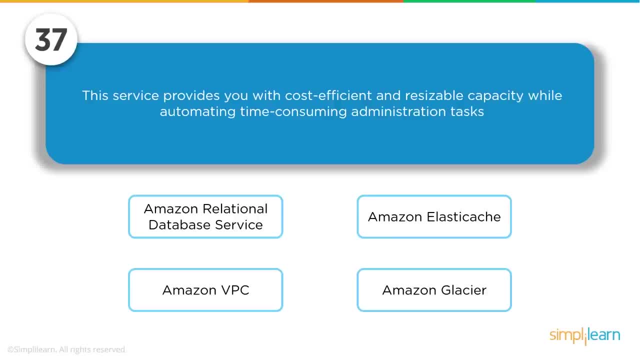 and resizable capacity while automating time consuming, Time consuming administrative tasks. So this question is very clear. It's a DB service we got to look for and it's a service that can provide automating some of the time consuming tasks. It has to be resizable at the same time. 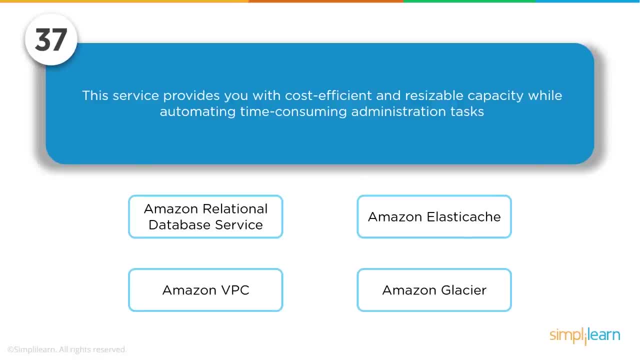 So let's talk about Amazon Rational Database. It's a database kind of matches the requirement. We can resize it as and when needed. All right, Looks like it's a fit as of now. It actually automates Some of the tasks. 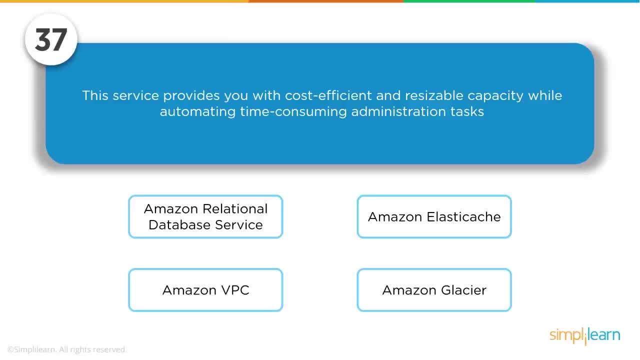 Some of the time consuming work looks like it's a fit as of now. Let's move on to Elastic Cache and then try to see if that matches the definition that we've figured out about Elastic Cache. It's actually a caching service. It's again an in-memory data store which helps in achieving high throughput and low latency. 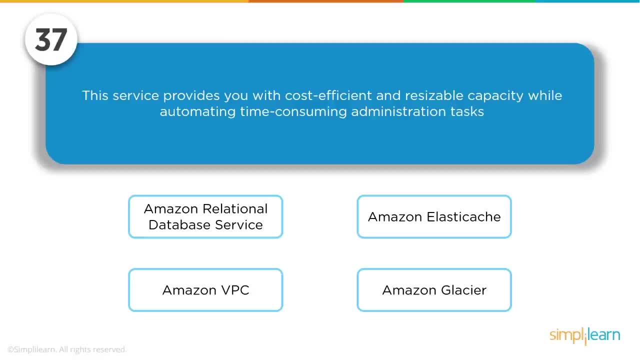 in memory data store. So it's not a full blown database and it does not come with any Amazon products. Okay, There's some provisioned automation in it for automating any of the administration tasks. No, it does not come up with anything like that. 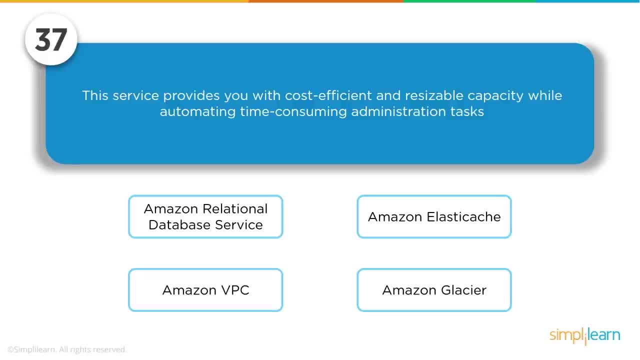 Yeah, we can resize the capacity as and when needed, but automation, it's not there yet And, moreover, it's not a database, So that's out of the equation. VPC is not a resizable one. Once we have designed VPC, it's fixed. 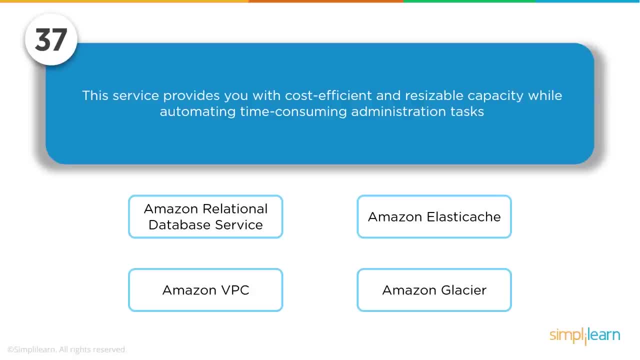 It can't be resized, So that's out of the equation. And Amazon Glacier Glacier- It's a storage but not a database, right? So that's again out of the equation. So the tie is kind of between Amazon Rational Database Service and Amazon Elastic Cache, because 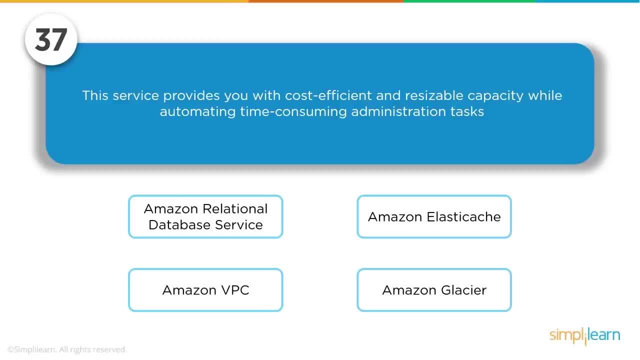 they both aid the database service, but Elastic Cache is not a full blown database. It actually helps the database, but it's not a full blown database. So it's Amazon Relational Database. That's the one which is a platform as a service. 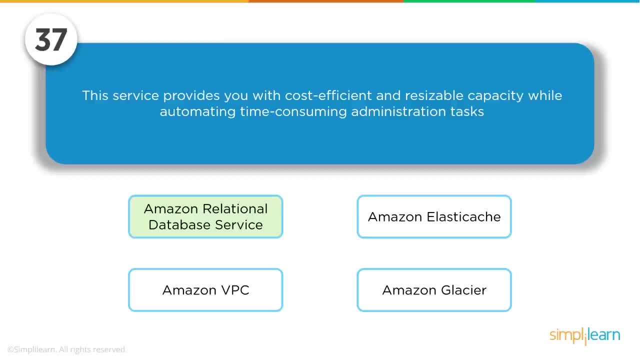 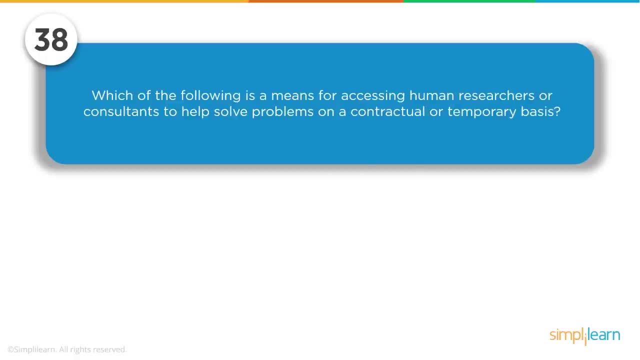 It's the one which can be resized. It's the one which can be used to automate the time control. It's the one which can be used to automate the time consuming administrative tasks. All right, let's talk about this one. Which of the following is a means for accessing human researchers or consultants to help solve? 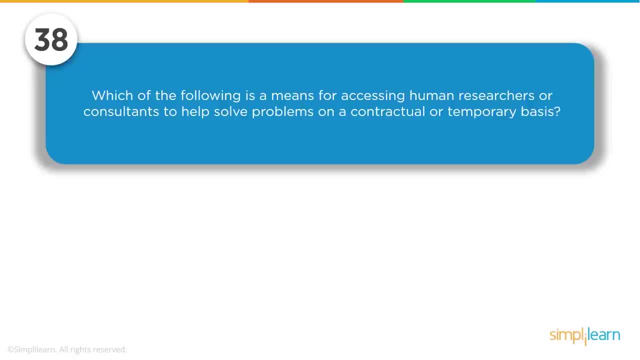 a problem on a contractual or a temporary basis. All right, let's read the question again. Which of the following is a means for accessing human researchers or consultant to help solve problems on a contractual or a temporary basis? It's like assigning task or hiring AWS experts for a temporary job. 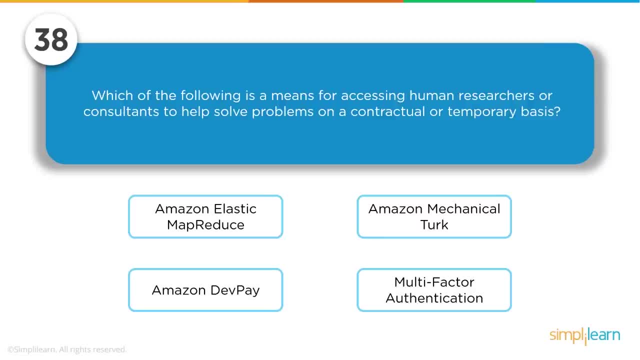 So let's try to find that kind of service in the four services that are listed: Amazon, Elastic, MapReduce. MapReduce is actually a framework service that makes it easy and cost effective to analyze large amount of data, but that has nothing to do with accessing human researchers. 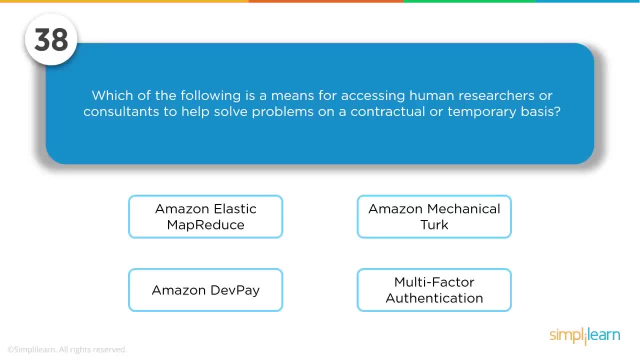 Let's talk about Mechanical Turk. It's a web service that provides a human workforce. That's the definition for it. For example, automation is good, But not everything can be automated. For something to qualify for automation, it has to be a repetitive task. 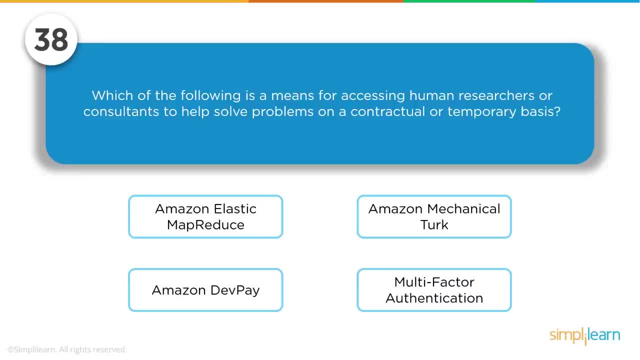 One-time task can't be automated, or the time and money that you would be spending in automation is not worth it. Instead, you could have done it manually. So that does not qualify for automation and anything that requires intelligence or anything that's a special case, right. 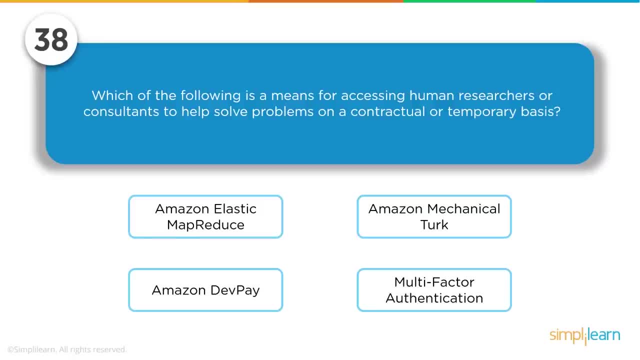 Automation can do repetitive tasks. Automation can do precise work, but it has to be a repetitive task. The scenario you know, it should have been there already. Only then that can be executed. But if it's a new scenario and it requires appropriate addressing, then it requires human. 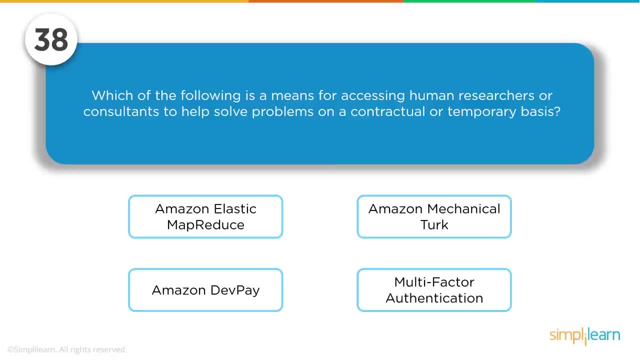 tasks, So we could hire researchers and consultants who can help solve a problem using Amazon Mechanical Turk. The other two are already out of the equation Now. DevPay is actually a payment system through Amazon and multi-factor authentication. As it says, it's an authentication system. 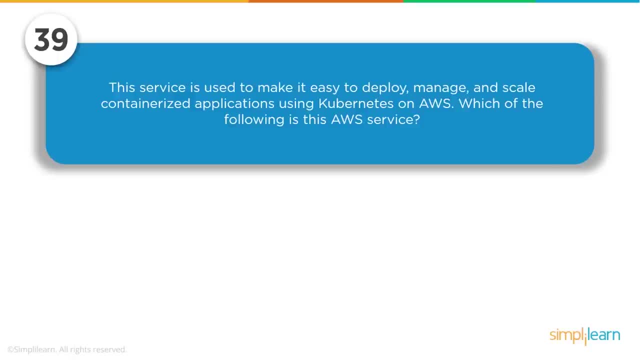 So the right answer is Amazon Mechanical Turk. All right, Interesting, Let's look at this one. This service is used to make it easy to deploy, manage and scale containerized applications using Kubernetes on AWS. Which of the following is this AWS service? 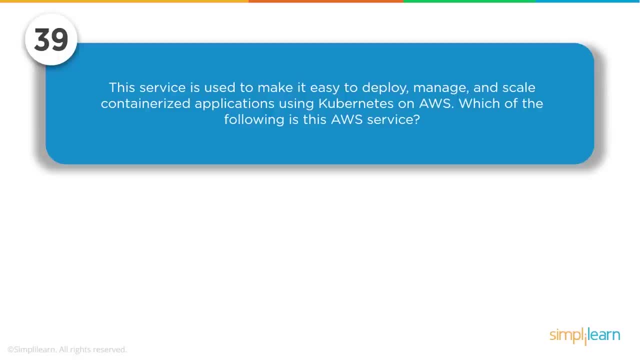 So it's a service to deploy, manage and scale containerized applications, So it deals with containers. It also should have the ability to use Kubernetes, which is a container orchestration service. All right, The first one: Amazon Elastic Container Service. 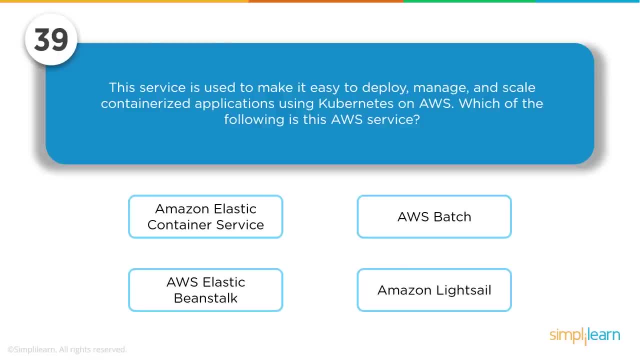 It kind of looks like it's the one. The name itself has the word and the relation. we're looking for: Elastic Container Service. So this container service is an highly scalable, high performance container orchestration service. Let's look at the other one. 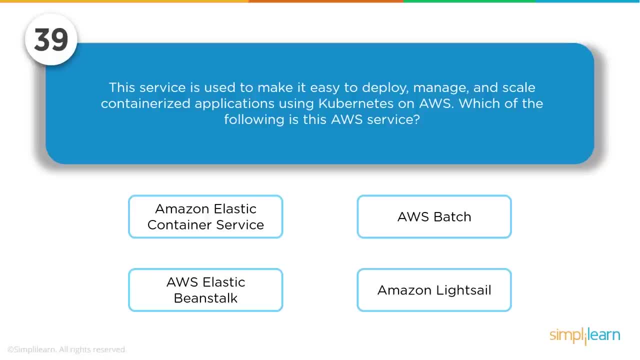 AWS Batch. It's a service that enables IT professionals to schedule and execute batch processing. I mean, the name itself says that that's meant for batch processing. Elastic Beanstalk: That's another service that helps us to deploy, manage and scale. 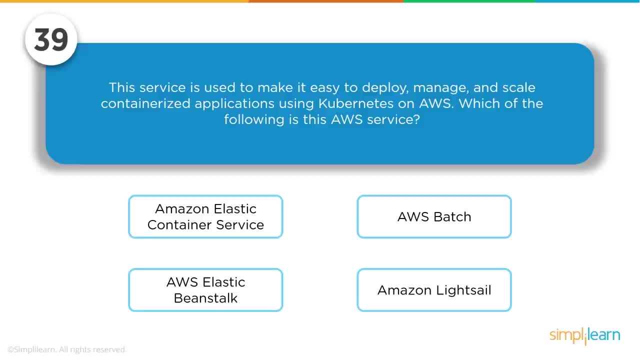 But it helps us with EC2 instances, not with containerized instances, So that's again out of the equation. Would LightSail be a good tie for Elastic Container Service? What's LightSail Now? LightSail is a service. 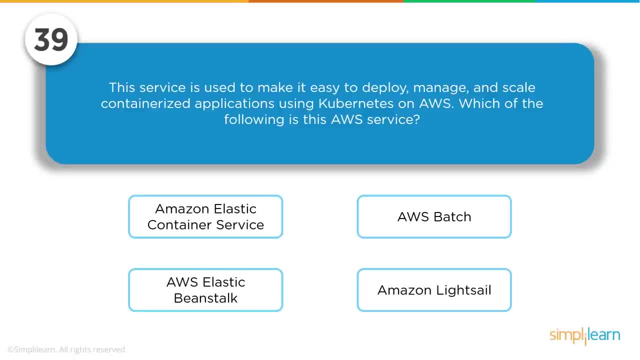 It's called as a virtual private server. without a VPC. It's called as a virtual private server. It comes with a predefined computer. It's called a virtual private server. It comes with a predefined computer. It has being able to set up remote dedicated devices for a lifetime. 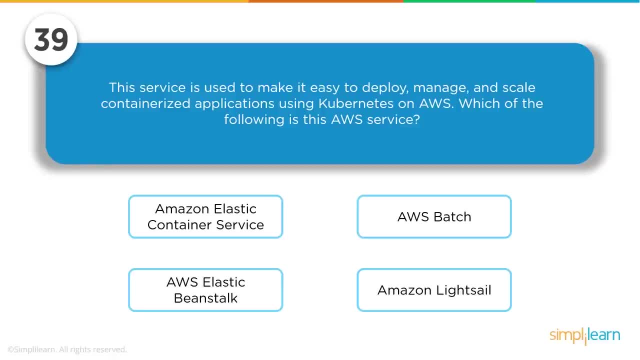 And then utilizes the security ermines So that it can take every passing data away from any virtual Werbe. Now let's move on to another service. So it's Amazon Elastic Container Source, And that's the one that helps us to easily deploy. 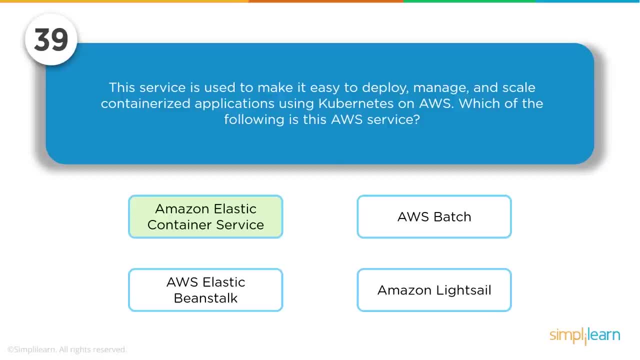 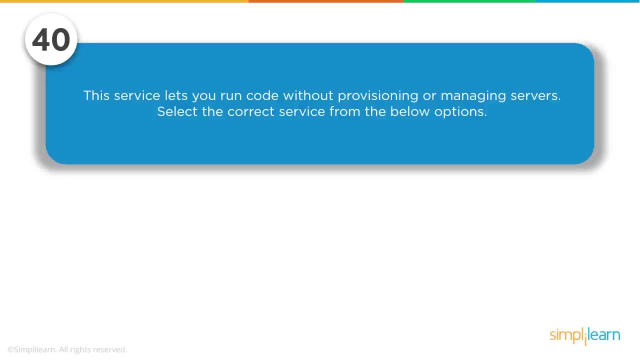 manage scale container services, and it helps us orchestrate the containers using Kubernetes. How about this one? this, just so, let's us to run code without provisioning or managing. so it's no. so it's run code. select the correct service from the below option. all right, so no servers, but we should be able to. 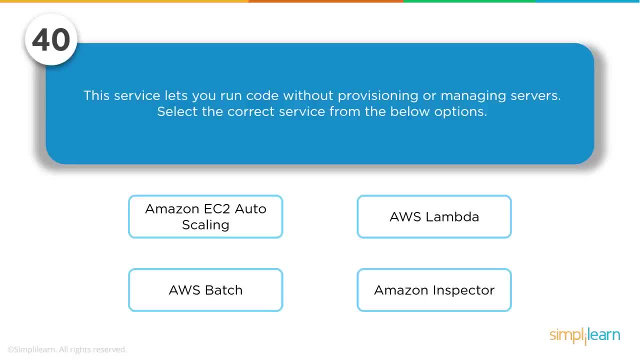 run code: amazon ec2 auto scaling- easy to auto scaling. ec2 is elastic compute cloud, which is a server, and auto scaling is a service that helps us to achieve scaling the server. so that's the definition for it could be that's out of the equation. aw is lambda. now, lambda is a service. 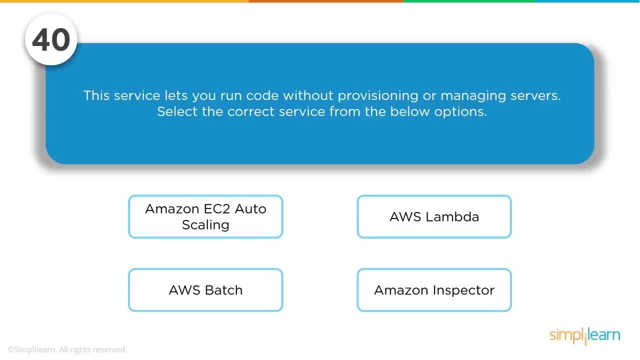 it's actually event driven serverless computing platform and lambda runs code in response to the event that it receives and it automatically manages the compute resource that's required for that code, as long as we have uploaded a code that's correct and set up events correctly to map. 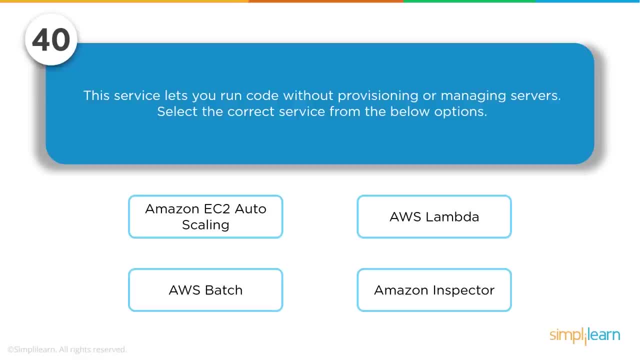 to that code. it's gonna run seamlessly. so that's about lambda. it kind of looks like it could be the answer because, uh, lambda runs code. we don't have to manage servers, it manages servers by itself. but we can't conclude as of now. we have other two service to talk about: aws batch all. 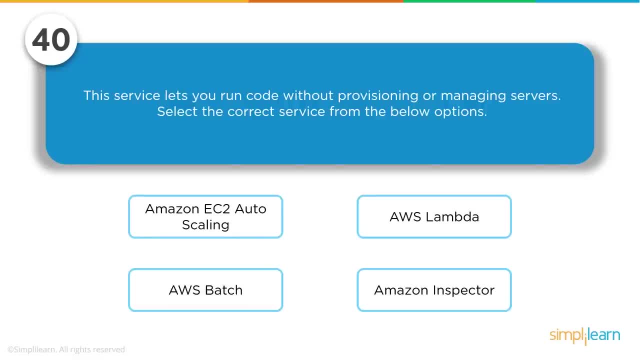 right batch is service that enables id professionals to run batch job. we know that. and about inspector amazon inspector, it's actually a service that helps us to increase and identify any security issues and align our application with compliance. well, that's not the requirement of the question. the requirement and the question was run code without provisioning a server and without any. 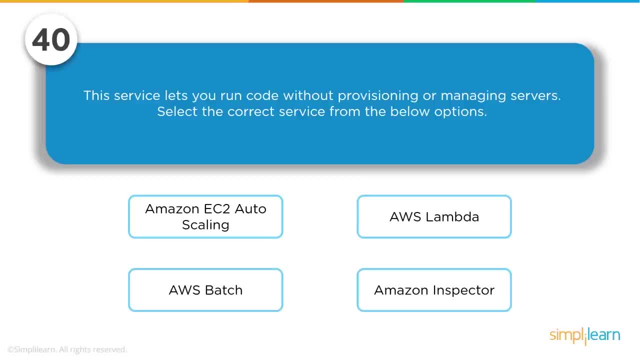 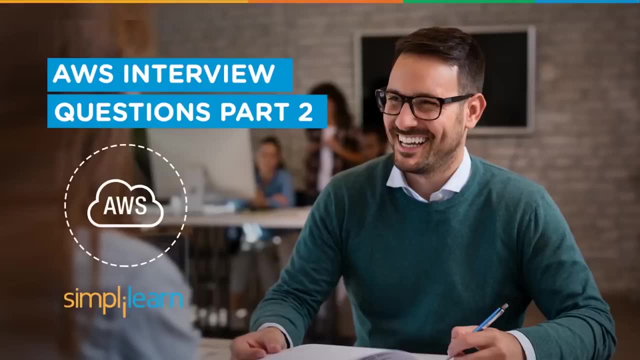 more space for confusion. aws lambda is a service or is the service that runs code without provisioning and managing services, right? the right one would be aws lambda, the second part in aws interview questions. if you haven't watched the first part yet, please go back and watch the. 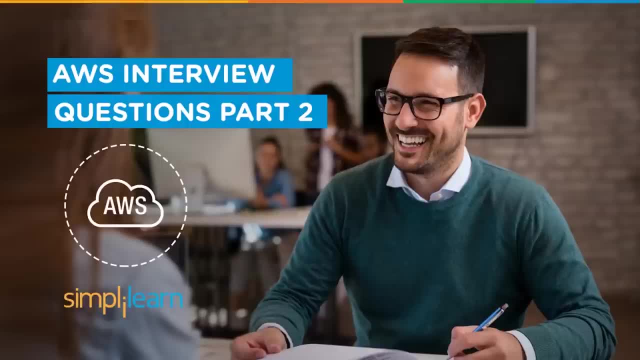 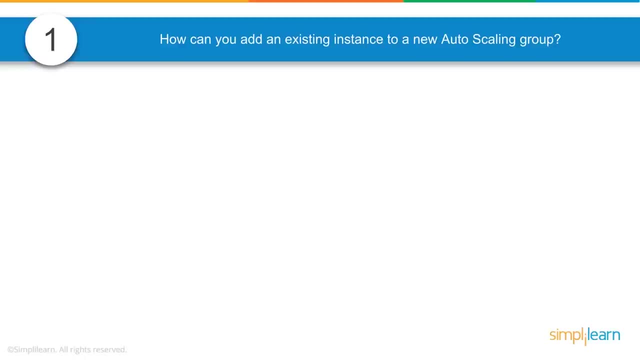 first part. we have a lot of interesting questions there which will better prepare you for the interview. all right, let's get started. so, in an environment where there is a lot of automation- infrastructure automation- you'll be posted with this question: how can you add an existing instance to a new? 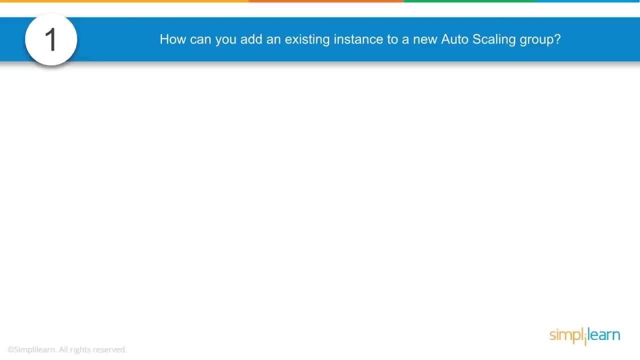 auto scaling group. now this is when you are taking an instance away from the auto scaling group to troubleshoot, to fix a problem you know, to look at logs, or if you have suspended the auto scaling, you know you might need to re-add that instance to the auto scaling group. only then it's going to. 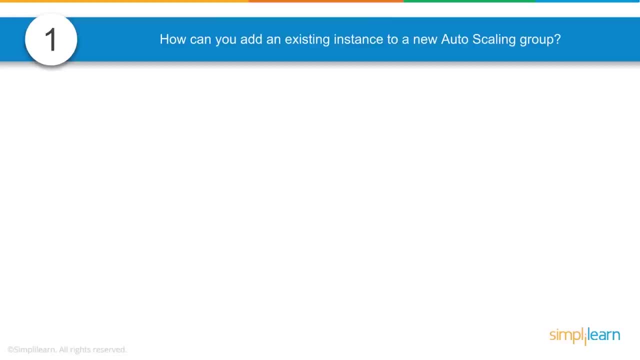 take part in it, right. only then the auto scaling is going to count it as part of it. it's not a straight procedure. you know, when you remove them, you know it doesn't get automatically re-added. i've had worked with some clients when their developers were managing their own environment. 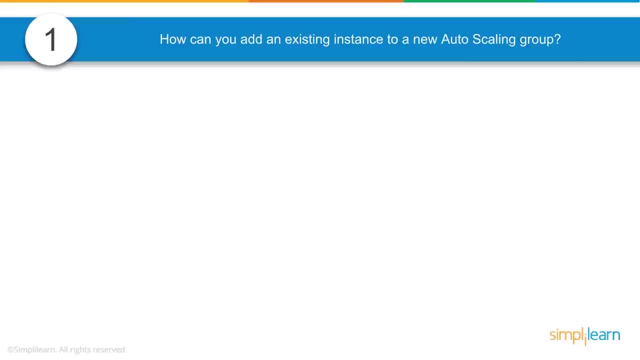 they had problems adding the instance back to the auto scaling group. you know, irrespective of what they tried, the instance was not getting added to the auto scaling group and whatever they fixed that they were provided, or whatever fix that they have provided, were not, you know, getting encountered. 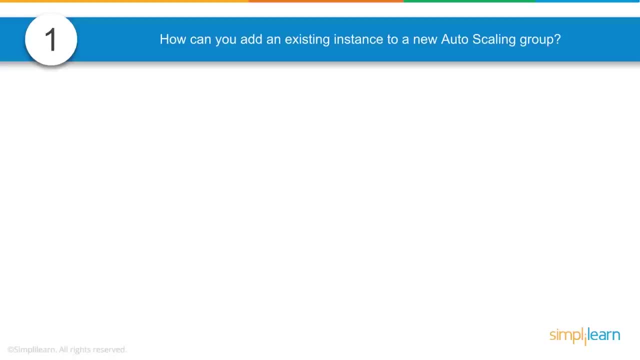 in the auto scaling group. so, like i said, you know you can't add a new instance to the auto scaling group. it's not a straight. you know a click button procedure. there are ways we'll have to do it. so how can you add an existing instance to the auto scaling group? there are few steps that we need to. 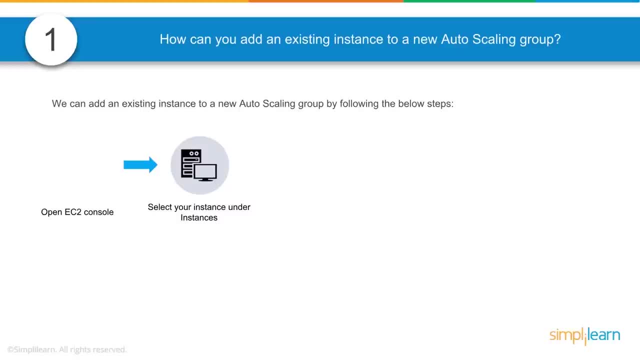 follow. so the first one would be to, under the ec2 instance console, right under the instance, under actions. in specific, you know there's an option called attach to auto scaling group right, if you have multiple auto scaling groups in your account or in the region that you're working in, then you're. 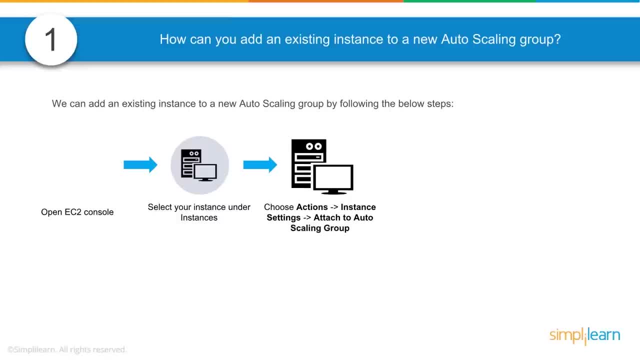 posted with the different auto scaling groups that you have in your account. let's say you have five auto scaling groups for five different applications. you know you're going to be posted with five different auto scaling groups and then you would select the auto scaling the appropriate auto. 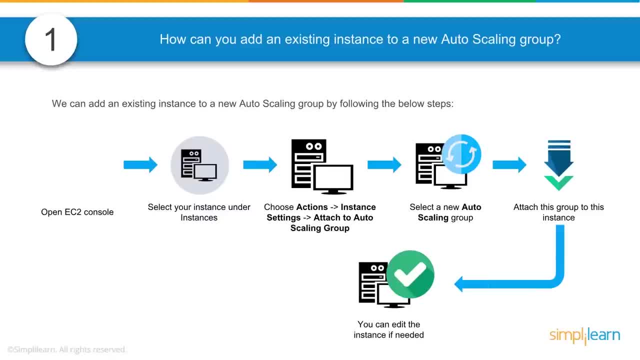 scaling group and attach the instance to that particular auto scaling group while adding to the auto scaling group. if you want to change the instance type, you know that's possible as well. sometimes, when you want to add the instance back to the other scaling group, there would be. 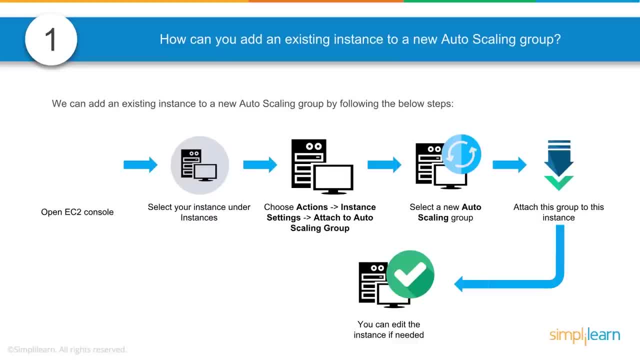 requirement that you change the instance type to a better one, to a better family, to the better instance type. you could do that at that time and after that you are, or you have completely added the instance back to the auto scaling group. so it's actually a seven step process adding an. 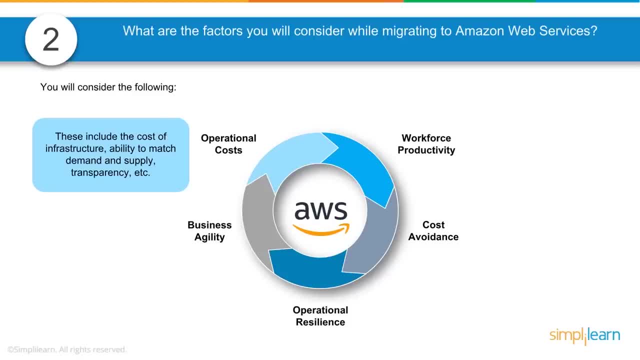 instance back to the auto scaling group in an environment where they're dealing with migrating the instance, or migrating an application, or migrating an instance migrating an vm into the cloud, you know if the project that you're going to work with deals with a lot of migrations, you 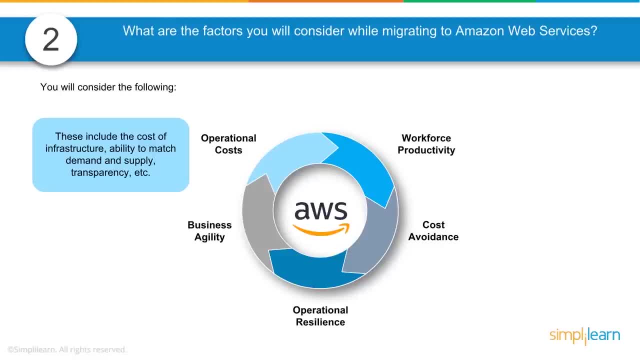 could be posted this question: what are the factors you will consider while migrating to amazon web services? the first one is cost. is it worth moving the instance to the cloud, given the additional bills and whistles features available in the cloud? is this application going to use all of them is? 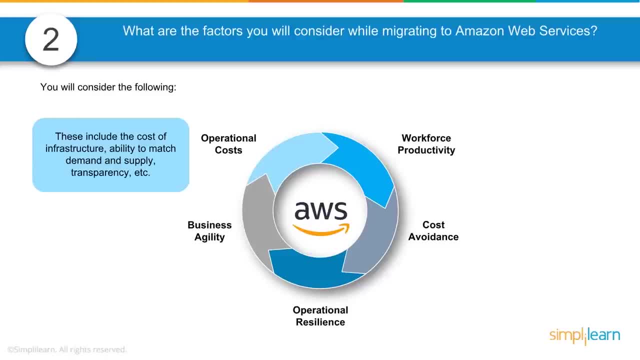 moving into the cloud, beneficial to the application in the first place, you know, beneficial to the users who will be using the application in the first place. so that's a factor to think of. so this actually includes no cost of the infrastructure and the ability to match the demand and supply. 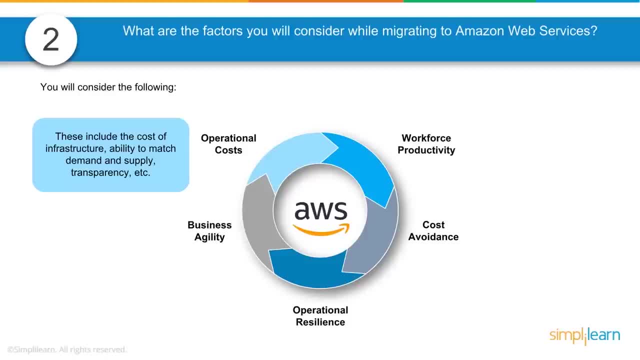 transparency. is this application in high demand, you know- is it going to be a big loss if the application becomes unavailable for some time. so there are a few things that needs to be considered before we move the application to the cloud and then, if the application does, the application. 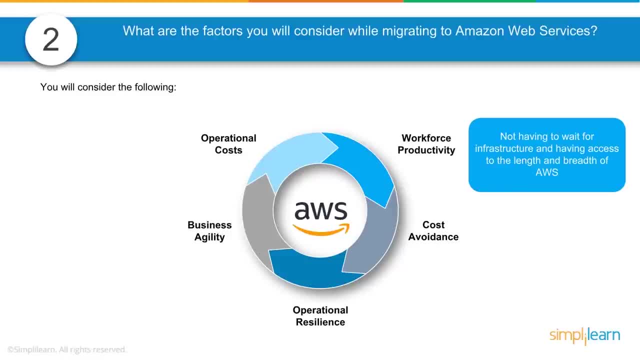 needs to be provisioned immediately. is there an urge? is there an urge to provision the application immediately? that's something that needs to be considered. if the application requires to go online, if the application needs to hit the market immediately, then we would need to move it to the cloud because in on-premises procuring, 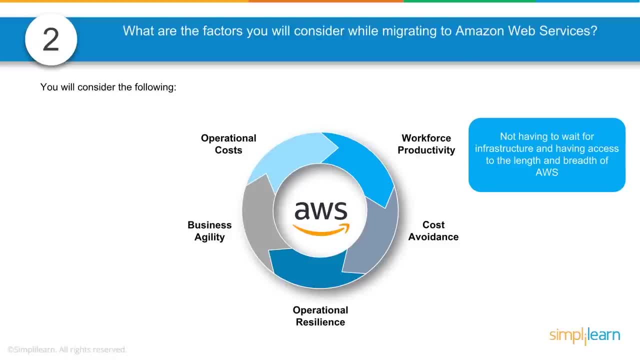 buying an infrastructure, buying the bandwidth, buying the switchboard, you know. buying an instance, you know. buying the software, buying the license related to it. it's going to take time, at least, like two weeks or so, before you can move it to the cloud. so that's a factor to think of, so that's a 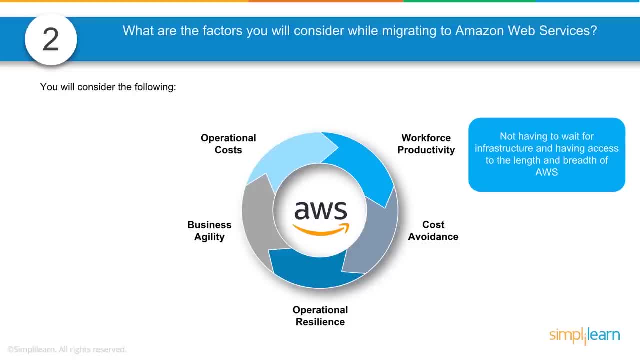 factor to think about. you can bring up an server and launch an application in it, right? so the application cannot wait, you know. waiting means, you know, workforce productivity loss, is it so we would want to immediately launch instances and put application on top of it. in those cases, if your 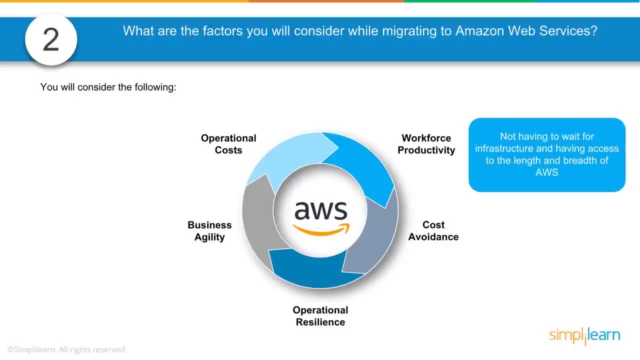 application is of that type, if that is the urge in making the application go online as soon as possible, then that's a candidate for moving to the cloud. and if the application, or if the software, the product that you're launching it, requires hardware, it requires an updated hardware. all the 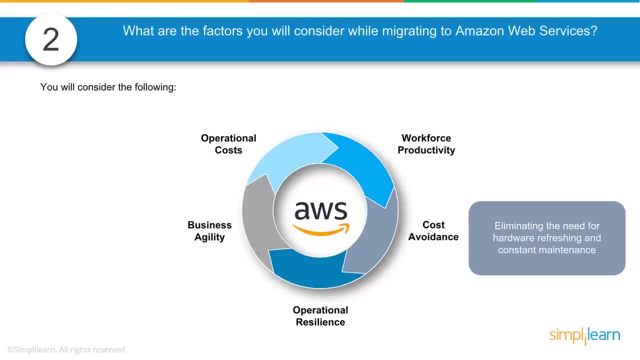 time. that's not going to be possible in on-premises. we try to deal with legacy infrastructure all the time in on-premises, but in the cloud they're constantly upgrading their hardwares. only then they can keep themselves up going in the market. so they're constantly. the cloud providers are. 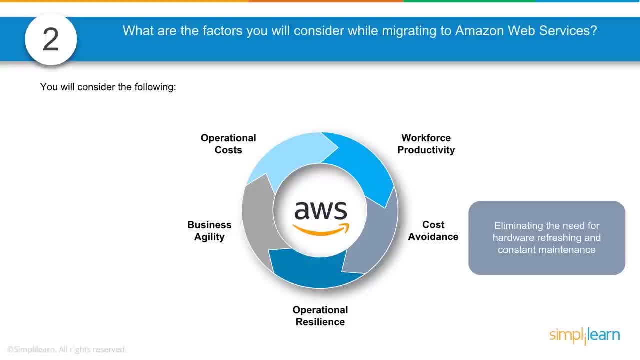 constantly updating their hardwares and if you want to be benefited of your application wants to be benefited by the constant upgrading of the hardware's, making sure the hardware is as latest as possible, the software version, the licensing, is as latest as possible, then that's a candidate to. 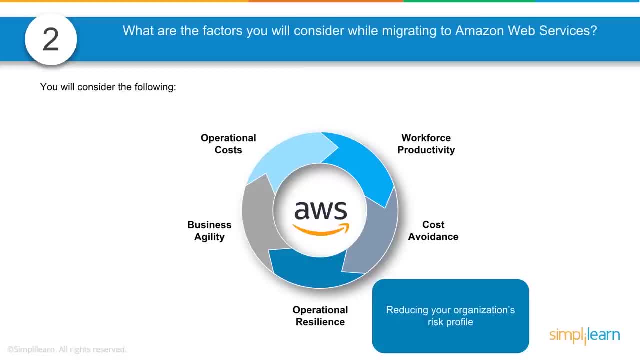 be moved to the cloud and if the application does not want to go through any risk, if the application is very sensitive to failures, if the application is very much tagged to the revenue of the company and you don't want to take a chance in, you know seeing the application fail and you know seeing 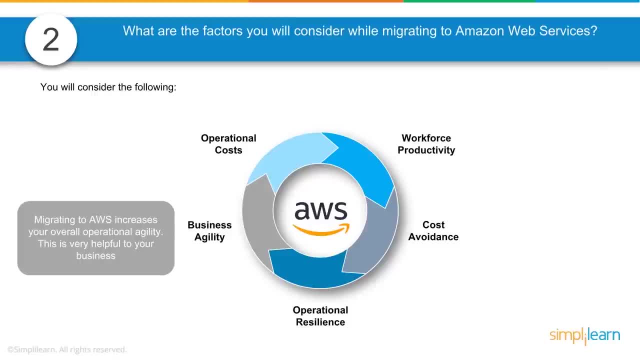 the revenue drop, then that's a candidate for moving to the cloud and business agility. you know, moving to the cloud, at least half of the responsibility is now taken care by the provider. in this case it's amazon. at least half of the responsibility is taken care by them, like if the hardware fails, amazon make sure. 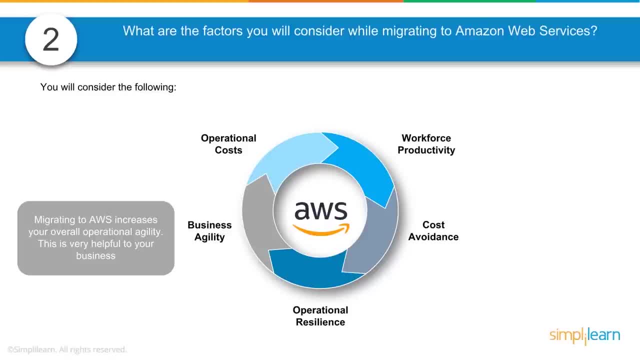 that they're fixing the hardware immediately and notifications. you know if something happens, you know there are immediate notifications available that we can set it up and make ourself aware that something has broken and we can immediately jump in and fix it. so you see, there are. the responsibility is now being. 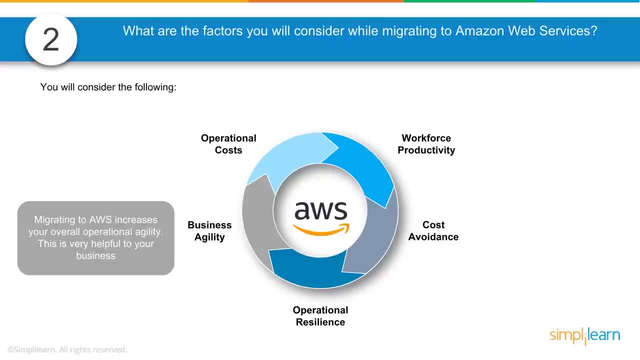 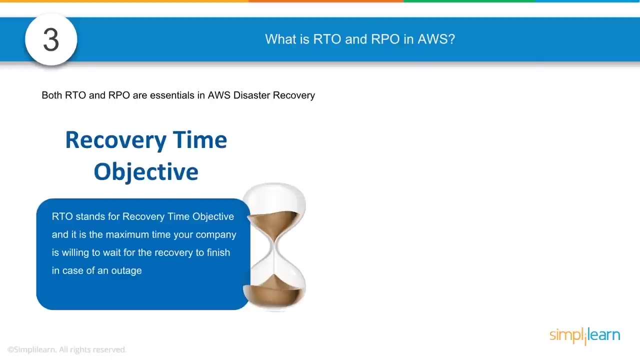 shared between amazon and us. so if you want to get that benefit for your application, for your organization, for the product that you're launching, then it needs to be moved to the cloud so you can get that benefit from the cloud. the other question you could get asked is: what is rto and rpo in aws? 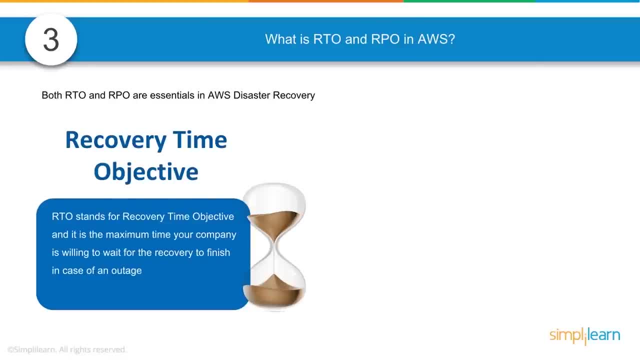 they are essentially disaster recovery terms. when you're planning for disaster recovery, you cannot avoid planning disaster recovery without talking about rto and rpo. now, what's the rto, what's the rpo in your environment, or how do you define rto? how do you define rpo? are some general questions. 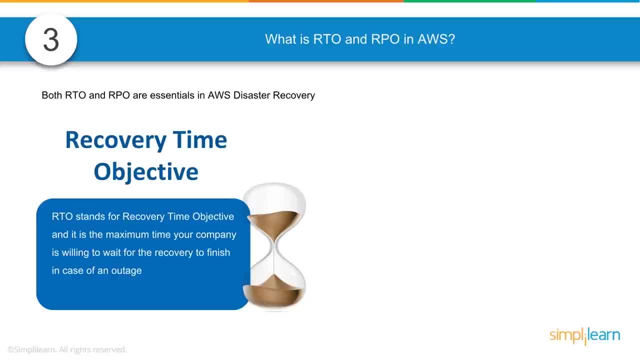 that get asked. rto is recovery time objective. rto stands for the maximum time the company is willing to wait for the recovery to happen or for the recovery to finish when a disaster strikes. so in the future, right, how much time is it going to take to fix and bring everything to normal? so 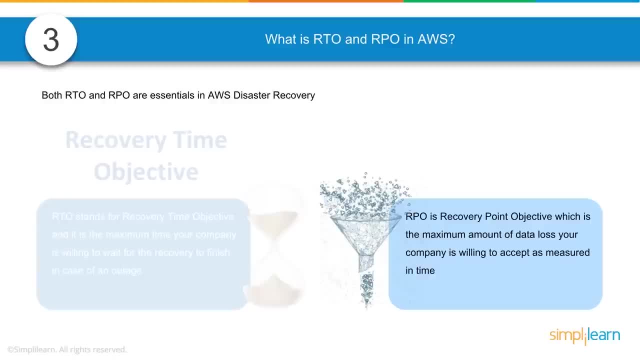 that's rto. on the other hand, rpo is recovery point objective, which is the maximum amount of data loss your company is willing to accept as measured in time. rpo always refers to the backups, the number of backups, the, the frequency of the backups. right, because when an outage happens, you can always go. 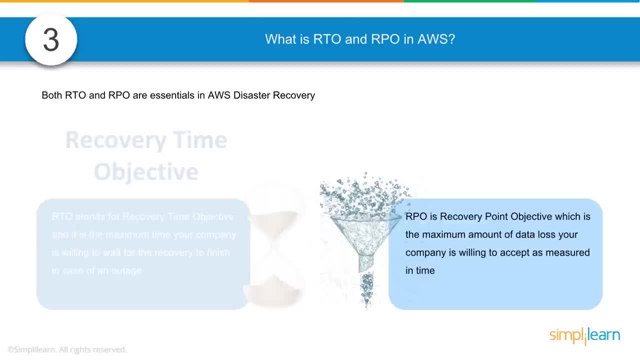 back to the latest data and you can always go back to the latest data and you can always go back to the latest backup right. and if the latest backup was before 12 hours, you have lost the in between 12 hours of data data storage right. so rpo is the acceptable amount. if the company wants less rpo. 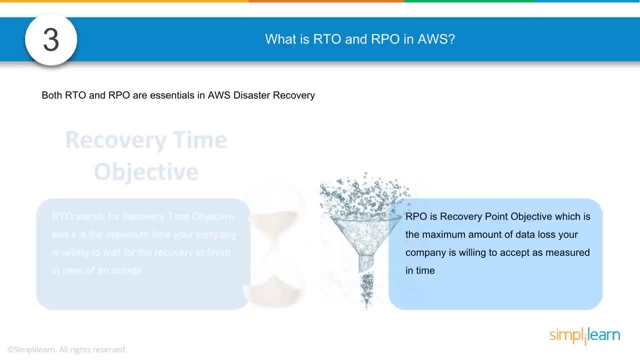 rpo is one hour, then you should be planning on taking backups every one hour. if rpo is 12 hours, then you should be planning on taking backups every 12 hours. so that's how rpo and rto, you know, helps disaster recovery. the fourth question you could get asked is: 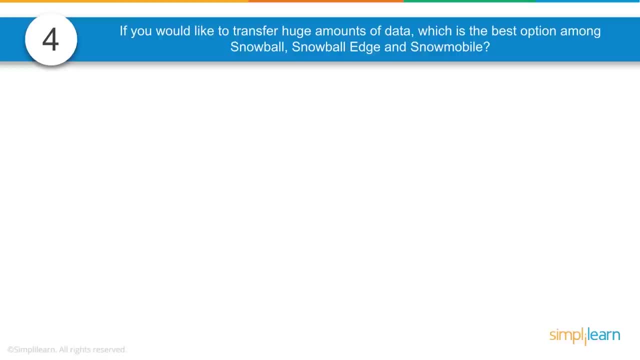 if you would like to transfer huge amount of data, which is the best option among a snowball, snowball edge and snowmobile? again, this is the question that get asked: if the company is dealing with a lot of data transfer into the cloud or if the company is dealing with migrating data into 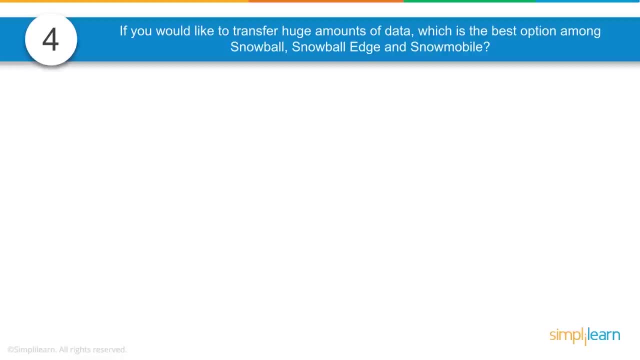 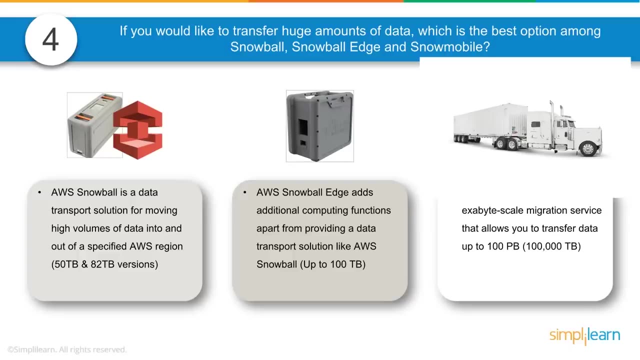 the cloud. i'm talking about a huge amount of data, data in petabytes. snowball and all of the snowball series deals with the petabyte sized data migrations. so if you would like to transfer huge amount of data, there are three options available as of now. aws snowball is an data transfer solution for moving. 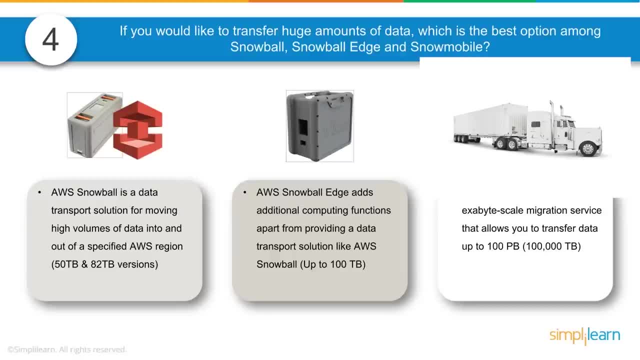 high volume of data into and out of a specified aws region. on the other hand, aws snowball edge has additional computing functions. snowball is simple storage and movement of data, and snowball edge has a compute function attached to it. snowmobile, on the other hand, is an exabyte scale. 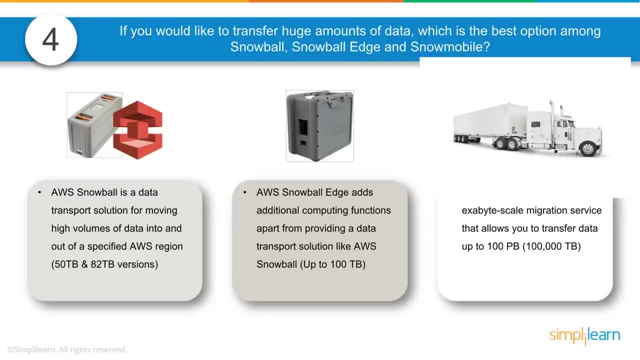 migration service that allows us to transfer data to the cloud, and we can transfer data to the cloud up to 100 petabytes, that's like 100 000 terabytes. so depending on the size of data that we want to transfer from our data center to the cloud, we can hire, we can rent any of these three services. let's 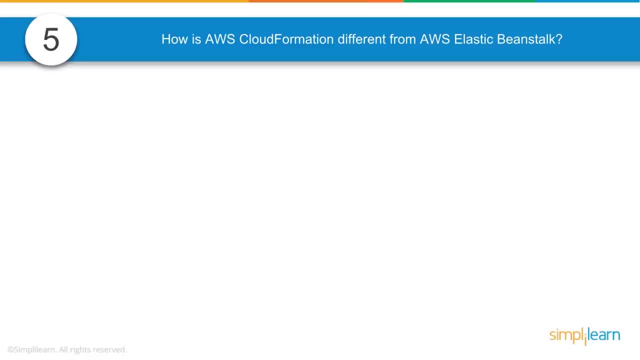 talk about some cloud formation questions. this is a classic question: how is aws cloud formation different from aws elastic beanstalk? you know, from the surface they both look like the same. you know you don't go through the console provisioning resources. you don't. you know you don't go through cli and provision resources. 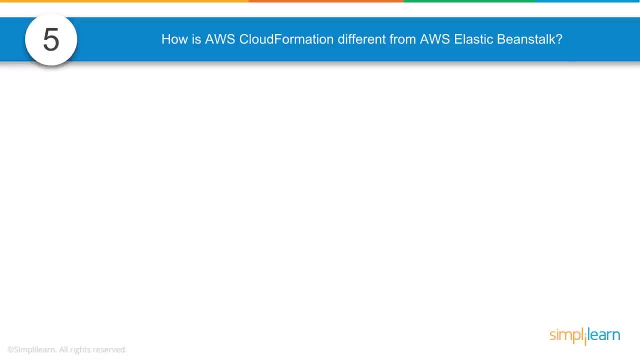 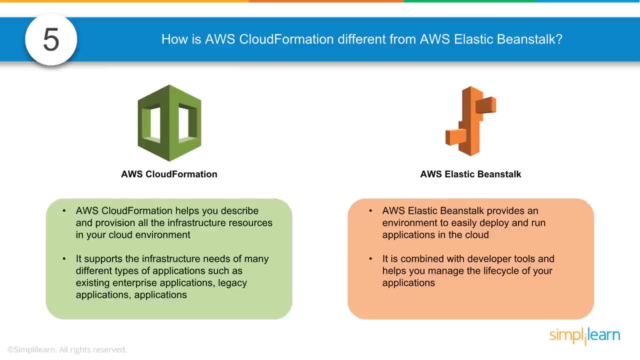 both of them provision resources through click button right, but underneath they are actually different services. they support, they aid different services. so knowing that is going to help you understand this question a lot better. let's talk about the difference between them and this is what you will be explaining to the interviewer or the panelist. so the cloud formation, the cloud formation. 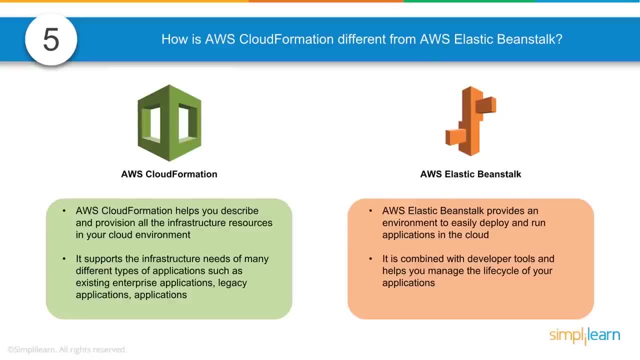 service helps you describe and provision all the infrastructure resources in the cloud environment. on the other hand, elastic beanstalk provides an simple environment to which we can deploy and run application. cloud formation gives us an infrastructure and elastic beanstalk gives us an small, contained environment in which we can run our application, and cloud formation supports the infrastructure. 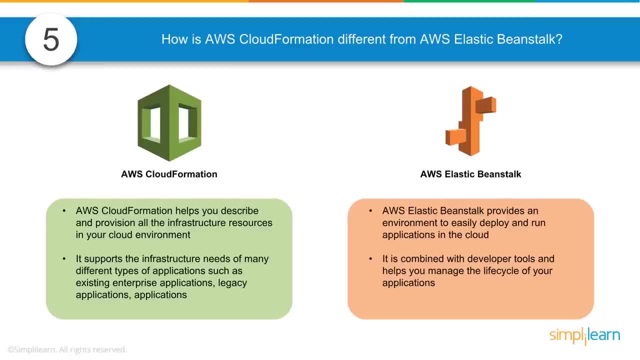 needs of many different types of application, like the enterprise application, the legacy applications and any new modern application that you want to have in the cloud. On the other hand, the Elastic Beanstalk- it's a combination of developer tools. They are tools that helps manage the lifecycle of a single. 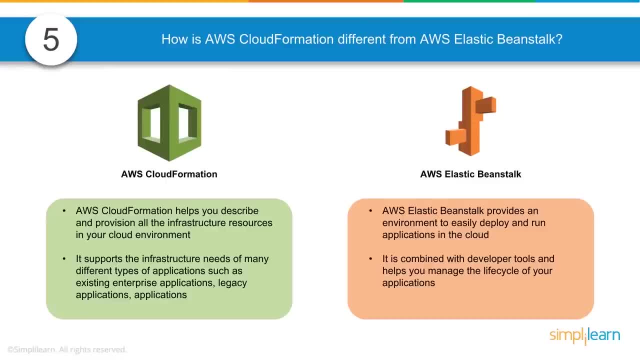 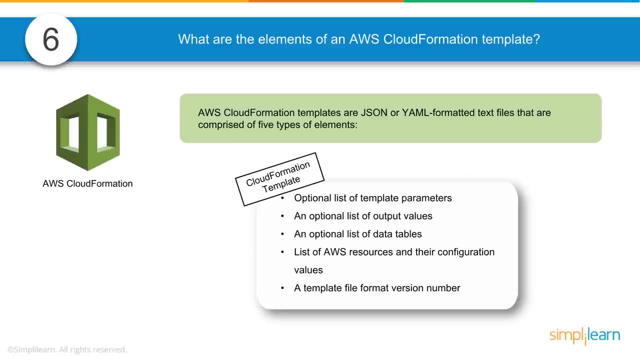 application. So cloud formation, in short, is managing the infrastructure as a whole and Elastic Beanstalk, in short, is managing and running an application in the cloud. And if the company that you're getting hired is using cloud formation to manage their 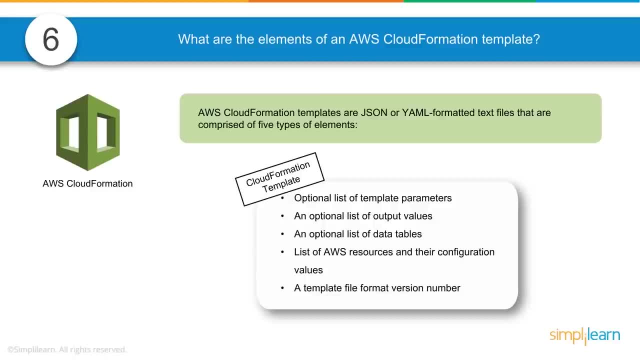 infrastructure, or if they're using infrastructure or any of the infrastructure as a code services, then you would definitely face this question: what are the elements of an AWS cloud formation template? So it has four or five basic elements, right, And the template is in the form. 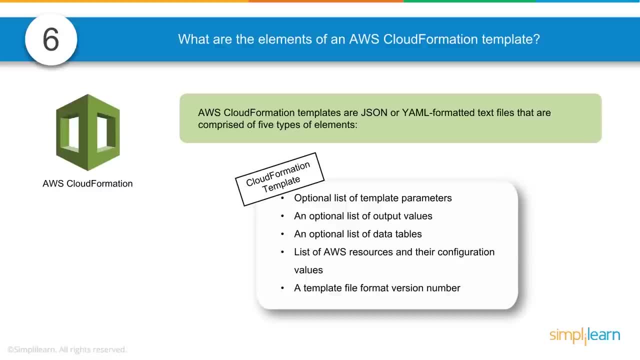 of JSON or in YAML format, right. So it has parameters, it has outputs, it has data, it has resources and then the format or the format version or the file format version for the cloud formation template. So parameter is nothing, but it. 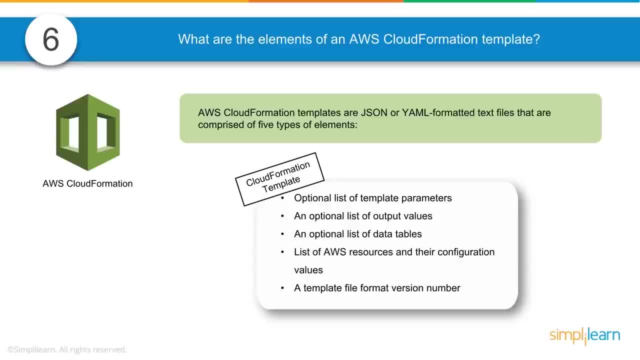 actually lets you to specify the type of EC2 instance that you want, the type of RDS that you want, right? So EC2 is an umbrella, RDS is an umbrella and parameters within that, EC2 and RDS are the specific details of the EC2 or the specific details of the RDS service. So that's. 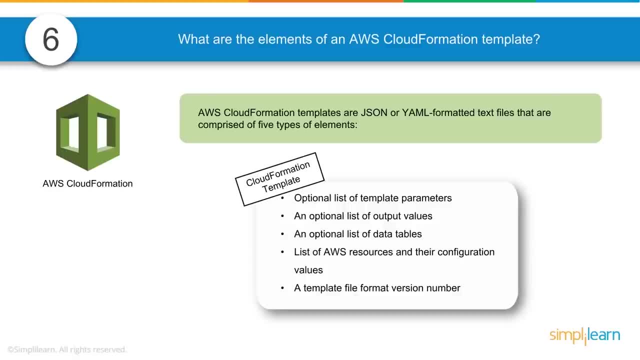 what parameters in a cloud formation template. And then the element of the cloud formation template is outputs. For example, if you want to output the name of an S3 bucket that was created, if you want to output the name of the EC2 instance, if you want to output the name of 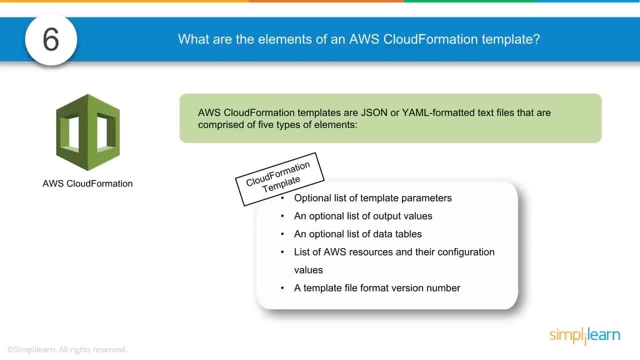 some resources that have been created. instead of looking into the template, instead of, you know, navigating through in the console and finding the name of the resource, we can actually have them outputted in the result section, So we can simply go and look at all the resources created through the template in. 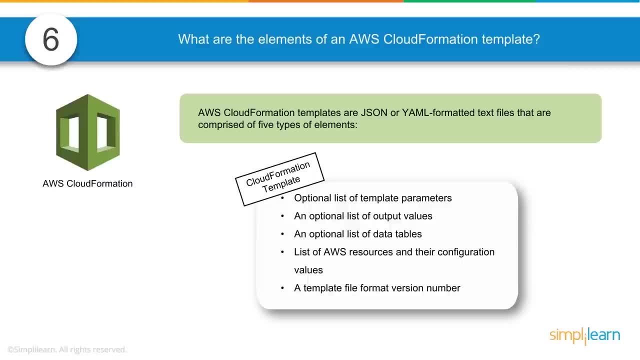 the output section And that's what output values or output does in the cloud formation template. And then we have the resources. Resources are nothing but what defines what are the cloud components or cloud resources that will be created through this cloud formation template. Now, EC2 is a resource, RDS is a resource And S3 bucket is a resource. Elastic load balancer is a resource. 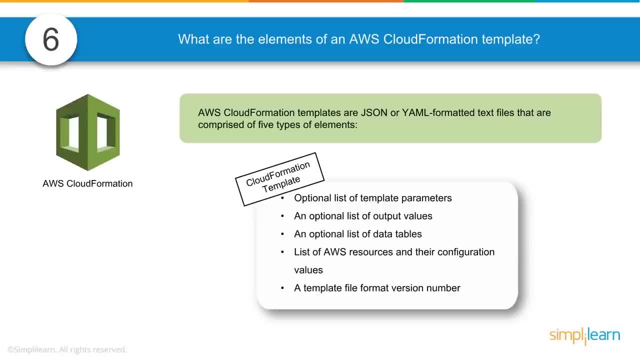 And NAT gateway is a resource, VPC is a resource. So you see, all these components are the resources, And the resource section in the cloud formation defines what are the AWS cloud resources that will be created through this cloud formation template, And then we have version Version actually. 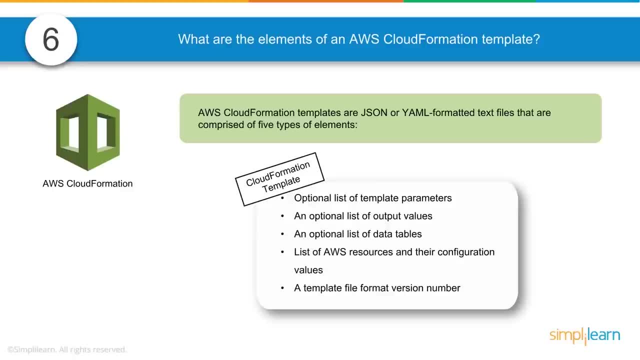 identifies the capabilities of the template. You know, we just need to make sure that it is of the latest version type, And the latest version is 0909 2010.. That's the latest version number. You'll be able to find that on the top of the cloud formation template And that version number defines: 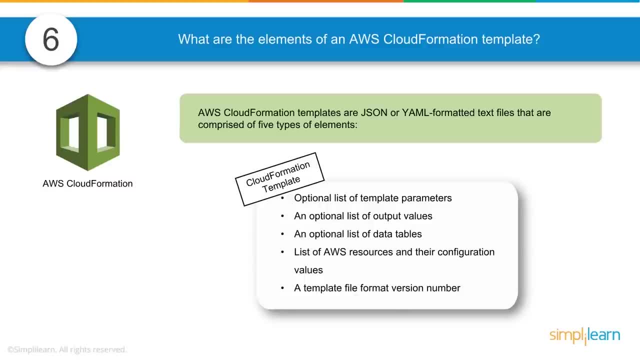 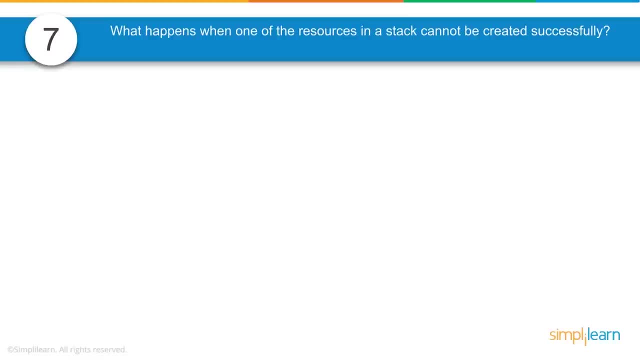 the capabilities of the cloud formation template, So just need to make sure that it's the latest all the time. Still talking about cloud formation, this is another classic question. What happens when one of the resources in the stack cannot be created successfully? Well, if the resources 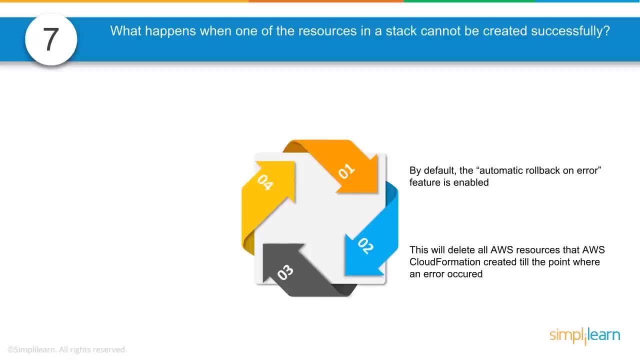 If a resource in a stack cannot be created, the CloudFormation automatically rolls back and terminates all the resources that was created using the CloudFormation template. So whatever resources that were created through the CloudFormation template from the beginning, let's say we have created like 10 resources and the 11th resource is now failing CloudFormation. 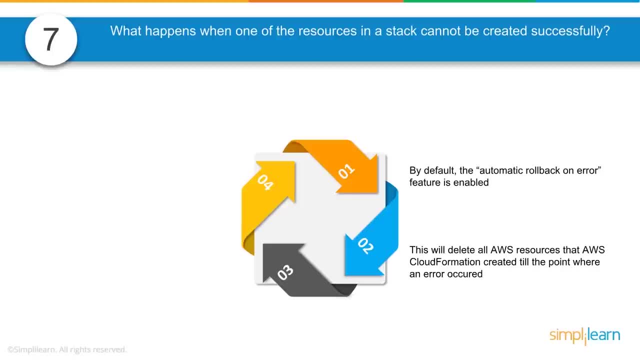 will roll back and delete all the 10 resources that were created previously, And this is very useful when the CloudFormation cannot go forward. CloudFormation cannot create additional resources because we have reached the elastic IP limits. Elastic IP limit per region is 5, and if you have already used 5 IPs and your CloudFormation 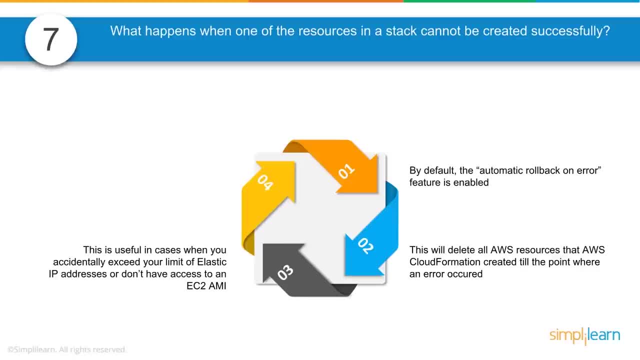 is trying to buy 3 more IPs. we have hit the soft limit. Till we fix that with Amazon, CloudFormation will not be able to launch additional resources and additional IPs, So it's going to cancel and roll back everything. That's true with a missing EC2 AMI as well. 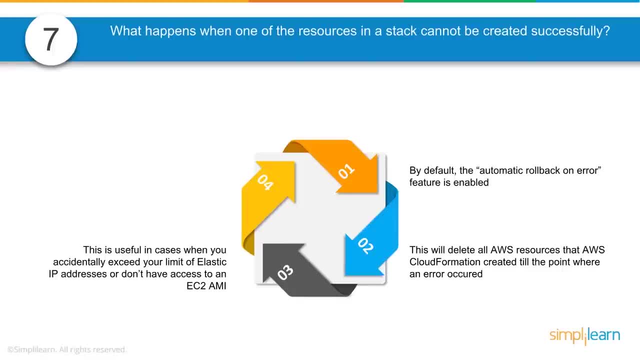 If an AMI is included in the template but the AMI is not actually present, then CloudFormation is going to search for the AMI and, because it's not present, it's going to roll back and delete all the resources that it created. 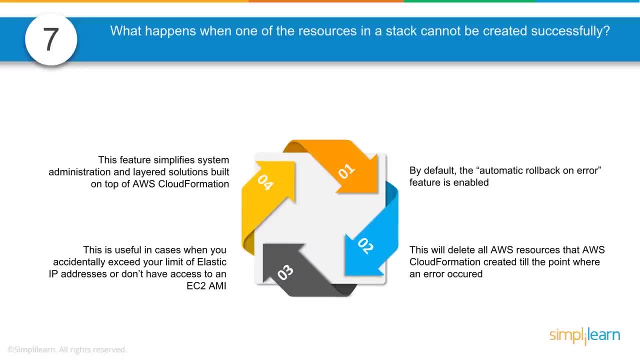 So that's what CloudFormation does: it simply rolls back all the resources that it created. If it sees a failure, it would simply roll back all the resources that it created, And this feature actually simplifies the system administration and layered solutions built on top of AWS CloudFormation. 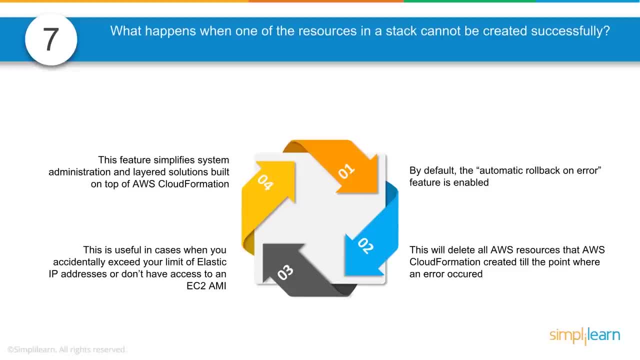 So at any point we know that there are no orphan resources in our environment because something did not work or because CloudFormation executed some. there are no orphan resources in our account At any point. we can be sure that if CloudFormation is launching a resource and if it's going, 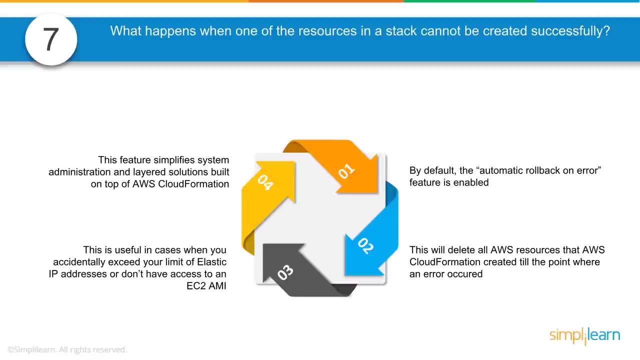 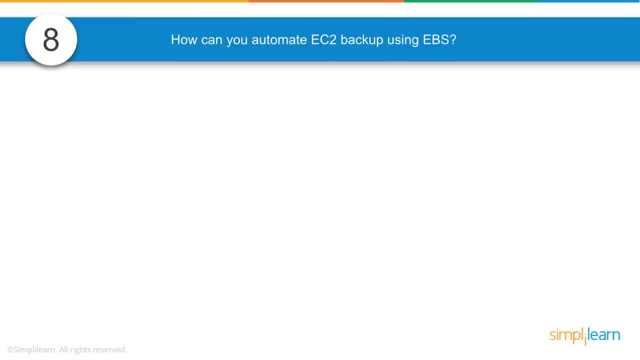 to fail, It's going to roll back all the resources it's created, so there are no orphan resources in our account. Now let's talk about some questions in Elastic Block Store Again, if the environment deals with a lot of automation, you could be thrown this question. 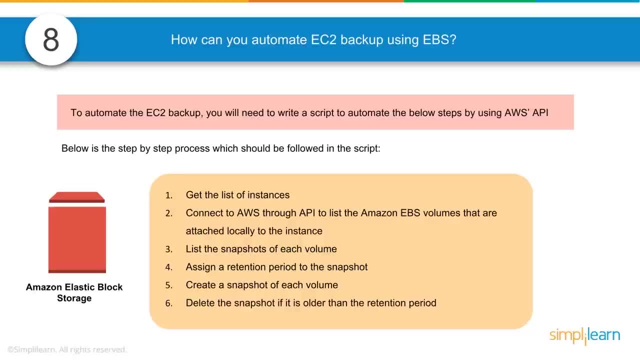 how can you automate EC2 backup using EBS? It's actually a six-step process To automate the EC2 backups. we'll need to write a script to automate the below steps using AWS API, And these are the steps that should be found in the scripts. 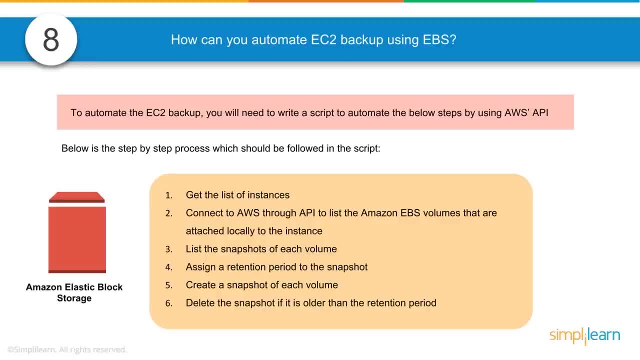 1. Connect the list of instances, And then the script that we are writing should be able to connect to AWS using the API and list the Amazon EBS volumes that are attached locally to the instance, And then it needs to list the snapshots of each volume. 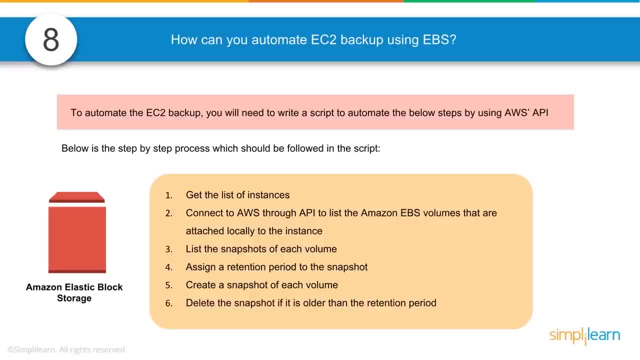 Make sure the snapshots are present And it needs to assign a retention period for the snapshot because over time the snapshots are going to be invalid. right Once you have some 10 latest snapshots, Any snapshot that you have taken before that 10 becomes invalid because you have captured. 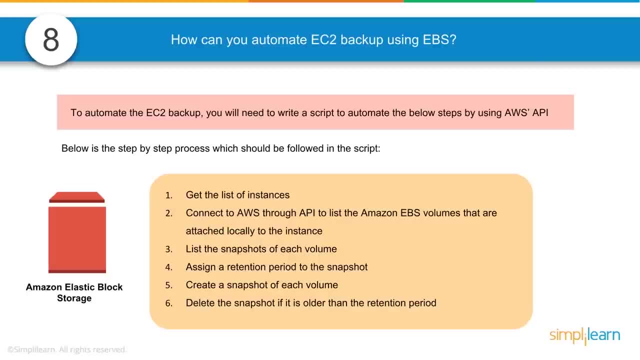 the latest and 10 snapshot coverage is enough for you. And then the fifth point is to create a snapshot of each volume, create a new snapshot of each volume and then delete the old snapshot Anytime a new snapshot gets created. the oldest snapshot in the list needs to go away. 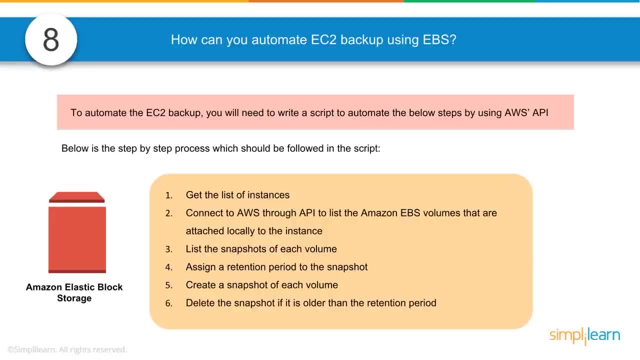 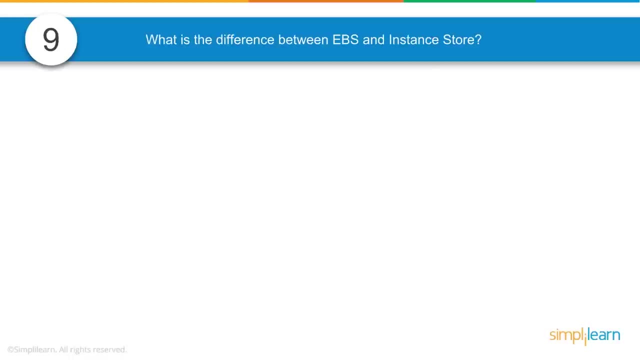 So we need to include options, we need to include scripts in our script, lines in our script That make sure that it's deleting the older snapshots which are older than the retention period that we are mentioning. Another question that you could see in the interview, be it a written interview, be it. 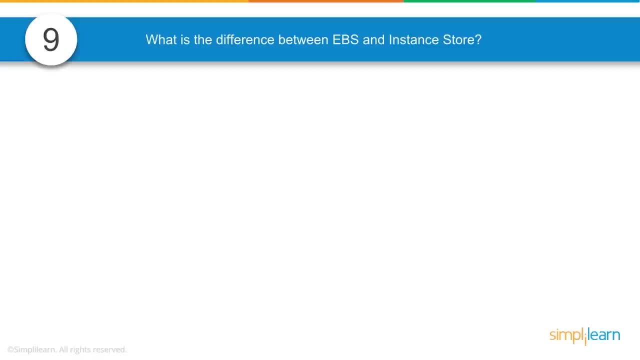 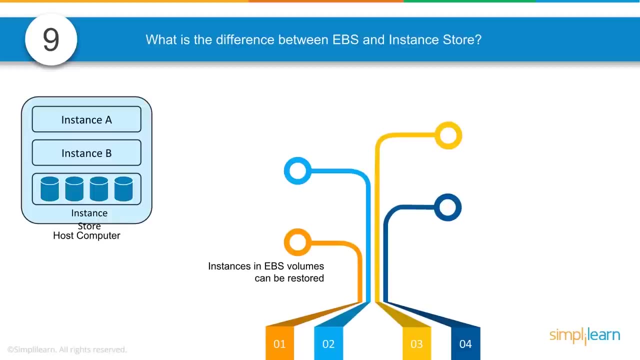 online interview, or be it a telephonic or face-to-face interview, is what's the difference between EBS and instant store? Let's talk about EBS first. EBS is kind of permanent storage. The data in it can be restored at a later point. 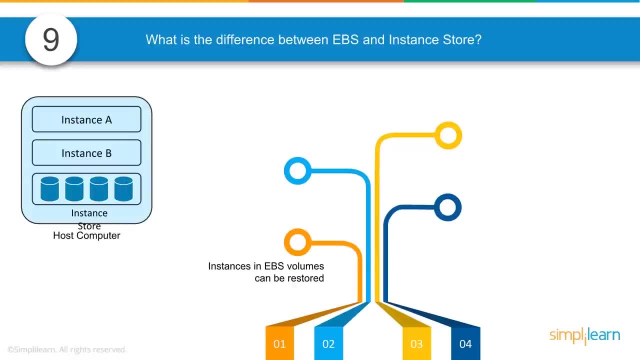 When we save data in EBS, we can save data in EBS. We can save data in EBS. The data lives even after the lifetime of the EC2 instance, For example. we can stop the instance and the data is still going to be present in EBS. 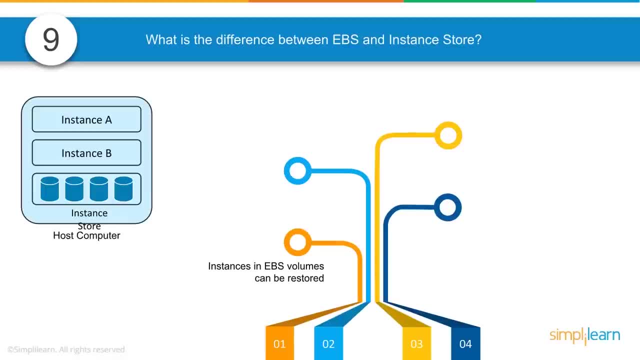 We can move the EBS from one instance to another instance and the data is simply going to be present there. So EBS is kind of permanent storage when compared to instance. On the other hand, instance store is temporary storage and that storage is actually physically. 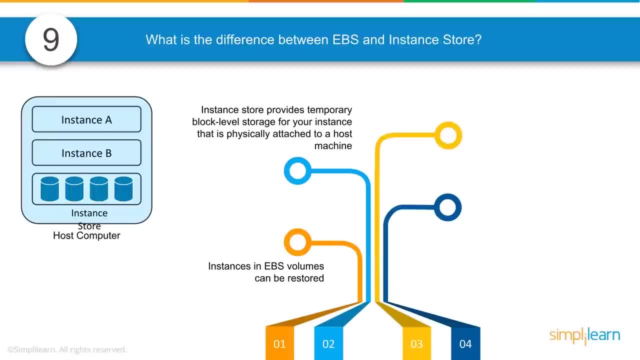 attached to the host. That's what we call EBS. EBS is an external storage and instance store is locally attached to the instance or locally attached to the host of the machine. We cannot detach an instance store from one instance and attach it to another, but we 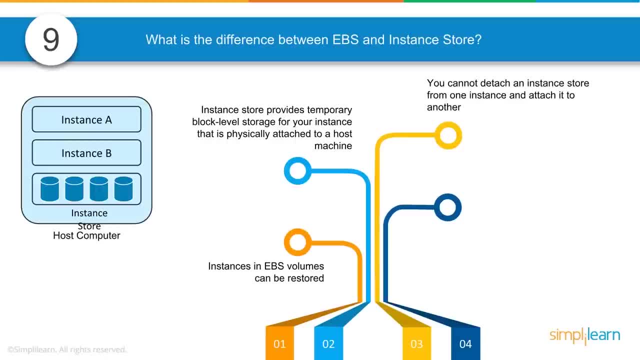 can do that with EBS. So that's a big difference. One is permanent data and another one is EBS is permanent. Instance store is a volatile data and instance store. with instance store we won't be able to detach The storage and attach it to another instance. 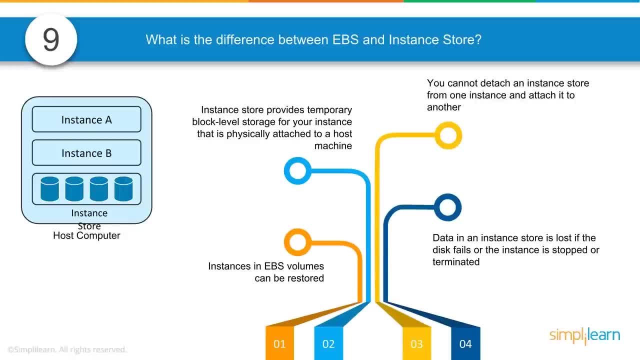 And another feature of instance store is data in an instance store is lost if the disk fails or the instance is stopped or terminated. So instance store is only good for storing cache data. If you want to store permanent data, then we should think of using EBS and not instance. 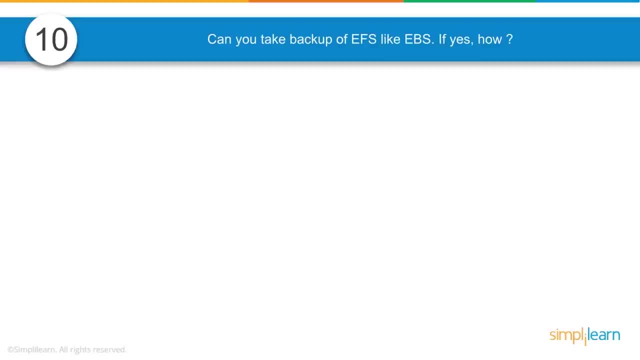 store. Well, talking about storage on the same lines, this is another classic question: How can you take backups of EFS? What is EFS Like EBS, And if you can take backup, how do you take that backup? The answer is yes, we can take EFS to EFS backup solution. 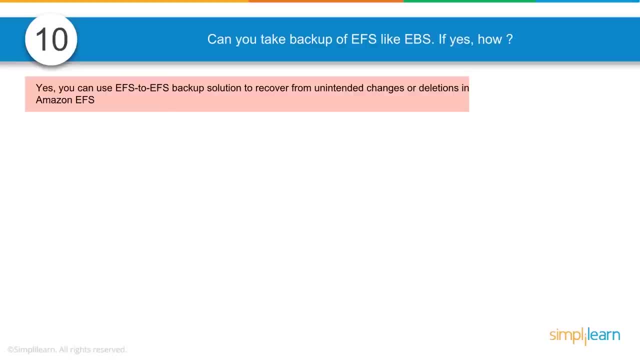 EFS does not support snapshot. Like EBS, EFS does not support snapshot. Snapshot is not an option for EFS elastic file system. We can only take backup from one EFS to another EFS And this backup solution is to recover from unintended changes or deletions of the EFS. 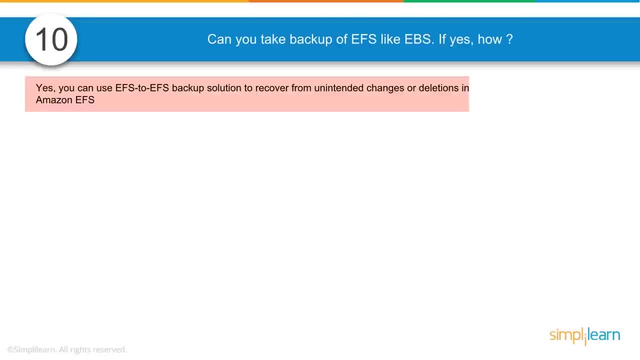 And this can be automated. Any data that we store in EFS can be automatically replicated to another EFS And once this EFS goes down or gets deleted, or data gets deleted or the whole EFS is for some reason interrupted or deleted, we can recover the data from. we can use the other. 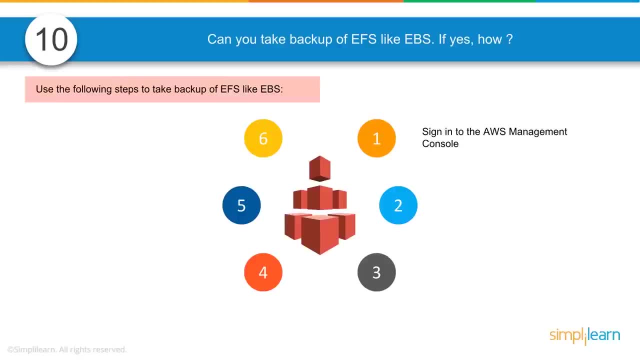 EFS and bring the application to consistency. And to achieve this it's not an one step configuration, It's a cycle. There are series of steps that's involved before we can achieve EFS. The first thing is to sign in to the AWS management console and, under EFS, or click on EFS to 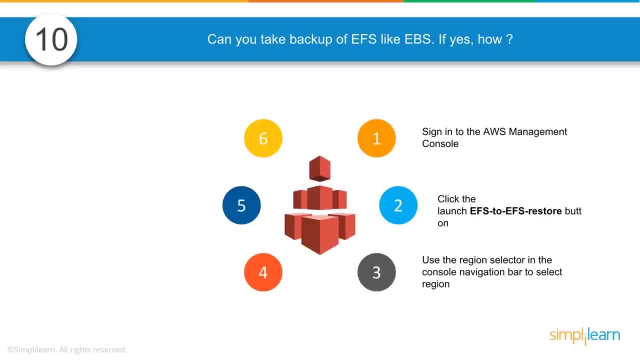 EFS restore button from the services list And from there we can use the region selector in the console navigation bar to select the actual region in which we want to work on And from there ensure that we have selected the right template. Some of the templates would be EFS to EFS backup. 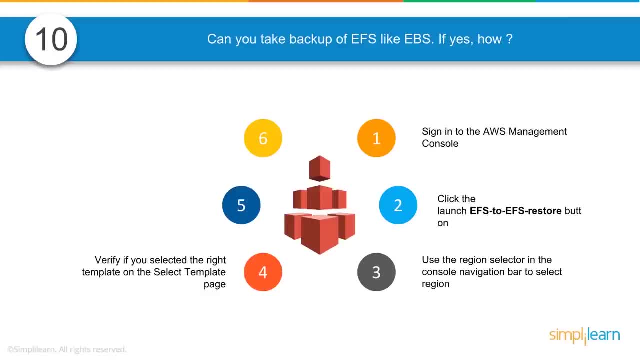 Granular backups, incremental backups. so there are some templates, the kind of backups that you want to take. Do you want to take granular? do you want to take increment backups, stuff like that, And then create a name to that solution, the kind of backup that we have created. 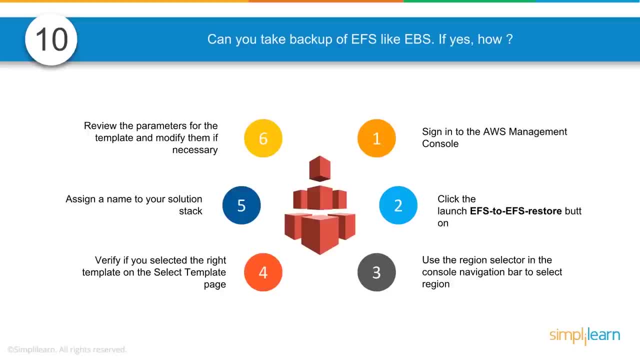 And finally review all the configurations that you have done and click on save And from that point onwards, the data is going to be copied And from that point onwards, any additional data that you put is going to copy it and replicated. Now you have an EFS to EFS backup. 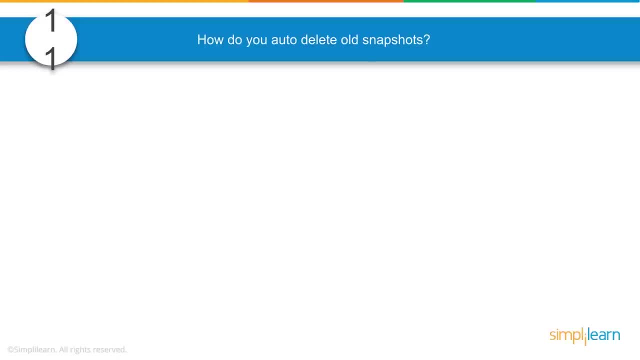 This is another classic question in companies which deals with data management. There are easy options to create snapshots, but deleting snapshots is not always a click button or a single step configuration. So you might be facing a question like: how do you auto delete old snapshots? 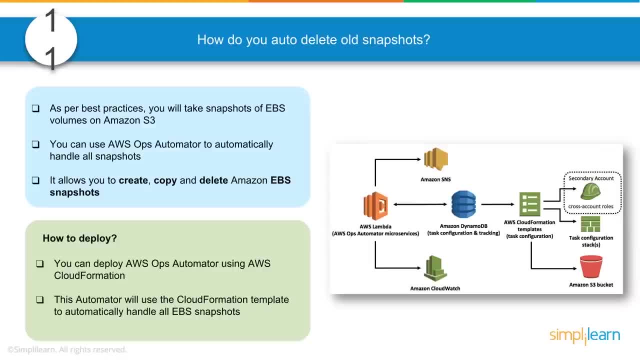 And the procedure is like this: Now, as best practice, We will take snapshots of EBS volume to S3.. All snapshots get stored in S3.. We know that now And we can use AWS Ops Automator to automatically handle all snapshots. 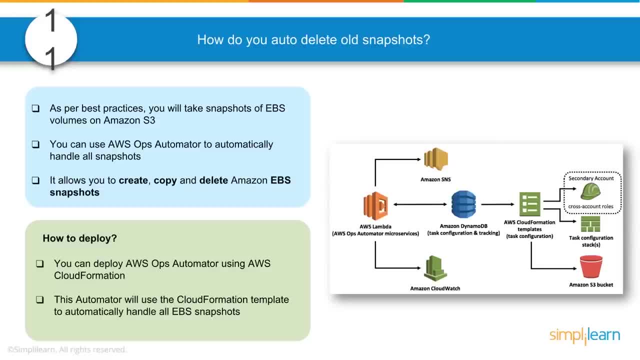 The Ops Automator service. it allows us to create, copy, delete EBS snapshots. So there are cloud formation templates available for AWS Ops Automator and this Automator template will scan the environment And it would take snapshots. it would copy the snapshot from one region to another region. 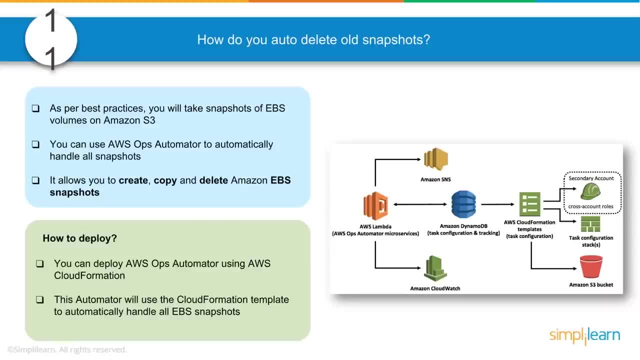 if you want. I know if you're setting up a DR environment, And not only that, based on the retention period that we create, it's going to delete the snapshots which are older than the retention period. So life or managing snapshot is made a lot easier because of this. Ops Automator cloud. 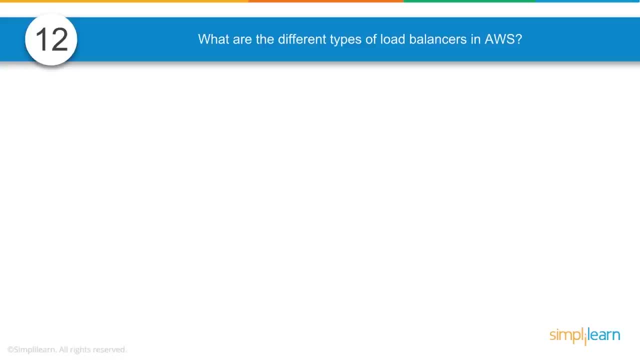 formation template. Moving into questions in Elastic Load Balancer, This again could be an A question in the interview. What are the different types of load balancers in AWS and what's their use case? What's the difference between them? And as of now, as we speak, there are three types of load balancers which are available. 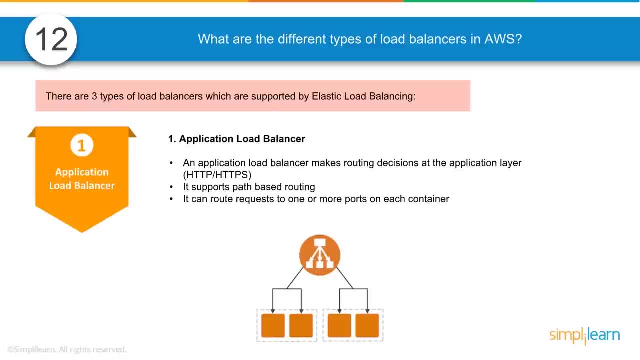 in AWS, The first one being application load balancer. Just like the name says, the application load balancer works on the application layer and deals with the HTTP and HTTPS requests, And it also supports path based routing, For example, simplylearncom. 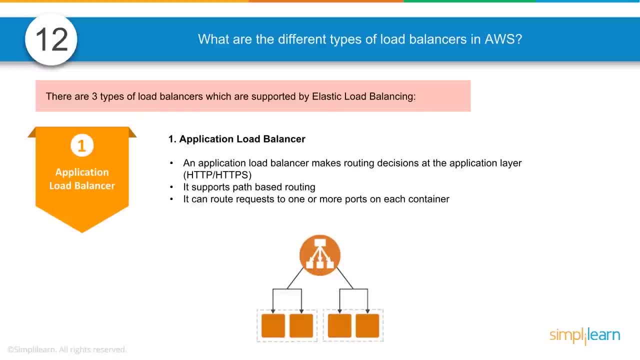 Slash some web page, Simplylearncom Slash another website, So it's going to direct the path based on the slash value that you give in the URL. That's path based routing. So it supports that, And not only that, it can support a port based colon 8080,, colon 8081, or colon 8090. 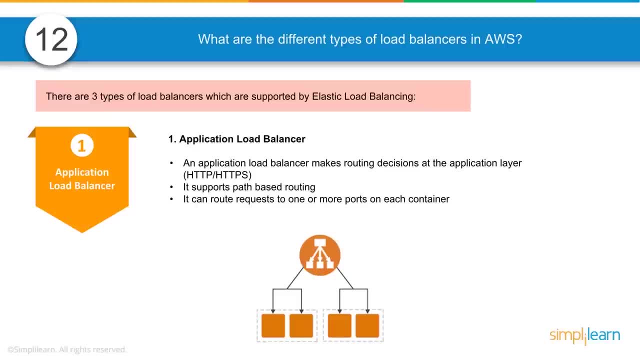 Based on that port. also, it can take a routing decision, And that's what application load balancer does. On the other hand, We have network load balancer And the network load balancer makes routing decisions at the transport level. It's faster because it has very less thing to work on. 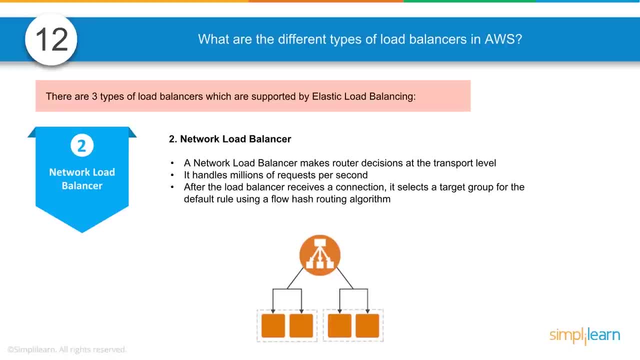 It works on lower OSI layer. It works on a lower layer So it has very less information to work with than compared with application layer. So comparatively it's a lot faster and it handles millions of requests per second. And after the load balancer receives the connection, it selects a target group for the default rule. 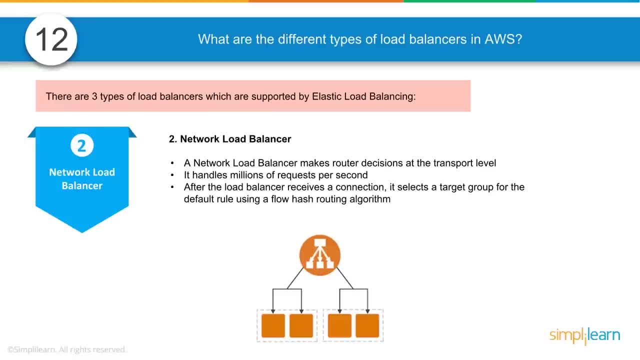 using the flow header. It's a slow, hash routing algorithm. It does simple routing. It does not do path based or port based routing. It does simple routing and because of it it's faster. And then we have classic load balancer, which is kind of expiring as we speak. 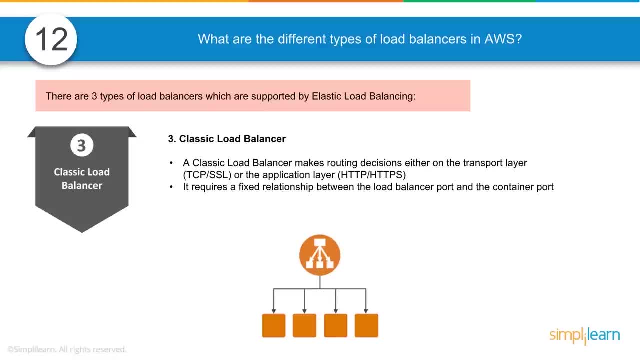 Amazon is discouraging people using classic load balancer, But there are companies which are still using classic load balancer. They are the ones were the first one to step into Amazon when classic load balancer was the first load balancer or the only load balancer available at that point. 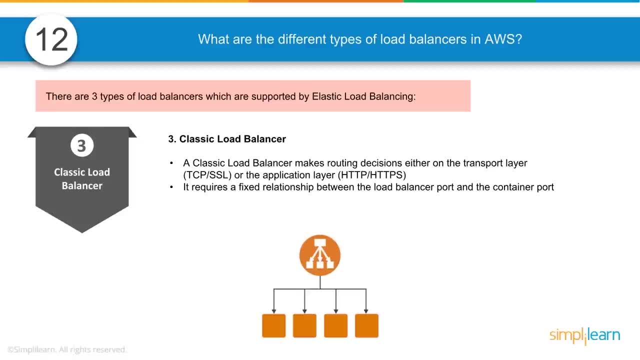 So it's a lot faster. It supports HTTP, HTTPS, TCP, SSL protocol And it has a fixed relationship between a load balancer port and the container port. So initially we only have classic load balancer And then after some point, Amazon said, instead of having one load balancer, address all type. 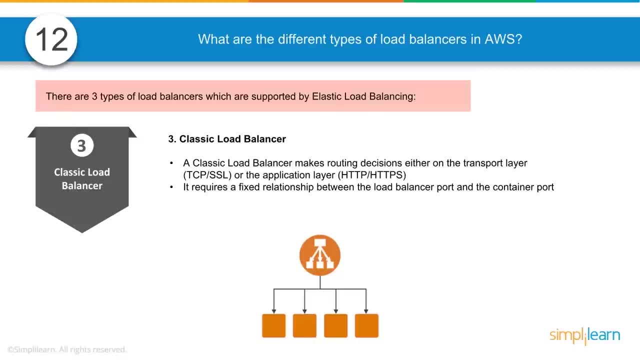 of traffic. we're going to have two load balancers, called as the child from the classic, two load balancer, And one is going to specifically address the application requirement and one is going to specifically address the network requirement, And let's call it as application requirement. 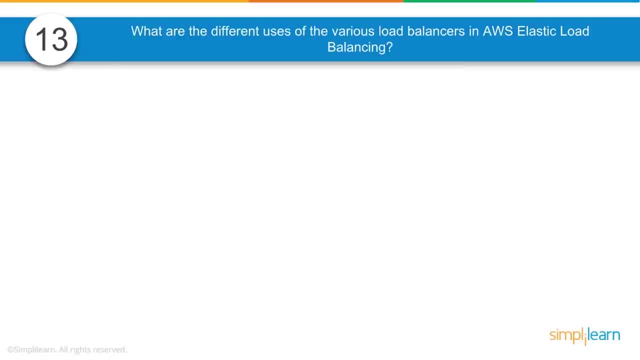 Application load balancer and network load balancer. So that's how now we have two different load balancers. Talking about load balancer, another classic question could be: what are the different uses of the various load balancer in AWS Elastic Load Balancing? 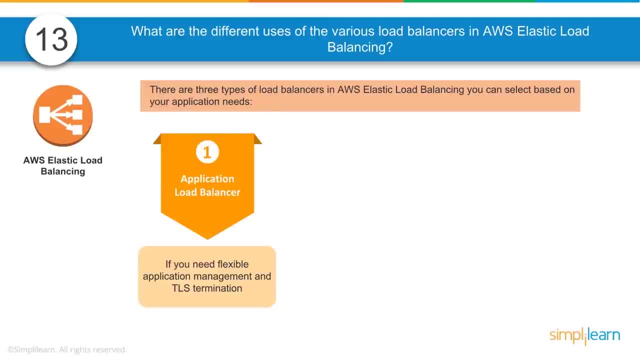 There are three types of load balancer. We just spoke about it. Application load balancer is used if we need a flexible application management and a TLS termination. And network load balancer if we require extreme performance and the load balancing should happen on based on static ID. 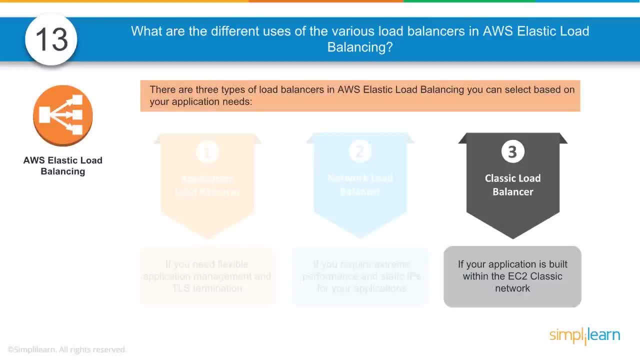 So that's how we have two different load balancers. Application load balancer is used if we need a flexible application management and TLS termination, And a classic load balancer is an old load balancer which is for people who are still running their environment from EC2 classic network. 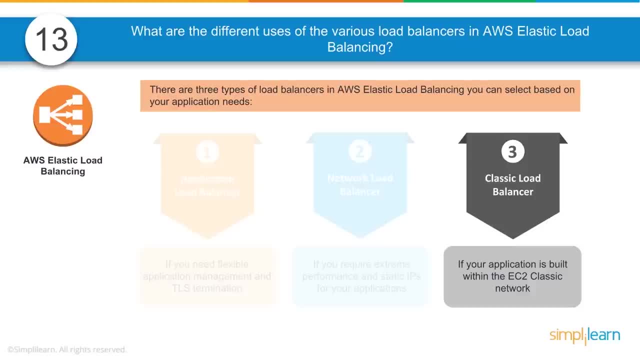 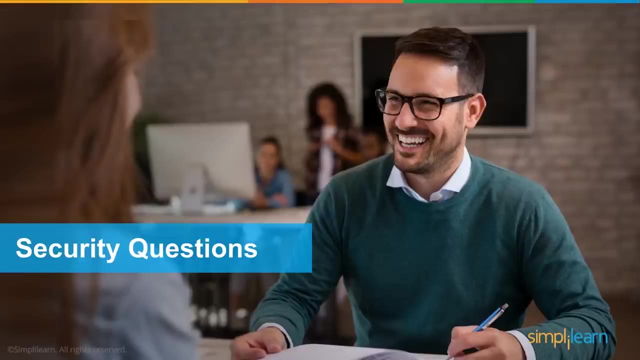 Now this is an older version of VPC or this is what was present before VPC was created. EC2- classic network- is what was present before EC2 was created. So they are the three types and they are the use cases of it. Let's talk about some of the security related questions you would face in the interview. 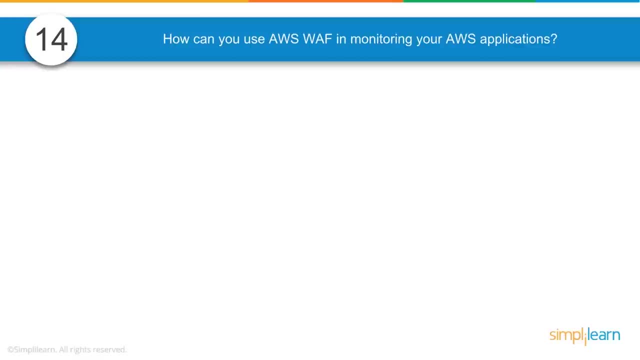 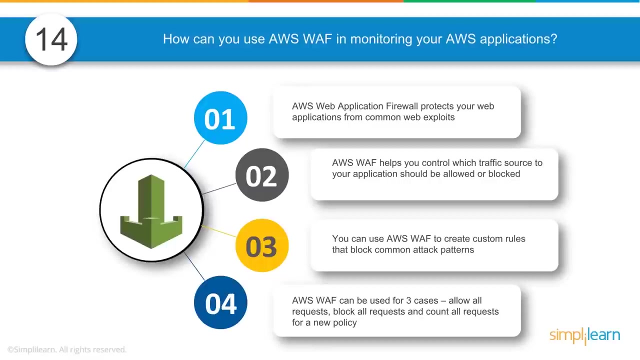 So on. talking about security and firewall in AWS, we cannot avoid discussion. talking about WAF, Web Application Firewall- and you would definitely see yourself in this situation where you have been asked: how can you use AWS WAF in monitoring your AWS applications? WAF, or Web Application Firewall, protects our web application from common web exploits. 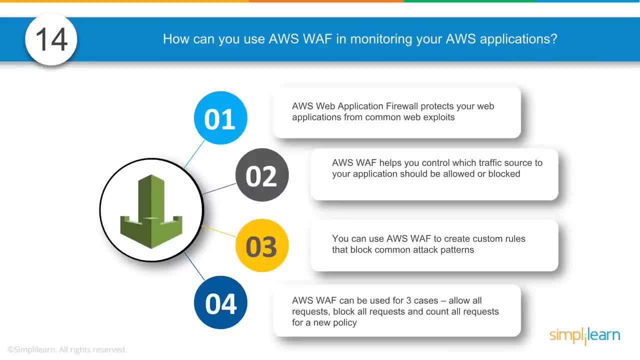 And WAF helps us control which traffic source your application should be allowed to access. We can use this information to control what traffic source your application should be allowed or a block, which traffic from certain source and which source or which traffic from a certain source should be allowed or blocked your application. 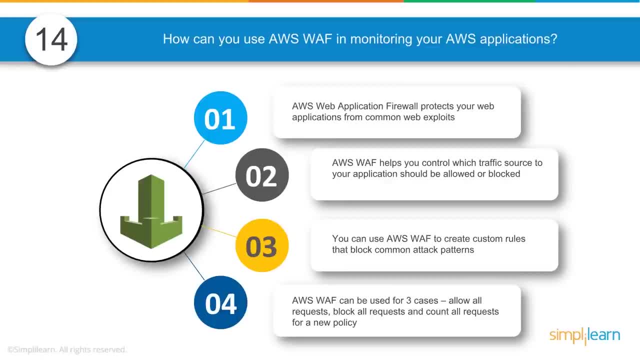 with WAF we can also create custom rules that blocks common attack patterns. you know, if it is a banking application, it has a certain type of attacks and if it is simple data management- data storage application it has. I mean content management application- it has a separate type of attack. so, based on the 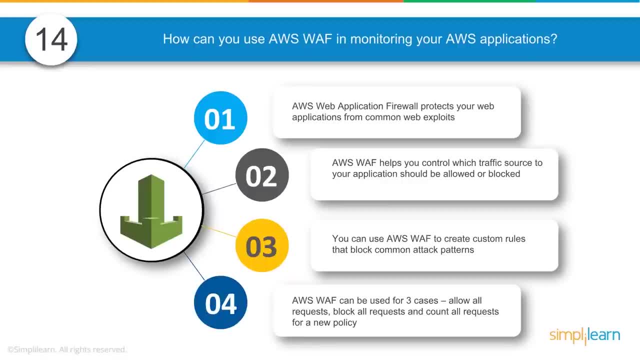 application type, we can identify a pattern and create rules that would actually block that attack based on the rule that we create. and WAF can be used for three cases, you know. the first one is allow all requests and then a block all requests and count all requests for a new policy. so it's also an monitoring. 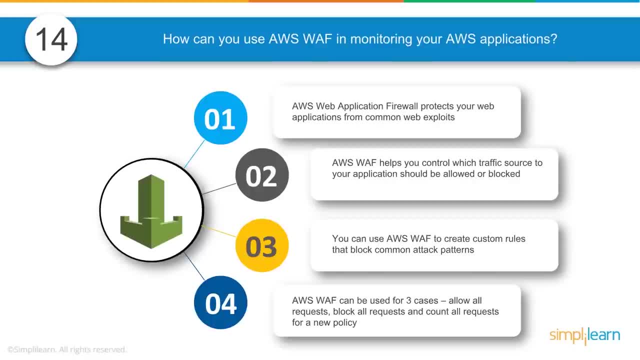 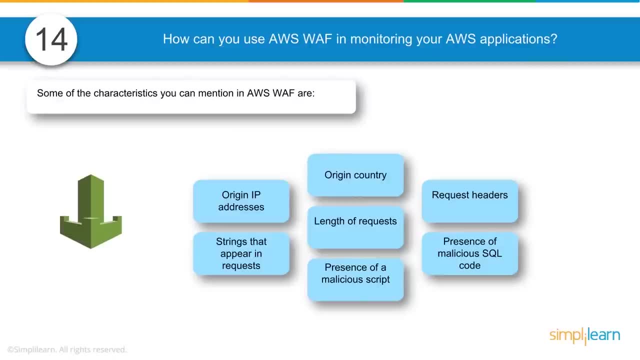 and management service which actually counts all the policies or counts all the requests that matches a particular policy that we create. and some of the characteristics of a WAF application are the following characteristics we can mention in AWS WAF or the origin IPs and the strings that appear in the request. we can allow block based on origin IP. allow block. 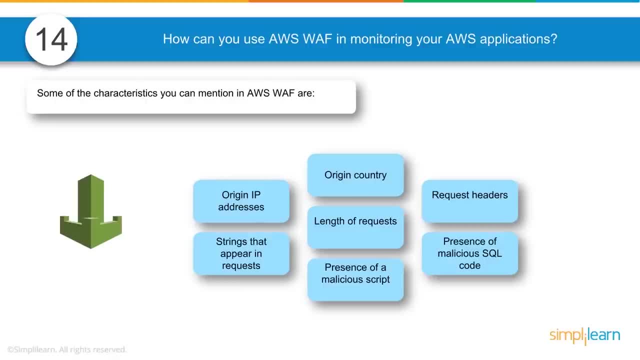 based on strings that appear in the request. we can allow, block or count based on the origin country, length of the request. yeah, we can block and count the presence of malicious scripts in an connection. now we can count the request headers. or we can allow, block a certain request header and we can count the. 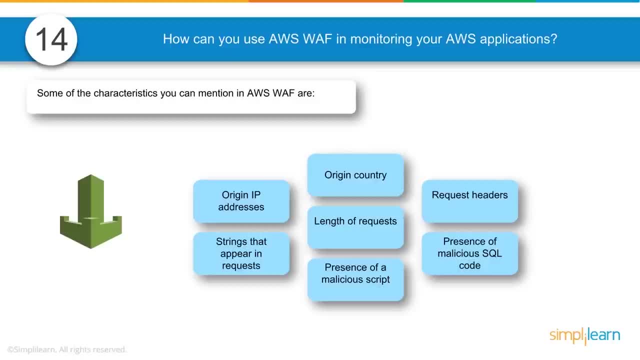 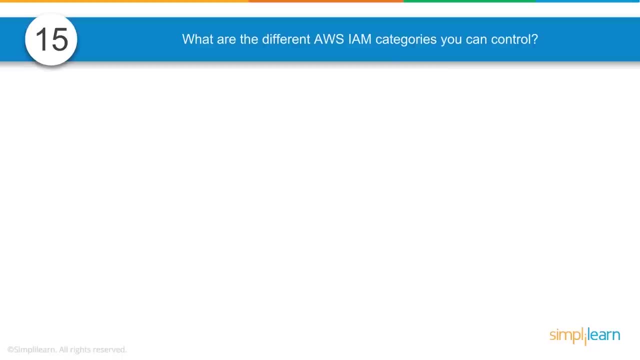 of malicious SQL code in a connection that we get and that want to reach our application. Still talking about security, what are the different AWS IAM categories we can control? Using AWS IAM, we can do the following. One is create and manage IAM users And once the user 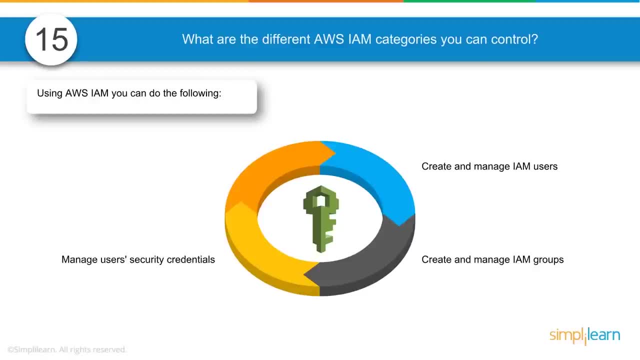 database gets bigger and bigger. we can create and manage them in groups And in IAM. we can use it to manage the security credentials kind of setting the complexity of the password. you know setting additional authentications, you know like MFA and you know rotating the. 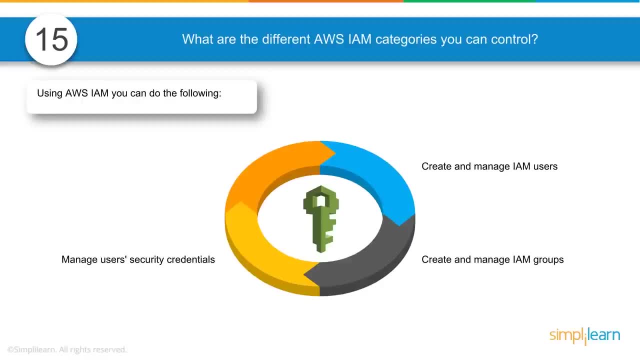 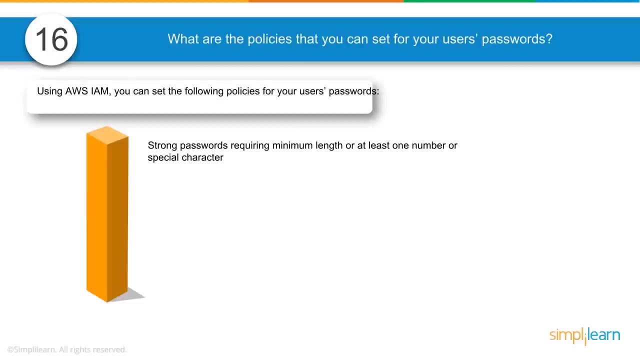 passwords, resetting the password. There are a few things we could do with IAM And finally, we can create policies that actually grants access to AWS services and resources. Another question you will see is: what are the policies that you can set for your user's password? So 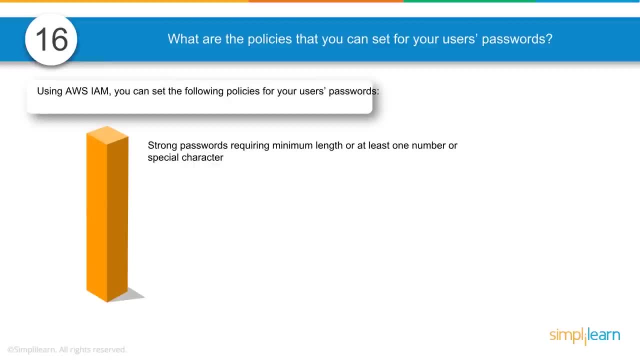 some of the policies that we can set for the user password is the minimum length, or you know the complexity of the password- by at least having one number or one special characters in the password. So that's one, And then the requirement of a specific character types, including, you know. 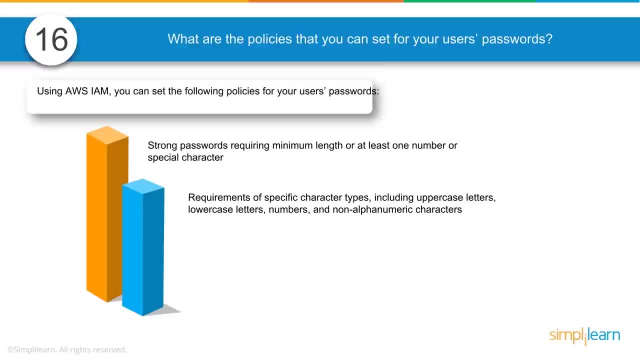 uppercase, lowercase, number and non-alphabetic characters. So it becomes very hard for somebody else to guess what the password would be and try to hack them. So we can set at the length of the password, we can set the complexity in the password And then we can set. 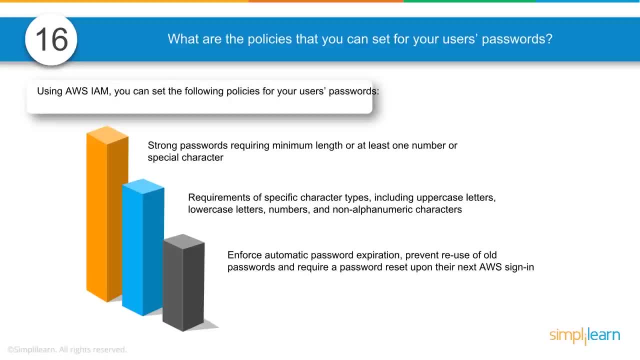 an automatic expiration of the password, So after a certain time the user is forced to create a new password. So the password is not stale, old and easy to guess in the environment And we can also set settings like the user should contact the admin, I mean when the password is about to. 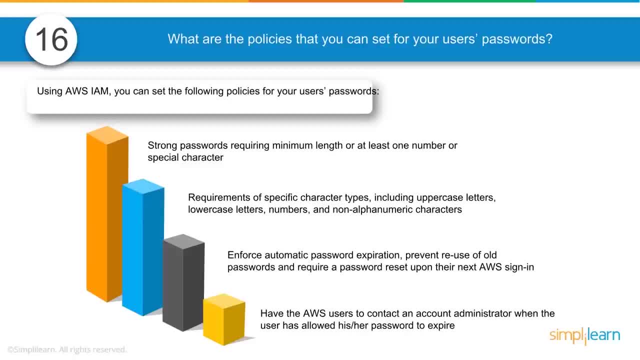 expire. So you know, you can get a hold of how the user is setting their password. is it having good complexity in it, is it meeting company standards or there are few things that we can control and set for the users when the users are setting or recreating the password. Another 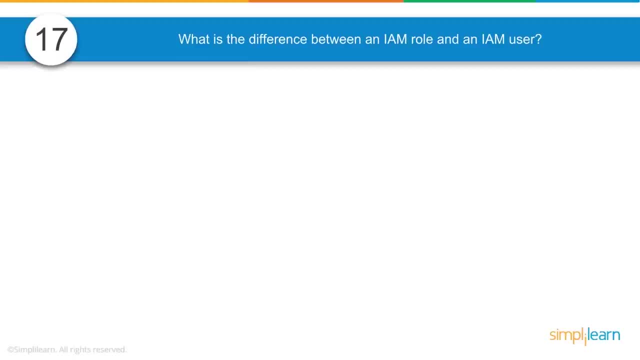 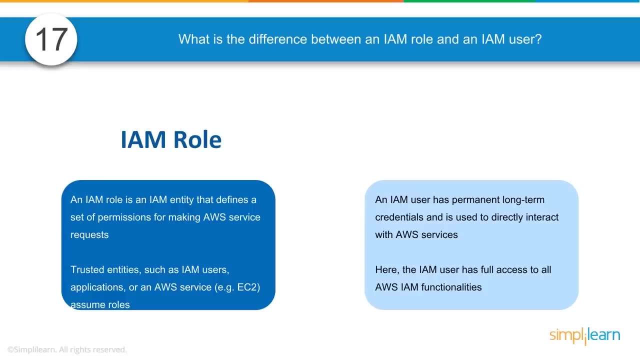 question that could be posted in an interview, so to understand your understanding of IAM, is: what's the difference between an IAM role and an IAM user? Let's talk about IAM user. Let's start small and then go big, or let's start simple and then talk about the complex one, The IAM user. 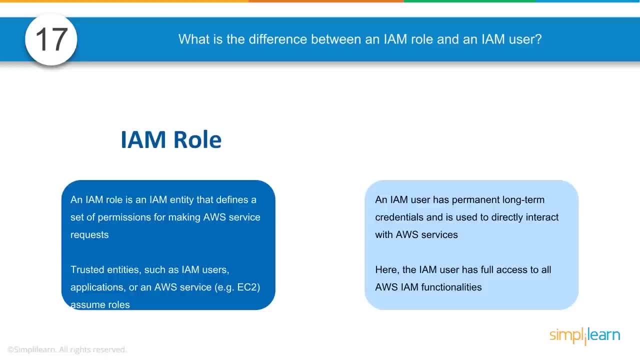 has a permanent, long-term credential and it's used to interact directly with AWS services and, on the other hand, IAM role is an IAM entity that defines a set of permissions for making AWS service request. So IAM user is an permanent credential and role are temporary credentials and IAM user 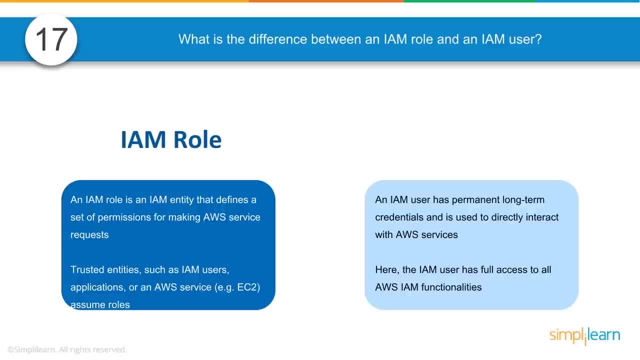 has full access to all AWS IAM functionalities and with role, trusted entities such as IAM users, application or AWS services assume the role. So when an IAM user is given a permission, you know it sticks within the IAM user. but with roles we can give. permissions to applications we can give. 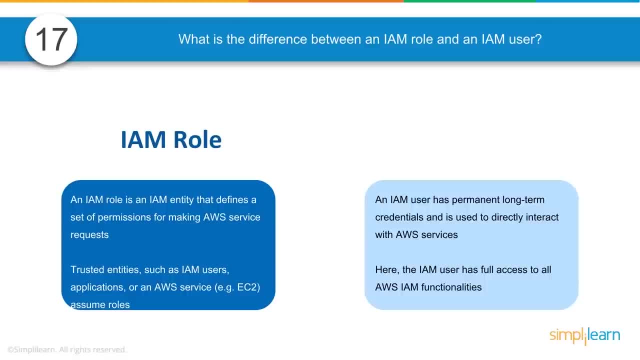 permissions to users in the same account. in a different account, the corporate ID- we can give permissions to EC2, S3, RDS, VPC and lot more. Role is wide and IAM user is is not so wide. you know it's very constrained only for that IAM user. Let's talk about managed. 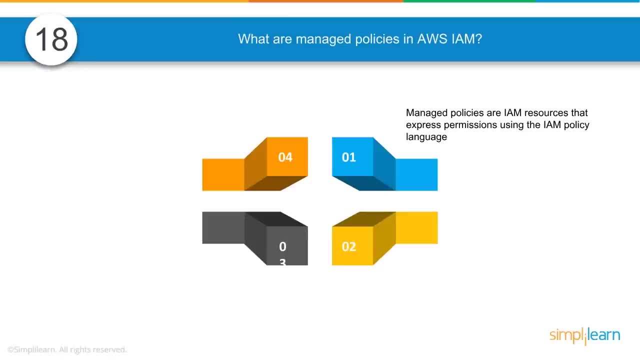 policies in AWS Managed policies. there are two types, you know: customer managed and Amazon managed. So managed policies are IAM resources that express permissions using the IAM policy language. Now we can create policies, edit them, manage them. manage them separately from the IAM. 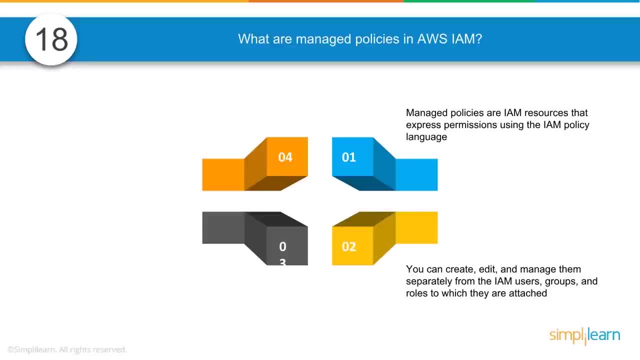 user group and roles which they are attached to the IAM user. So we can create policies, edit them, manage them separately from the IAM user group and roles which they are attached to the IAM user. So they are something that we can do to managed policies if it is customer managed And we can. 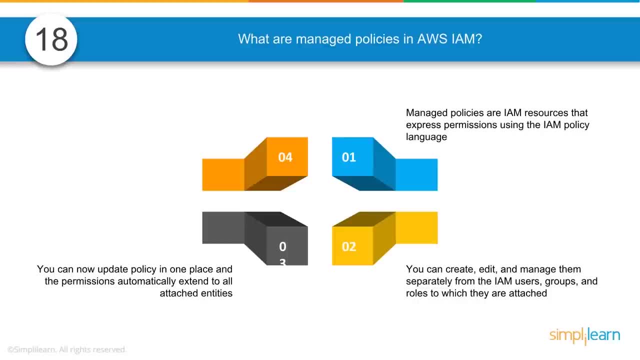 now update policy in one place and the permissions automatically extend to all the attached entries. So I can have like three services. four services point to a particular policy and if I edit that particular policy it's going to reflect on those three or four services. So anything that I allow. 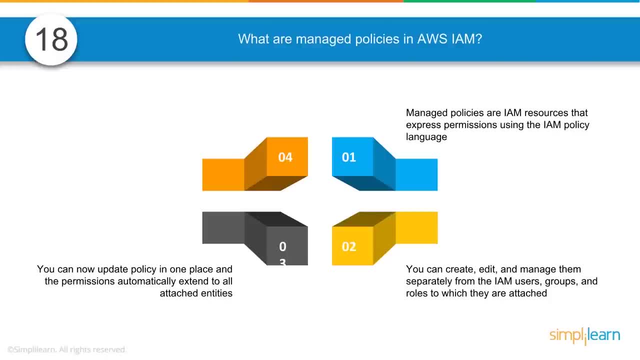 is going to be allowed for those four services. Anything that I denied is going to be denied for the four services. Imagine what would be with a four services So I can have a four services without the IAM managed policy. We'll have to go and specifically allow deny on those different. 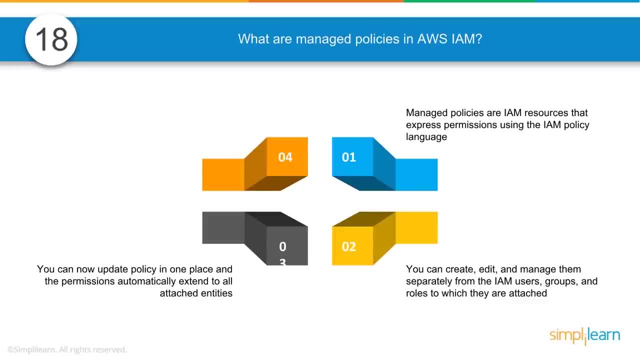 instances four or five times, depending on the number of instances that we have. So, like I said, there are two types of managed policies. One is managed by us, which is customer managed policies, and then the other is managed by AWS, which is AWS managed policy. This question, can you give an? 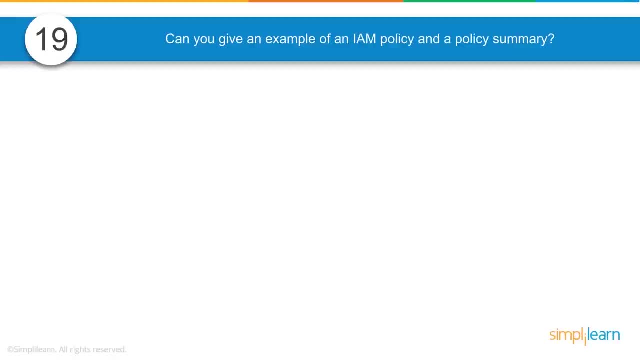 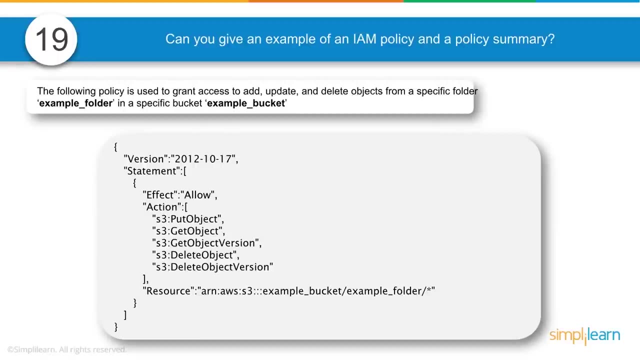 example of an IAM policy and a policy summary. This is actually to test how well versed are you with the AWS content. So let's say you have a policy and you have a policy and you have a policy console. The answer to that question is: look at the following policy. This policy is used to grant. 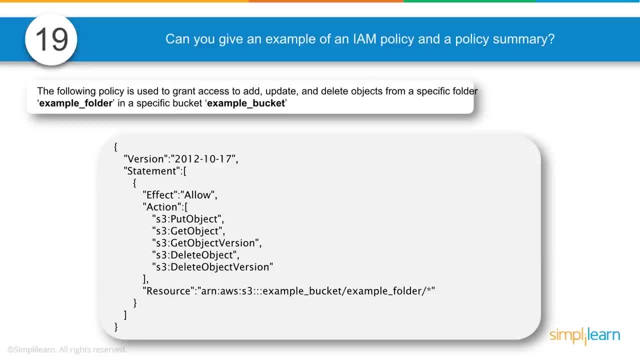 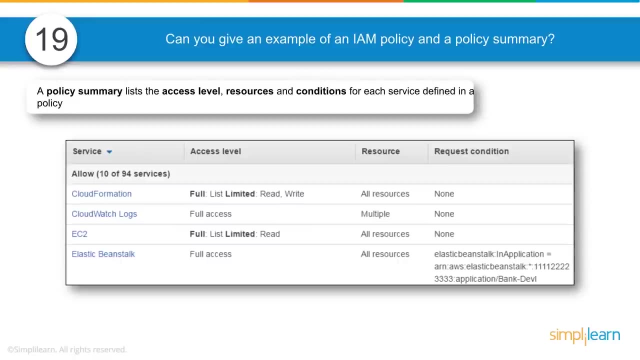 access to add, update and delete objects from a specific folder. Now, in this case, name of the folder is example folder and it's present in a bucket called example bucket. So this is an IAM policy. On the other hand, the policy summary is a list of access level, resource and conditions. 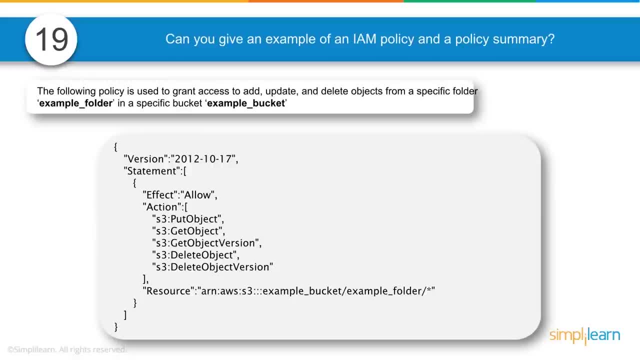 for each service defined in a policy. So IAM policy is all about one person. one person one particular resource, and the policy summary is all about multiple resources. With IAM policy it was only talking about S3 bucket and one particular S3 bucket. Here it talks about cloud formation. 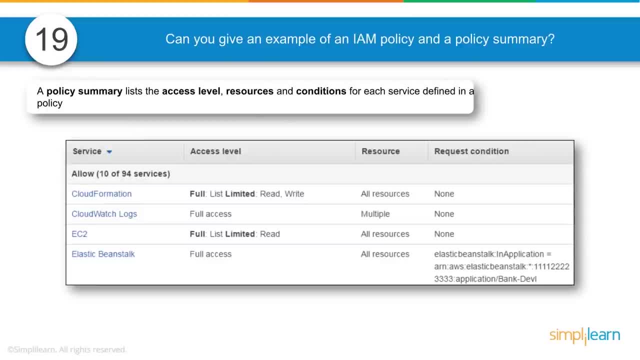 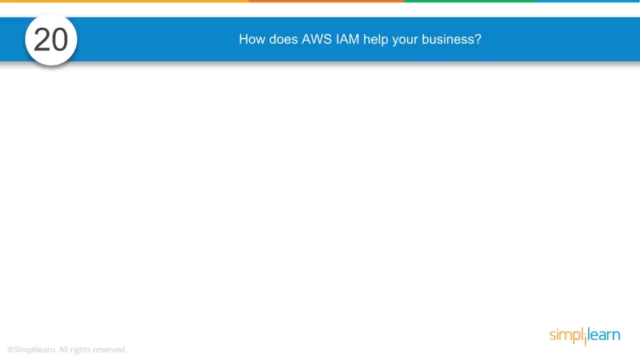 template, cloud watch logs, EC2, elastic beanstalk services- Summary summary of resources and the permissions and policies attached to them. That's what policy summary is all about. Another question could be like this: What's the use case of IAM and how does IAM help your business? 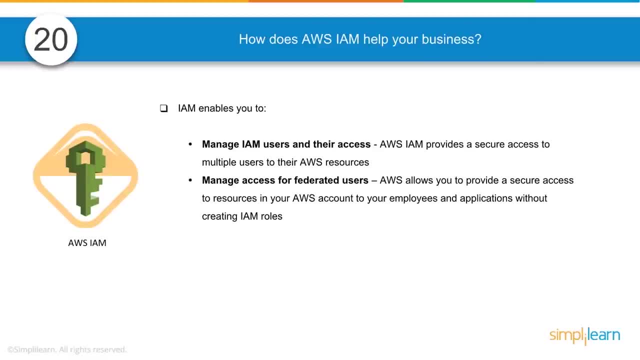 Now, two important or primary work of IAM is to help us manage IAM users and their access. It provides secure access to multiple users to their appropriate AWS resources. So that's one it does. And the second thing it does is manage access for federated users- Federated users or non-IAM users- and through 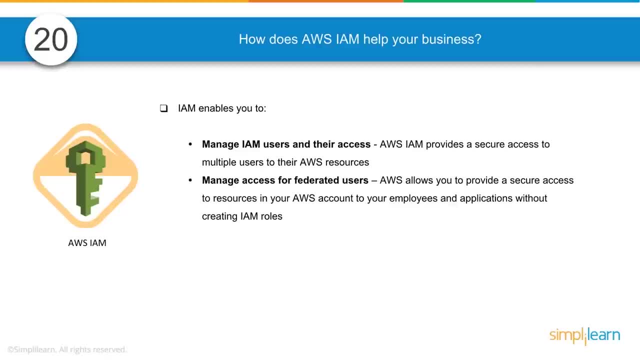 IAM. we can actually allow and provide a secure access to resources in our AWS account to our employees without the IAM user. Now they could be authenticated using the active directory. They could be authenticated using the Facebook credential, Google credential, Amazon credential and a couple. 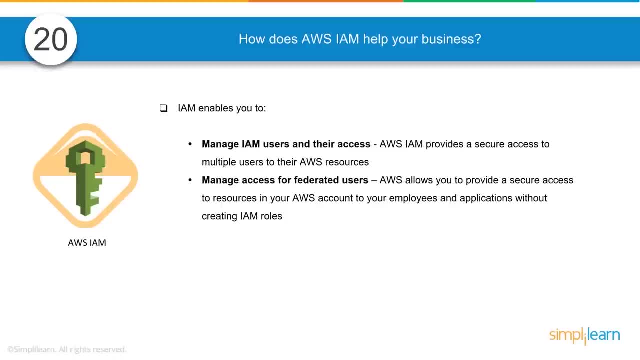 of other credentials, third-party identity management, So we could actually trust them and we could give them access to our account based on the trust relationship that we have built with the other identity systems. So two things: One is manage users and their access for manage IAM user and their access in our AWS environment. And second is manage 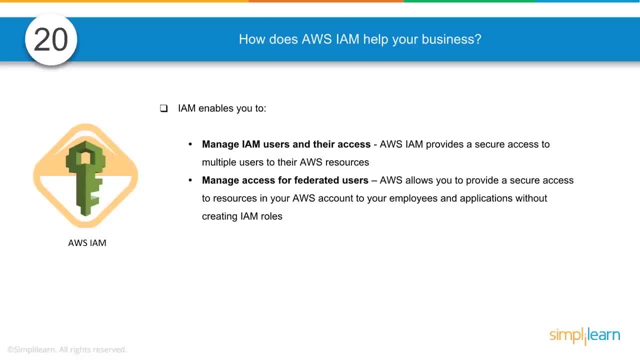 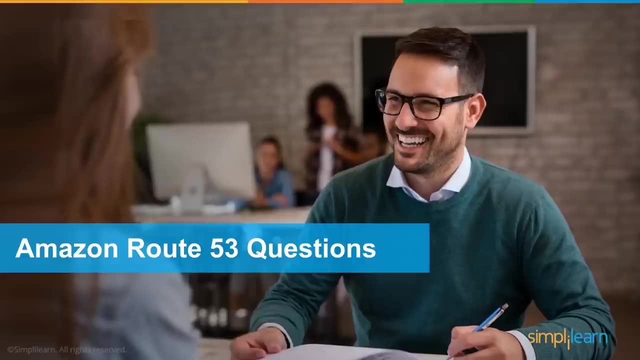 access for federated users who are non-IAM users. And, more importantly, IAM is a free service and with that will only be charged for the use of the resources, not for the IAM username and password that we create. All right, Let's now talk about some of the questions in Route 53.. One classic: 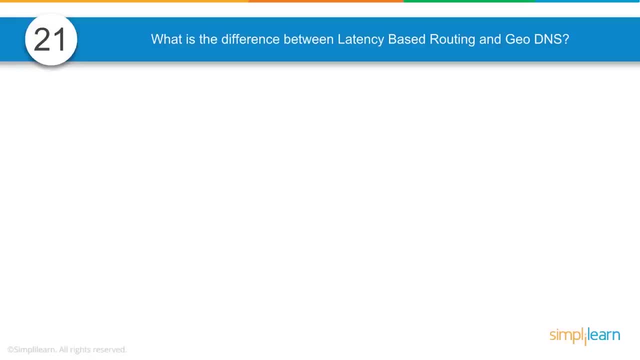 question that could be asked in an interview is: what is the difference between latency-based routing and GeoDNS or Geo-based DNS routing? Now, the Geo-based DNS routing takes routing decisions on the basis of the geographic location of the request And, on the other hand, the latency-based 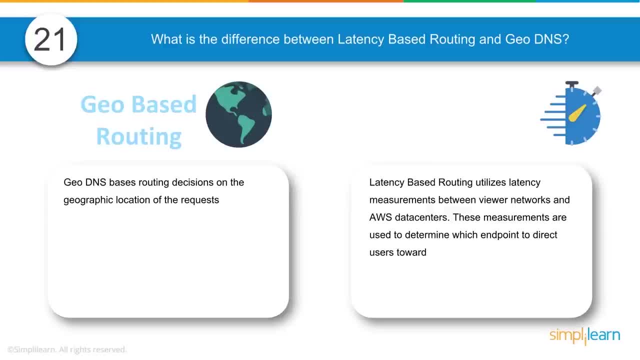 routing utilizes latency measurements between networks and data centers. Now, latency-based routing is used where you want to give your customers the lowest latency as possible. So that's when we would use latency-based routing And, on the other hand, a geo-based routing is when we want to. 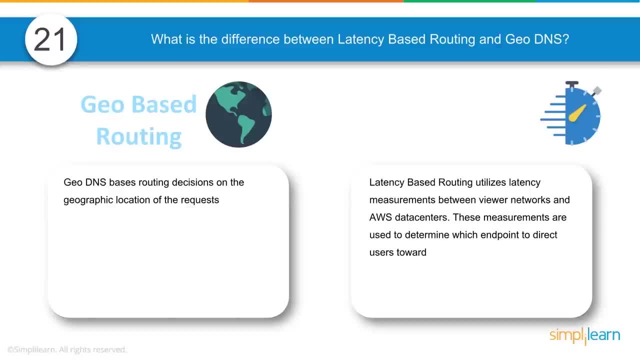 direct customers to different websites based on the country they are browsing from. You could have two different or three different websites for the same URL. Take Amazon, the shopping website, for example, For example, when we go to Amazon, the shopping website, for example, when we go to Amazon. 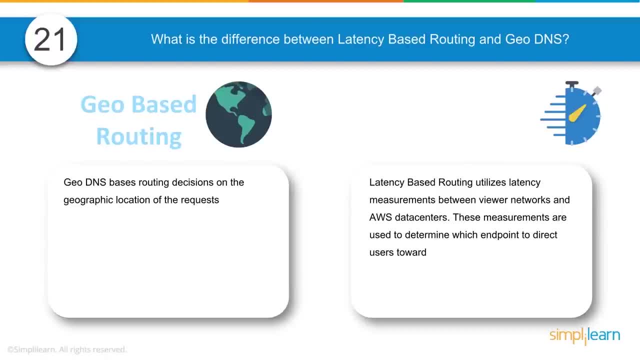 when we go to amazoncom from in the us, it directs us to the us web page where the products are different, the currency is different, right and the flag and and a couple of other advertisements that shows up are different. and when we go to amazoncom from india, it gets directed to the amazoncom 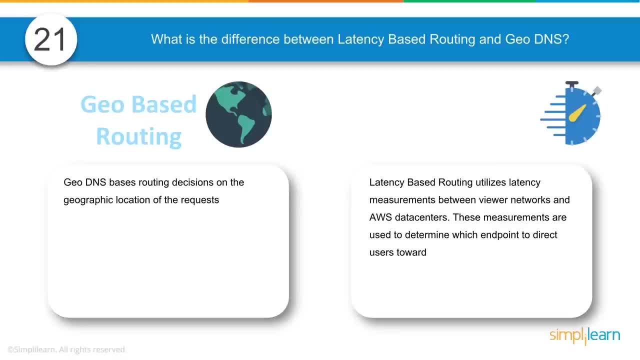 indian site where, again, the currency, the product and the advertisements- they're all different right. so depending on the country they're trying to browse, if you want to direct customers to two or three different websites, we would use a geo-based routing. another use case of geo-based 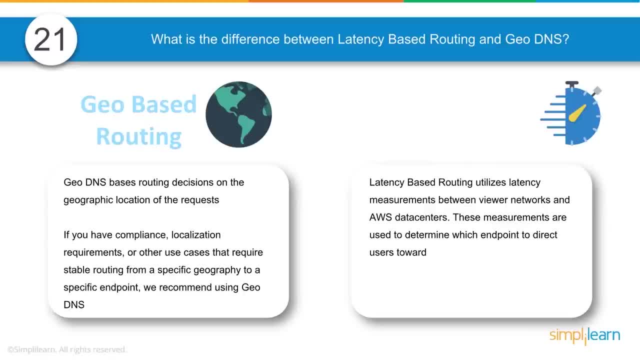 routing is if you have a compliance that you should handle all the dns requests, or if you should handle all the uh requests you know from a country within the country, then you would do geo-based routing. now you wouldn't direct the customer to a server which is in another country. 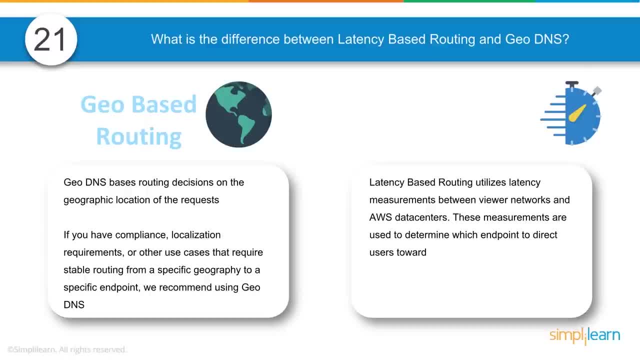 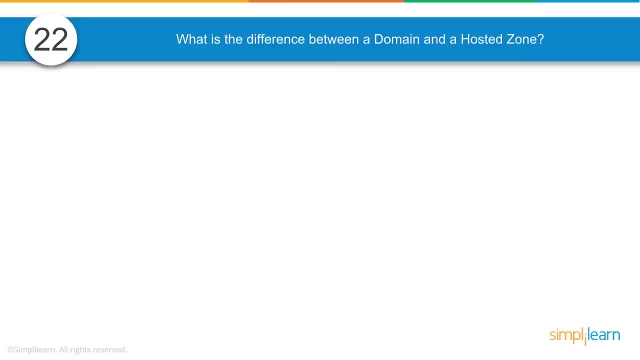 right, you would direct the customer to a server which is very local to them. that's another use case of geo-based routing and, like i said, for latency based routing, the whole goal or aim is to achieve minimum end user latency. if you are hired for the architect role and if that requires working, 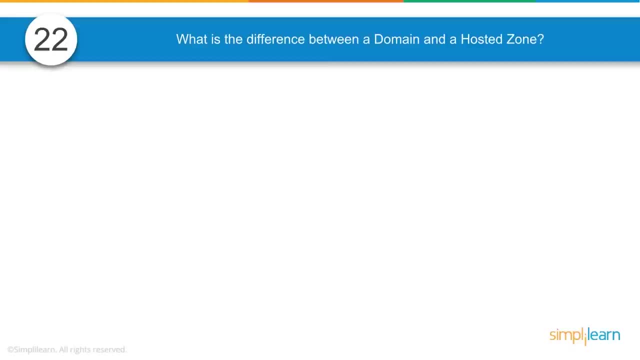 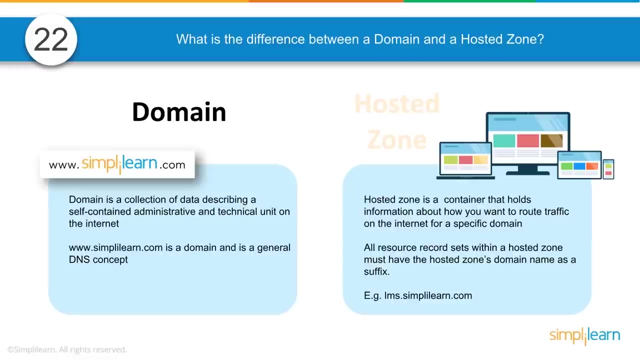 lot on the dns, then you could be posted with this question: what is the difference between domain and a hosted zone? a domain is actually a collection of data describing a self-contained administrative and technical unit on the internet, right? so, for example, you know, simplylearncom is actually a domain. on the other hand, hosted zone is actually an container that holds information. 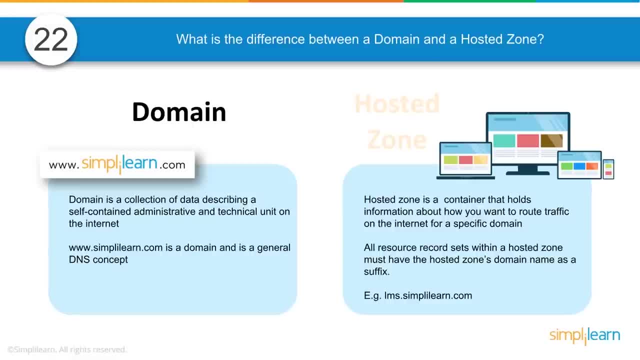 about how you want to route traffic on the internet to a specific domain. for example, lmssimplylearncom is an hosted zone whereas a simplylearncom is an domain. so in other words, in hosted zone you would see the domain name plus an upload link where you will get have the name of the. 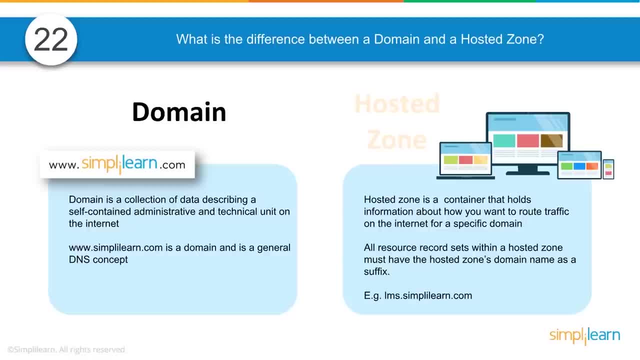 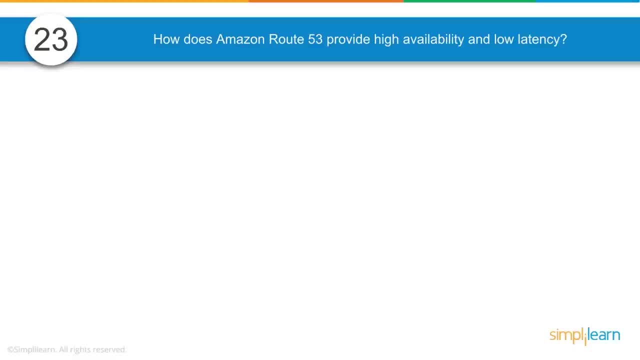 prefix to it. LMS is a prefix here, FTP is a prefix, Mailsimplylearncom is a prefix. So that's how you would see a prefix in hosted zones. Another classic question from Route 53 would be: how does Amazon Route 53 provide high availability and low latency The way Amazon Route 53 provides? 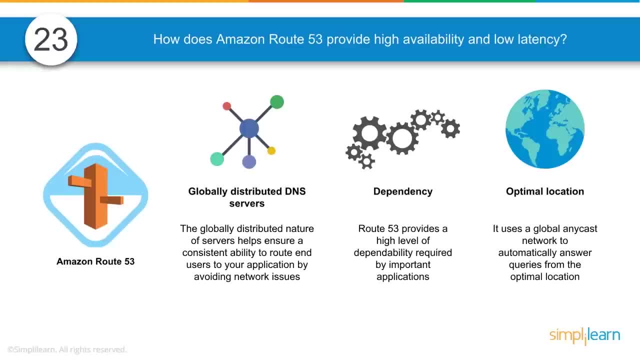 high availability and low latency is by globally distributed DNS service. Amazon is a global service and they have DNS services globally. Any customer doing a query from different parts of the world, they get to reach an DNS server which is very local to them, and that's how it provides. 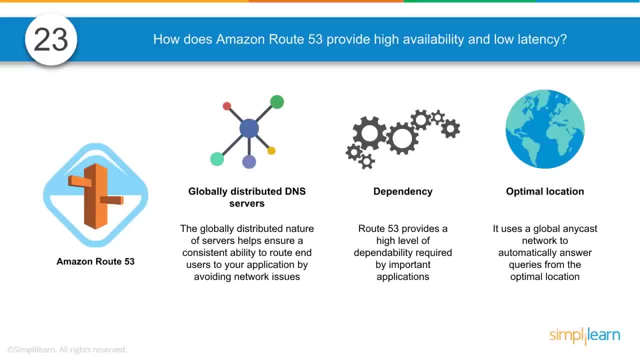 low latency. Now, this is not true with all the DNS providers. There are DNS providers who are very local to a country, who are very local to a continent, So they don't- they generally don't- provide low latency service, right? It's always high latency. It's low latency for local users. 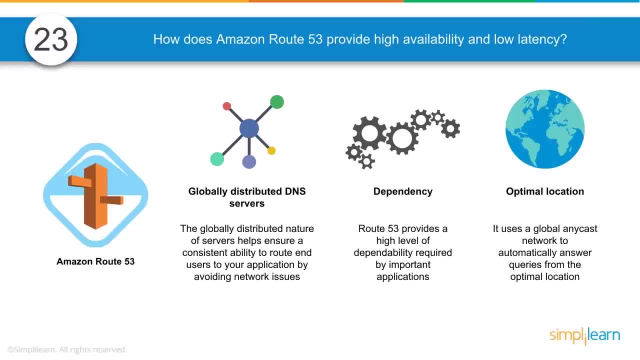 but anybody browsing from a different country or a different continent. it's going to be high latency for them, But that's not again true with Amazon. Amazon is a globally distributed DNS provider. It has DNS service global wide And, like I said, it has optimal location. It has got a. 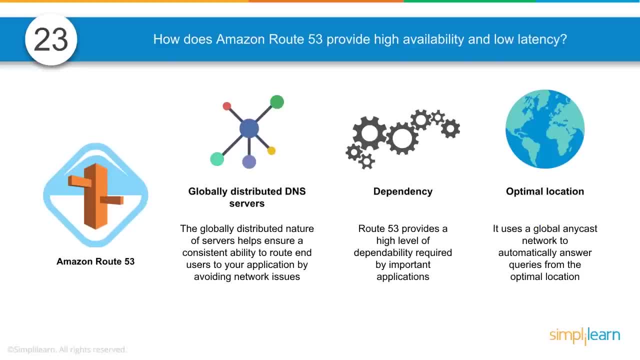 global service, or in other words, it has got servers around the globe, different parts in the globe, and that's how they are able to provide high availability. And because it's not running on just one server, but on many servers, they provide high availability and low latency. If the 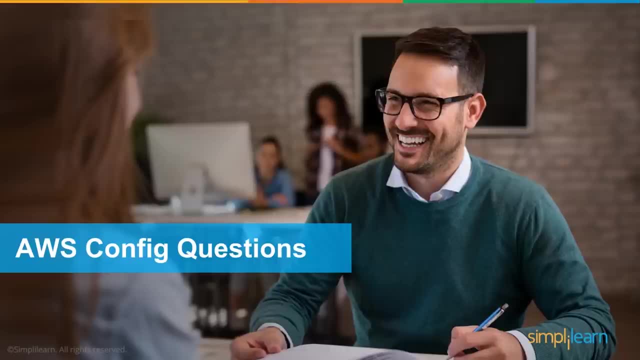 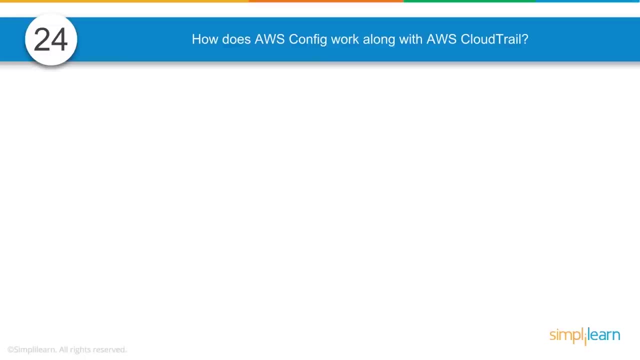 environment that you're going to work on is going to take a lot of configuration backups, environmental backups. then you can expect questions in AWS config. A classic question would be: how does AWS config work along with AWS CloudTrail? AWS CloudTrail actually records user. 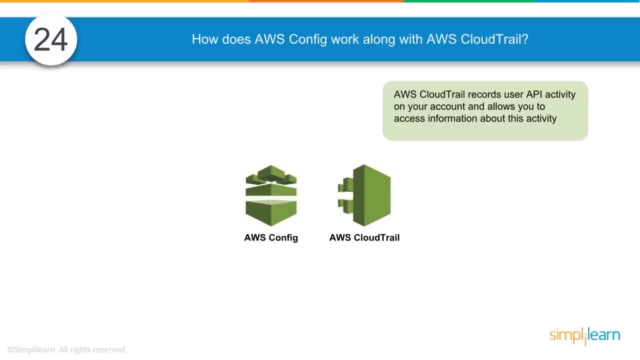 API activity on the account and you know any HTTP, HTTPS access or any, any sort of access. you know that's made it to the cloud environment. that's recorded in the CloudTrail. In other words, any API calls, the time is recorded, the type of call is recorded And what was the response given. 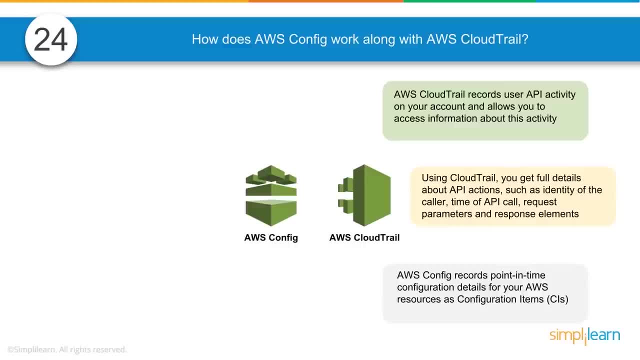 Was it a failure? Was it successful? They also get recorded in CloudTrail. It's actually a log. It actually records the activity in your cloud environment. On the other hand, config is an a point in time configuration details of your resources, For example, at a given. 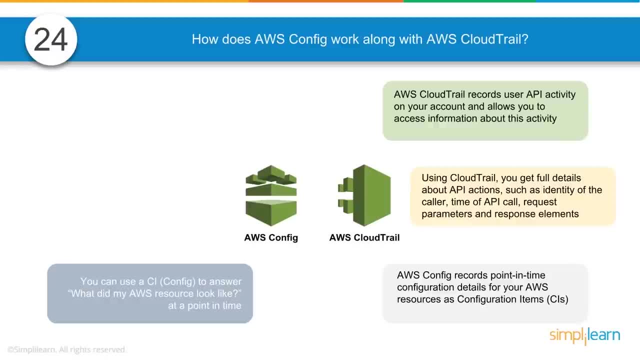 point. what are all the resources that were present in my environment? What are all the resources or what are the configurations in those resources at a given point? They get captured in AWS config, All right. so with that information you can always answer the question: what did my 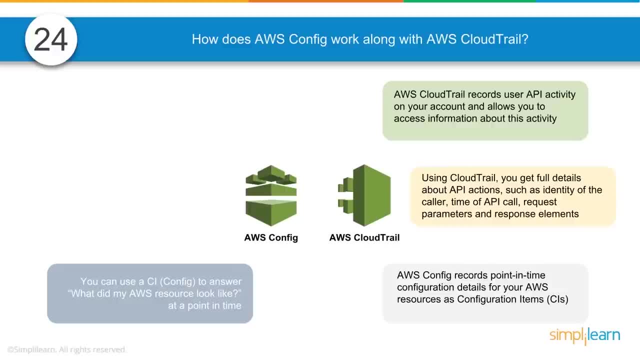 AWS resource look like at a given point in time. That question gets answered when we use AWS config. On the other hand, with CloudTrail you can answer the question. I mean by looking at the CloudTrail or with the help of trail, you can easily answer the question. who made an apa call to modify this resource? that's answered. 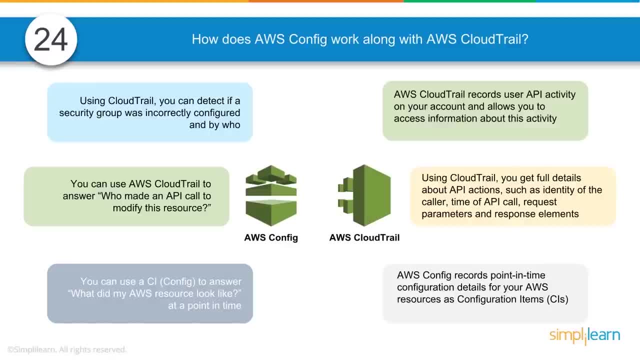 by cloud trail and with the cloud trail we can detect if a security group was incorrectly configured and who did that configuration. let's say that happened to be in downtime and you want to identify. let's say there happened to be a downtime and you want to identify who made that. 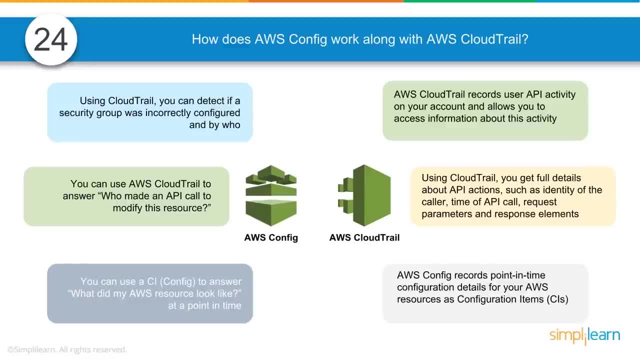 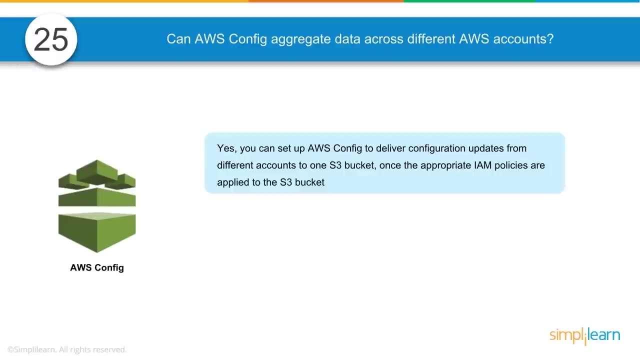 change in the environment. you can simply look at cloud trail and find out who made the change. and if you want to look at how the environment looked like before the change, you can always look at aws config. can aws configure or aws config aggregate data across different aws accounts? yes, it can. 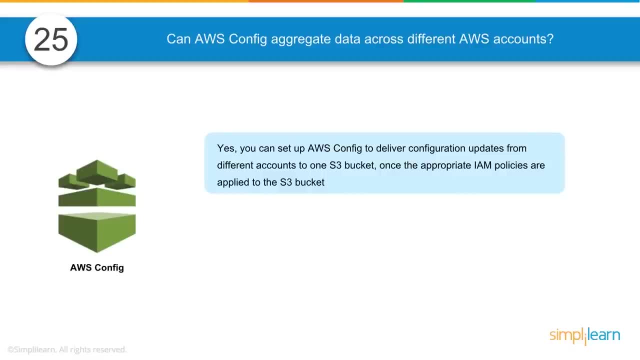 now, this question is actually to test whether you have used aws config or not. i know some of the services are very local, is it? some of these services are availability zone specific, some of them are regional specific and some of them are global services and amazon. and though some of the 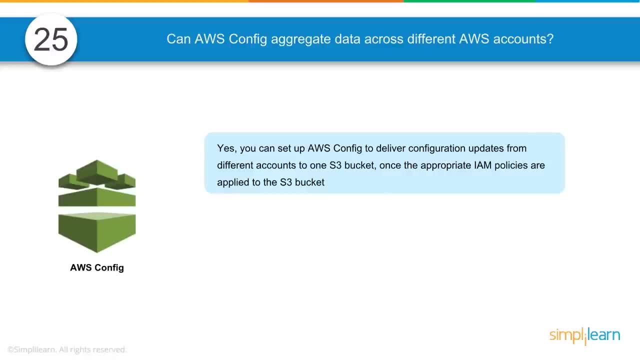 services are very homophobic, also have doors in most versions of amazon. we do consider our skills services or region services. you still can do some changes, you know, add some configuration to it and collect regional data in it. for example, s3 is a regional service, but still you can collect. 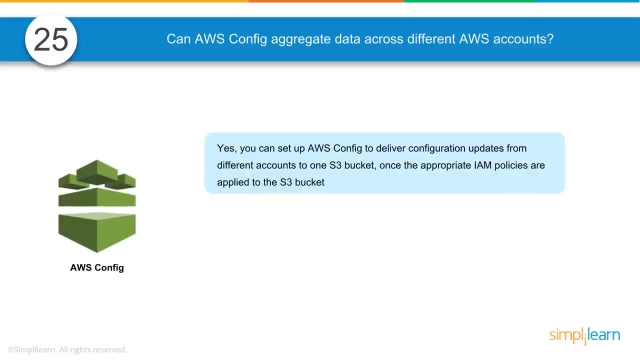 logs from all other regions into an s3 bucket in one particular region. that's possible and cloud trail is an cloud watch is an regional service but still you can, with some changes to it, with some adding permissions to it. you can always monitor the cloud watch that belongs to cloud watch logs. 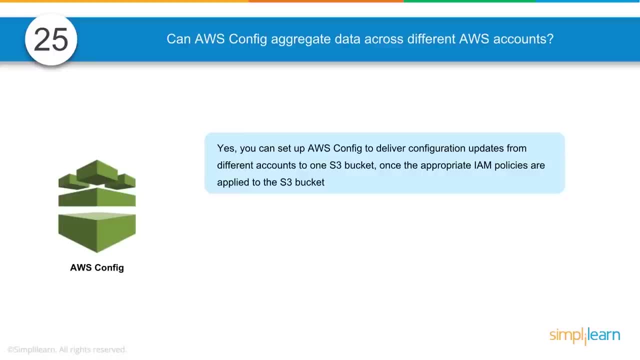 that belongs to other regions. you know they're not global by default, but you can do some changes and make it global. similarly, aws config is a service that's a region-based service, but still you can make it act globally. you can aggregate data across a different region and different 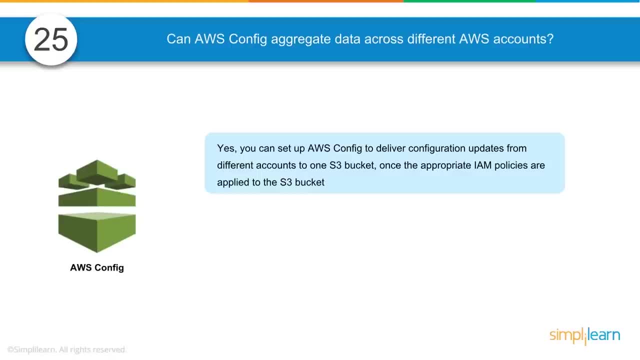 accounts in an aws config and deliver the updates from different accounts to one s3 bucket and can access it from there. aws config also works or integrates seamless with sns topic, so you know anytime there is a change, anytime a new data gets collected, you can always notify yourself or notify a group of people about the new log or the new config or new edit. 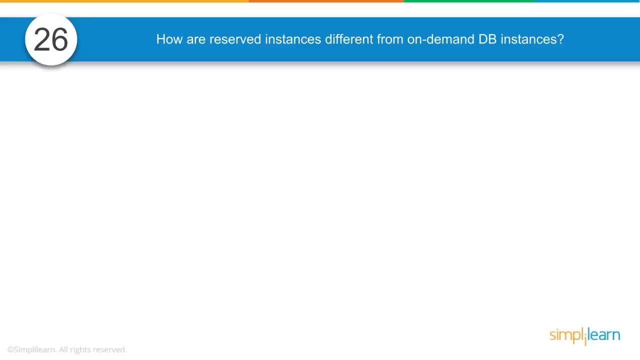 that happened in the environment. let's look at some of the database questions. you know database should be running on reserved instances. so, whether you know that fact or not, the interviewer wants to understand how well you know that fact by asking this question: how are reserved instances different from on-demand db instances? reserved instances and on-demand instances are exactly the. 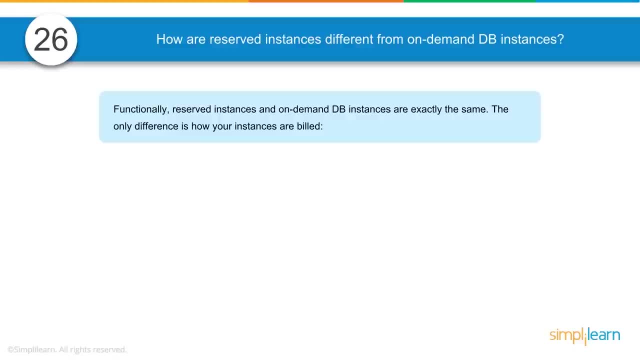 same when it comes to their function, but they only differ based on how they are built. reserved instances are purchased for one year or three year reservation and in return we get a very low per hour pricing because we're paying upfront. it's generally said that reserved instance is 75. 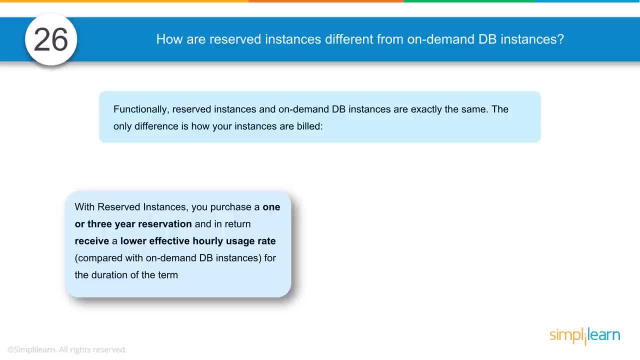 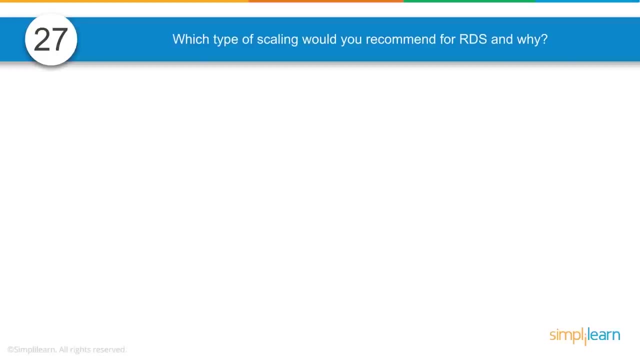 percentage cheaper than on-demand instance, and amazon gives you that benefit because you know you're committing for one year and sometimes you're paying in advance for the whole year. on the other hand, on-demand instances are built on an hourly hourly price. talking about auto scaling, how will 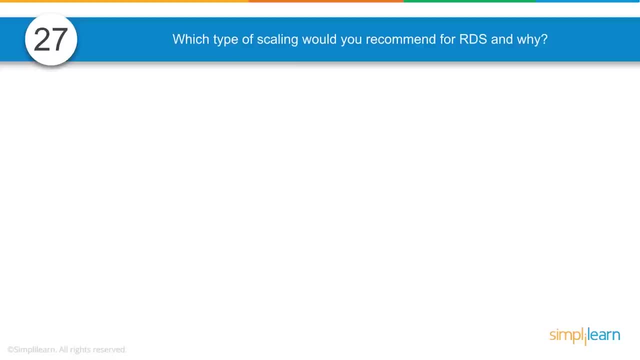 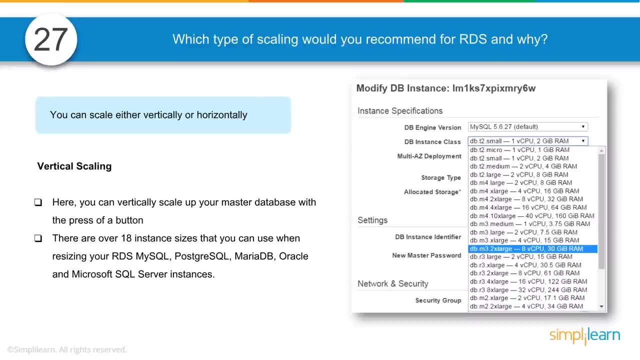 you understand the different types of auto scaling. the interviewer might ask this question: which type of scaling would you recommend for rds, and why the two types of scaling? as you would know now, vertical and horizontal? in vertical scaling, we can vertically scale up the master database with a couple of clicks right. so 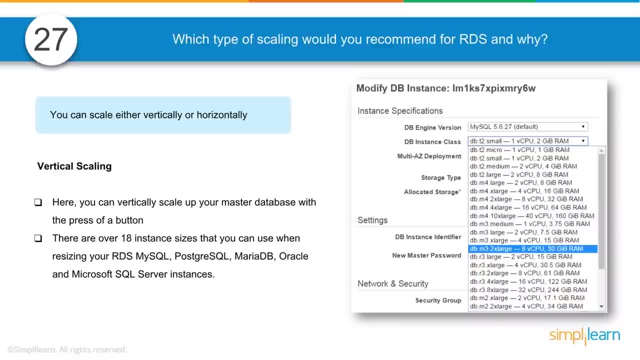 that's vertical scaling. vertical scaling is keeping the same node and making it bigger and bigger. if previously it was running on t2 micro, now we would like to run it on m3, two times large instance. previously it had one virtual cpu, one gigabit. now it's going to have eight virtual cpu and 30 gigabit. 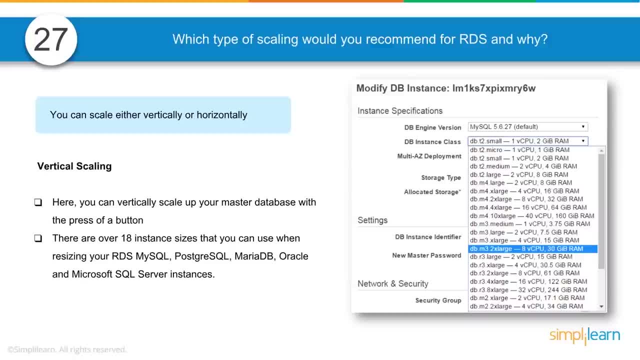 of ram. so that's vertical scaling. on the other hand, the horizontal scaling is adding more nodes to it. previously it was running on one vm, now it's going to run on two, three, ten vms. right, that's horizontal scaling. so database can only be scaled vertically, and there are 18. 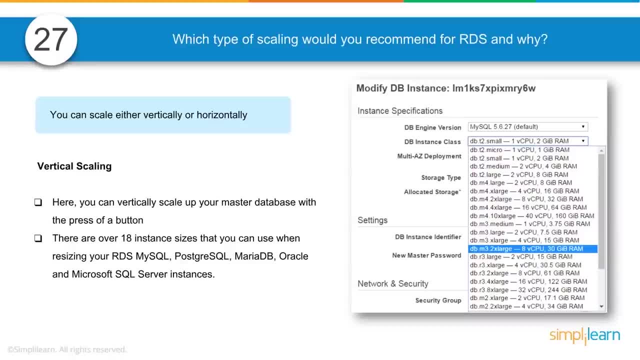 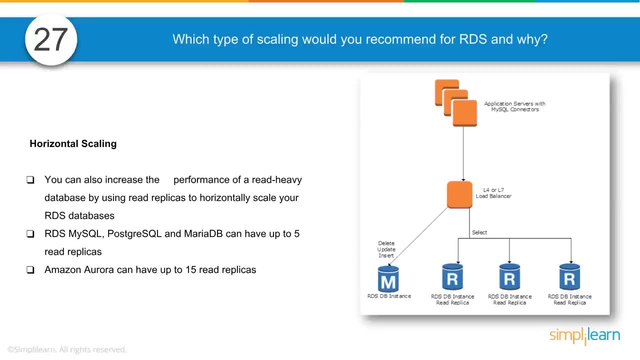 different types of instances. we can resize our rds2 right, so this is true for rds, mysql, postgres, sql, maria, db, oracle, microsoft sql servers. there are 18 type of instances we can vertically scale. on the other hand, horizontal scaling are good for replicas, so they are read-only replicas. we're not. 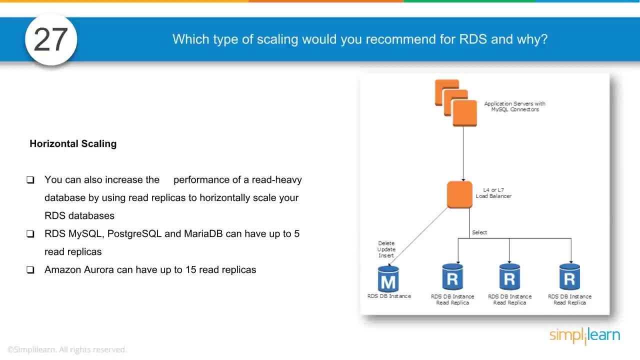 going to touch the master database. we're not going to touch the primary database, but i can do horizontal scaling only with amazon aurora and i can add additional read replicas. i can add up to 15 read replicas for amazon aurora and up to five read replicas for rds, mysql, postgres, sql and maria. 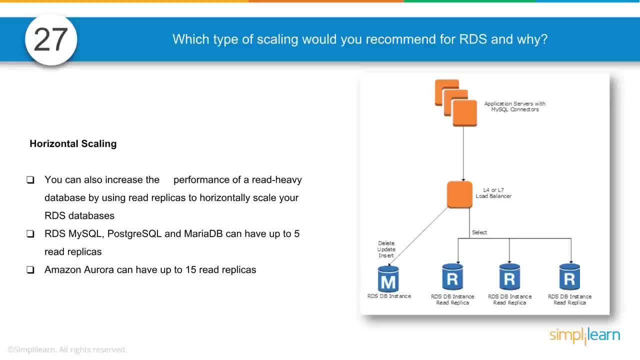 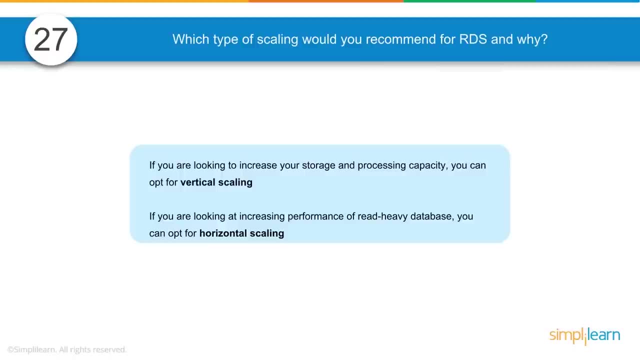 db instances and when we add replica, we are horizontally scaling, adding more nodes. right read, only nodes, so that's horizontal scaling. so how do you really decide between vertical and horizontal scaling? if you're looking in to increase the storage and the processing capacity, we'll have to do a vertical scaling. if you're looking at increasing the performance, or of the 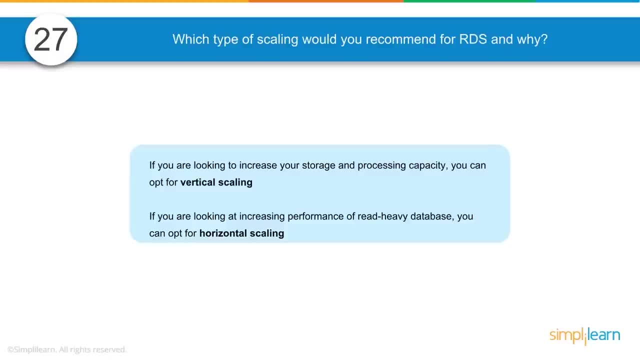 read heavy database. we need to be looking for horizontal scaling or we need to be implementing horizontal scaling in our environment. still talking about database, this is another good question you can expect in the interview: what is the maintenance window and amazon rds: will your db instance be available? 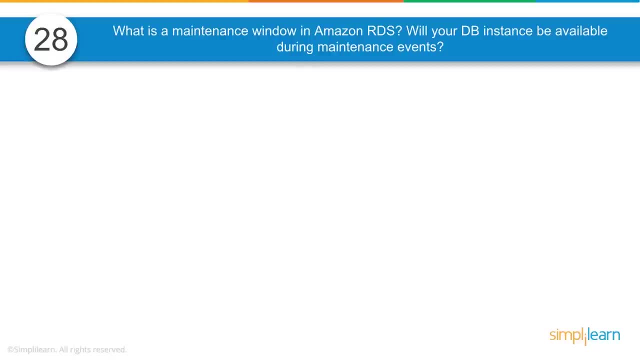 during the maintenance event. right, so this is really to test how well you have understood the sla, how well you have understood the amazon rds, the failover mechanism of amazon rds, stuff like that. so rds maintenance window: it lets you decide when a db instance modification. 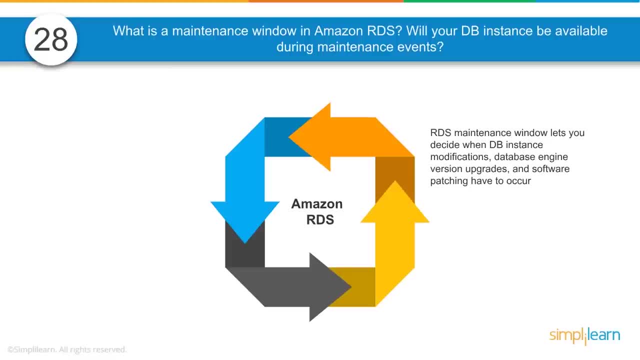 a database engine, upgrades or software patching has to occur and you you actually get to decide should it happen at 12 in the night or should it happen at afternoon, should it happen early in the morning, should it happen in the evening? you actually get to decide an automatic scheduling. 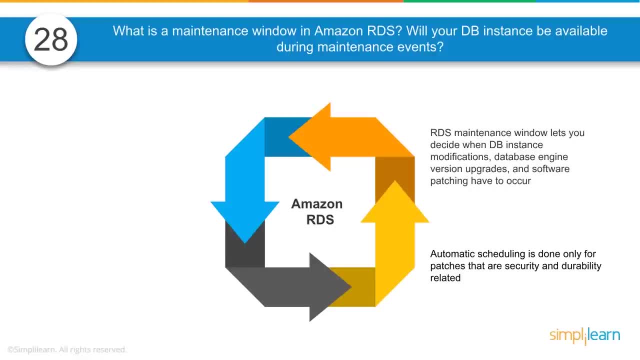 by amazon is done only for patches that are security and durability related. sometimes amazon takes down and does automatic scheduling. if you know if there is a need for a patch update, that is done. you can do that with the db instance. you can do that with the db instance. you can do that with. 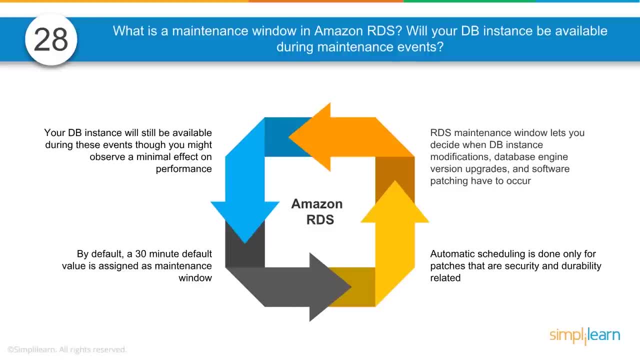 security and durability and by default the maintenance window is is for 30 minutes and the important point is the db instance will be available during that event because you're going to have primary and secondary right. so when that upgrade happens, amazon would shift the connection to the. 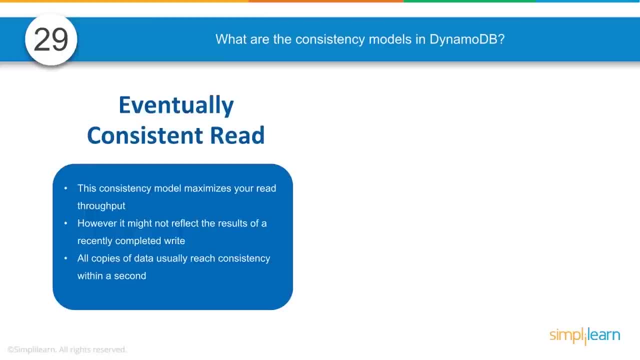 secondary, do the upgrade and then switch back to the primary. another classic question would be: what are the consistency models in dynamo db? in dynamo db, there is eventually a change in the eventual consistency. read this eventual consistency model. it actually maximizes your read throughput and 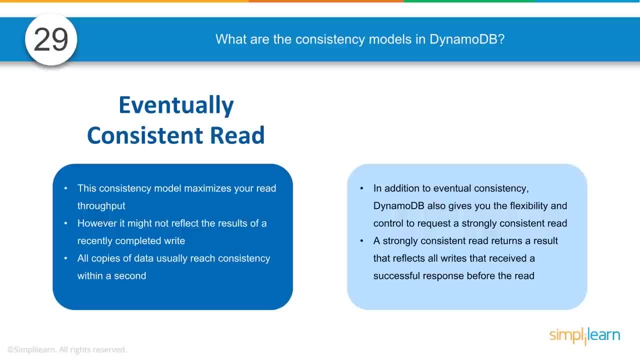 the best part with eventual consistency is: all copies of data reach consistency within a second and sometimes when you write and when you're, you know, trying to read immediately, chances that you you would still be reading the old data. that's eventual consistency. on the other hand, there is 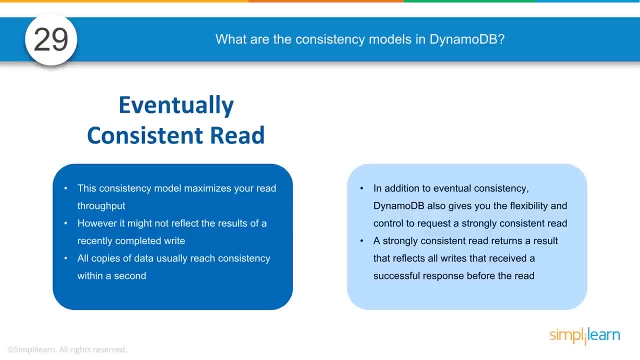 another consistency model called the strong consistency. you are strongly consistent. read where there is going to be a delay in writing the data. you know making sure the data is written in all places. but it guarantees one thing, that is, once you have done a write and then you're trying to do a read, it's going to make sure that it's going to. 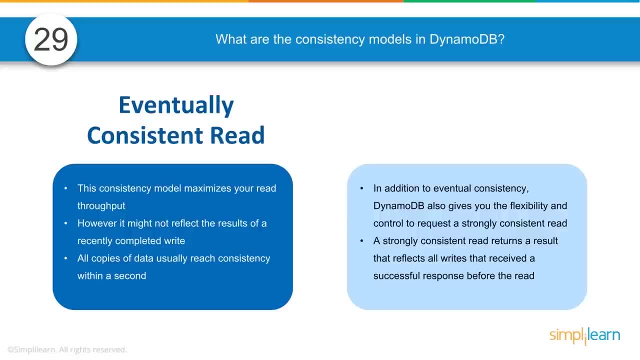 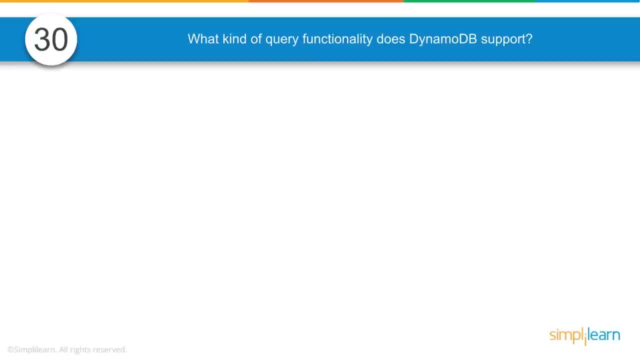 show you the updated data, not the old data. now you can be guaranteed of it, that it is going to show the updated data and not the old data. that's strongly consistent. still talking about database, talking about nosequel DynamoDB or NoSQL database, which is DynamoDB in Amazon- you could be asked this question. 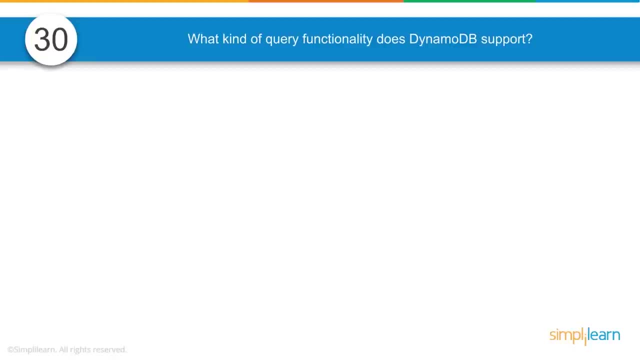 what kind of query functionality does DynamoDB support? DynamoDB supports get and put operation. DynamoDB supports or DynamoDB provides flexible querying by letting you query on non-primary key attributes using global secondary index and local secondary indexes. A primary key can be either a: 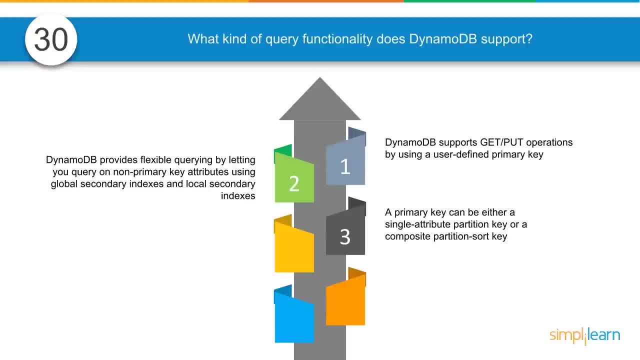 single attribute partition key or a composite partition sort key. In other words, DynamoDB indexes a composite partition sort key as a partition key element and a sort key element And by holding the partition key you know when doing a search or when doing a query. by holding, 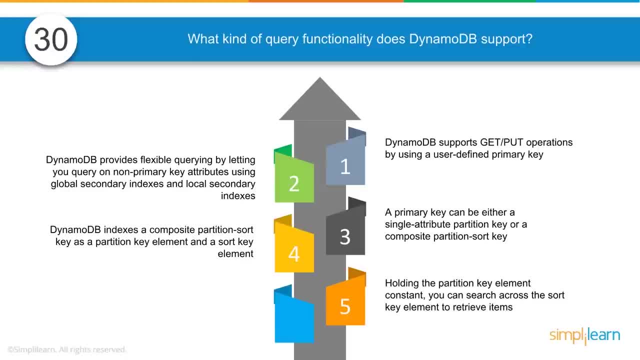 the partition key element constant. we can search across the sort key element to retrieve the other items in that table. And the composite partition sort key should be a combination of user ID, partition and a timestamp. So that's what the composite partition sort key is made of. Let's look at some. 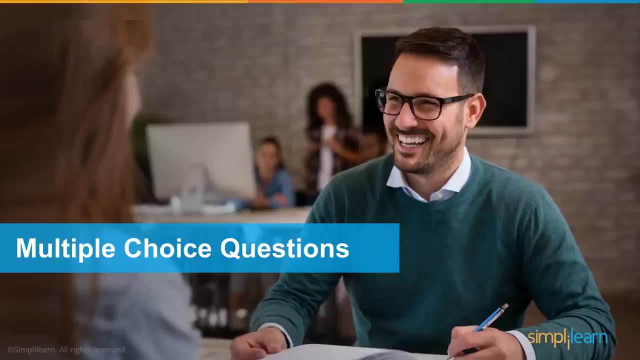 of the multiple choice questions. You know, sometimes some companies would have a written test or an MCQ type online test before they call you for the first level or before they call you for the second level. So these are some classical questions that companies asked or companies ask. 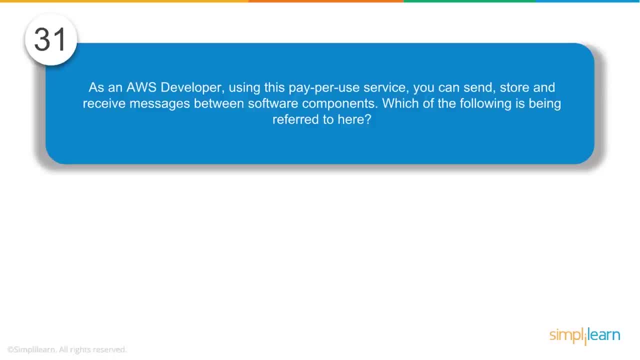 in their multiple choice online questions. Let's look at this question. As a developer, you can send, store and receive messages between software components. Which of the following is being referred here? Let's look at it right. We have AWS, step functions, Amazon, MQ, Amazon- simple. 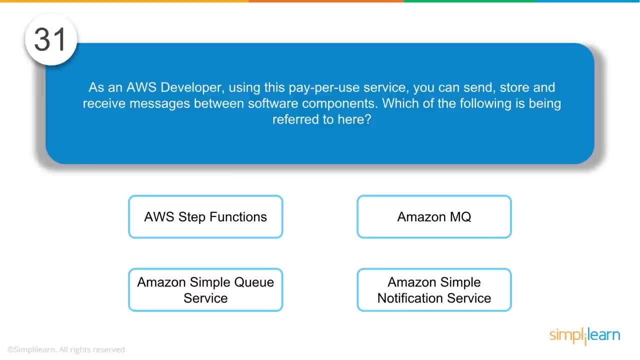 queue service- Amazon simple notification service. Let's read the question again As a developer using this pay-per-use service. so the service that we are looking for is a pay-per-use service. you can send, store and retrieve messages between two software components, kind of like a queue. 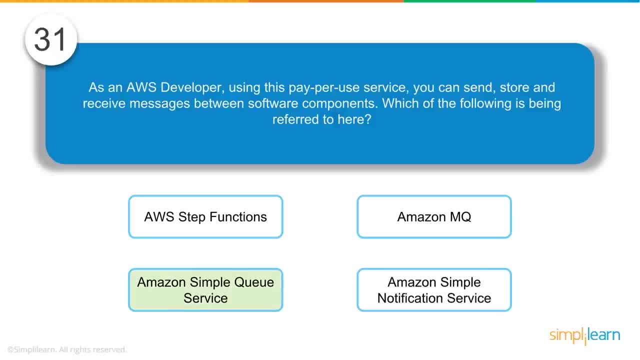 there. So what would be the reference? You can send, store and retrieve messages between two software components. So what would be the correct answer? It would be Amazon simple queue service. Now, Amazon simple queue service is the one that's used to decouple the environment, You know. 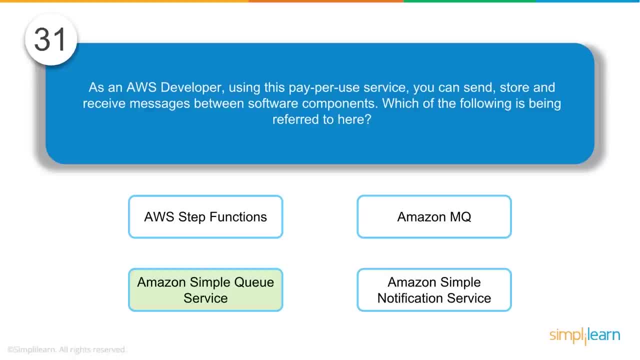 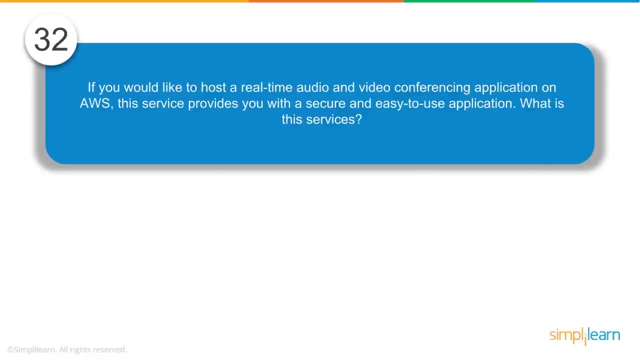 it breaks the tight coupling and then it introduces decoupling in that environment by providing a queue or by inserting a queue between two software components. Let's look at this other question: If you would like to host a real-time audio and video conferencing application on AWS, 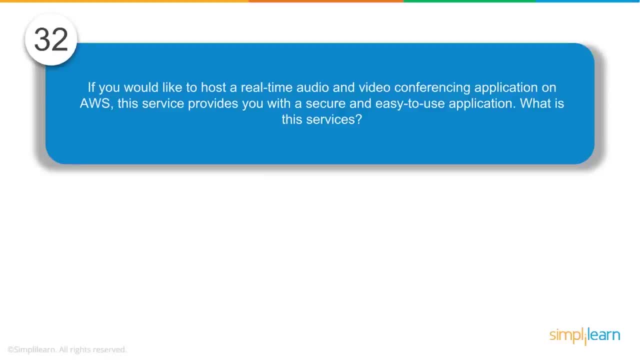 it's an audio and video conferencing application on AWS. This service provides you with a secure and easy to use application. what is this service? let's look at the options. they are: amazon chime, amazon workspace, amazon mq, amazon app stream you might tend to look at. 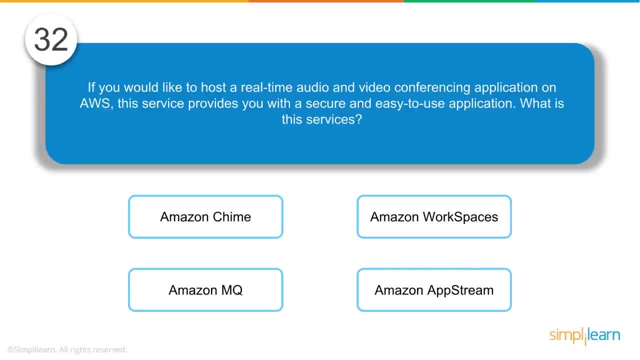 amazon app stream because it's real time and video conference, but it's actually for a different purpose. it's actually amazon chime that lets you create chat and create a chat board and then collaborate with the security of the aws services. so it lets you do the audio. it lets you do the. 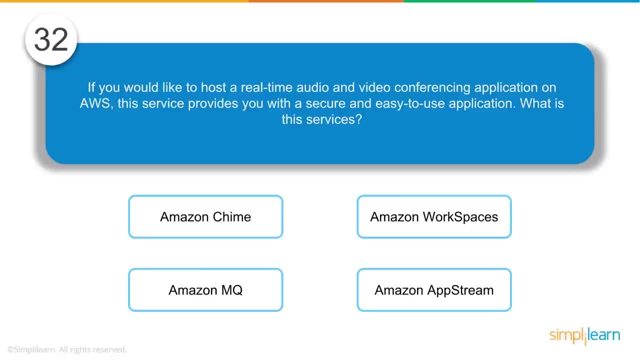 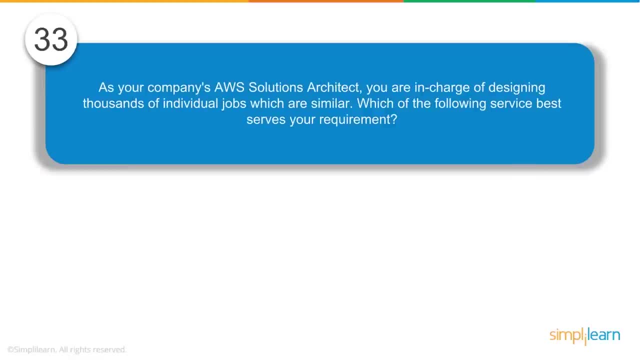 video conferencing, all supported by aws security features. it's actually amazon chime. let's look at this question. as your company's aws solution architect, you are in charge of designing thousands of individual jobs which are similar. which of the following service best serves your requirement? aws, ec2, auto scaling aws, snowball aws, fargate. 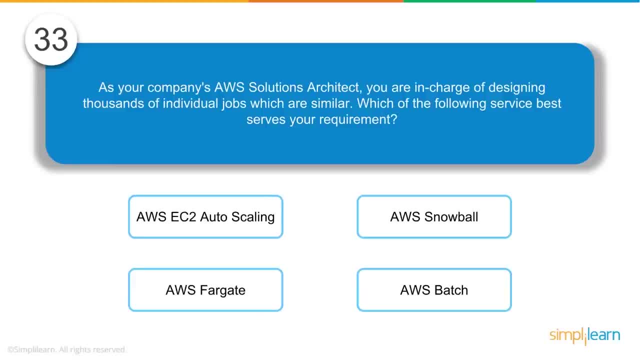 aws batch. let's read the question again. as your company's aws solution architect, you are in charge of designing thousands of individual jobs which are similar. it looks like it's batch service. let's look at the other options as well. aws snowball is actually an storage transport service, ec2 auto. 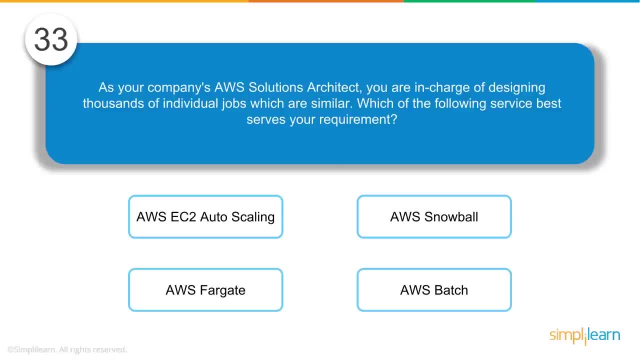 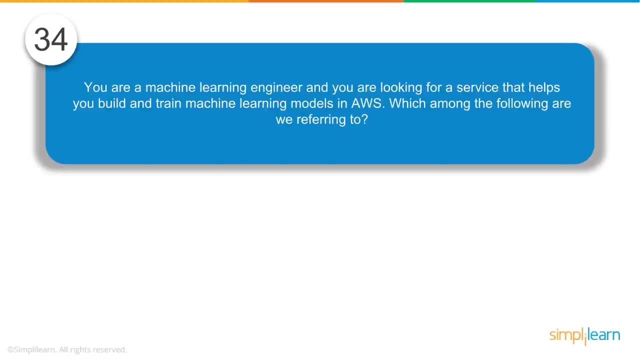 scaling is, you know, in introducing scalability and elasticity in the environment, and aws fargate is container services. aws batch is the one is being referred here that actually runs thousands of individual jobs which are similar aws batch. it's the right answer. let's look at the other one. you 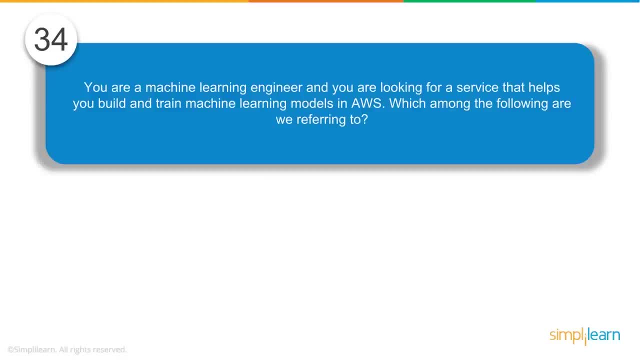 are a machine learning engineer and you're looking for a service that helps you build and train machine learning models in aws. which among the following are we referring to? so we have amazon sage maker and aws deep lens, amazon comprehend, aws device farm. let's read the question again: you are a machine learning engineer and you're looking. 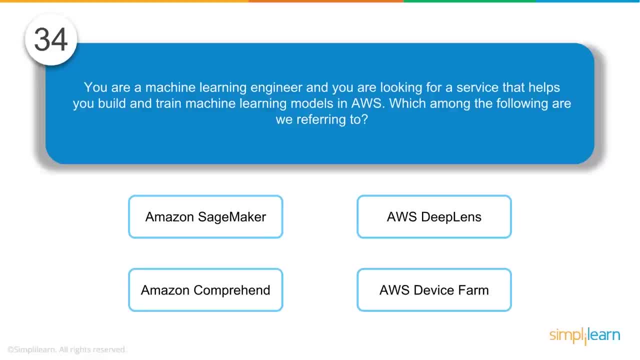 for a service that helps you build and train machine learning models in aws, which, among the following are referred here. the answer is sage maker. it provides every developer and data scientist with the ability to build, train and deploy mission learning models quickly. that's what sage maker does. now, for you to be familiar with you know the products i would recommend you. 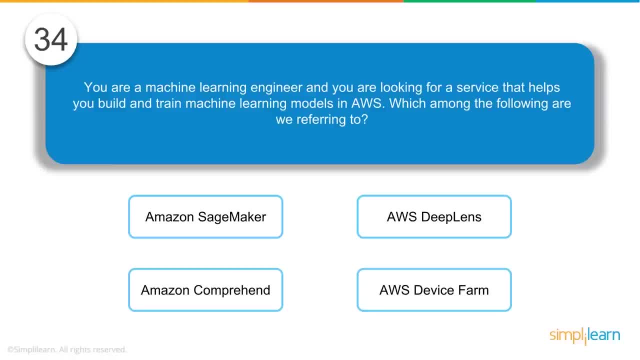 to you know. simply go through the product description. you know. there's one page available in amazon that explains all. the products are quick, neat and simple and that really helps you to be very familiar with you know what the product is all about and what it is capable of. you know, is it? 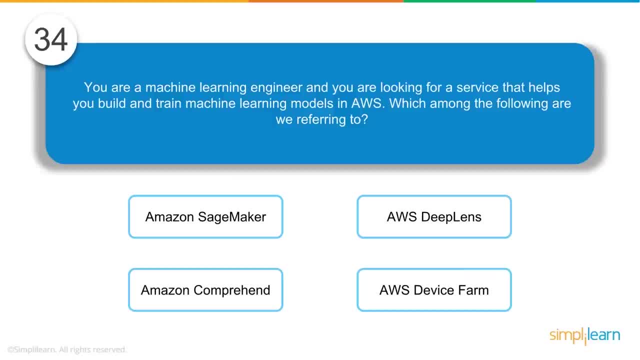 a db service? is it a machine learning service or is it a monitoring service? is it a developer service, stuff like that? so get that information, get that details before you attend an interview and that should really help to answer or face such questions with great confidence. so the 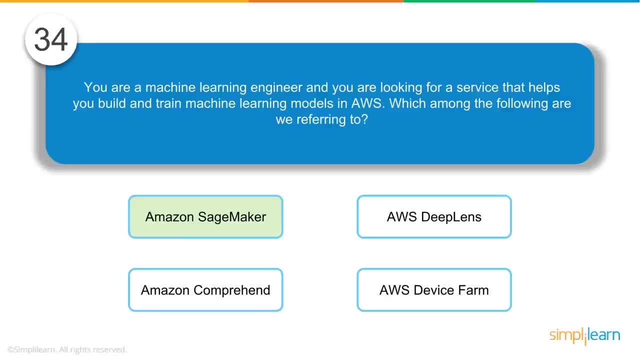 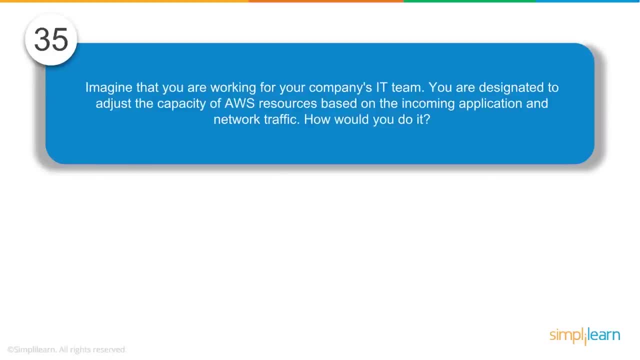 answer is amazon sage maker, because that's the one that provides developers and data scientists the ability to build a train and deploy mission learning models quickly as possible. all right, let's look at this one. let's say that you are working for your company's id team and you are 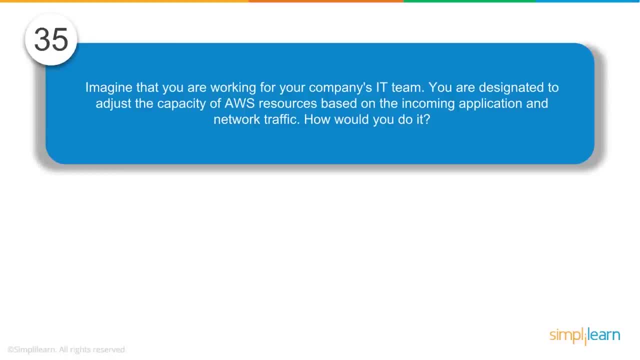 designated to adjust the capacity of the aws resource based on the incoming application and network traffic. how do you do it? so what's the service that's actually helps us to adjust the AWS resource based on the incoming application? Let's look at it: Amazon, VPC, Amazon IAM. 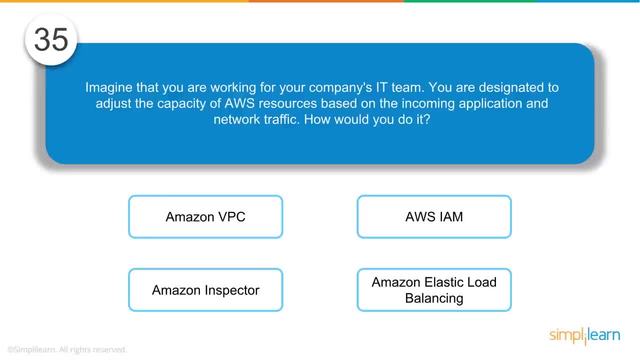 Amazon Inspector, Amazon Elastic Load Balancing, Amazon VPC is a networking service, Amazon IAM is an username password authentication. Amazon Inspector is a service that actually does security audit in our environment And Amazon Elastic Load Balancer is a service that helps in scalability. That's, in one way, indirectly, that helps in increasing the availability of. 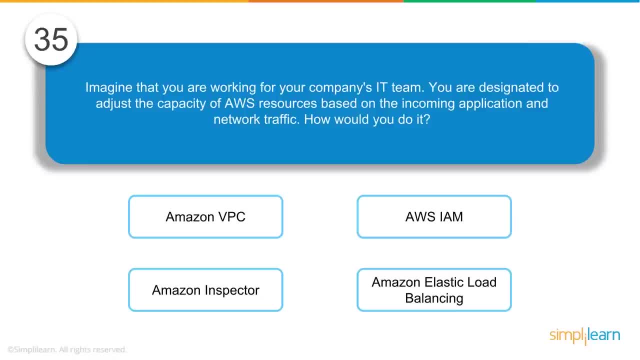 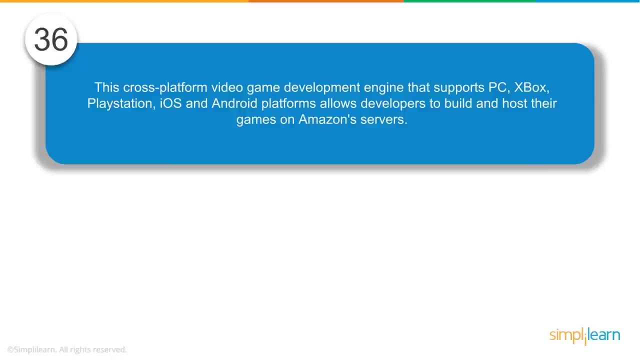 the application And monitoring it, monitoring how much requests are coming in through the Elastic Load Balancer, we can actually adjust the environment that's running behind it. So the answer is going to be Amazon Elastic Load Balancer. Let's look at this question, This cross-platform. 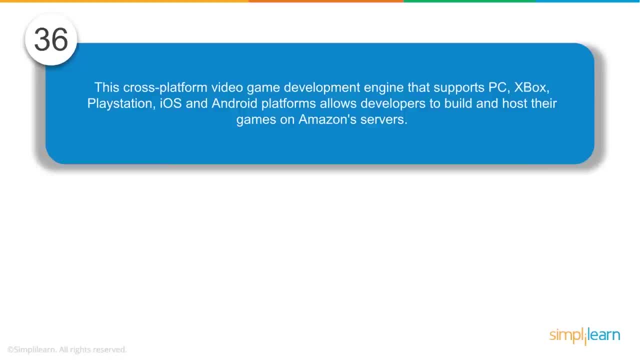 video game development engine that supports PC, Xbox, PlayStation, iOS and Android platforms, allows developers to build and host their games on Amazon's servers. So we have Amazon Gamelift, Amazon Greengrass, Amazon Lumberyard, Amazon Sumerian. Let's read the. 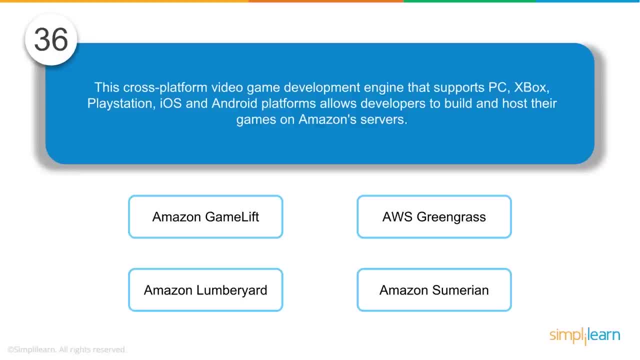 question again. This cross-platform video game development engine that supports PC, Xbox, PlayStation, iOS and Android platforms allows developers to build and host their games on Amazon servers. The answer is Amazon Lumberyard. This Lumberyard is a free AAA gaming engine deeply integrated with AWS and Twitch with 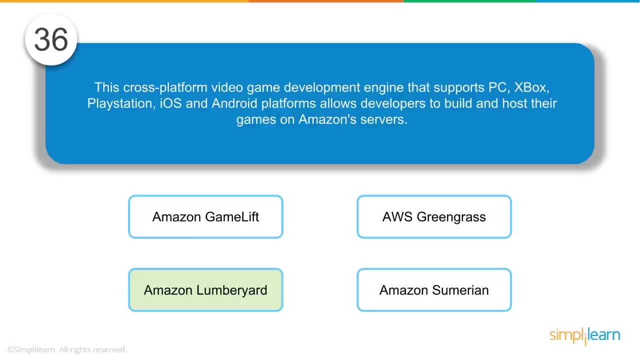 full source. This Lumberyard provides a growing set of tools that helps you create the highest game quality applications And they connect to a lot of games and vast compute and storage in the cloud. So it's that service they are referring to. Let's look at this question. You are the 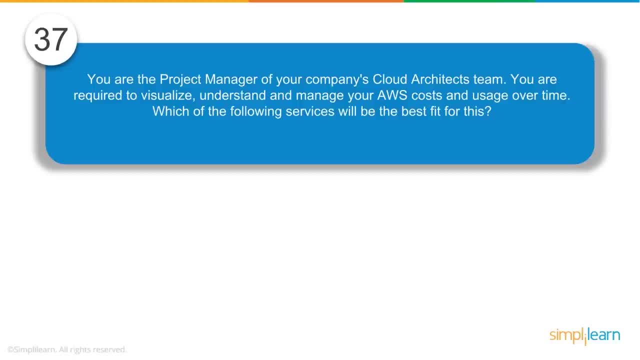 project manager of your company's cloud architect team, You are required to visualize, understand and manage your AWS cost and usage over time. Which of the following service will be the best fit for this? We have AWS Budgets, We have AWS Cost Explorer, We have Amazon. 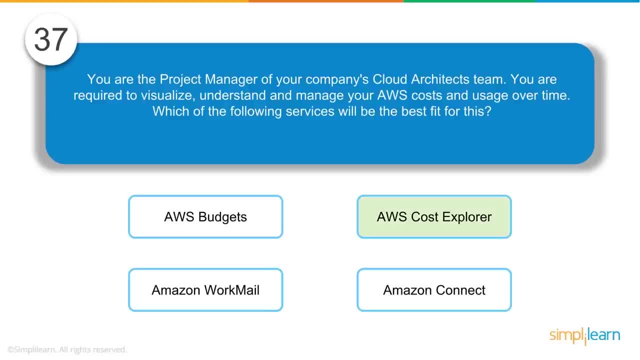 Workmail. We have Amazon Connect And the answer is going to be Cost Explorer. Now, Cost Explorer is an option in the Amazon console that helps you to visualize and understand and even manage the AWS cost over time. Who's spending more, Who's spending less? 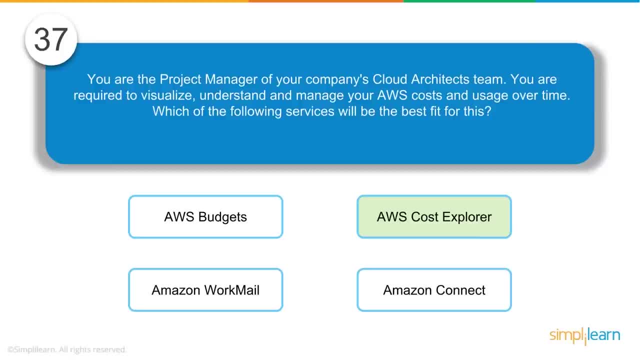 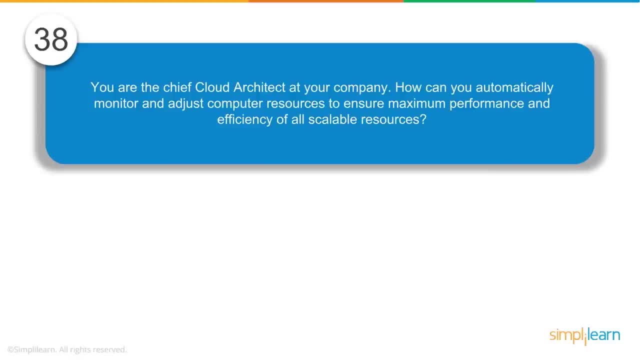 And what is the trend? What is the projected cost for the coming month? All these can be visualized in AWS Cost Explorer. Let's look at this question. You are a chief cloud architect at your company, And how can you automatically monitor and adjust computer resources to ensure? 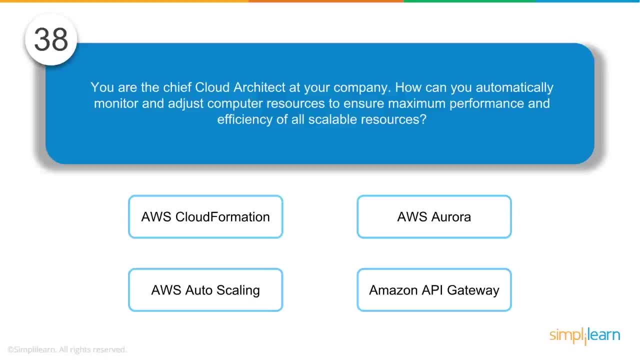 maximum performance and efficiency of all scalable resources. So we have a cloud formation as a service, We have AWS Aurora as a solution, We have AWS Auto Scaling and Amazon API Gateway. Let's read the question again: You are a chief cloud architect at your company. How can you automatically monitor and adjust? 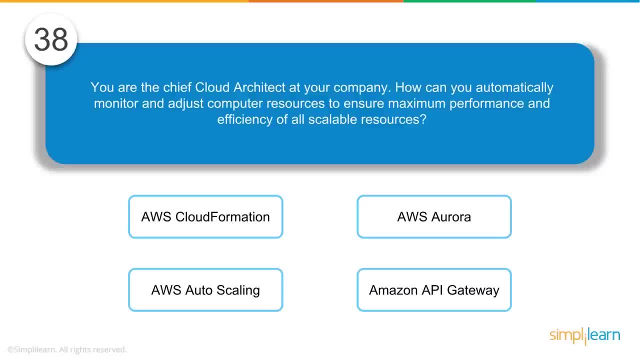 computer resources. How can you automatically monitor and adjust computer resources to ensure maximum performance and efficiency of all scalable resources? This is an easy question to answer. The answer is Auto Scaling. That's a basic service and solution architect course. Auto Scaling is the service that helps us to easily adjust, monitor and ensure the maximum. 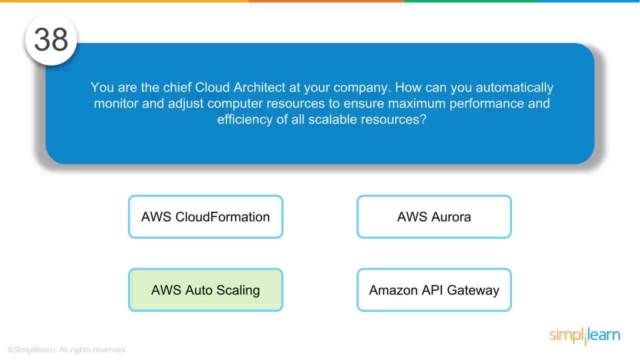 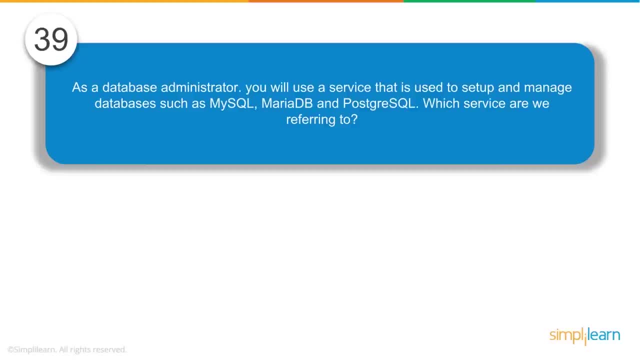 performance and efficiency of all scalable resources. It does that by automatically scaling the environment to handle the inputs. Let's look at this question. As a database administrator, you will use a service that is used to set up and manage databases such as My SQL, Myidb and Postgres SQL. Which service? 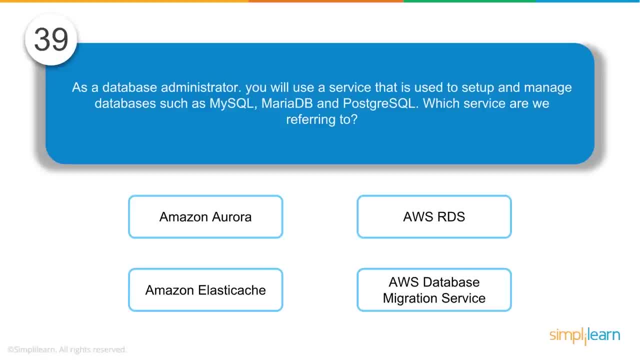 are we referring to Amazon Aurora, Amazon, ElastiCache, AWS, RDS, AWS Database Migration Service? Amazon Aurora is Amazon's flavor of the RDS service, and ElastiCache is the one based on that platform. And then there is also Arabérieur, which can be referred to as a database service. Well, that is going ahead. Let's start with the 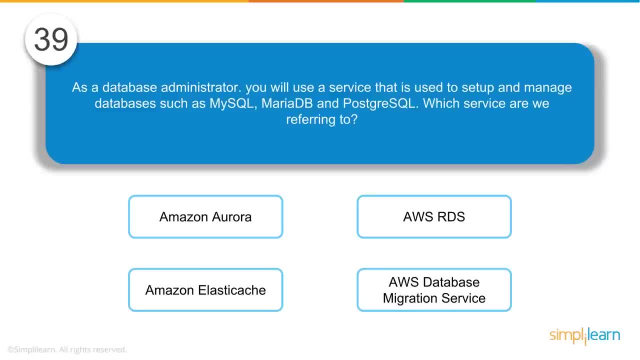 and Elastic Cache is the caching service provided by Amazon. They are not full-fledged database And database migration service, just like the name says. it helps to migrate the database from on-premises to the cloud and from one database flavor to another database flavor. 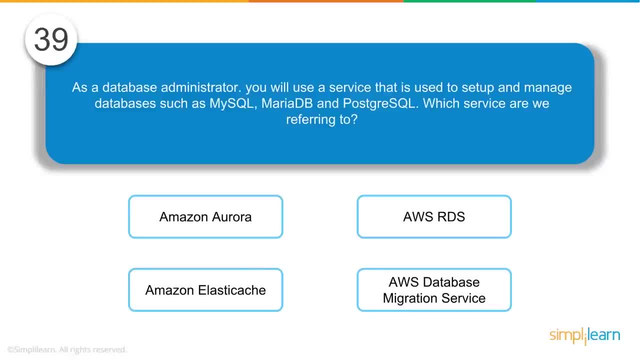 Amazon RDS? is the service? is the console? is the service? is the umbrella service that helps us to set up, manage databases like MySQL, MariaDB and Postgres SQL? It's Amazon RDS. Let's look at this last question. 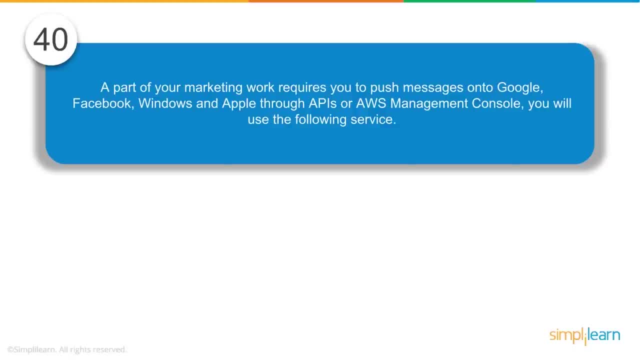 A part of your marketing work requires you to push messages onto Google, Facebook, Windows and Apple through APIs or AWS Management Console. You will use the following service. So the options are: AWS CloudTrail, AWS Config, Amazon Chime, AWS Simple Notification Service. 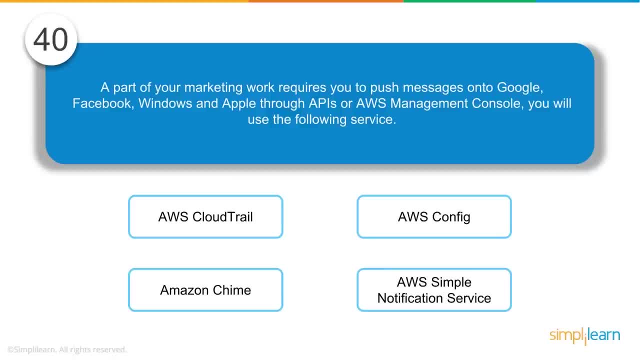 It says: a part of your marketing work requires you to push messages. it's dealing with pushing messages to Google, Facebook, Windows and Apple through APIs or AWS Management Console. You will use the following service: It's Simple Notification Service. Simple Notification Service is a message-pushing service. 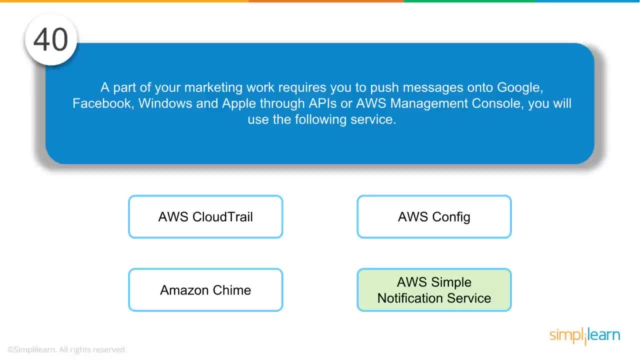 SQS is pulling. Similarly, SNS is pushing. Here it talks about a pushing system that pushes messages to Google, Facebook, Windows and Apple through API, and it's going to be a simple notification system or a simple notification service. I would like to welcome you to this. 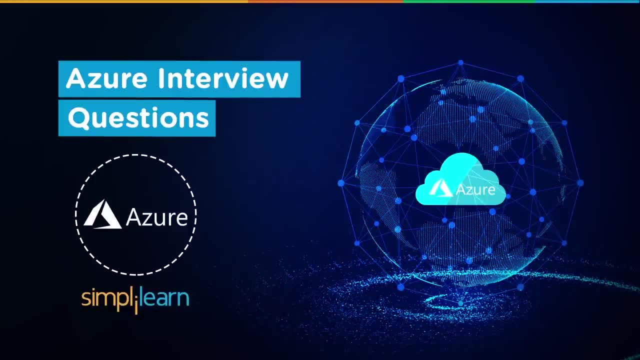 Azure Interview Preparation Session. Knowing Azure is one thing, having worked on Azure is another thing, and being able to answer interview questions in Azure is a totally different thing. Although one helps the other, it's still different skills And our aim through this video is to prepare you with common product. 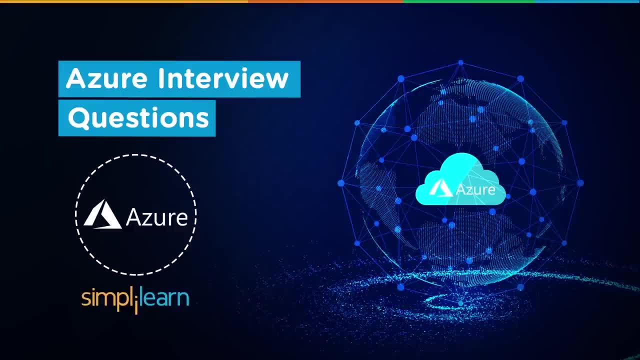 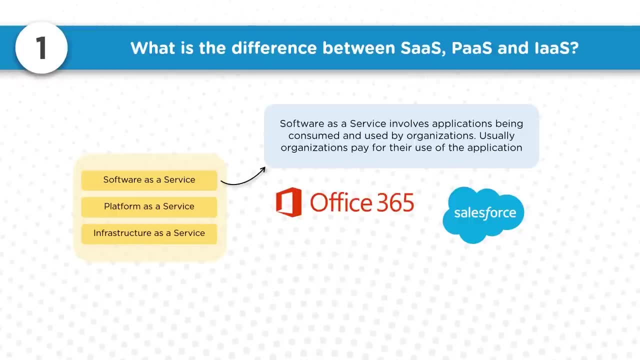 and scenario-based interview questions. So why wait? Let's get started. A common cloud interview question is: what's the difference between Azure and Azure? What's the difference between SaaS, PaaS and IaaS? We all know that a software as a service is thin client model. 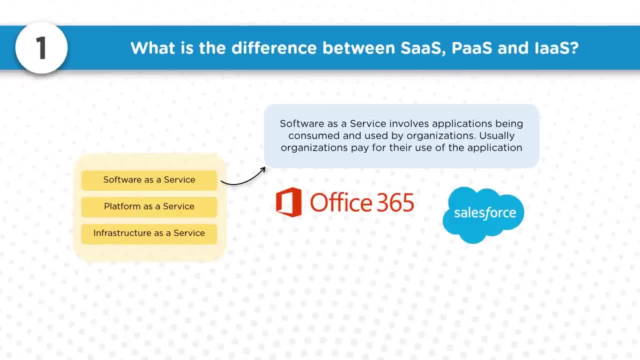 of software provisioning where client, in this case, usually is simply a web browser providing the point of access to software's running on the servers. Now SaaS is the most familiar form of cloud service for customers. SaaS moves the task of managing software and its deployment. 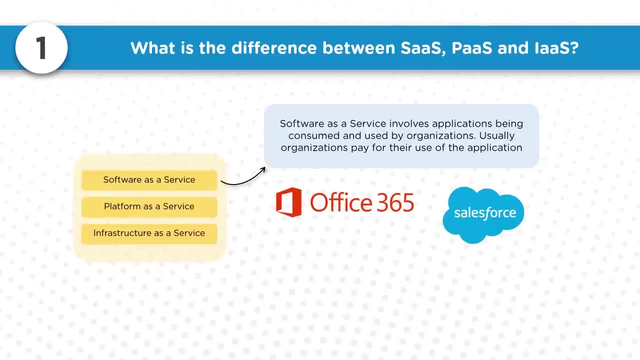 to third-party services, meaning the vendor actually gets to manage all that. So SaaS is software as a service involving applications being consumed and used by organizations. So it's generally using an application And usually organizations pay for their use of this particular application. 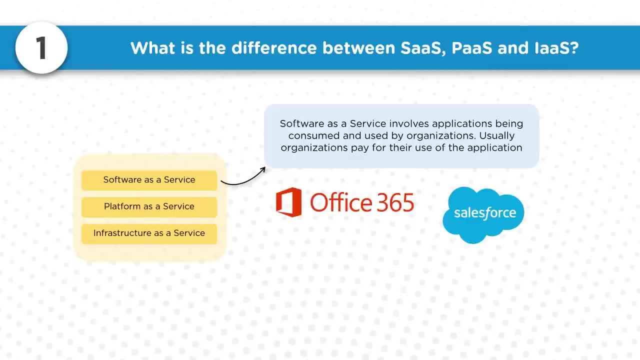 Now some examples of SaaS would include Office 365.. Salesforce is another very good example of SaaS, And a lot of Google apps and storage solutions like Box, Dropbox are a very good example of software as a service. Talking about platform as a service or PaaS. 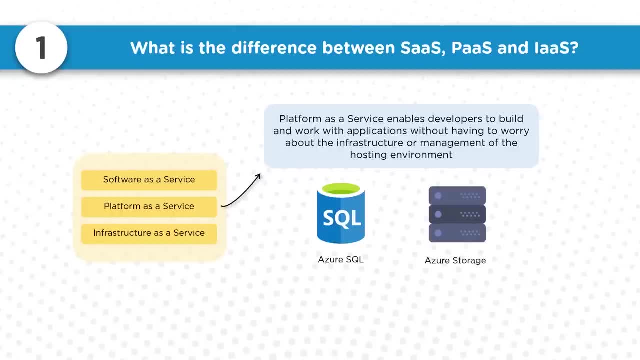 it actually functions at the lower level than SaaS. Now, typically, it provides a platform on which software can be developed and deployed. Now here, we develop the software, We deploy the software. Now, PaaS actually provides an abstract of much of the work. 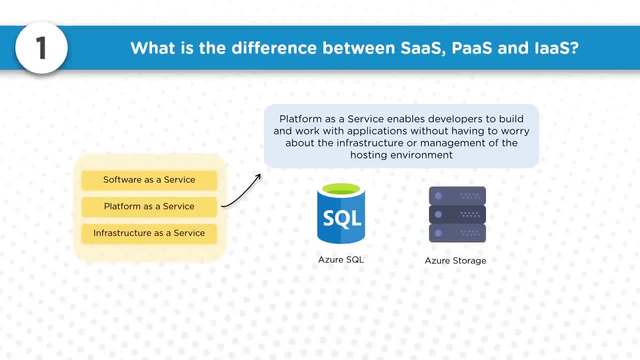 dealing with servers and giving client an environment in which the operating system and the server software and the hardware and the network are managed and taken care, In other words, with a platform as a service. all the things that I've mentioned, like the servers, the server software, the hardware. 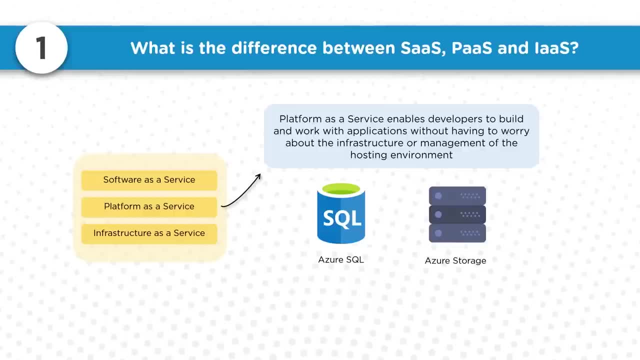 everything is managed by the provider And we can focus on business side of the scalability And we can focus on application development of our product or the service. So, in short, platform as a service is a service that enables developers to build and work with applications. 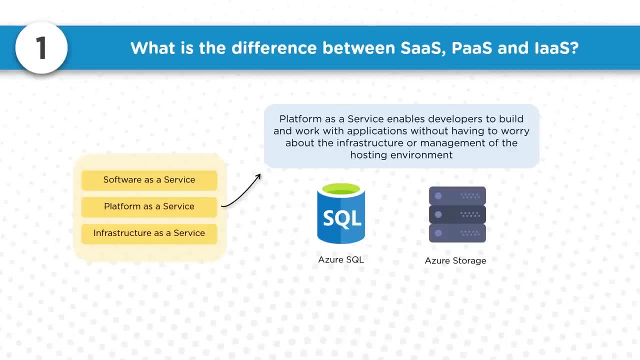 without even having to worry about the infrastructure or management of the underlying hosting environments. And some examples of PaaS in Azure is SQL and Azure Storage. Talking about infrastructure as a service- IaaS- Now this is moving down the stack even further. 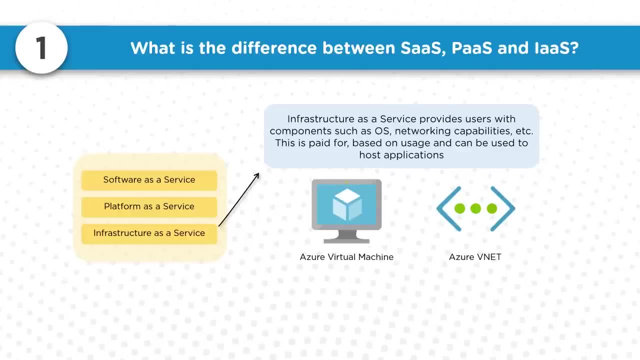 Now we get to the fundamental building block of the cloud service, which is infrastructure as a service, IaaS. Now, IaaS is fully of highly automated, scalable computer resources. IaaS is full of storage. IaaS is full of the network capability. 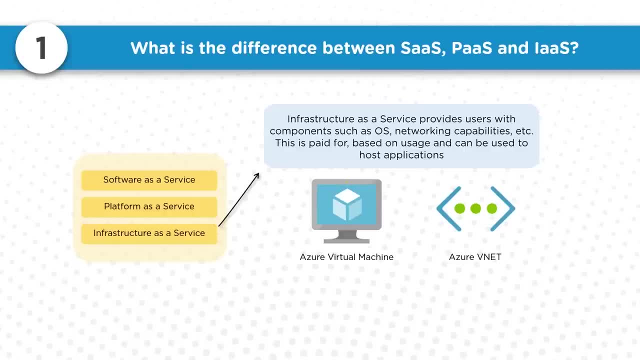 That's what IaaS is Now. IaaS clients have direct access to the servers and storage, just as they would to do traditional servers, But in this case it's going to be in the cloud. In this case, it's going to be more scalable. 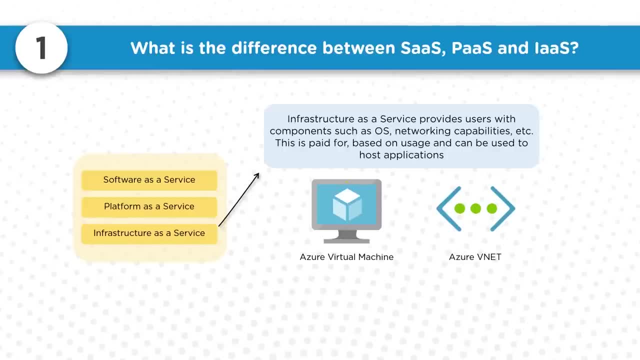 So IaaS is very similar to what you would do in your on-premises. So IaaS is a physical data center. But when we talk about IaaS, we get to do everything, but it's stored in the cloud. So if we need to build a definition around IaaS, 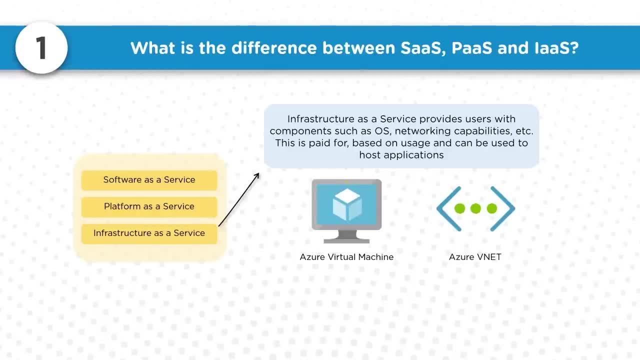 IaaS, or infrastructure as a service, provides users with components. It provides components. It does not give us a built environment. It simply provides a component, such as operating system, networking capabilities and a lot more. Now, this is a paid for based on the usage. 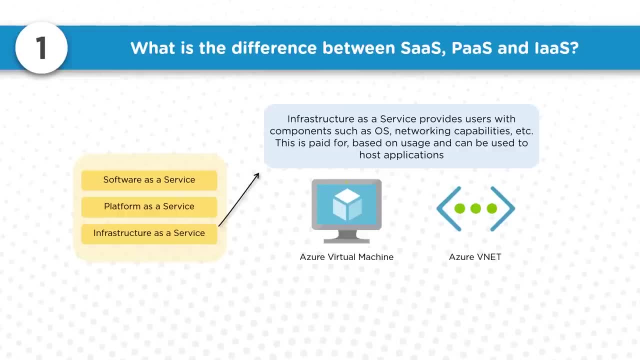 and can be used to host applications. In other words, this is a paid for, This is pay as you go type: The more you use, the more you pay. The less you use, the less you pay. And some of the examples of IaaS in Azure is a virtual machine. 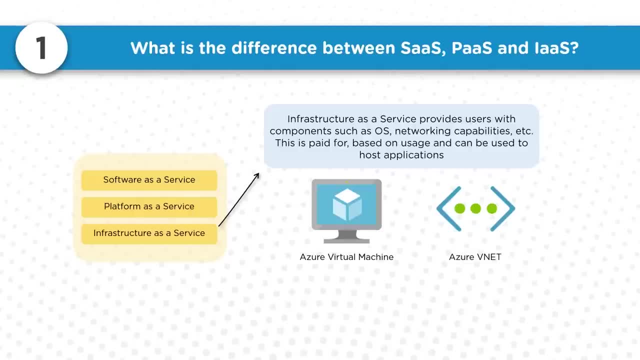 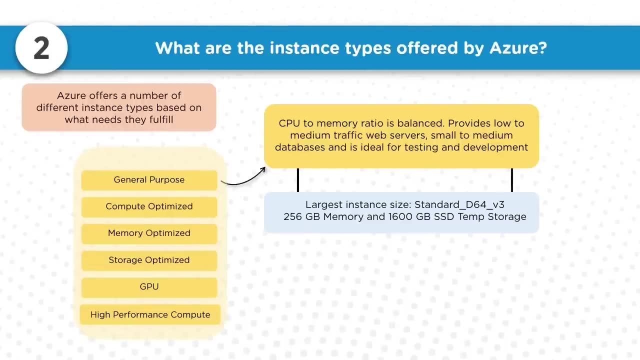 That's a great example for IaaS And VNets for networking. that's another good example for IaaS in Azure. Another common question in Azure interview is: what are the instant types offered by Azure? The main intention of this question is: how well have you understood the different offerings? 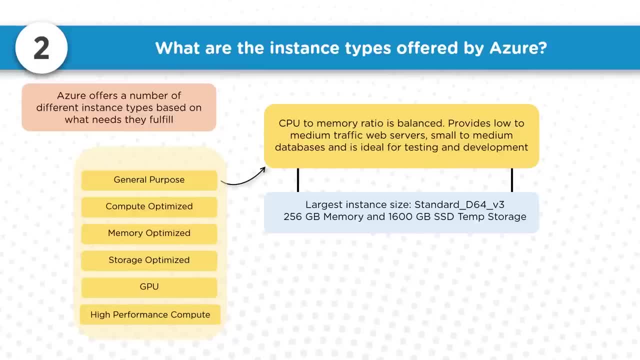 in Azure, And how well are you trained To pick the right offering for the right service? Now, one size does not fit all And there are a lot of services in Azure that, under the carpet, it does the same thing, But depending on how different your requirement is. 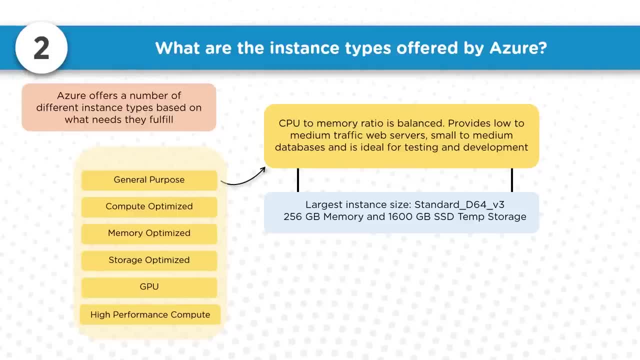 we'll have to pick the appropriate service. So this, actually this question: what are the different instant types offered by Azure? it's to test how well have you used the product and services available in Azure and how well have you applied them for the given requirement. 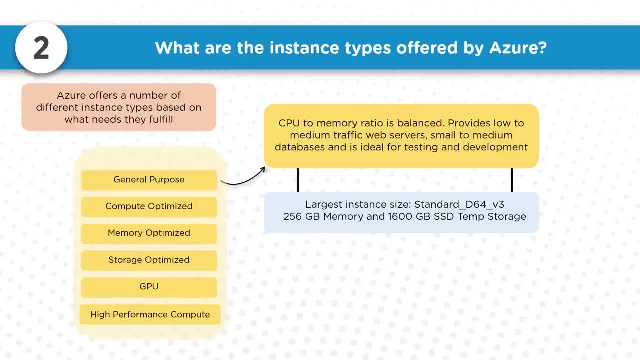 You shouldn't be provisioning more, You shouldn't be provisioning less at the same time. So it's kind of matching the right service to the right requirement. So what are the instant types offered by Azure? As you see in the list, we have general purpose. 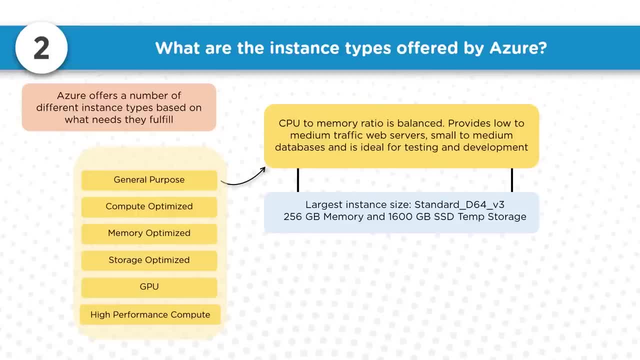 compute: optimized memory, optimized storage, optimized GPU virtual machines and high performance compute virtual machines. Now, answering just the names won't be enough. in an interview You'll have to go further and explain why and in what scenario you would use general purpose. 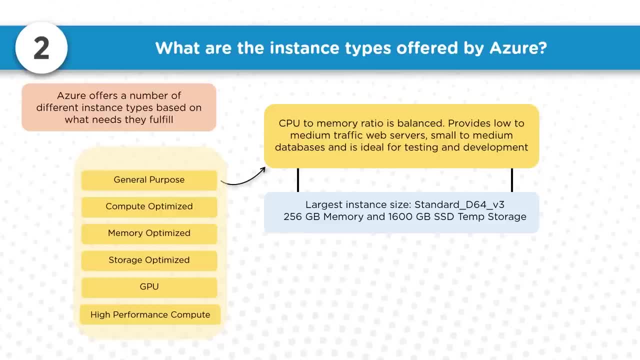 and what are the use cases. what type of servers is a good fit for a general purpose and what type is a good fit for compute optimized, so on and so forth. And that's exactly what we're going to do now. So the general purpose VMs: they provide a balanced CPU. 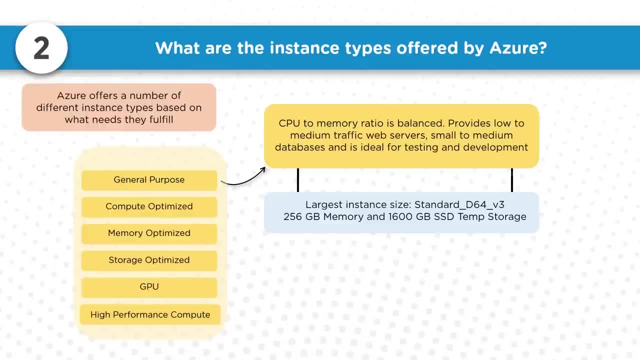 to memory ratio And it's very good for testing, very good for a development environment, very good for small and medium databases and also for low to medium traffic web servers. And some of the use cases are, Like we said, test servers, low traffic web servers. 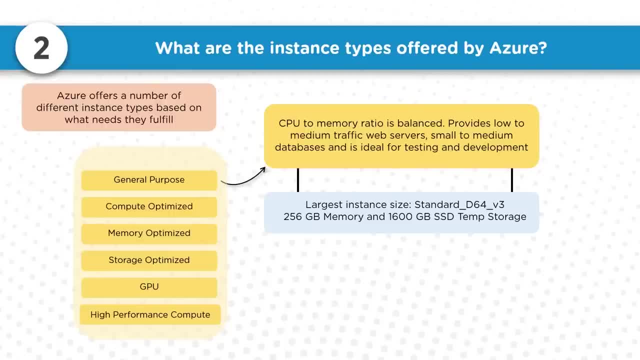 small to medium databases, some enterprise grade applications. It's also good for relational database. It's also good for servers used for in-memory caching. It's also good for some small analytic database, very good for microservices And if you're trying to build a proof of concept for an idea. 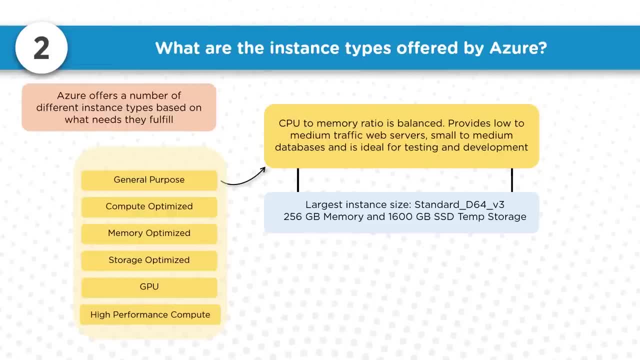 that you just have or just parked. this is another good server for doing proof of concepts, Because you're not going to send actual traffic to it. I just want to show that your idea works. So general purpose server is a very good use case for those scenarios. 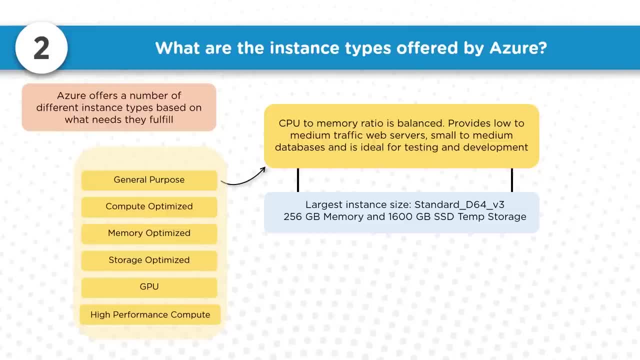 And the largest instance size we can get in general purpose is standard D64v3,, which comes with 256 gigabit of memory and 1,600 gigabit of SSD temporary storage. On the other hand, compute optimized VMs have a high CPU to memory ratio and are very good for. 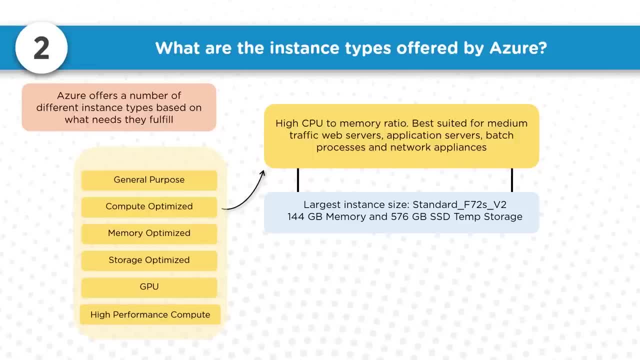 medium traffic web servers. very good for batch processing servers. very good for application servers. Now, because it's compute optimized and compute means a CPU. it's an excellent choice for workloads that demand faster CPU but does not need as much memory or temporary storage. virtual CPU. 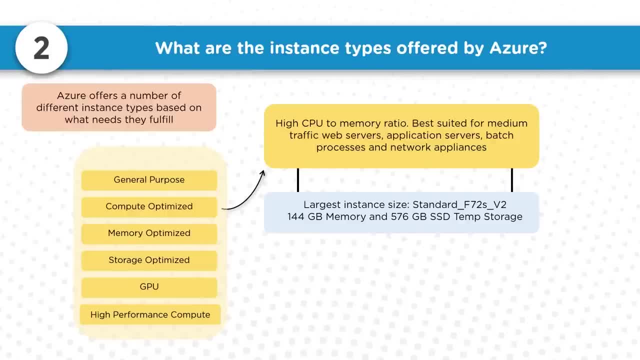 Some of the workloads that run very well on compute optimized are analytic workloads. gaming servers require more CPU. They run really well. batch processing are some of the applications that can be placed in Compute Optimized and by doing that we get the actual benefit of the Compute Optimized instance. 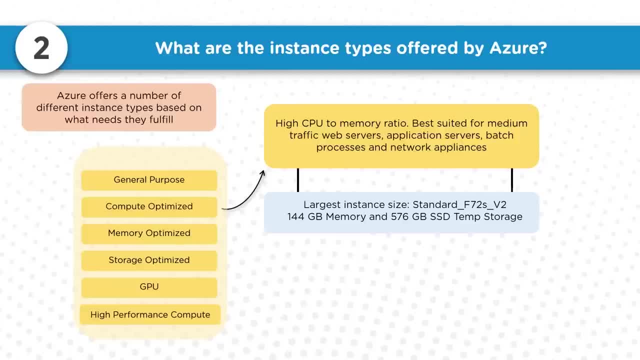 And the largest instance size or the largest instance size type is standard F72's V2.. And here we get 144 gigabit of memory and 576 gigabit of SSD temporary storage in Compute Optimized VMs In the same lines Memory Optimized to VM. they offer high memory to CPU ratio and that. 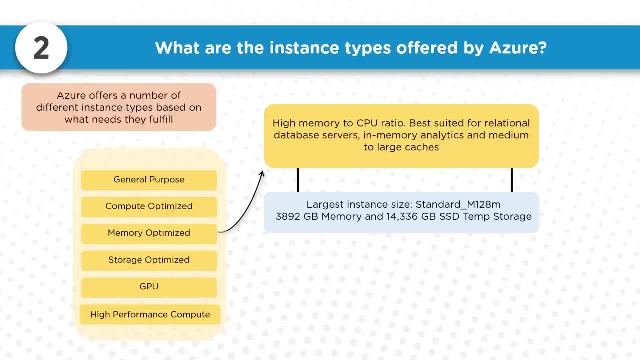 are great for databases. Databases require more memory, So it's a great fit for database, and it's a great fit for medium to large scale caches- applications that require in-memory analytics. So this Memory Optimized memory- is more, so it's very good for in-memory analytics applications. 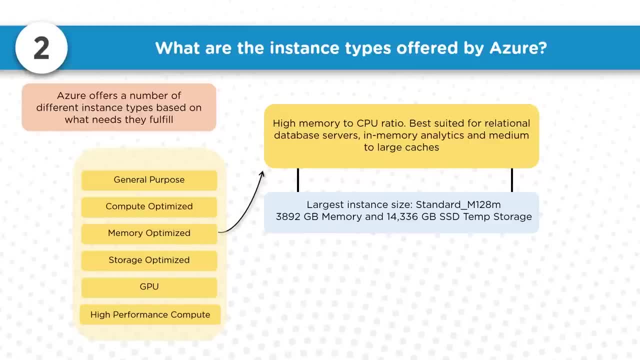 And the largest instance size we get here is standard F72.. It's standard M128M. and look at the gigabit of memory: it's 3,892 gigabit of memory. And look at the temporary storage: it's 1,436 gigabit of temporary storage. 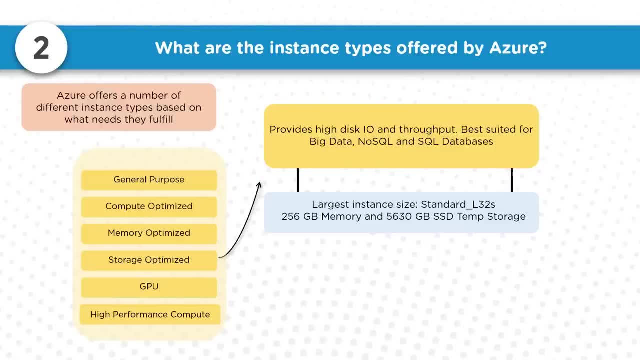 On the same lines. Storage Optimized. Now I guess I don't have to explain to you what Storage Optimized is used for. You might have easily guessed looking at the flow: Yes, Storage Optimized VM Offer High disk throughput and IO and are very ideal for big data SQL, NoSQL databases. 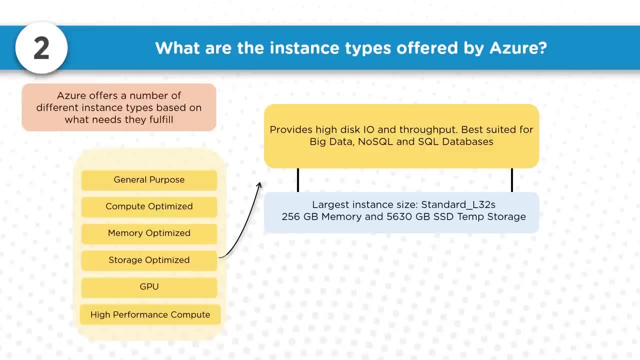 data warehousing servers, large transactional databases and lot more, And some of the examples of the applications that can be launched on Storage Optimized are Cassandra, MongoDB, Cloudera, Redis. These are some familiar applications that can get benefited when we run them on Storage. 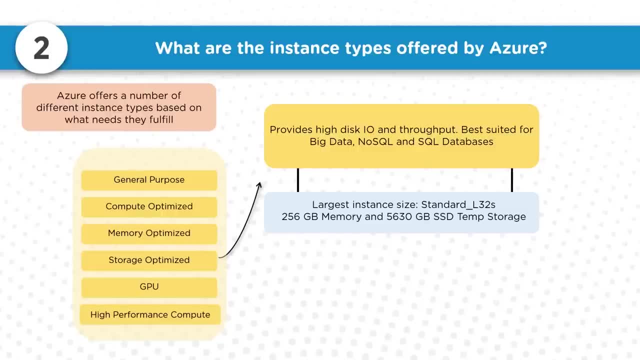 Optimized And one different. The other one is that between Storage Optimized and the other servers are, they are generally optimized to use the local disk on the node attached directly to the VM rather than using an durable disk which is actually an remote disk space. 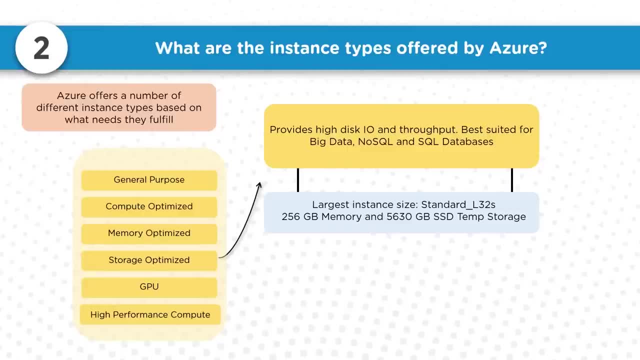 Now, what does this allow? This allows for greater input outputs per second or throughput for the workload. So that's what we get: a greater throughput, a greater input outputs per second is what we get. And when we use Storage Optimized- And the largest instance size available in Storage Optimized is standard L32S and the 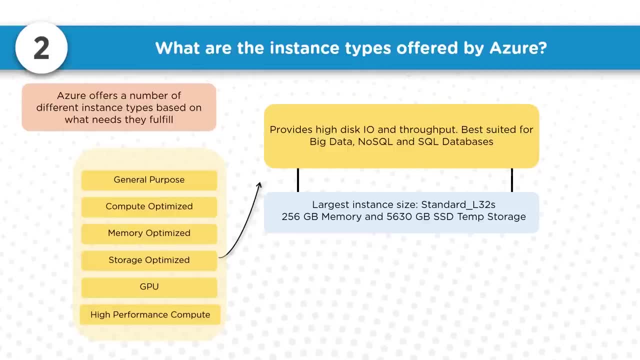 memory is 256 gigabit. And look at the temporary storage: It's 5,630 gigabit of temporary storage. GPU type VMs- easy to guess. GPU optimized VMs are specialized virtual machines available with multiple GPUs attached to them. 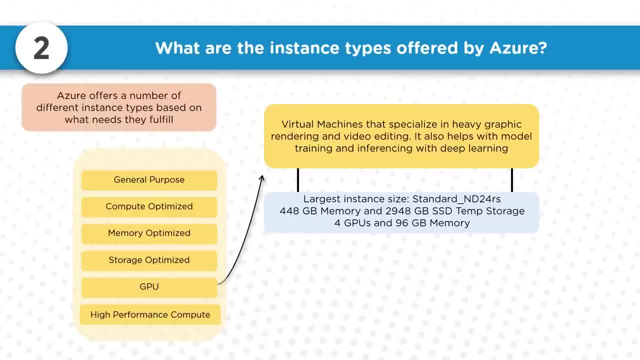 Now these sizes are designed for, or These VMs are designed for, computer intensive, graphic intensive visualization workloads that require a lot of graphical processing unit attached to it. So, in short, these are virtual machines that specialize in heavy graphic rendering and video editing. 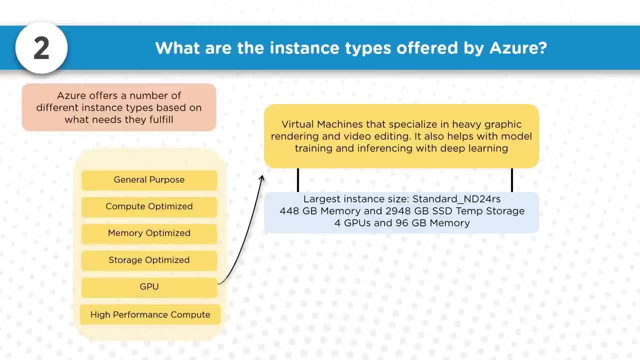 It also helps with model training and interferencing with a standard ND24RS which has 448 gigabit of memory and 2948 gigabit of temperature. So, in short, these are virtual machines that specialize in heavy graphic rendering and video editing. 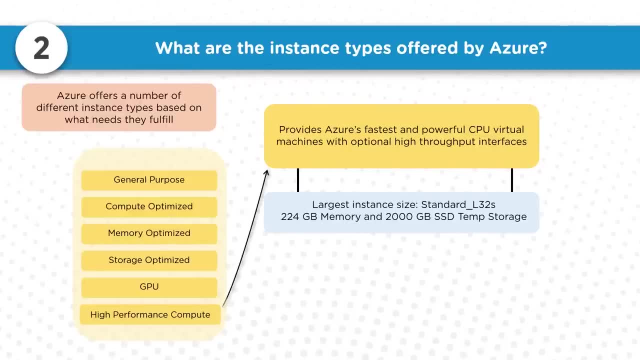 And the last but not the least, but the best. last but the best is high performance compute, or Azure H series virtual machines. Now, they are the latest in high performance computing VMs and are aimed to handle workloads like batch processing, analytic molecular modeling and fluid dynamics. 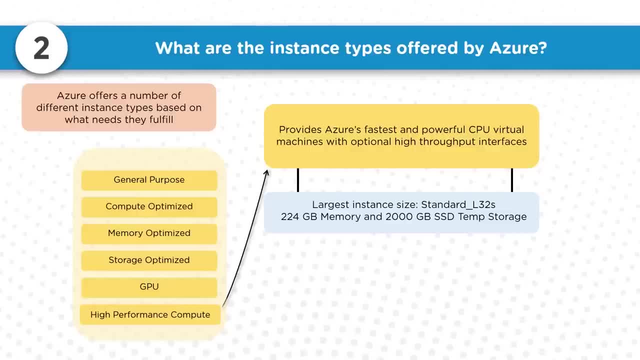 A lot of complicated applications in this VM and this is the fastest and powerful CPU virtual machine And the largest instance size that's available is a standard L32S, which comes with 224 gigabit of memory and 20,000 gigabit of SSD temporary storage. 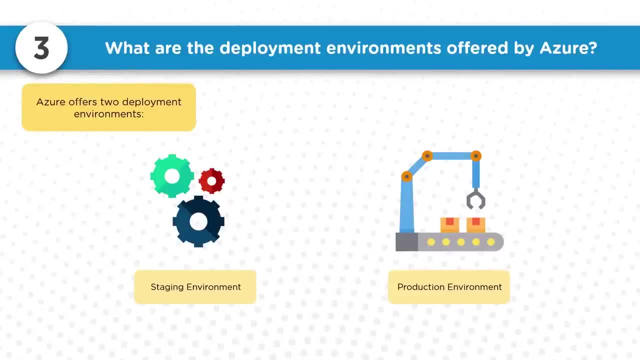 And a third common question is: what are the deployment environments offered by Azure? There are two main deployment environments. One is the staging environment and the other one is the production environment. Now, in staging environment, Let's talk about staging first, So when you're deploying a web app or web app on Linux, you can deploy them to a separate. 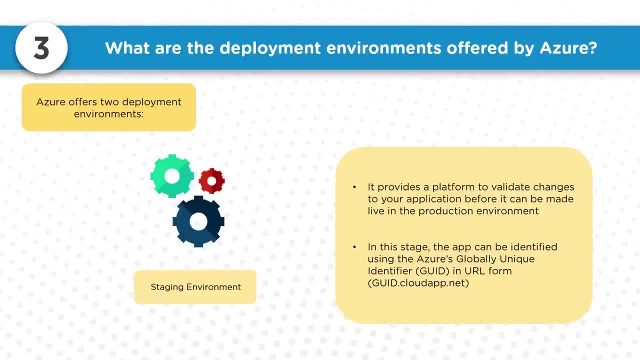 slot instead of the default production slot when running them in standard, premium or isolated app service plan tiers. Now the deployments slots are actually live app with their own host name And, at a later point, that the staging environment can be swapped with the production environment. 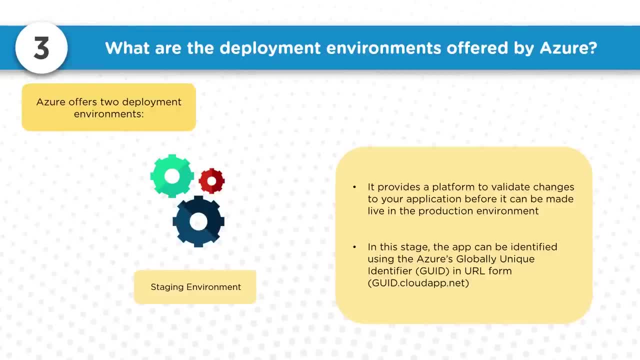 So why do we need an staging environment? What are the benefit of it? So the benefit of deploying our application to a non-production or staging environment: it provides a platform to validate changes to our application before it can be made live in the production environment. 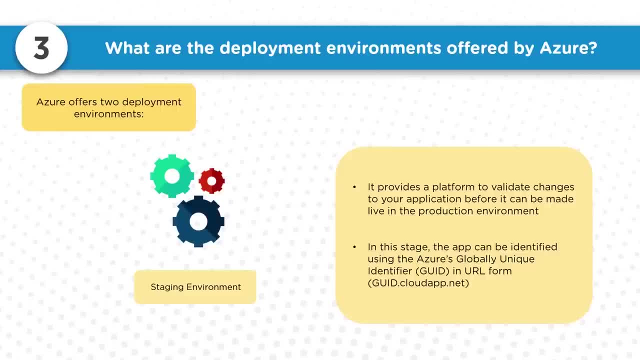 And in the staging environment. the app can be identified using the Azure's global unique identifier, also called as the GUID URL, And it's very, very similar to the production URL, except that it has a custom name in the front of it that identifies it as the staging environment. 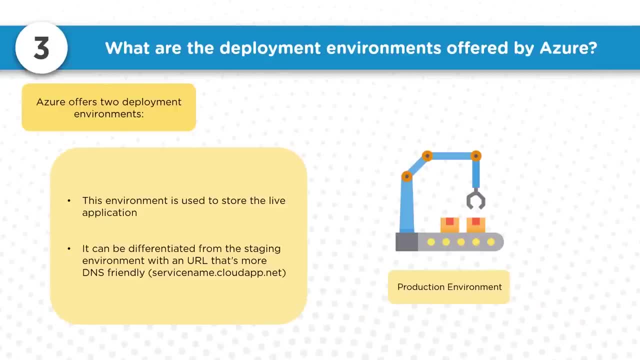 And for production environment. this is the live production environment. that's serving customers request. that's serving the customer content. Now it can be slightly different from the staging environment in a way that the URL that's used to identify the production environment that's more often DNS friendly name, like the. 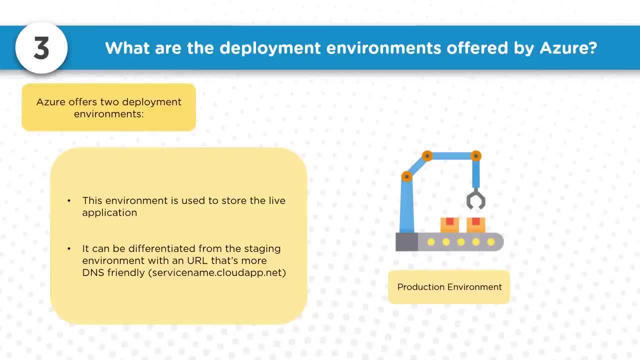 name of the actual servicecloudappscom. So that's a little bit different. So let's talk about staging environment. So in the staging environment you have a custom name right before it, So the custom name and then the cloudappnet. 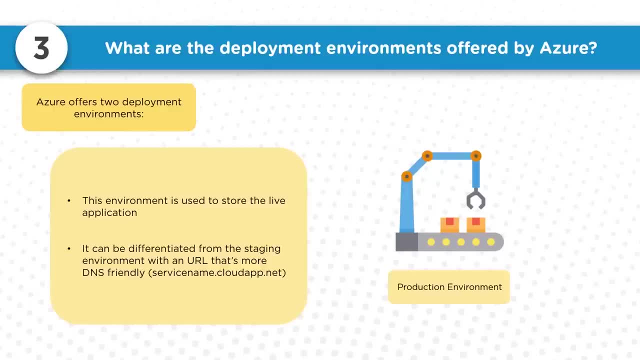 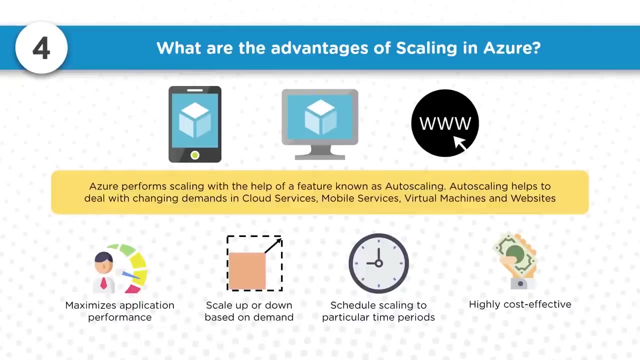 But in this case you get the direct service name as the name of the URL. So this is live production environment which receives and handles and serves customer traffic. Another commonly asked question in Azure is: what are the advantages of scaling in Azure? The actual thought behind the question is to see: 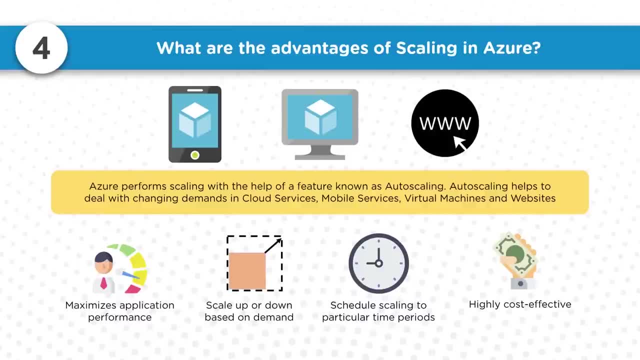 How much have you understood scaling? How much have you seen and how much have you applied the scaling effect in the production environment and have received benefits in return? So let's talk about it. Advantages of scaling in Azure. Some of the advantages are: we get the maximum application performance. 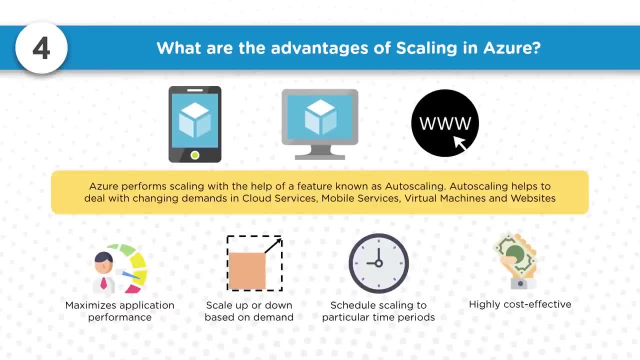 Now, auto scaling is a built in feature for the cloud services, be it AWS, Azure, Google and a couple of other cloud service providers. It's a built in feature for a cloud service. A cloud service should be auto scalable, And that includes mobile services, virtual machines. 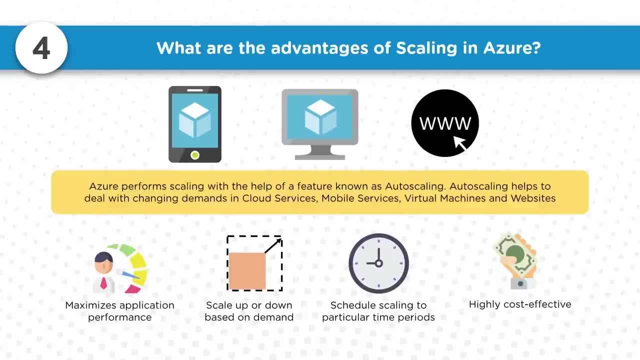 And when we run our applications on mobile services or virtual machines, the website actually gets the best performance during the change in the demand. Again, different applications might require different performance needs. For example, for some apps, the performance is measured based on memory. 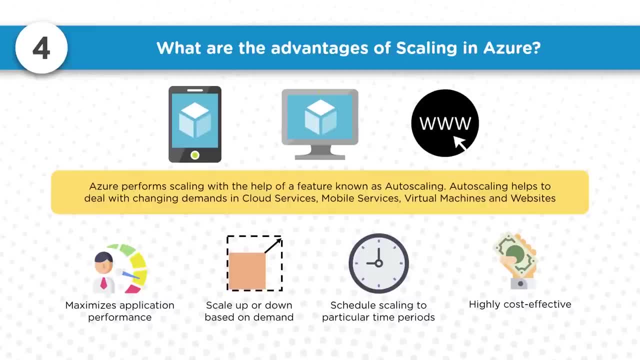 And another good example is the software. So the software is based on memory. The performance is measured based on the fluctuating demand. For example, you could have a web app that handles millions of requests during the day and literally nothing at the night. 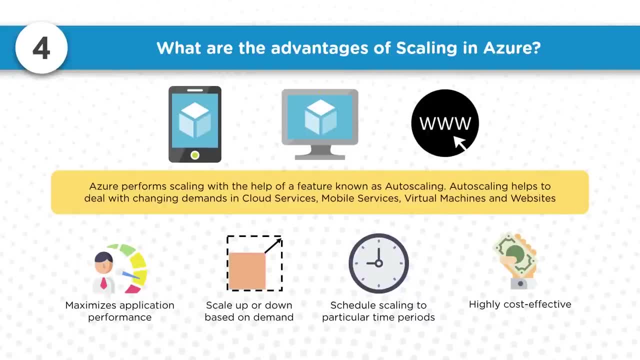 And auto scaling this environment. auto scaling any of these environment will automatically scale or fatten your environment So to receive the all the incoming traffic and during lean period it actually gets slimmer and slimmer. So to help you with the cost, 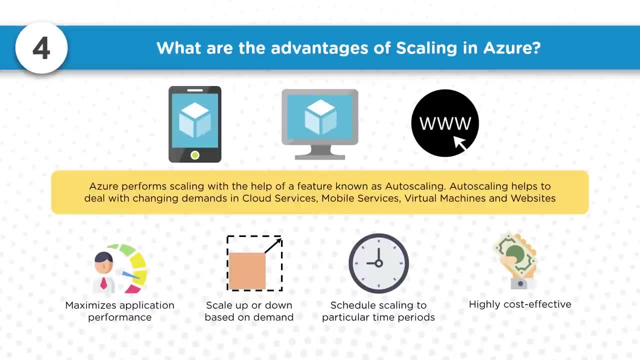 So it actually maximizes the performance. That's what auto scaling does And, like we said, auto scaling, It scales up and scales down based on demand. It not only scales up, but also scales down. So to help you with the cost, 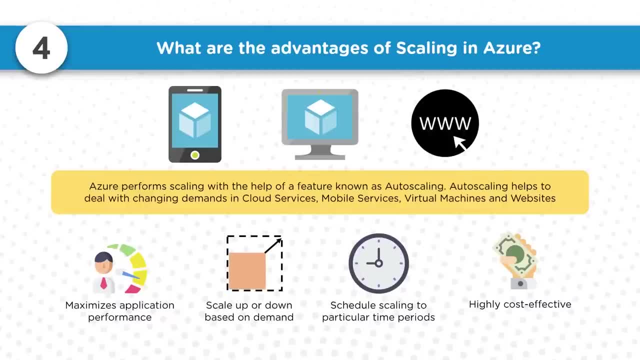 And if you know the particular pattern in which the application is going to receive traffic, then we can very well go ahead and schedule scaling to our application or schedule scaling that infrastructure based on time, If we already know that Monday to Friday that's the traffic that I would get. 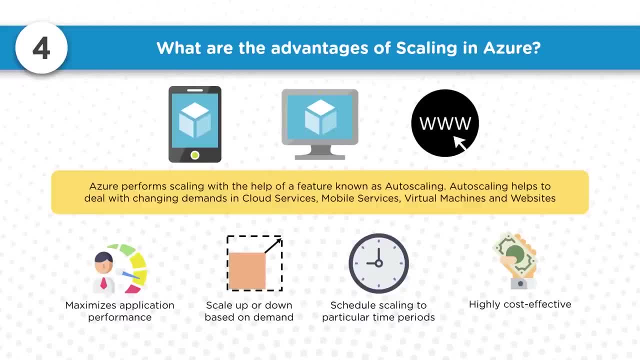 And it's a constant one. It's not a public facing, But you know it's an internal application. So I know all the 500 users or the 1000 or the 5000 users who will be using it. So at any given point it's just 5000 users. 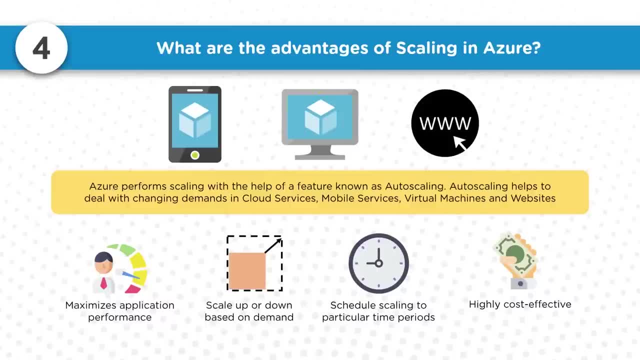 It's not going to go beyond that, And during Saturday and Sunday literally nobody's going to be in office, So no load at all. So in that case I pretty much know how the pattern is going to be. I can go for scheduled scaling if I know the pattern. 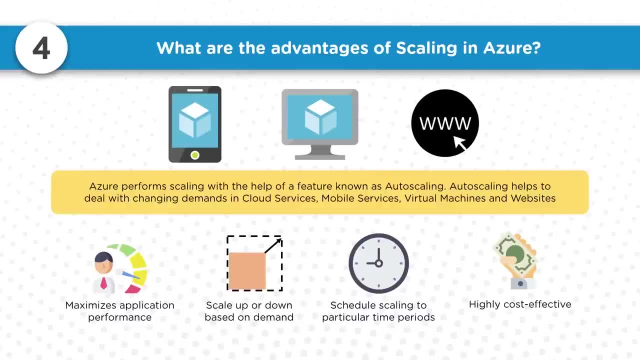 And auto scaling, like I said, not only helps with keeping the application highly available, it also helps with the cost effectiveness Of our infrastructure. So anytime there's a VM or a group of VMs running on less CPU, auto scaling is going. 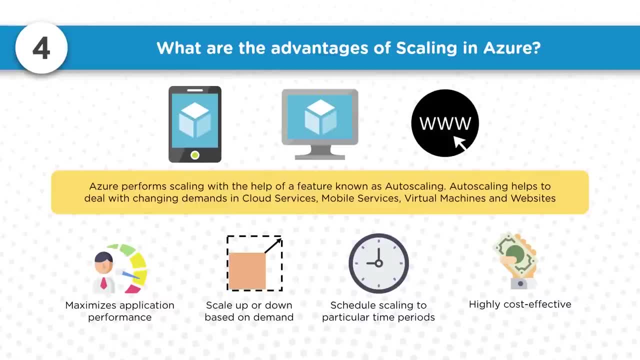 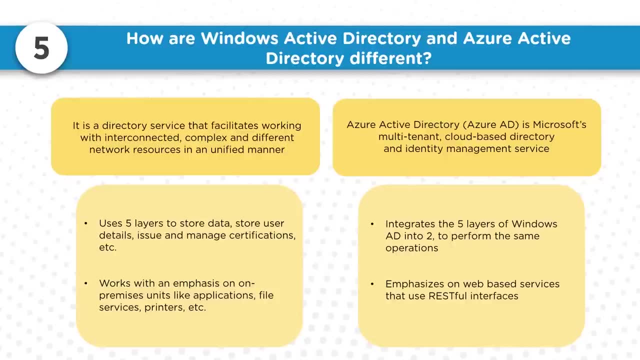 to actually get the environment slimmer and slimmer, So we're not unnecessarily running any resources and paying for it. If you're being interviewed for the infra site in Azure, this is another common question that gets asked. How are Windows Active Directory and Azure Active Directory different? 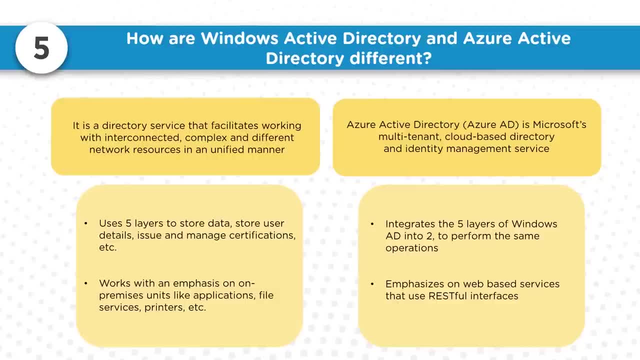 Let's talk about the Windows Active Directory first, The non-cloud Windows Active Directory. The service was released along with Windows 2000 Server Edition And this Active Directory is essentially a database that helps organizations to organize the users, organize the computers and a lot more. 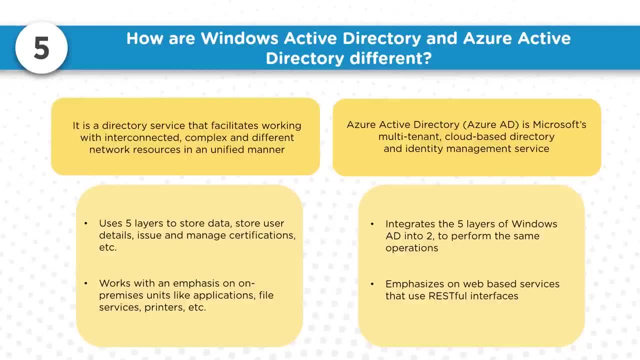 It provides authentication and authorization to the applications- Not only to the applications, but also to file servers, to printers and a lot of other on-premises resources. That's what the basic non-cloud Active Directory does. On the other hand, the Azure Active Directory is not designed to manage web-based services. 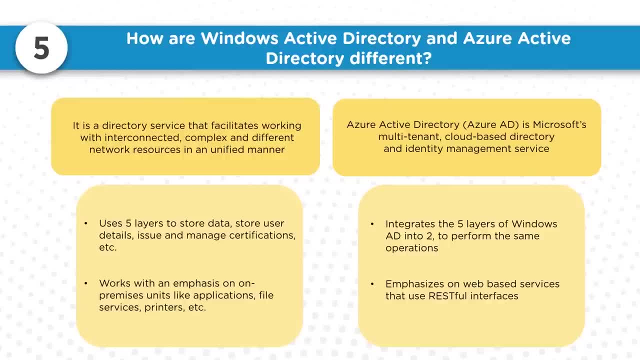 The Azure Active Directory, on the other hand, was designed to support web-based services that use REST API interfaces for Office 365, Salesforcecom, etc. Unlike the plain Active Directory, this uses a completely different protocol, So protocol-wise it's different. 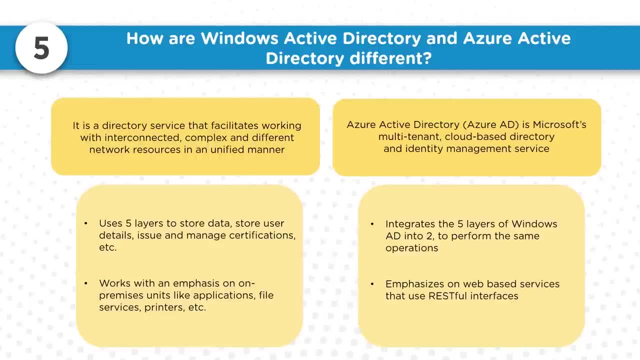 And the services that it supports is quite different. Now, besides that, it also has a couple of other differences as well, And let's look at them. So the actual Active Directory, or the Windows Active Directory, is a directory service that facilitates working with interconnected, complex and different network resources in a very 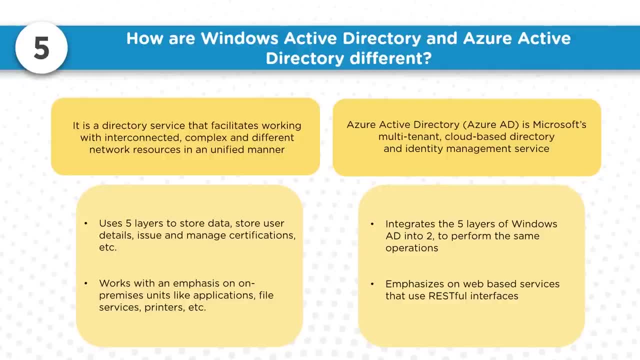 unified manner. On the other hand, Azure Active Directory is Microsoft's multi-tenant cloud-based directory and identity management service, And the Windows Active Directory has five layers: to store data, to store user details and to issue data. On the other hand, Azure Active Directory integrates or compresses the five layers into 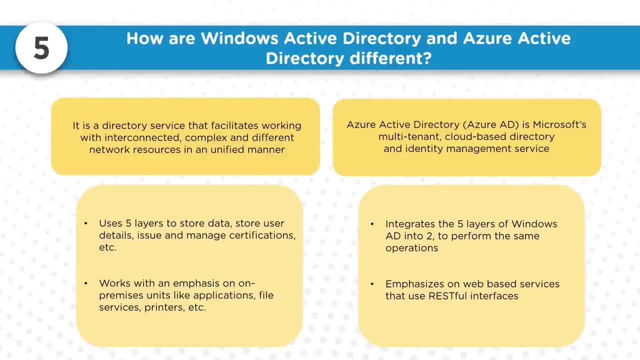 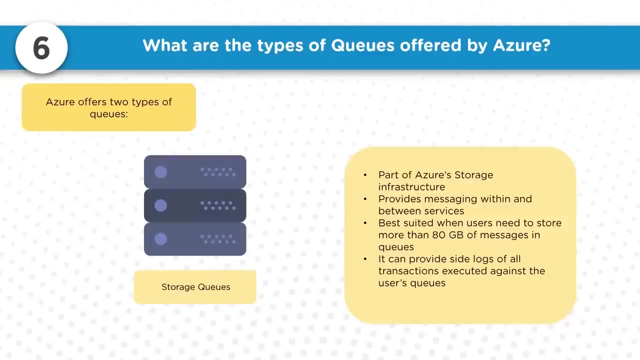 just two layers Here. Windows Active Directory works with on-premises servers like applications, file servers and printers, etc. On the other hand, Azure Active Directory- it works on web-based services that use RESTful interfaces. If you're being hired for the development environment or for the cloud-based services, 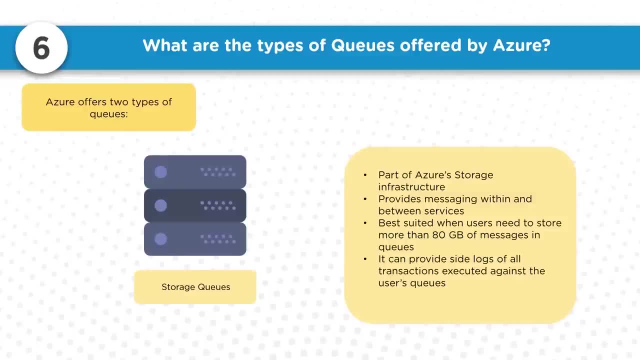 the cloud DevOps support environment, or even for the production support environment. you might find yourself being asked this question: What are the types of queues offered by Azure? Now, Azure supports two types of queue mechanisms: the storage queue and the service bus queue. 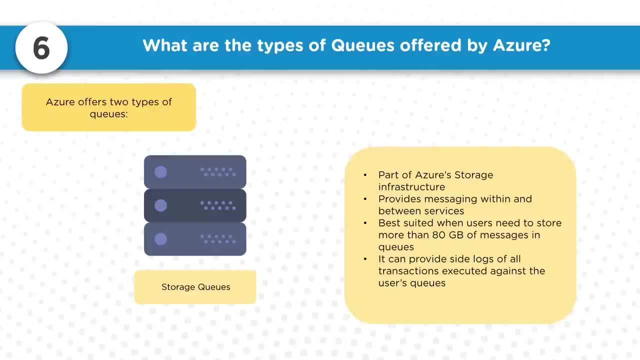 Let's talk about storage queue first, Now the storage queue, which are part of Azure storage infrastructure. it provides a simple REST-based interface, Simple REST-based get put and pick. It provides reliable, persistent messaging within and between the services. 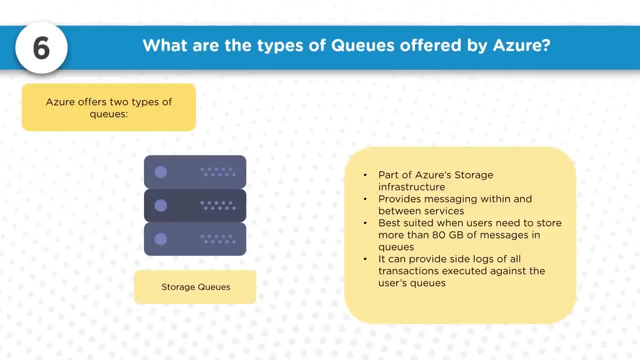 It follows the Pub-Sub model or a Pub-Sub messaging infrastructure, and it's best suited for users that need to store more than 80 gigabit of messages in the queue. It can provide logs for all the transactions executed against the user's queue. 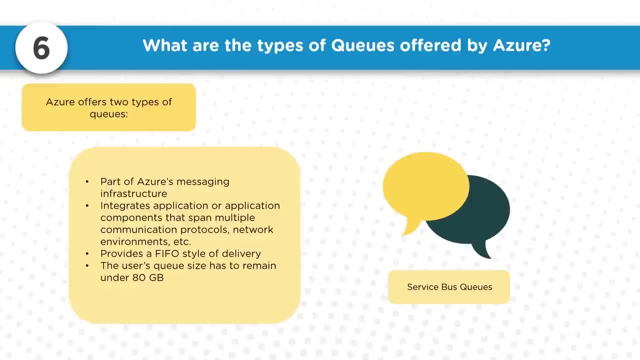 So that's what we get with storage queue And, on the other hand, service bus queue. the service bus queues are built on top of broader messaging infrastructure and they are designed to integrate applications and applications component that can span multiple communication protocols. So that way it differs. 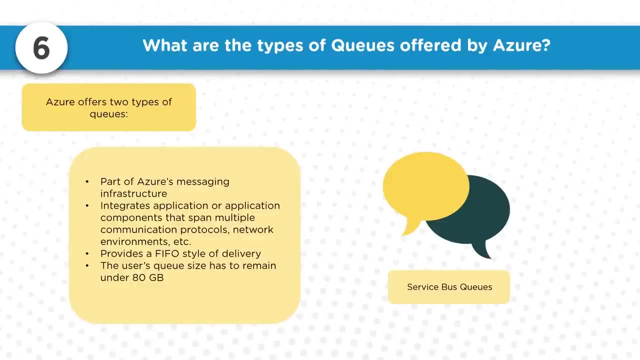 So this is good for applications and components that may span multiple communication protocols and even different, totally different network environments. So, in short, these service buses, or the service bus queues in Azure, are part of Azure's messaging infrastructure. They integrate applications or application components that can actually span multiple. 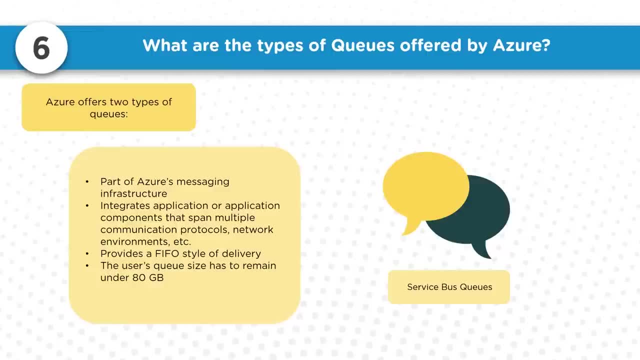 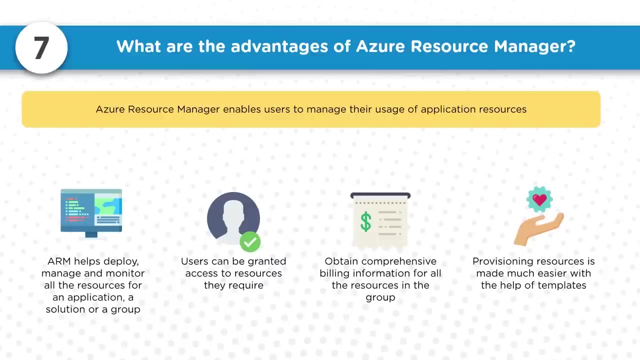 different protocols and multiple different network environments. It also provides a first-in-first-out style for delivery, and the user's queue size has to remain under 80 gigabit. Another familiar question is: what are the advantages of Azure Resource Manager? Now, the Resource Manager helps us to manage the usage of the application resources. 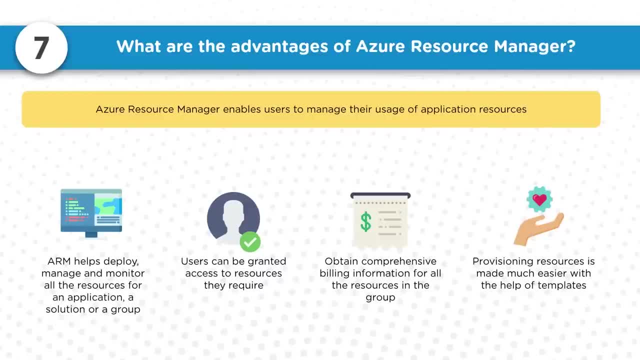 This question is actually to test how well have you tested, how well have you used Resource Manager And have you gotten the benefit of it? This question actually tests how easy it has become after the introduction of Resource Manager, compared to when doing deployments or when provisioning resources without the 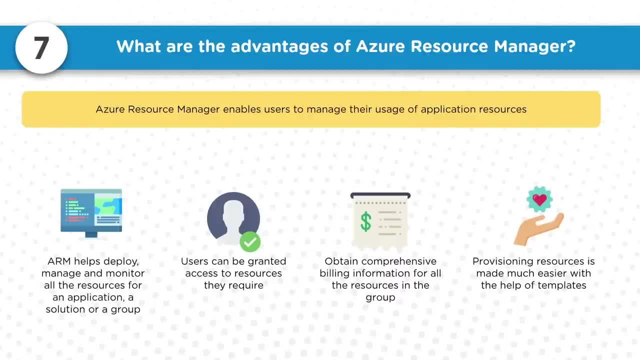 Resource Manager. So let's get into the answers for the question. What are the advantages of Azure Resource Manager? The, in short Resource Manager, is called ARM. So the ARM helps deploy, manage and monitor all the resources for an application, a solution. 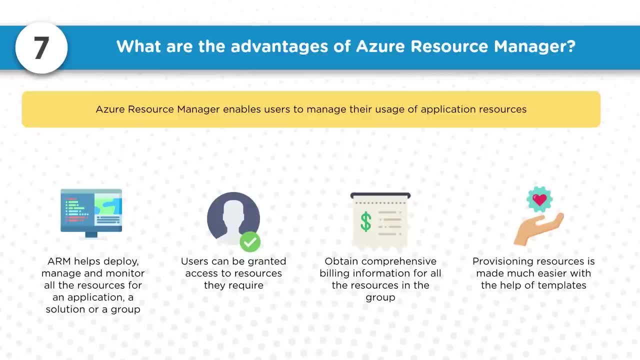 or a group. So all the interconnected application, all the interconnected services can be monitored as group using Resource Manager And users can be granted to access to resources that they require within a Resource Manager. So in an account I can have like 10 different resources created by a Resource Manager or 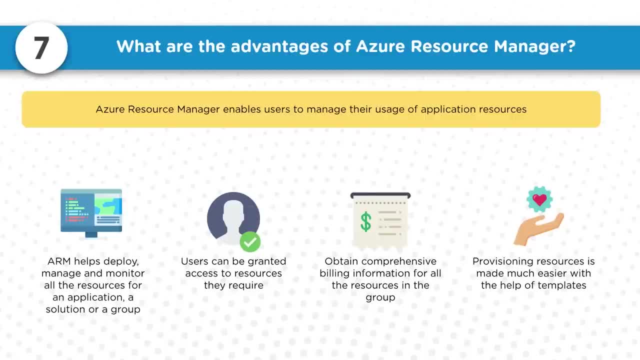 a resource group created by Resource Managers, and I can allow deny connection to those services or only to those services, based on whether the user should be accessing one and not accessing the other. So that way it becomes easy to give access to a group of application. 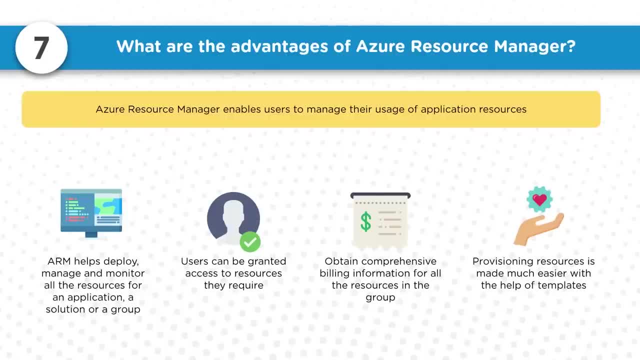 It helps in getting billing details for the group of resources- Now which group is using more, Which group is using less And which group has contributed more to this month's bill Stuff like that. So those details can be obtained using Azure Resource Manager. 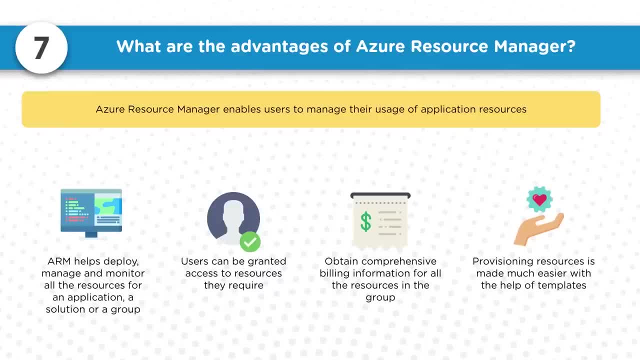 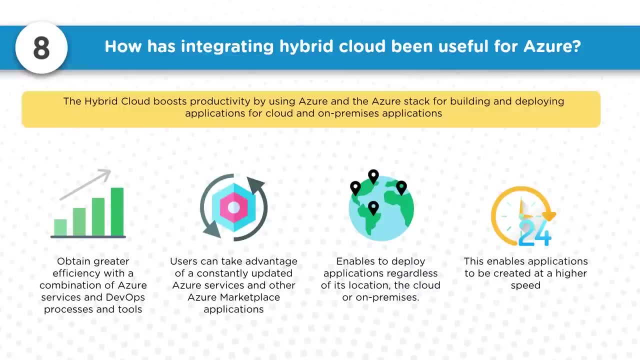 And provisioning resources is made much easier with the help of this Resource Manager. Another question is: how has integrating hybrid cloud been useful for Azure? Well, with the use of hybrid cloud, we get the best of both the worlds. So what's hybrid cloud? 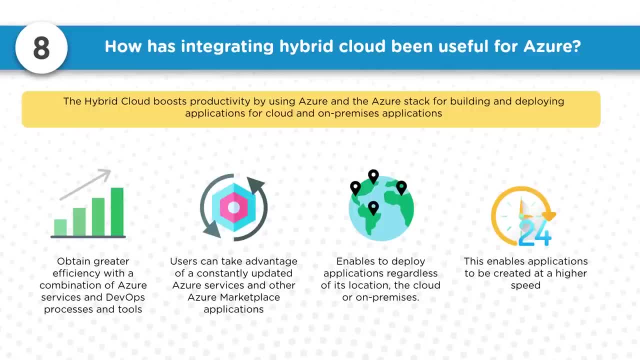 It's nothing but combining the public cloud and the private cloud and allowing data and applications to be shared between them. So whenever the compute or the processing demand fluctuates, hybrid cloud computing gives businesses the ability to seamlessly scale their on-premises infrastructure in. 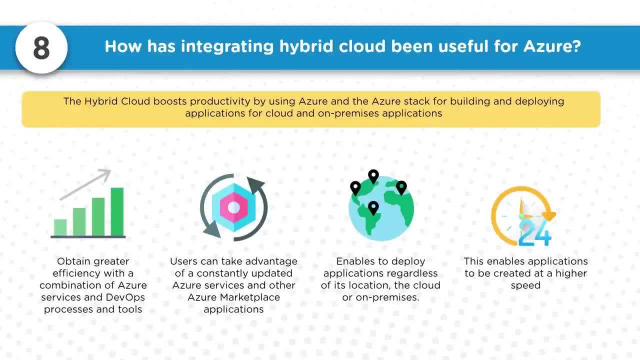 the public cloud and handle any kind of overflow in the required infrastructure. So that's what we're doing. So hybrid cloud gives us the ability to really see what's happening within the requirement or overflow in handling the application. So it really helps. It helps boost the productivity of our on-premises application. 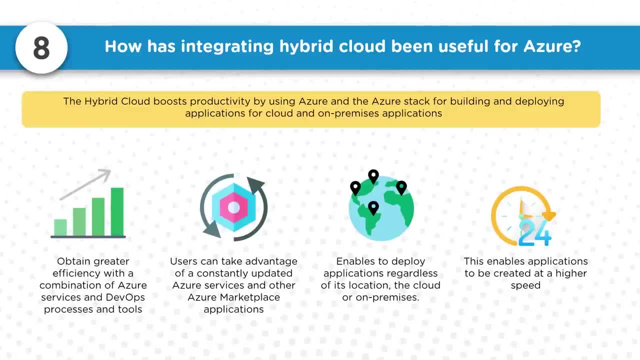 So with the hybrid cloud we get a greater efficiency with combination of Azure services, DevOps process and tools for the application running in on-premises, And by having a hybrid cloud environment users can take advantage of a constantly updated Azure service. 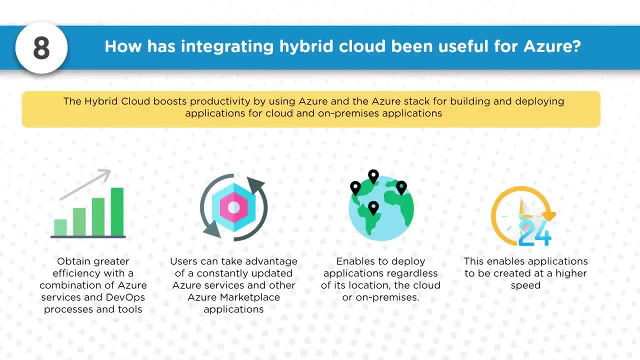 applications for their on-premises environment. and the other benefit is, with hybrid cloud environment, we can simply deploy applications regardless of its locations. in case of on-premises, we'll have to worry about the location, but when we expand our on-premises environment in the cloud- and they can or 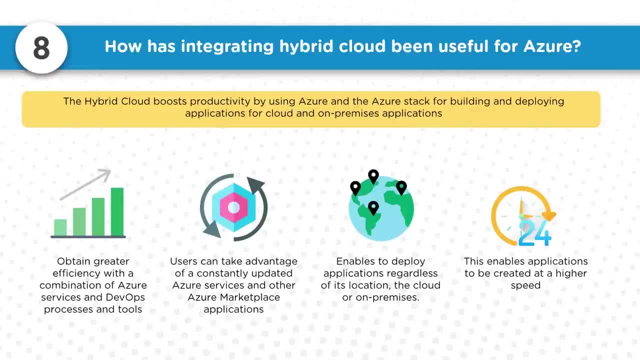 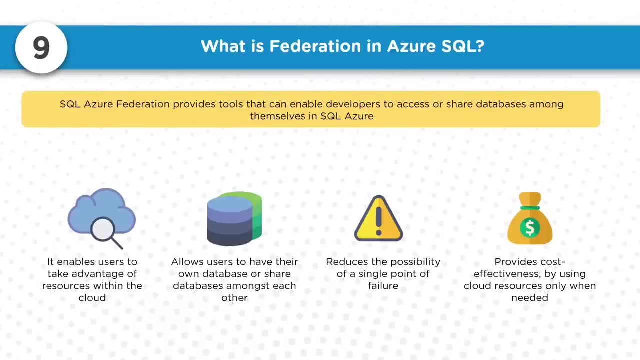 we can pick any of the locations and simply deploy it in them, and this enables the applications to be created at a greater speed. what's federating in Azure SQL? now, this question is very specific about SQL. how can we scale the SQL database? now? this is a very good question, or a valid question, or an 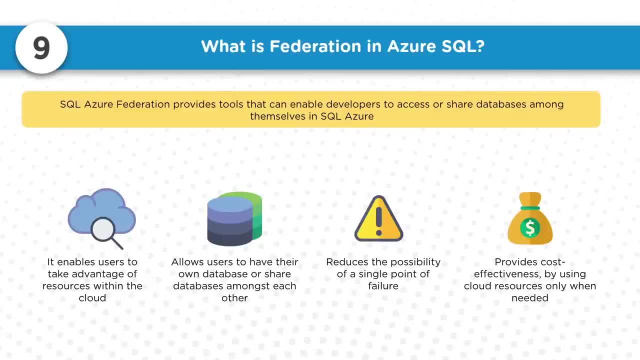 important question in the interview because many customers or companies have and not been able to meet the user demand because they could not scale out the databases. the theory of scaling out or adding servers to accommodate the increased workloads and traffic is not hard to understand, but the implication 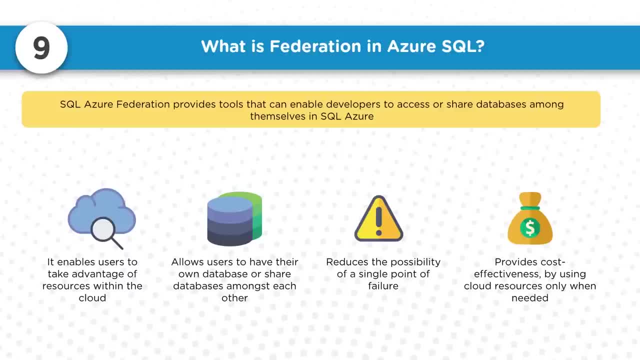 of this question is that we can scale out the database and we can scale out the the database and we can scale out the database and we can scale out the applications can be very complicated. the implications can be very expensive. we're well aware of scaling the web servers. that's very common. but how do we scale? 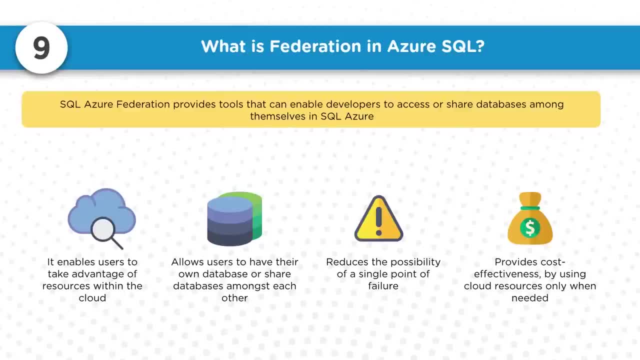 the database. so Microsoft provides the tools and technologies so we can scale out the database in the cloud and that's what is called SQL or Federation in Azure SQL. so the way we scale out the SQL database is by sharding- sharding the database. so sharding actually enables users to 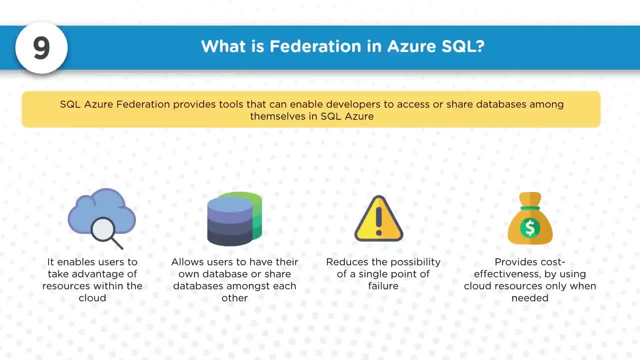 to scale out the databases and actually vanigned the databases for the advantage of the resources in the cloud. not only that, it allows users to have their own database or a shared database amongst each other because we're creating and highly available database, because we're having shards in a database. it 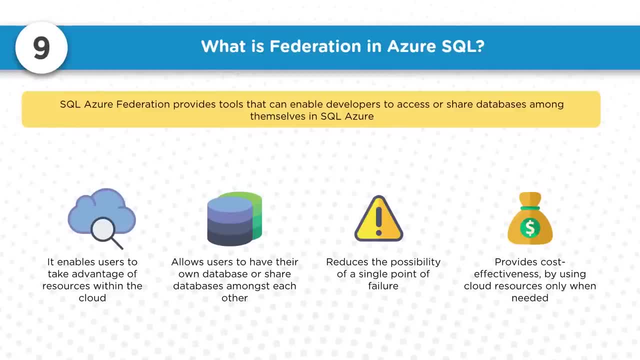 actually reduces the possibility of a single point of failure for our database and, more importantly, because we're shining, because we're using Federation and Azure SQL, it provides an cost-effective scanning of our databases by using cloud services and because we're cloud resources, or by using billing only for the cloud resources that we have used. So no, 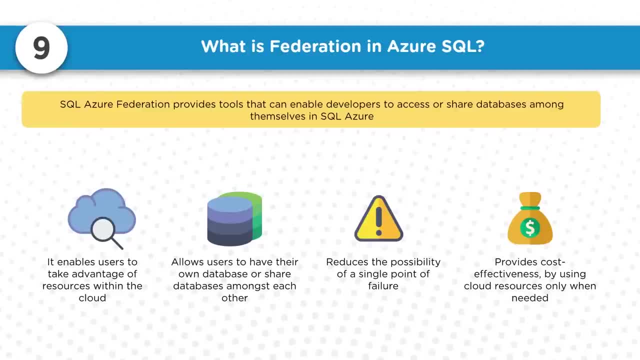 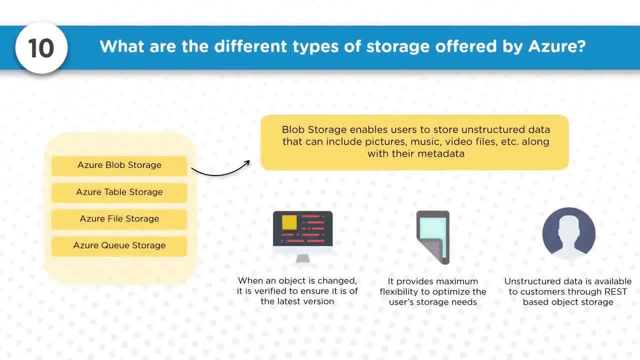 pre-provisioning: no over-provisioning. It provisions the right amount and we pay the right amount. Let's talk about this one: What are the different types of storage offered by Azure? Now, the different types of storage offered by Azure are, as you already know and as you can see, 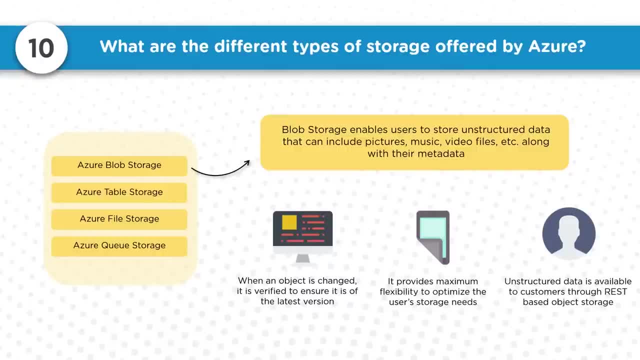 they are Azure blob storages, table storages, file storage and queue storage. So let's expand one after the other. Now, blob storage are nothing but a massive scalable object storage, and that's very good for storing text and binary data. And Azure blob storage is Microsoft's object storage. 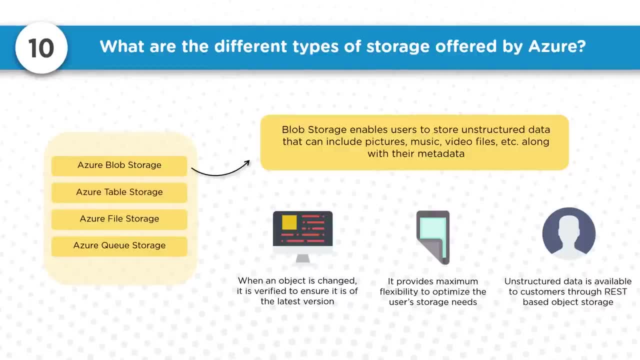 solution for the cloud. A blob storage is optimized for storing massive, massive amount of unstructured data that can be in form of text or in form of binary data. So, in short, blob storage enables users to store unstructured data, And those data can be in the format of pictures, music, video files and a lot more, And it stores. 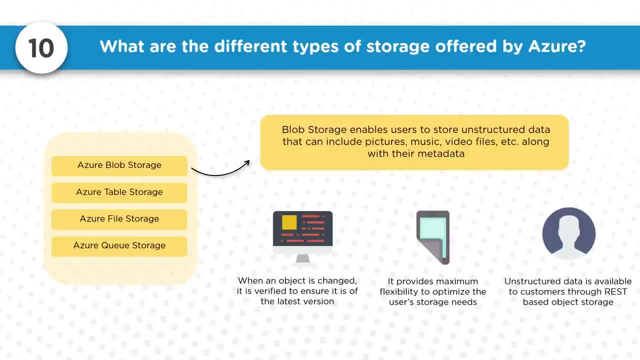 them, along with their metadata. And another advantage or another feature, benefit that we get from blob storage is when an object is changed, it is verified to ensure it is of the latest version. number one And number two: it provides maximum flexibility to optimize the user's storage. 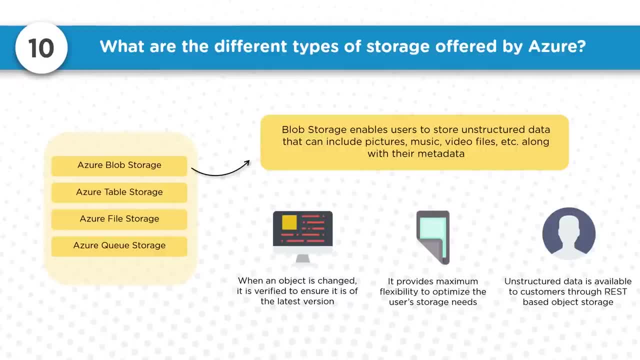 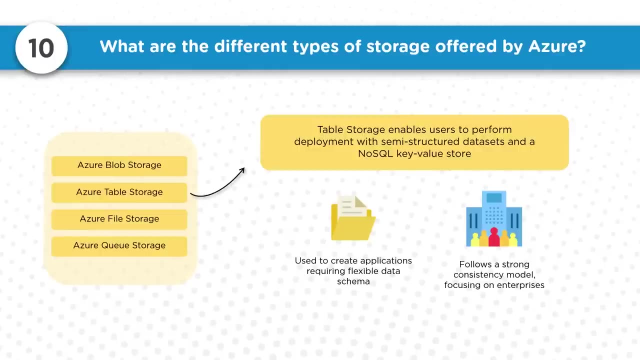 needs, And this unstructured data is available to customers through an URL or an REST-based object, So that's the benefit that comes along with the blob storage. Table storage, on the other hand, is a NoSQL store for schemaless storage of secured data. 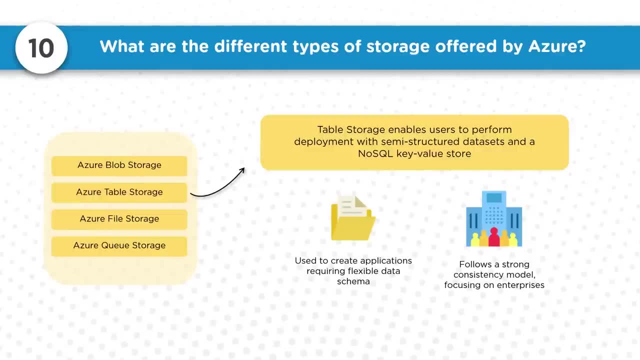 Now, this Azure table storage is a service that stores structured NoSQL data in the cloud And because this table is schemaless, it's very easy to save your data. It's very easy to adapt your data as the need for your application grows, And this table storage is very fast. 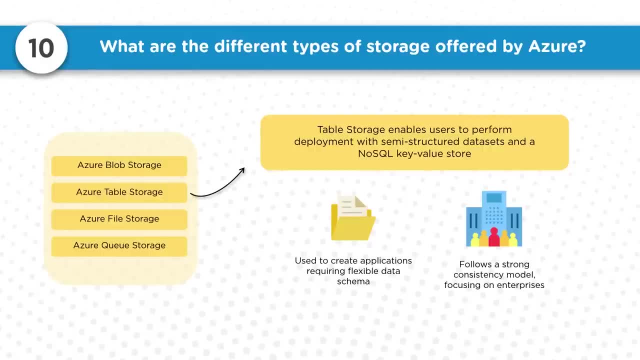 and cost effective for many type of applications. So some of the type of data that we can store is: table storage is good for flexible databases like user data for web applications, address book storage, device information storage And if you want to store metadata, this is a very good use case to store them in Azure. 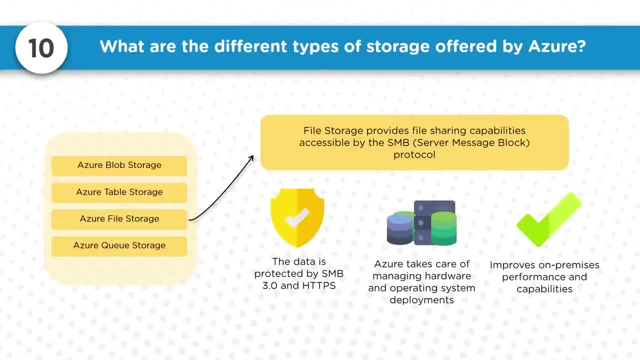 table storage. Azure files is another storage. Here it's a managed file share for cloud or on premises. So file storage provides file sharing capabilities accessible by the server messaging block protocol and this can be accessed from the cloud and this can be accessed from on-premises as well. 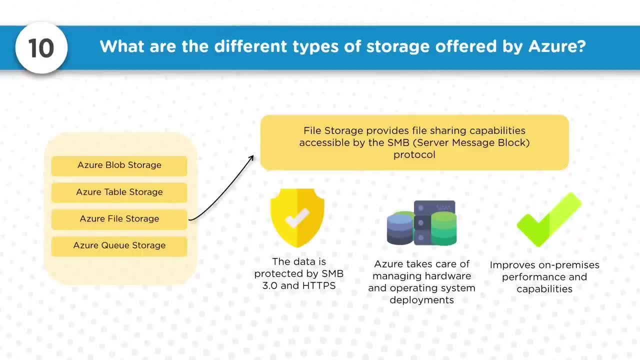 Here in file storage. the data is protected by SMB 3.0 and HTTPS protocols and the more important thing is, Azure takes care of managing hardware and the operating system deployments for Azure file storage. So this additional file storage can be used when we want to burst the storage capacity in on-premises. 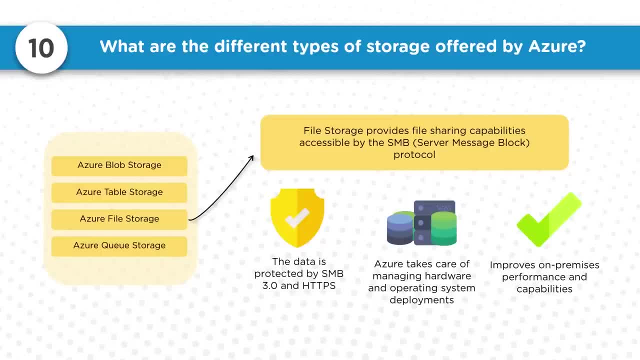 So on-premises the primary, and cloud is the secondary or the extended on-premises storage, So it actually improves the on-premises performance and capabilities for our on-premises data center. And then we have Queues, Azure Queues. 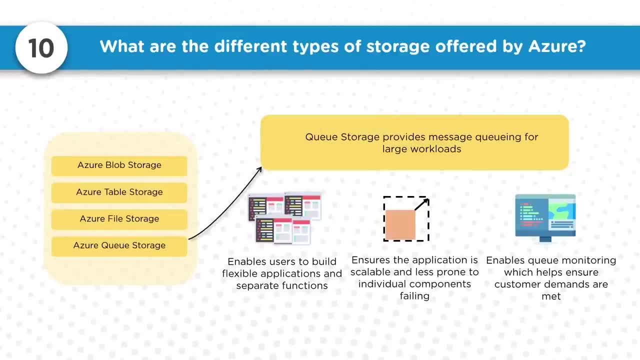 It's a messaging store for reliable messaging between the application components. We spoke a little about this in the previous question. So the Azure Queue storage is a service for storing a large amount of messages that can be accessed from anywhere in the world via HTTP or HTTPS protocol. 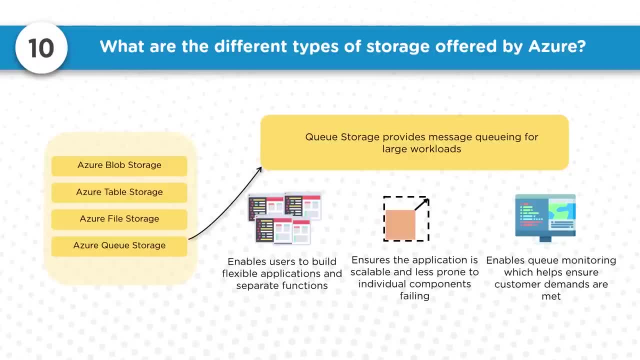 In here. a single message can be up to 64 kilobits in size, and in a queue we can have millions of messages and the limit can actually go up if we have not reached the limit of the storage account. So it's millions and millions of messages. 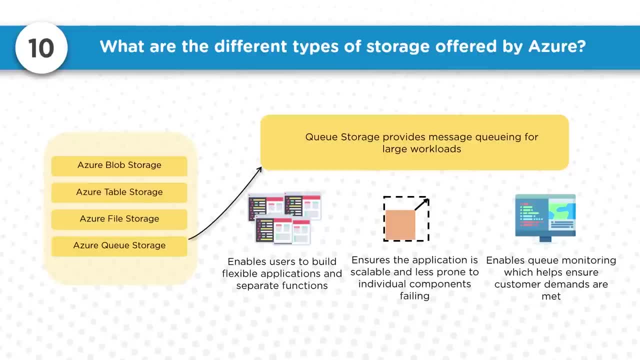 So it's millions and millions of requests that can be stored in the storage queue or the queue storage. So the queue storage, in short, provides message queuing for large workloads and it enables users to build flexible applications and separate the functions one from another. 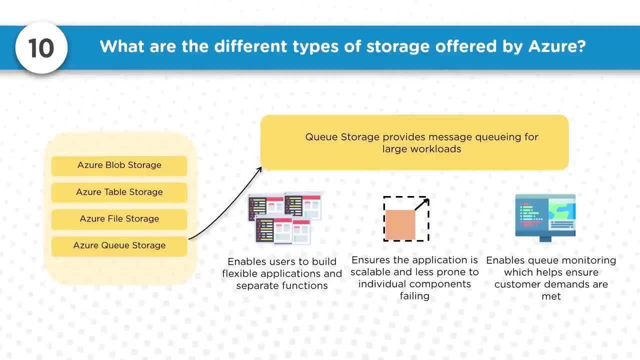 So one failing doesn't affect the other application, which is running healthy, And this queue storage. it ensures the application is scalable and less prone to individual component failures because they are decoupled separate now. It also ensures that the application is scalable and less prone to individual component failures because they are decoupled separate now. 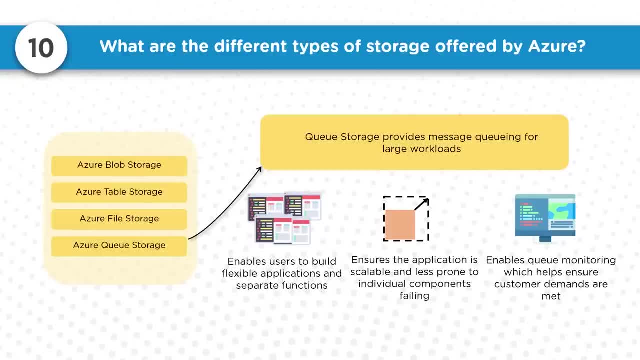 And this queue storage. it ensures the application is scalable and less prone to individual component failures because they are decoupled separate now. It also helps in monitoring the queue, which ensures the customer's demands are met. So queue is a great place to monitor or a great component to monitor. 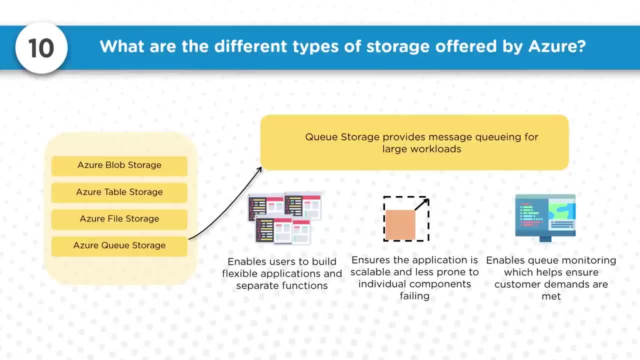 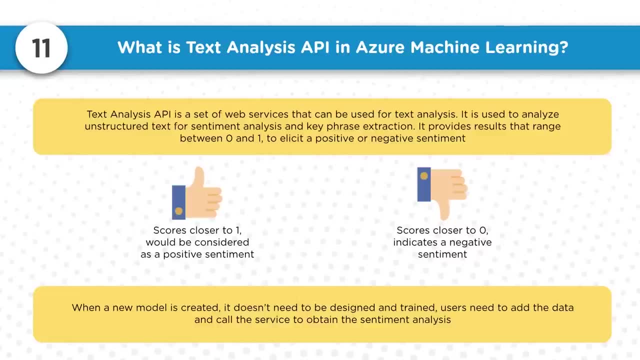 So we understand how much a peak heavy reached for a particular application service or a container. What is text analysis API in Azure machine learning Now? a text analysis actually, and cloud based analytics API, and it provides an advanced natural language processing over the raw text. 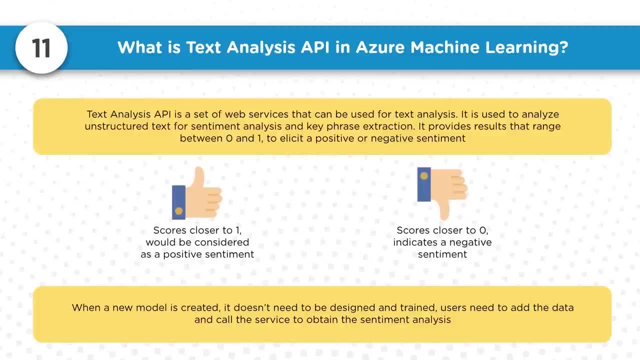 And it provides an advanced natural language processing over the raw text And it has got four main functions like the sentiment analysis and the key phrase analysis, language deduction and a few other things. Now, what do you mean by sentiment analysis? Now, sentiment analysis is from the logs, from the comments, from the text comments that we receive. do an analysis and find out whether that's a positive or a negative statement. 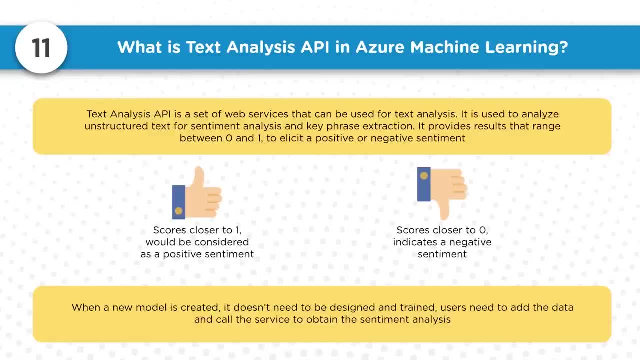 Now, if it is the API, the API returns and sentiment score between zero and one, and one is positive and zero is negative. And then in text analysis we have a key phrase extraction, which is: it will automatically extract the key phrase to quickly identify the main points in that key phrase. 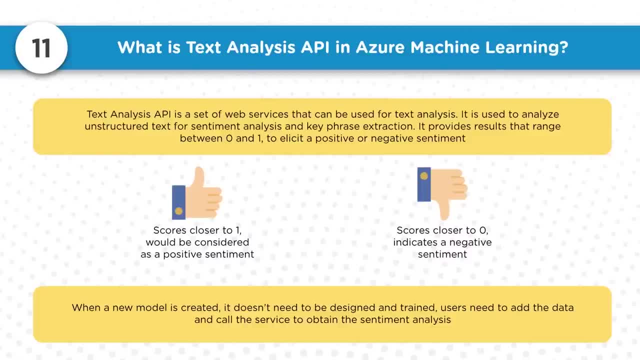 For example, if you're analyzing and text which says the food was delicious and there were wonderful Stuff, then the API returns the main talking points of that phrase, like food. food is the main talking point and wonderful stuff. That was a main talking point. 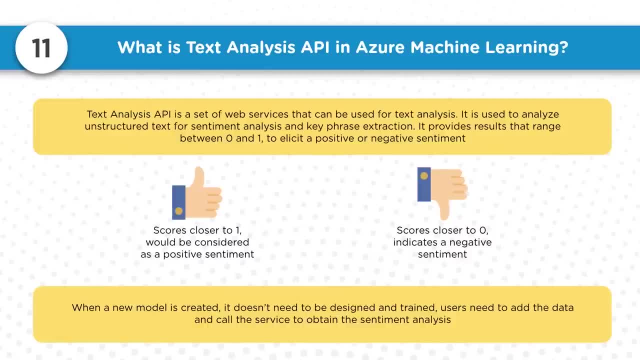 So that's another feature that this text analysis has. And then we have language deduction in text analysis. irrespective of what you paste, It can try to gauge and try to align it to the 120, or up to 120 languages that it supports. 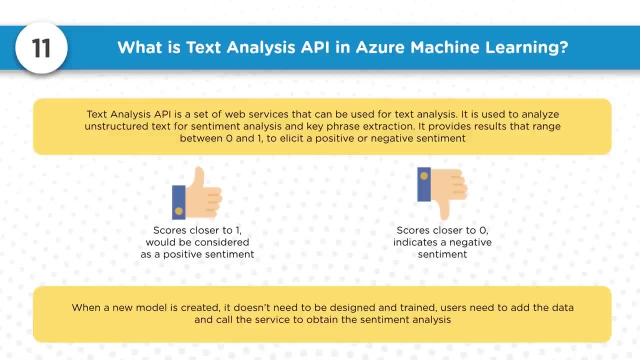 So I can simply Take text from the Internet and I can paste it and text analysis software is going to identify the language and then can run phrase and sentiment analysis on those texts. So, in short, text analysis is an API, a set of Web services that can be used for text analysis. 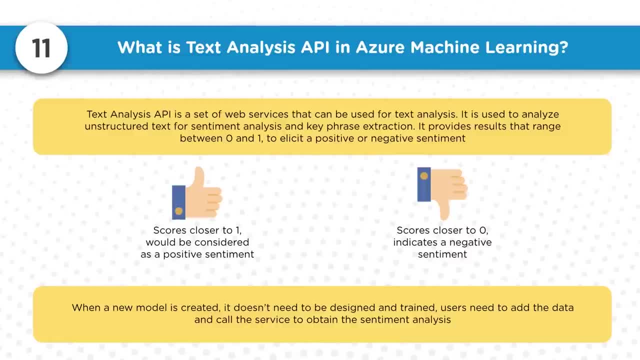 It can be used to analyze unstructured statement, sentiment analysis, key phrase extraction and a lot more, And the results are generally between zero and one, and one being positive and zero B Being the negative sentiment. There is no much training, or in other words, this is not as complicated as a couple of other text analysis softwares are available in the market. 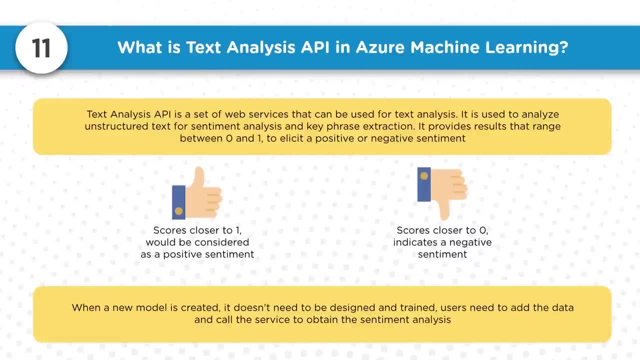 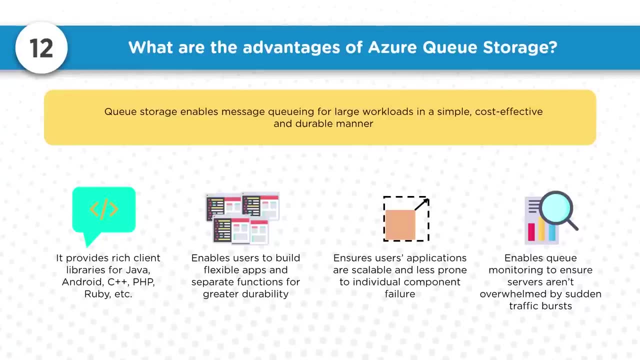 We can simply paste, We can simply upload the text and we can call the service and it runs a sentiment analysis on it. all by itself. Let's look at this question: What are the advantages of Azure Q storage If you're going to work in a development environment, if you're going to work in an environment that embraces DevOps? this could be a question. 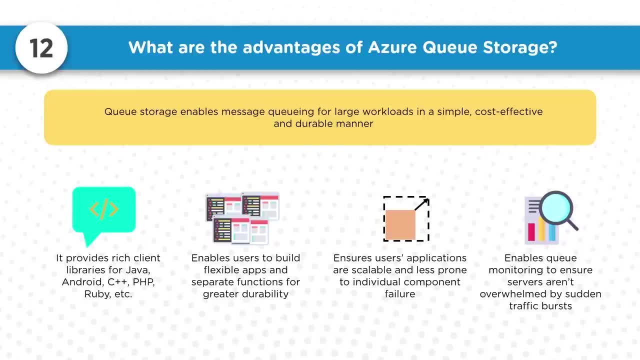 What are the advantages? What are the advantages of Azure Q storage? Now, Azure Q storage is built to flexibly operate the applications and separate the functions between the applications that run large workloads. So when we design applications for scale, these applications can be decoupled so that they can scale independently. 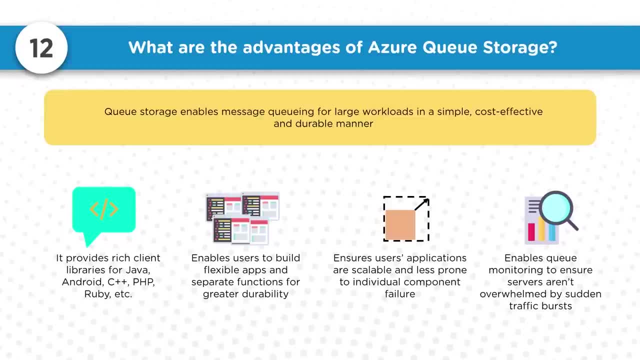 You know, a thing happening on an application is not dependent on another application and anything happens to a section of the application Right The application will not affect the other application because they are now decoupled and connected through the Q storage. So the Q storage gives us asynchronous message queuing for communication between the applications, irrespective of whether they are running in the cloud or whether they are running in desktop, or whether they are running on premises or on mobile devices. 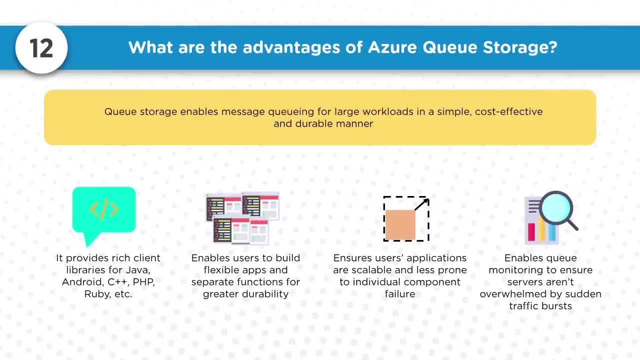 So, in short, this Q storage enables message queuing for large workloads in a simple and cost effective and durable manner. Excellent, talking about the advantages. advantages is it provides rich client libraries for Java, Android, C++, PHP, Ruby and lot other services getting added during every new. 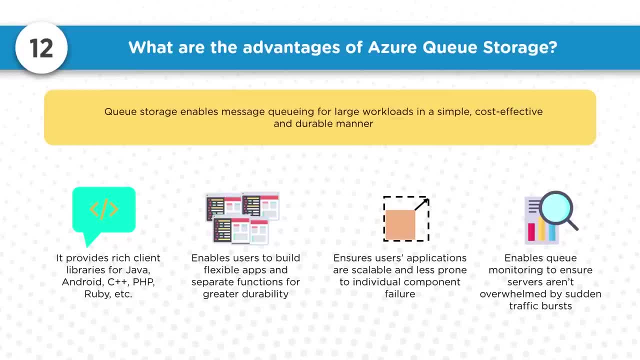 release from Azure and the main advantage again is it enables users to build flexible apps and separate the functions for bigger or greater durability. again, introduction of queues into our application. it ensures our users applications are scalable and less prone to individual component failures, meaning one component failing is not going to take the whole application down. 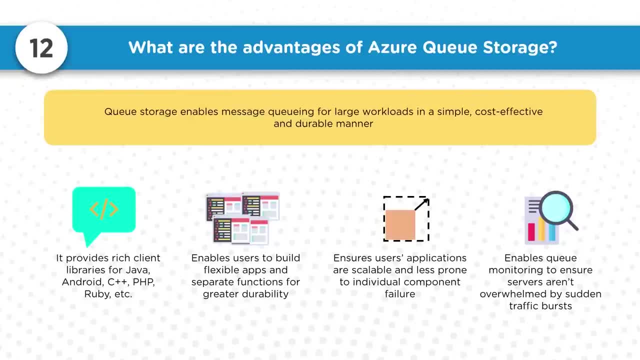 right. if one component fails, it's just that component that stays fails. the rest are healthy and the rest are going to function. it also helps us to monitor the queues and ensure the servers are an overhelmed by sudden traffic, a burst. so how much do we need to do to make sure that the servers are not overhelmed by the? 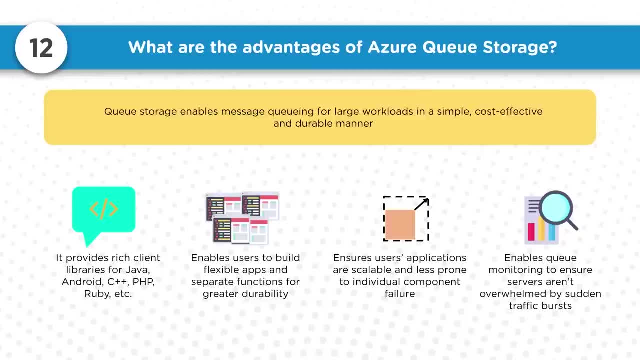 I have in the queue kind of determines the traffic for my application and if the queue is more I can always go and auto scale my environment. and the queue is less, I can always go and shrink or make my environment thinner so it can save cost. and anytime there is more data in the queue I can auto scale monitor. 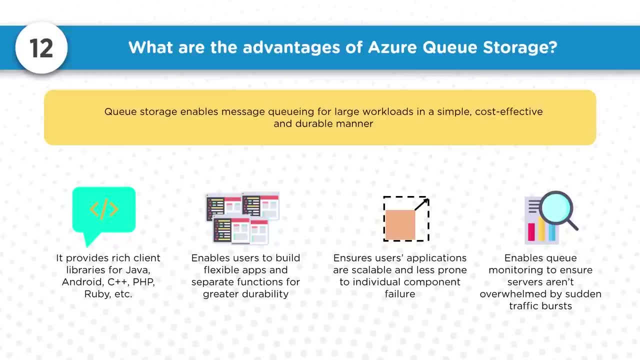 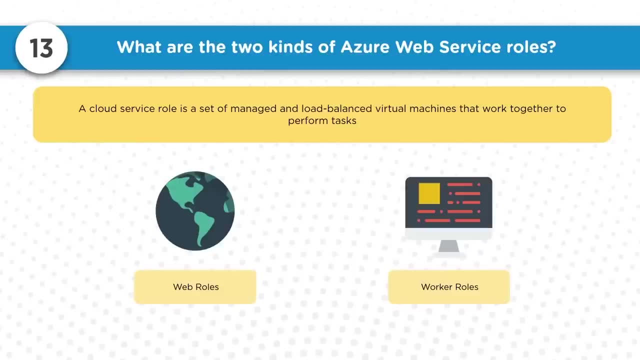 the metric and do auto scaling based on that metric. so the environment knows that there are more data is coming in. I need to expand myself to handle that much money. this is a very common question. what are the two kinds of as your web service roles? now, a service role is a set of managed and load-balanced virtual. 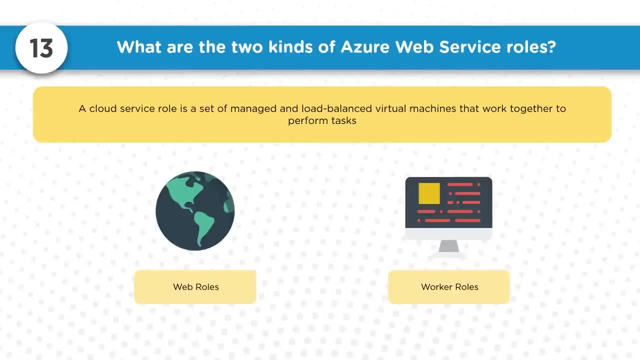 machines that work to perform some tasks and based on what it's going to run on top of it- is it going to run a web service or is it going to run a worker service- defines what kind of roles that gets attached or that goes on this virtual machines. so we have two types: web role and worker roles. the web role: 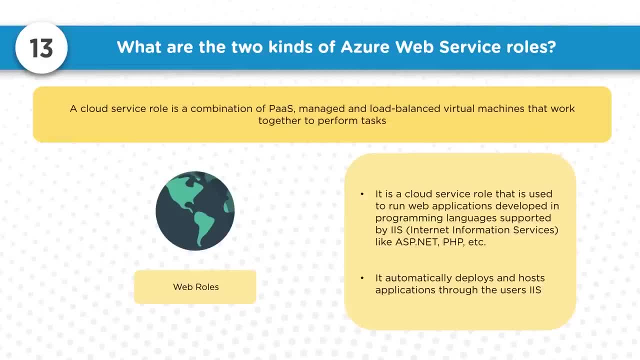 is a cloud service role that's configured to run web applications developed on programming languages technologies and majorly they support IIS internet information service and they support aspnet, PHP, a Windows communication foundation, and so on. so that's web roles and these web roles it. 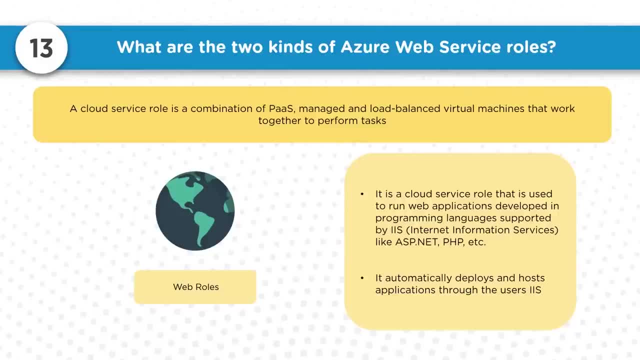 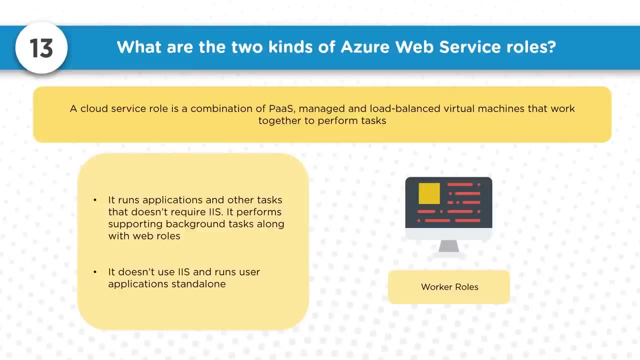 automatically deploys and hosts application through the users IIS internet information service. on the other hand, worker roles are roles that runs applications and service level tasks which generally do not require IIS. so IIS is actually the differentiating factor. so in worker roles IIS is not installed by default. the worker roles are mainly used to 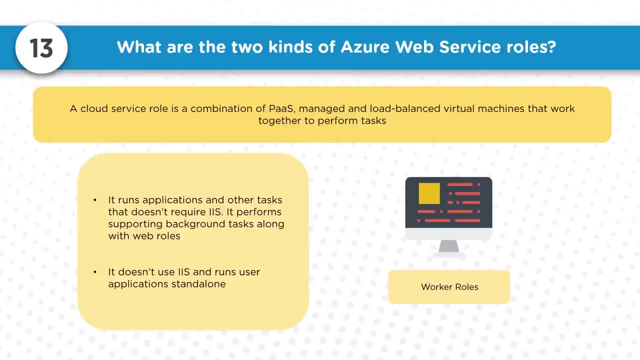 perform supporting background process along with web roles, and do tasks automatically: compressing or uploading the images, running scripts, and are doing some changes in the database, getting new messages from the queue and processing and a lot more. you know the work. the applications are the work that does not require IIS. that's what this worker role does. again, the 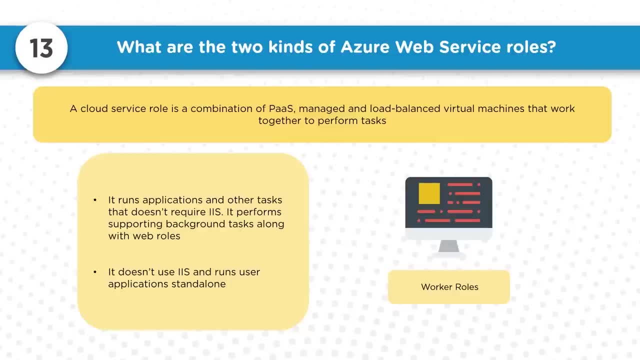 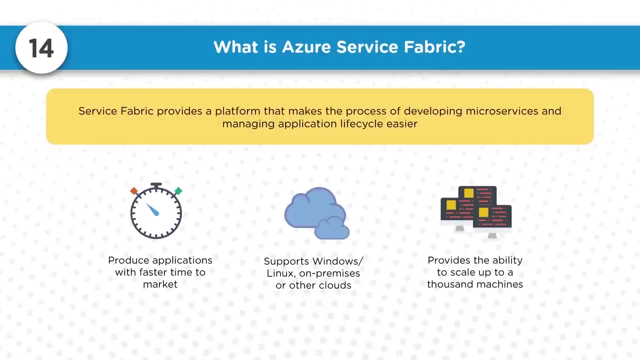 main difference between the web role and the worker role is that the web role automatically deploys and hosts your application through IIS, whereas the worker role does not use IIS and runs our application as standalone. this is another classic question: what is Azure Service Fabric? so Azure Service Fabric. 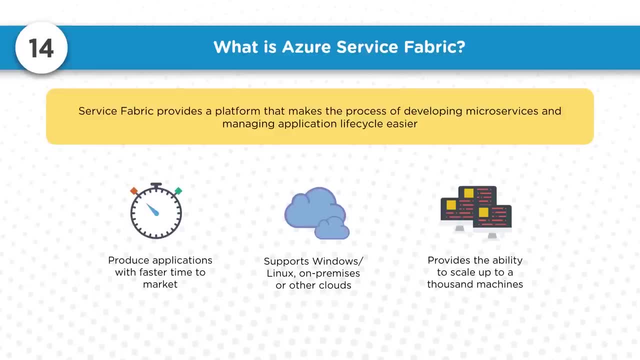 is actually an distribution system platform that makes it easy to pack, deploy and manage a scalable and reliable micro services and containers. now, service fabric also addresses some of the significant challenges in developing and managing cloud native applications, and the problem that it addresses and fixes is now developers. 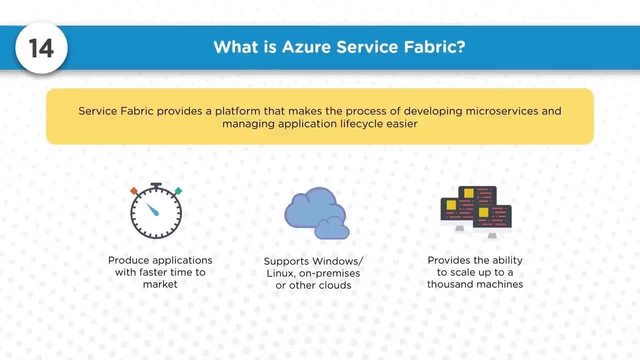 and administrators can avoid complex infrastructure problems and focus on implementing mission critical and demanding workloads that can be scaled and that can be managed through the console or from the single place. in short, service fabric provides a platform that makes the process of developing micro services and managing application lifecycle lot easier, and the advantages 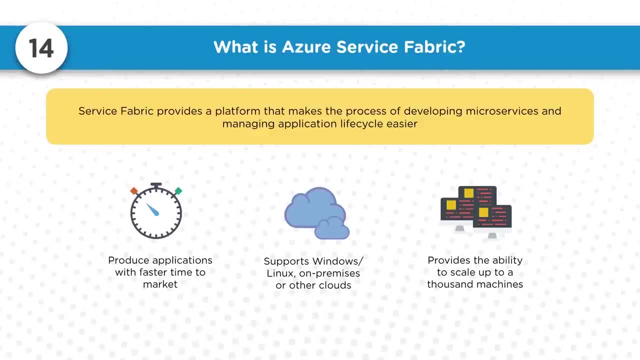 of service fabric is that now we can produce application with faster time to market because all the worry about the infrastructure is taken away from us. we don't have to design an infrastructure. all that we need to worry about is simply the application and the application lifecycle. again, the advantage is it supports Windows. it supports Linux, not 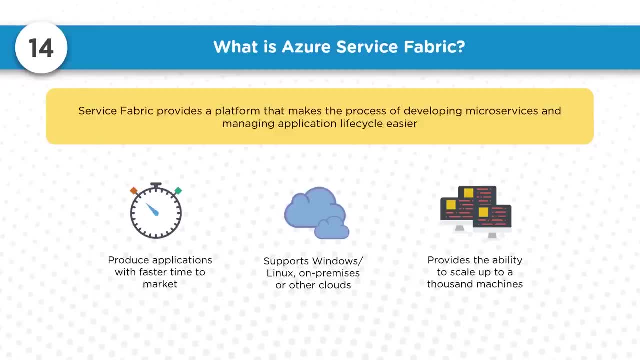 only that, it supports servers on-premises and in the cloud. with service fabric, we can scale up our environment to even thousand machines in just a single command, or if there is a immediate need for thousand machines, I can immediately scale them up to thousand machines. that's possible with. 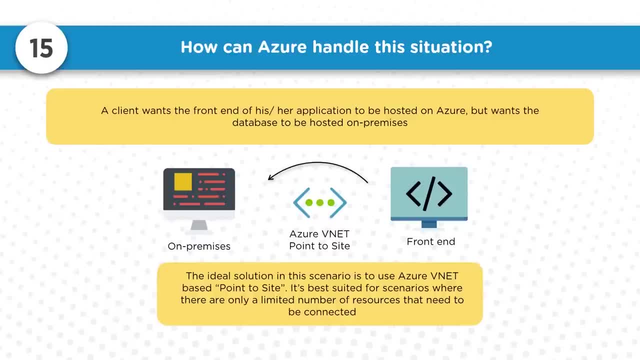 service fabric. now let's look at this question. you can expect this question if the customer is running a secure environment- meaning having some of the applications and on-premises and running some of the applications from the cloud- and for some reason, when classifying the application, that goes to the cloud and that stays on-premises. 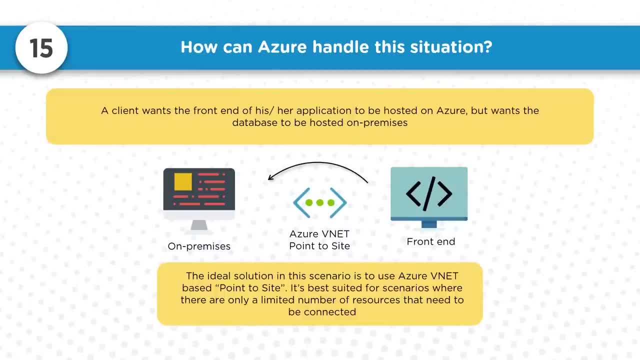 they have decided to keep the database in-house. so in that environment a lot of customers do that. so in that environment, this is a classic and a scenario based question. a client wants the front end of their application to be hosted on Azure in the cloud, and once the database to be hosted in on-premises for security. 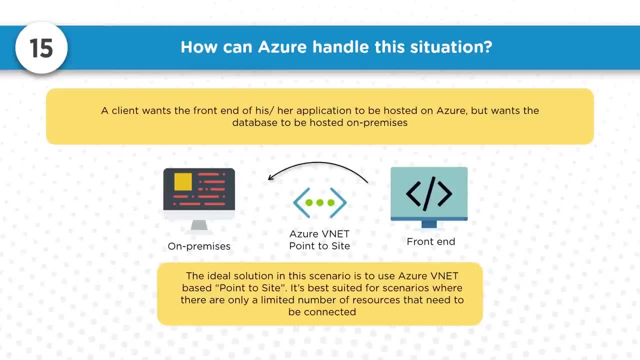 reasons or to have full control on their databases. how do we go about suggesting a solution for this customer? the ideal solution in this scenario is to use the V net based point-to-site VPN solution. so all the front-end applications will be in the cloud and they'll be hosted in a V net and from the V net they'll be. 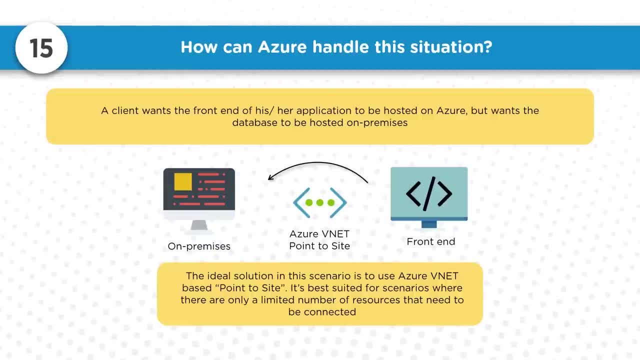 connecting to the database through an point-to-site VPN. so the traffic and the writings and the deeds are not coming through the internet but through a point-to-site VPN link that's connecting the Azure V net and on-premises environment. and this model or this approach or this solution is 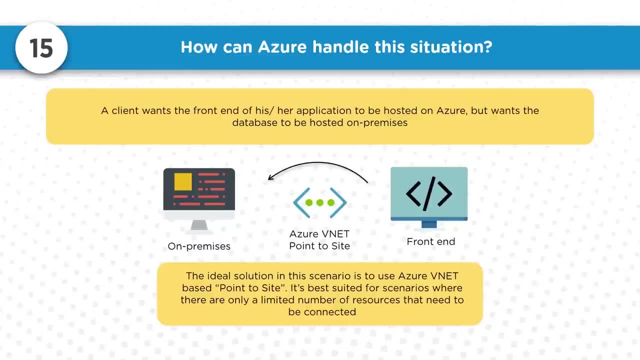 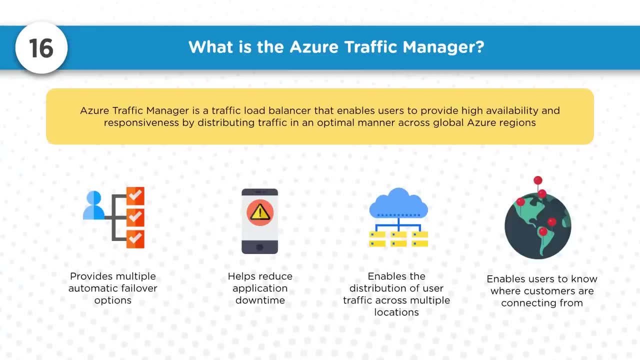 best suited for scenarios where there are only a limited number of resource that needs to be connected between on-premises and the cloud. this is a very common question. what's as your traffic manager? of course, we no more running applications on a single server. we no more running applications on or? 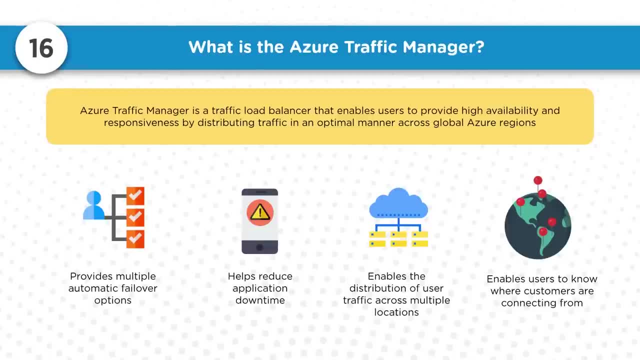 from a single environment. the same application is being run from multiple environments within Azure and we can be running from Azure and on-premise as well, so multiple environments between Azure and on-premises and a lot of customers have such environment and if you are facing an interview with such customer. 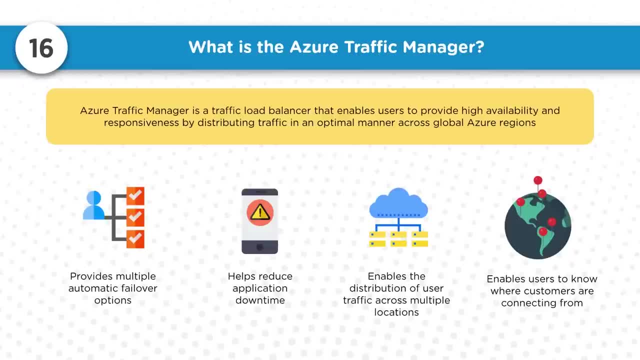 this could be an ideal question. what is as your traffic manager now? the Azure traffic manager is a DNS based traffic load balancer that actually enables us to distribute traffic between services accordingly across Azure global regions, and by doing this, it provides a good availability and a good responsiveness to the application and this traffic. 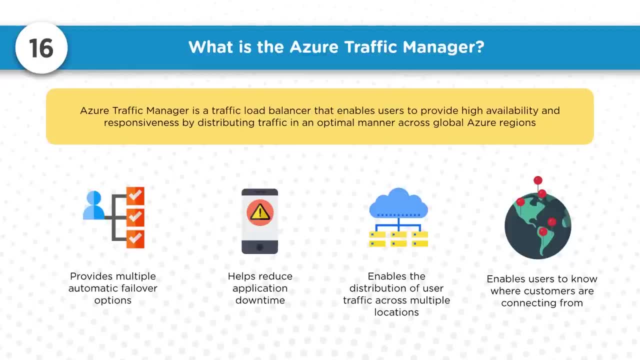 manager. it uses DNS to direct client requests to the most appropriate service endpoint, based on the traffic routing logic and the health of the endpoints that it maintains. so, in short, this traffic manager is a load balancer that enables users to provide high availability and responsiveness by distributing traffic in an optimal manner across the Azure when we run the 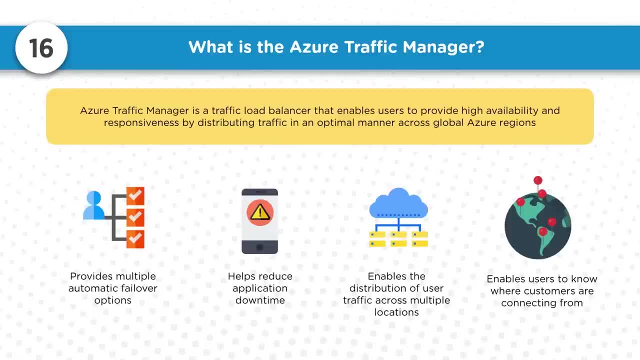 same application in different regions. so some of the advantages or some of the use cases of using as your traffic manager is: it provides multiple automatic failover options. it also helps with reduced downtime. it also helps with the distribution of user traffic across multiple locations, so one location is. 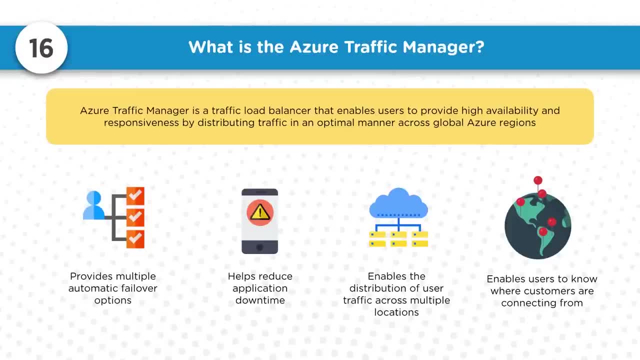 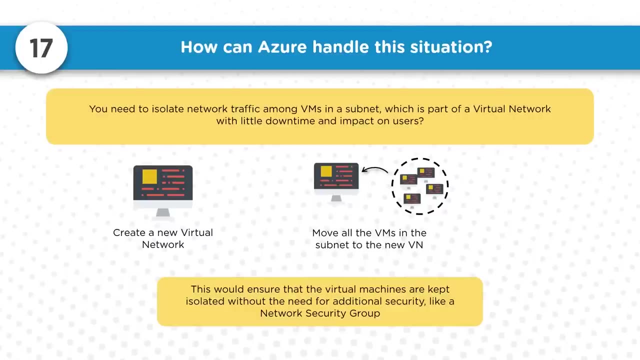 not overloaded, and then it helps with users knowing from where our customers are getting connected from. that's another big use case with Azure traffic manager. let's look at this question right. this is an ideal question. now there are a group of servers connected together within an virtual network and 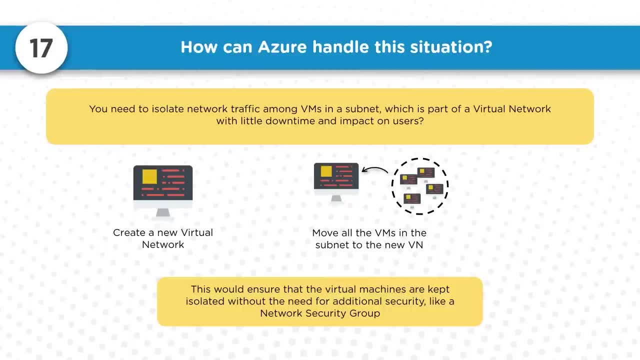 now we need to move them or create a separation between them. how do you go about achieving it? so the question goes like this: you need to isolate network traffic among VMs in a subnet which is part of a virtual network, with little downtime and impact on the user. so that's the 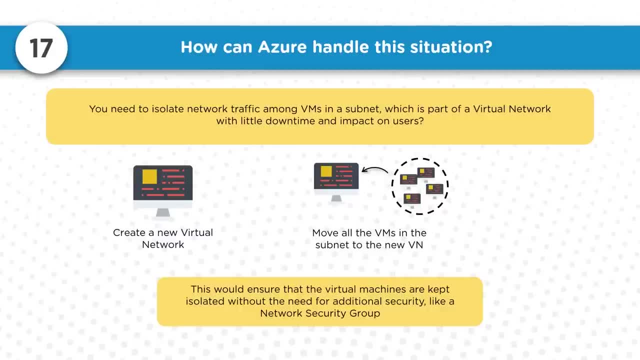 given scenario and the best way we can do it is create a new virtual network and move all the VMs in that subnet to the new virtual network. now this feature is not possible with a lot of other cloud service providers like AWS and a lot of other providers. now in those environments we might need to shut down. 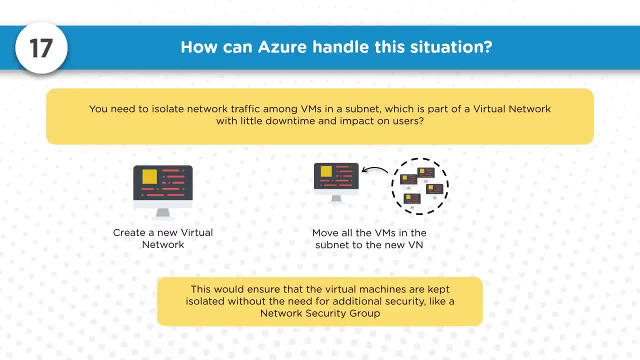 we might need to stop the VM, create a new VM based on the image, and it's an hefty process. but here in Azure I can simply move the VMs from one subnet to another virtual network without needing for any additional security. like the network security group, I can simply isolate them. 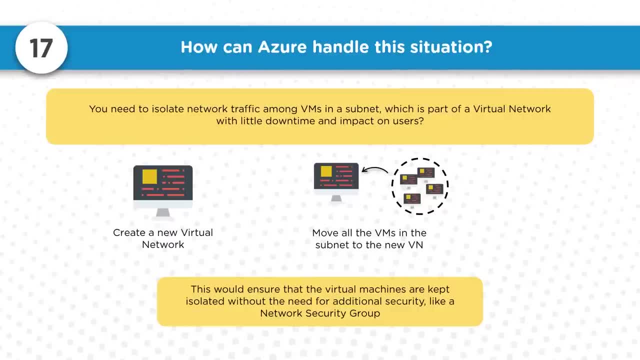 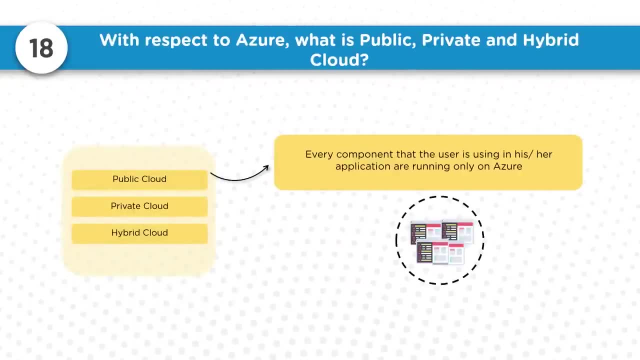 if I need to, by creating a simple, a new virtual network and moving the servers to the new virtual network. look at this one. this is another common question with respect to Azure: what is public, private and hybrid cloud? so this is really to test how well have you understood the different cloud offerings in the market. 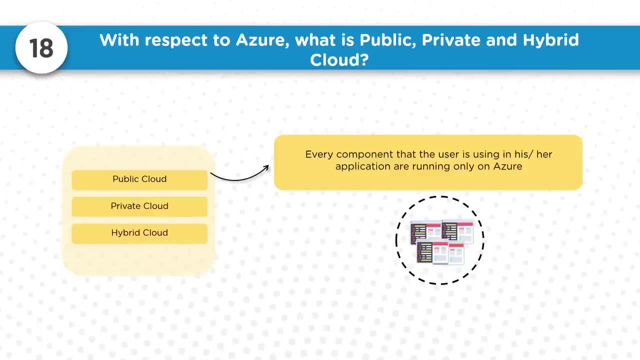 and hybrid, or at least three basic offerings in the market: public, private and hybrid cloud. now, the public cloud is the most common way of deploying cloud computing applications and it has resources like servers, storage, and are owned and operated by third-party cloud service providers like Microsoft Azure. 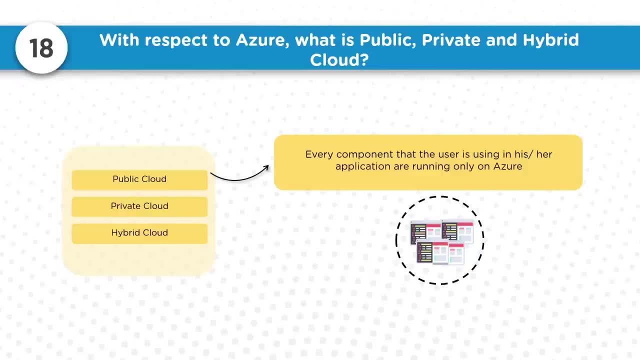 Microsoft Azure is a very good example of public cloud, so here every component that the user is using is running only on Azure. that's public cloud. let me talk to you about some of the advantages of public cloud. some of the advantages is low cost, because there is no need to purchase hardware or software and we pay. 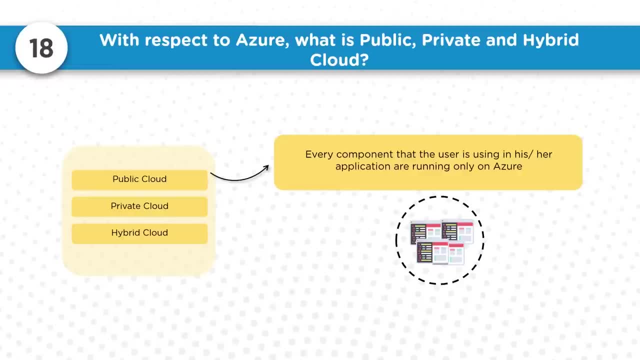 only for the services that we use in public cloud and there is literally no maintenance because the service provider maintains the environment for us and with public cloud we have nearly unlimited scalability, meaning we can get resources on on demand and can meet our business requirements on demand and the public. 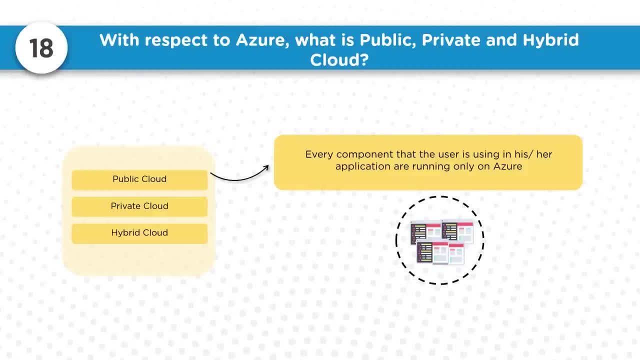 clouds are very highly reliable because they have a vast network of servers and they ensure that our application does not fail. so there are some advantages of public cloud. let's talk about private cloud now. private cloud consists of compute resources used extensively by one business or one organization. now 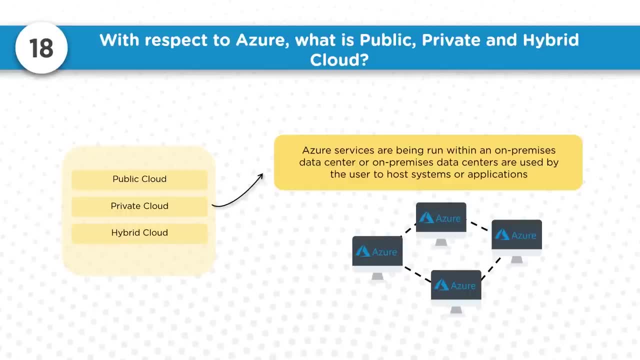 this private cloud can be physically located at our organizations on site data center, or it can be hosted by a third-party service provider. whichever the case, the private cloud, services and infrastructure are always maintained on a private network and they're maintained on hardware and software that are 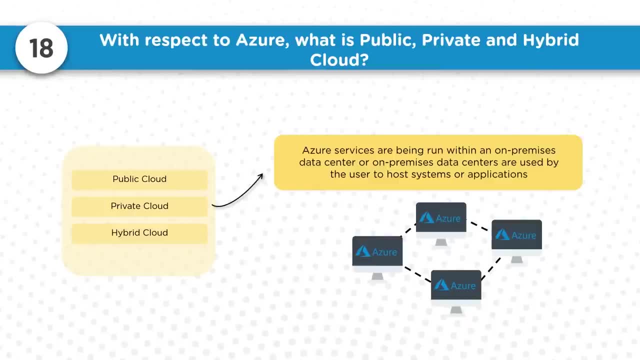 dedicated solely for one organization or solely for your organization. so, in short, private cloud in azure is azure services being run within an on-premises data center or on-premises data center used by the user to host systems or applications. and some of the advantages, some of 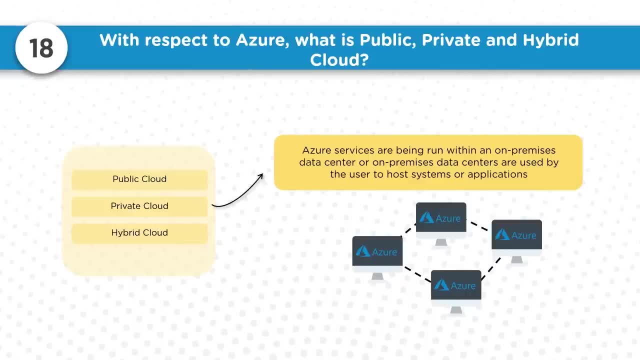 the advantages is it gives more security. resources are not shared with others, so a higher level of control and security over our resource and application is possible. and then we have a hybrid cloud. now, hybrid cloud is the best of both worlds. it combines the features of both public and private cloud and some of the user. 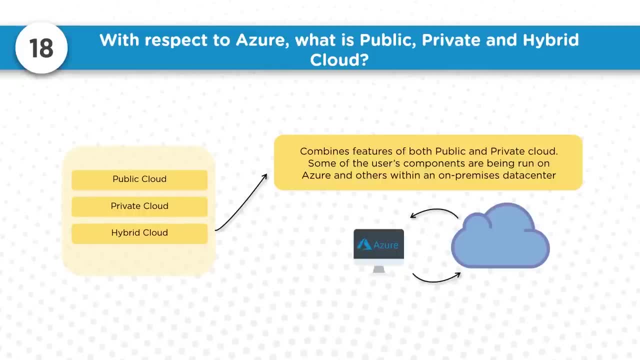 components are being run on azure and others within on-premises data center, so they kind of share the resources. in other words, they kind of share the application. half of the application would be running in on-premises and half of them would be in the cloud and they would be working in harmony to support. 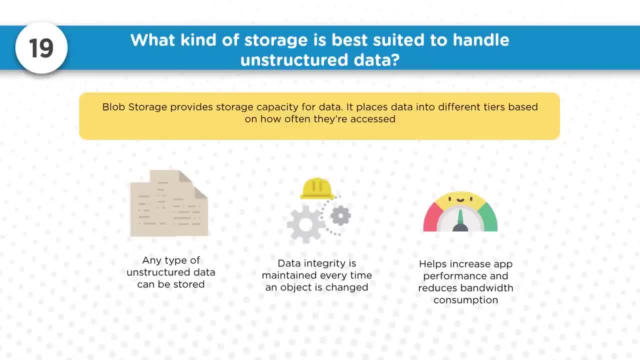 the application and the business need. so that's hybrid cloud. this is one another good example question that wants to test how well you pick services, or how well have you understood the azure products and services and are picking the right service for the need. so the question would go like this: what kind of 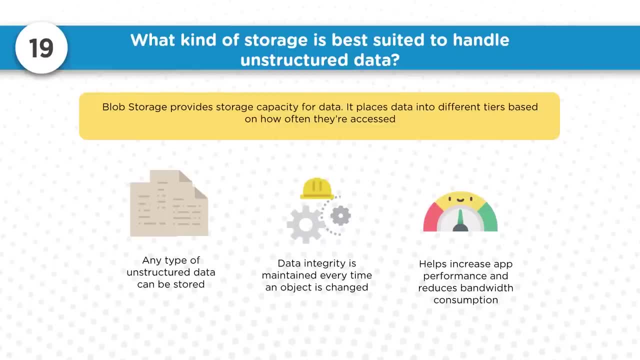 storage is best suited to handle unstructured data. there are a lot of storage options available, and the requirement here is: what or which one would you choose for unstructured data? the answer for that question is blob storage, because blob storage is designed to support unstructured data. it works. 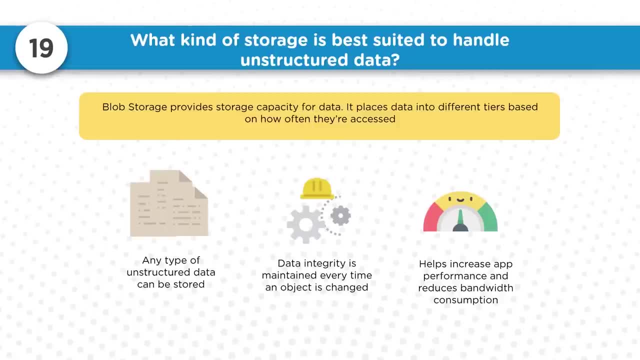 in this way, it places the data into different tiers based on how often they are accessed. different tier means different performance. different performance means different cost associated with it, so a lot of add-on advantages will we get when we use blob storage for unstructured data. in addition to it, any type of unstructured data can be stored in blob storage. this. 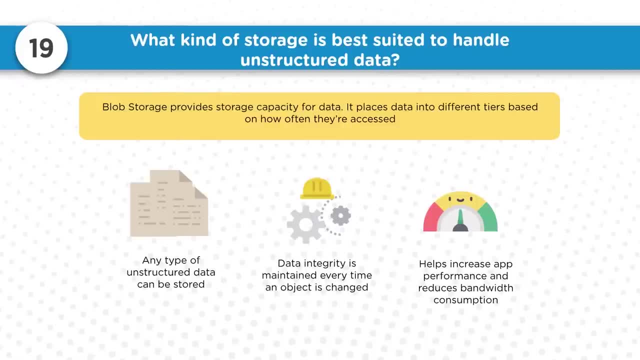 is not true with a couple of other storage options that we have in azure. only with blob storage we can store any type of unstructured data and the data integrity is maintained every time and whenever you do that. this is how it is done. object is changed in the blob storage and the best part is the blob storage helps increase. 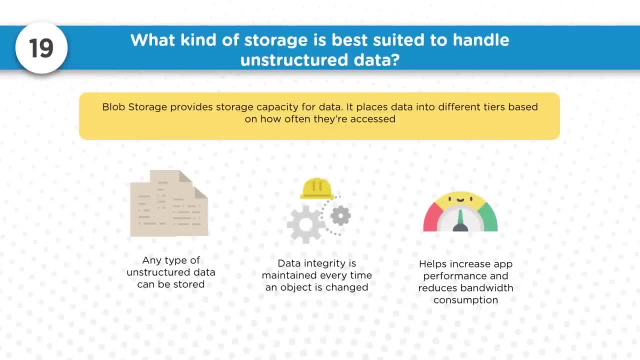 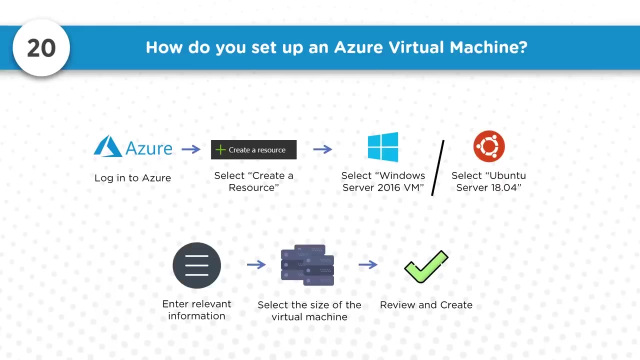 applications performance and reduces the bandwidth consumption and reduces the bandwidth consumption for that application. so they are the benefits that we get, for block storage and blob storage are the ones that are well suited for unstructured data, and that's what your answer should be. it's really an five-step process and if you have worked and if we have done some labs, some basic 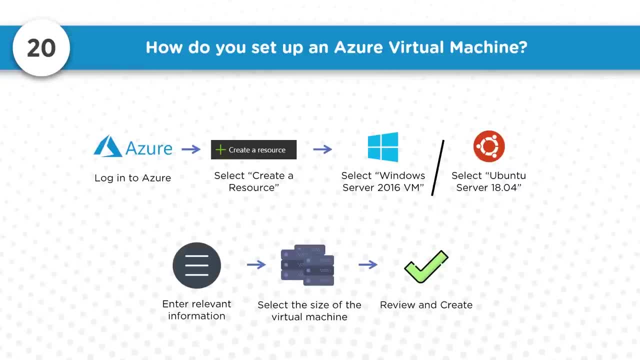 labs. with azure, you can easily answer this question. so it's a five-step process. first step is to log into the azure. the second one is to create an resource, a resource or a resource manager, and within the resource manager you would be selecting the resource and then pick the. 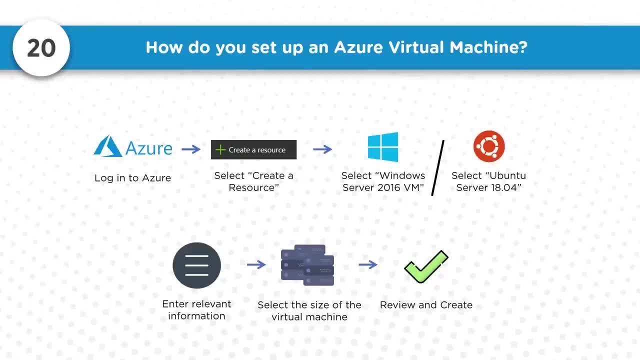 operating system. do you want windows or linux? and within windows, what's the flavor you want, or within linux, what's the flavor you want? to decide on it. and then entering the relevant information. relevant information like the name of the instance or the vm that we're going to launch and the password, the url that goes with it, and 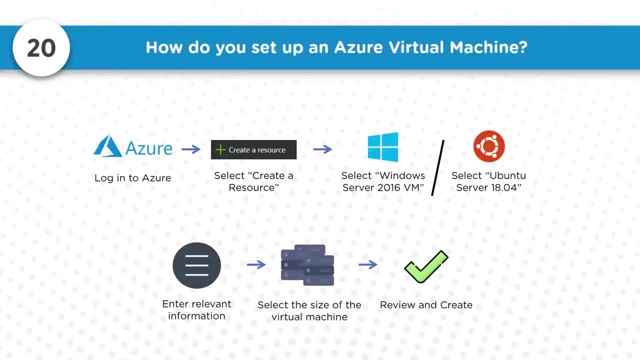 a couple of other relevant information. that goes, gets itself attached with the vm and then select the size of the virtual machine: different size, different types available for the kind of application and for the intensity of the application that will be running on top of it. so select the virtual, select the size of the virtual machine, review everything, whether they're good or 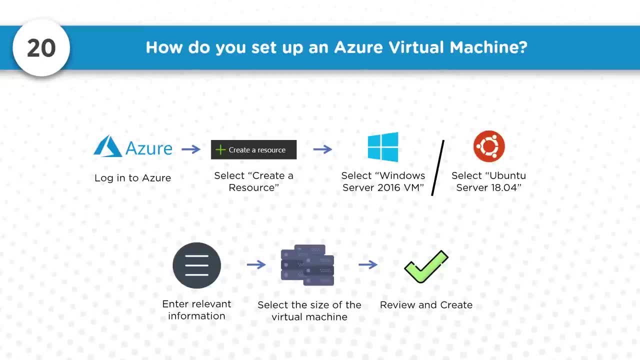 not if there are any changes required. go back and see if you need to set up a virtual machine and then edit them and then come back and launch and your vm is there for you to start working within like three or four minutes, not even five minutes- within three or four minutes it gets ready and you can start working on it. so it's a quick and 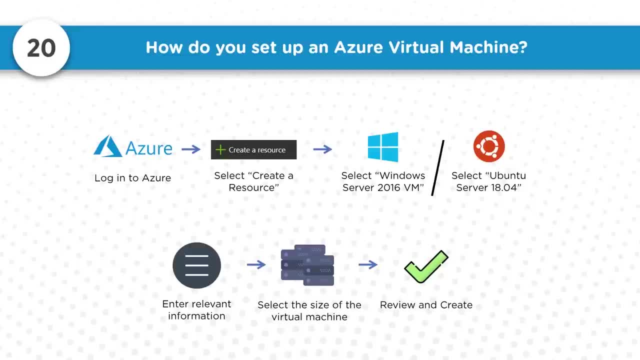 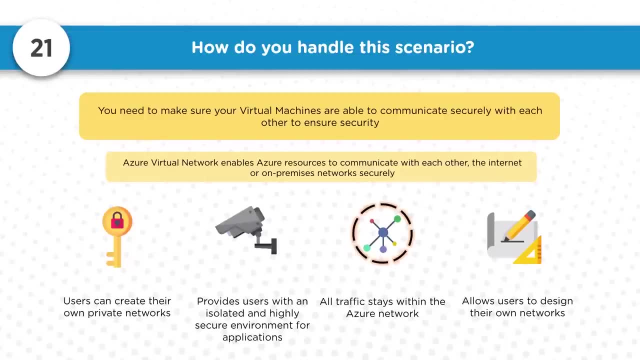 it's a five step process and you should be able to answer it easily if you have done few labs in azure. let's now look at some scenario based question. you've been posed with a scenario, so we thought through it and we picked some common scenario based questions that are being asked and 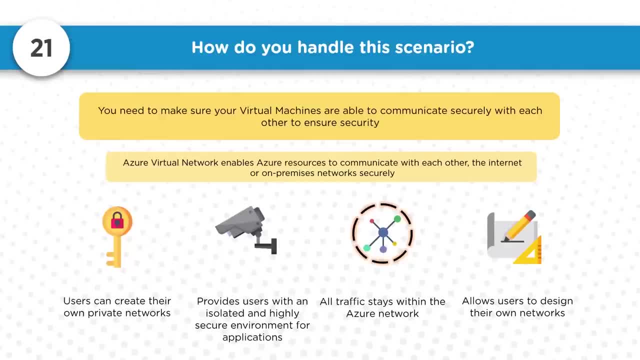 interview and I thought we'll present it for you with answers, with explanation, so you can get benefited through it. So let's look at this question. You're asked to make sure your virtual machines are able to communicate securely with each other, to ensure security or to have good 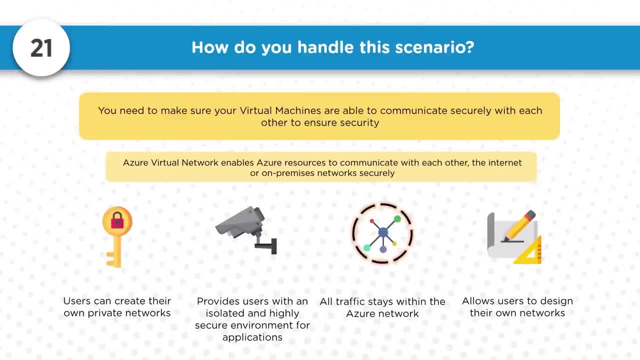 amount of security. What would you do? And the correct and the best answer for this would be using virtual network in Azure, which enables us to communicate with the internet securely, which enables us to communicate with the on-premises data center in a secure fashion. 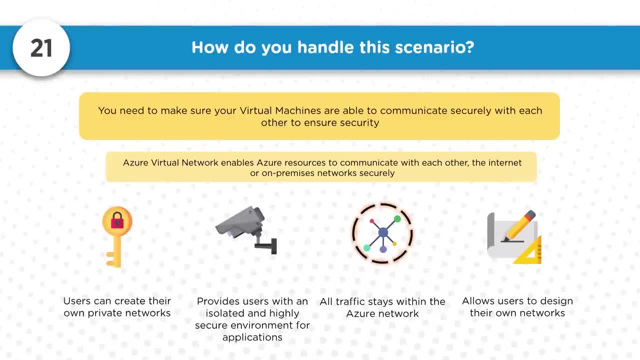 So the advantage of using virtual network is users can create their own private network. Users can pick their own private IP ranges. Users can create their own subnet. Users can create their own routing between those two subnets. A lot more goes into that virtual network, So it's very 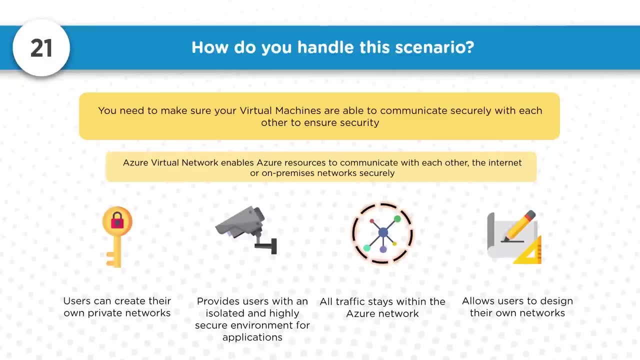 customizable and the users are provided with an isolated and high-resolution virtual network. So it's very customizable and the users are provided with an highly secure environment for applications. It's completely isolated from other customers. It's completely isolated from other applications that are running in other virtual network that we own. 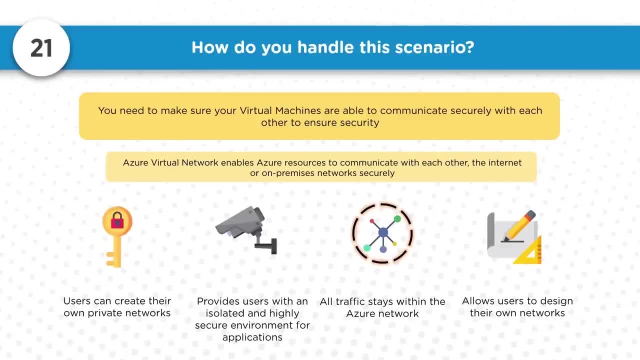 So within our account we can have multiple virtual networks and one application running on a virtual machine is completely isolated from other applications running on other virtual machines And of course, all traffic stays within the Azure virtual machine or within the Azure network, depending you set up the routing. if you have set up a routing to go or reach the internet, it's going. 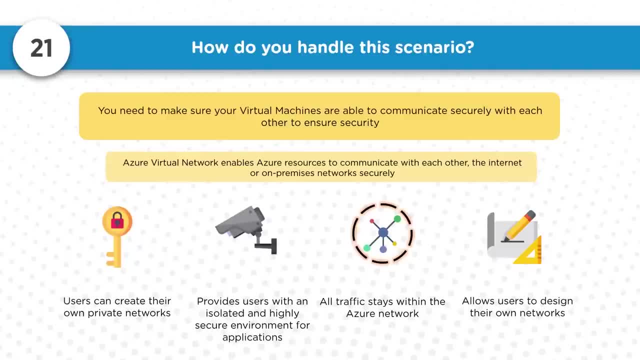 to go, otherwise it's going to stay within azure. if you have set up routing to reach on-premises, then it's going to go and reach on-premises. otherwise it's not going to go and reach on-premises, it's going to stay within the azure, and it also allows users to design their own. 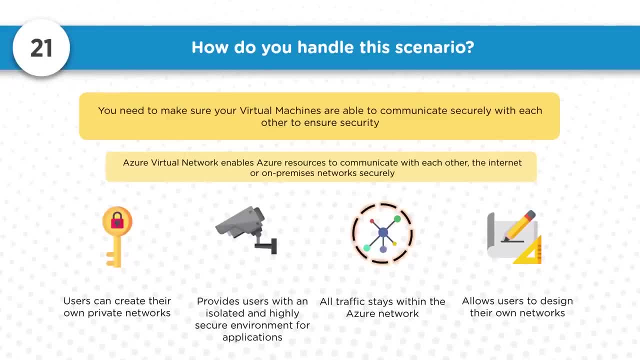 network, like we already discussed: picking up ips, picking routing, you know, picking subnets, you know how many servers should be present in that particular subnet or how many servers should that subnet accommodate. the size of the subnet, the ip ranges, the natting, the masking of ips, creating of vpn- all that's possible with the virtual network so it really allows users to. 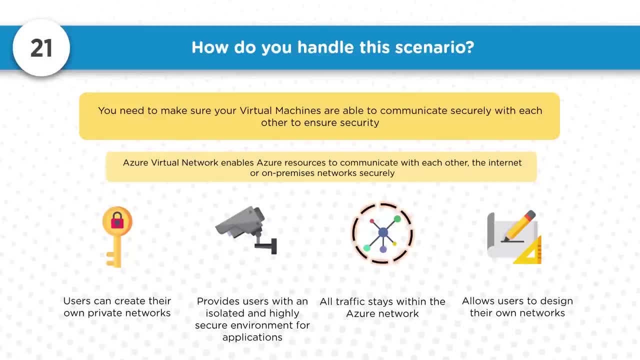 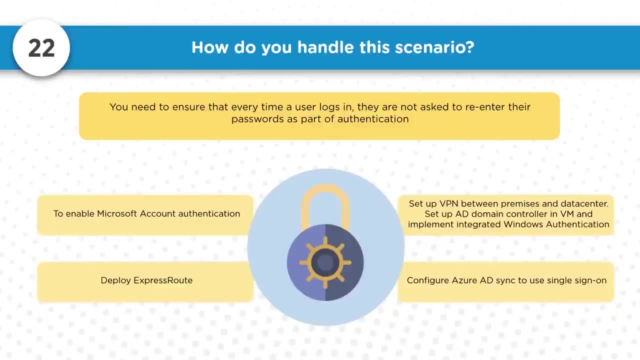 design their own network and using virtual machine is how we secure applications in the cloud. let's look at this other scenario. how do you ensure that every time a user logs in, they are not asked to re-enter the password as part of authentication? so you really don't want. 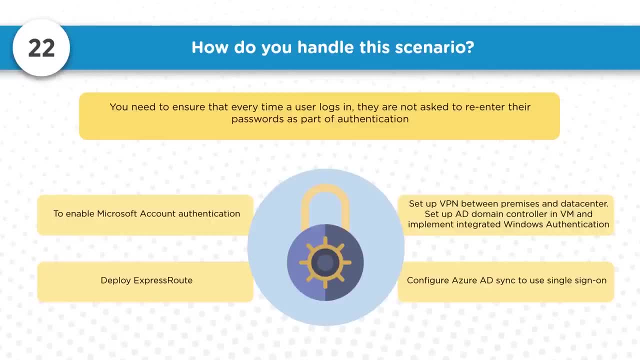 your users to re-enter the password every time they log in to a different application. well, all the applications have their authentication mechanism in place. all of them wants to authenticate the user before they log in. ensuring the user does not log in every time does not mean that no wiping away all the authentication and authorization that's present in that application. 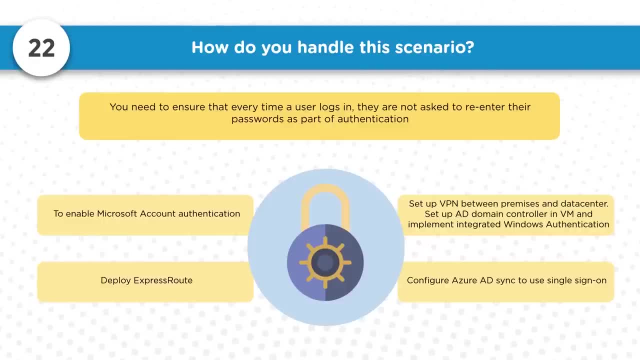 you still need that in place. but how do you make the user hassle free so they're not asked to re-enter the password or the same password again and again? let's look at the options available. the first one is to enable microsoft account authentication. well, it's not going to fix, because with that the user will still need to. 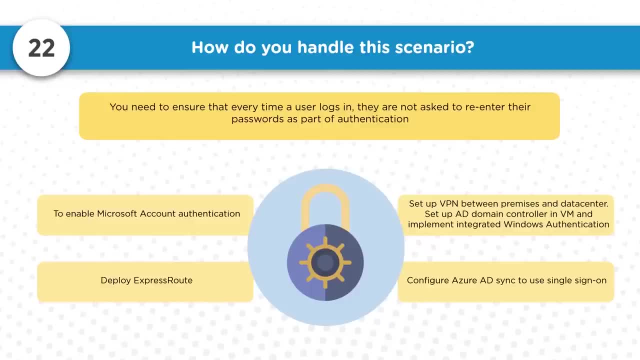 re-enter the username and password, deploy express route. it's not going to fix either, because express route is a network level service that connects on-premises to the cloud. so that has got nothing to do with prompting or otherwise. but it's going to be very important to be able to connect with the cloud. so that has got nothing to do with prompting or 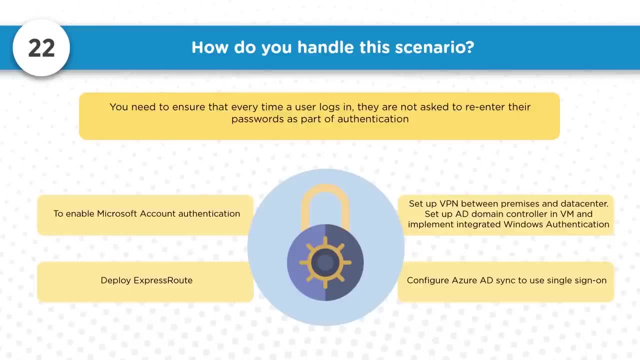 not prompting for password. and then we have set up VPN between on-premises data center and Azure, set up AD domain controller in VM and implement integrated Windows authentication. well, you can use the same username and password for on-premises and the cloud, but this setup the VPN and the AD. 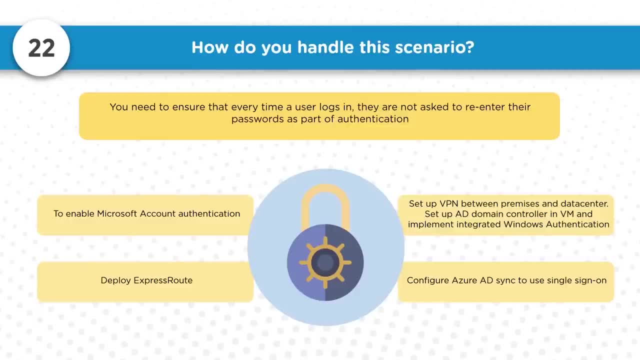 controller setup, it's not going to stop you asking for repetitive passwords. so this is all about using the same password in on-premises and in the cloud, and this has got nothing to do with not prompting the user to re-enter the password. all right, that's same password is different from not prompting the user. 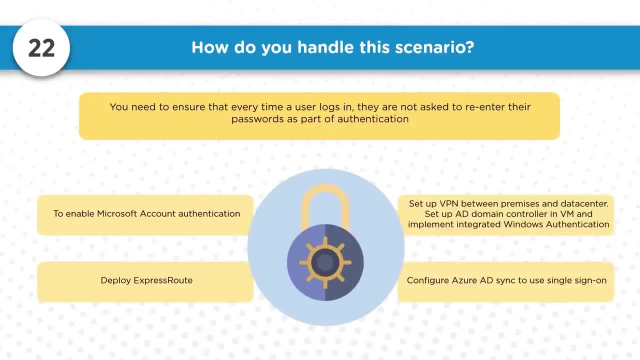 to re-enter the password. they are two different scenarios, so that is also out of the equation. and the last one is configure AD sync to use single sign-on. that's the right one. so when we configure the AD to use single sign-on, you can configure AD to use single sign-on. you can configure AD to use single sign-on. 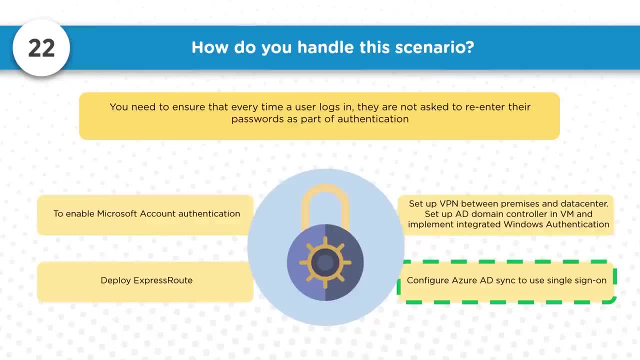 then it's going. it's not going to ask for the username and password every time we access an application because we have logged in and that login is gonna stay active for like 24 hours or so, depending on how you configure it, and within that time you can access a lot of other applications and it's not gonna ask for. 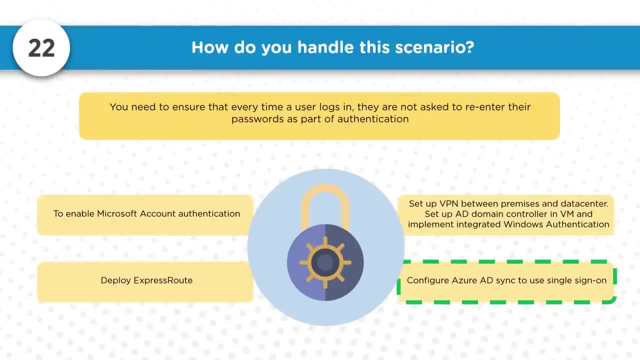 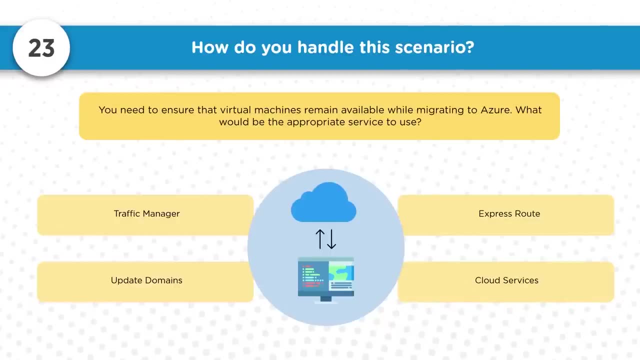 the username and password, because you already have a single signed on and you have signed in using the right credentials. let's look at this one. you need to ensure that virtual machines remain available while migrating to Azure. what would be the appropriate service to use? let's look at the options. 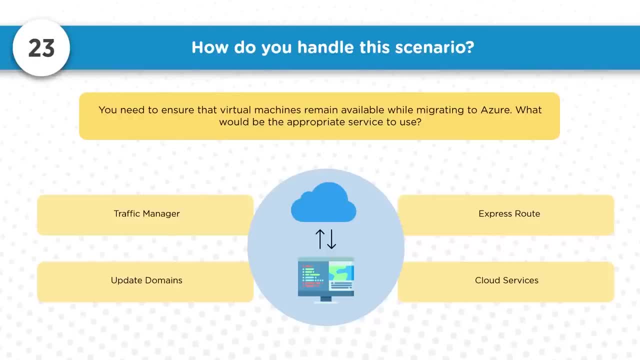 traffic manager. traffic manager is is literally a DNS service. and then let's look at the other one: update domains. it again has to do with traffic manager updating the URL. so now the traffic manager gets updated and then starts sending requests to that particular URL. it's gonna take some downtime because 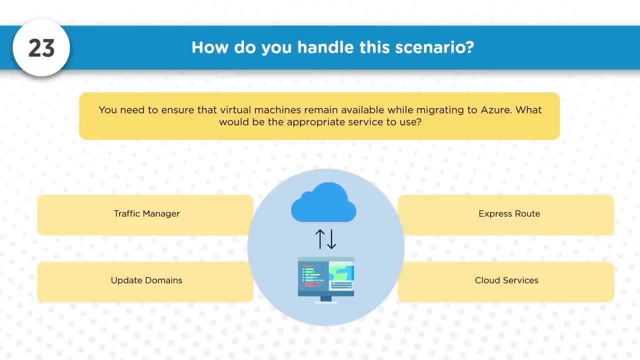 when we update the URL, they will have to be populated to all different places and and it takes time. so within that time any user trying to access it's going to fail. and then we have express route and cloud services. express route could be the. in fact, it's the right answer. 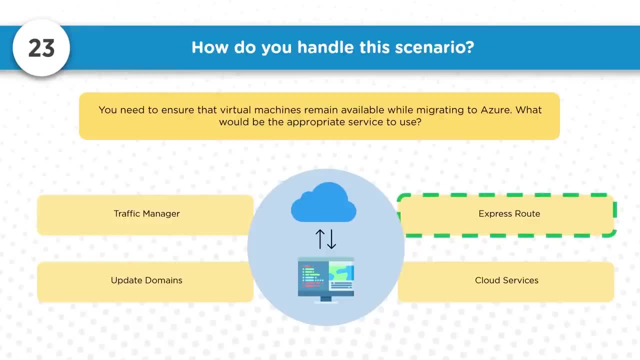 because express route, it's an extension of our on-premises and cloud environment and in this question it really comes out from a customer who's having an hybrid environment. so they have applications running in on-premises, they have applications running in the cloud and they want. 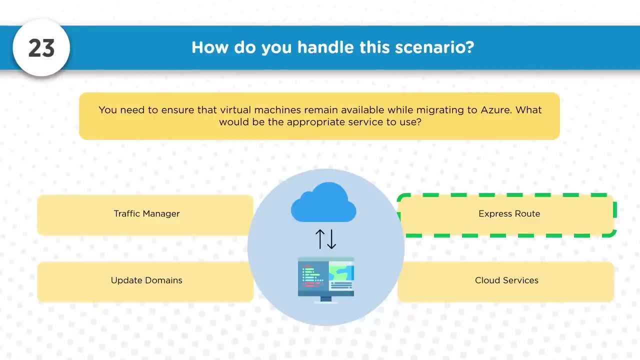 to have a way to migrate applications from on-premises to the cloud. in other words, kind of do a cutover between on-premises and the cloud, and this express route is a service that connects between on-premises and the cloud. so when you do the cutover, the traffic is now sent to the cloud. 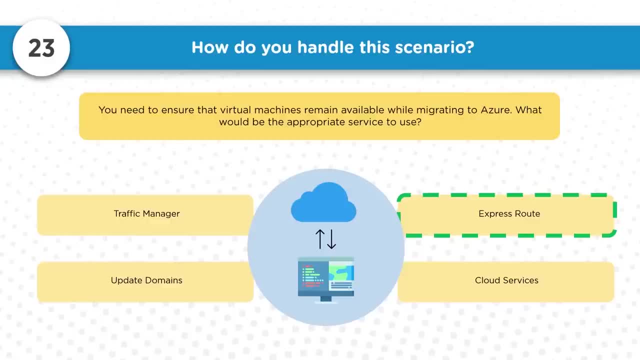 instead of being handled in on-premises. in fact, the services and the application is getting down- are getting shut down in on-premises, so the request will come in the same pattern. instead of they being handled in on-premises, they are now routed. 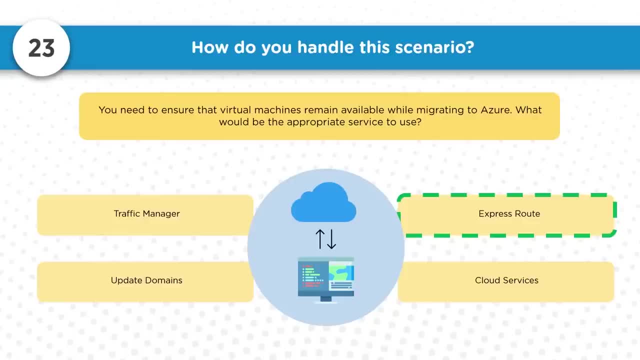 to the cloud using express route and the api calls get addressed or the the queries gets answered in the cloud through the express route service. look at this question. you are an administrator for a website called web game and you are required to validate and deploy changes made to your website. 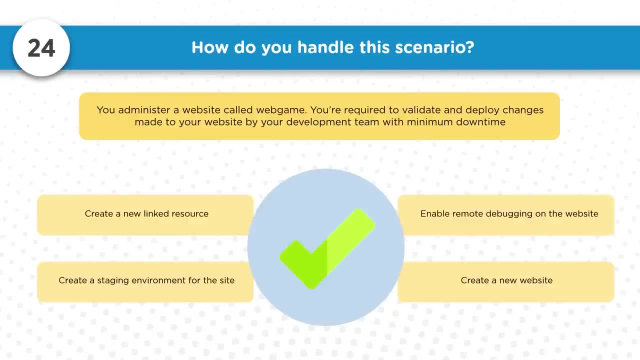 by your development team with minimum downtime. so the real question is: how do you validate the deployment changes that's made by the development team? let's look at the options: create a new linked resource, create a staging environment for the site, enable remote debugging on the website and then create a new website. well, why would you want to create a new website just to validate? 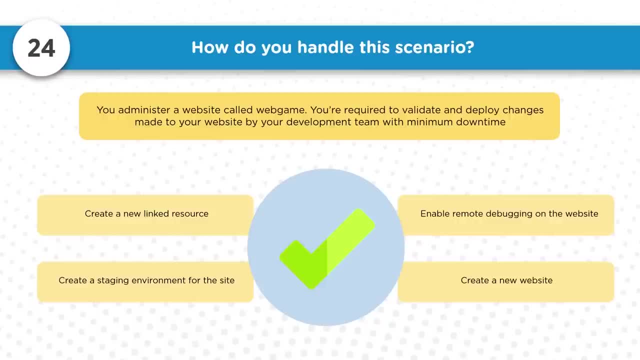 the changes and doing a remote debugging is not going to help, because debugging only captures logs of the changes happening. it does not do anything with validating the changes. create a staging environment could be, or is, the right answer, because when we have staging environment, anything that we run on production can be run on staging environment and any failures that would. 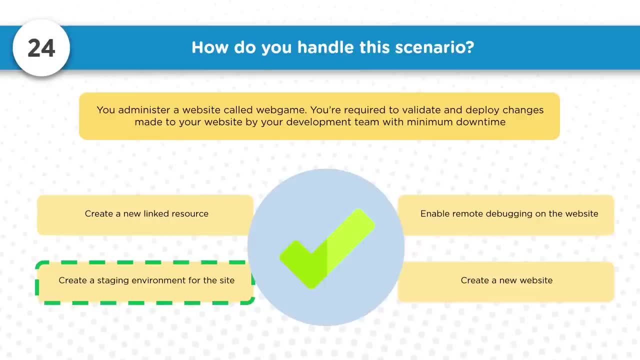 happen in production, if we simply run it in production, can be captured when we run the application in the staging environment. so that way, staging environment is a very helpful and useful service, and that way i can catch any errors, in other words, i can validate the changes that were. 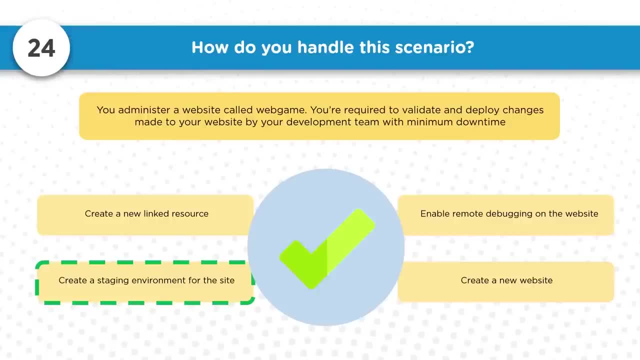 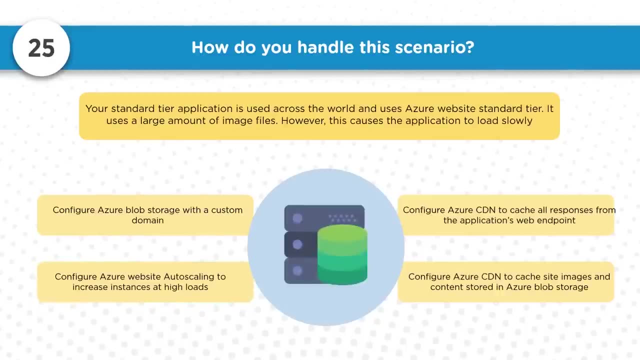 done by my development team before i move it to production, and that reduces the downtime in the production environment. Look at this one last question that we have for you. It's a standard tier application is used across the world and uses Azure website standard tier. It uses large amount of image. 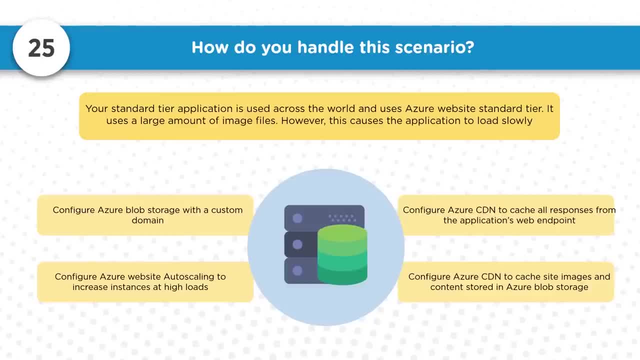 files so you can get it. This could be an e-commerce website which has a lot of pictures in it and this is causing the application to load slow. How can we handle this situation? Let's look at the options given. Configure blob storage with custom domain. Well, this application has pictures, but the 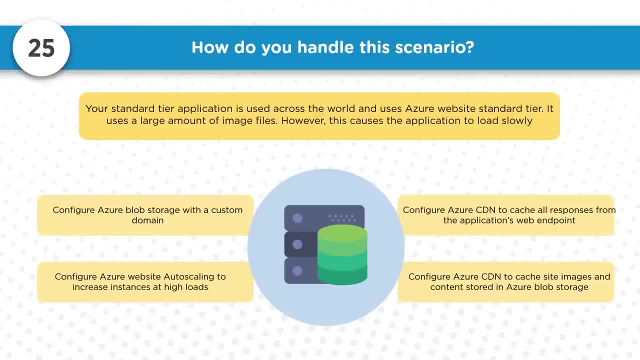 pictures only. the pictures is not all that. the application has right, So configuring blob storage might not help. This could be a very interactive website and that can't be run from blob storage. Let's look at the other options: Configure Azure website auto scaling to increase instances at. 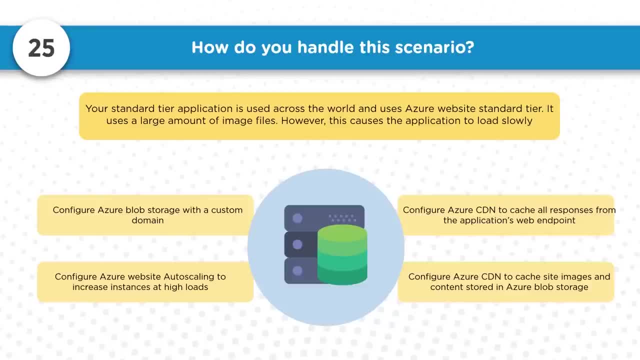 high loads. Now it's the picture that's causing issues for the website. It's not the CPU, or it's not the memory- unavailable memory, not enough- that's causing the application to be slow. So we need to identify what's. 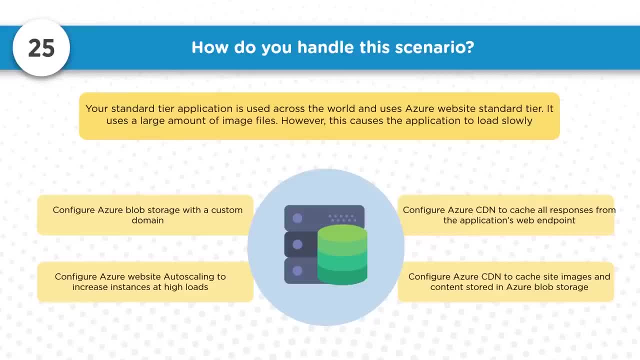 causing the application to be slow. So it's not the CPU, it's not the memory. So configure Azure for auto scaling is not going to help. And then what are the other options? Let's see Configure Azure CDN to cache all responses from the application's web endpoint. CDN could be the right answer, but 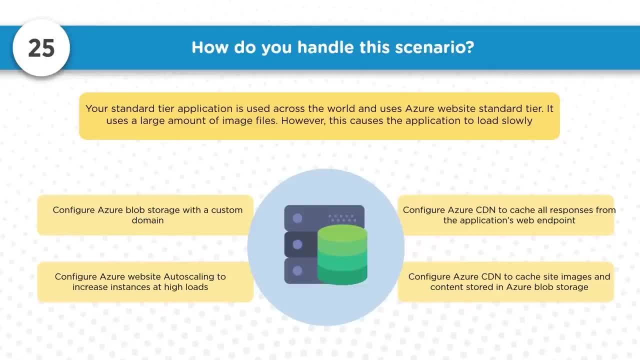 look at that. It says CDN to cache all responses from the application's web endpoint. CDN is not designed for that. Though it can do it, that's not the best way to use CDN to capture all responses from the application's web endpoint. The proper design for CDN would be to cache the frequently used 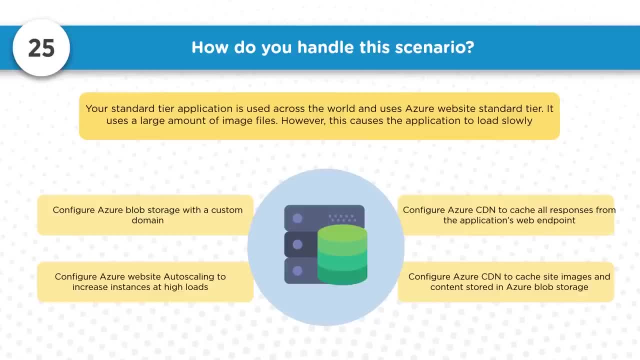 ones, In other words, cache the static content, which are photos, videos, logos and pictures and lot more Static content that never changes. Let's look at the last option: Configure Azure CDN to cache site images and content stored in Azure blob storage. Absolutely correct. So here we will. 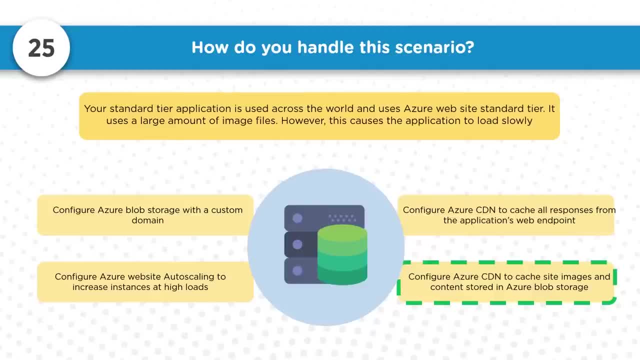 have to redesign the application to store the pictures- High quality, lazy loading or slow loading pictures because of the high quality and the bigger size. So store them in CDN and then the content let it be stored in Azure blob storage. That's the right way of designing the application and if we do it, this application is going to run.